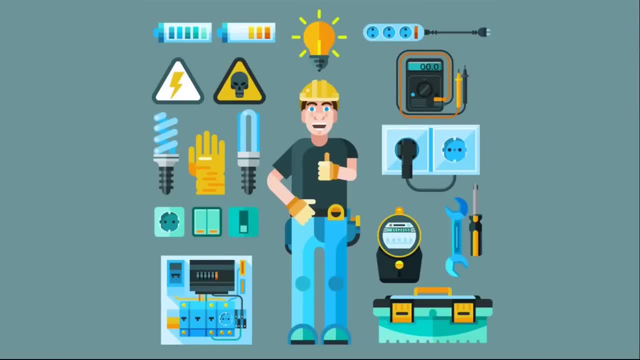 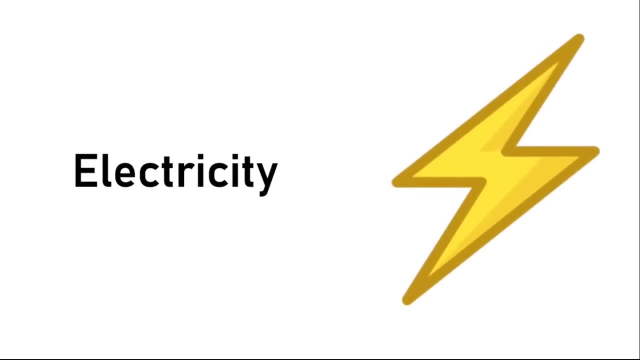 You can always revisit this section if you find any term confusing or you need to understand something again. So let us start with electricity. I'm pretty sure that you all must have heard of this term at least once in your lifetime. If not, let me tell you that electricity has played. 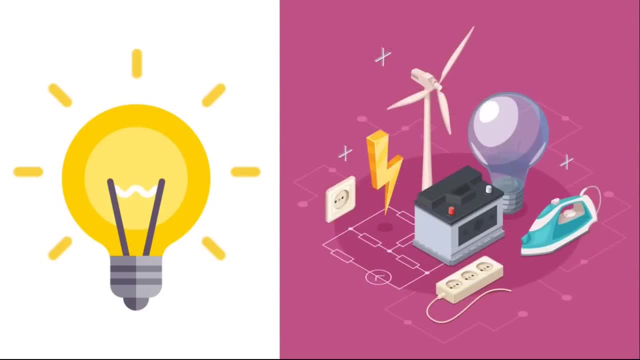 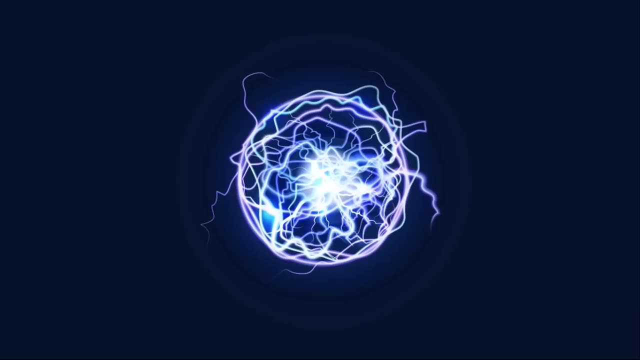 a major role in letting you watch this video on your computer or your laptop. Electricity is a type of energy that can be built up in one place or flow from one place to another. When electricity gathers in one place, it is known as static electricity, and electricity when moves from one place to another is called current electricity. 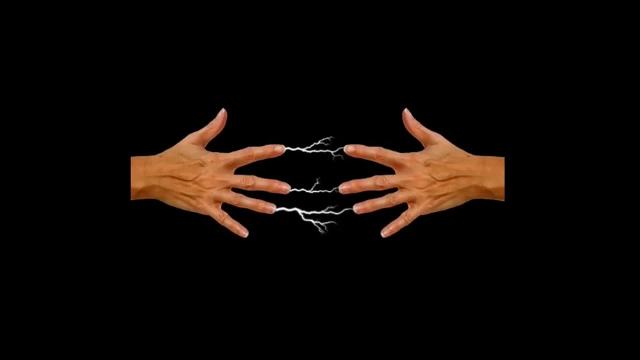 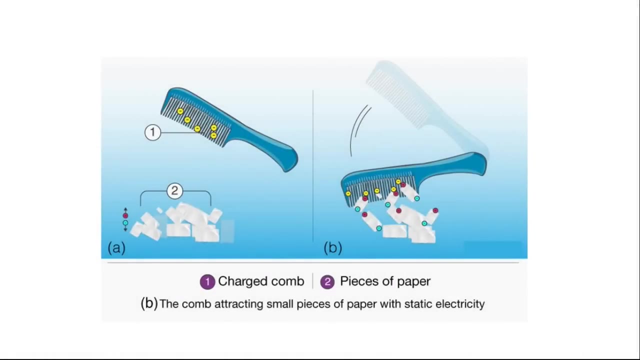 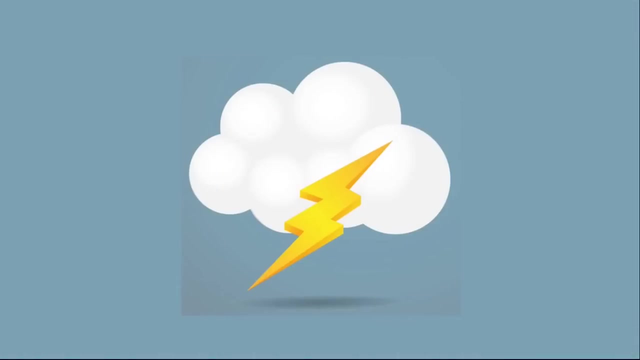 Have you felt a sudden painful jolt when you brush someone's arm, or crackling sounds when you take off your sweaters? or have you tried to attract paper bits by a comb? All this happens due to static charges that were accumulated in the space, Believe it or not. even the lightning that happens in the sky. 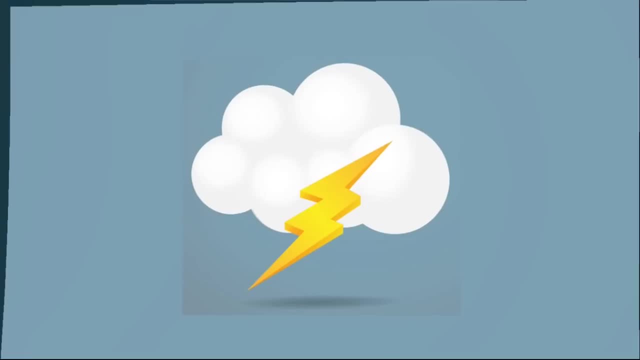 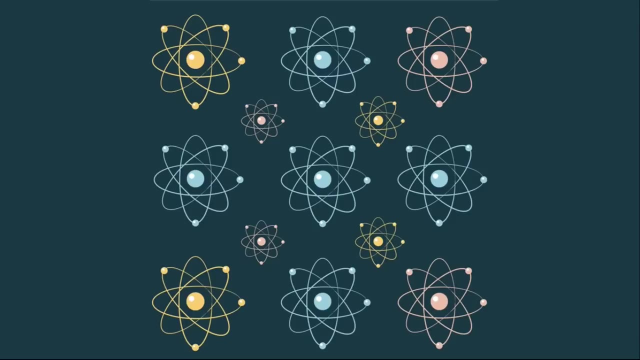 happens due to static electricity. So why does this happen? Everything in this universe is made up of atoms, which are made up of protons and electrons. Protons are positively charged and electrons are negatively charged. In an atom, generally, the number of protons and electrons 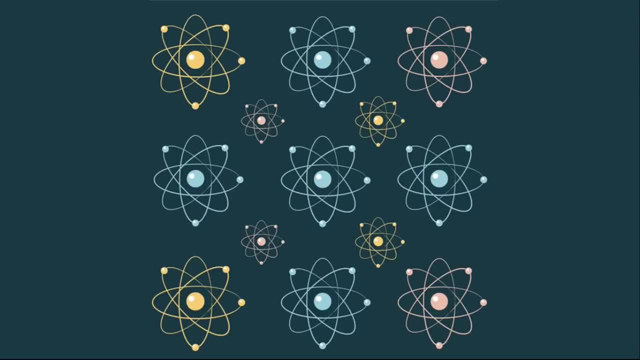 are equal. hence, the electric state of atom is neutral. but when some atoms lose their electrons, they become positively charged. when some atoms gain electrons, they become negatively charged. The short learning which I want you to take from this lesson is that similar charges repel. 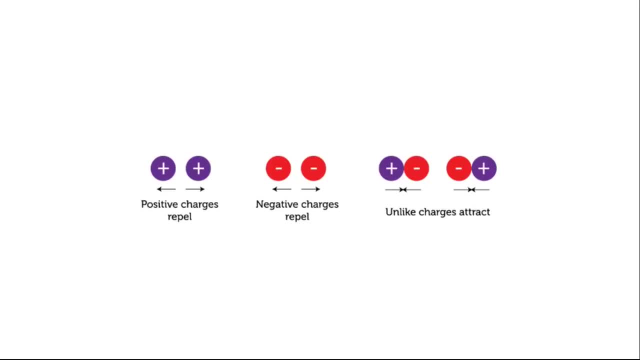 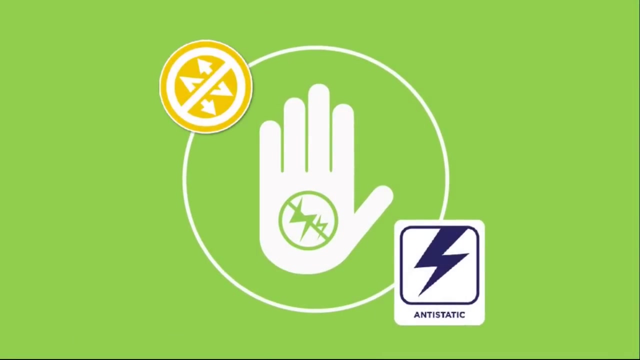 and opposite charges attract each other, as shown in this diagram. Static electricity is a very deep topic and has a separate study, called as electrostatics, which will go beyond the scope of this course. The other reason I told you about static electricity is that the static electric charges in our 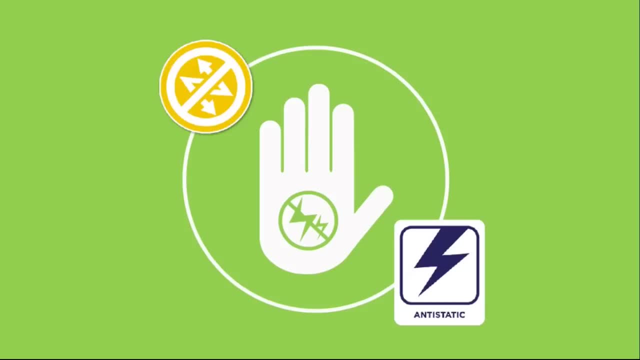 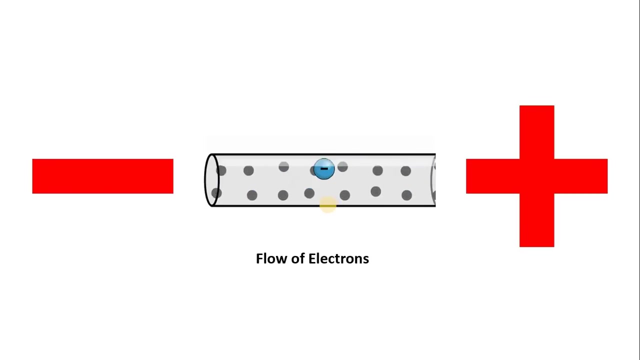 hands may damage your electronic components sometimes, so just make sure you keep your stuff on hard and solid surfaces and keep your components back in the anti-static packets which you got along with the components. Current electricity is the form of electricity which makes all of our electronic gadgets. 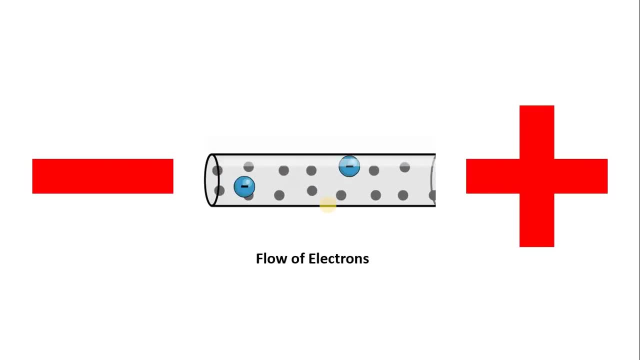 work. This form of electricity exists when charges are able to constantly flow, As opposed to static electricity, where charges gather and remain at rest. current electricity is dynamic: Charges are always on the move. We will be focusing on this form of electricity throughout the rest of our course. 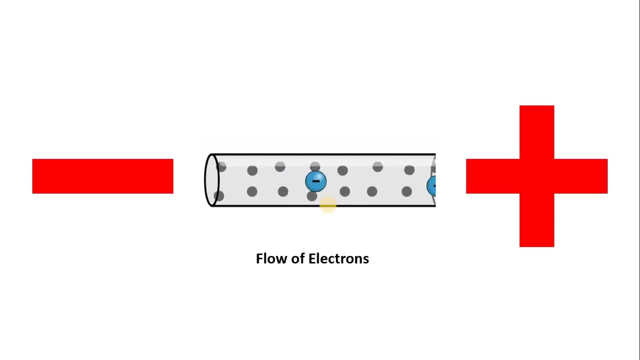 In the next video we will talk about voltage, which is one of the most important concepts for the existence of current electricity. So I will see you in the next video. In this video, we will learn about voltage. Voltage is a force that makes electrons move through a wire. 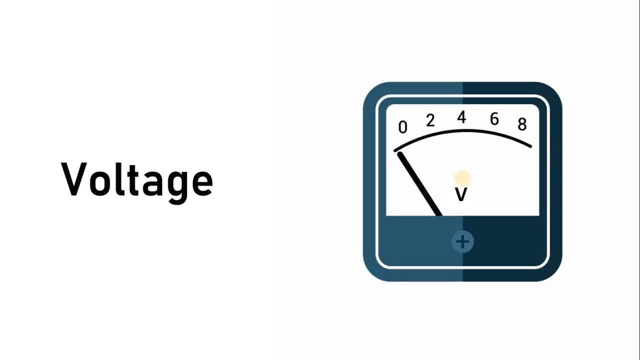 It is measured in volts and the symbol is V. Voltage is also called as electromotive force Or EMF. Voltage is also called as elektronoid force, which drives electrons inside a wire. Voltage was named after a scientist called Alessandro Volta. 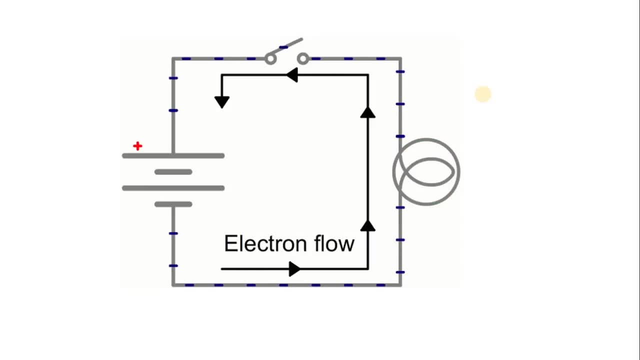 Technically speaking, voltage is a: the difference in electric potential between 2 points, For example the difference between the positive and negative terminal of a battery. Let's say this battery is of 5 volts, So the potential at this point can be. 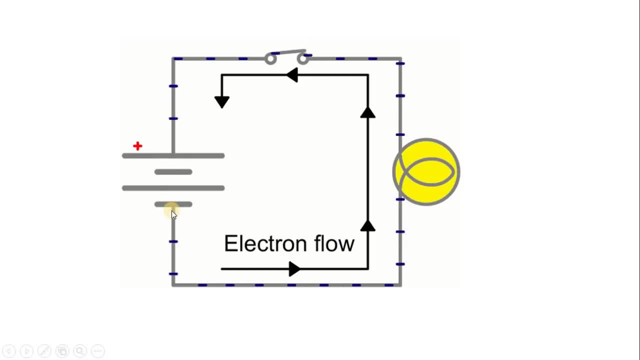 0 volts, 5 volts- okay, it can also be 10 volts here and 5 volts here, resulting into a difference of 5 volts. it can also be 0 here and minus 5 here. then also, the difference will be 5 volt. so this battery. 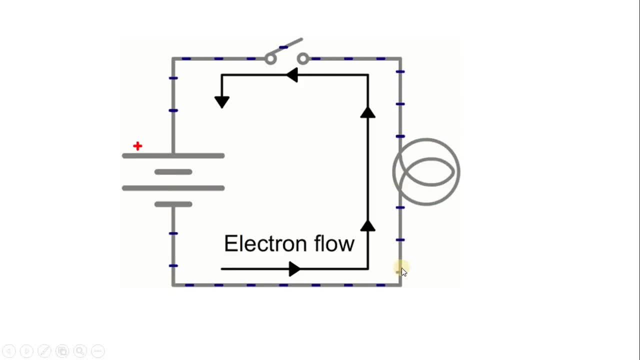 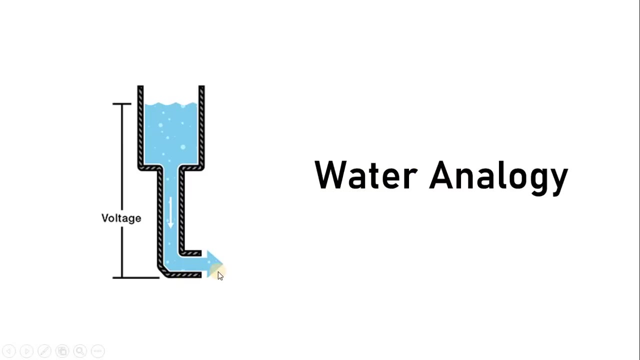 provides some force on electrons so that they can move inside a wire like this. you can see these electrons are moving inside a wire and and this bulb is glowing. now let us understand voltage by a water analogy. this is a water tank and the pressure at the end of the hose can represent 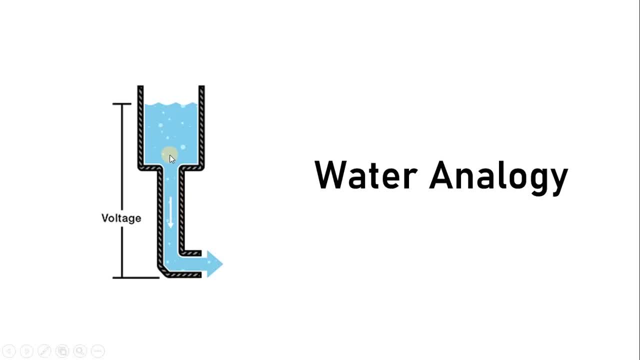 voltage the water in the tank represents charge. more the water in the tank, the higher is the charge and more is the pressure at the end of the hose. we can think of this tank as a battery, a place where we can store certain amount of energy and then release it if we drain our tank. 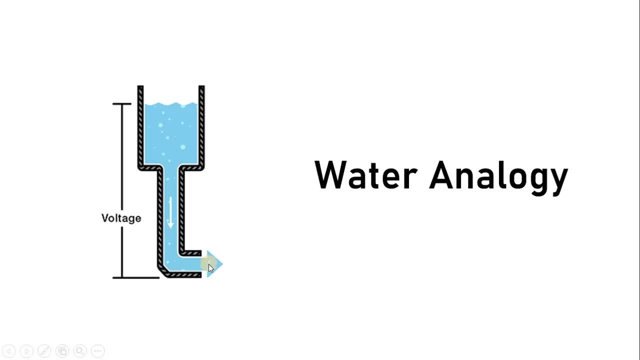 a certain amount, the pressure created at the end of the hose also goes down right. what i mean to say is we can think, Think of this as a decrease in voltage, like when the flashlights which use batteries glow dimmer as the batteries run down. 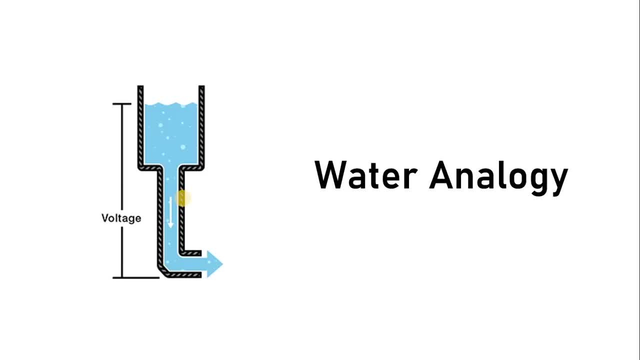 And then there is also a decrease in amount of water that will flow through this hose. Less pressure means less water is flowing, So we can consider this flowing water as current, which we will discuss in the next video. In this video, we will learn about current. 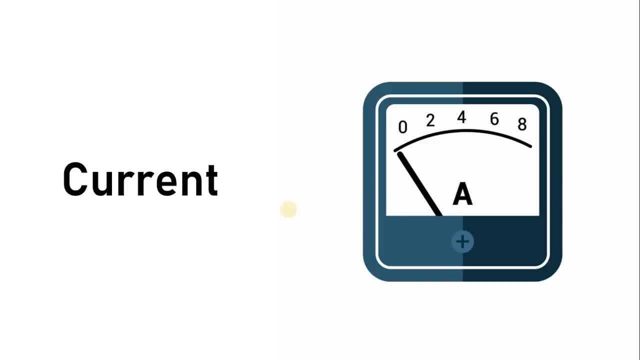 On a very basic note, the rate of flow of charge is known as current. When electrons move from a negative terminal to a positive terminal of a battery, they give rise to current. The unit of current is amperes, And the direction in which the current flows is the opposite to the direction of electrons. 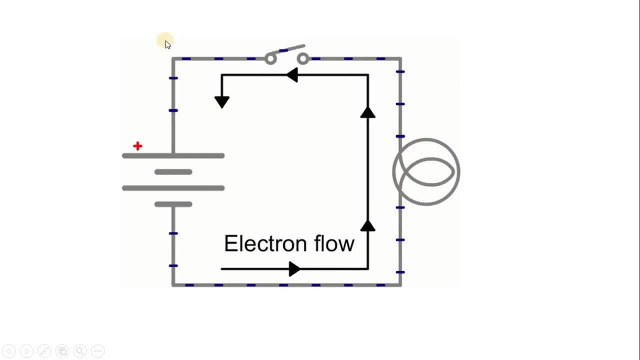 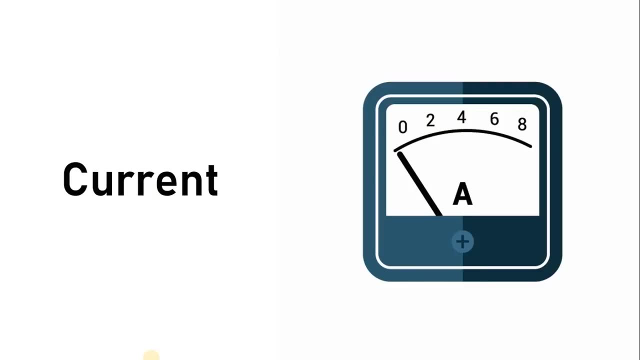 What that means is, if electrons are moving in this direction, then the current will move in this direction. So now on a more technical note. current is the amount of electric charge that flows when one coulomb of charge moves past somewhere in 1 second. 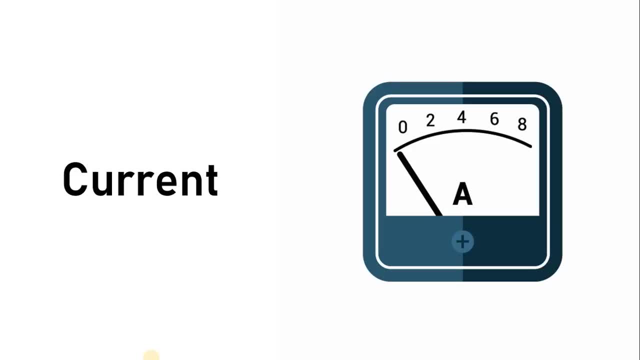 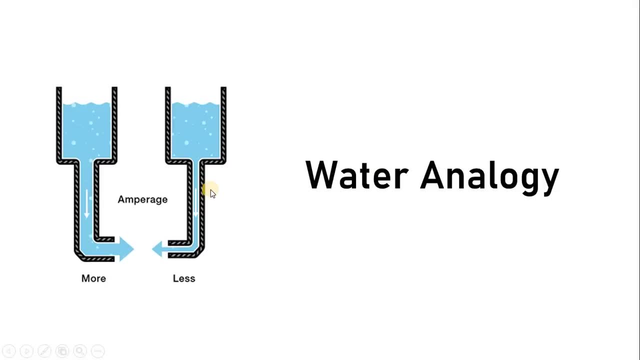 And that current is 1 ampere. Coulomb is the measuring unit of charge, Alright, And to measure the current at any point we can use an ammeter. We can also understand the flow of current by water analogy. Let's say this is a tank filled with water. 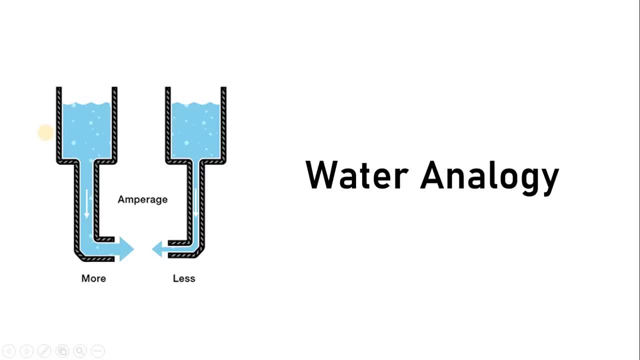 And this water is flowing due to potential energy of water, which we learned is called as voltage in the previous video. So here the size of hose is acting as resistance: A bigger size hose offers less resistance and the smaller size hose offers more resistance. 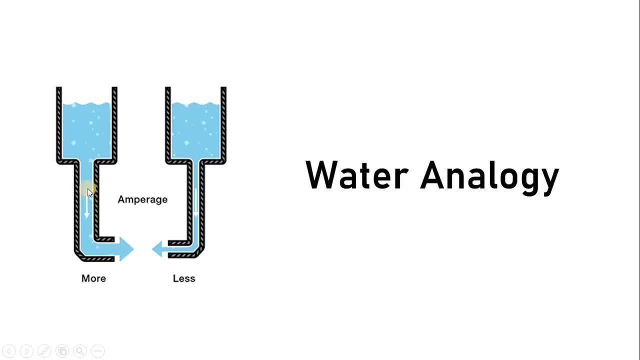 So the path which has low resistance is called the ammeter. The path which offers low resistance, more current can flow through that path, And the path which offers more resistance, less current can flow through that path. Okay, So here, since the voltage is equal and resistance is lower, in this case the water flowing here. 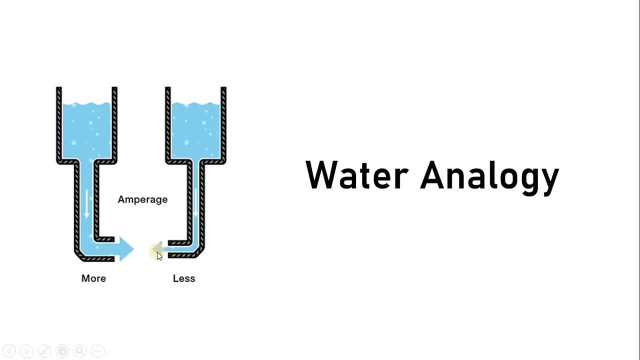 will be more and the water flowing here will be less. Okay, So this has given rise to another term called as resistance, And we will learn about resistance in next video, But before that, I would like to tell you that there are two types of current. 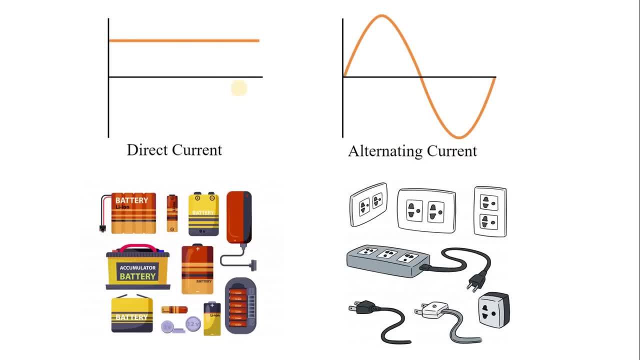 One is direct current and one is alternating current. In DC current, the flow of electrons stay in the same direction and the voltage stays steady with the time, as you can see from the graph, While in AC, the flow of electrons change and the voltage does not stay steady with. 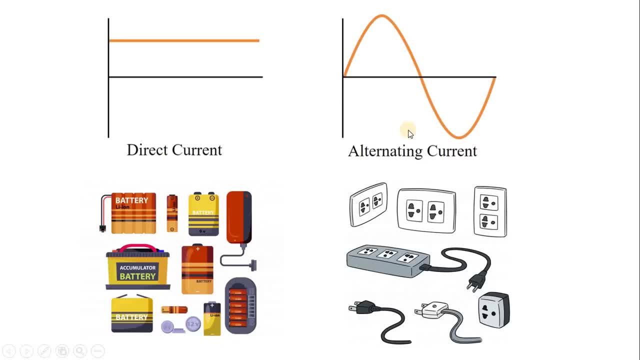 time. That also you can see from the graph. Don't worry if you could not understand all this at this moment. At this point, you only need to understand that the current which you see in your home, that is The current which drives your fans and other appliances like air conditioners, televisions. 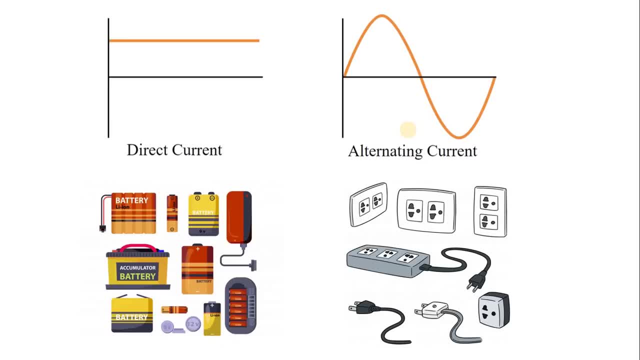 etc. is known as AC current, And the current which you get from the batteries or specific power supplies is DC or direct current. The current you get from your laptop or computer's USB port is also DC current And for our course, we will be dealing with the DC current only. 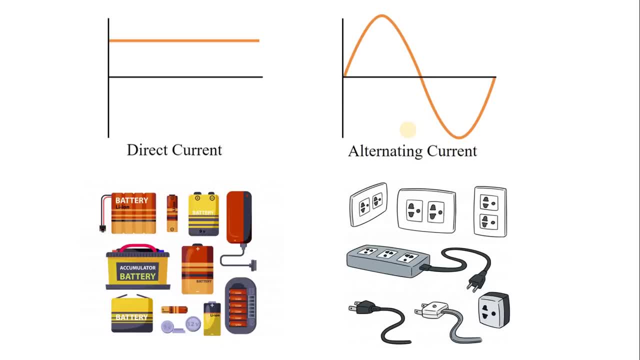 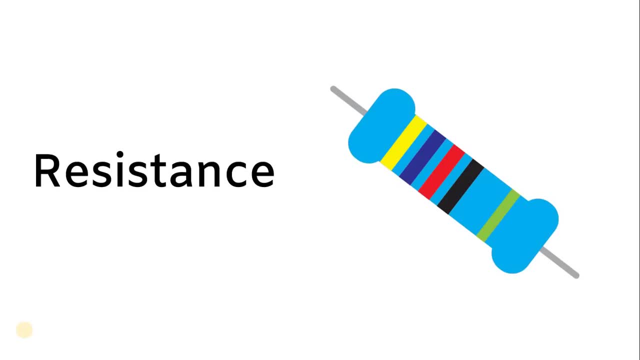 If you have understood just this part, you are good to go, So I will see you in the next video. Now Let's take a look at resistance. The electrical resistance of any component is a measure of the difficulty of passing an electric current through that substance. 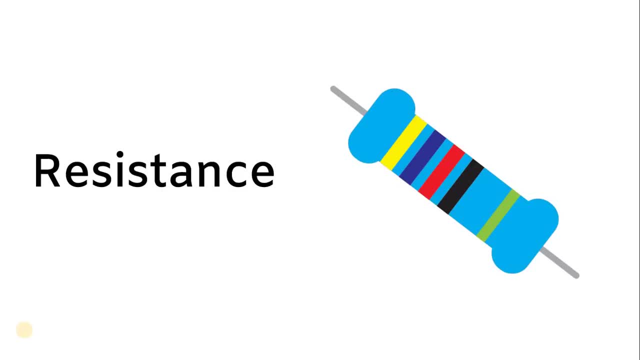 With more resistance in a circuit, less electricity will flow through the circuit. Based on this term, resistance, there is an electrical component known as a resistor. A resistor is a device which limits the flow of a current in a circuit. We may need a resistor in a circuit where we need to drive LEDs which require limited 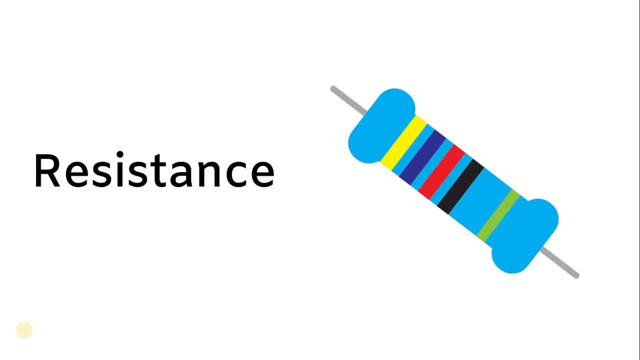 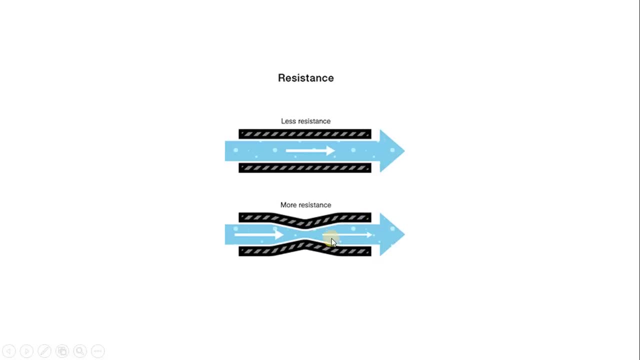 amount of current so that we can prevent it from burning off. Right Now, if we see the resistance, with the water analogy, we can see this is a pipe and this is one another pipe. The water can flow easily through this pipe because it offers less resistance. 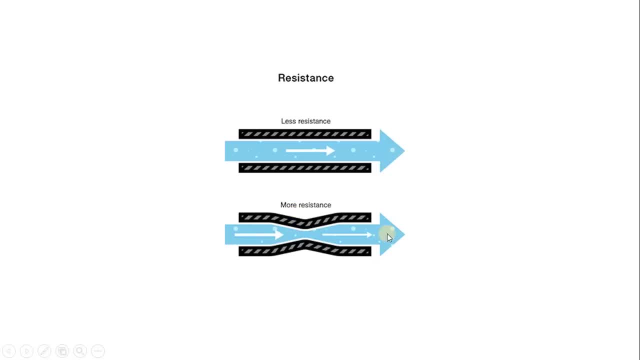 The flowing water can be synonymous to flowing current. Okay, And when there is more resistance, less current will pass through it. One important thing which you would like to know is that the current always takes the least resistive path. For example, if you offer two paths for current to flow, it will try to flow from the least. 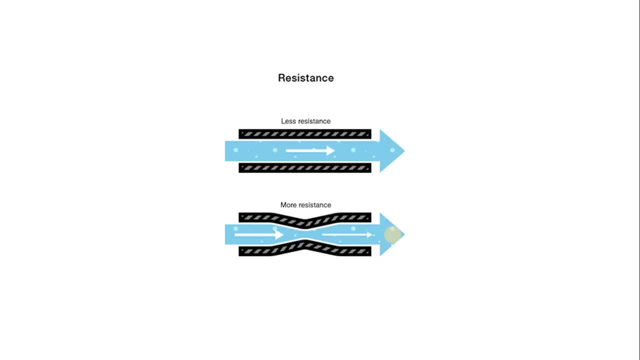 resistive path out of this. Okay, So in the next video we will study the relation between current voltage and resistance, And in upcoming videos we will also learn how to identify the value of the resistor. The value of the resistor is measured in ohms. 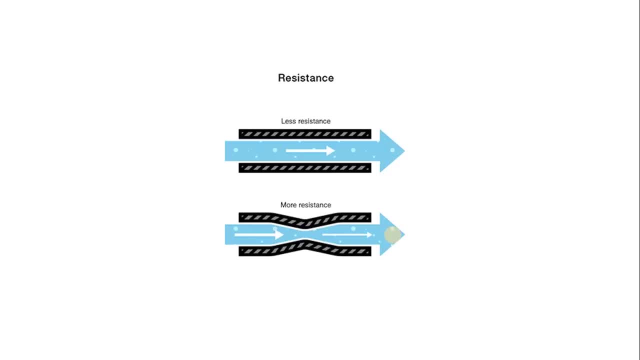 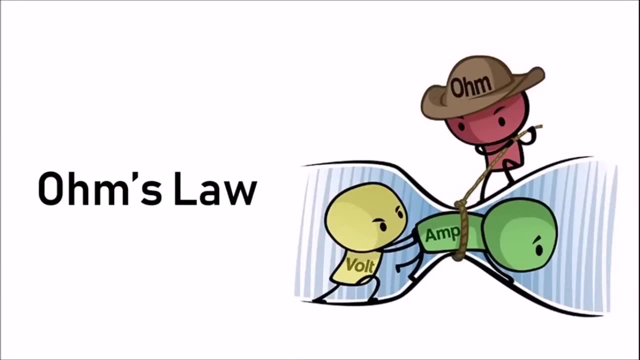 More the value of the resistor, more the resistance it will offer in the circuit. So now I will see you in the next video. So till now, I am sure that you all must have inferred that somehow all these terms are interconnected. If you have, then you are absolutely correct. 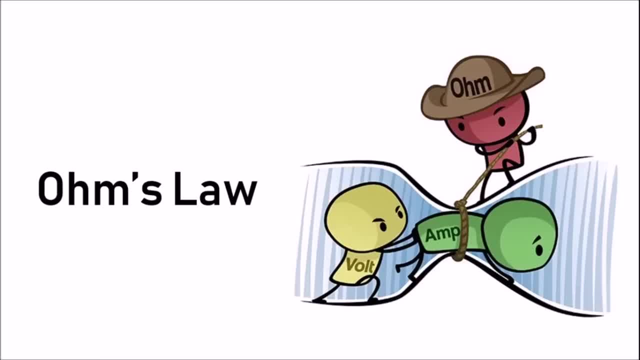 There is a law known as the Newton's law. There is a law known as Ohm's law which tells the correlation of these terms. A German physicist, George Simon Ohm, stated that the electric current flowing through a metallic wire is directly proportional to the potential difference across it, provided 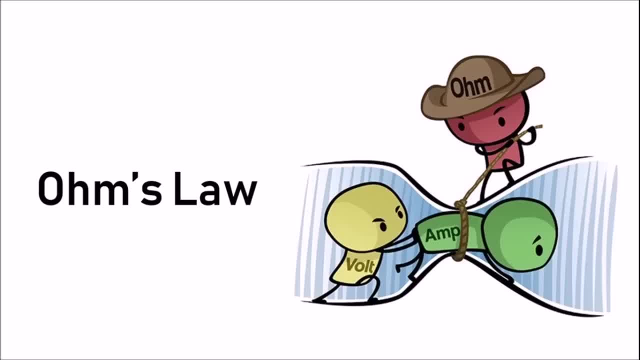 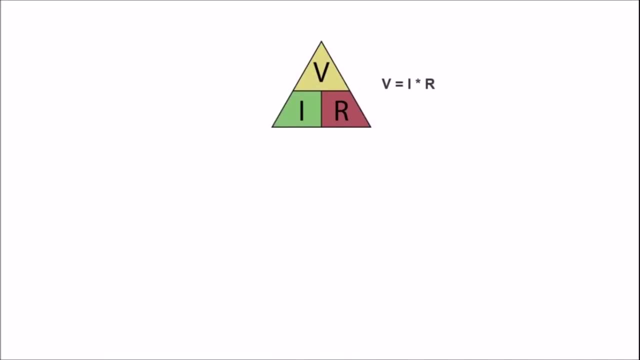 temperature remains the same. That means, like I said earlier, more the force, more the current. The potential difference is the force here which we talked about earlier. So mathematically, we get voltage, We get voltage. V is equal to the product of resistance R and current A, or I for that matter. 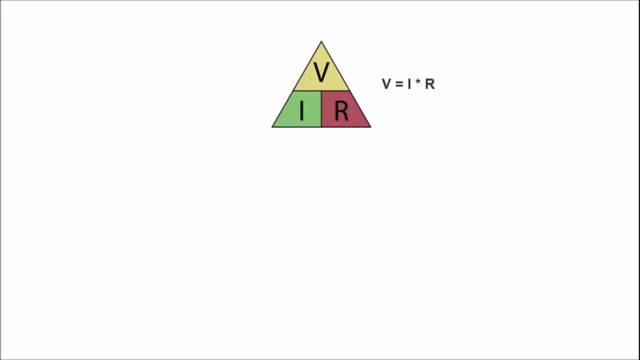 If any one of them is unknown, we can find out by doing the math. There is an easy way to find that out. There is a triangle known as Ohm's law triangle. We just hide the unknown quantity and we get the answer. 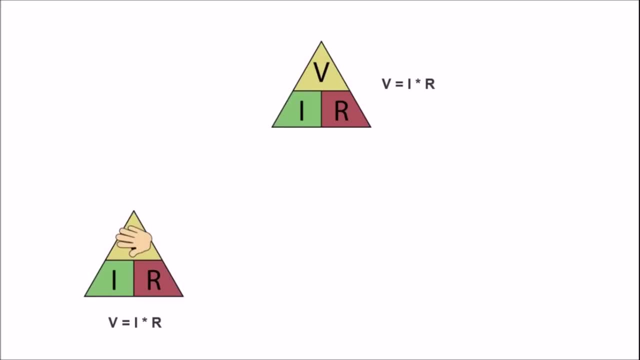 For example, If we hide V, We get the answer. So I and R looks in a multiplication position. So V is equal to I multiplied by R. If we have to find resistance we will cover up R, Then V and I appear in a division like position. 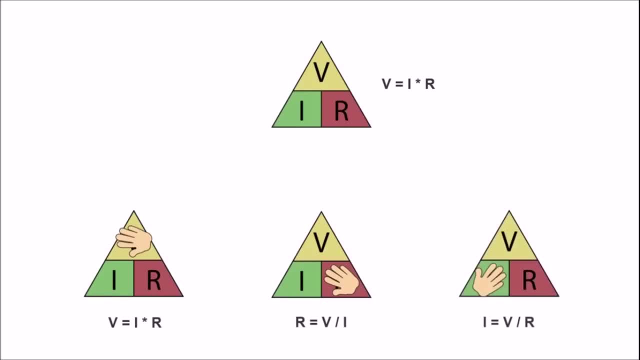 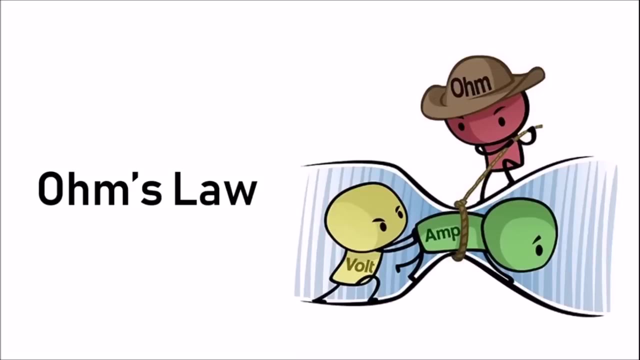 So R is equal to V divided by I. Then we have I as unknown quantity. Then we can do: I is equal to V by R based on the similar reason. This interesting image shows That if we consider voltage, current and resistance, as people 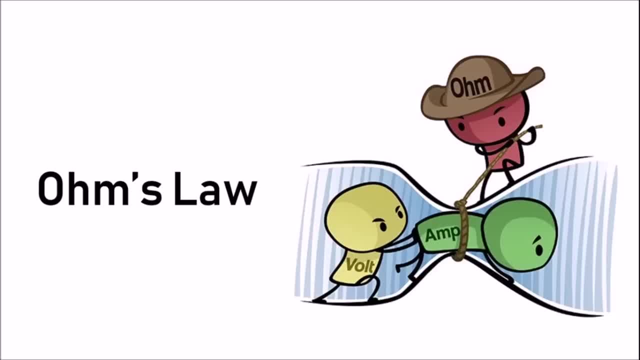 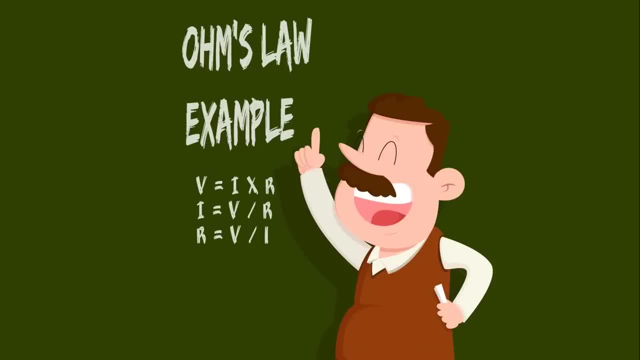 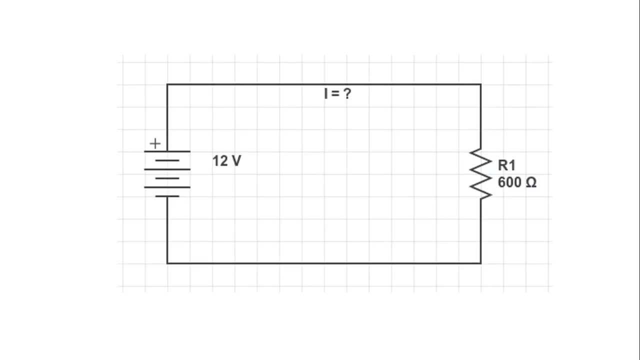 How would they behave? The voltage would keep pushing the current and resistance would create a difficulty for it to pass. Isn't it funny? So now let's see. how do we use Ohm's law to calculate the unknown values in a circuit. This is a circuit, and this is a very basic circuit, right? 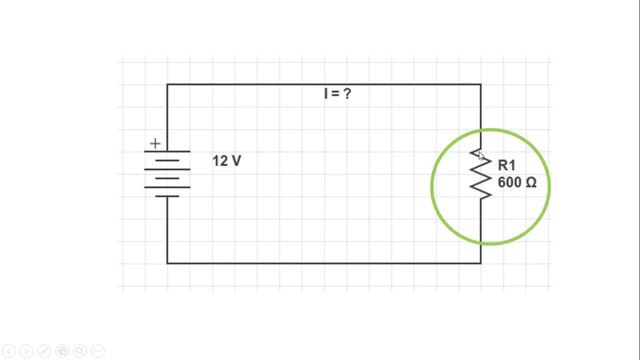 And here is the resistance of value 600 ohms. And this is the circuit representation of a resistance Which is a 0.5 ohm. And this is the resistance of value 600 ohms. That's the exact line, right. 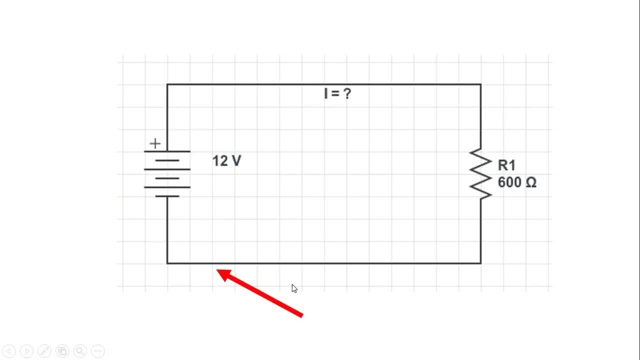 Here we have a battery which measures 12 volts, And this is the connecting wire. So can you figure out how much current is flowing in the circuit right now? We will use Ohm's law to find out, okay, So here, what quantity is unknown. 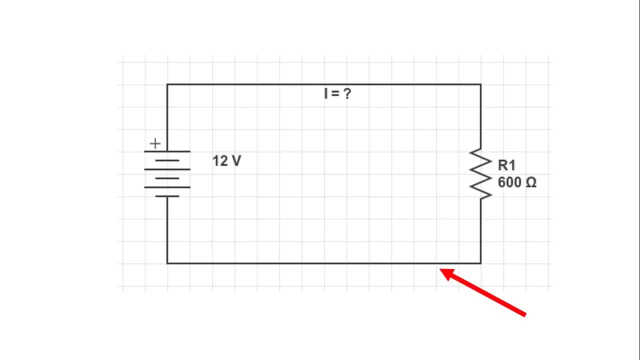 I, which is current right, So we will be using I- is equal to V by R, So we will do 12 upon 600, which would be 0.02 amperes. Okay, Now, if we change the value of our resistance and make it 6 ohms instead of 600. 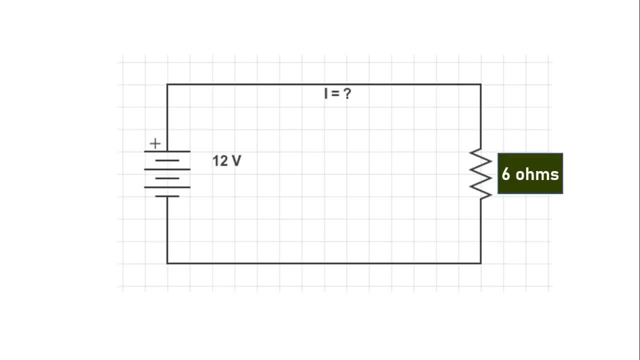 So can you tell me the new value? We just need to do 12 by 6 now, which would turn out to be 2 amperes. Alright, So did you observe that if we reduce the resistance in a circuit, the current flowing in the circuit increased? 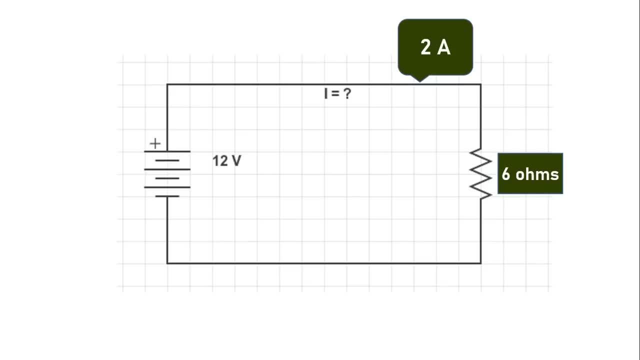 Earlier it was 0.02 amperes and now it is 2 amperes- Right Now, if we change the voltage of the battery as well, let's say 24.. So now the current flowing will be 4 amperes. 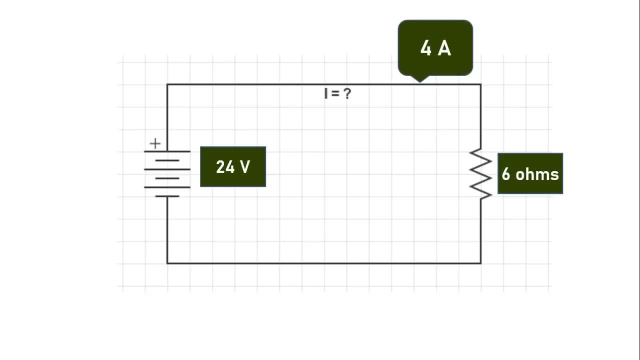 Right. So we increase the voltage and reduce the resistance. So the overall current flowing in the circuit was 4 amperes. So I guess you must be able to see the relation between voltage, resistance and the current flowing in the circuit. 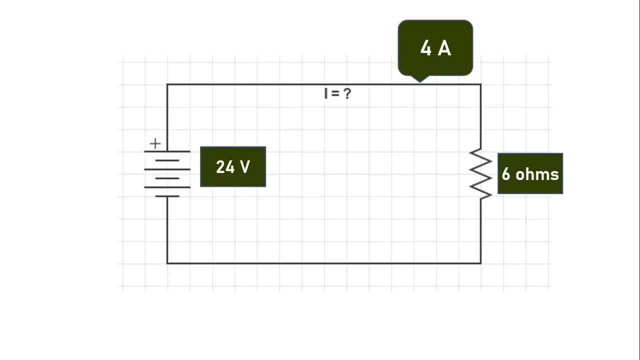 One thing you need to learn about using resistances in a circuit is that there are multiple ways we can use resistances. Like we can use them in series, we can use them in parallel. So now I will show you how to use resistances in series and parallel. 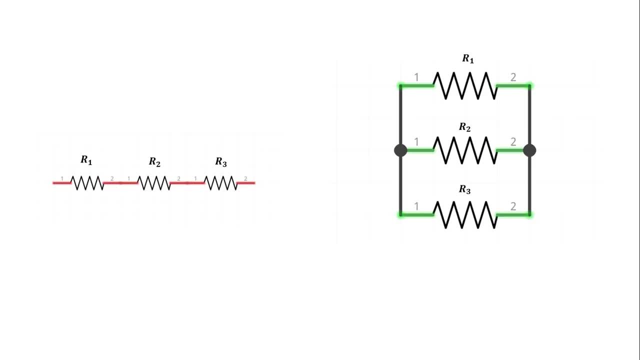 If I give you a general idea about resistances in series and parallel, I would say In a series circuit the output current of the first resistor flows into the second resistor and into the third resistor. Therefore the current is the same in each resistor. 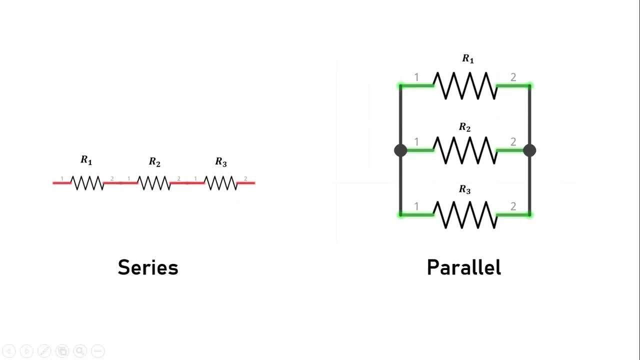 While in parallel all the resistors are connected to each other in a manner shown here right, all the ends are connected to each other like this. so now we will look at series circuit in a bit more detail. so if we look at the circuit here, we can: 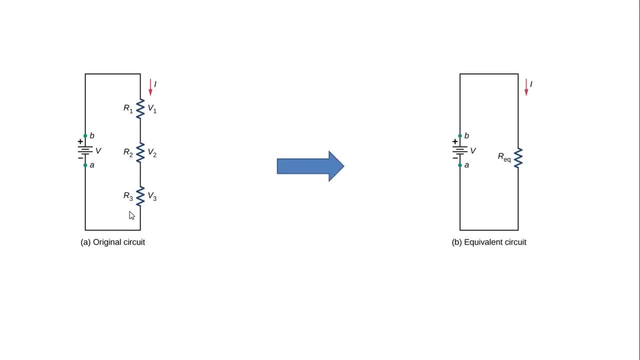 see that three resistances, R1, R2 and R3, are connected in series across the battery of a certain voltage. okay, we don't know what voltage is that right now, but let's say that voltage is V, right. so now, since there is just one path for current to flow in the circuit, the value of current flowing in the 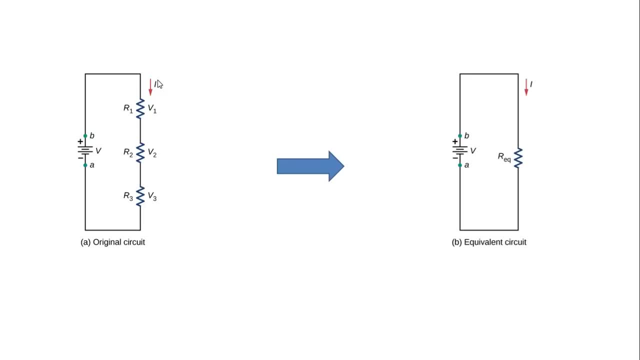 circuit would be same. let's say it would be equal to I. okay, so due to that in a series circuit the voltage drop across each resistor would be different and, interestingly, the sum of V 1, V 2 and V 3, that is the voltage across each resistor. 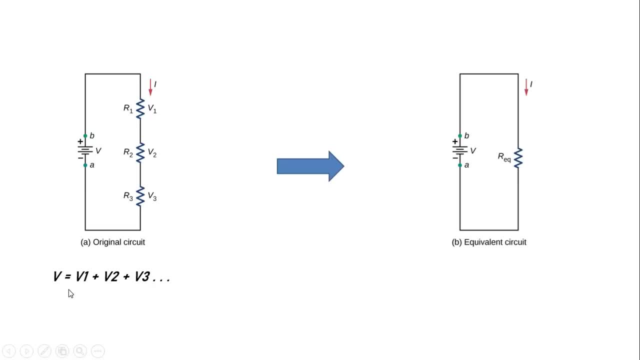 will be equal to the voltage of the battery, right? let's say, if the voltage of the battery is 12 volts, okay, so the voltages which we will get across these resistances would add up to 12 and from this circuit we can create an equation of the voltage across each resistor and we can also write the. 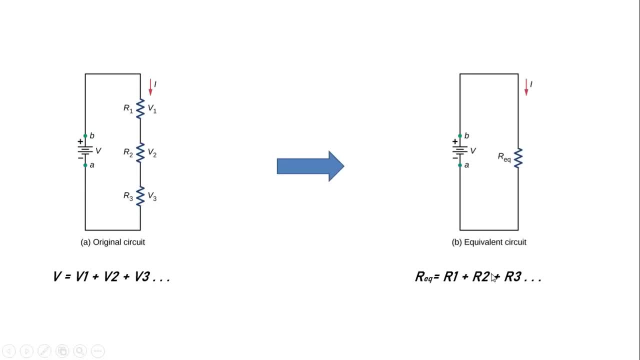 circuit like this, where, where the equivalent resistance is the algebraic sum of all the resistances which we have used. so let us now see an example where you can apply this learning right. so here we have a circuit with five resistances connected in series and which are connected across a battery. 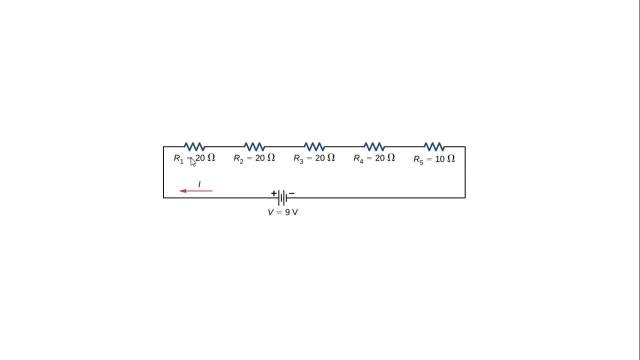 which measures 9 volts. so what we need to do is we need to find the equivalent resistance, the current flowing in this circuit and individual voltages across each resistance. right, let's have our diagram handy with ourselves, which we use to remember the Ohm's law. so let us first calculate the equivalent. 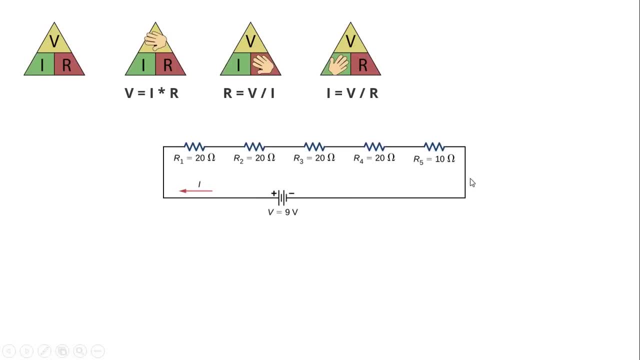 resistance. as I told you, to calculate the equivalent resistance in a series circuit, we just take the algebraic sum of all the resistances right. so here it will be 20 plus 20, plus 20 plus 20 and plus 10, which is equal to 90 ohms. 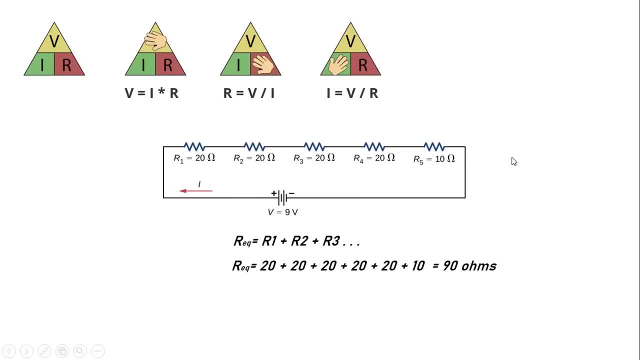 right now, since we have this equivalent resistance to calculate the current flowing in the circuit, we would use this formula: I is equal to V by R right. the only difference is, instead of using R, we will use R equivalent, because we will be using the equivalent resistance in the circuit right, that will be 9 upon 90. 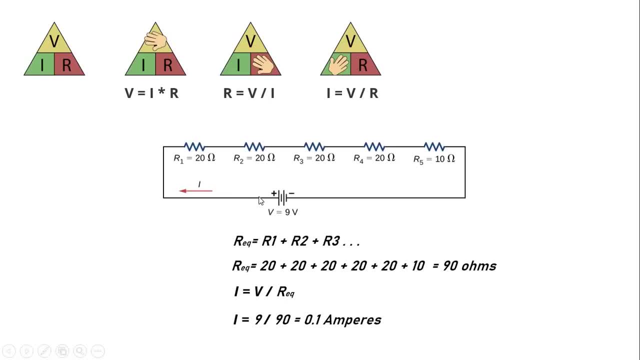 which is 0.1 amperes. so now we know that 0.1 amperes is flowing in this circuit, so to calculate individual voltages across the circuit, we need to know that 0.1 amperes is flowing in this circuit so to calculate individual voltages across. 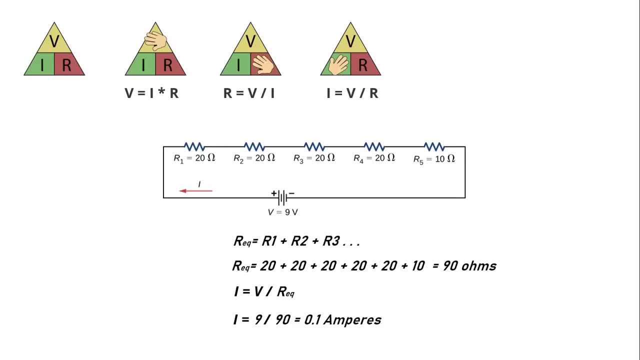 the resistances, what we can do. we will use the Ohm's law once again, but this time we will use this formula. we need to calculate: V is equal to I into R, so I is 0.1 and R is 20, so 0.1 into 20 is 2 volts. okay. similarly, this will also measure 2. 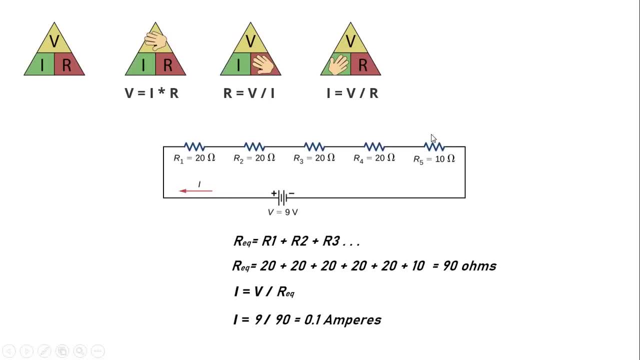 volts. this will also measure 2 volts. this will also measure 2 volts and this one will be 1 volt, because 0.1 into 10 is 1, right? so now you notice that 2 plus 2 plus 2, so that is equal to 2 volts, and that is equal to 10, and that is equal to. 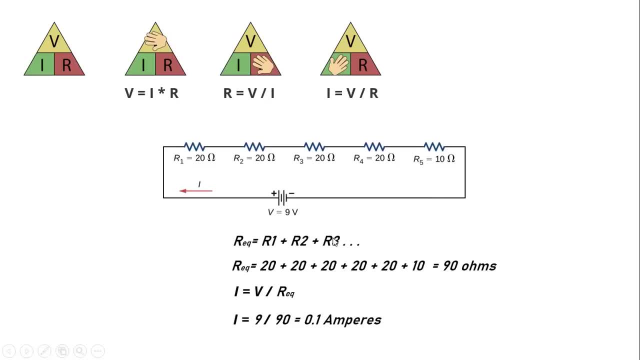 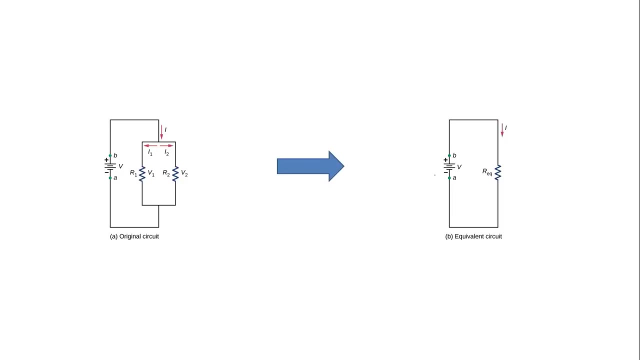 2 plus 2 and plus 1 is equal to 9, right, as we saw earlier as well. all the voltages also add up to the voltage of the battery, which is 9 volt. all right, so this is about cd circuit. now we will look at the parallel circuits. so the resistors are in parallel when one end of all the resistors 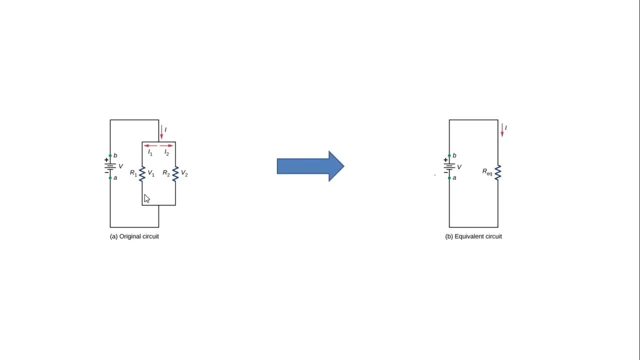 are connected by a continuous wire of negligible resistance, and similarly other ends are also connected to each other through a similar wire. since all the resistances in parallel are connected directly to the battery, you can say the voltage across all of them is equal, right. but unlike the 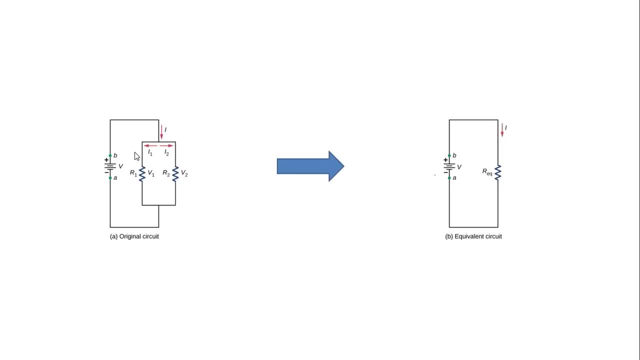 resistors in series where there is just one path for current to flow. in parallel circuits there are multiple paths for resistance to flow, like in the circuit you can see current has two paths. if the current flowing in the circuit is i, then it will divide into two parts. let's say i1 and i2. 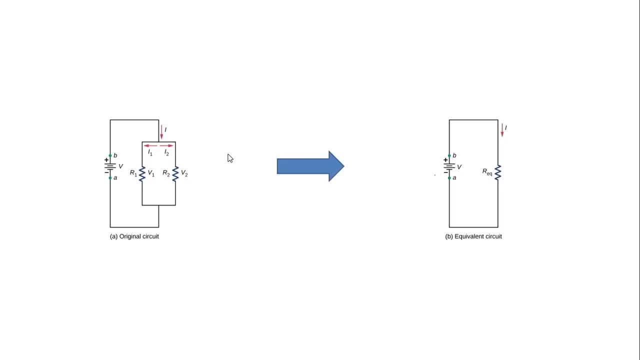 if there were more resistances we would say like i3 and i4 etc. and when that current flows it comes back and it adds up and becomes i again. and if we wish to calculate the values of i1 and i2 again we can use the ohm's. 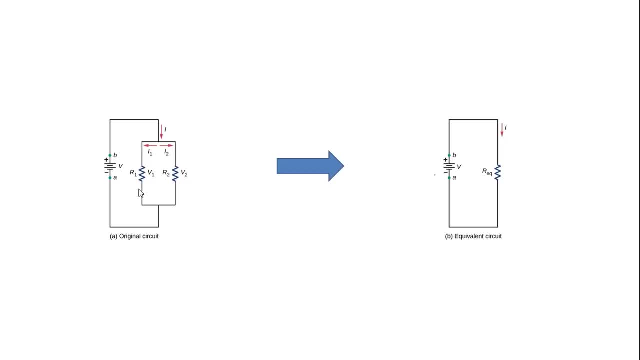 law here, right, because the voltage across this resistor is equal to the battery's voltage and the value of resistor is also known. so we can calculate i using ohm's law, right? you should remember that v1 and v2 will always be equal to v and i will be equal to i1 plus i2. right now we can. 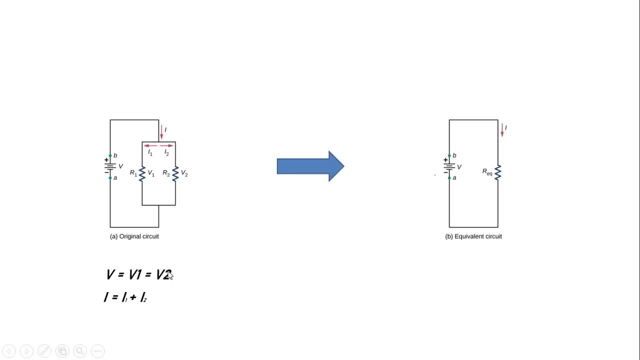 also calculate the equivalent resistance this combination of resistors will offer in the circuit. and to do that there is a very simple formula: one upon r, that is, equivalent resistance is equal to one by r1 plus one by r2 plus one by r3, and so on. right, so let us see one example, and let us 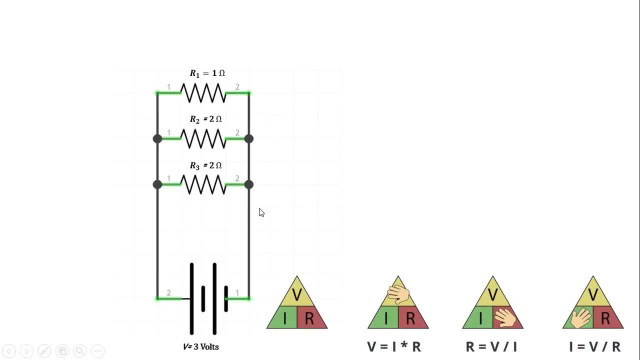 keep that diagram handy again, right? so what we need to do in this question is we need to find out the current flowing in this circuit and the individual current flowing in these resistances. So one approach can be: we can find out the equivalent resistance first using the formula. 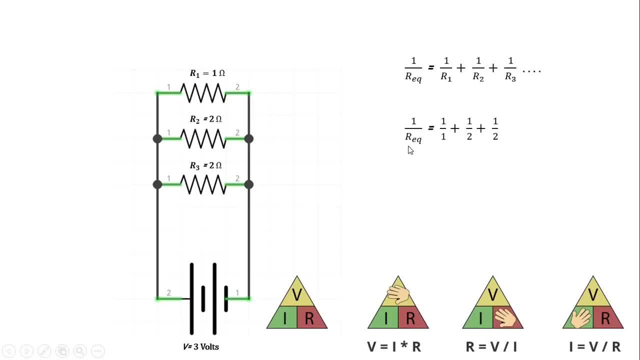 we just saw. Let us place the values inside it: 1 by Req is equal to 1 by 1 plus 1 by 2 plus 1 by 2.. We have just replaced these values by the values of the resistors. 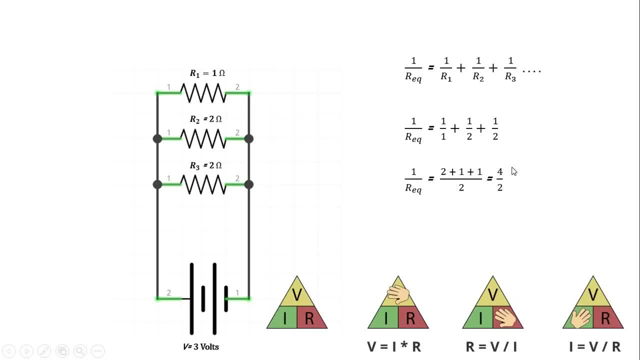 So now we will take LCM and, which turns out to be 4 by 2.. But please note that this is 1 by R equivalent. So to calculate R equivalent, we will take the reciprocal of this value, which will turn out to be 0.5 ohms. 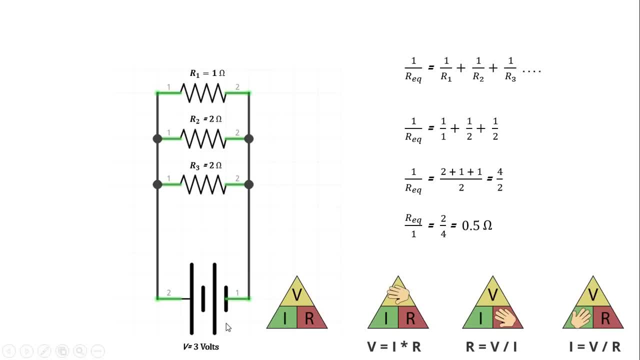 So now we have the equivalent resistance of this circuit, We can simply use the formula: I is equal to V by R, V is 3. and R is 0.5. so the answer would be 6 amperes. right, so 6 amperes will be. 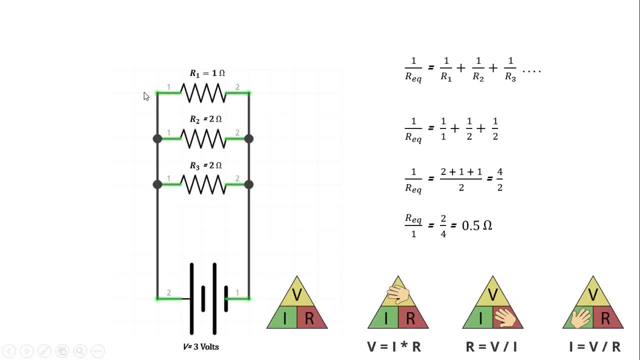 flowing in this circuit. now, if we want to calculate the individual currents in these resistances, what we will do is we will use this formula again, because V is same and R is known right. so in this resistor V is 3 and R is 1. so in this, 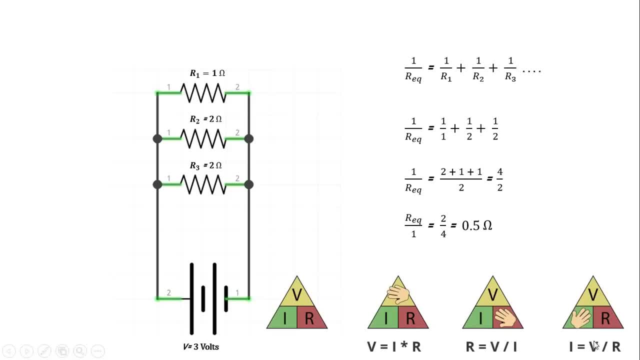 resistor 3 amperes will be flowing. in this resistor, 3 by 2 that means 1.5 would be flowing right, and in this resistance as well, 1.5 amperes would be flowing. so now, if we add up all these currents in these three resistances, that 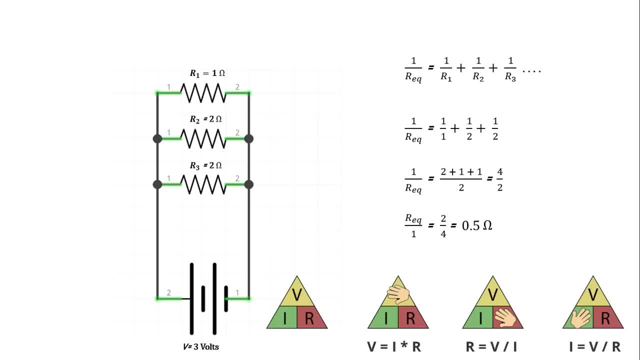 would come out to be 6. so again, we verified the things we just studied and I don't know if you noticed or not- the equivalent resistance of 0.5 was even lesser than the lowest of the resistances used right. so this will always be the case. the equivalent resistances in the parallel: 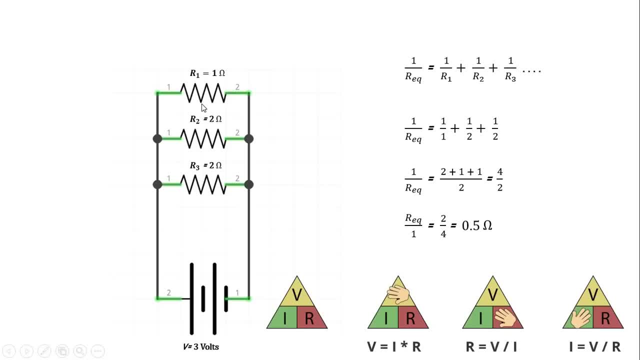 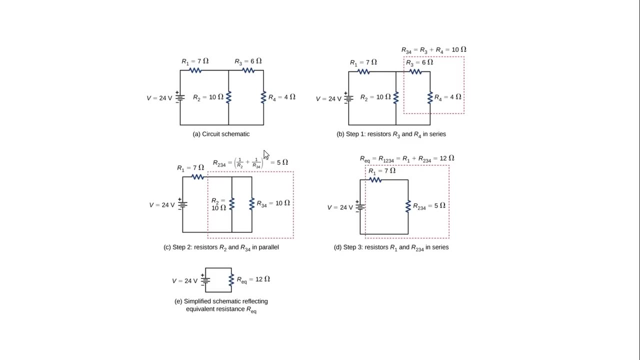 circuits will always come out to be lesser than the lowest value of the resistance in those combinations. alright, so this was about parallel circuits, and now we will see a slightly more complicated circuit which involves series and parallel circuits- both. so here we have such a circuit where resistances 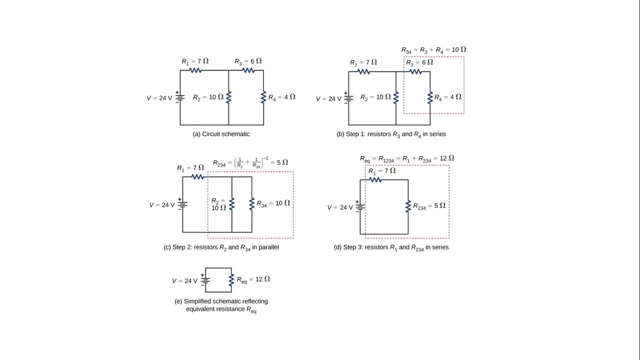 are present in series as well and parallel as well. so now I will tell you how to find out unknown values in such kind of circuits, right? so first of all, we need to work in sections of the circuit. for example, in this circuit- I have taken up this section- we can see that these two resistances, R3 and R4, are in series. 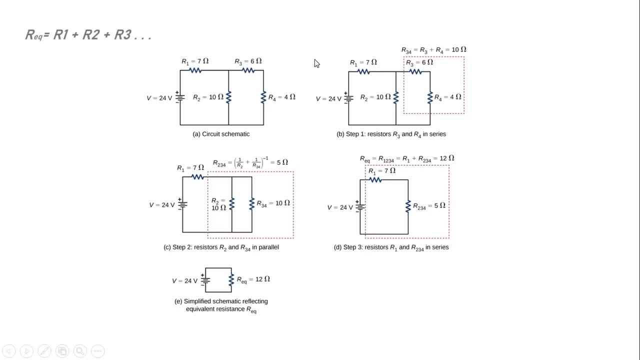 right, so using a regular resistances in series formula which is R equivalent is equal to R1 plus R2 plus R3 and so on, right? so here are two resistances. so we have just taken some of those two resistances, which is 10 ohm then. 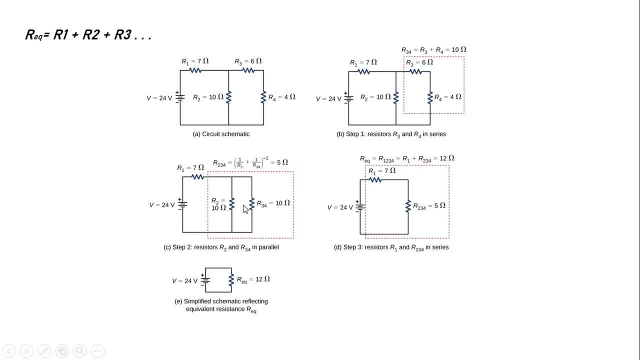 we will reduce the circuit in our mind. we will think of it as one single resistor right which is in parallel with this resistance right. so now we will use our parallel formula, which is 1 by R equivalent is equal to 1 by R1 plus 1 by. 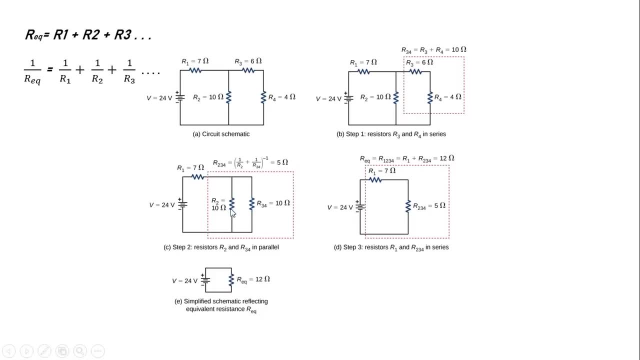 R2, right? so both of the resistances are of 10 ohms. so if you plug the values in this formula you will get 5 ohms. you can try it on your own right. then we will reduce that circuit in our mind only with 5 ohms, right? so this is the resistance. 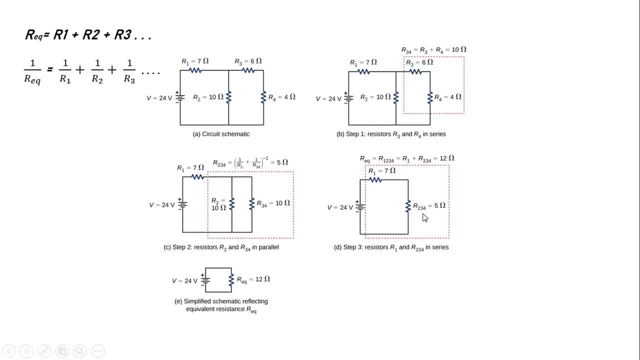 which is in parallel with this resistance. right, so now we will use our parallel formula, which is 10 ohms, as a resistance. then this equivalent resistance is in series with 7 ohm resistor. right again, we will use our resistance in series formula, so the equivalent resistance will turn out to be 12 ohms. so now let's. 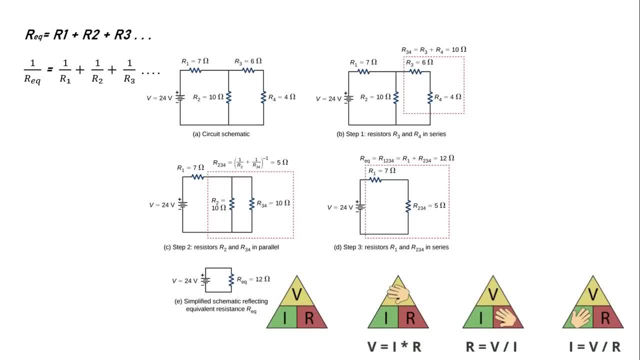 have our Ohm's law formula handy right. so what we can find out now is how much current is flowing in this circuit. how we can do that, we will use this formula: I is equal to V by R, where V is 24 and R is 12, so we will get 2 amperes right. so now, if we want to know voltages across each, 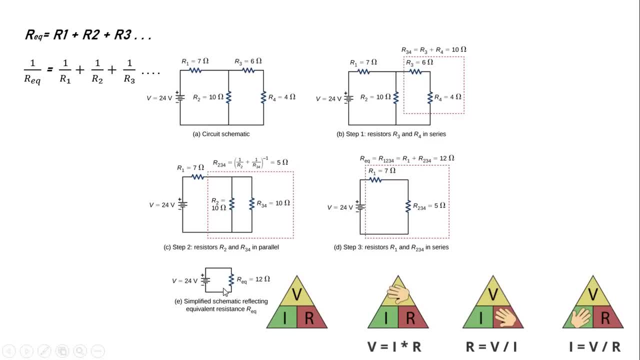 resistance and current flowing in each resistance. we can work our way backwards. now, right, so we know 2 amperes is flowing in the circuit, so we can calculate the voltages across these two resistances. right, so first we will calculate across 7 ohm resistor. so how will we do that? we'll use V is equal to. 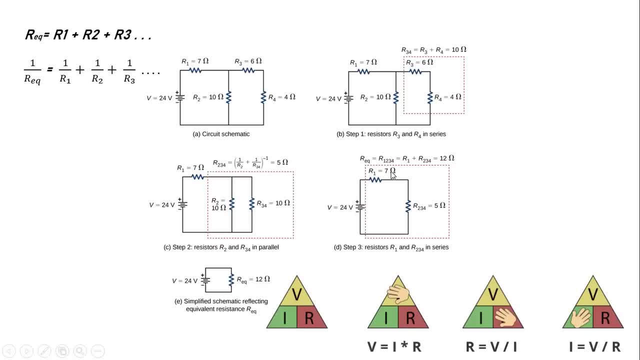 I into R. I is two and R is seven, so we will get 14 volts across this, okay, and here we will get 2 into 5- 10 volts, right, so you can see, 14 plus 10 is 24. we are satisfying the things which we have studied so far. 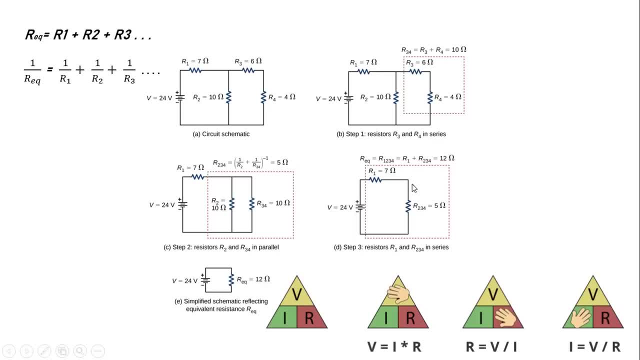 now we'll move one step back. so we knew voltage across this resistance was 10 volts, right? so in this section also the voltage will be 10 volts. so now, since this is a parallel circuit, in both of the resistances voltage will be 10 volts. so now we can calculate current in this right. 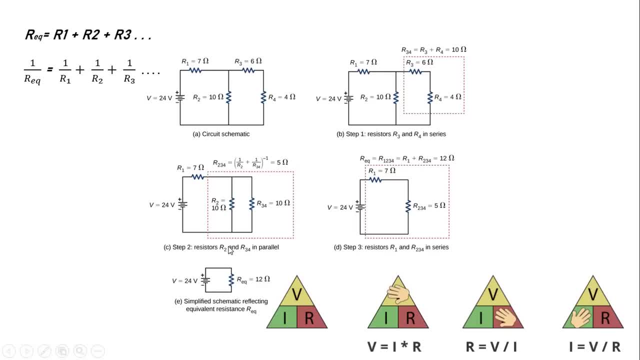 by using this formula again: right, v is 10 and r is also 10, so 1 ampere would be flowing inside it. the answer would be same for this one as well. right now, if we take one step back again, we'll have to calculate voltage across these two resistances. how will we do that? again, we 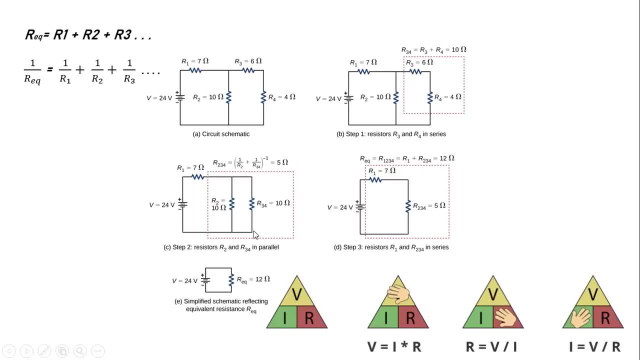 use this formula: v is equal to i into r, so current was 1 ampere in this, so in this as well it will be 1 ampere. so we know 6 into 1 is 6 volts and across this one we'll have 4 volts using the same formula. right? so we have all the unknown values right now, since 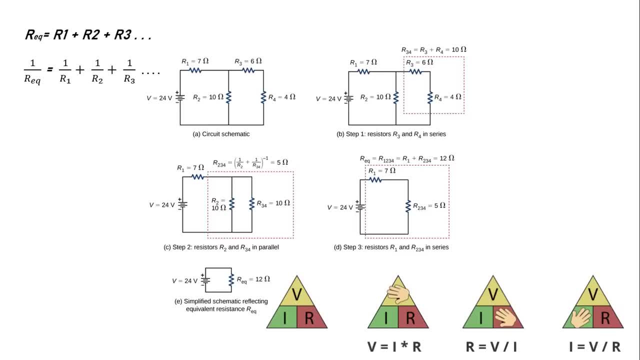 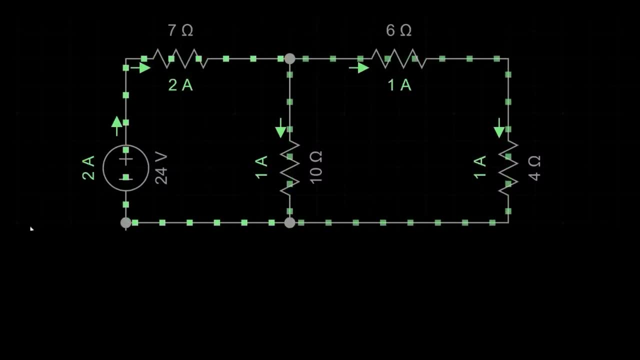 there were so many values, i can understand it must be a little difficult for some of you to visualize it, so i have created a circuit to help you visualize a little right. let's have a look at exactly similar circuit which we saw earlier, and i have written all the values of current. 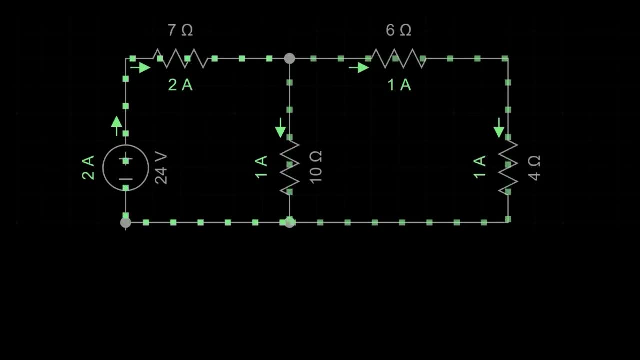 flowing in each resistance. and now i will show you the voltages across each resistance. let's keep this formula handy, as always. now i will show you voltage across each resistance. it is 14 volts across 7 ohms, 6 volts across 6 ohms, 4 volts across 4 ohms and 10 volts across. 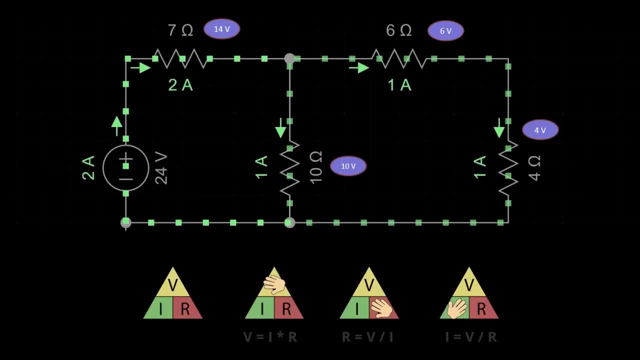 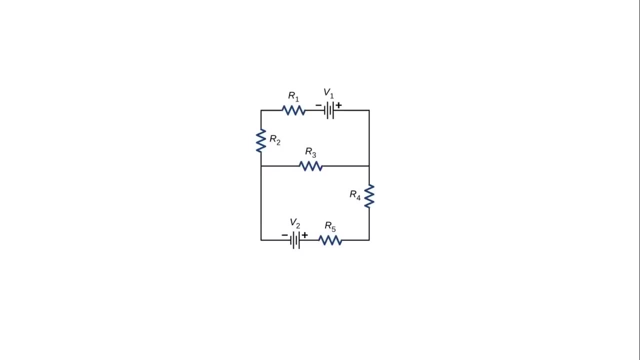 10 ohms right. so if you have understood this part, i can say you have understood really important fundamental about using resistances in series and parallel. but you may also find circuits like this, okay, where we have two batteries right in circuits like these you cannot simplify the circuits which we have seen so far. so there, 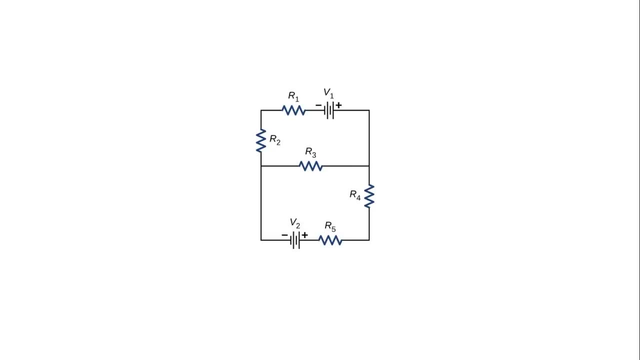 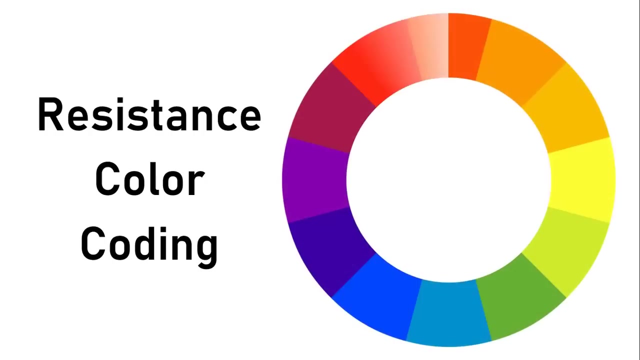 are some advanced concepts, such as kirchhoff's law, okay, which is used to calculate the unknown values in this circuit, but that will go beyond the scope of our course right now. so one last thing about resistances i want to tell you is identifying the resistances based on their color bands. let's have a look at that now. resistances- 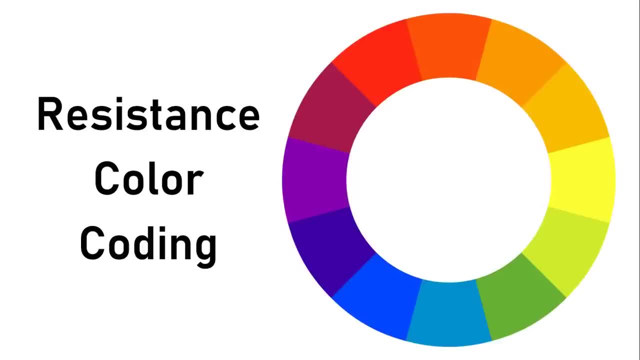 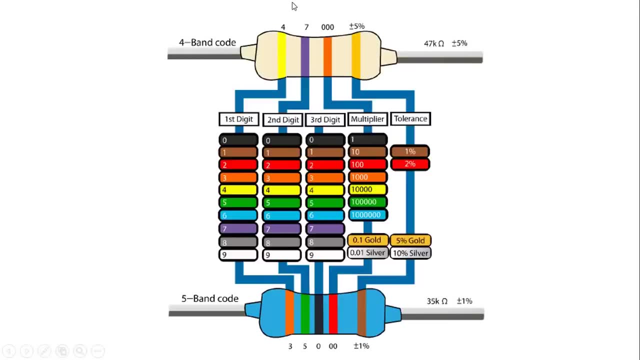 come with the four or five color bands denoting the value of resistance it will offer in the circuit. so you see in this diagram there are four band resistors and there are five band resistors. okay, in a four band resistor the first band will tell you the first digit. the second band will tell: 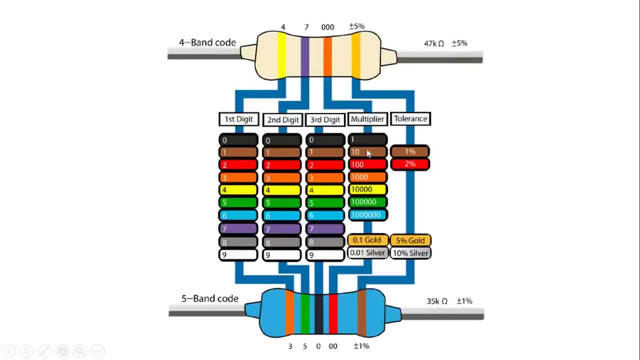 you the second digit. the third band will tell you the number of zeros which you need to put after the first two digits and the fourth band tells the error. percentage means it can be that much percentage above or below the stated value. now see the first band in this case is yellow. so it the first digit. 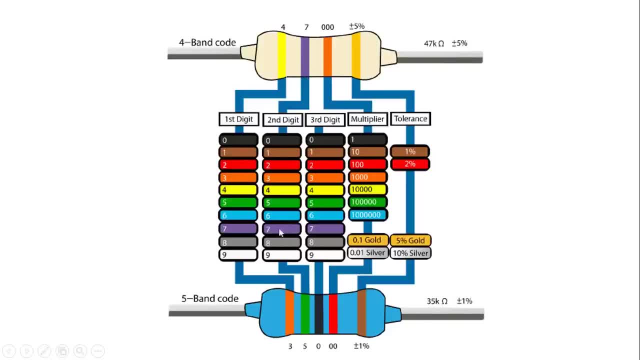 will be four. the second band is violet, so the second digit will be seven. the third band is orange in color, so the multiplier will be one thousand, so we get the value of 47 000, and the fourth band is gold, so that means it will have a tolerance of. 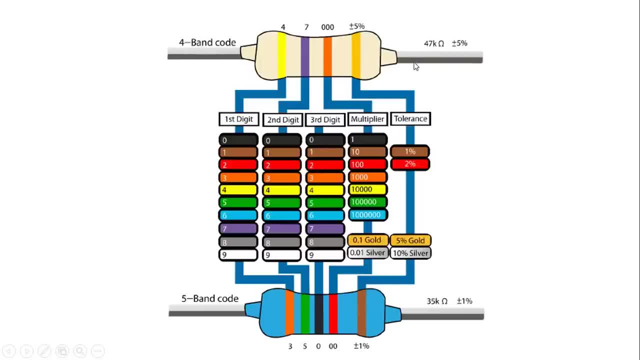 plus minus five percent. so the net value of this resistance is 47 000 ohms, or you can say 47 kilo ohms with the tolerance of five percent. now we see the five band code. okay, the first band tells you the first digit. the second band tells you the second digit. the third band tells you the third. 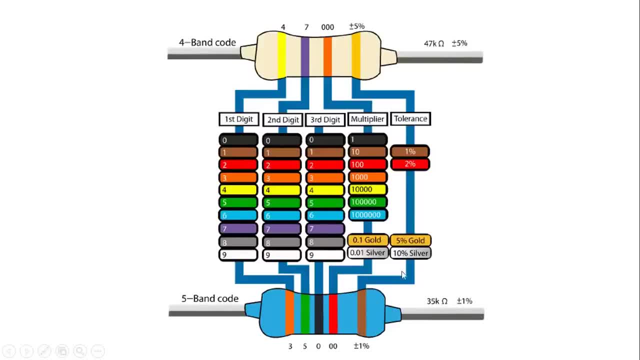 digit. fourth band tells you the multiplier here and first bank tells you the tolerance. we'll consider this example. first band is orange in color, so the first digit will be three. second band is green, so the value will be five. the third band is black in color, so the third value will be zero. 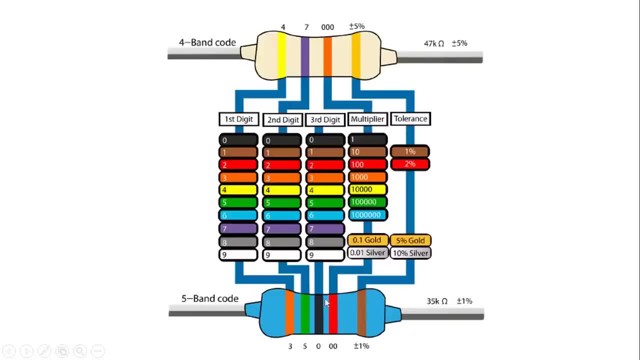 and fourth band is red, so the multiplier will be 100. till now we get 34000 and 00, so this is 35,000, and the last band is brown in color, so 1% of tolerance. so the net answer will be 35 kilo ohms with a tolerance of 1%. You can refer to this chart whenever you need. 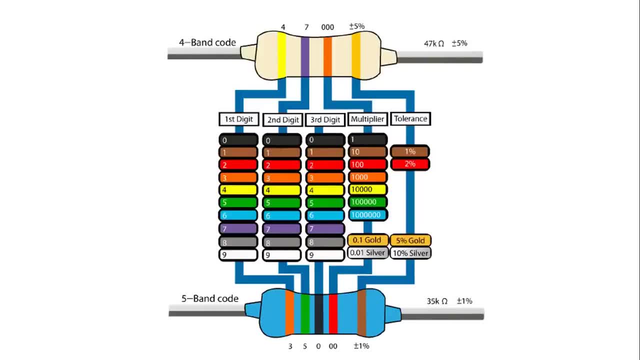 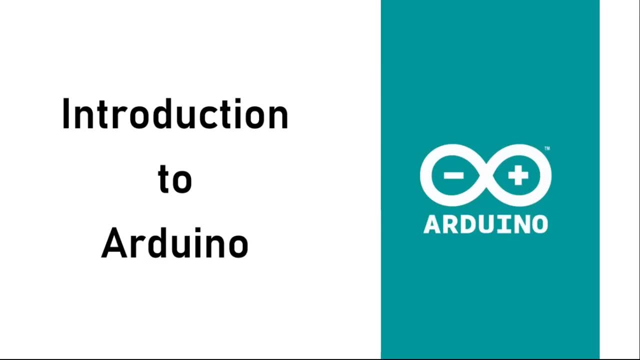 to find the value of your resistances, and I understand this might be confusing at first, but with practice you can understand this very easily. In this section we will finally take a look at the main thing. Most of you must be already waiting for the section to come up, so 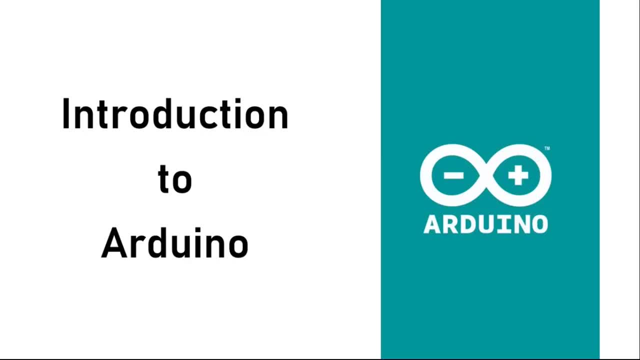 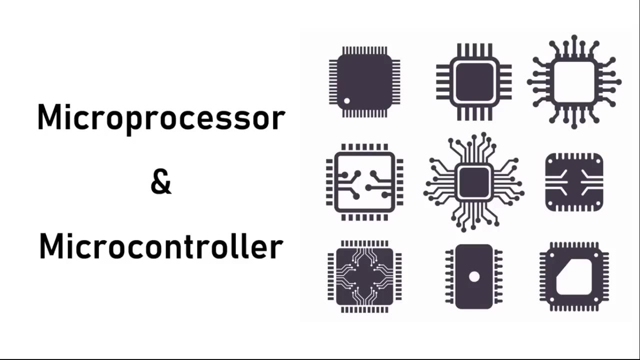 this blue colored thing which is present in your kit is the Arduino board. I will tell you what is it, what it can do and how to start using it. finally, but before that, I would like to tell you about some terms which you may or may not have heard about before starting this course. 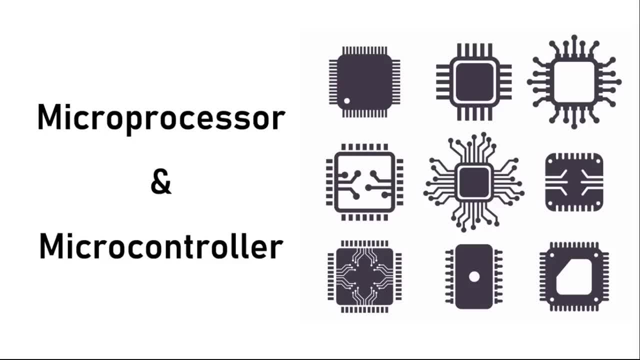 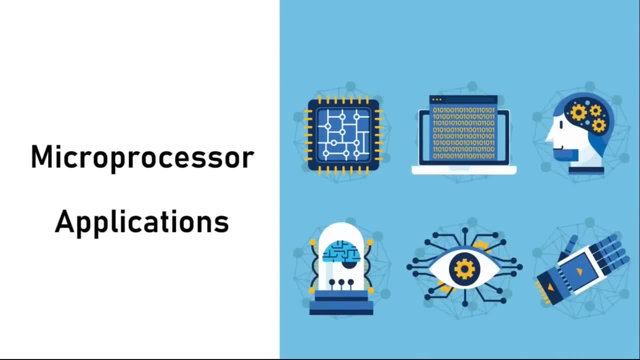 So these terms are microprocessor, micrometroller, memory, integrated circuits, etc. Microprocessors are known as a brain of any computer. They consist of a CPU, which stands for Central Processing Unit, which is responsible for doing all the computations and calculations which 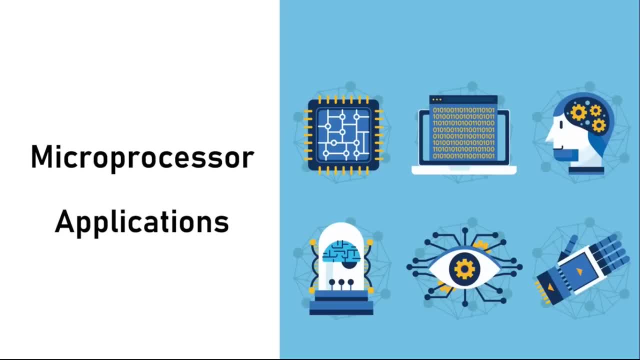 we need to carry out. They need additional peripherals like RAM and ROM in order to function. Example of a microprocessor is the CPU which is being used in your computer right now. If you go and check the history of microprocessors, you will see the microprocessors have come a long. 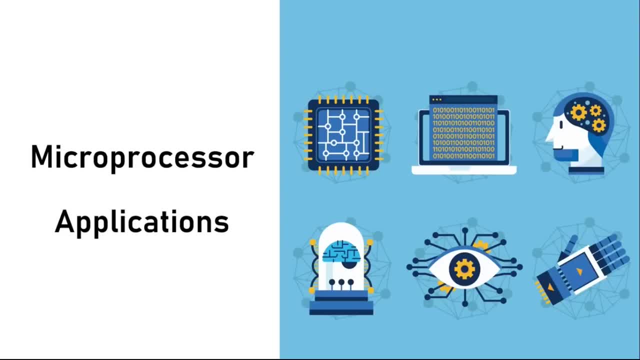 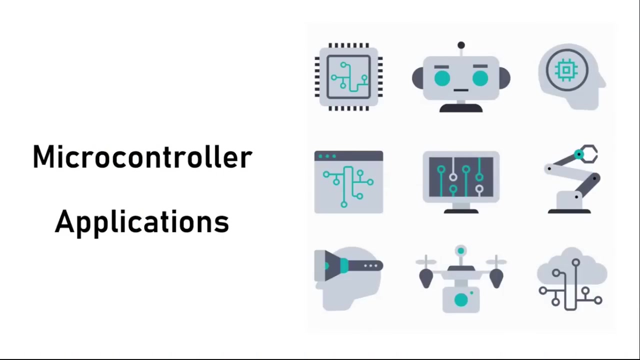 way in improvements and developments. Microprocessors and graphic processors are used where there is a need of heavy computational cycles, like artificial intelligence, deep learning, self-driving cars and high-end robots. Our daily applications, like playing games, movies, browsing internet, also requires a microprocessor. And then there are microcontrollers. Microcontrollers are 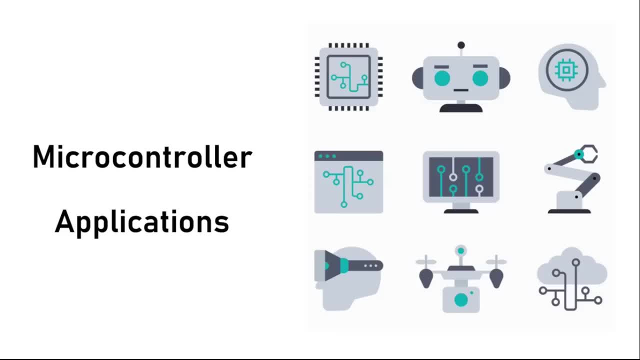 integrated chips that are basically tiny computers but are powerful enough to do a lot many tasks, like controlling motors, pumps, other appliances, or they can send some sensor data to internet, cloud, control basic displays and even act as brains of some intermediate level robots. Applications are endless. trust me, The power requirements of such integrated chips. 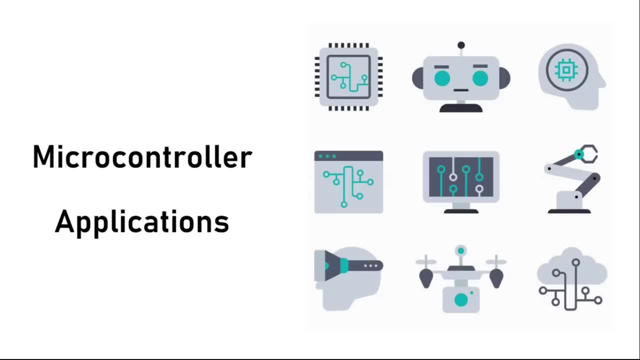 is very low and you can even run these chips on batteries for days or even months. They have all the peripherals, like memory and flash storage, built on the same chip. If we compare the power requirements of these chips with the power requirements of other chips, 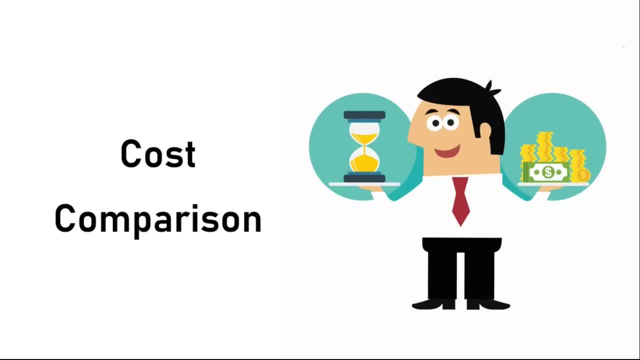 we can see that the microcontroller is far cheaper than the microprocessor. However, microcontroller cannot be used in place of a microprocessor and using a microprocessor is not advised in place of a microcontroller as it makes the application quite costly. If we compare them in terms of speed, if we say human brain is fast, 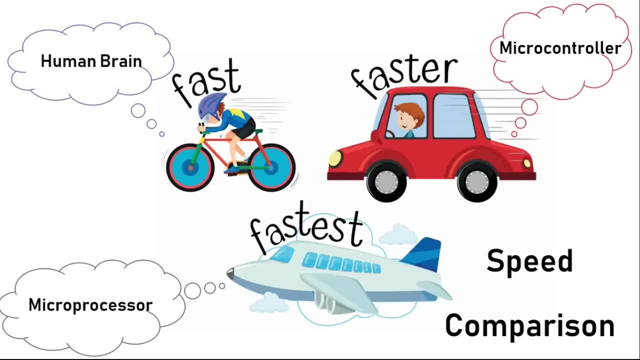 then microcontroller is faster and microprocessor is fastest. But please note we are talking in a very general way. This won't be applicable if you compare an old generation thing with a new generation thing. As technology advances it won't make any sense to compare. And also some exceptions: 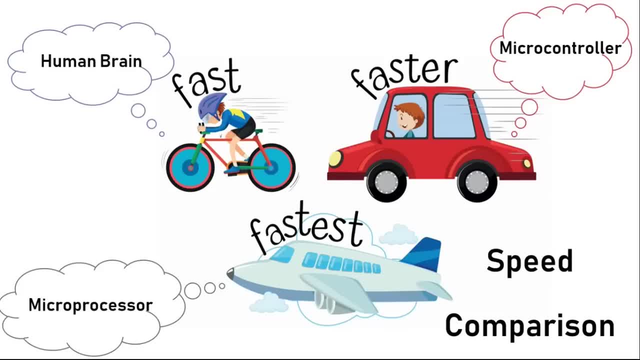 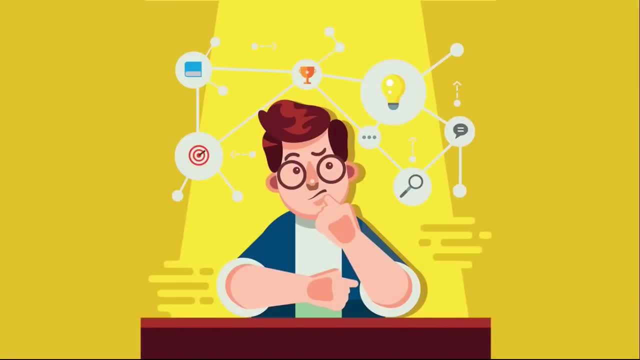 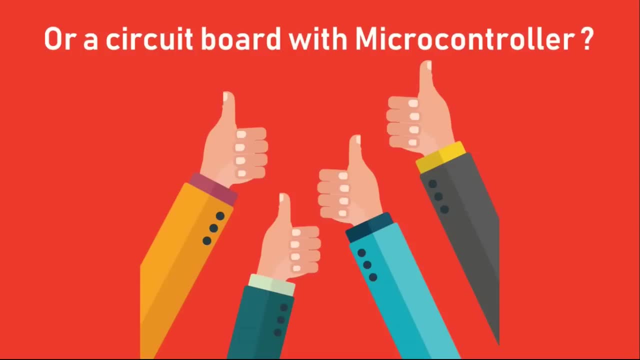 are always there. It is really possible that you, or any human may be faster. So do you have any guesses in which category a Arduino board will fall? If you said microcontroller, then you are partially right. An absolutely correct answer is that our 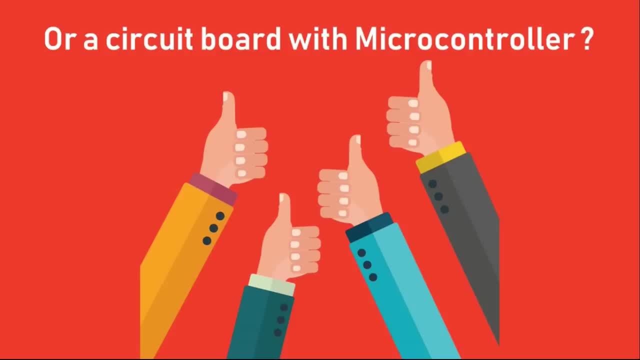 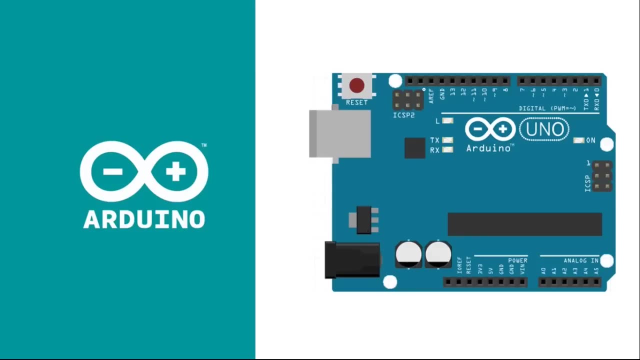 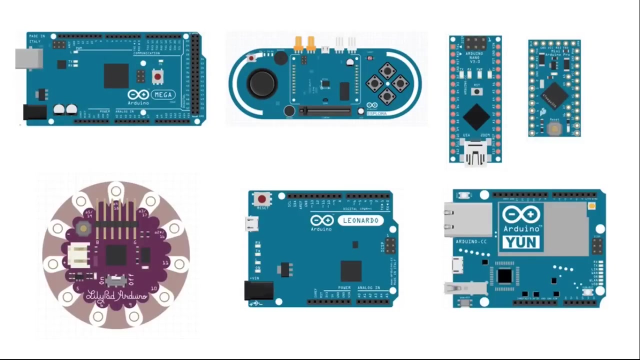 Arduino is a circuit board which has a microcontroller on it which acts as the heart of that board. The Arduino board given to you in your kit is Arduino Uno, which uses microcontroller Atmega328.. There are many more kinds of Arduino boards available with other microcontrollers. 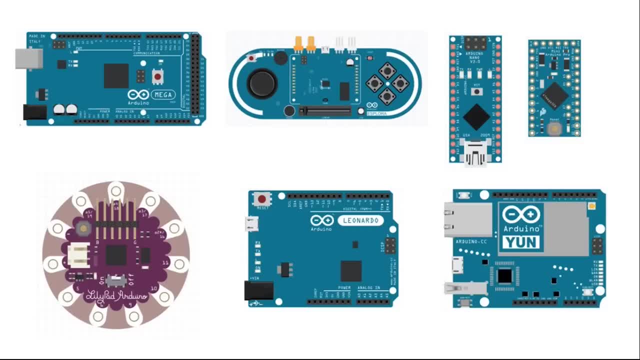 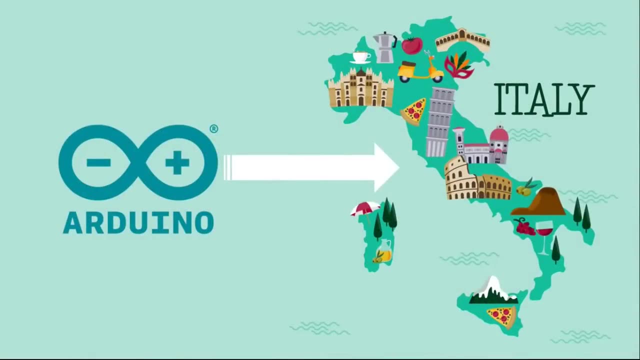 which may be superior or inferior to Atmega328, but Arduino Uno is just right for our applications. You may want to pause the video here to have a look at all these boards and admire how beautifully they are made. So Arduino is basically a company in Italy. 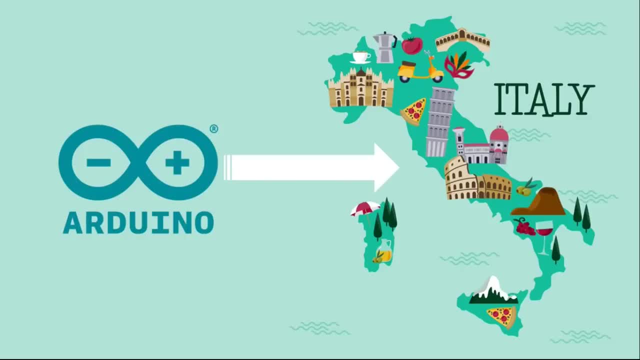 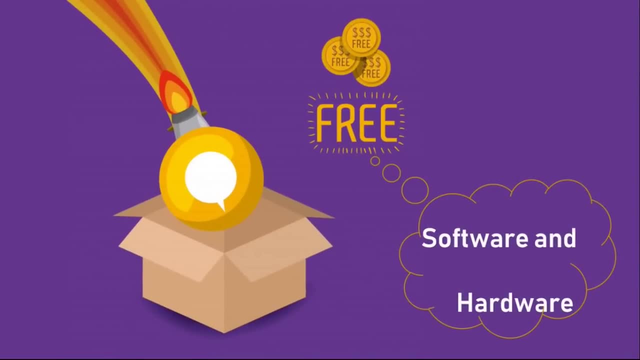 which made it really easy for people to use microcontrollers for their application. The hardware and software of Arduino is open source, which means one can have access to the files and even modify them for their own work. Since it is open source, many other companies 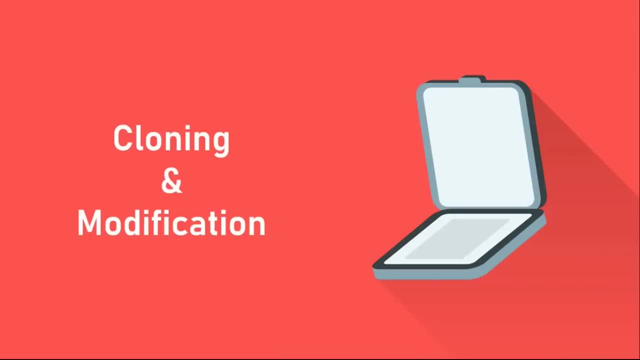 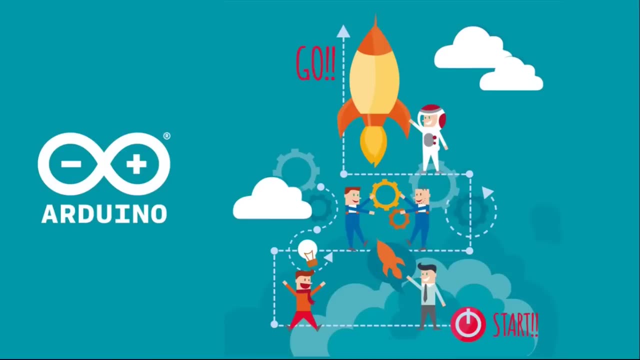 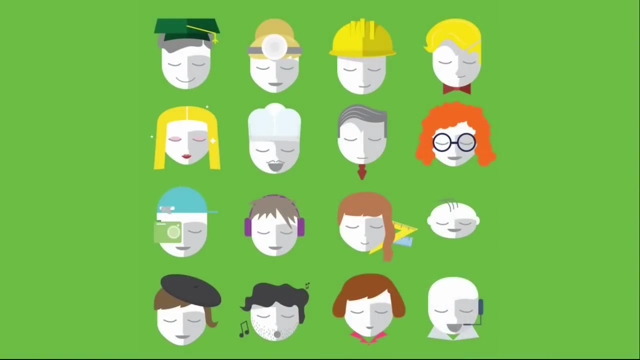 take their design and manufacture their own versions of Arduino. It is really easy to clone and modify the Arduino board. What makes Arduino a beginner friendly tool is their easy to use hardware and software. It can be used even by people having no technical background. 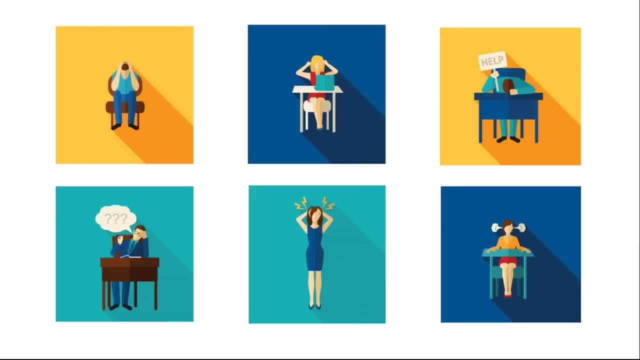 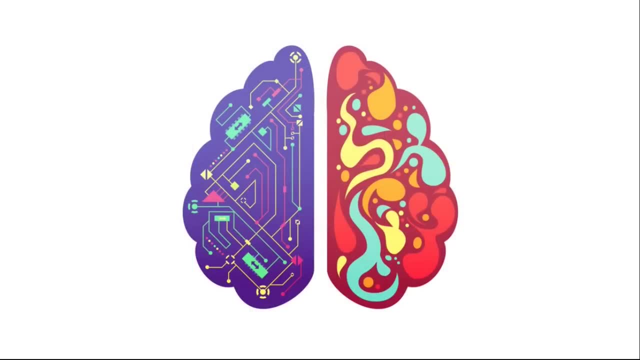 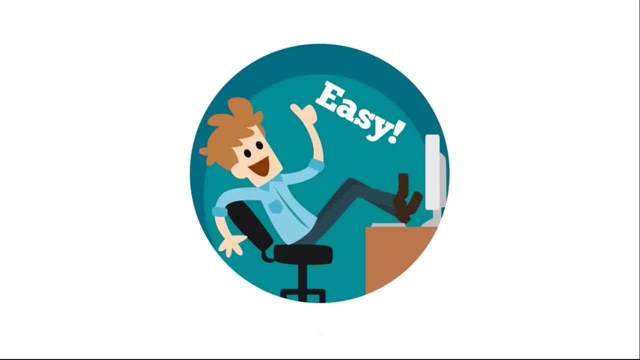 Earlier people would have to use very difficult assembly language to control their boards, But it is not the case with Arduino. As you progress with the course, you will see yourself with how easy and intuitive this tool is. You will see that uploading the code is as simple as plugging a USB cable and clicking upload button. 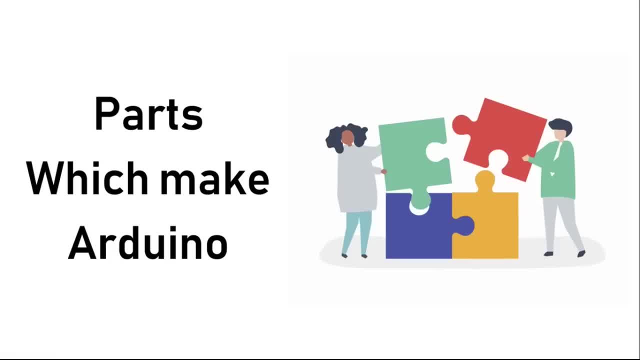 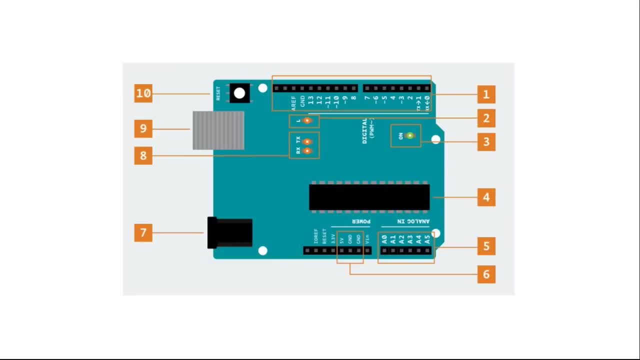 In this video we will see the parts which make up the Arduino board. So this is the diagram of Arduino board, which shows the typical components which are placed on it. So we will begin by the digital pins, The pins which you see here, which are numbered 0 to 13. 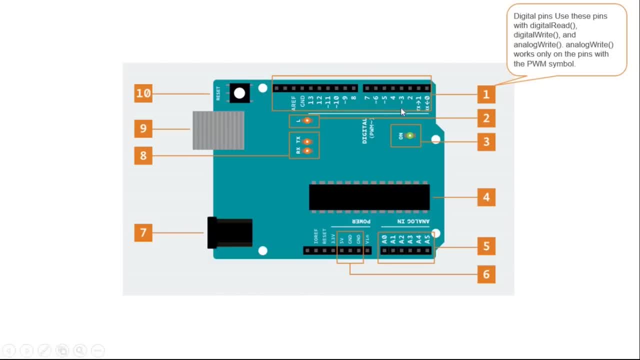 and some pins have a special symbol, like this curvy symbol on it. This symbol denotes PWM capability. That means these pins support PWM. Other than that, these pins take digital input from sensors and give digital output to some of the components. So then we move to the built-in LED, which is shown by this LED. 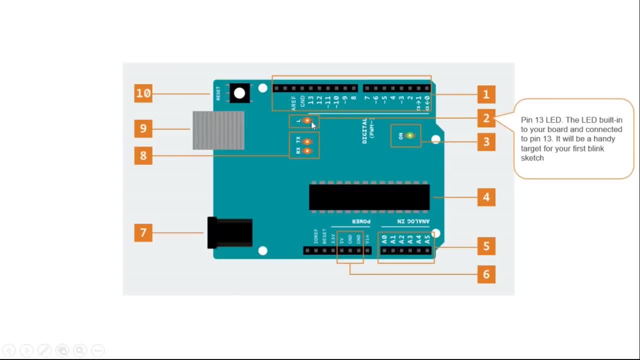 This LED, by default, is connected to pin number 13.. So whenever pin number 13 goes high, this LED will turn on, And when that pin goes low, this LED will turn off And then we will see the power LED. This is the power LED. 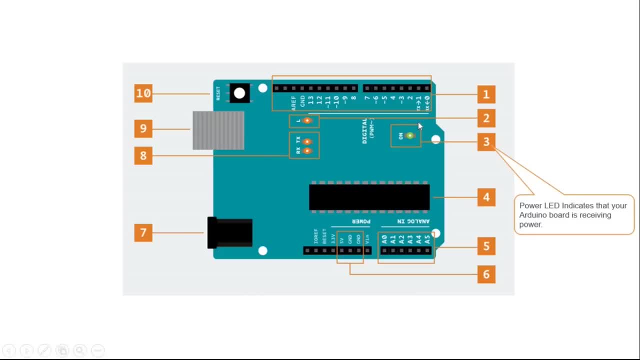 If this LED is turned on, that means your Arduino is plugged in. That means it's turned on right now. Then we have the main component, the ATmega328 chip. It controls all the main functions of this board. Whatever is happening on this board is due to this chip. 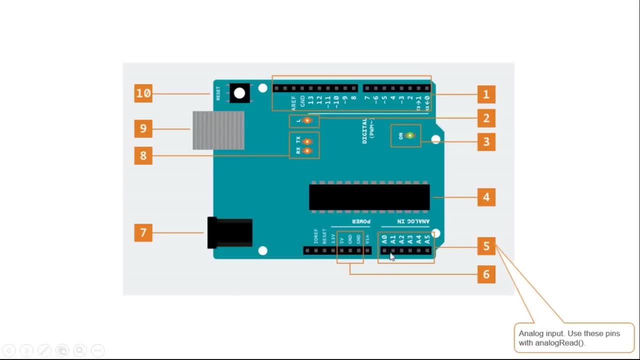 Then we have analog pins. We have 6 analog pins on this board, numbered from A0 to A5.. We can connect any analog sensor on these pins. Then we have the power pins. These are the power pins. You can power any component using these. 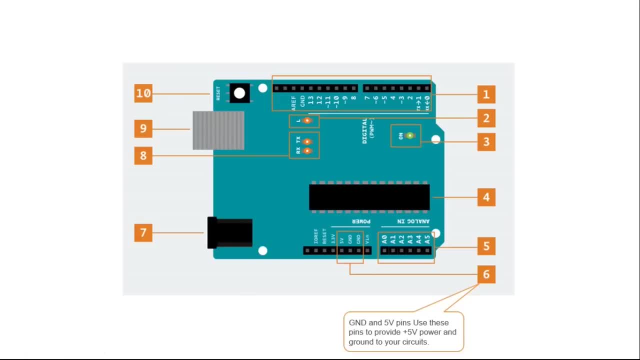 pins, But make sure that your components are not drawing a lot of current Basic sensors and basic breadboard circuits are fine with these pins. Then we see the power DC jack. If you want to connect your Arduino externally through a DC jack, you can connect it through this jack. The voltage input it can accept is 7 volts to 12 volts. 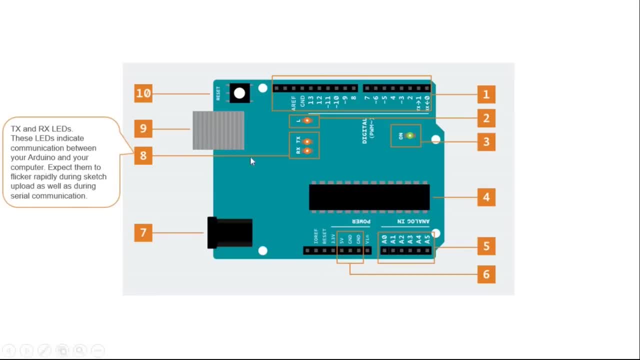 Then we have TX and RX LEDs. These are the TX and RX LEDs. RX means receive, TX means send, transmit, Okay. So whenever these LEDs are blinking, that means the Arduino board is either communicating with the current or with the DC. 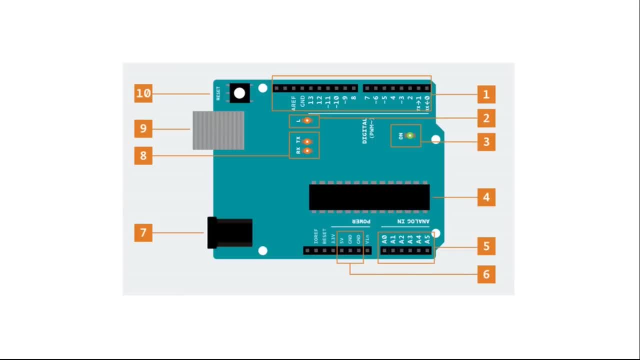 Then we have the USB jack. You can connect your Arduino board with your computer using this jack. Then we have the reset button. This button reloads the entire code which is running on the Arduino board. But please note that this button does not clear the memory of Arduino. 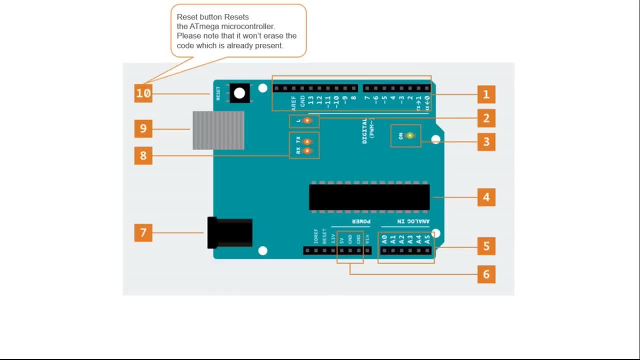 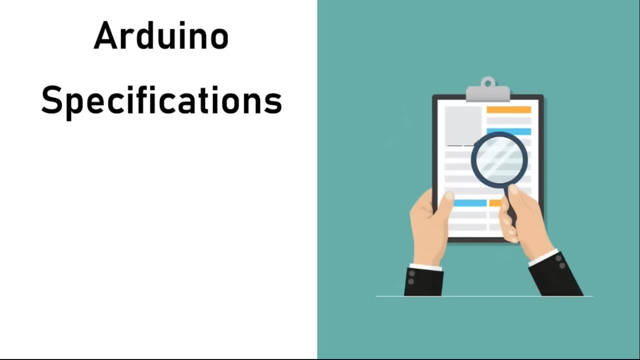 Here are a few technical specifications of Arduino Uno. My technical specifications are as follows. The first one is the USB jack. By technical specifications I mean the information which you look while buying any item or a computer. Like in a computer you see how much disk space is there. 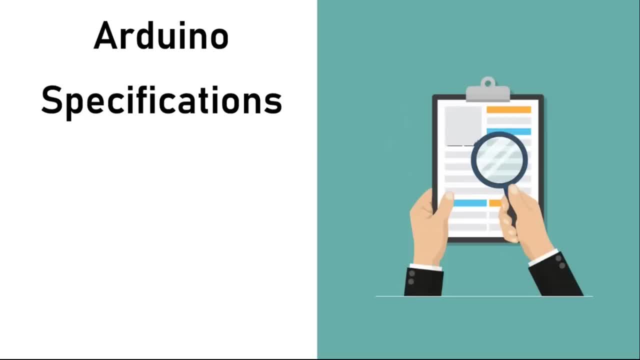 how much RAM does it have? or processor it has? Similarly, Arduino, being a microcontroller board, has some technical specifications. Like it, has ATmega328 as the main chip which does all the work. It operates at 5 volts. The input voltage which it can accept is 5 to 12 volts. 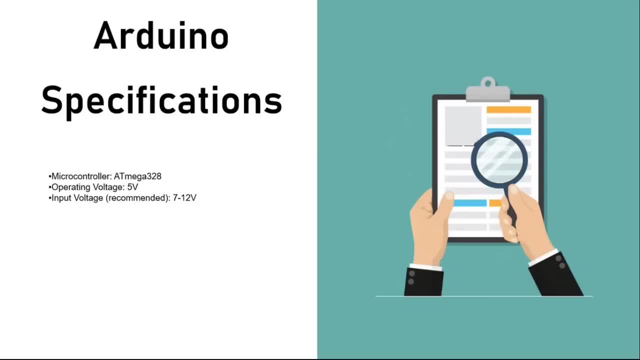 Although, according to the datasheet of Arduino, the recommended voltage is 7 to 12 volts and the limits are 6 to 20 volts. So I recommend that 5 to 12 volts is a good enough voltage to operate Arduino with. 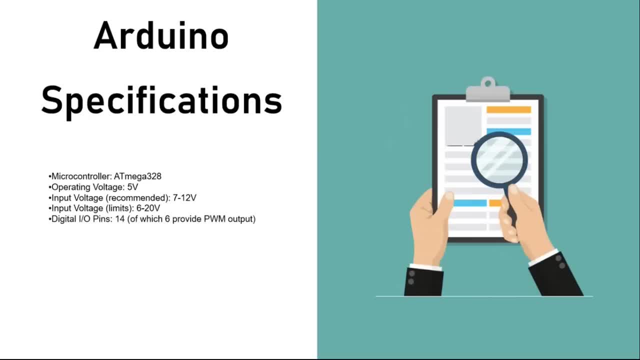 And then there are 14 digital pins, out of which 6 are PWM capable. Don't worry about PWM right now, but just think having PWM capability is a good thing. The 6 analog pins are the main transition pins. The 6 analog pins are the Osmo's pin, thegua and thessus pins. Then there are 6 analog pins to be uh. connected to the Arduino board of Arduino with an именно, So that is only the pin number. and then there are 6 data pins where it is the PWM Islands. Then there are 6 analog pins to be uh connected to the Arduino board of Arduino. Then there are 6 analog pins to be uh connected to the Arduino board of Arduino. 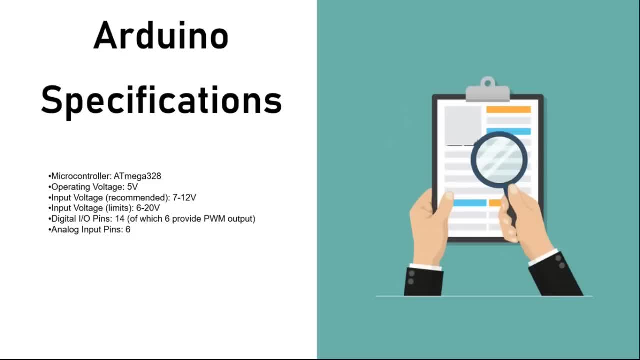 pins which are used to connect analog sensors to the Arduino. you can understand that these pins are connected to Arduino through a 10-bit ADC. an ADC is an analog to digital converter. we'll talk about ADC in further lectures. the IO pins are capable of supplying 40 milli amperes of current, so these pins 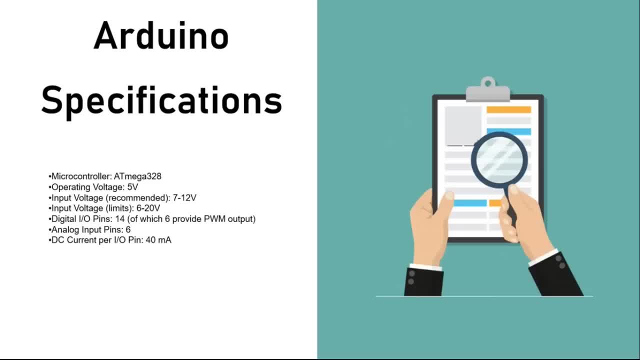 cannot drive large appliances or the things which require more current like motors, and it is or not even recommended that you run motors through Arduino. but few LEDs and most sensors which we use in this course do not draw very large amount of current, so these pins are just fine. there is a 3.3 volt. 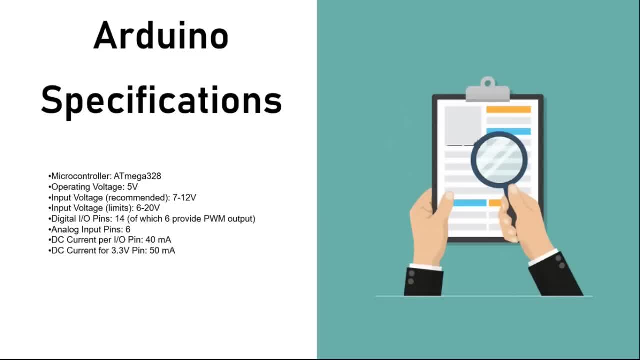 pin as well, and the maximum current you can draw from it is 50 milli amperes, and there is a flash memory of 32 KB which we use to store all the programs into it, and the flash memory of 32 KB which we use to store all the programs into it. 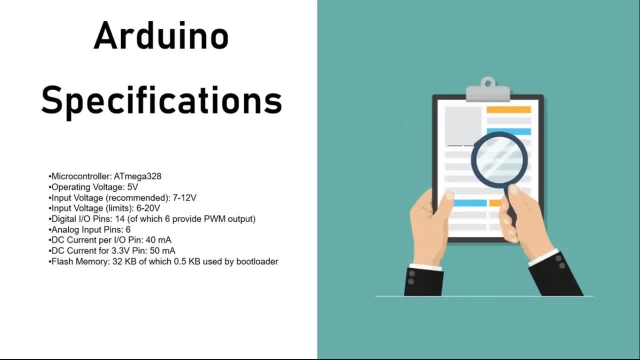 32 KB must be seeming like a very less amount, but trust me, you can store lines of thousand, even 2,000 lines of code in this and it won't even exceed 10% of the storage. then it have SRAM of 2 KB, which is a volatile memory, or more generally, 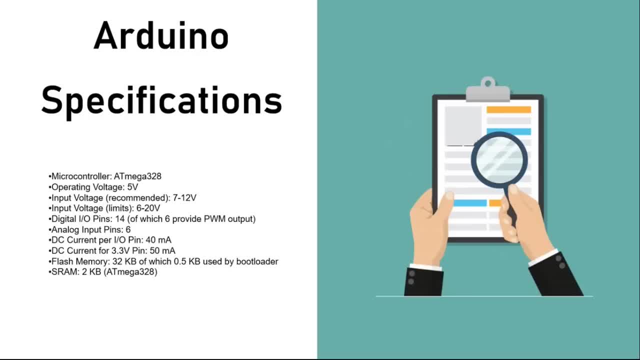 it is similar to RAM on a computer. again, it would seem to less and I would repeat what I said for the flash memory, that it is more than enough. it also has 1 KB of EE p rom which can store some variables even after you search of the. 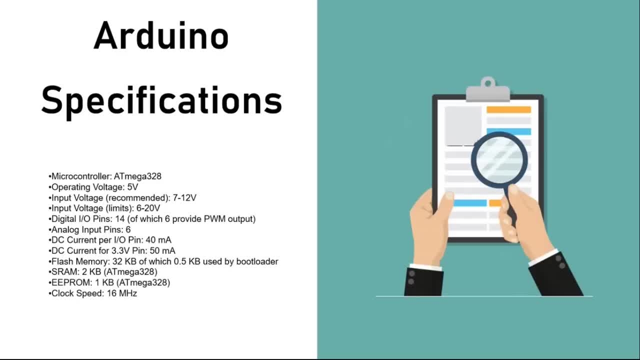 Arduino clock speed is 16 megahertz. clock speed is the speed that microprocessor executes each instruction. 1 megahertz representing 1 million cycles per second. I understand a lot of information in this video. might have just bounced over your head and it's perfectly okay if you don't understand. 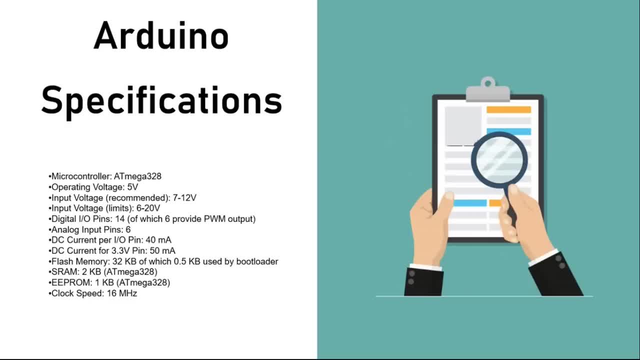 some portion of it. I would just say: don't lose your motivation and just stick with us, and I promise you you will understand each of this information needed if you learn this guide on oliverferchcom in every part of it by the end of the course. If not, we are always here for help. 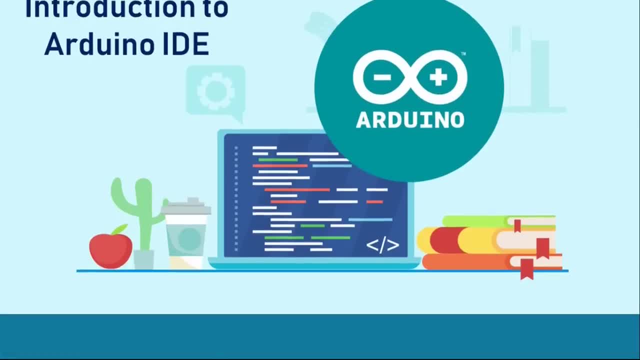 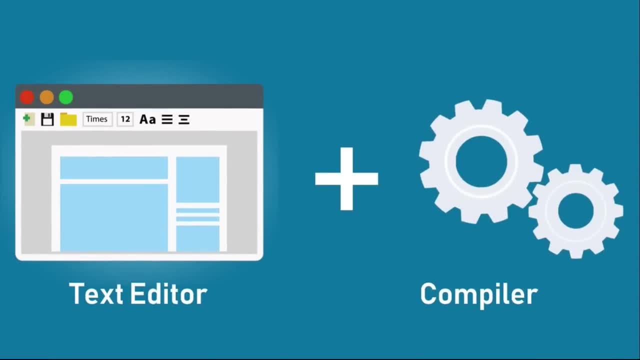 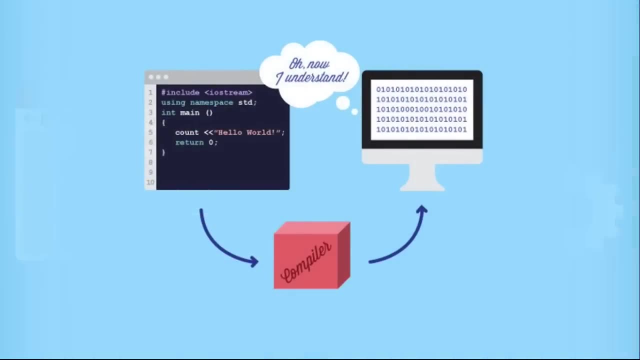 In this section I will tell you about Arduino IDE. But before we jump into that, first of all we need to understand what an IDE is. A text editor like a notepad, along with a compiler is a bare minimum requirement to start coding. But wait, what is a compiler? 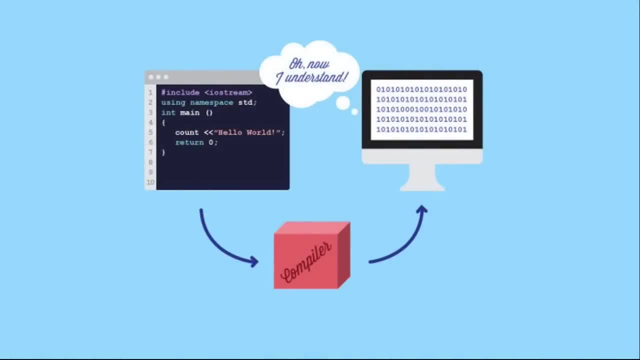 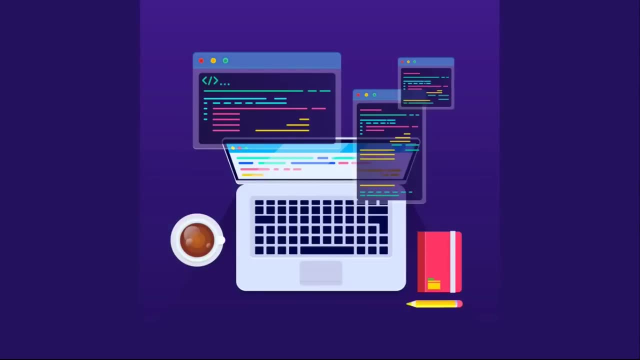 Compiler is a special program that processes statements written in a programming language and turns them into a machine language, which are basically zeros and ones which a computer can understand. But unlike text editor, an IDE, which stands for Integrated Development Environment, is a software tool which has a lot more functionality to make programming. 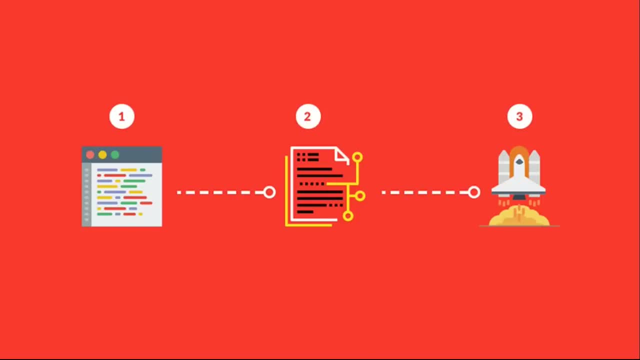 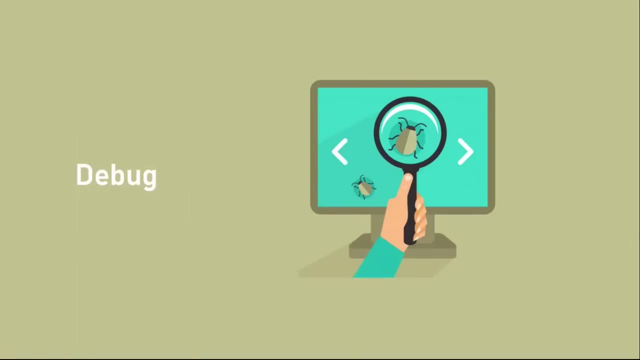 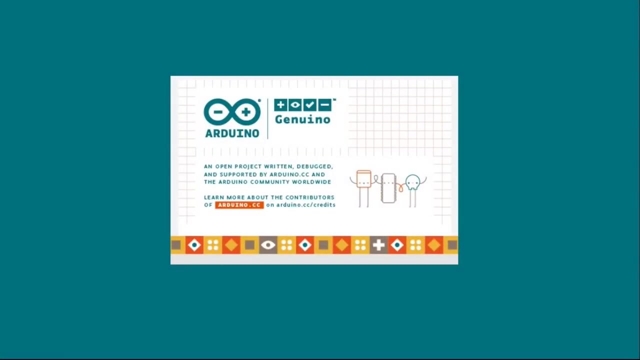 easier for the user. It has a built-in text editor and compiler, along with easy-to-use tools, menus and buttons to compile, run, debug and run. It also has the ability to analyze and save the programs. Considering Arduino, they also have one official IDE, which has buttons to verify and upload. 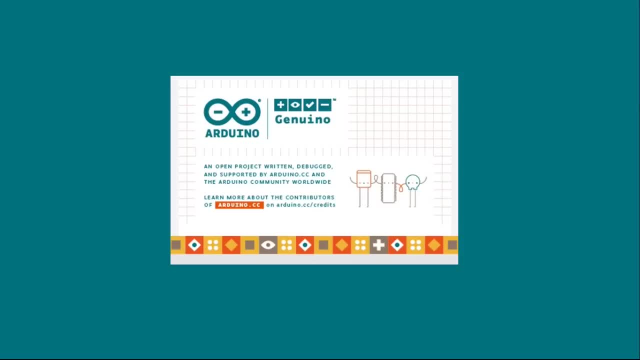 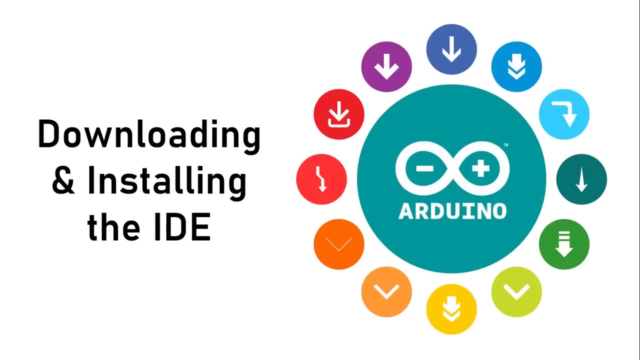 the sketches. They also have easy-to-use menus to select boards and ports. Throughout the course we will be using the official Arduino IDE And for that, in the following sections, we will be downloading and installing the official Arduino IDE. Now I will tell you how to install the Arduino IDE. 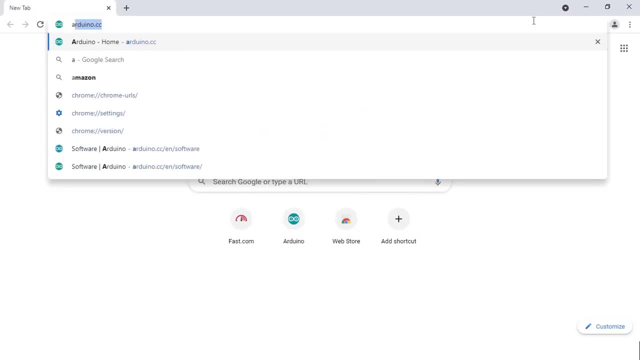 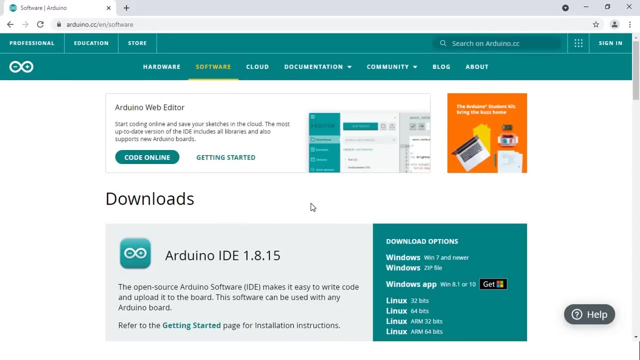 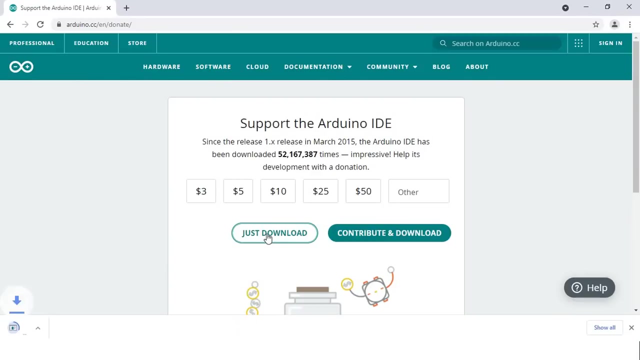 First go to any browser and go to Arduinocc. Then click on the software tab. You will find many options here. We will go with the Windows installer. Click on Just download if you don't wish to donate anything. Donations like these help. 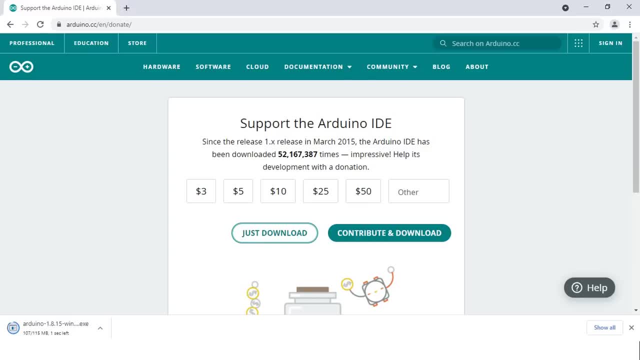 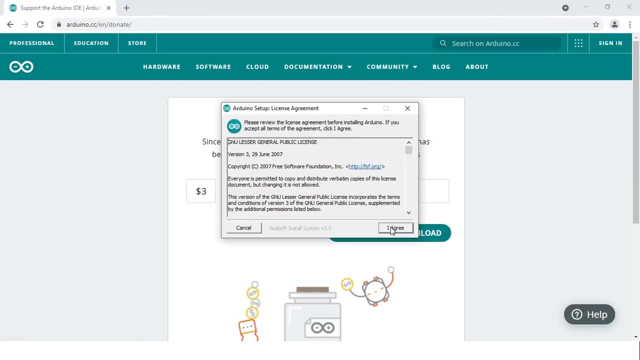 open-source communities to fund themselves. Once the download completes, click on the install button. We will click on it, And when the installation starts, click on. I agree, Make sure that all these boxes are checked. These are the essential drivers, which are: 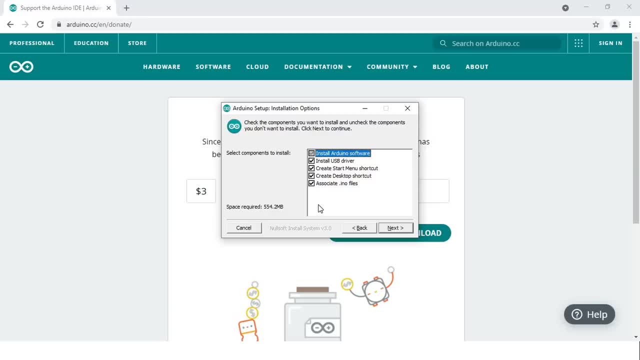 required for your computer to detect and communicate with the Arduino board right. We will click on next. Then we will choose the destination folder. I will go with the default one And click on install. This process may take some time, So let's start. 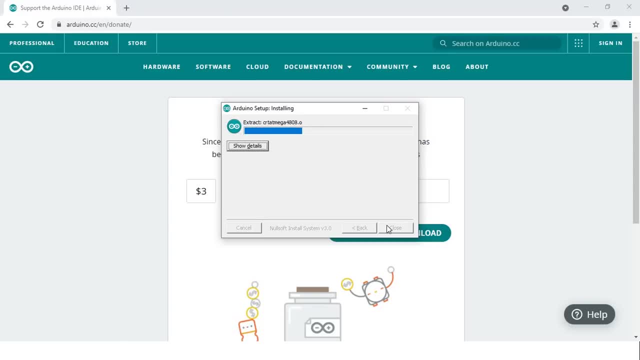 Let's wait for it to finish. In my screen it says completed, But some people may get additional prompts to install those additional drivers. All you need to do is just click on install on them as well, And then, once it is completed for you, click on close And then you will find the Arduino. 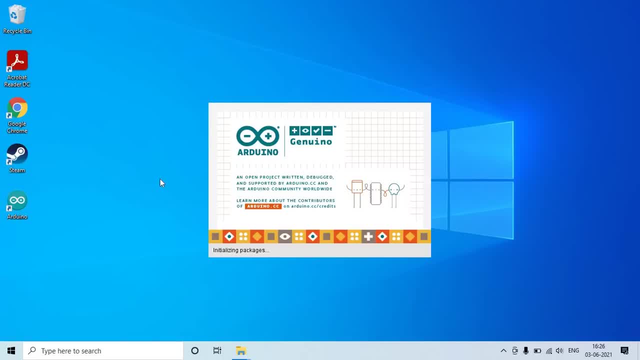 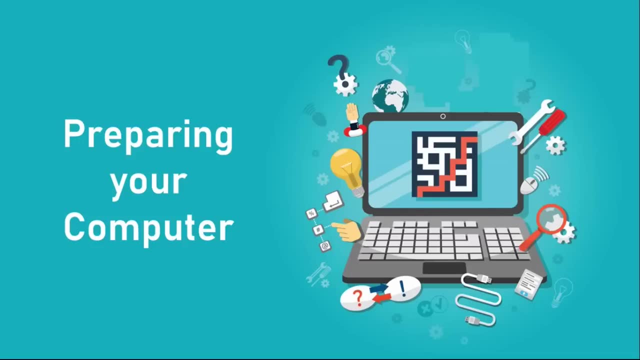 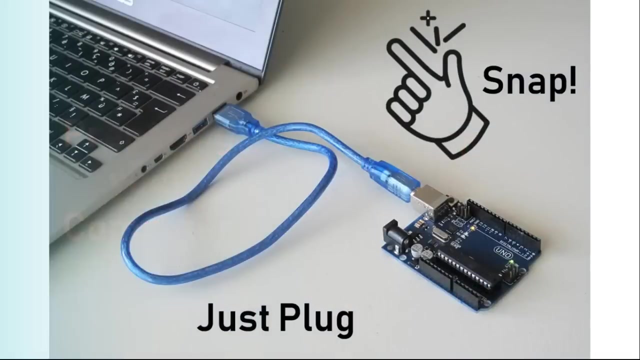 icon on your desktop. Then you just double click on it And here is your fully functional Arduino IDE window. So now we will set up our computer for uploading our first basic sketch. There is nothing complicated we need to do. The first step is we need to plug in our Arduino board with the USB cable. 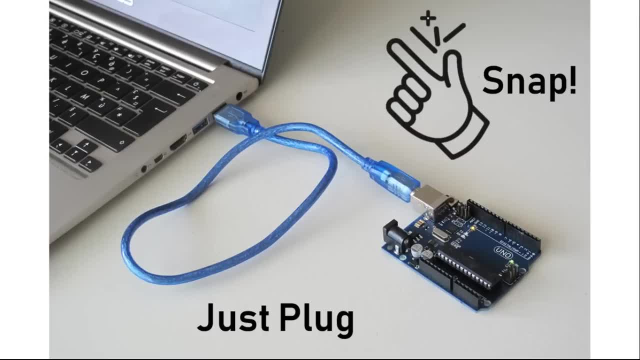 given in the box, And once you do that, your computer will automatically detect that Arduino has been plugged in And it will list it out on a specific serial port In Windows- it is known as a COM port- which you need to go. 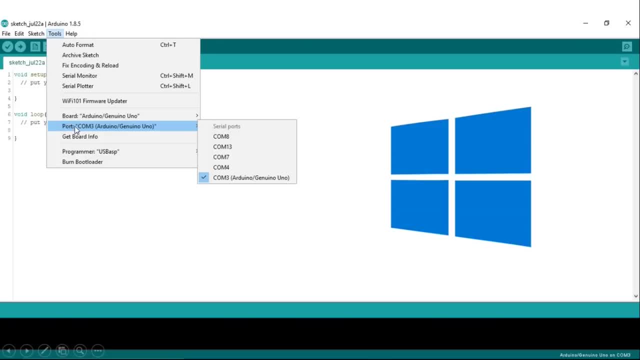 And select using tools, Go to tools and then go to port and you will automatically see a COM port here. It is very likely that you see COM 3 if you have plugged your Arduino for the very first time. Okay, So you will see Arduino Genuino Uno written over here. 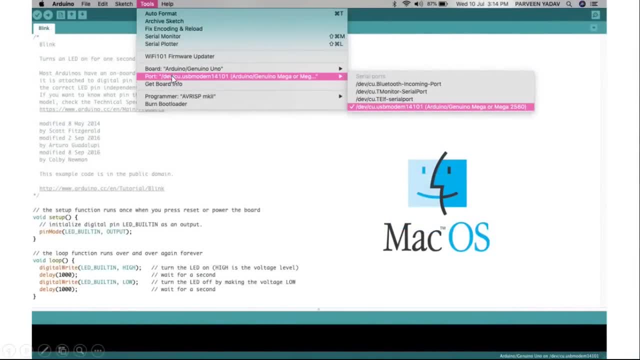 If you are using Mac, then you will see something like this: forward slash dev dot. forward slash cu dot USB modem. This is the port number And you will see Arduino Uno. You will see Arduino Uno here instead of Arduino Mega. I have tested with Arduino Mega, that's. 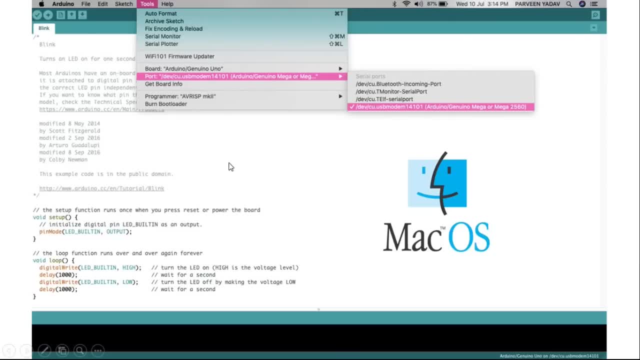 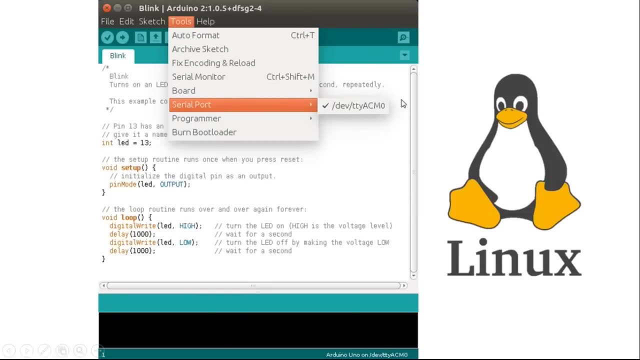 why it is showing it like that, but you will see Arduino Uno right. If you are using Linux, you will see serial port as forward slash dev tty acm0.. It is most likely you will find it at acm0.. After this step, we are just ready to upload our first basic sketch. 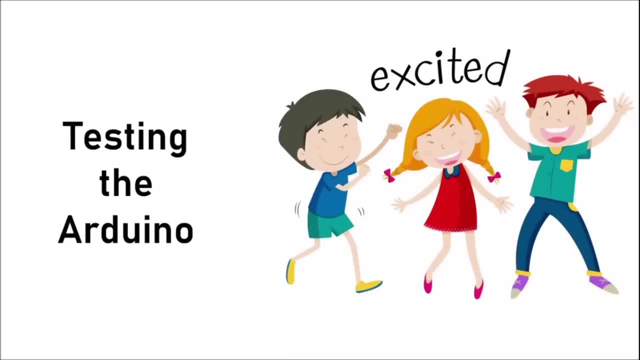 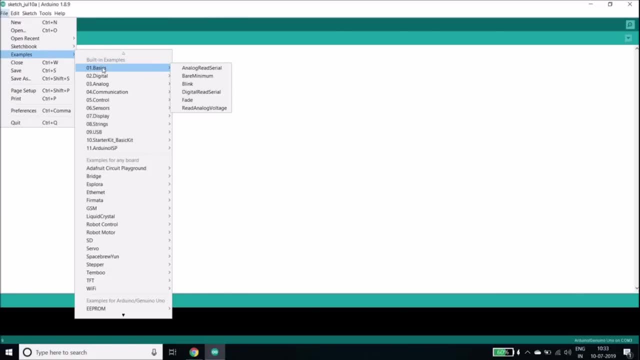 So, finally, we will be testing our Arduino boards And for that we will be using the built-in example sketches. So, in order to upload our first sketch, we will go to examples, we will go to basics and then we will select the blink sketch. 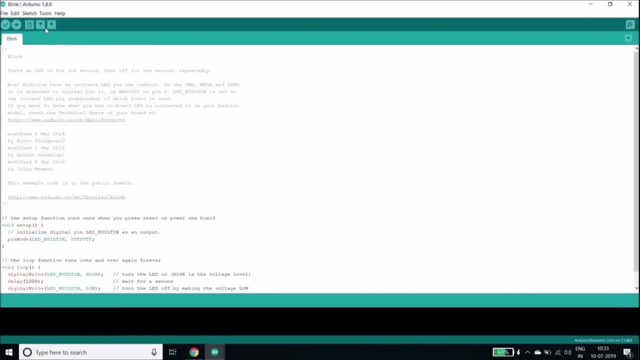 This is the first sketch which we will be uploading on our Arduino board. We will go to tools, we will select our board as Arduino Uno and we will select our port as COM 3.. And then we will go to upload button. We will click on upload in order to upload the code. 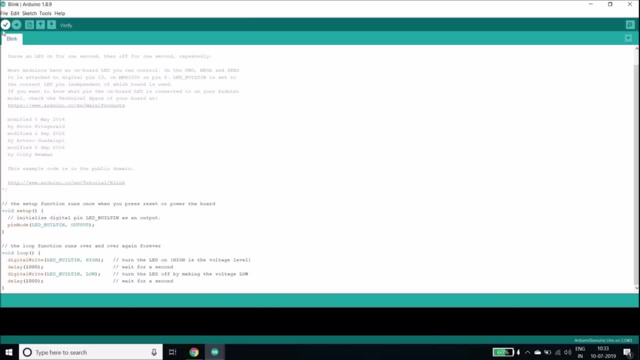 There are more buttons like verify, save, open. We will talk about these buttons in upcoming videos. Thank you, Bye. Write a reply. It will first compile the sketch and then it will upload the code to the board. After uploading, you will see done. uploading will appear in the messages. 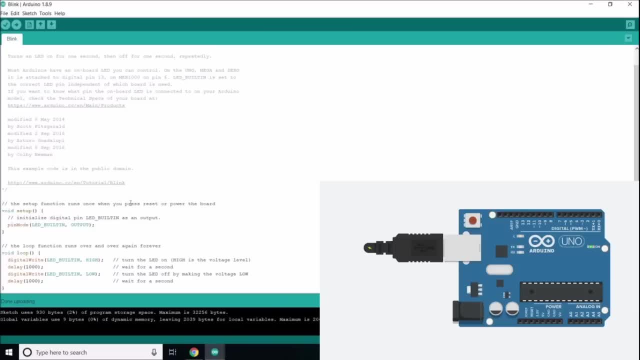 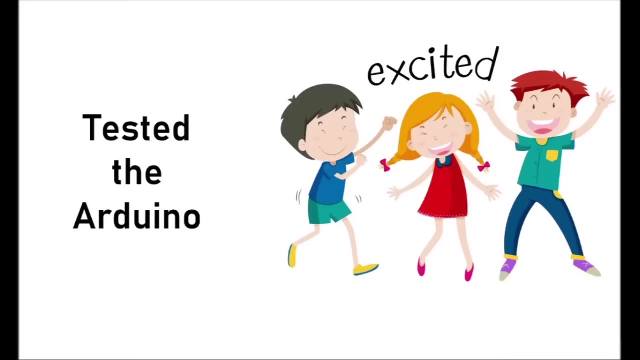 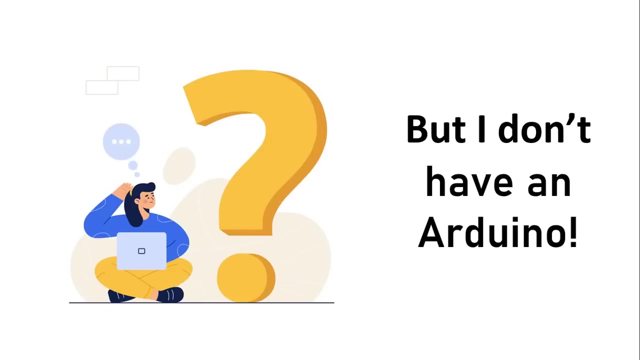 Done uploading right And you will see that LED is blinking with this gap of one second. Is it blinking Right? If it is blinking, then congratulations. You have done your first example. Thank you, paints. At this point the viewers without an Arduino must be feeling a little stuck, but please. 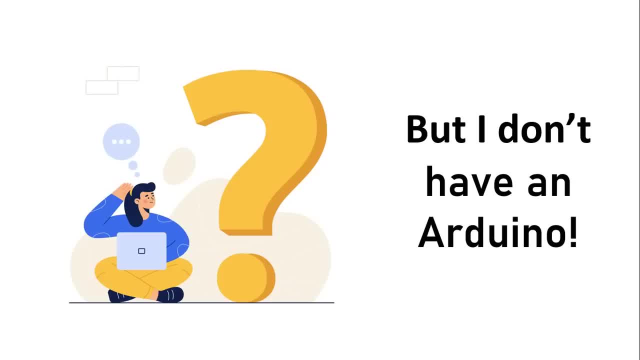 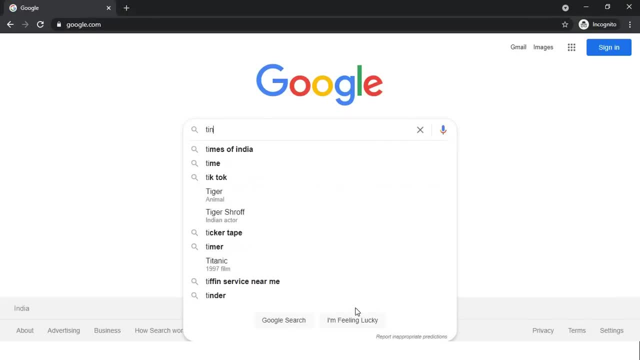 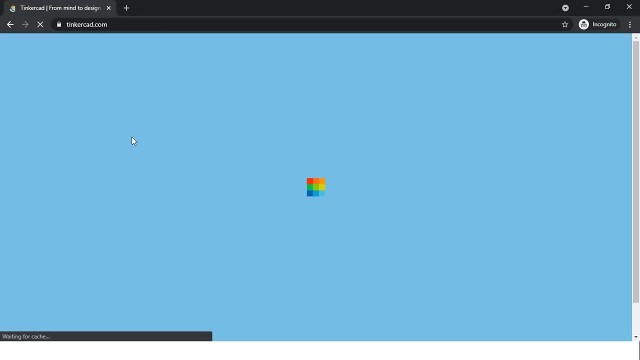 don't worry, I've got you covered. All you need to do is use an online simulator like Autodesk Tinkercad, and for that you need to go to the website of Tinkercad- right This one, And you need to create an account. 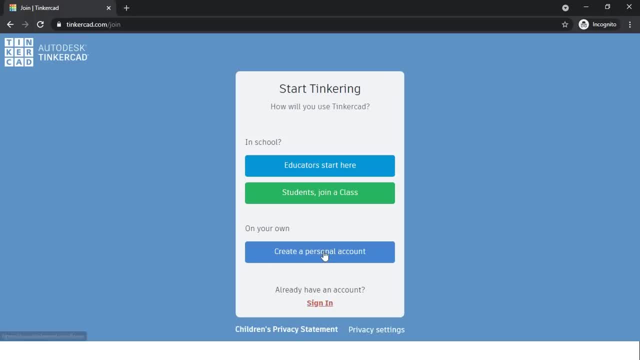 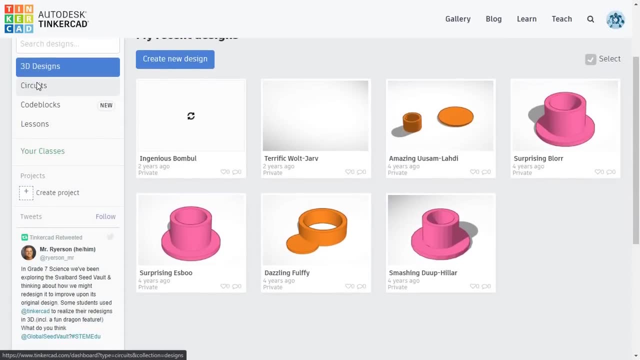 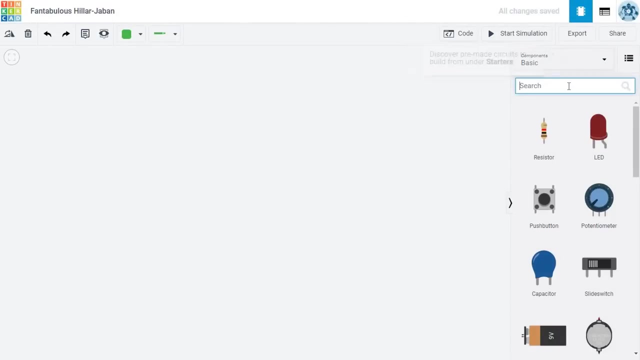 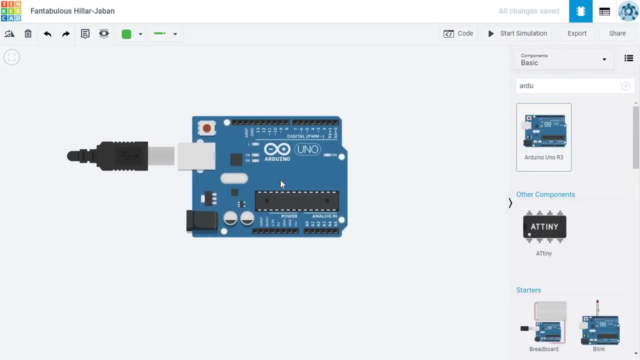 If you don't have it already, you can choose the option relevant to you, Make an account And after creating your account, you will see a screen like this. All you need to do is click on circuits and create a new circuit. At this window, you need to search Arduino Uno R3 and just drag it over here. 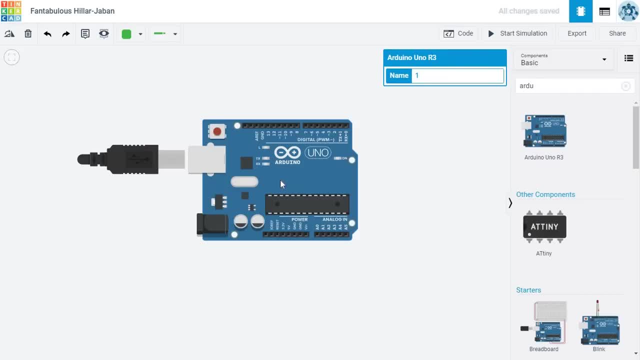 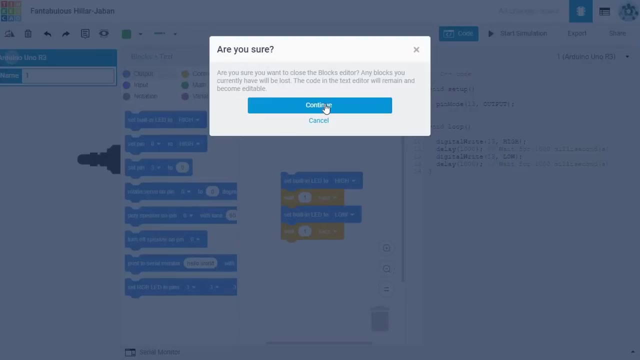 Right, So now you have your virtual Arduino board. It will just function exactly like the actual Arduino board, And whatever code I write in official ID in the following videos, you need to write that into this window, right? So you will have this window over here. 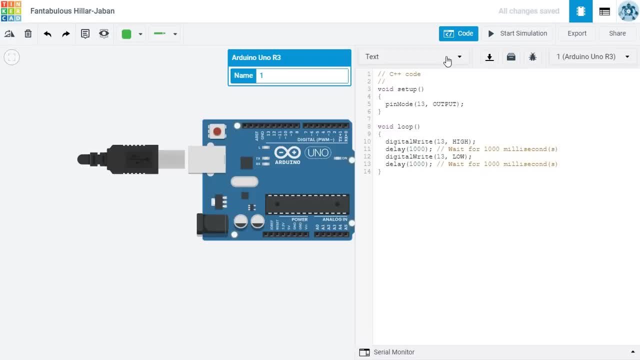 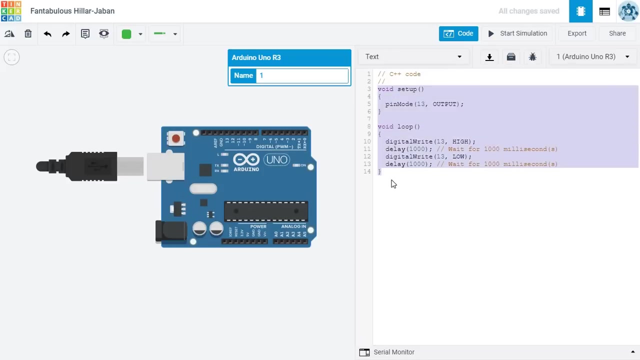 Whatever code I'm writing in the official ID, you just need to write that in this area. Okay, As you saw a few moments ago that we tested our Arduino board, So we will now test our Arduino board over here, right? So this is the same code which we wrote over there. 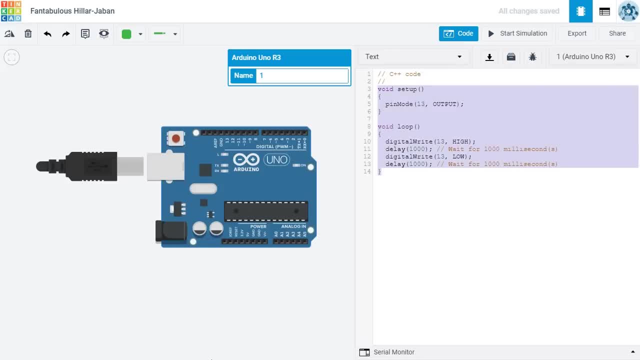 Only the comments are not here, right? So this is exactly the same code, And what we need to do after that is start simulation. okay, So it will be plugged in and you know. we can see the outcome of our code over here. 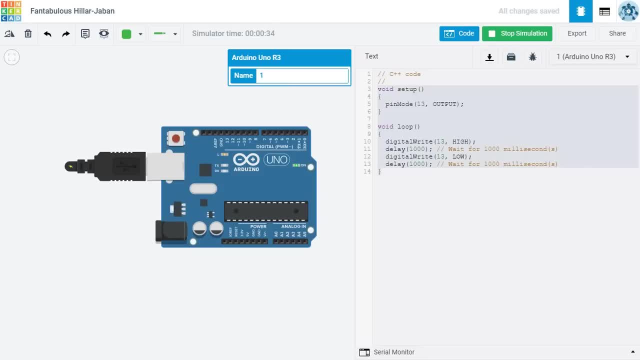 And in some portions of the video You will also see that I am printing out the outputs of some code on the serial monitor. So the serial monitor in this simulator is this right? So you will see whatever outputs I'm showing in the videos. you can see them here. 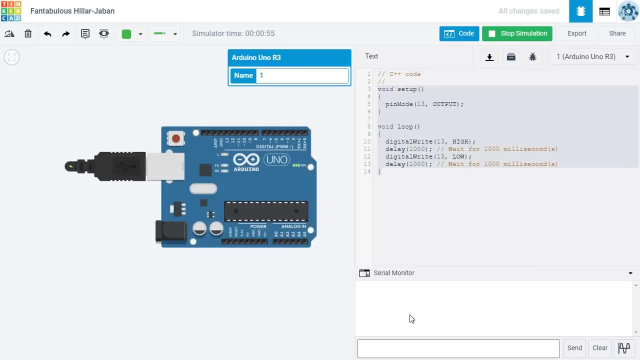 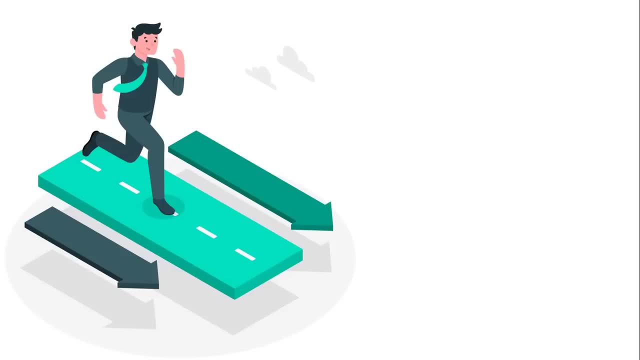 Okay, So don't worry if you don't have an Arduino at this point. you can still follow along the video. So, before we move forward from this point, having the knowledge of a few more things would be greatly beneficial, Things such as breadboard. 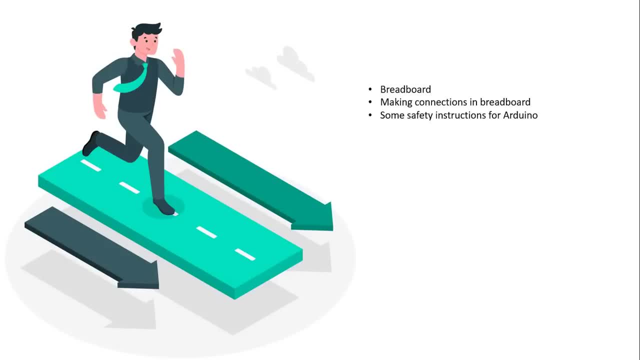 How to make connections in breadboard, Some safety instructions for the Arduino And some basic terms like input, output sensors, analog digital bit and byte. You may want to revisit this section as well if you find yourself forgetting about these. 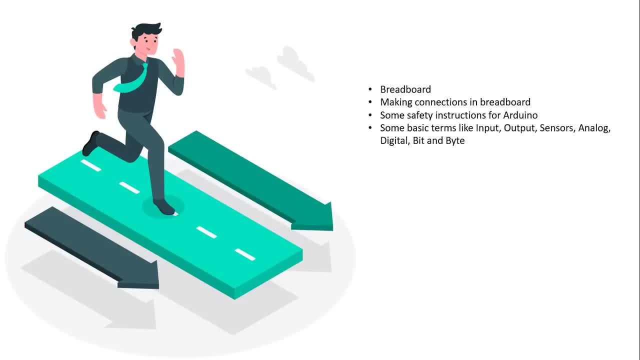 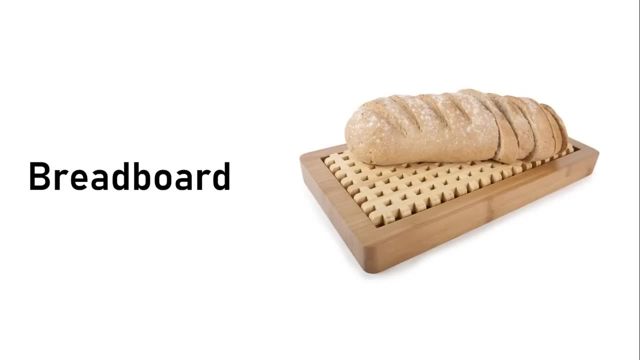 concepts as we proceed, All right, so let's start with breadboard. Is this the first thought which came to your mind when you heard of breadboard? Well, that's a perfectly genuine thought. When I stepped in the field of electronics, I myself had this thought. 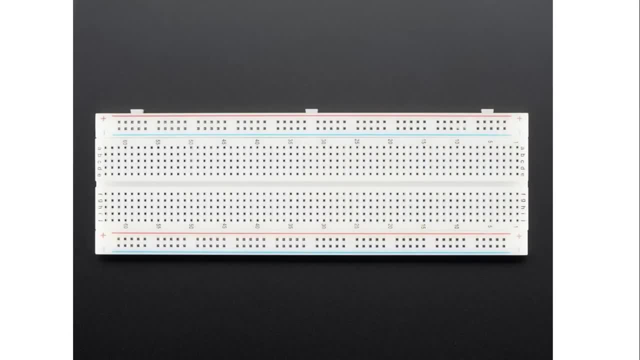 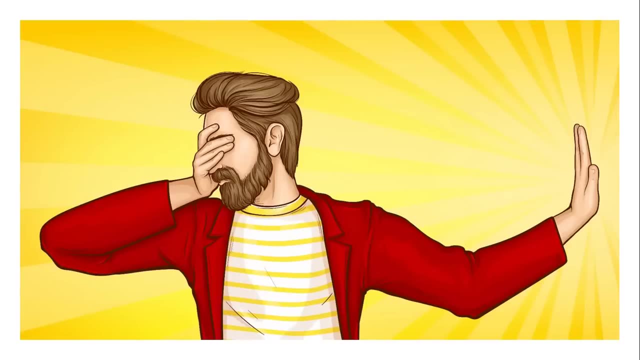 But when I learned that a breadboard in electronics is a completely different thing, I had a really big face-thumb moment. Let's discuss this in the comment section as to why it is called as breadboard or from where it got its name. We will just talk about breadboard in terms of electronics. 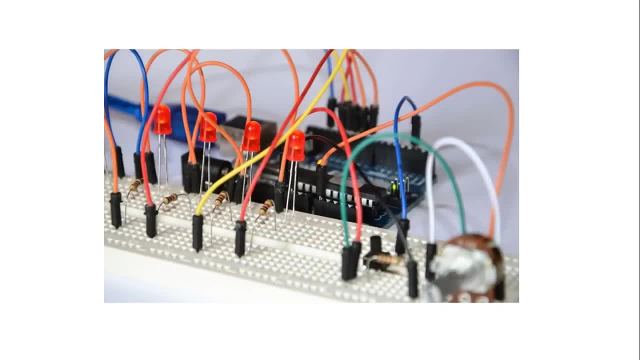 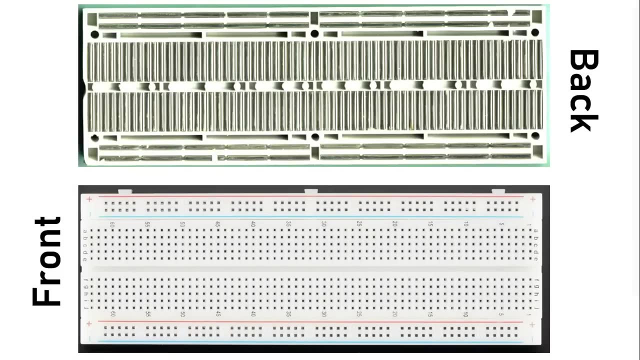 Breadboards are meant to make quick, non-permanent connections between electronic components, And they are covered with tiny socket holes Which are connected. in this way, The breadboard itself is broken into four sections. There are two inner sections full of short horizontal rows and two outer sections with 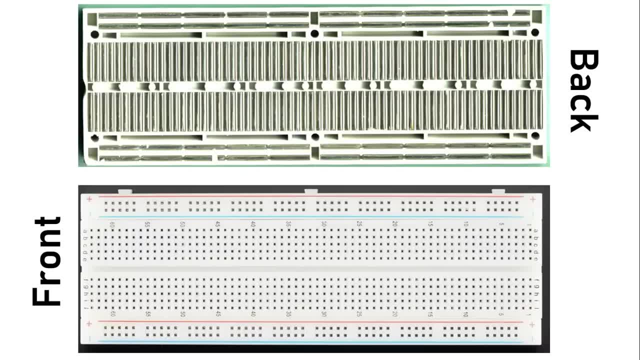 long vertical rows. If we remove the adhesive which is present on the back side of the breadboard, we would see something like this: A series of metal connections. Do you see that? We will discuss what this means in a few moments, But before that I would like to show you the strip which is connected to the breadboard. 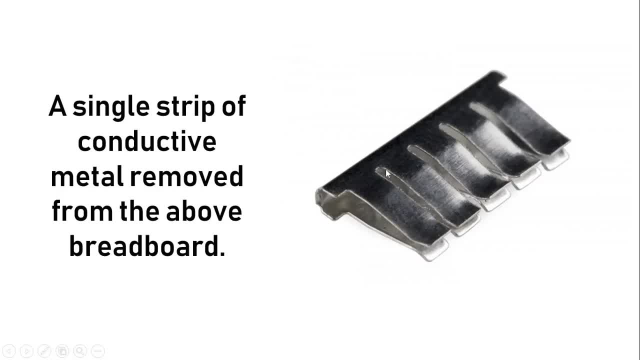 The strip which is connected to the breadboard. The strip which is connected to the breadboard, The strip of metal here It is a single strip which is taken out from that breadboard and it would look like that. You see this entire metal piece when we make a connection on that. it is internally connected. 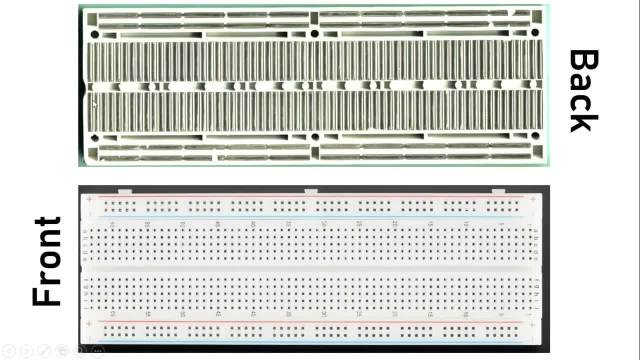 automatically. Coming back to this, if you consider, this row corresponds to this. Alright, That means that these points are connected among themselves automatically, and like these rails are connected, so these points are also connected from inside. we'll discuss this in detail. we'll also make circuits, don't worry about that. 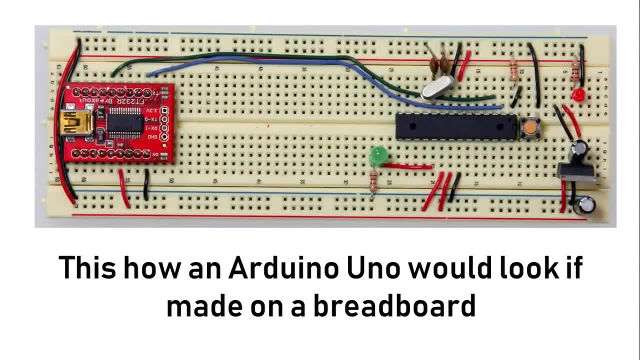 if you're wondering what kind of circuits which we can make on a breadboard, i would like to tell you that you can also make your arduino uno on the breadboard, and it would look like this. now we will see how to use a breadboard. we'll also understand the connections. 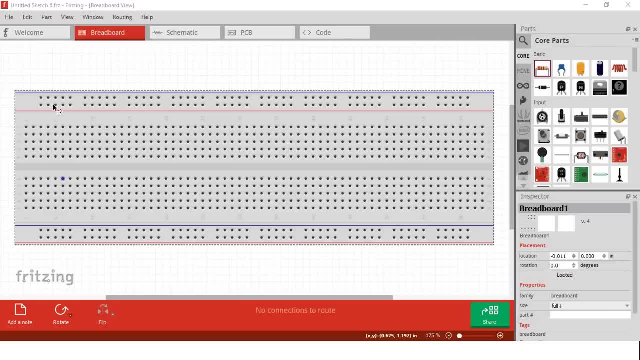 in details. all right, so this is our breadboard. okay, can you see all these holes like this which are getting highlighted in blue right? these are the holes which i was talking about in the previous video. okay, so i'll now show you how they are interconnected. for example, these points are: 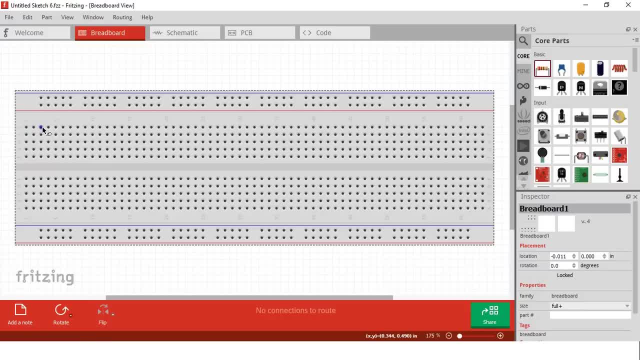 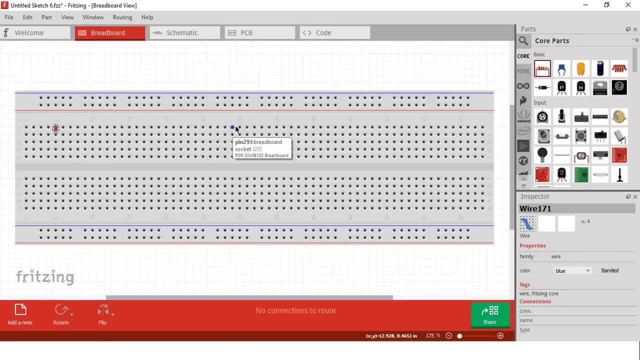 interconnected. the yellow ones, all of these are interconnected within themselves. right like these. all these points are connected among themselves. but please note that this point is not connected to this point internally. this point is only connected to these points like: can you see, right like this, all these points are interconnected, all right, so then we'll see these points. 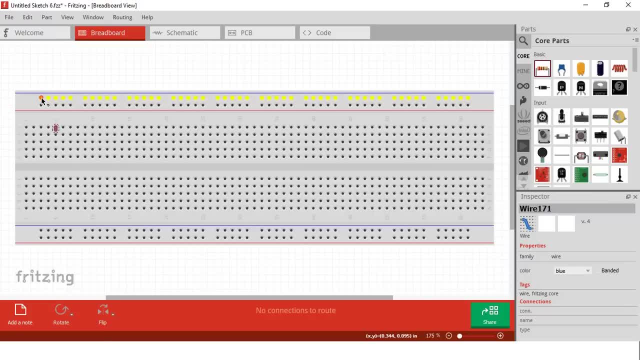 these are the external points. all of these points are interconnected like this, right, like this and like this, just like this. in some breadboards there are connection break at this point, so you will just see that the points are connected only till here and these points are connected till here, but this point is not connected to this point in some breadboards. 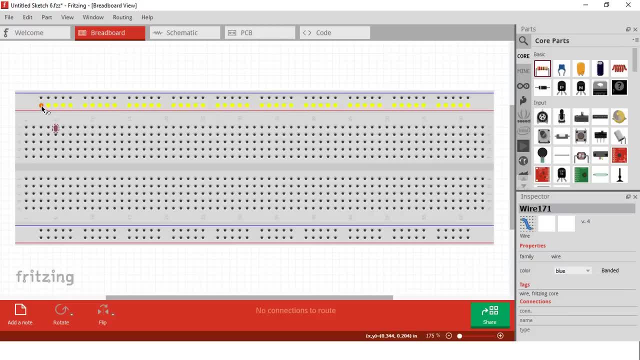 but in most breadboards they are all connected like this. can you see that? okay, so now i'll tell you: if we want to connect some two points, for example, we'll take a wire and we will take a thread, will join this. So now these points are connected among themselves, Right? No matter how many? 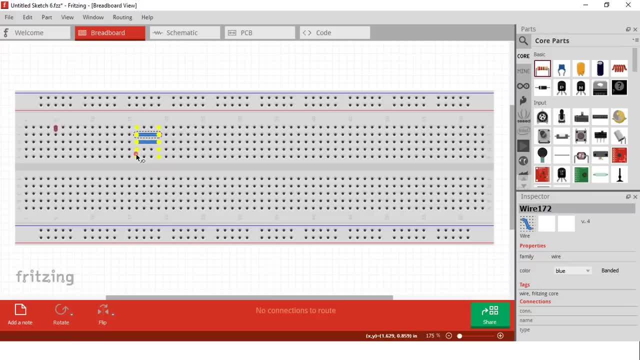 wires we join here, these will still stay connected. Okay, And what if I connect a wire here? Then all these points will get connected. You see that Right? I think it is really interesting to see that, how easy it makes for us to make connections on the bread board. 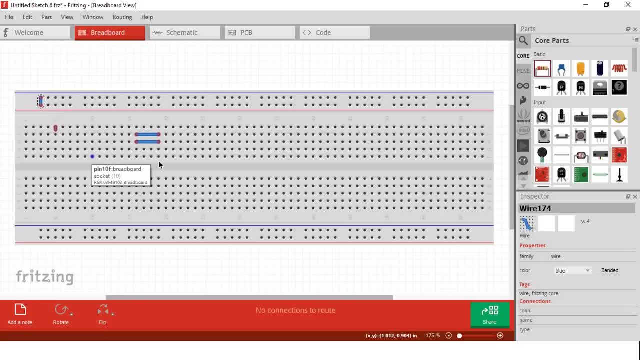 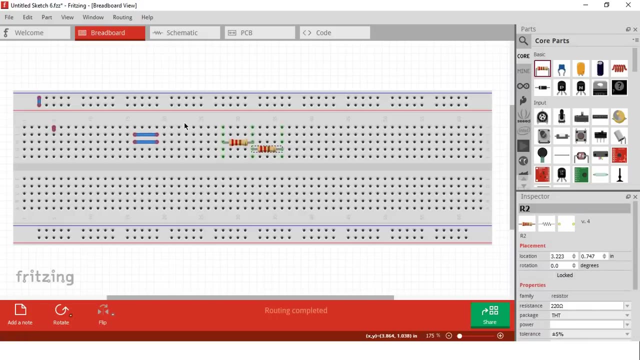 Right Now we'll see how to make a series connection right. We tell you the distance, like this, Okay, And we'll place it here. Okay, now I will take another resistance and connect it here, Okay, So now these resistances are in series. 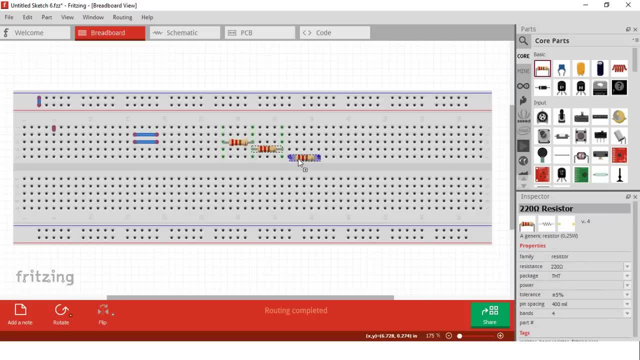 Now, if I make, want to make another resistance, which I want to make Catalie and the link, which one are connected here, Close, I want take in series. i'll place them here all right now. these three resistance are connected in series. how, for example, these points were interconnected okay, and so we connected our resistance here. so 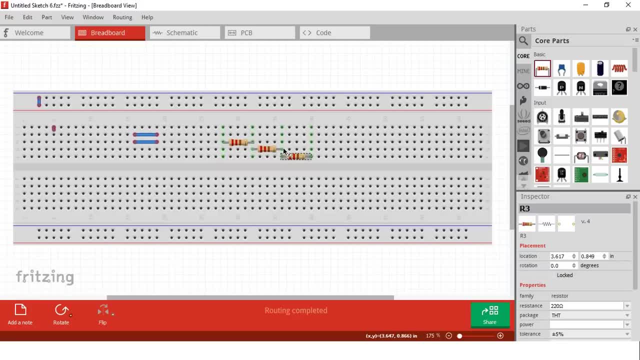 that means they are in a continuous position. now, similarly here as well. okay, i would like to tell you that some people make a mistake and to make a series connection, they would go like this: they will place the resistance here instead of placing it here. right, this is a series connection, but this is a no connection at all, because these points are not. 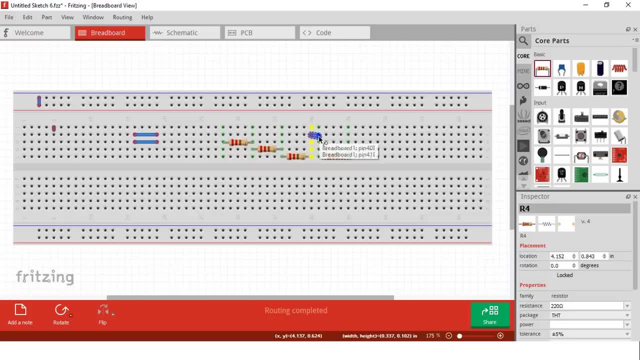 interconnected, however, if we join a wire like this. okay, so now these points are interconnected. okay, i hope i'm making you myself clear. now we'll try to understand a parallel connection. similarly, we'll take resistance and we'll place it here now, since in parallel connections all of 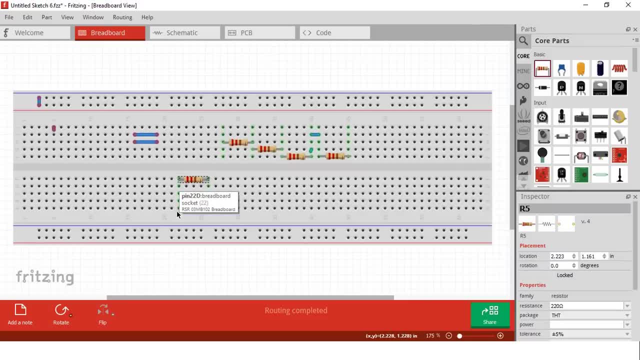 the points are, you know, originating and ending at the same point and these points are interconnected. so we'll take another resistance and place it here. so these two resistance are in parallel. now, if you want to take a third resistance as well, and we'll take it and place it here, now, these three resistances are in parallel. okay, now we 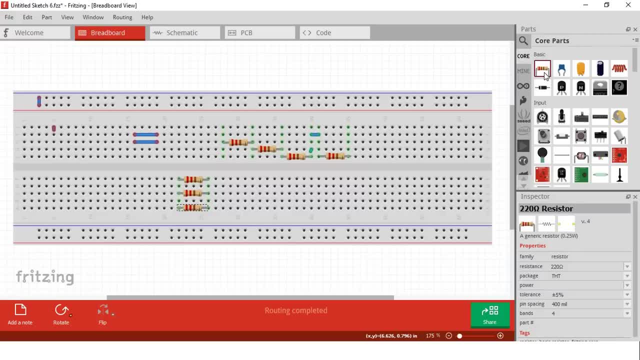 want to make a connection in which there is a resistance in series and then there are two resistances in parallel. we'll try to make that circuit. this is one resistance, okay, and then if we make it like this, like this, okay, and we take another resistance and we place it like this, okay. so what that is. 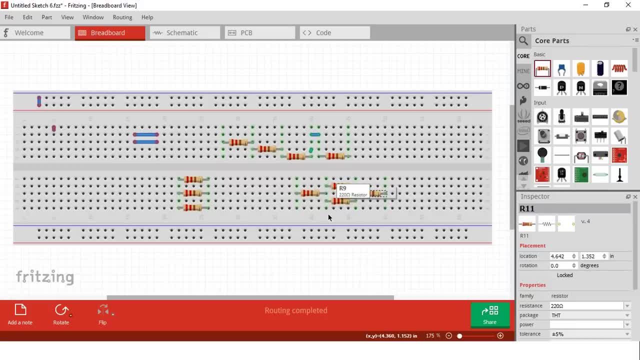 representing. it is one resistance which is in series with this, resistances which are in parallel among themselves, and then there's another resistance which is in series with that. okay, okay, it's all right. if you don't understand what i'm trying to say right now. we'll understand. 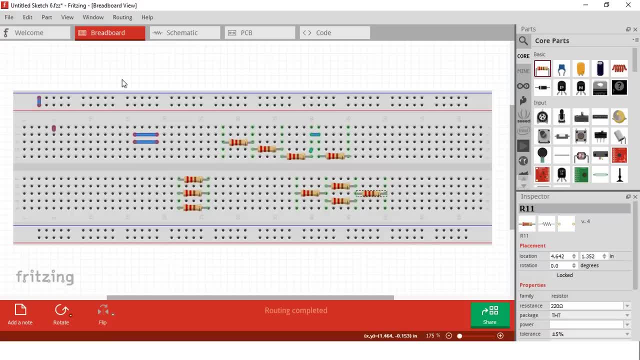 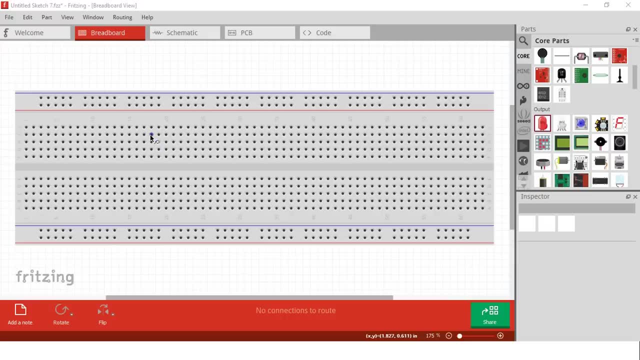 this with one more example. so before i begin with my second example, i would like to tell you a few more things. like i told you in the previous video, if we connect a wire like this, the points become interconnected. but if you take a resistance and connect it like this, 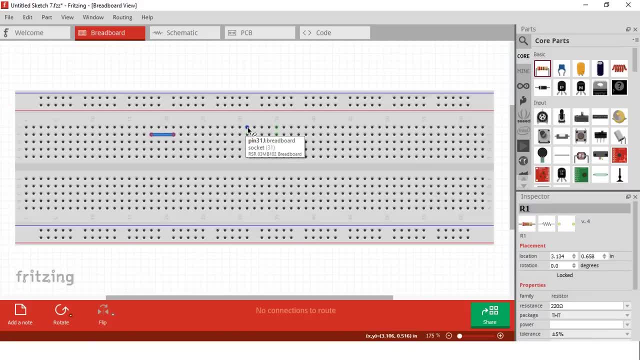 so these points are not connected to these points? right, because it is a resistance. you see that in this case these points are interconnected, but in the case of resistance, these points are not interconnected. now, another point which i want you to notice: if you connect a wire like this, it won't make any sense, as these points are already interconnected. 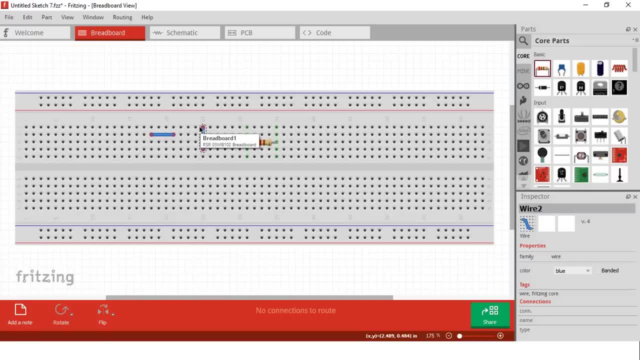 right, so this wire will not make any difference. so now another thing which i want you to notice: if you take a resistance and if you place it like this, like this, then also it won't make any difference because, as we all know, the current always takes the least resistive path. so connecting a resistance like this won't make any difference. 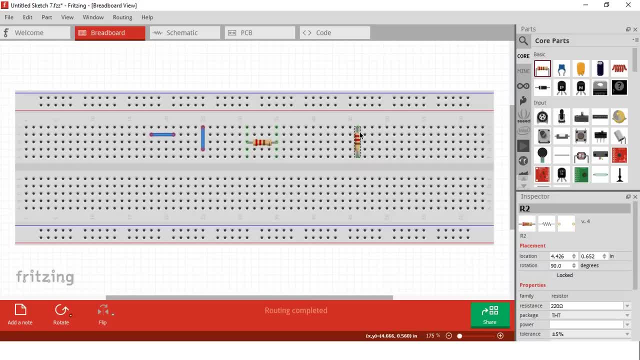 because the current will travel through the rails only. this resistance will not add any value to the circuit. okay, but however, if you connect a resistance like this, then it would make some sense. okay, how it will make some sense, we will see. for example, we can connect it like this: 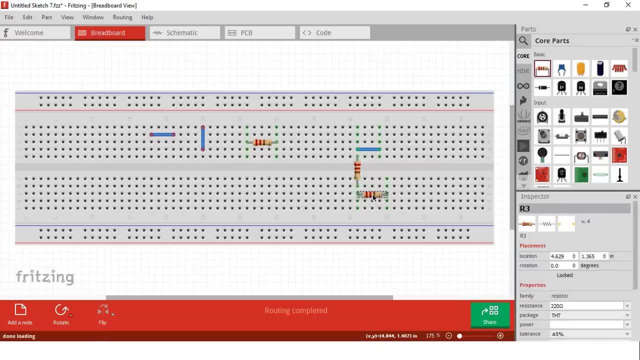 and like this. okay, so this is a series connection. these two resistances are in series, but, yeah, please note that these resistances are not in parallel. you can connect a resistance as such with a push button or a battery. okay, let's see how i can connect a resistance like this. 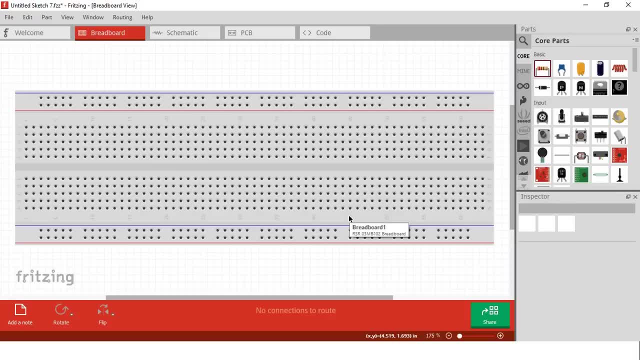 but please note that these resistances are not in parallel, because these points are not connected. okay, now we will begin with our second example. in this example, we will just connect an led with a push button and a battery. okay, so when we press the push button, that led will glow. okay, we will. 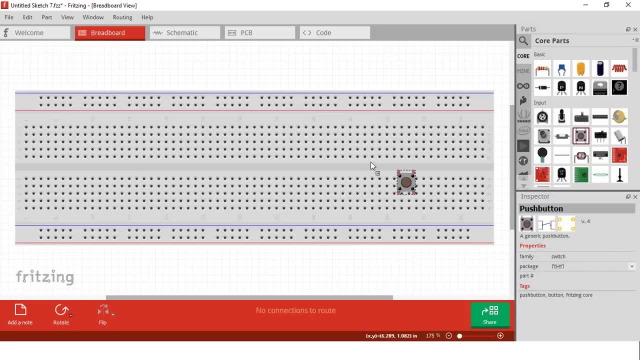 make a circuit on that. so for that we will take a push button and a battery and we are going to make a battery in these resistances, that we will take a push button circuit first of all. okay, this is a push button circuit. i'll tell you about push button circuit that internally this terminal is connected to this terminal. 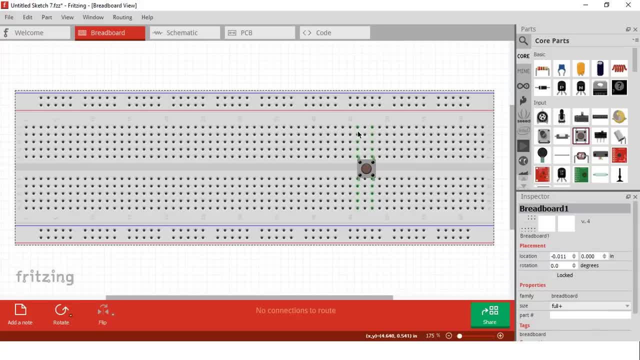 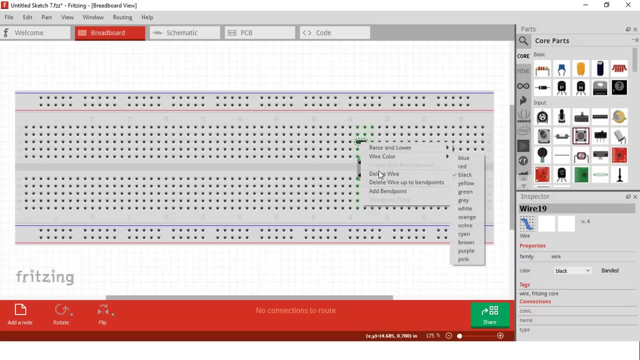 okay, so automatically this rail will get connected to this rail. okay, like this: and this terminal is connected to this terminal, so these points will also get interconnected. okay, so when you press this button, this terminal gets connected to this terminal. okay, so these points will get connected when you press the switch. 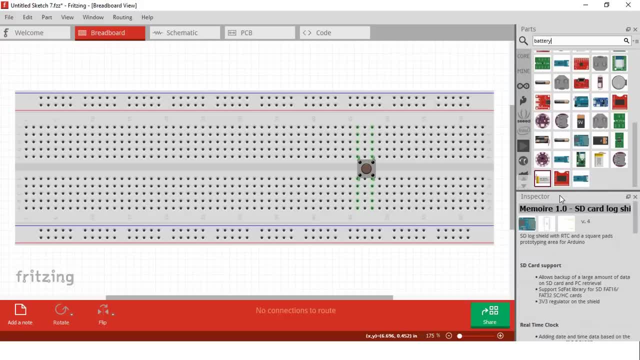 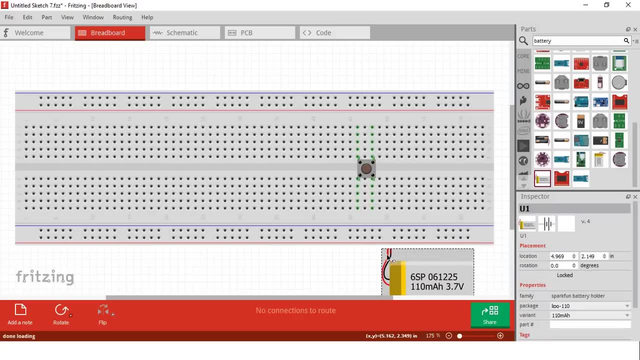 all right, then we will take a battery. let's take this battery. this is a simple battery, 3.7 volts. let's place it here. this has a positive terminal and a negative terminal. we'll try to connect it on a rail. okay, let's make this wire as red color and the black wire as 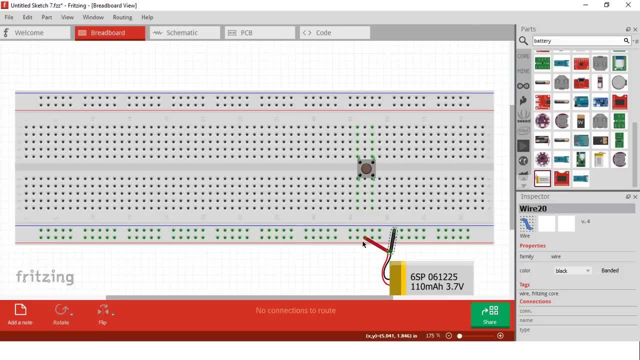 the black one. okay, in general electronics, this is also a convention that the red wire represents positive terminal and the black wire represents the negative terminal. okay, so now these and this entire rail. okay, so now this entire rail is connected to the black line. okay, so now this. 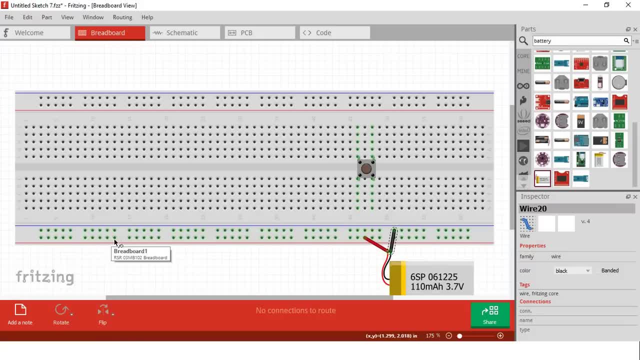 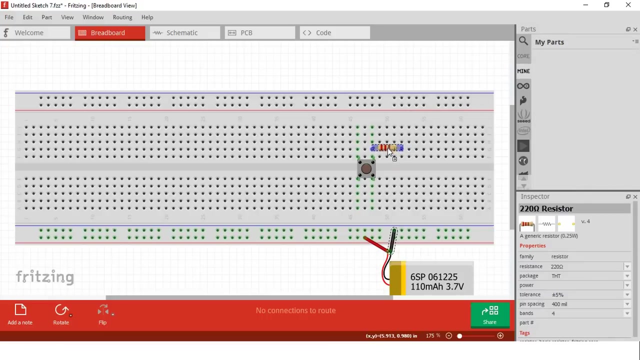 this entire rail is positive, okay, as we have connected the positive terminal of the battery here, just see that. and this terminal is negative. this entire rail is negative. okay, so we will start replacing a resistor, as we should always connect a resistance in series when using a LED. replace it like this, okay. so that means. 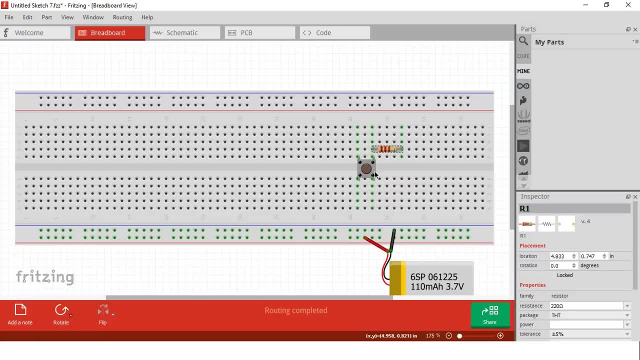 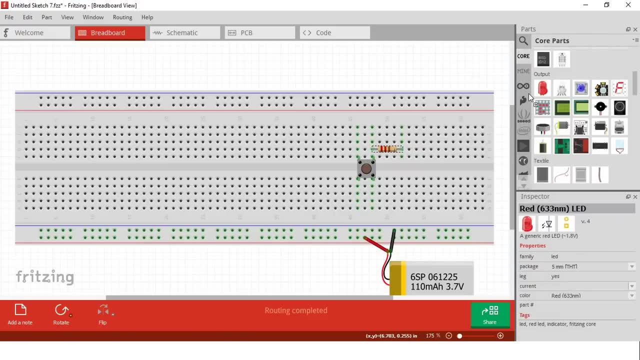 this point and this point are interconnected, so this resistance is in series with this switch, and then we will take one LED. this is the LED. okay, as we all know, there is a positive end and the negative end of the LED. okay, so this is the positive end and this is the negative end. we have connected the. 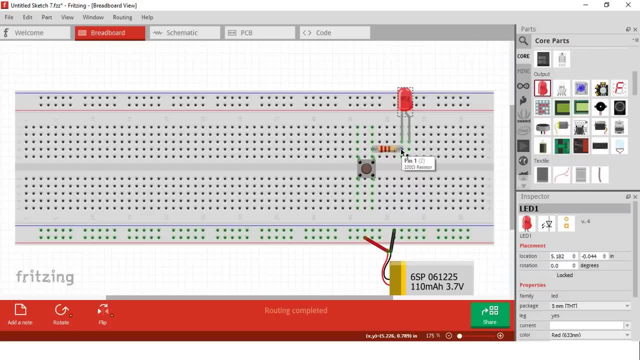 negative end to the resistance. okay, to make the LED glow, we have to always connect the positive end of the LED to the positive end of the battery. okay, so, first of all, what we'll do is we'll take a positive wire from here, right, as we know, although this entire rail is positive from any point on this rail, we 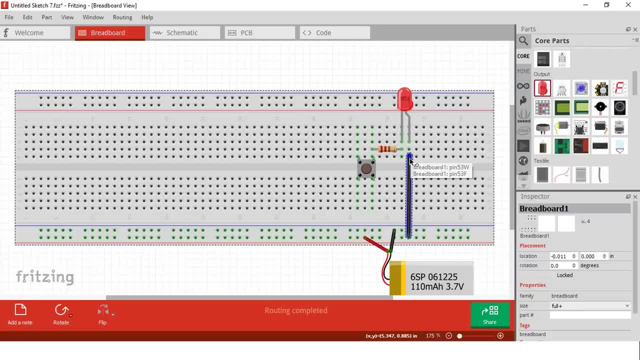 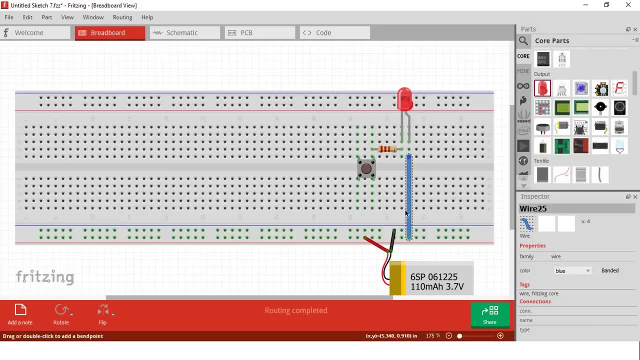 can take positive line. we will take a positive line from here and connect it here, okay, this is wish to the general wire, so we'll make it blue, alright. and then what we want is we need to complete the circuit like this: will take a black wire from here and connect it here, okay. so this is. 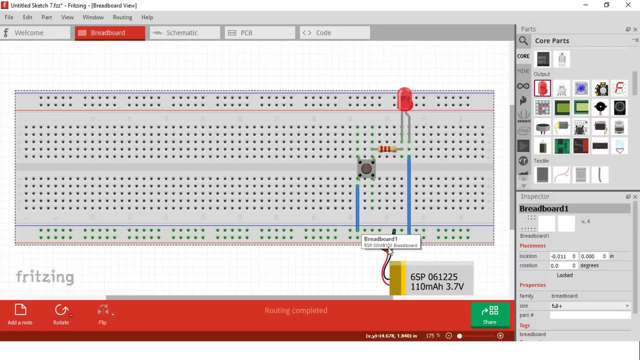 a circuit completed. whenever we press this switch, this circuit will get completed. the positive wire will go from here, the current will slowly switch and again the majority can get connected. if we click a couple of times now, if anything, is片 wire will go from here. the current will flow from positive terminal like this: 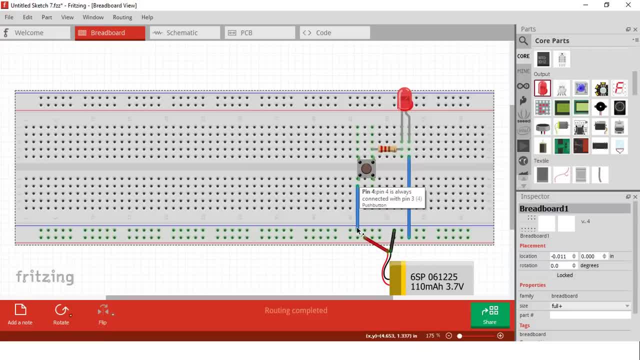 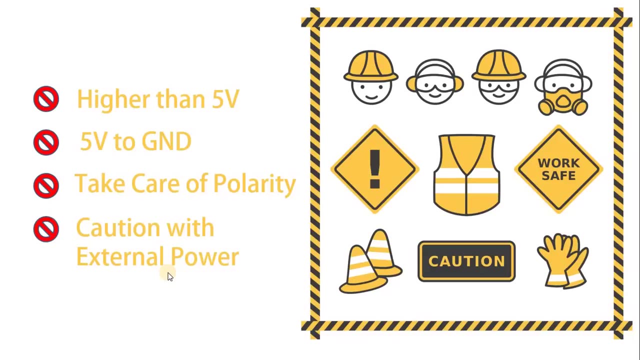 it will flow from resistance and it will go from circuit and then to the negative end, back to the battery. But whenever we release the switch the circuit will break and the LED will stop glowing. This was the very basic example of a LED in a breadboard. In this video we will discuss about some of the safety instructions. 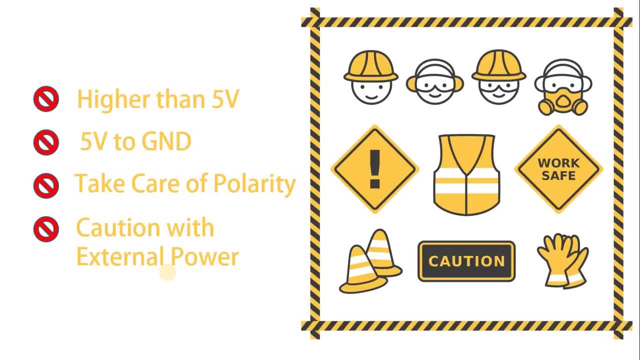 Which we need to follow while using our Arduino board. the first thing which you need to keep in your mind is you never have To connect any voltage of over 5 volts on any IO pin. Okay, any IO pin means any input output pin, be it the digital pins or the analog pins. 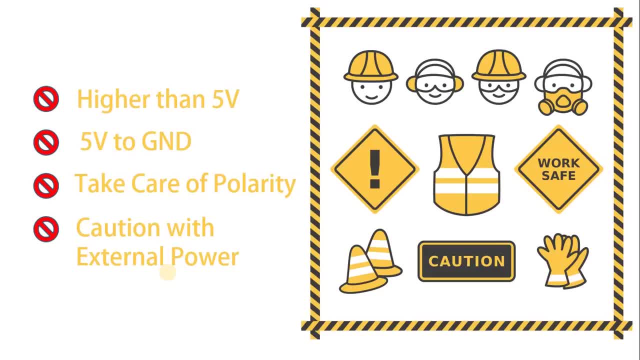 You just don't have to connect any voltage over 5 volts on those pins. you can only use any voltage over 5 volts to power the Arduino through VIN pin, and You cannot connect any pin to a voltage over 5 volts. Okay, next, The next important thing you need to notice. 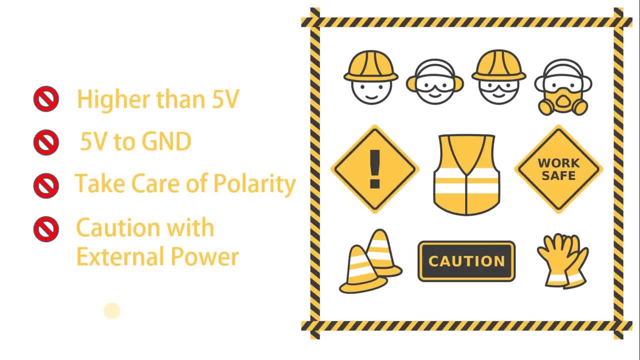 You never have to connect a 5-volt pin to a ground pin. This way you will short it down and Arduino will turn off. The next point is you have to take care of the polarity. Polarity means you cannot connect positive and negative terminals in opposite ways. 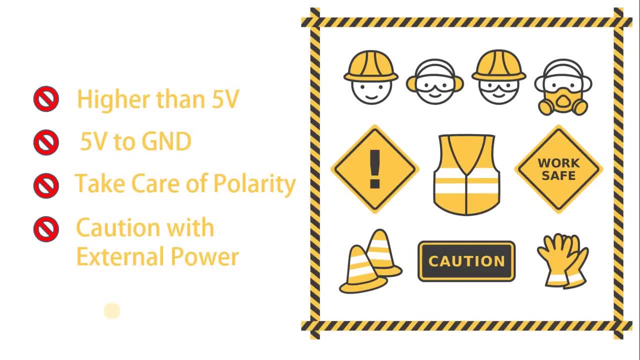 What I mean is you cannot connect a positive pin to a negative pin of some other component and vice-versa. If there is no polarity management circuit on the device which you are using, it will simply damage the device. one more point else: You have to Be careful while using external power in this course. for all the project, the USB power would be more than enough. 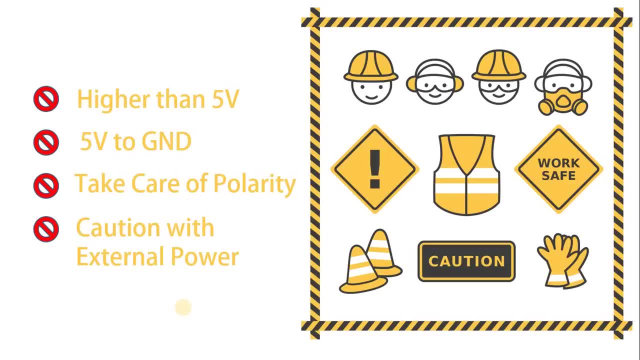 But still, if you need any external power, you can use it through DC jack or VIN pins, And in that case also, please make sure you don't connect any voltage above 12 volts, Although Arduino can tolerate up to 20 volts, but still I advise you that don't use above 12 volts. 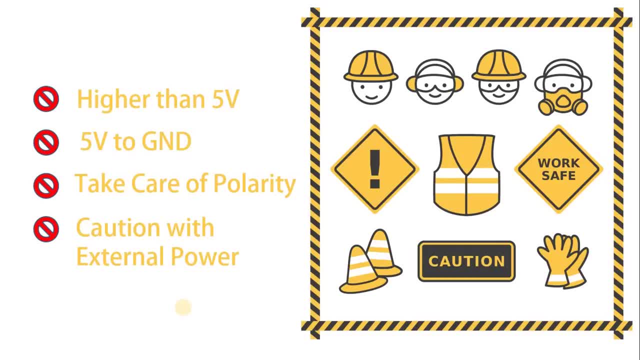 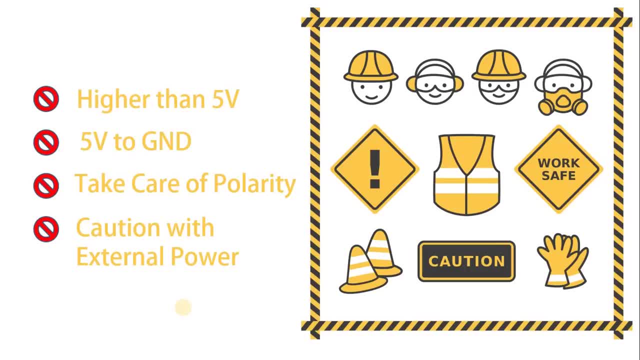 Or you may need to follow the safety instructions, Or you may need to follow the safety instructions And, while doing our experiments, I will also tell you about more safety instructions, if they are required. Okay, so now I will see you in the next video, in this video. 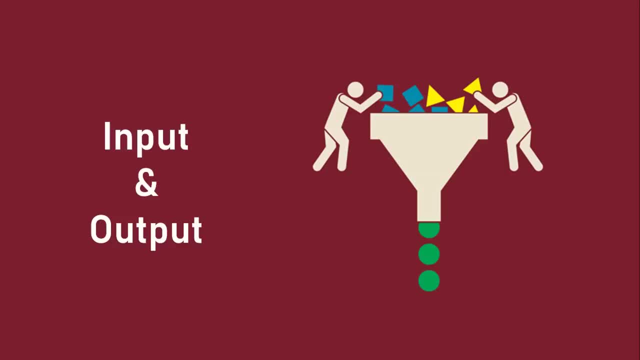 I will talk about input and output and how to understand it with respect to Arduino. You may want to revisit this video. when we study pin mode function, It has been taught in Arduino programming section. so, generally speaking, input is something which goes inside and An output is something which comes outside. 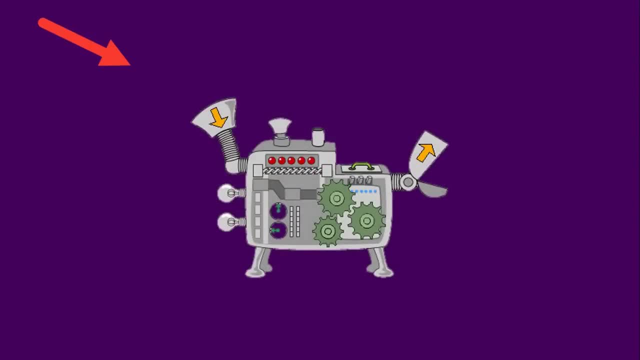 An output is something which comes outside. Speaking technically, input is some data or signal which goes into the system and output is some processed information or signal which comes out of that system. The system may be anything Like. in our case, the system would mostly be Arduino. 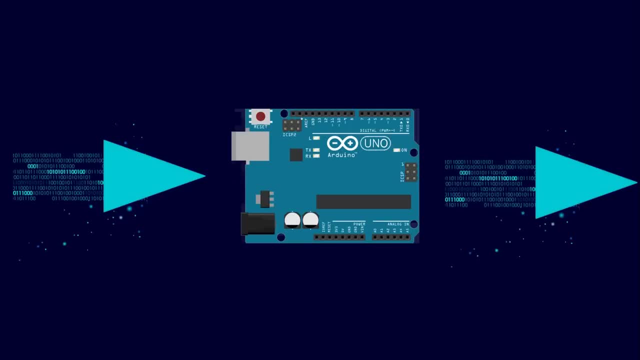 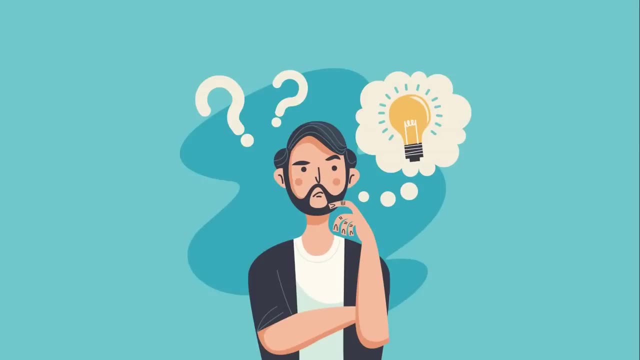 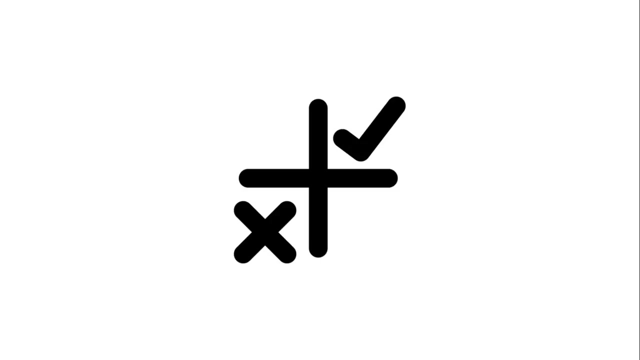 The sensors would be giving the data to the Arduino and Arduino would act on that data and give an output based on how you have programmed it. Please bear in mind that input and output is never absolute. It is always relative to something. As you may have been told in junior classes that input and output devices are fixed. 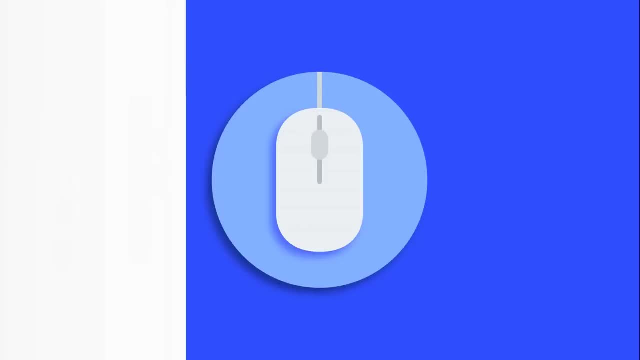 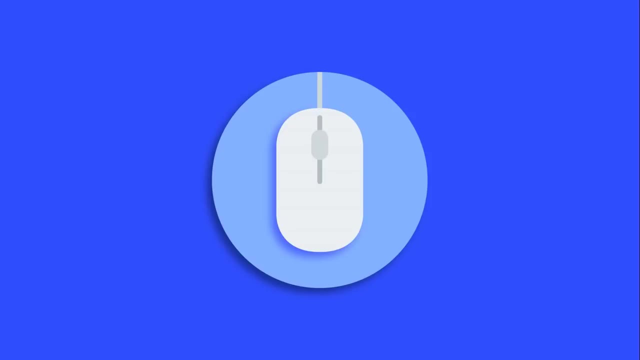 Yes, they are fixed, but with reference to the computer. Like a mouse is an input device to the computer, but if we look in the mouse itself, there would be several more devices, like an optical reader which takes the movement of the mouse as input and gives its output to the chip inside which processes it and gives the cursor. 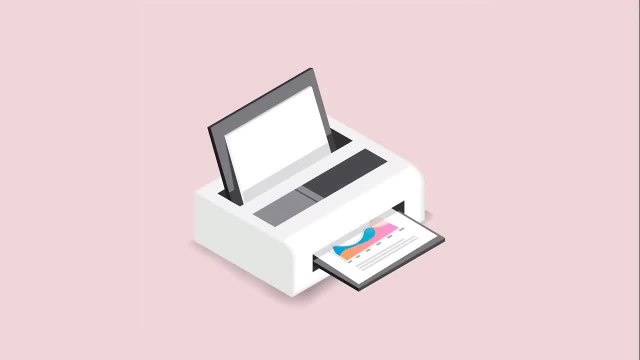 position as output. Similarly, we have been told that a printer is an output device. Yes, it is certainly an output device, but with reference to the computer. Now, if we see, in a printer as well, there is a main controller board which takes the 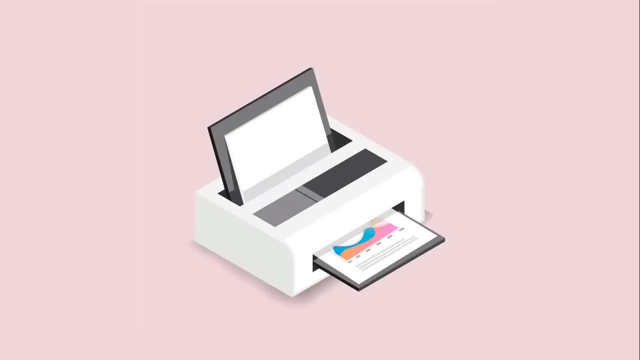 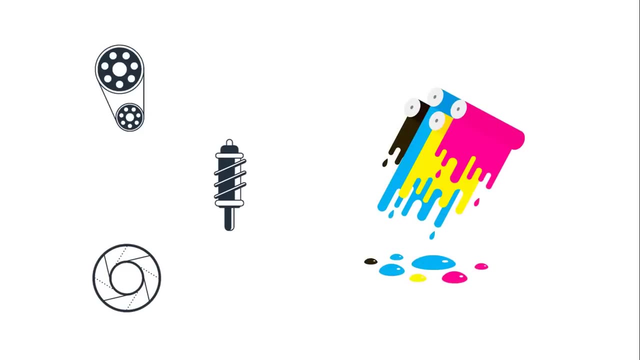 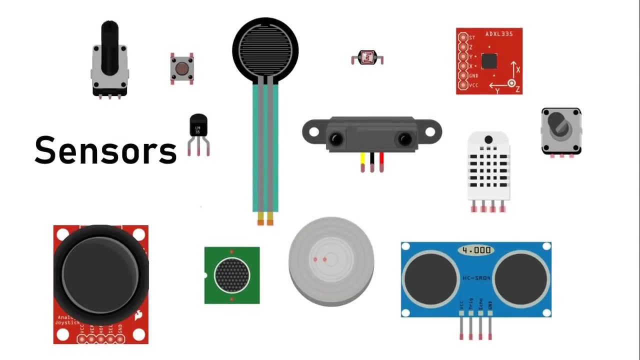 input signal which is coming out from the computer and then that controller takes the decision that how to move the motors, which colors to select in order to print the page. I hope I am making some sense to you Now. if we see in reference to our course, there are lot many things and sensors. 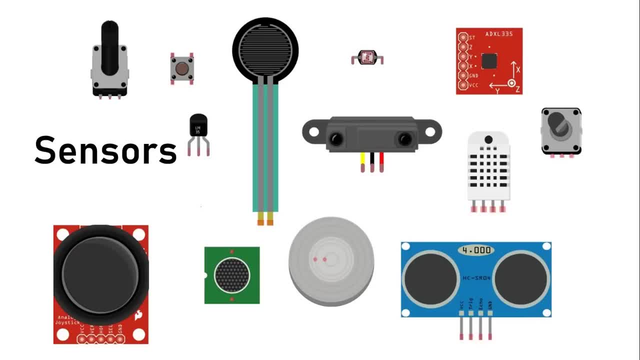 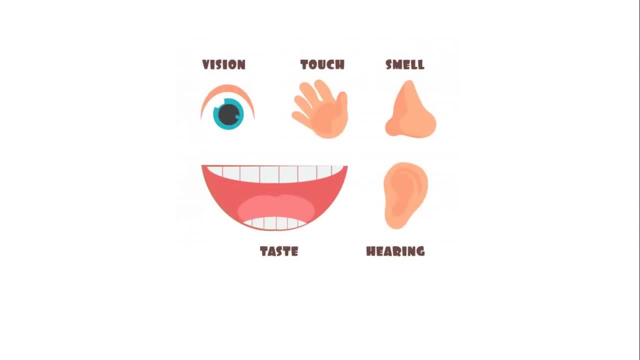 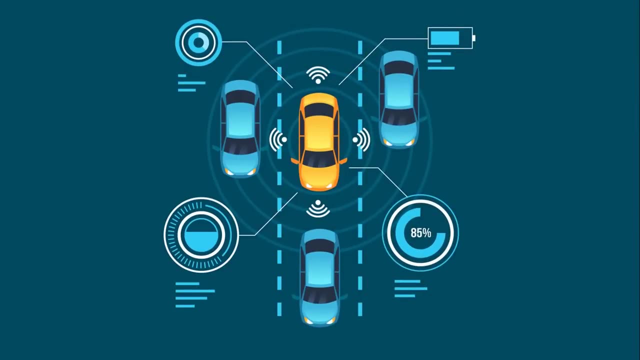 There are sensors which act as input devices for the Arduino, like these sensors which you can see on the screen. But wait, what are sensors? Like humans, have 5 sensors which help us get aware of our surroundings and act accordingly. Similarly, in electronics, sensors help the controller to take decisions and give output. 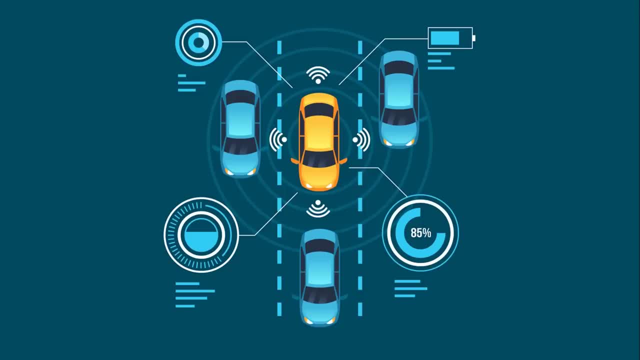 based on the environmental data which is given by them. Sensors tell something to the controller by changing its voltage. The change in voltage is read by the controller. Like we see in this image, There is an autonomous car which has n number of sensors placed on it which are telling. 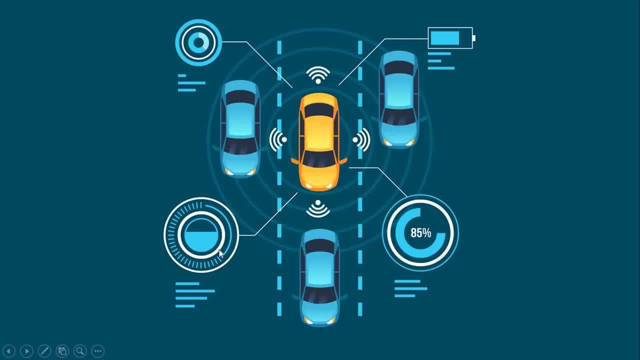 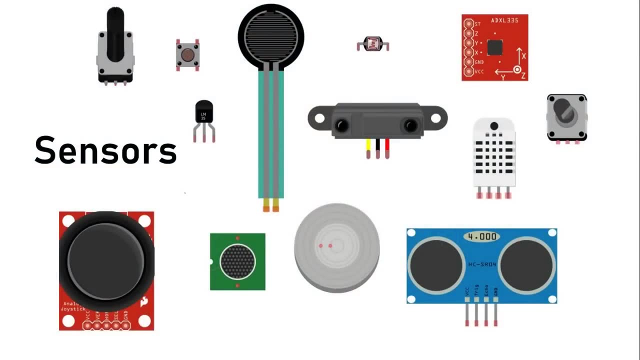 it about the other cars: battery level, fuel level, humidity level, etc. Now I will briefly discuss about these sensors which you see on the screen. We will also discuss these sensors in detail. when we use these particular sensors? First of all we see is a Rotatory potentiometer. 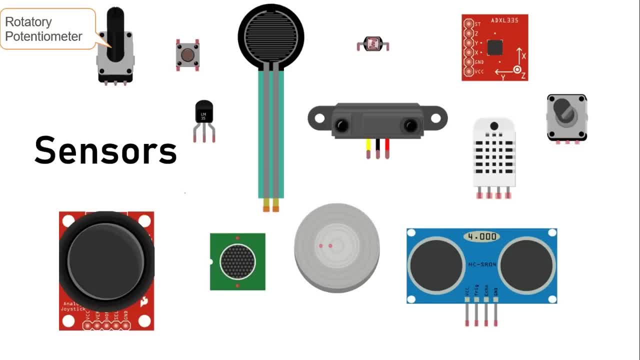 This device would change the resistance it offers. if we rotate the knob clockwise or anticlockwise, Then we have a Momentary push button. When we press this switch, it will close the circuit. When we release the switch, it will open the circuit. 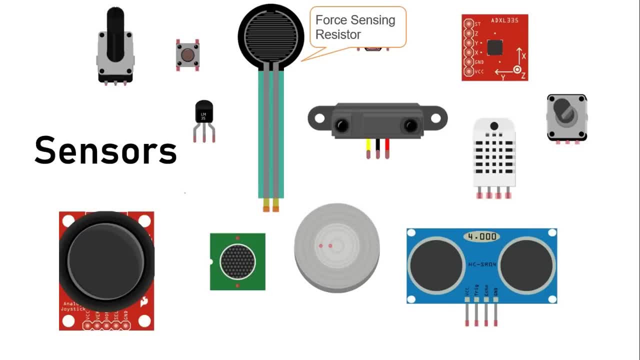 Then we have a Force sensing resistor. This resistor changes its resistance based on the force applied on it. Then we have a Light dependent resistor. This resistance changes its resistance based on the light falling on it. Then we have a Triple axis accelerometer. Usually we see accelerometers in phones and gaming devices. 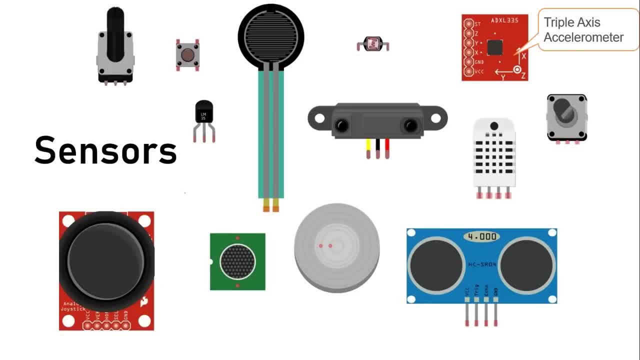 Okay, What does this tell us? what kind of position is the object placed on? We have a Joystick. A joystick is nothing but a basic input controller. You must have seen it on the gaming consoles. Then we have a microphone or a sound sensor. 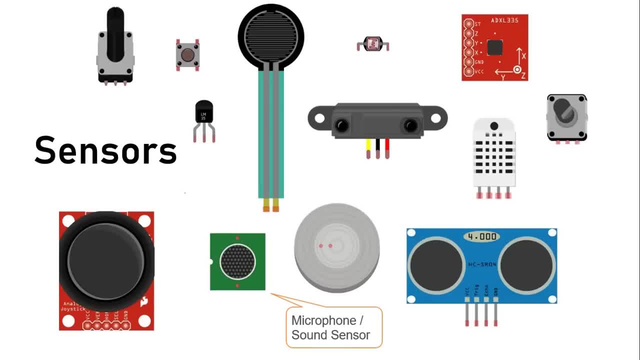 It will capture the environmental sounds and noises. We may want to record them or take some decisions based on that. Then we have a touch sensor. It will just see if someone is touching it or not. Then we have a Rotary encoder. Now you might wonder what is a rotary encoder? 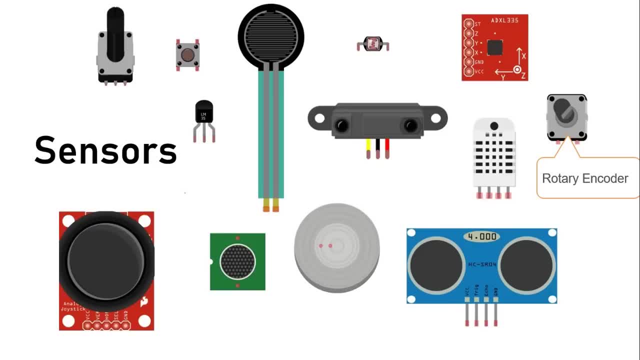 sensor senses the rotation basically, for example, you can attach this rotary encoder to a motor sharp and we can see the rotational speed of that motor, how many rotations it have taken. you must have seen a rotary encoder in a volume knobs in your music systems. then we have an 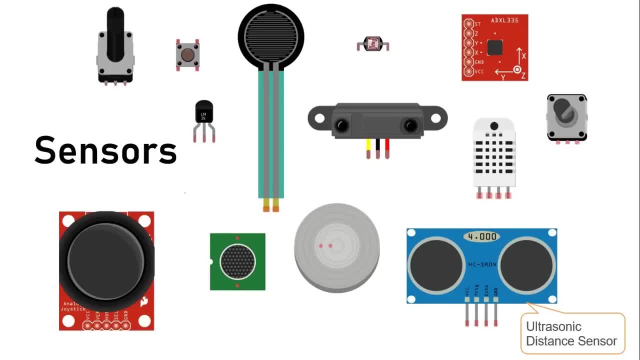 ultrasonic distance sensor. it uses ultrasonic waves, like in a sonar, to tell the distance between the sensor and the object in front of it. then we have a temperature sensor. as the name suggests, it will tell the temperature around it. we have a temperature and humidity sensor: it tells. 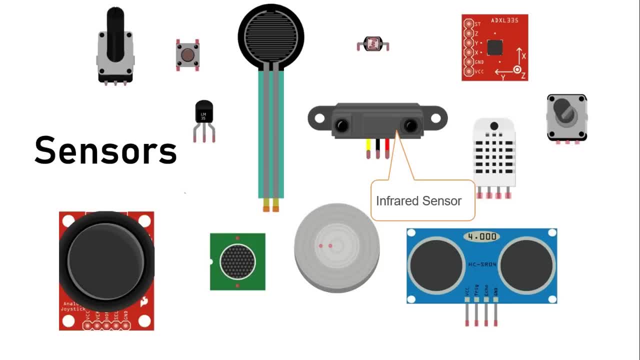 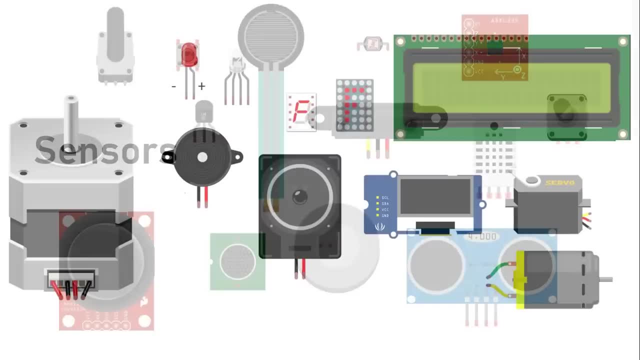 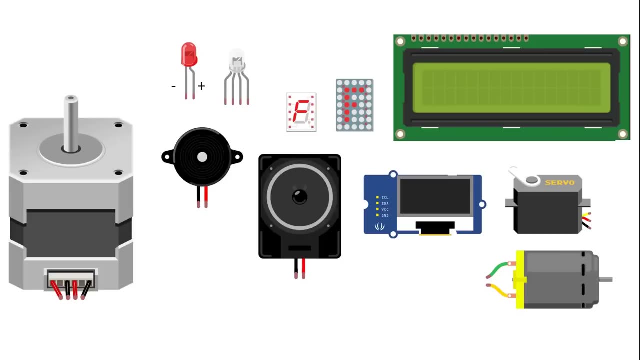 humidity as well, along with the temperature. then we have an infrared sensor. this is basically an obstacle detection sensor. it can tell if an object is there in front of it or not. then we also have output devices. output devices are those devices that can convert the output given by the ardeno to some human readable form. right, for example, i'll tell you there is an. 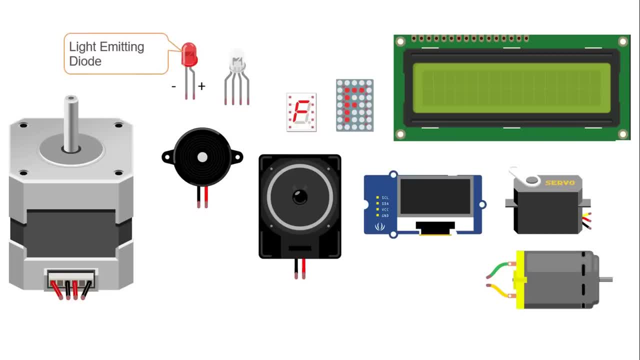 led, which is known as light emitting diode. it will basically just glow if any pin on ardeno is set to high and we have an rgb led. this is a special led. it has all the colors: are red, green and blue leds and it can form any number of colors. and we have a buzzer. it will make some sound if high voltage. 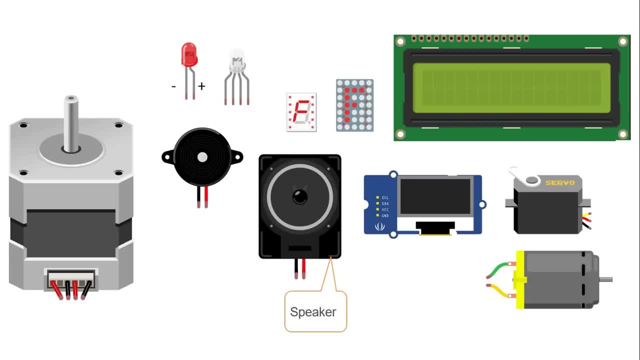 is given to it, it will make some sound. then we have a loudspeaker, like it is general speaker, which you have seen in your mobiles and your laptops, which you know you play music through. we have an oled display. it is a full fledged display. you can display graphics on it. we have 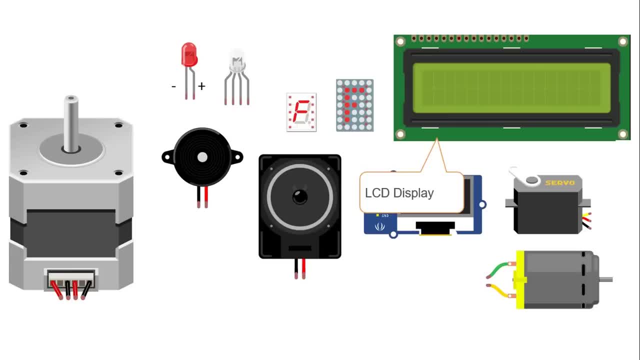 lcd display. this is liquid crystal display. you can display characters on it, okay, for example some value of a sensor or someone's name, etc. the seven segment display consists of seven leds arranged in a rectangular fashion, as shown. it is used to display numbers on it. for example, if we 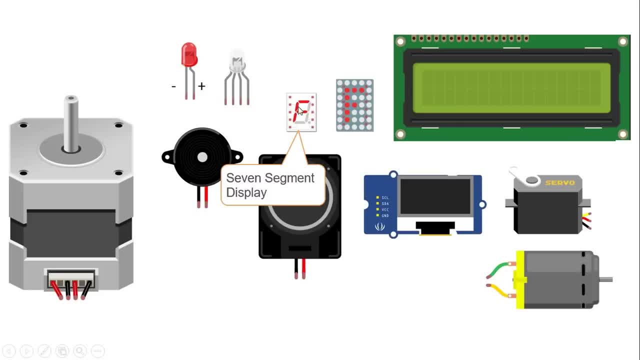 want to display seven, so we will highlight this one, this one and this one. so we will see that if we show zero, then we will highlight these ones. okay, and if you want to display eight, we will highlight all of them and it will look like it is coming on and we have a dot matrix display, dot. 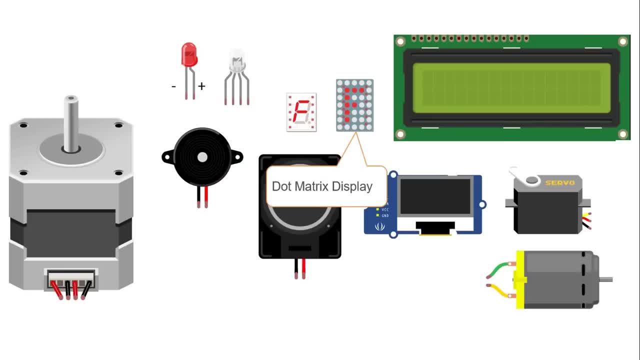 matrix display is an array of multiple leds. okay, we can show even characters on it. you must have seen a dot matrix display in delhi, metro display, or even, you know, scrolling displays. you must have seen in front of some shops which display the shop's name. so that is a dot matrix display then. 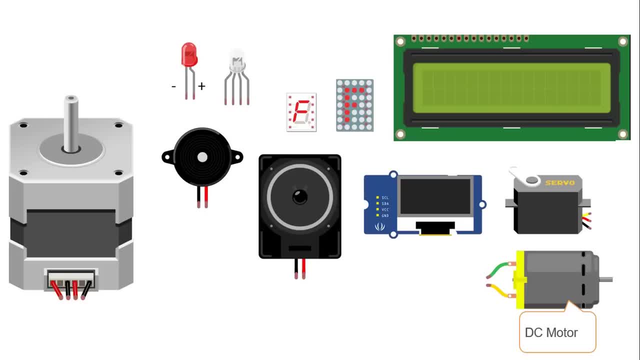 we have a dc motor. it basically moves clockwise or anti-clockwise if it is given some voltage across it. then we have server motor. so this is a special kind of motor. we can stop it at specific angles. then we have a stepper motor. a stepper motor is just like a dc motor. 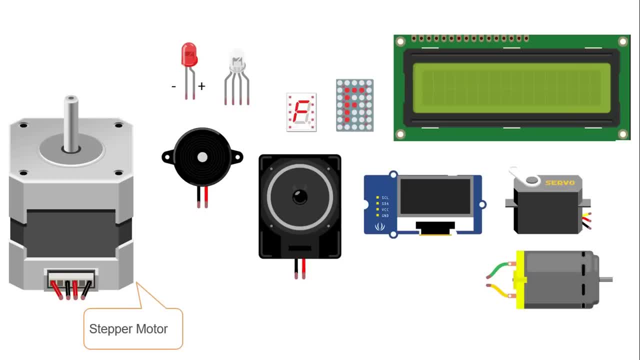 but you know, the entire rotation is divided into equal steps. so, like server motor, we can also stop it at specific angles and even lift heavier loads. we can drive heavier loads using a stepper motor. so to conclude this video, i would like to say, since we know about input: 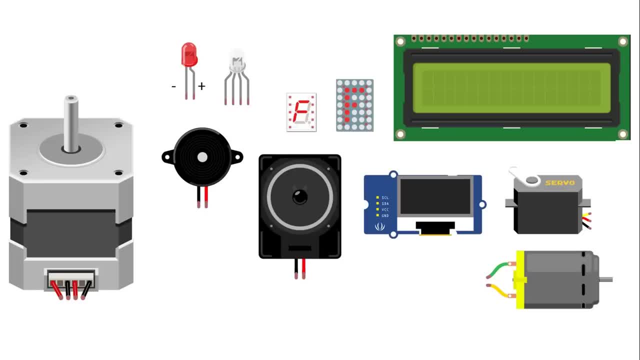 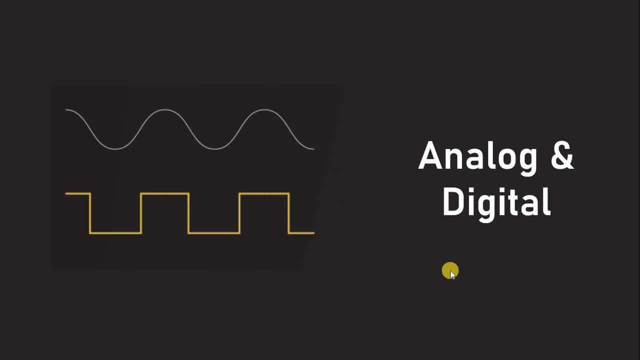 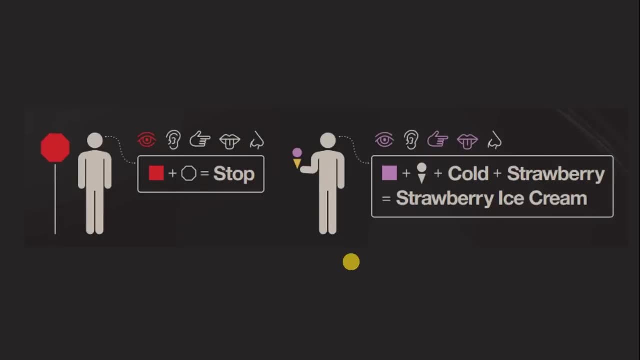 output properly. now we can easily understand how arduino interacts with the environment and we can make some meaningful projects after knowing this. see you in the next video. in this video, we will talk about analog and digital. so to begin with, i would like to tell you that our world is full of analog information, like the colors we see, fragrances, we smell, flavors. 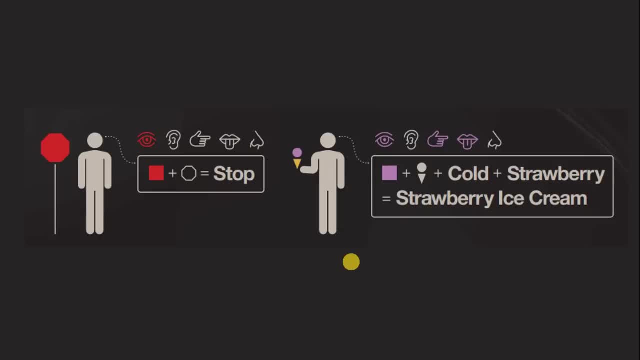 we taste sounds, we hear temperature, we feel- all these have just endless number of values. there can be millions of colors, smells, flavors, sounds, etc. this was in a very general sense. now, if we see in the terms of electronics, something which is analog can have infinite number of values. let's say, your wall clock, it can show. 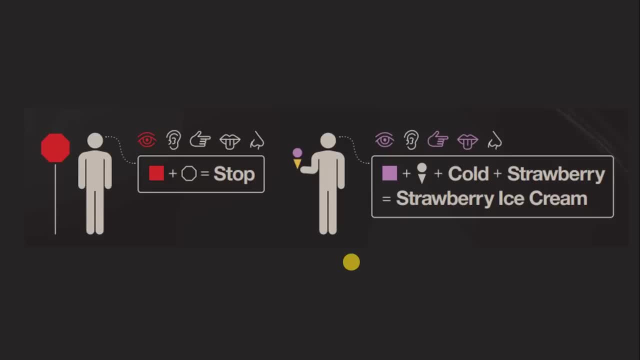 endless number of time intervals, though they are not marked on it, but yet it holds the capability to tell you even smaller fractions of time, while digitally something with discrete or limited number of values, like a digital clock, that clock can show you limited number of digits. let's say: 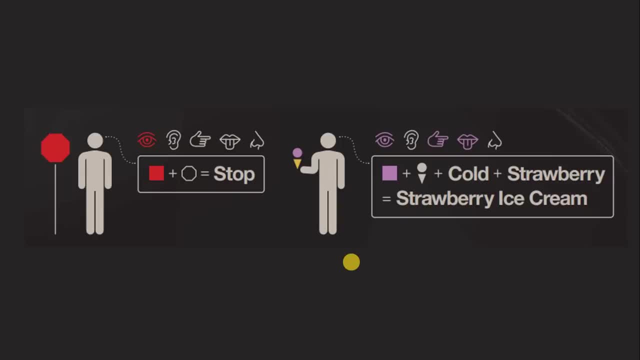 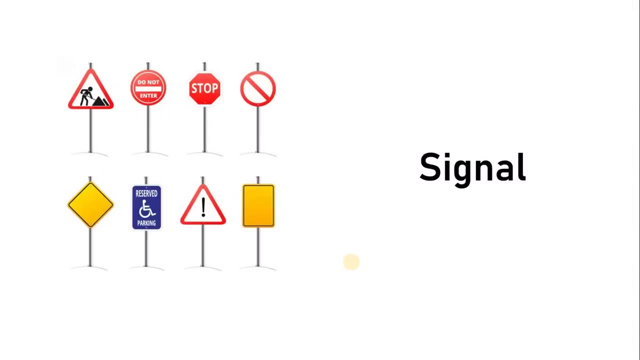 10 minutes past 2 pm. depending on the precision of that clock, it may still show you seconds, but it is still limited to some values only. so before we move further, we also need to understand one more term, called as signal. signals are used to convey some information to someone. 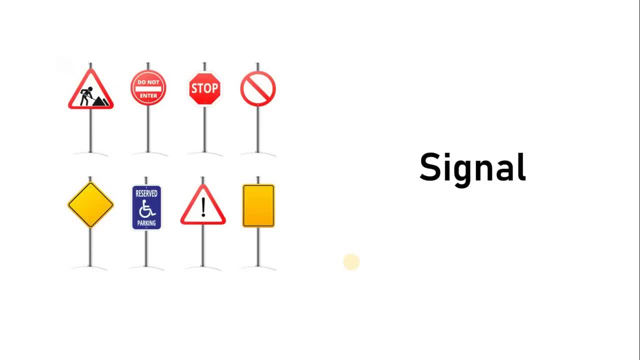 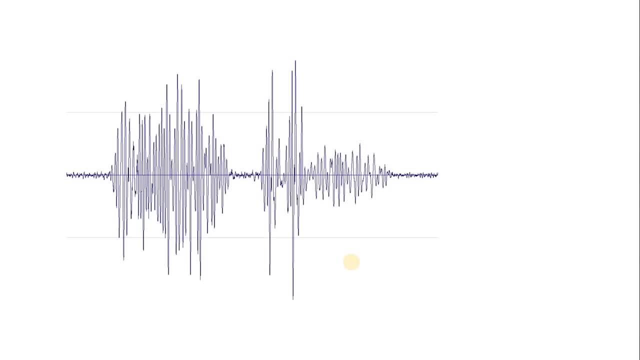 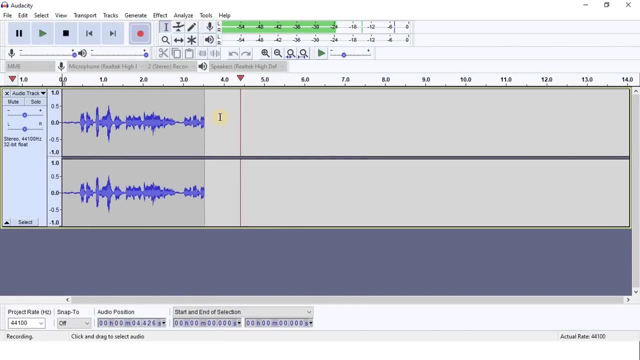 like these road signs are passing on some information to us, like that we need to stop or we cannot park here, etc. similarly, when we speak, we generate a signal and that signal contains the information which we want to pass on to the listener. like i'm speaking right now, i'm generating an audio signal which you can see on this screen. 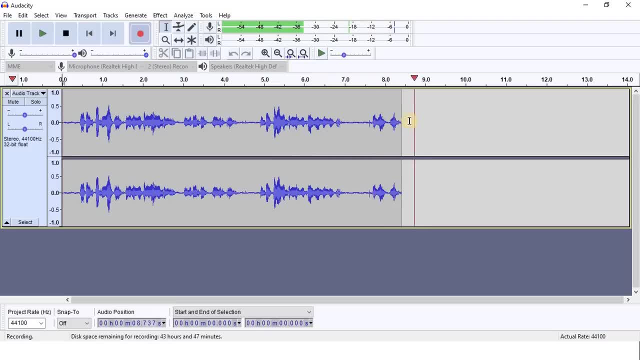 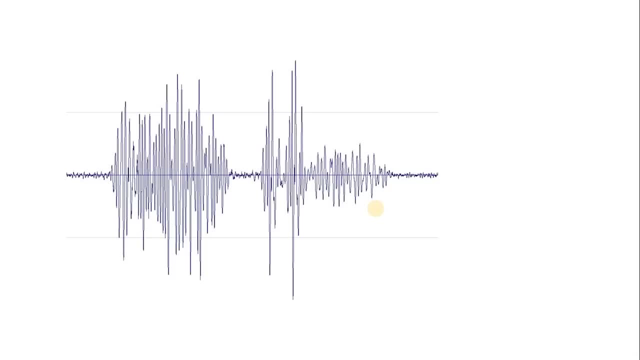 this is the audio signal which i have generated with my voice. okay, so this signal passes through my mouth, through air and to your ear and you make some sense out of it. okay, this audio signal is analog in nature because there are infinite number of values which are changing. okay, in electronics, signals are some time varying quantities which convey some. 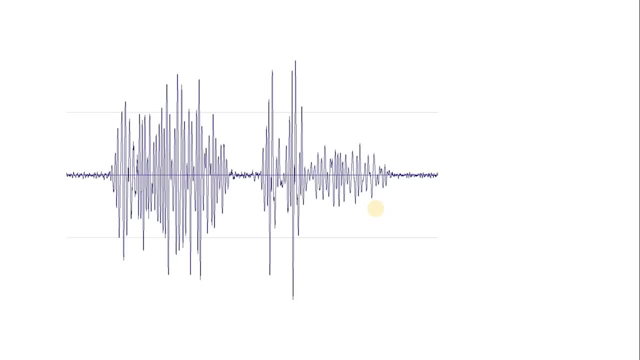 sort of information. usually that time varying quantity is voltage. that means with time the voltage changes, okay, or sometimes it is also current, but usually it is voltage. then those time varying signals are passed between the devices in order to send and receive information, which might be video, audio or some sort of encoded data. usually signals are transmitted. 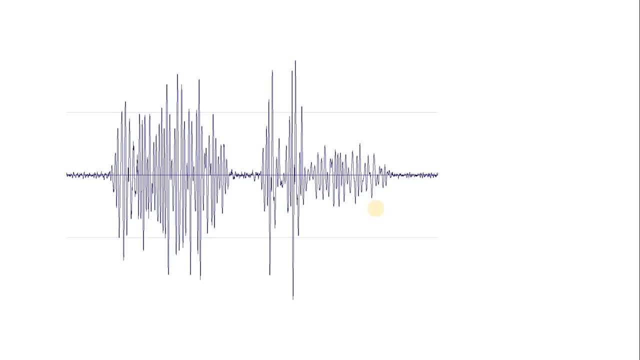 through wires, but they can also be passed through air, wirelessly. okay, so there is an entire field study which is based just on signals, like digital signal, processing signals and systems. there are some entire subjects based on signals only. okay, but for the scope of this course we will just tell. 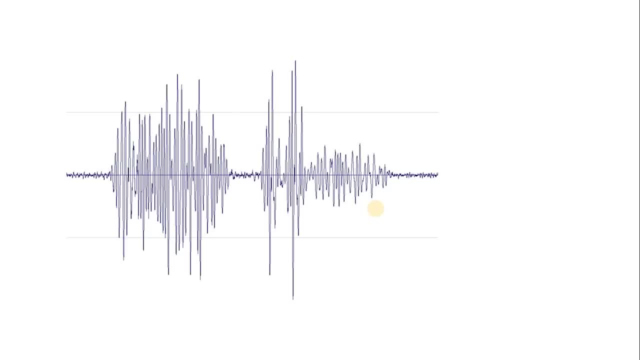 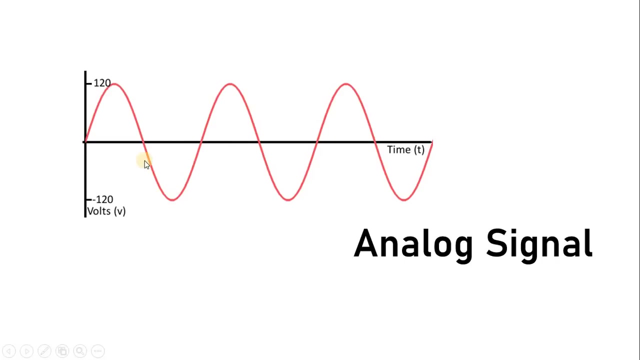 you the required information. so now there are two types of signals. one is analog signal and one is digital signal. like we just saw, that, our sound is a type of analog signal. similarly, there can be other analog signals as well. typically, an analog signal would look like this: that means we have: 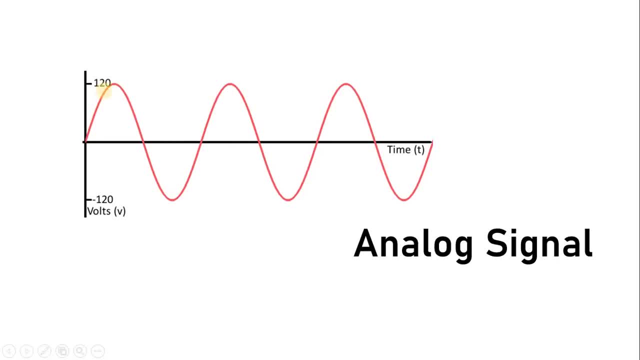 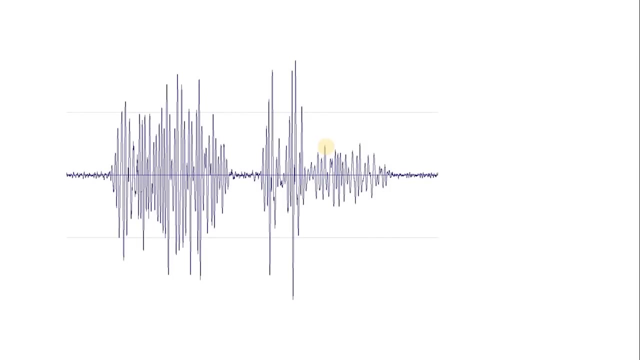 plotted time on the x-axis and voltage on the y-axis. so with time the voltage is increasing, then decreasing, then going into negative part, then increasing. this is an analog signal. it is not necessary that it stays this smooth. it can be little messy as well, like this. this is also 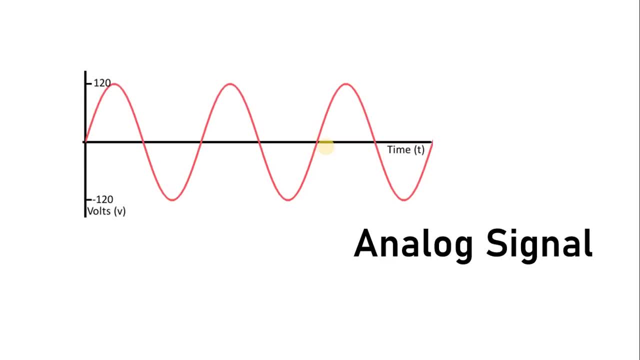 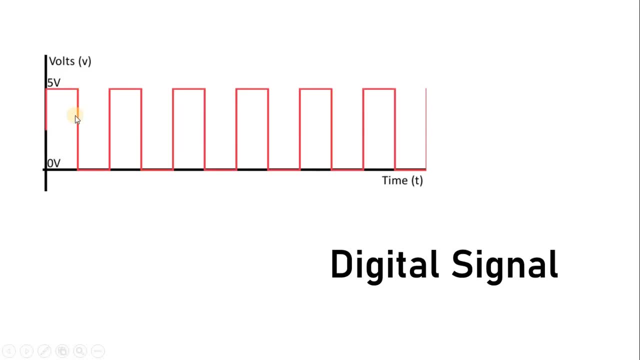 an analog signal, okay, and then there is a digital signal. in digital signal, there are only two discrete values: either it is on or either it is off, where 5 volts represents on and 0 volts represents off and 0 volts represents on and 0 volts represents off and 0 volts represents on. 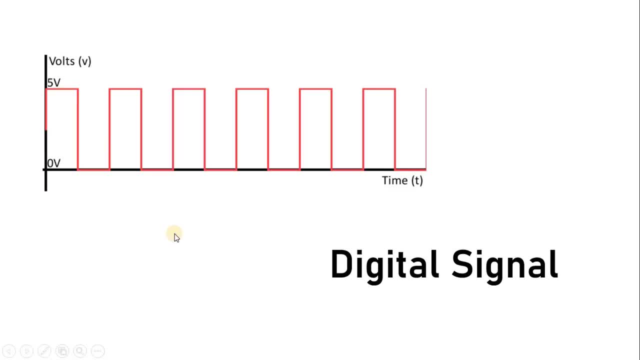 represent off. so you can see, with time, here it is on, it is off, on, off, on, off, on and off. right now, the sensors, and the sensors which we use in our course, will either give analog signal or either digital signal, and we have to use arduino to read those signals. okay, we will. 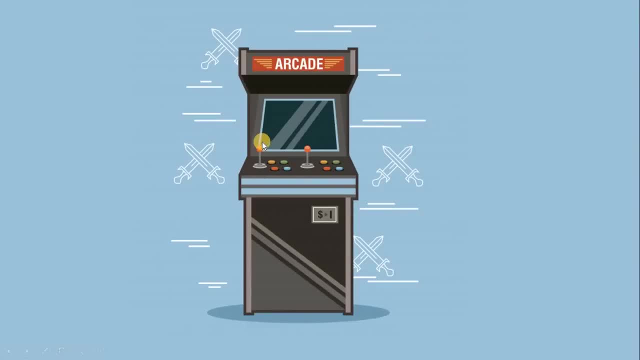 see an example. let's say we have a gaming console here. this is the joystick, this is a device which would give some analog signal and these are the buttons. and these devices will give some digital information, so this game machine can be programmed to read this state of the joystick. 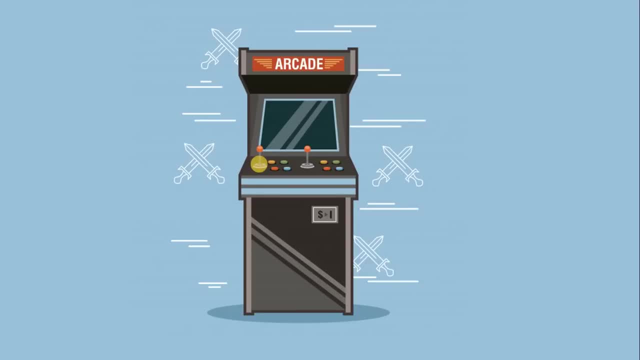 for example, we can make a character move forward. when the joystick is moved forward, we can also control the moving speed of that character. for example, if we make the joystick move a little forward, then it will move slow, and if we move it a little more ahead, then it will move. 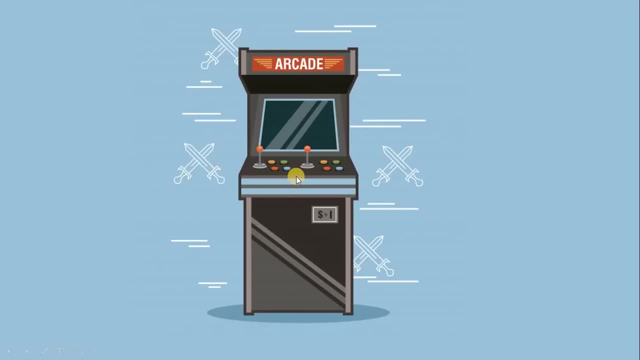 faster. but this cannot be the case with the digital button. we can just press the switch and tell the character to move forward. we cannot decide the speed. we can only set one speed there, or we can program it to move forward fast based on some time- okay, but we cannot input the speed. 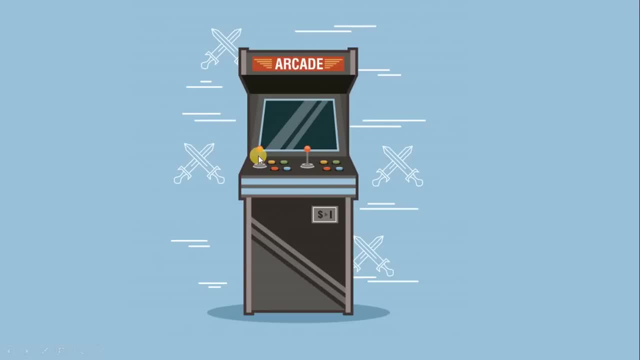 through buttons. right, so this joystick is sending some analog signal into the computer or the controller which is placed inside this gaming machine, and these buttons are sending some digital information, like either they are pressed or not, they are on or off. okay, so this is a digital signal. i'll give you one more example. we have potentiometer here and we can move it as a knob. 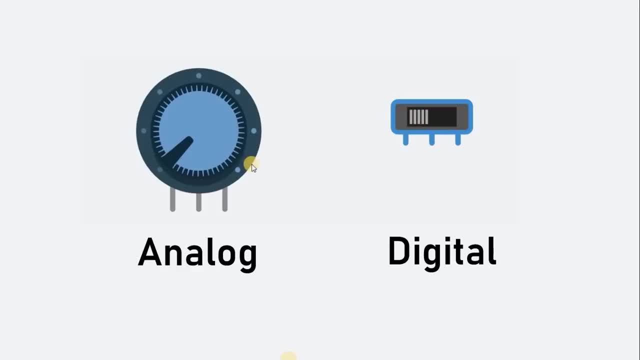 and we have infinite number of values. here we have a switch which is either on or off. this represents analog and this represents digital. so whenever we use analog sensor or component, we will use analog pins of the arduino and we use digital pins for digital sensors or components. 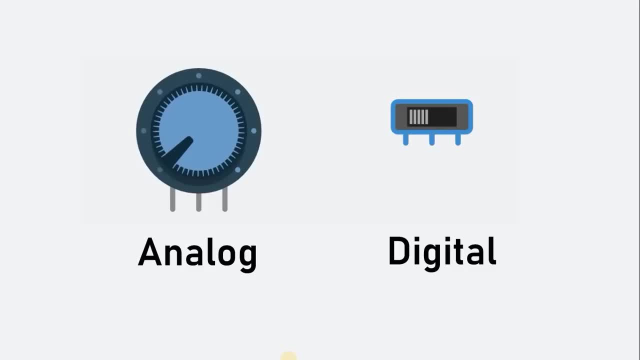 okay, i have given more insights on this topic in analog read and digital read video in programming section. once you reach there and watch those videos as well, it will be crystal clear to you, and if not, you can just comment down below or send us a message in this video. 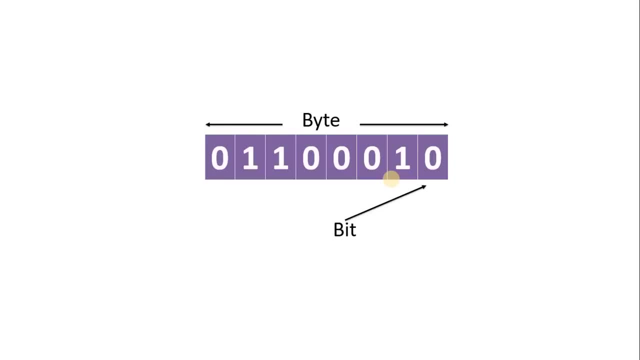 we'll talk about bit and byte. so basically, what is bit? bit is the smallest storage or memory size which can store a value of either 0 or either 1.. this box represents a bit here, okay. similarly, if 8 bits are combined then it forms a byte, okay. so we can say: 8 bits is equal to 1 byte. so 1 byte. 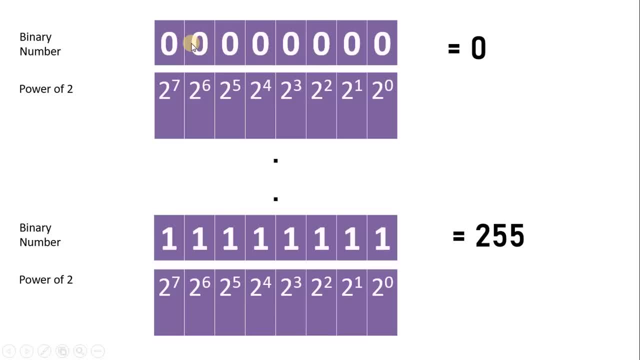 can store 0 as the smallest number. why? because in that case all the 8 boxes or all the 8 bits are 0 inside it. as i told you, it can either store 0 or 1. okay, so each box has a multiplier and we take the value from this box and we multiply it with this box, okay, and calculate. 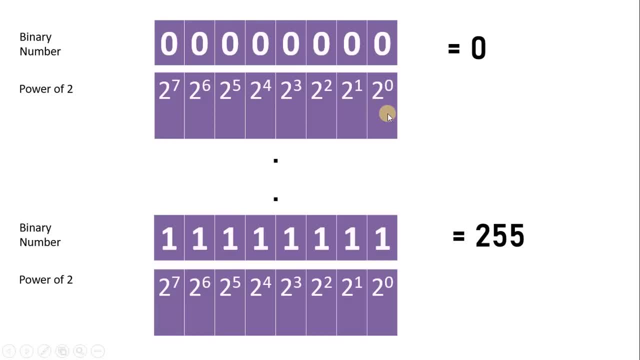 the value here and in the end we take sum of all the values. so here what will happen: 0 multiplied by 2 to the power 0, 2 to the power, 0 is 1.. 0 into 0 is 0, 0 into this is 0, 0 into anything is 0.. 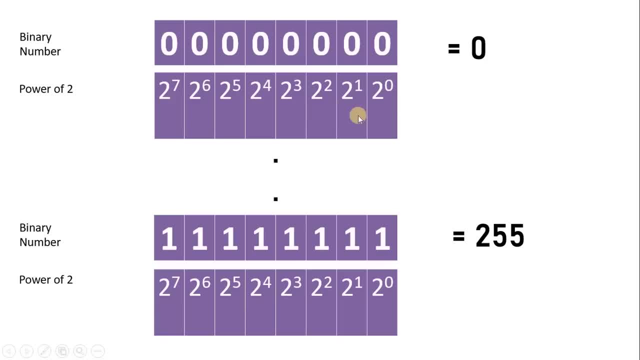 in all the boxes we'll get 0, so hence the smallest value will be 0, and when will be the maximum value? if all the boxes are 1, right? so here we will get 1 into 2 to the power, 0, that is, 1 and 2 to the power. 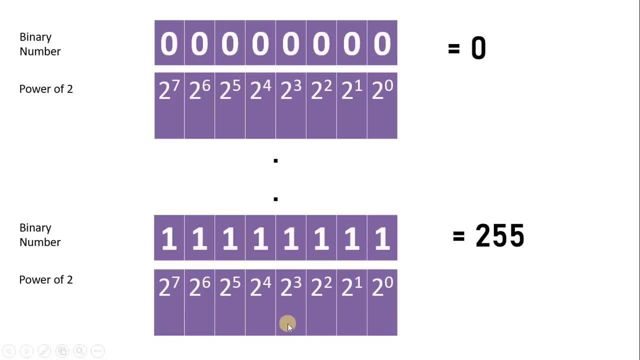 1 is 2. here we'll get 2, here we will get 4, here we will get 8. here it will be 16, here it will be 32, 64 and 128.. now, if you take a sum of all these value- you can calculate it on your own- you will get 255.. 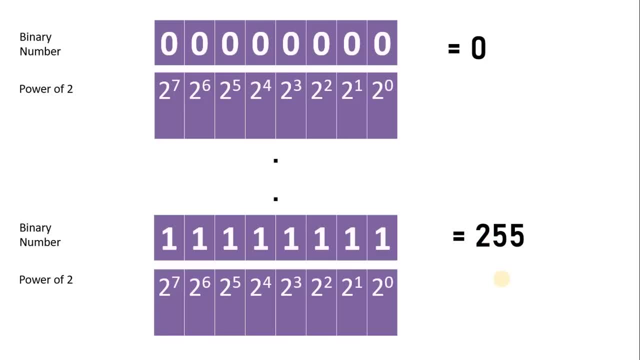 now in case, if we want to store a value greater than 255, so now, in that case we will have to take one more bit aside this, so it will become 9 bit. so the 9 bits can store 511 values. and what? if we have to store a bigger number than that, then we will add another bit here as well, and 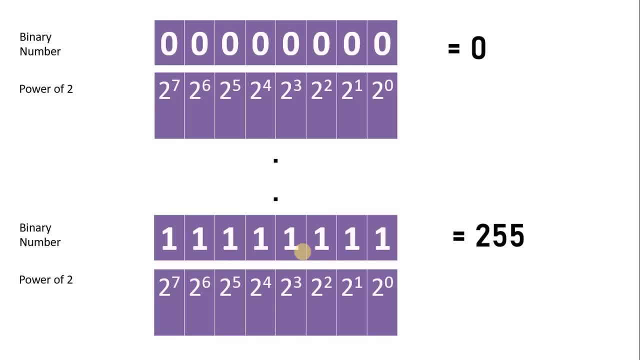 it will become 10 bits, so 10 bits will be able to store a value till 1, 0, 2, 3.. so now what you have to keep in mind is you will be needing this information whenever i say 8 bits, 10 bits, 12 bits. 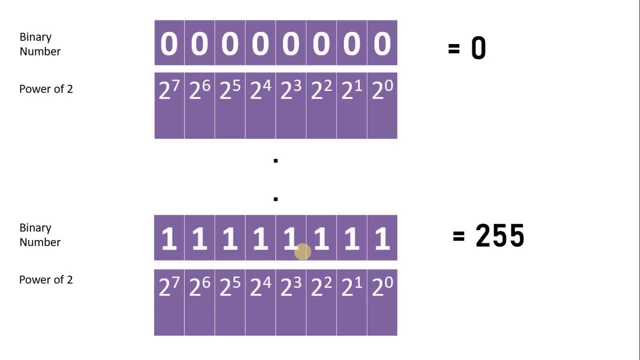 in the course, so you can only store values up to the upper limit of that space. okay, so this information will be sufficient for you to carry on the course. but yeah, if you want to know more about binary maths, you can just google binary maths and you will get really good links from wikipedia and 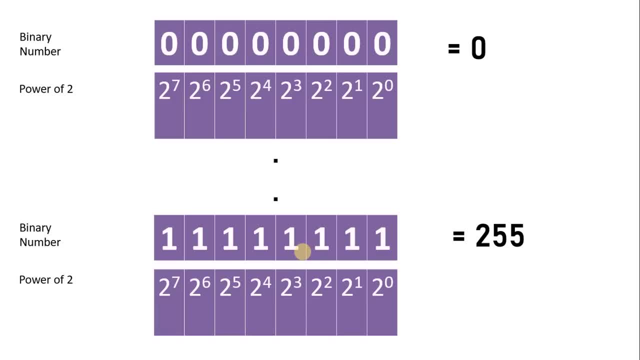 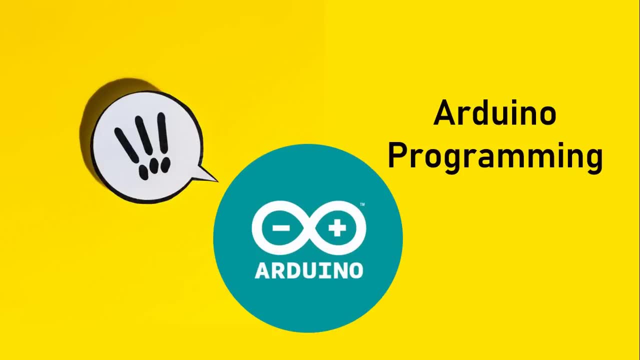 other websites and you can just read them. if you face any problem, you can always comment down below and we will get back to you. in this section i would cover all the essential programming concepts that you would need to get working and make projects with arduino. i would like to tell 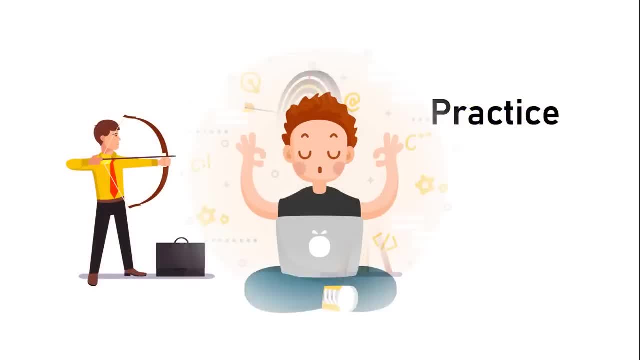 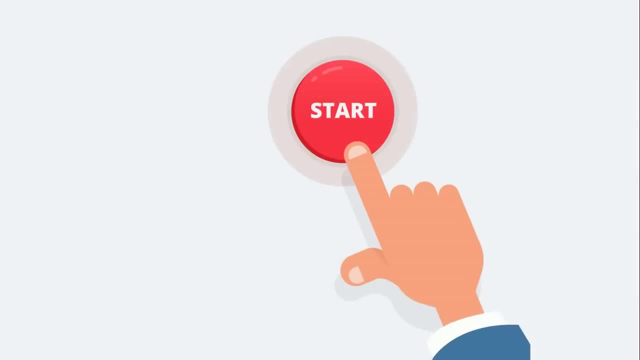 you that programming is a game of practice. the more you practice, the more you get better at that. so i would cover all the essential topics to get you started, and i will also tell you about concepts as we progress ahead. so let's get started. before we know about arduino programming we need to 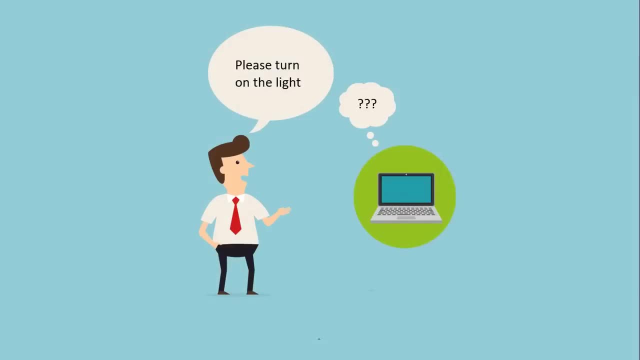 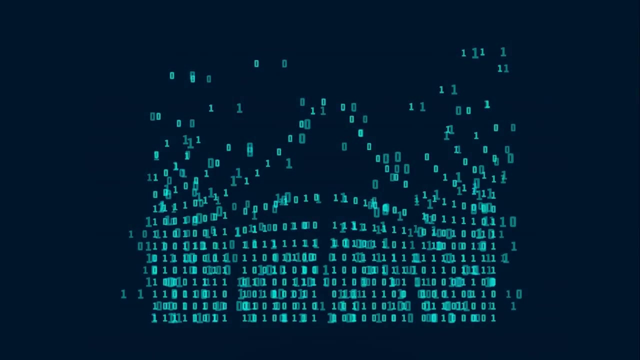 understand what programming is. programming is something which we do to tell a computer or a controller what to do. computers don't understand the language which humans use to communicate with each other. computers only understand the zeros and ones, so by programming, we tell it what to do in our 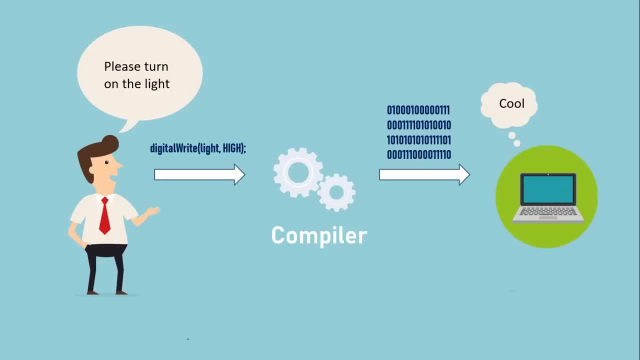 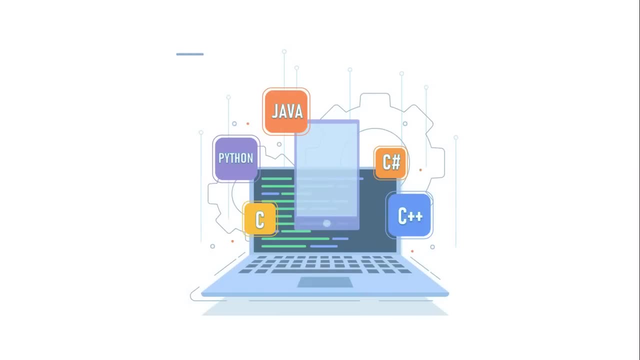 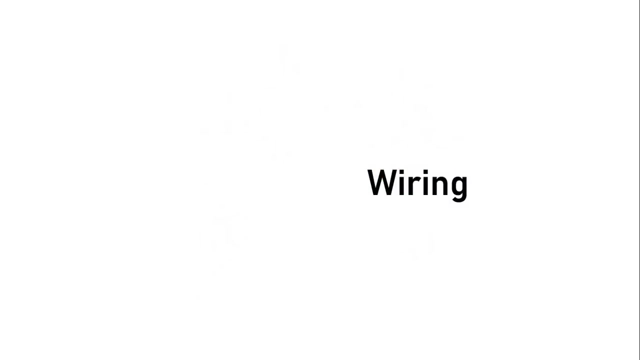 computer, the compiler or an interpreter converts that into a language which computer understands and the computer finally acts on it. so there are many programming languages over there, like c, c plus plus c, sharp, python, java, etc. all of them have their own benefits and drawbacks. the language which we use to program the arduino is a mixture of c and c plus plus, which arduino 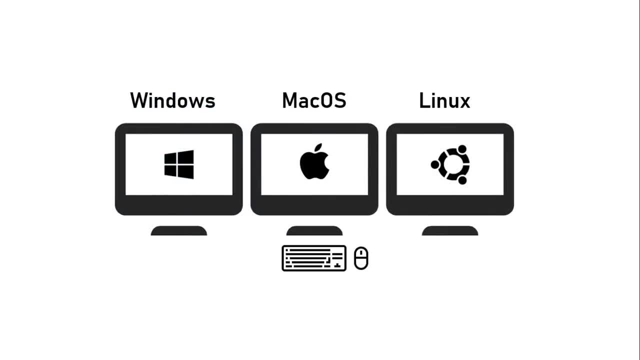 makers call as wiring. the best part of this arduino language is that it is uniform across all platforms. that means it won't matter if you use windows, mac or linux that would have. the code would be the same. so in the next video we will start to look at arduino programming. 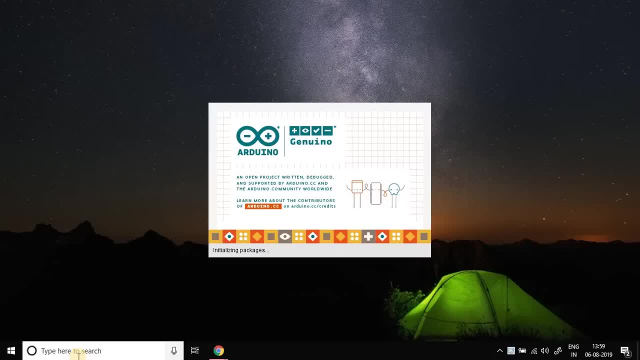 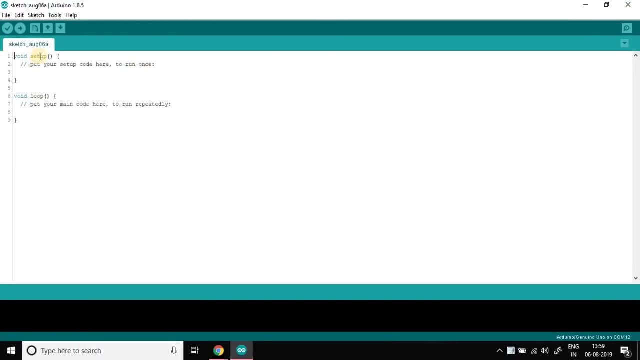 in a bit more detail. so let's start by opening up our arduino ide. once it opens, you would see this window all right, and we see void setup and void loop is written over here. so let's discuss whatever we see on the screen. the first line which we see is white: setup right, it says void. 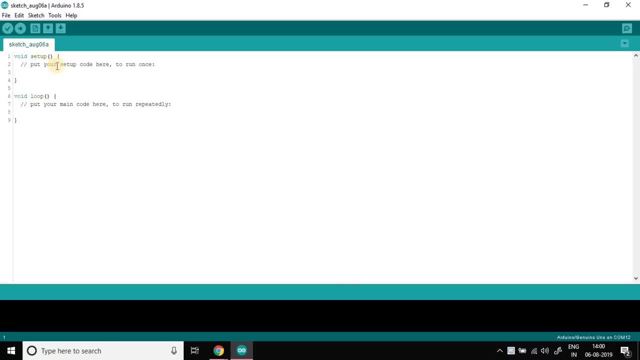 then setup, then a pair of brackets, then a curly bit bracket, then we have two forward slashes. then it says: put your setup code here to run once, and then we have another curly bracket. so what we have done here is we have declared a mandatory function known as setup, and this is how you declare functions in arduino. then we have a. 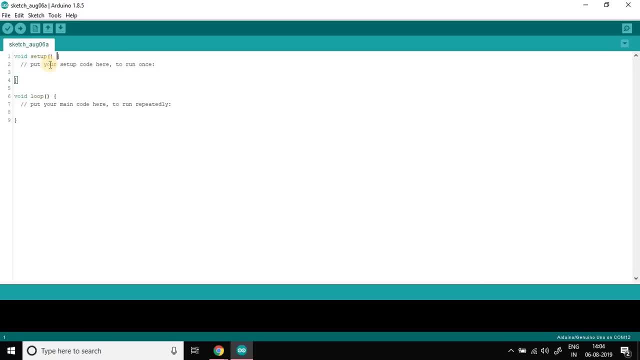 curly bracket. in most programming languages, these curly brackets indicate a block of code. this left curly bracket means the start of the block and this right bracket shows the end of the block. whatever code which goes inside this block belongs to this function. the id would help you recognize the blocks of codes when you click on these brackets, for example, 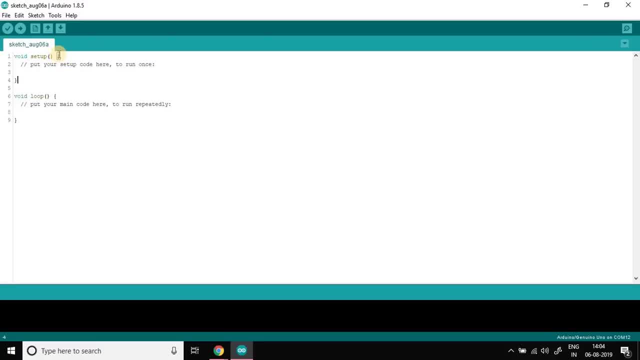 when you click here, it would highlight this bracket automatically. that means this is the start of your function and this is the end of your function. whenever you click here, then it would highlight the ending. can you see that? all right, then we see these two forward slashes: these: 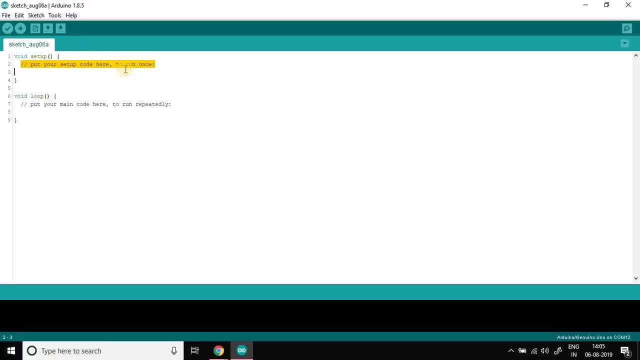 forward slashes mean a single line comment. whenever we write a comment, compiler entirely ignores whatever is written after that. so, coming back to void setup, this mandatory function contains all the lines of code which we want arduino to run once when it is turned on or when we press. 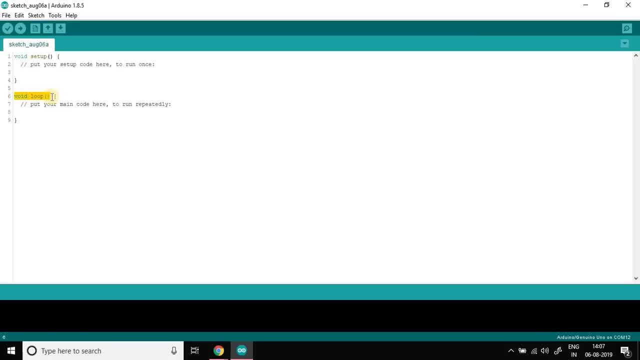 reset button. we'll talk more on this in coming lectures. similarly, there is void loop. in this section we write all the code which we want arduino to run all the time repeatedly. that means whatever is written in this section would run until the arduino is switched off- the void loop. 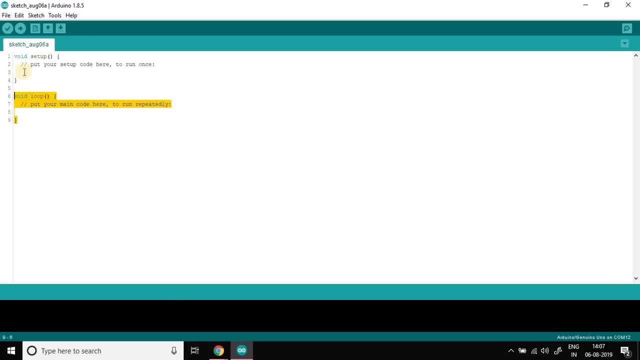 runs after void setup. so in the next lecture we would see the blink led example which we use to test our arduino, in a little more detail. we will understand each part of that code. so see you in the next lecture. so till now we have understood that the two functions void setup. 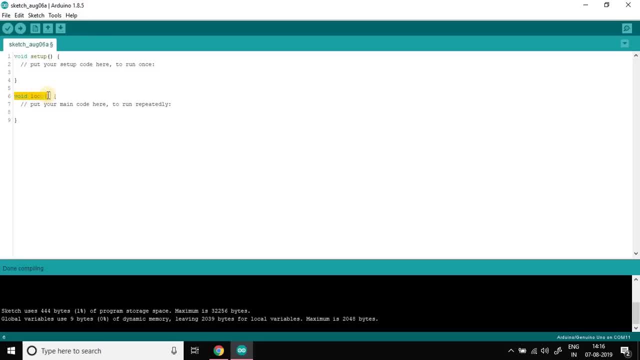 and void loop are the bare minimum requirement to run our code successfully. why are they mandatory? i will just show you in a moment. i'm removing these functions and i'm hitting compile. the compiler has bashed us with errors. just read them. undefined reference to setup. undefined reference. 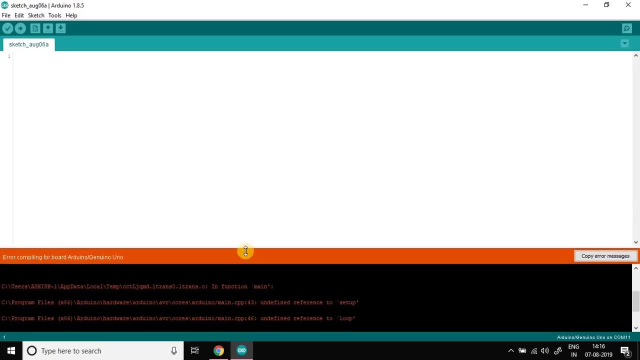 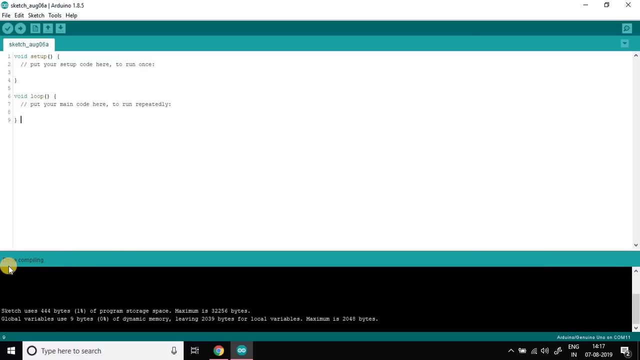 to loop. that means it is expecting that we must define these functions. now i will bring back these functions now. i'll hit compile once again. now the compiler has successfully compiled the code. so with that we can say: arduino ide's compiler expects these two functions, like some other programming languages expect a. 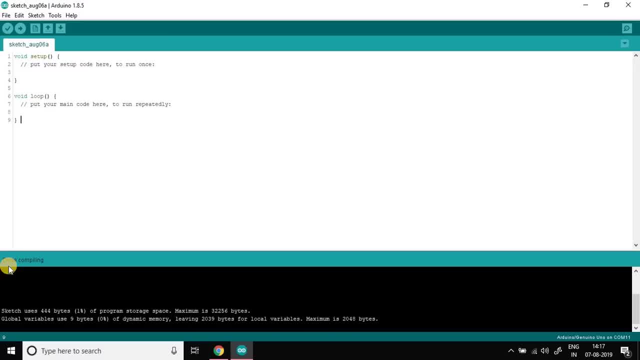 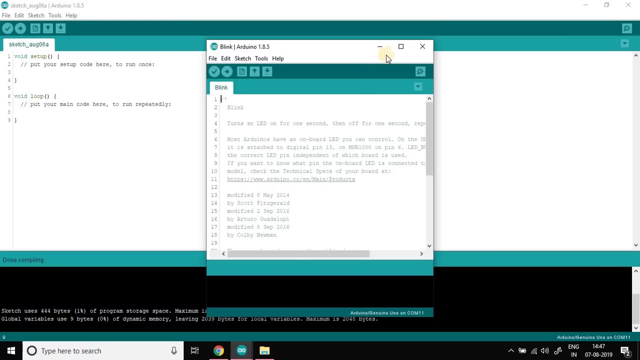 main function. without that we won't be able to run the code. we would get an error, as you saw. so now we will see some more concepts in the blink led experiment. so for that we'll go to files, examples, basics, and then blink. all right, so this is our blink example. this is that same code that. 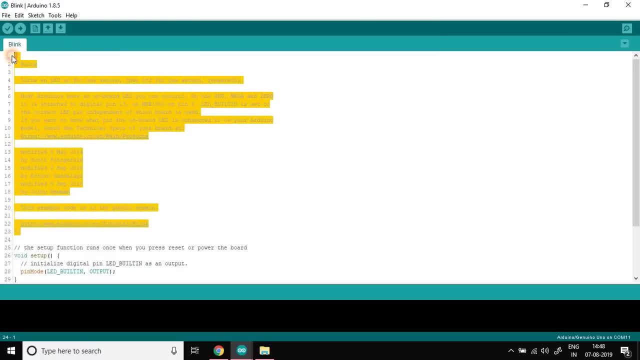 we used to test your arduino. so we see a huge chunk of lines here, which is a block of multi-line comments, like we saw a single line comment in the previous video. we start a multi-line comment by a forward slash followed by a star, and then we write whatever we want and then we end it by a star. 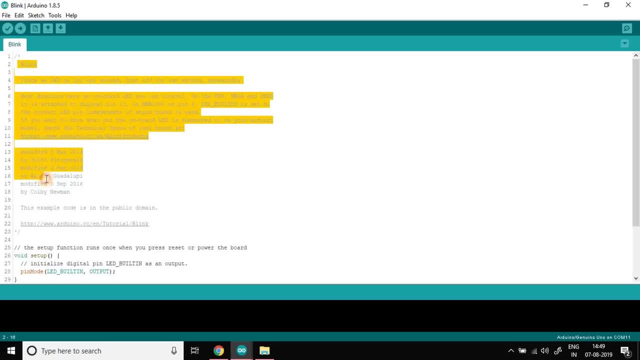 followed by a forward slash, so anything which is written in between is ignored by the compiler. you may ask then, why do we write comment? the answer is: the comments help us to document the code and they also help the other readers of the code to understand what is done by the author of the code. 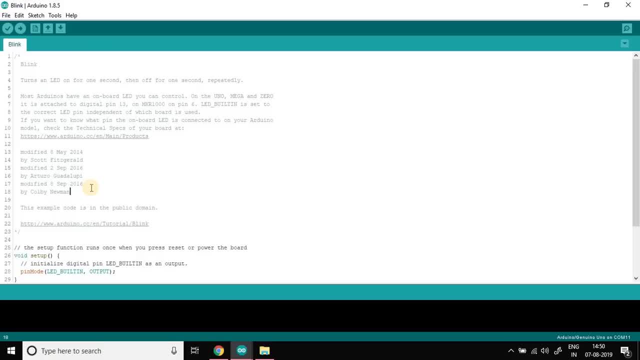 comments also help the author himself to recall what he did when he sees his code at the latest date. since comments are totally ignored by the compiler, not writing them won't make any difference. for example, if i remove this comment and compile the code, it will still compile, and with the 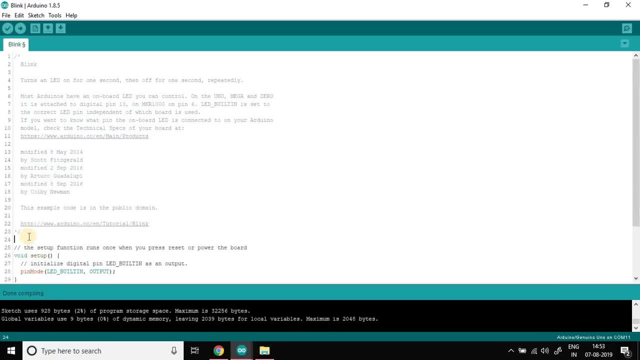 comments also, it will run just like that. since these comments don't serve any technical purpose in the code, most developers develop a habit of not writing that comment, which is certainly not a good practice. it is always advised to write comments in the first place, because it will be. 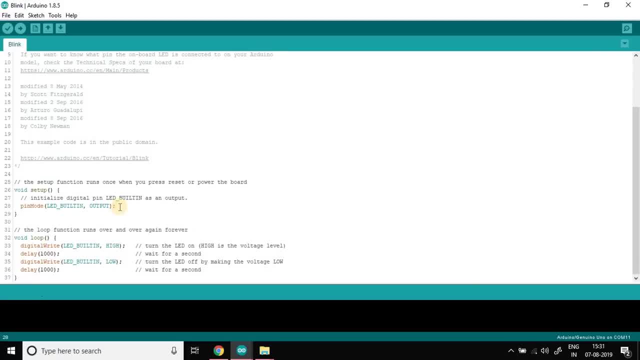 for the reasons which i have already told. so now i will tell you about the white spaces and case sensitivity. the spaces which you see here, here, here, etc. like here, here, won't make any difference, as the compiler would ignore them, like the comments. now, what i mean to say by this is: 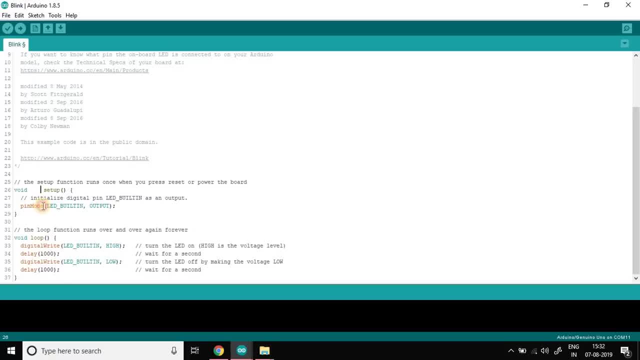 that we can add as many spaces as we want, wherever we want, and the compiler won't say anything to us. it will still successfully compile the code like this, all right. but what we can't do is we can't add spaces in between like this, otherwise you will get an error if you compile now. just see that: how many errors. 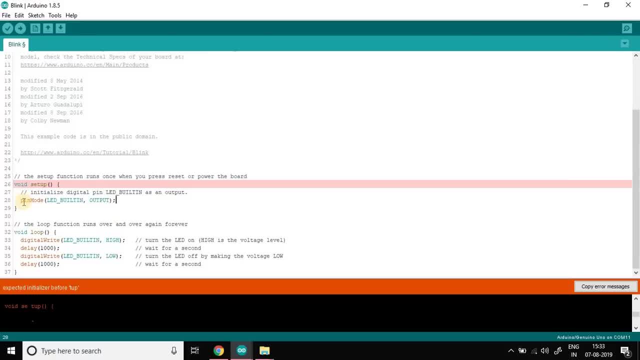 we have got. so now you will ask: what's the purpose of white spaces? white spaces basically help us indent the code. it makes it easier for us to identify the blocks of code. it also makes the code look beautiful. for example, if i write something like this: what do you think this code looks better? or this code looks better? obviously this one. 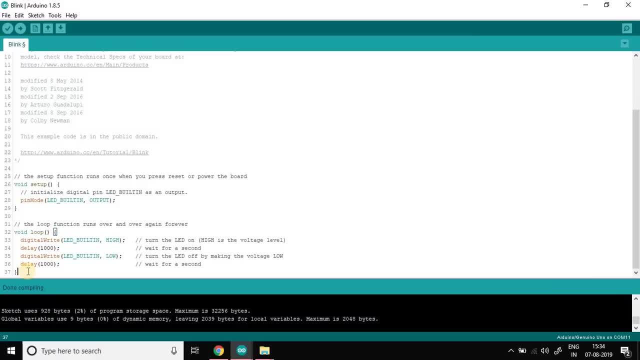 all right. so proper indentation is important. now coming to case sensitivity: arduino language is case sensitive. what i mean by that is the small character would come as small and the capital character would come as capital. you can't interchange that. for example, this void cannot be written as this. it will give an error. void does not name a type. 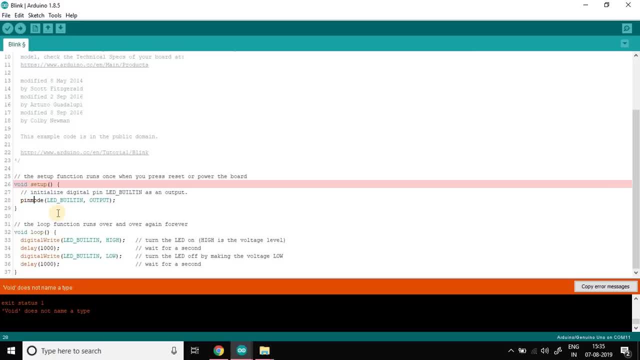 right in this pin mode. you see, we cannot write pin mode as this pin mode, right, then also it will give an error. so same goes for everything what you see here, like this high, cannot be written as hi, anything for that matter. you have to write it exactly like this. don't worry if you find it too. 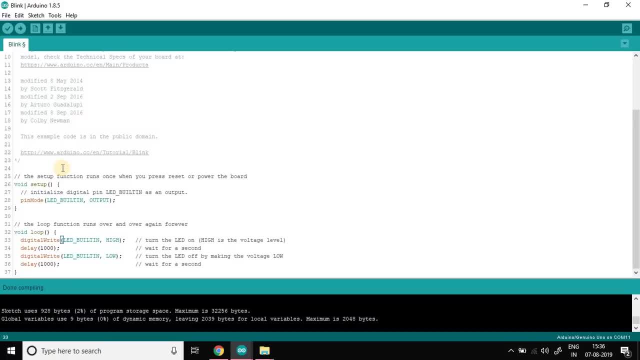 difficult to remember. you will get a hang of it very soon. remember what i told about programming. it is the game of practice. it is very common to mess up, so the arduino id has built-in provision to help us with that. what i mean to say by that is, if you ever mess up the casing by mistake. 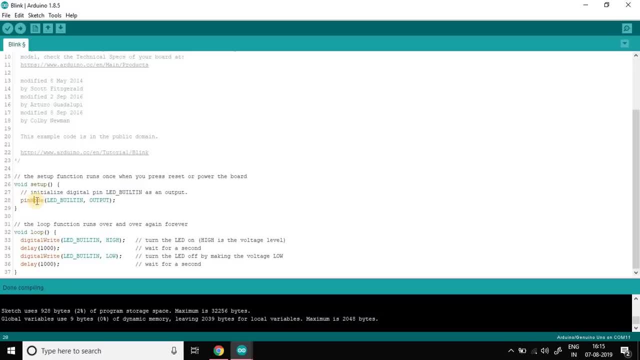 you would see that this is no more coming in orange color right now. it is coming back in orange color. same goes here. so if you ever see that these critical words are not showing up in color form, you can guess that you have made a mistake. now let's see what is done here. in void setup it says pin mode: led builtin output. this pin mode is a. 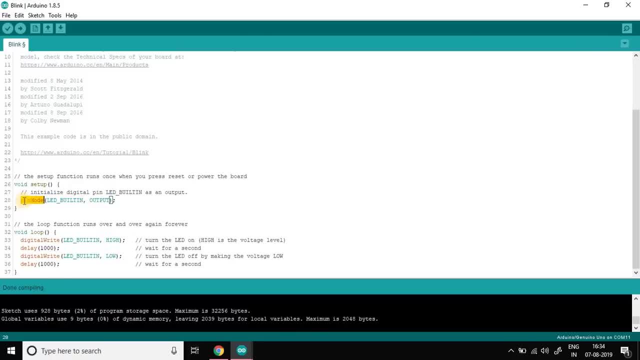 built-in function which configures the specified pin to behave either as an input or an output. this input and output is in reference to the arduino. if something is going into the arduino through that pin, we would configure it as input. or if something is coming out of arduino through, 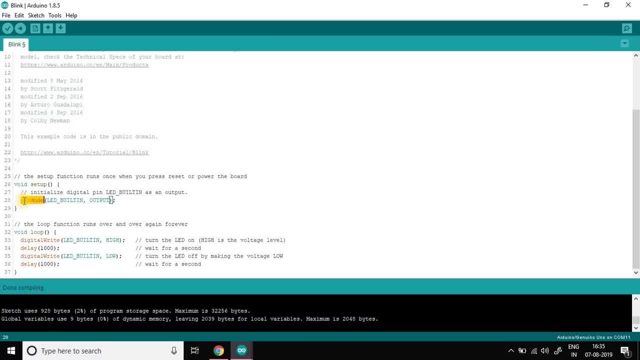 dart pin, it will be output. in our case the built-in led would need some sort of output from arduino, so we will use output. so if we see this line in a little more detail, we have written pin mode, then there is an open bracket. then we have written led built-in, then there is a comma. 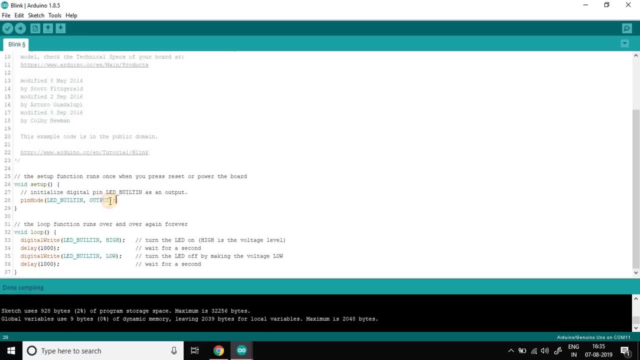 then this is output and there is bracket close and there is a semicolon. i won't be surprised if you have not noticed this semicolon till now. i won't be surprised because it is very, very common to forget this semicolon. this semicolon marks the end of a statement. that means we are telling the 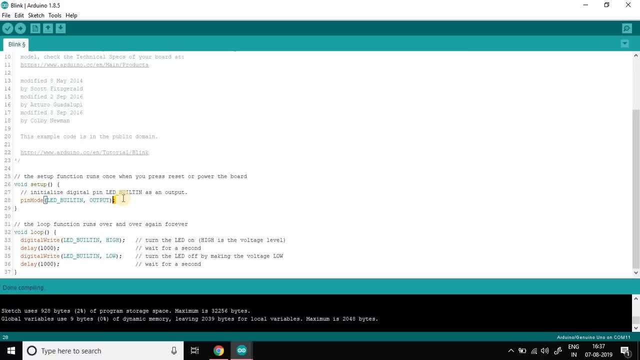 compiler. we are done with the statement. we have finished one line. if we remove the semicolon we would get an error. you see expected semicolon before this. so back to that. what this line means is we have called a built-in function called pin mode, which has two arguments. the first argument: 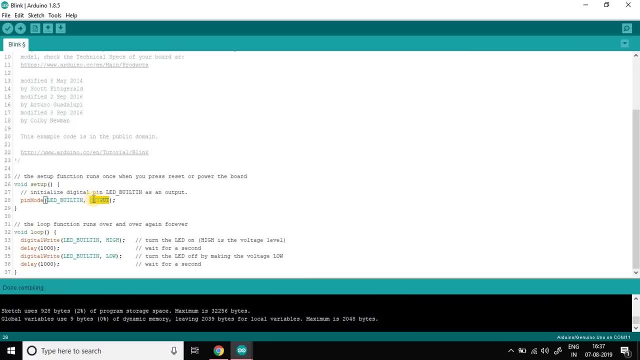 is the pin number which we want to configure, and the second argument tells the configuration which we wanted to act as this built-in led is connected to pin number 13 on the compiler of arduino, so we are telling arduino to set the configuration of pin number 13 as output. okay, 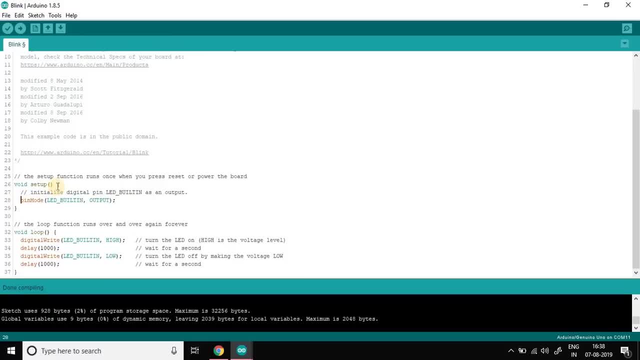 this is what this line is doing. also note that this line is written inside the block of void setup. can you see that right? one more thing which i would like you to notice: this led built-in. the compiler is automatically replacing this led built-in with pin number 13.. also note that the 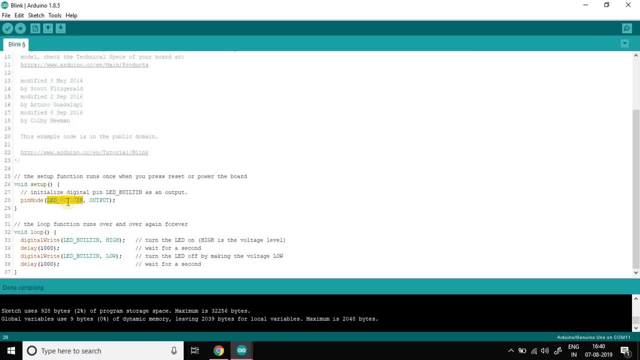 compiler is not changing the led built-in to 13. magically, it has been fed somewhere else in the. we will talk about libraries in coming lectures, but what i want to say right now is this is equivalent to this for those people who felt a little uncomfortable when i said we are calling. 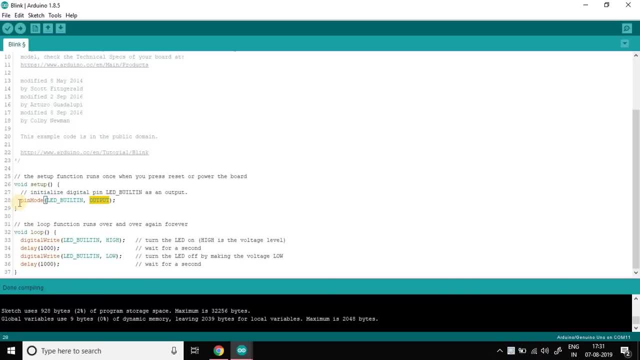 a function here which has two arguments. i just want all of those people to know that we will talk about functions- calling functions, arguments of the functions- in a lecture in which we talk about creating custom functions. then you will be able to relate what i said here exactly. 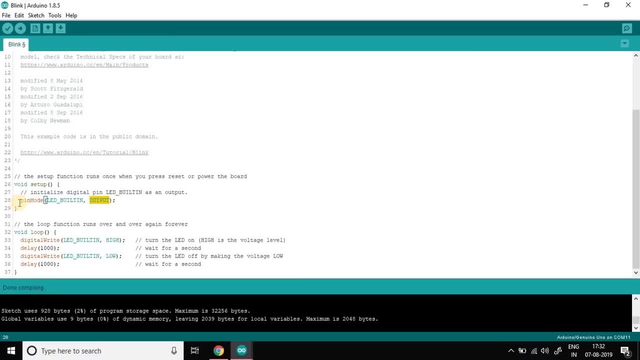 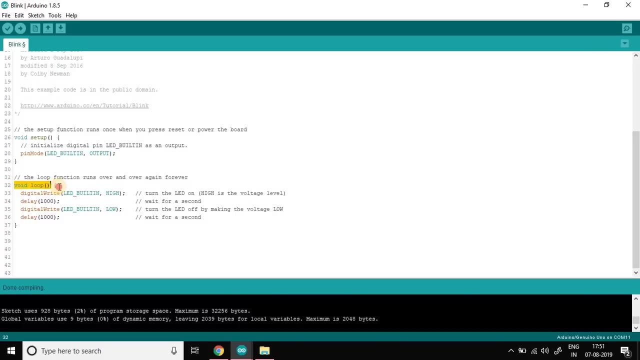 but for now, just understand. we use pin mode function like this. we will have to use it whenever we have to configure a pin, and using this inside setup means that we want this function to run once whenever we turn on the arduino or reset our arduino. all right, so now we will see what we have done in void loop. the first thing: 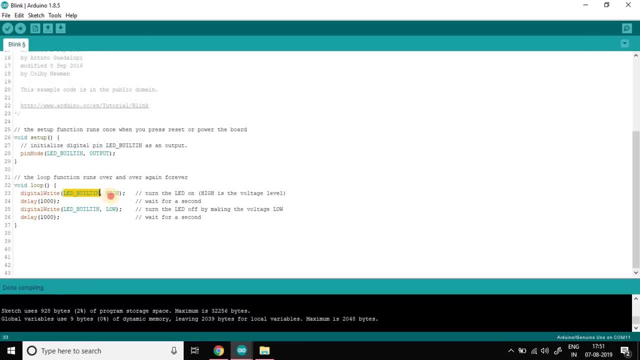 which we see is digital right, then it is led built-in, then we have high, okay. so the digital right is an inbuilt function which is used to manipulate the digital pins, and we can also use it to locate analog pins using digital right if the pin is declared as output in setup using 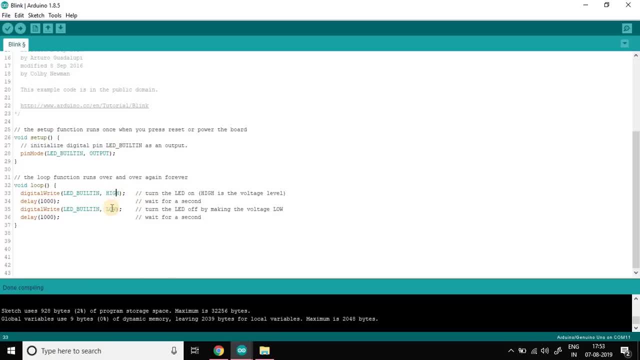 pin mode digital right will write a value of 5 volt if we use high and to 0 if we use low. but do make sure that you have declared the pin as output, otherwise you may see unexpected results. then, after this line, we have delay in a value of 1000 and that, as the name suggests, the function would 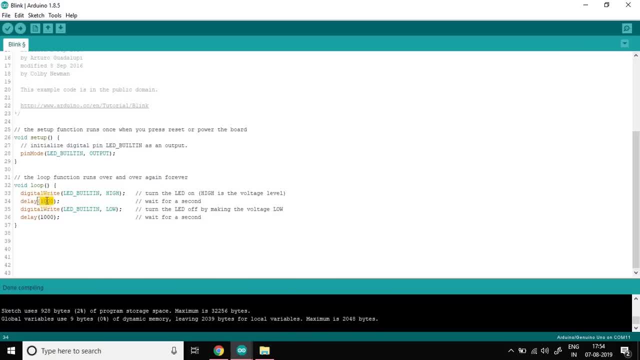 pause the code here for a specified amount of time. in our case it is 1000 milliseconds, which is one. The entire state of Arduino is preserved and nothing happens during that time. Then we have another digital write which would write low to the LED built-in. 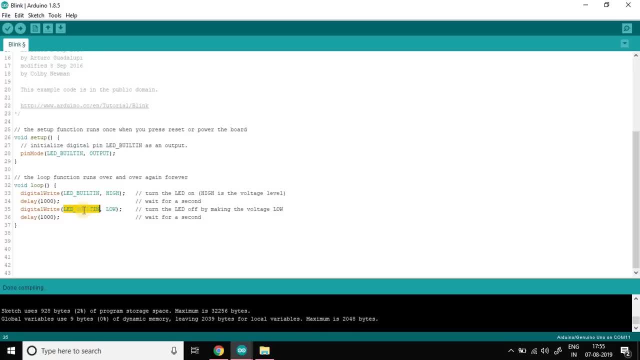 That means the LED will turn off Here. the LED will turn on here it will turn off, And this another delay will keep it off for one second And this entire process would keep on repeating unless we turn off the Arduino, as this is inside void loop. 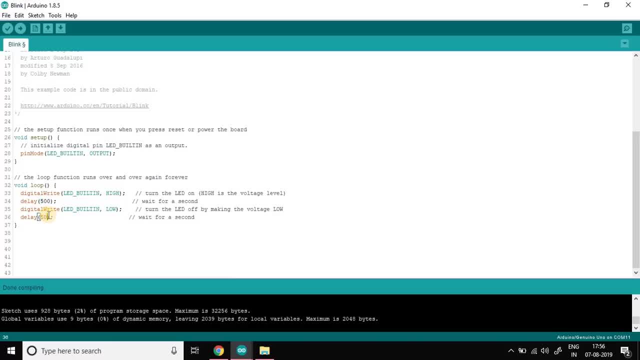 So if we change the value of this delay to 500, we would see the change in blinking pattern. I would like you to try changing the value to your desired value and comment down below if you were able to see the change. Now I would like to tell you that you can also store this delay value into an imaginary 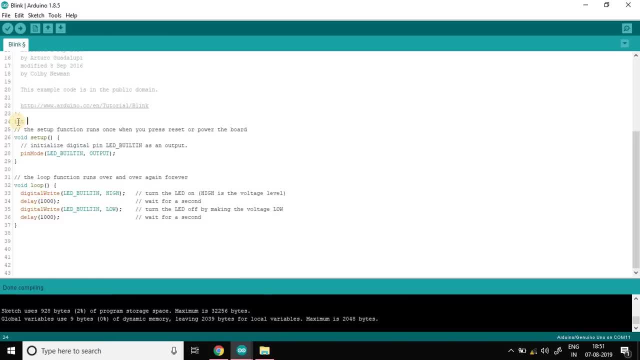 container known as a variable. We can do that by writing int. myDelayValue is equal to 100.. You can also choose some other name over here. There are some rules to deciding the variable name and you would gradually get to know those rules as we progress along the course. 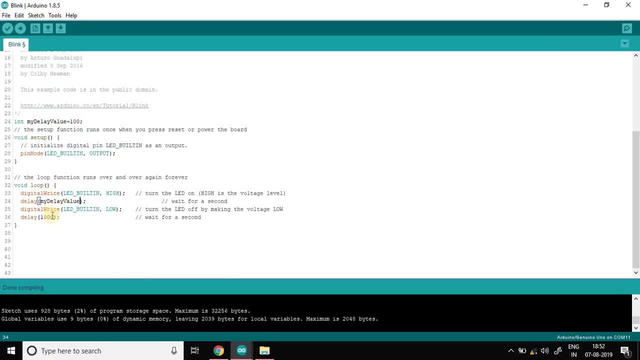 So now we can take this value and replace it here. So now, while the Arduino is looping on this code, it will take my delay as 100 instead of some other value. What benefit do we have to use this? We can change our value to any other value like this or this. if we need to change the 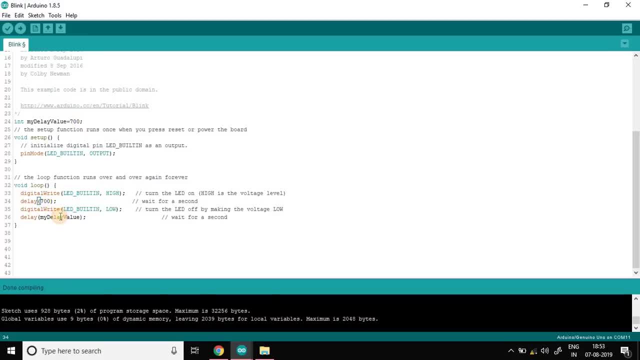 value Instead of changing here twice and making our code error prone. So now we can take this value and replace it here. We can just change the value here. It will save our time and also make our code less prone to errors. We can also make our own variable to define ledPin, and we would do that by int. ledPin is. 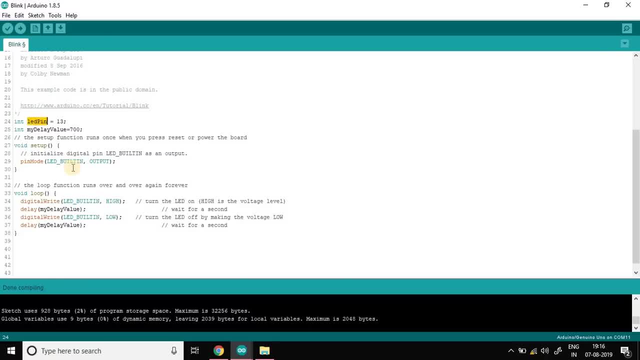 equal to 13.. And now we will take this ledPin and we will replace it here, Right, So this code will work Exactly like the earlier code, and it would work flawlessly. The benefit of using our own pin is that we can change the pin which we want to use later. 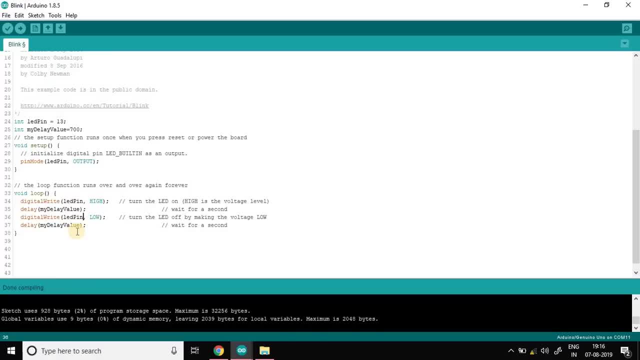 For example, now I have decided to use pin number two instead of pin number 30. So instead of changing the pin number from 13 to two everywhere, I can just change it to two here. So now, automatically, the compiler will pick the value of two of led pin and replace them. 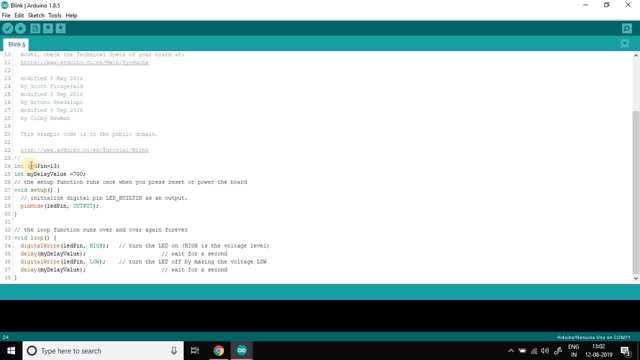 here Now. some of you must have noticed the way how I am writing led pin, like small l and then capital P. What's the reason Now? since we cannot keep spaces between our variable names, and led and pin are two different names, so the compiler will throw an error. 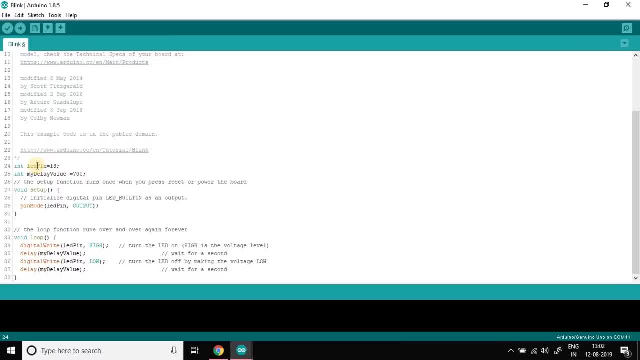 And some people came up with a solution that, to name variables like this, we can keep the first character of the second word, capital, in order to differentiate. So now our eyes are able to differentiate between led and pin properly, And this technique is known as camel casing. 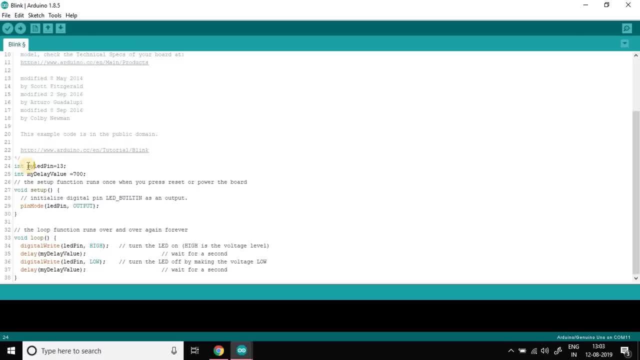 If I have to use more than two words, what I can do is like this: So now I can differentiate between led and pin, And this technique is known as camel casing. If I have to use more than two words, what I can do is like this: 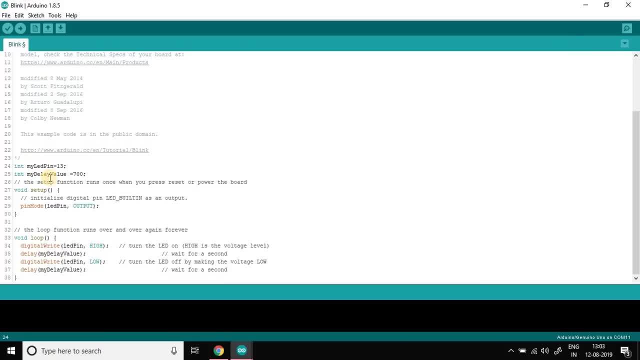 So now my eyes are able to read my led pin as three different words instead of one word, But for the compiler it is just the one word. And now some of you must be wondering what is int why we have declared it here, right? 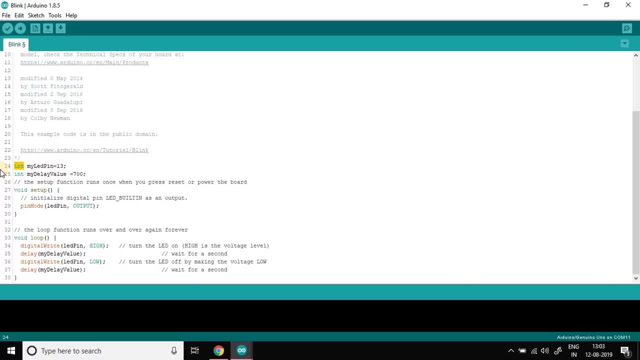 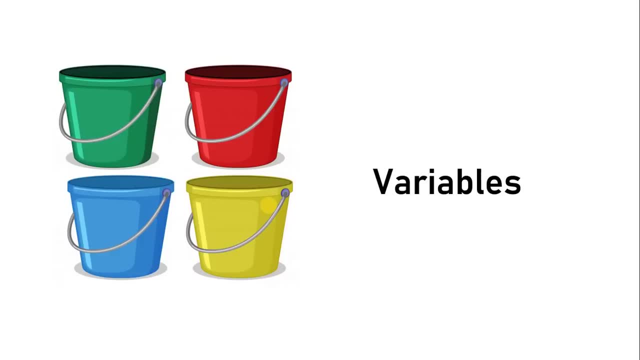 So in the next video we'll talk about this, int and the other data types, variables and more about variable scope. See you in the next video. So now we will discuss about variables. What exactly are variables? Variables are nothing, but they are kind of a virtual containers which is used by a compiler. 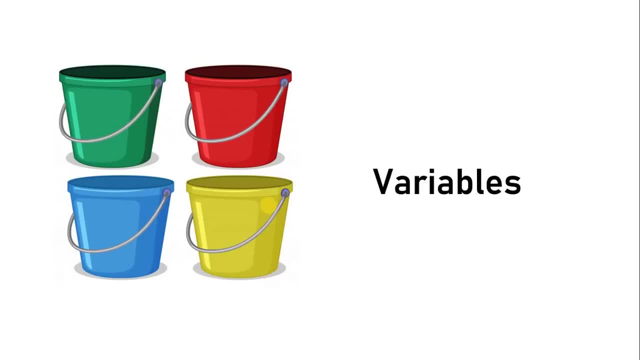 And we store some values in those containers. There are different kinds of data which we can hold in different kinds of container. For example, at your home you store sugar in some kind of specific container. You store tea in the tea container, oil in the oil container. similarly, in programming, 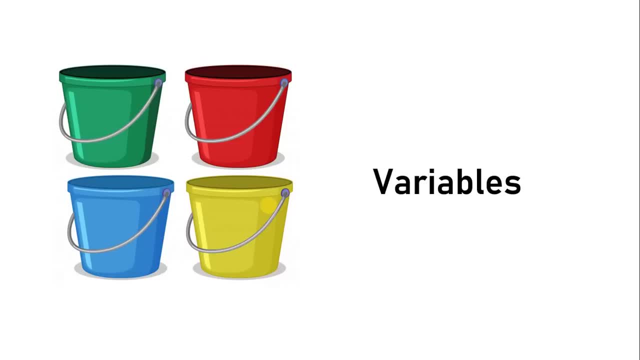 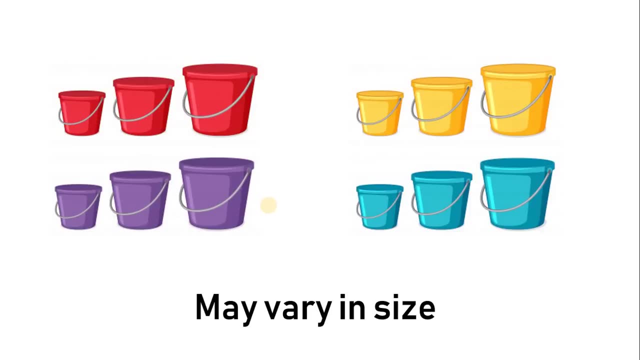 as well. We have some sort of containers and those can store some sort of specific data. The variables are available in different sizes, And we will be talking about just that, The default variables which are used in the Arduino programming. The thing to note here is the bigger the container, the bigger the value it can store. 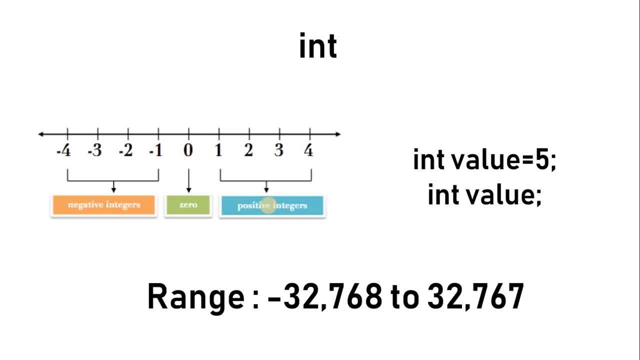 The first kind of data type which we will see is int. If you can recall, we used int in the previous video when we declared our LED pins and our own delay values right. So int is basically a container which can hold integer values. 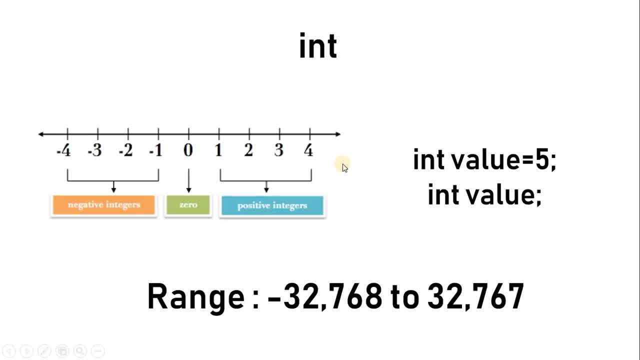 And I hope you're aware what integers are. If not, I will just quickly tell you that the number line is there. The whole numbers, from negative infinity to positive infinity are all integers Which you can see here in this video, like minus 4, minus 3, minus 2,, 0, 1, 2, 3, 4.. 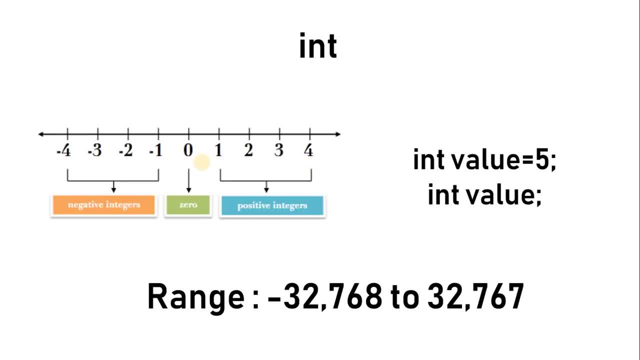 The numbers greater than 0 are positive integers and the numbers less than 0 are negative integers. The default integer which we use in our Arduino programming has a range of minus 32,768 to positive 32,767, right. What this means is the size of integer can hold these many values. 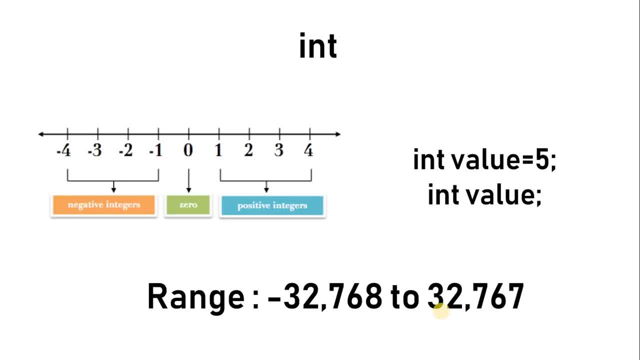 If you try to store value beyond this range, the values will overflow. Now I will tell you how to declare an integer in programming language. First of all, we write int. then we name the variable, like in this case, the name of the. 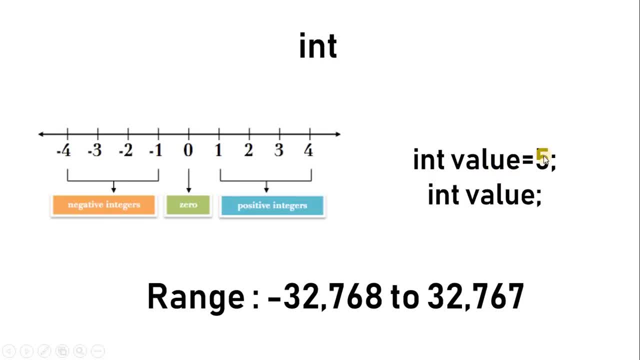 variable is value, and then we assign a value to it. For example, we have assigned a value of 5 here, right, And then a semicolon. We can also assign it like this: We write int, then value, and we do not initialize it with any value. 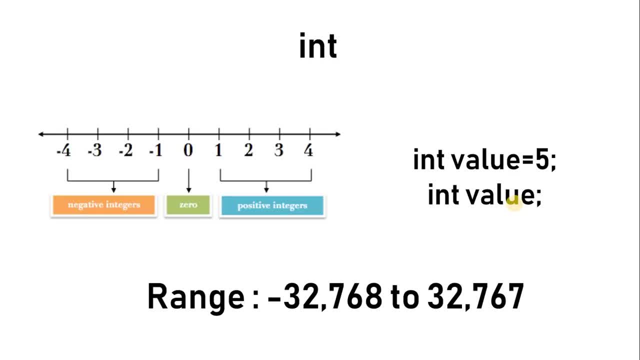 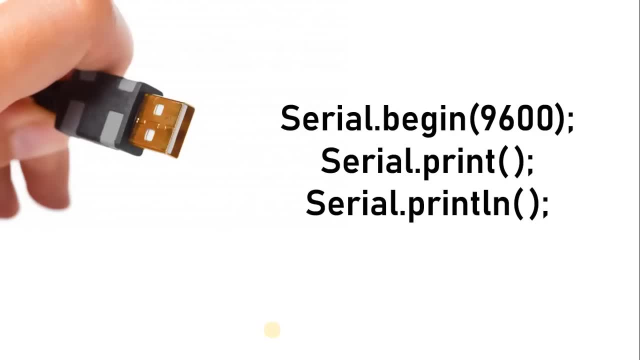 If we do not initialize any value, the default value is 0.. I mean to say, if we do not initialize a variable, The default value which it holds is 0.. We will see more about integers in a moment. So before I can demonstrate how int exactly works in the code, I need you to understand. 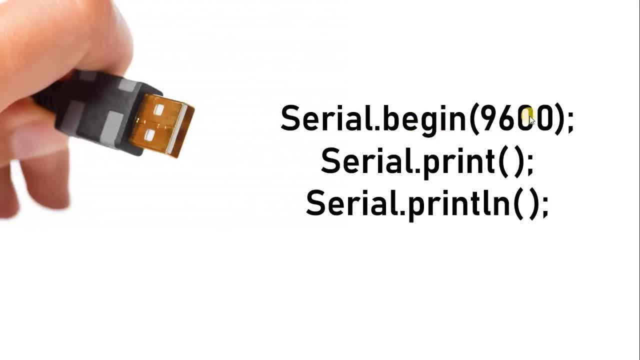 these three critical functions. First, one of them is serialbegin. Basically, this function enables the serial communication between Arduino and the computer. What serial communication is and what these functions are, we will talk in detail in coming lectures. Just understand, we have to write this statement whenever we want any communication to happen. 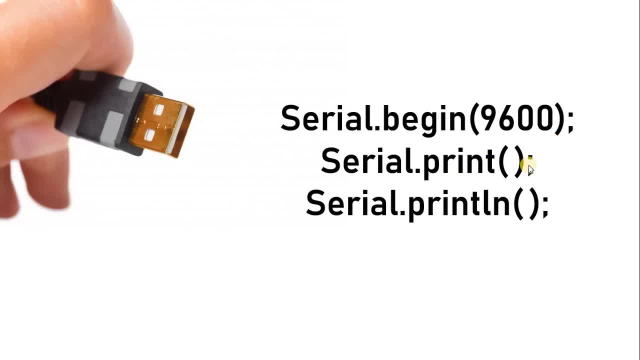 between the Arduino and the computer. Then there is serialprint. we use this function whenever we want to print something on the serial monitor. We will see serial monitor in a moment. And then we have serialprintln. The difference between serialprint and serialprintln is that serialprintln just adds an additional. 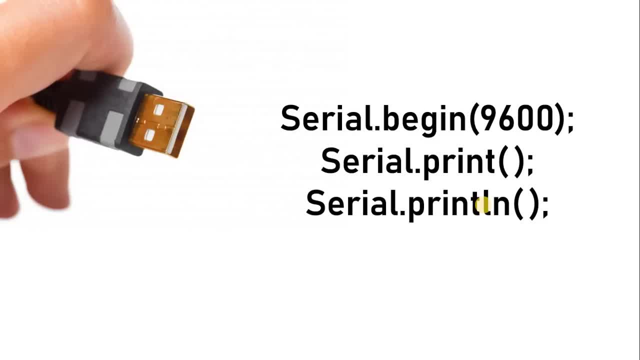 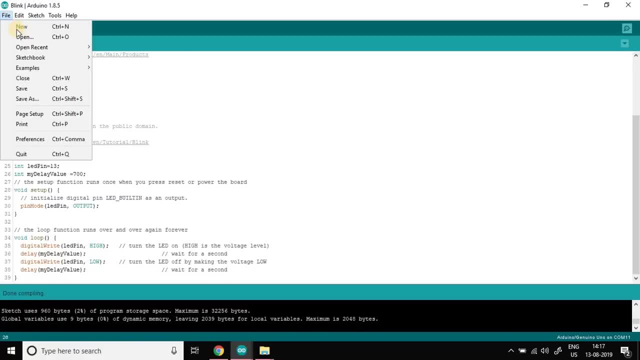 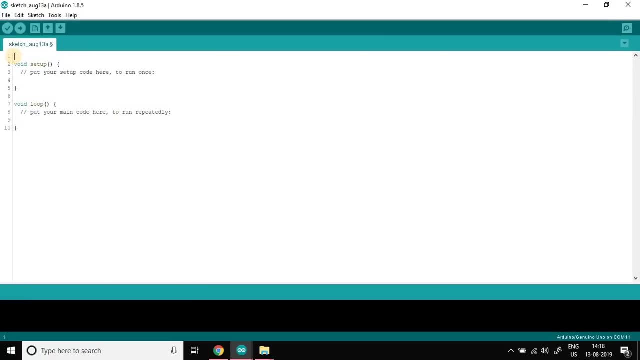 line after printing whatever is asked to print Now, without any further delay. We'll just see How integer works. So now let's start afresh by learning about integers. Let me open a new file. Alright, so I am declaring my first ever integer above void setup like this: int, my variable. 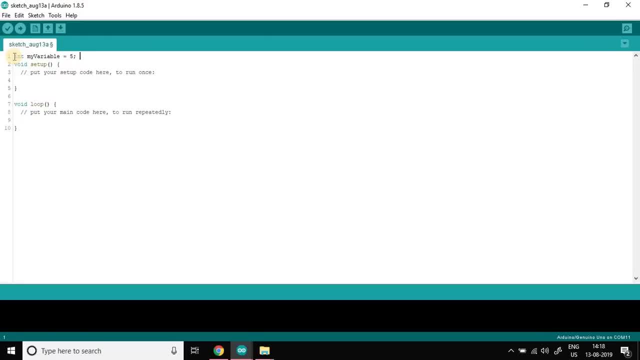 is equal to 5.. It is similar to something which we saw in the presentation when I told you about integers. Now to see the value of my variable, I will start serial communication with my computer. And now to see the value, I will print the value. 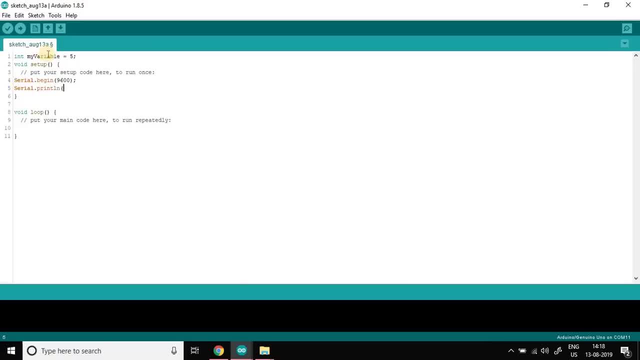 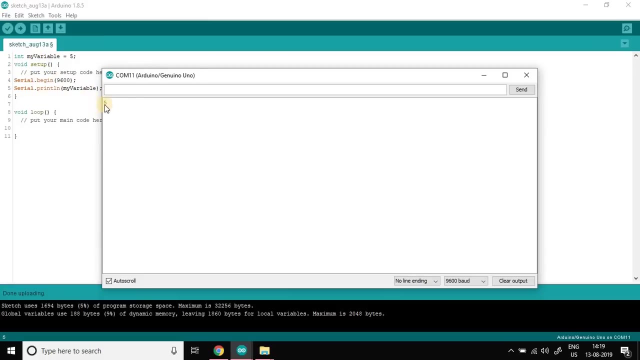 Serialprintln. So now I will upload the code. It is done uploading and now I will see the serial monitor. So you see It has printed the value of 5.. That means the value of my variable is 5, as we have declared. 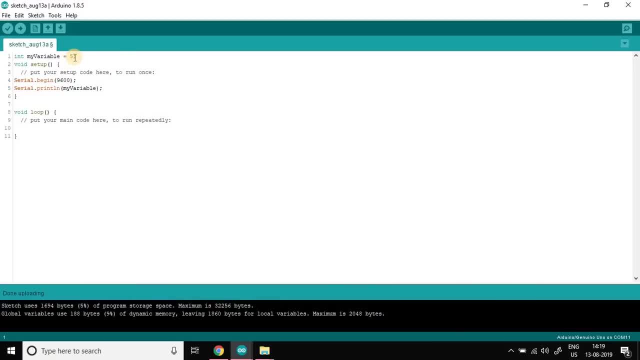 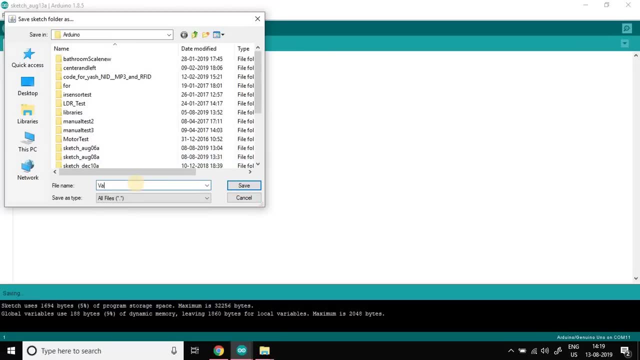 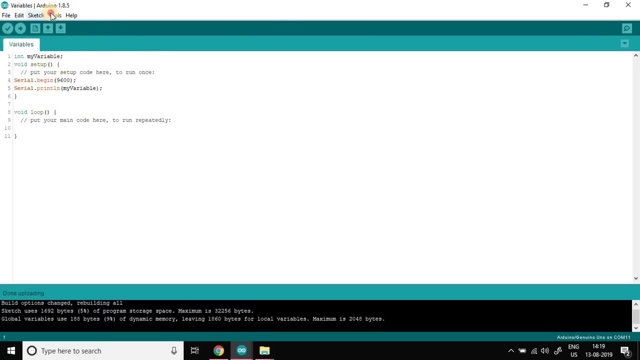 Similarly, when I said, if you don't initialize it, The value is 0, we'll upload the code and see it again. Let me name the file first. Right, if now we have not declared it, so now we will see the value. It says 0. so now I will be telling you about how we can modify our variables, for example, 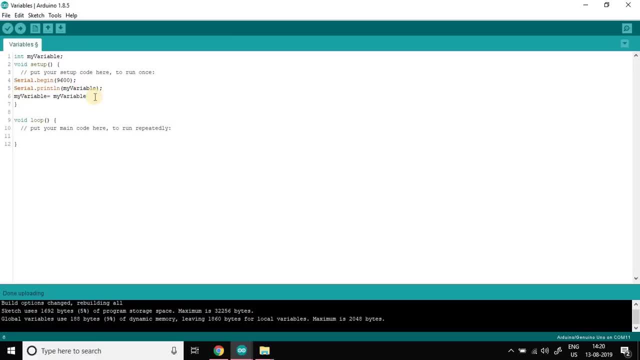 The first thing which we can do is we will take our variable and add 2 to it. So first operator which you see is plus. these are arithmetic operators and we will be discussing more about these shortly now. If we print our variable- Serial dot, println- My variable- 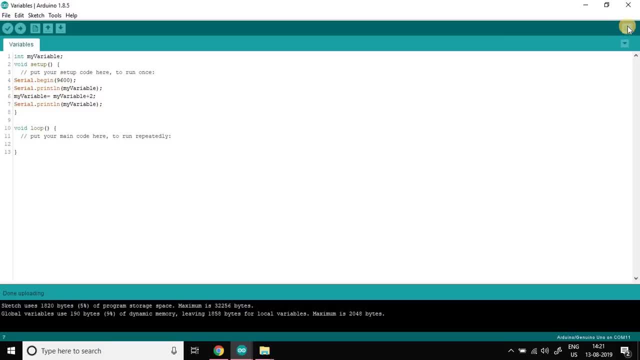 Right, so the answer would be 2. The value of my variable initially was 0 and now we have added 2 to it, So we have 2 here now. for example, If we had initiated it with 5, so now we will get 7 right. 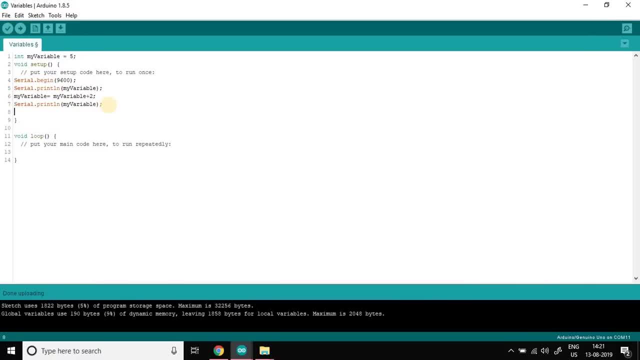 Okay, as expected, now the variable value is 7, right, so now we will manipulate it by Subtracting 2 from it. now again We will get 5. let me tell you that shortcut to open the serial monitor is this button, And then we will print it. 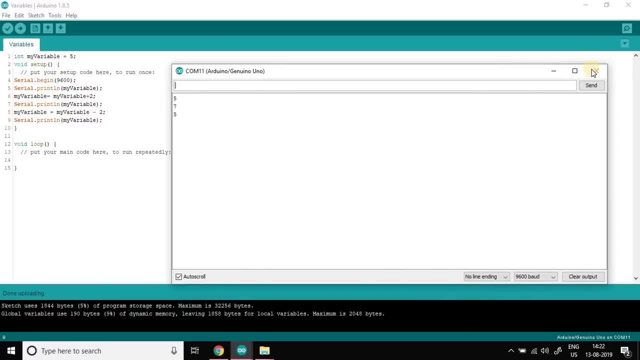 Right, 5, 7 and 5. I hope I'm making some sense. Similarly, there is a multiplication operator and a division operator. What we can do is: Let's say, My variable is equal to my variable into 5. let's say: Now we will print my variable. 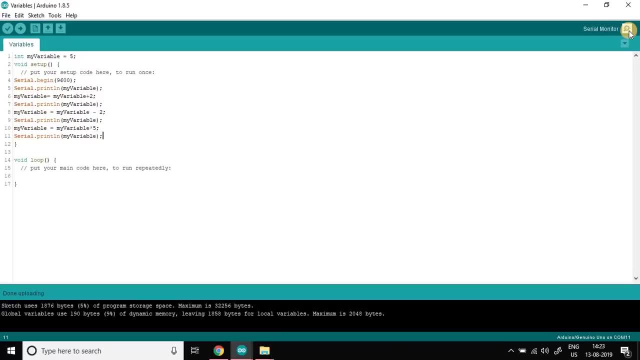 So what will we get? Any guesses: we'll get 25 right. the 5 was the value of my variable and we multiplied it by 5, so we have 25. now let's divide my variable by 25, divided by 20, what will we get? one right. 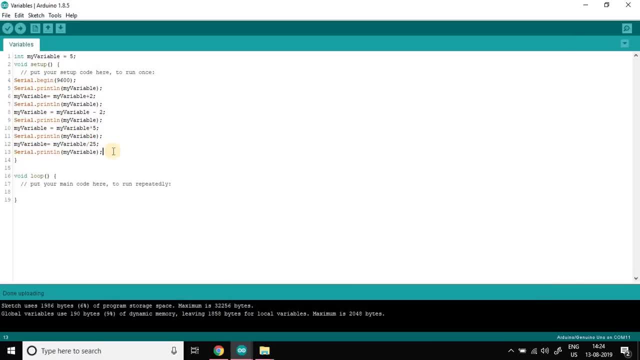 right, we got one. now, the important thing which I want you to notice: the integer variable can only hold integers. it cannot hold fractions. for example, I'll tell you, let me delete all this code. for example, if my variable was 3, right, and what? if we divide my variable by 2, mathematically, the answer should be 1.5. 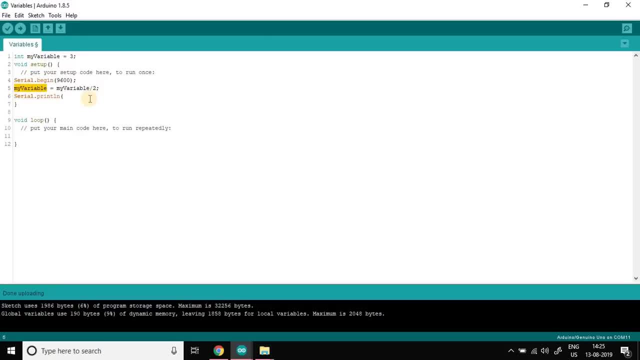 but since our integer variable can't hold decimal values, so can you guess what will it print now? it will print 1, why? because it can only hold integer part of any decimal. the answer was 1.5, but it will pick only the integer value. so if you want decimal values as well, 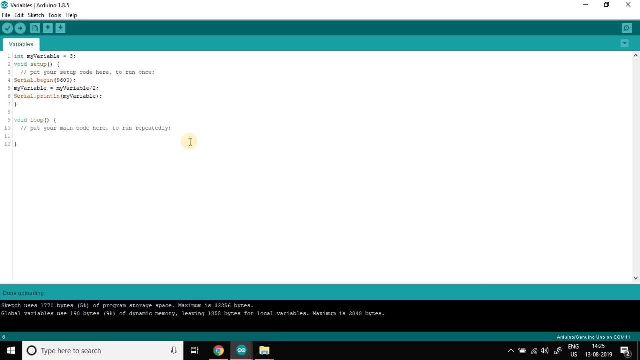 we will use float and we will soon learn about float. now there is another interesting operator known as modulo. it will give us the remainder after division. let's say my variable is 6- okay, and I want to get the value of the remainder. we'll say: my variable is equal to my variable modulo. 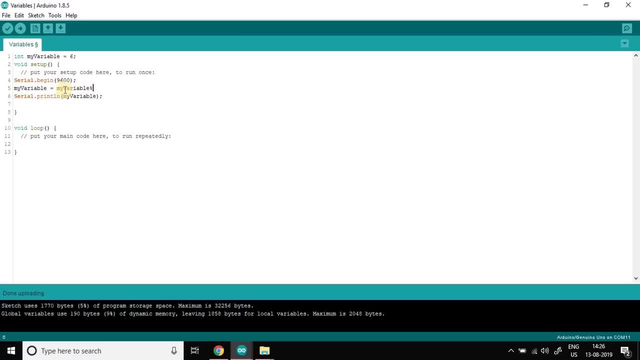 the symbol of modulo is percentage sign. if we divide 6 by 2, so it will completely divide by 2, right? so the remainder will be 0. so if we print my variable, we should get a value of 0, right, as expected. if we divide 6 by 3, then also we'll get. 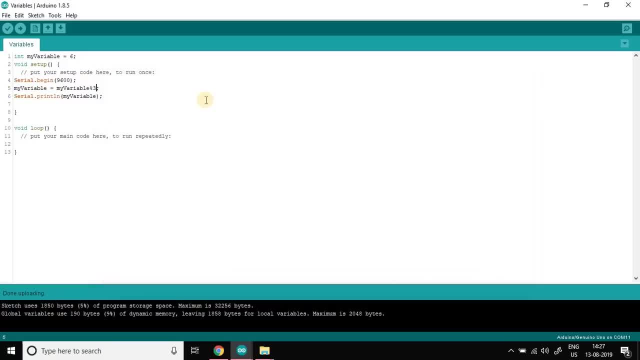 a remainder of 0. but if we divide 6 by 4, we get a remainder of 2. right, we will get 2 here now, as expected. now can you guess what? if we divide it by 5, what remainder will we get? we'll get 1 right, as expected. so these were the main. 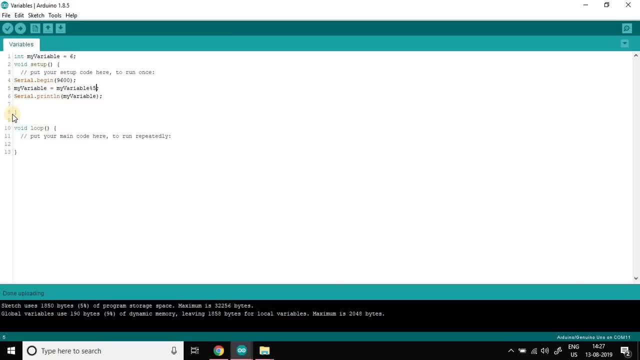 arithmetic operators which we can use to modify our variables. now, for example, if you want more than one, the same the formula code we can take one. we can say my Pool and our cod co. that followed by my second variable. we have more than one variables in our code: my second variable and the 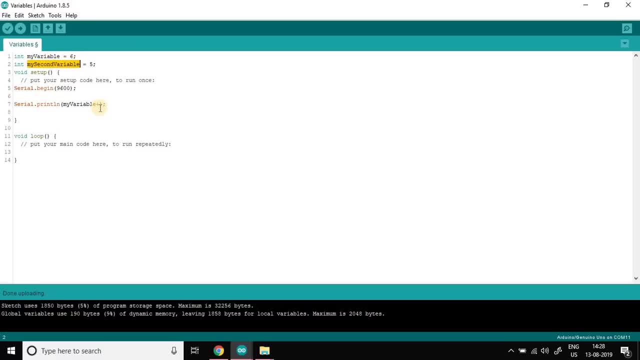 value of that is 5. now what we can do is: now let's see what will we get. my variable plus, We'll get 11 Right as expected. and what if we subtract it? Are we correct? absolutely similarly, we can also multiply. What should we get? 6 multiplied by 5 is 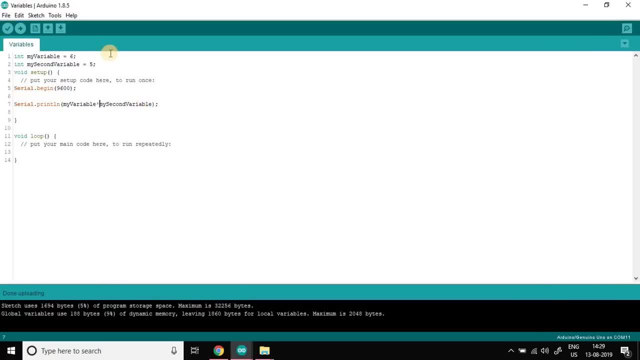 30, right? What? another thing which we can do is we can store these values Here. our results are not getting stored here, They are just being displayed. What if we want to store it? we can take another variable, my third variable, and let's not initialize it. 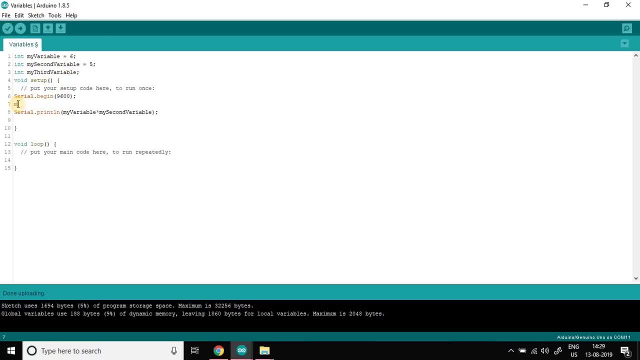 Okay, so what we can do is: Let's take my third variable, Okay, and let's store the value of my variable, And let's print the third variable Plus my second variable And let's print The third variable. we should get 11 here, exactly. So, similarly, we can do whatever we want with the variables. 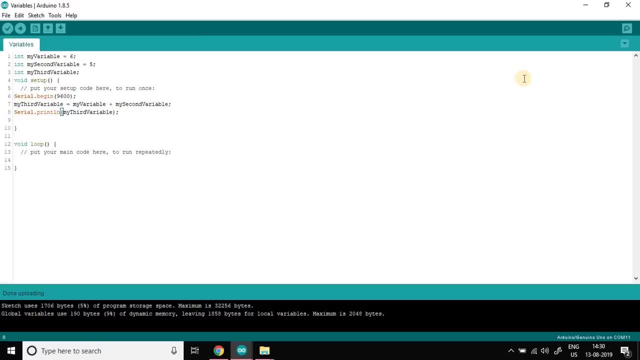 But the most important thing which I want you to notice is, before using the variable, we have to declare it. for example, if we do not Declare my third variable Okay and Try to do something with it, The compiler will throw us an error. My third variable was not declared in the scope. 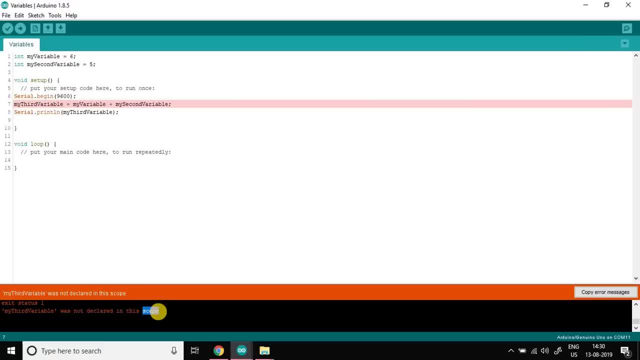 Alright, we'll discuss about scope in coming videos. Just wait for some time. You also need to note that you have to declare the variable before using it, right? You cannot do this as well. For example, you try to declare your third variable here. 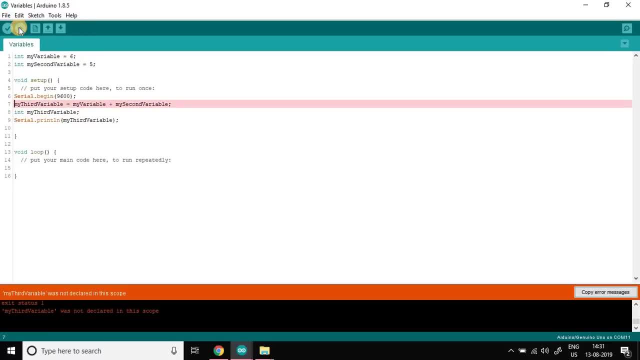 right, then also We'll get an error. you have to declare it Before using it. You cannot declare it after using it, right? The last important operator which you need to know to be comfortable with the course is the increment and the decrement operator. There are two types of each. one is post increment and pre increment and post decrement and pre decrement. 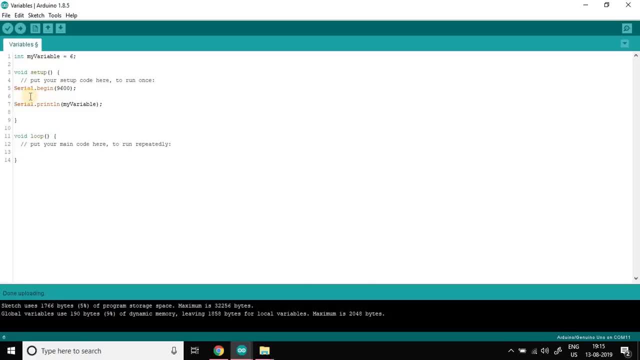 alright. the purpose of increment operator is to increase the value of variable by 1, and the purpose of Decrement operator is to decrease the value of our variable by 1. I'll show you this By an example. we have my variable and the value of my variable is 6. 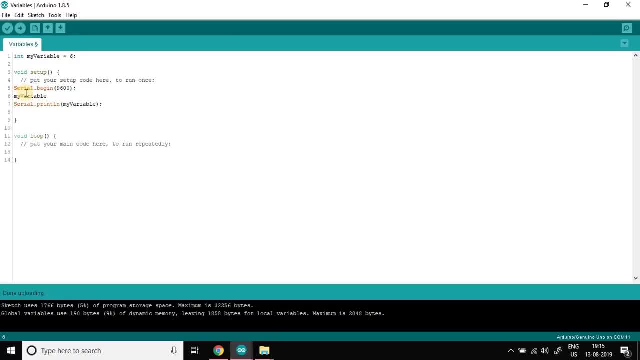 So now if I take my variable and do plus plus, this plus plus is post increment operator. Okay, and now if I print my variable, you will see that we will get 7 Right. so now If I use pre increment operator, then also will get the value of. 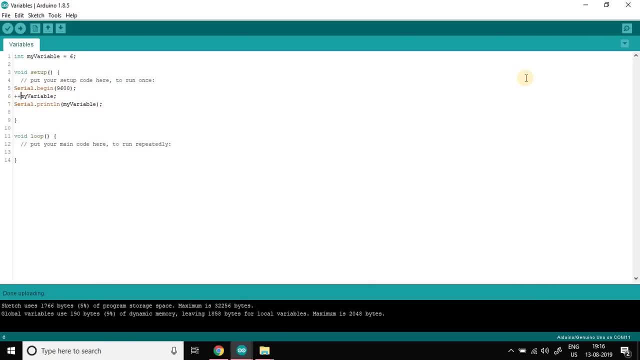 7: see. So now you may ask what is the difference between post increment and pre increment? Well, there is actually a difference, and you will get to know that difference when we use this operator in some expression. for example, Let's see it here: If I increment the value of my variable like this, like you seen, serial print, Ellen, then we will get value of 6. 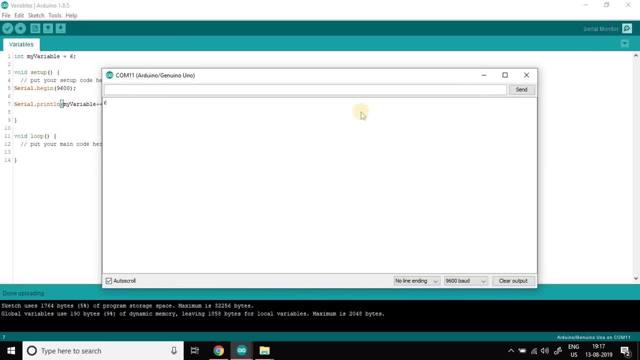 Right, as you can see, And the reason behind this is in a post increment operator the value is first used in the expression and then it is incremented. Now, if I use a pre increment operator, then we will see we get 7.. So by this we can understand: by pre increment operator the value is first incremented and 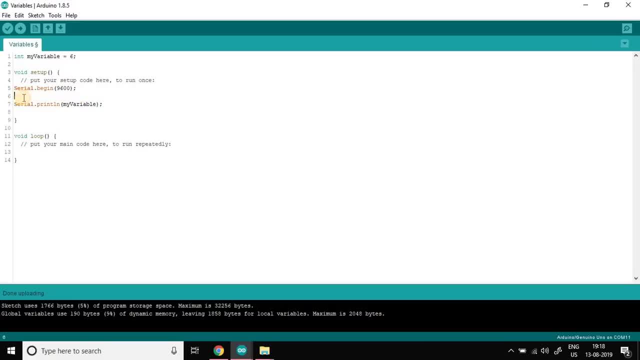 then used in the expression. Similarly, there is a decrement operator. If I do my variable minus minus, we will get 5, because my variable was originally 6, so we decremented it by 1, so hence we get 5.. I hope this concept was clear to you. 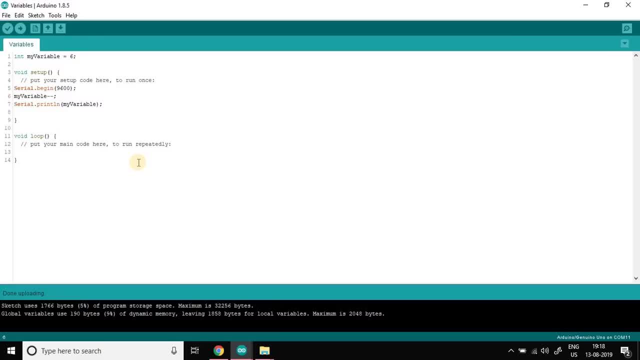 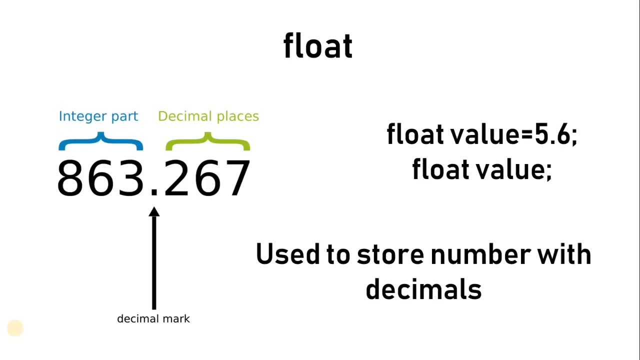 This concept will be used multiple times during our course, So if you have any questions, you can comment down below, And in the next video we will look at the float data type. So now we will look at the float data type. This data type is capable of holding decimal places as well. 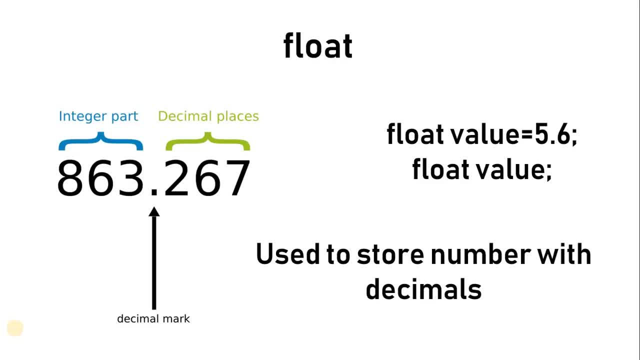 Like we saw in the integer, it cannot hold decimals. The float can hold decimals as well, And the default float which we use in Arduino programming is precise up to 7 decimal places. Let me explain you in a better way. Like, for example, the number you see here is a real number. 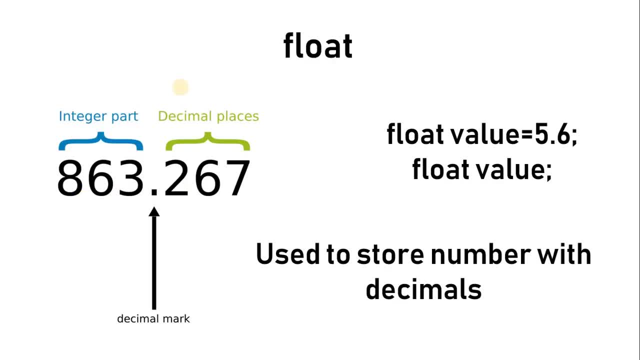 It is 863.267, right? So in integer, if we try to store this, that would store only 863.. It will just ignore 0.267.. So if you want to use 0.267 as well in our memory, so we will use a float data type. 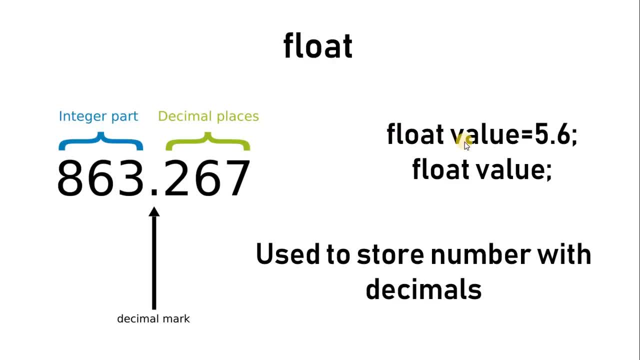 So how do we declare that? we write float, then space and the name of that float variable. In our case it is value equals to 5.6.. Or some other value, The value which you want, Then a semicolon. You can also start a float uninitialized. 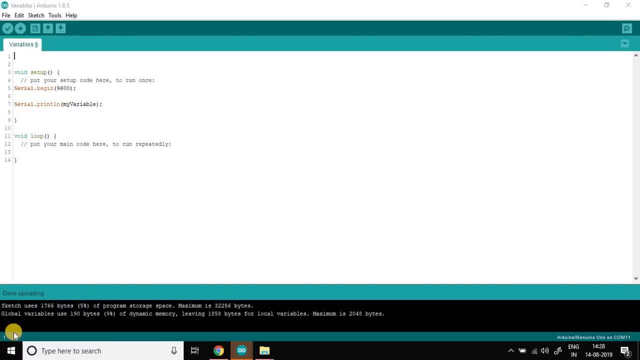 Like we have done here. So let's now see the demonstration of how float is used in our programming. We will declare the variable. myFloatVariable is equal to 7.8, for example. Let's see right, we can see the value of 7.8.. 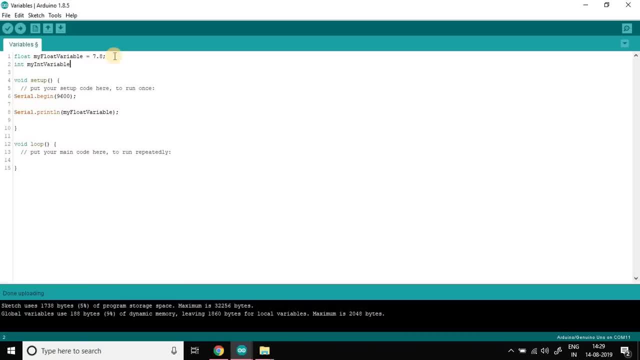 Now let's see what happens if we try to Store 7.8 in an int variable. As I told you in the presentation, we will get 7, right? Can you see the difference now? Now we will just quickly see the limitation which we had while using int variable that. 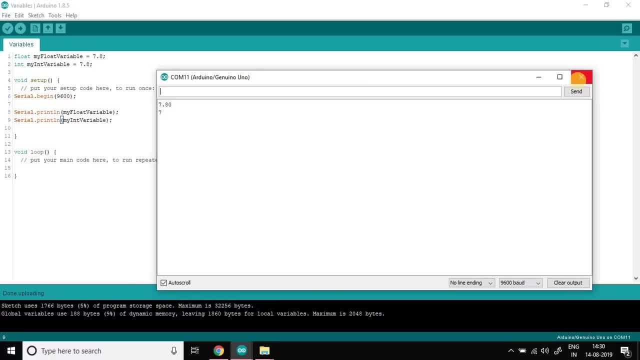 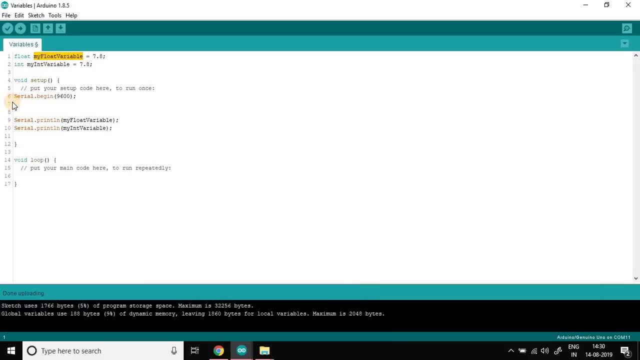 while dividing, We could not store The decimal part, So we will see if we can store that in float variable or not. Let's see it quickly. I'll take my float variable And I'll divide it by 2.. Okay, 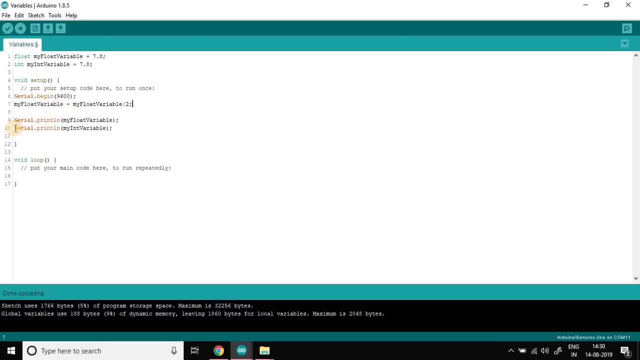 We will see the myFloat variable. then Let's comment the statement. All right, 7.8 divided by 2 is 3.9.. We can use all the operators, We can use all the data which we used in the int variable, like plus, minus, divide, multiply. 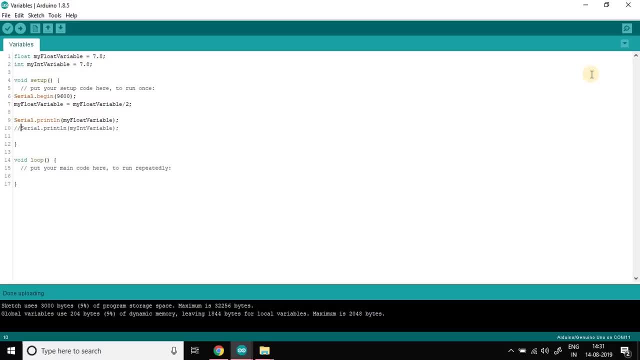 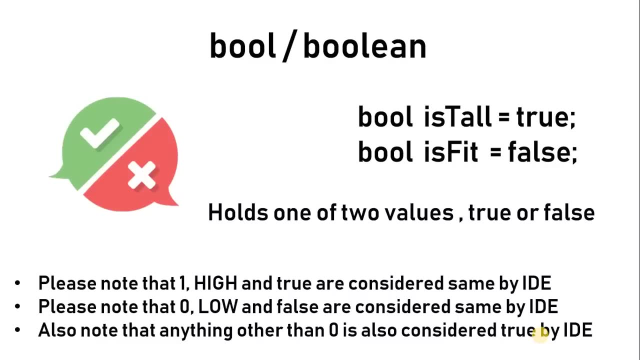 increment, decrement and floats as well. Okay, So you can try that on your own and comment down below if you face any problem. So now we will take a look at the bool or boolean data type. They can be used interchangeably, right, but we prefer to use bool. 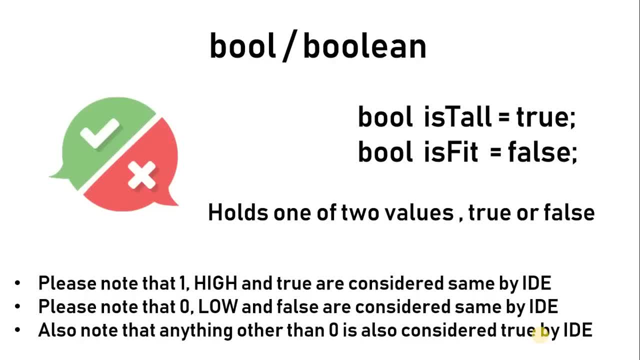 So the bool data type holds one of the two values: true or false. That means If something is true or if something is false. For example, we can declare a boolean variable by writing bool. then the name of the boolean variable- in our case it is isDoll- equals to true or false. 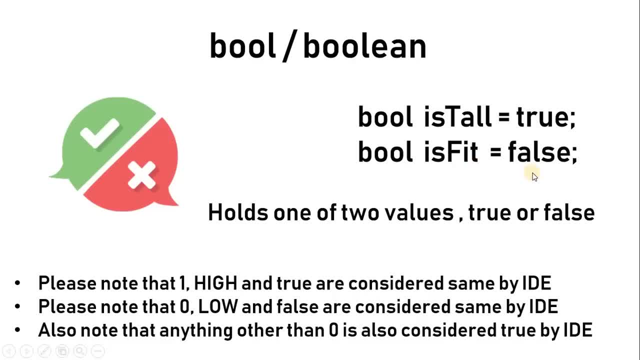 We will take another example. bool isFit is equal to false semicolon, So this way we can declare a boolean variable. but I want you to notice that one high or true by the ID, also 0, low and false are also considered same by ID. by ID I mean the. 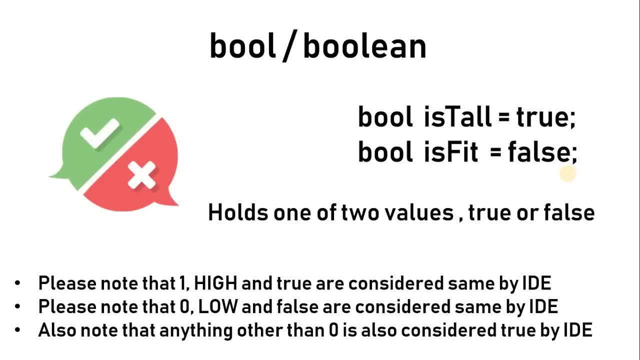 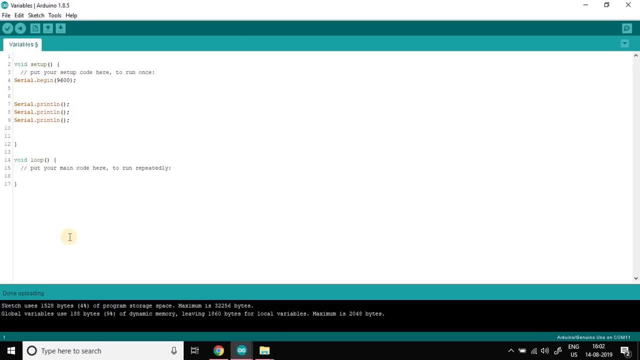 Arduino ID right and anything other than 0 is also considered true by the ID. we look at what exactly this means in the coding. now let's understand the boolean variable in the coding. we will initialize it by writing bool. we will then name it and initialize the value of say 1, as I told you: 1 high or true all. 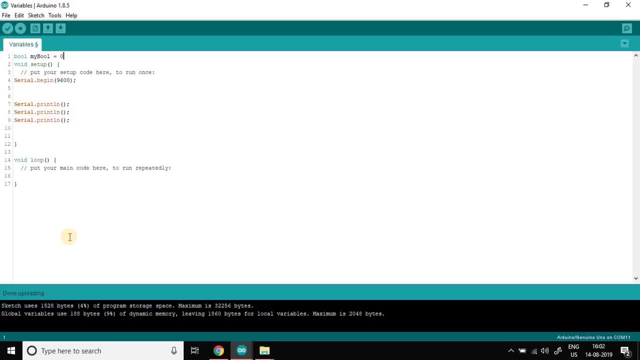 these three hold the same meaning. and similarly, 0, low and false all hold the same meaning. if we try to print the variable, let's see what happens. it will print 0, right, because false is true and false is false is true and false is true. if we use low, then also it will print 0. same goes for true. if I use true here, 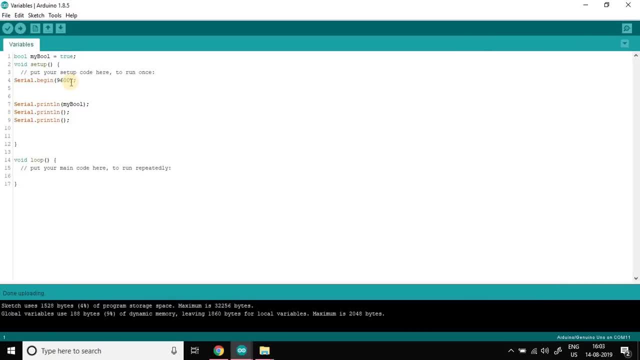 it will print 1. and the other thing which I told you: if we use anything other than 0, that would evaluate to 1. let's see that also. for example, I used 78. let's see what happens. it still gave 1. okay, so that means bool can either. 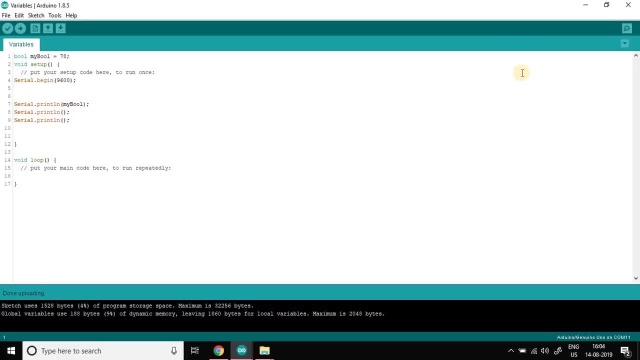 store 0 or 1. that's all. and what's the purpose of boolean operator? we check if something is true or false, and if it is true then it will print 0 and if it is true in the code. we'll see examples while doing our experiments shortly. I 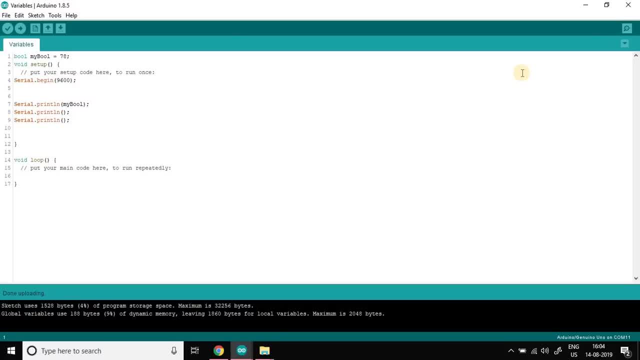 will like to tell you, if you want to check some condition is true or false, or we can initialize our condition as well. if something is true, then only we have to do certain task. you will understand more about boolean data type when we progress in the course, like when we study about conditional or when we 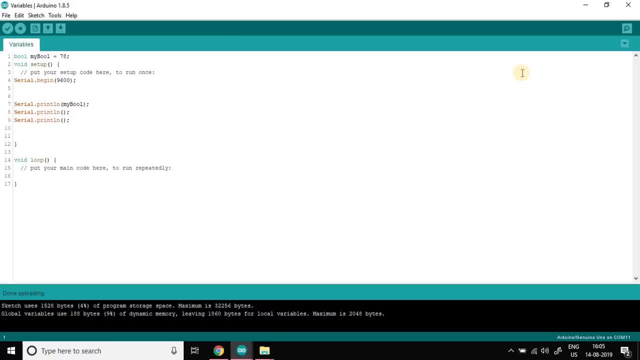 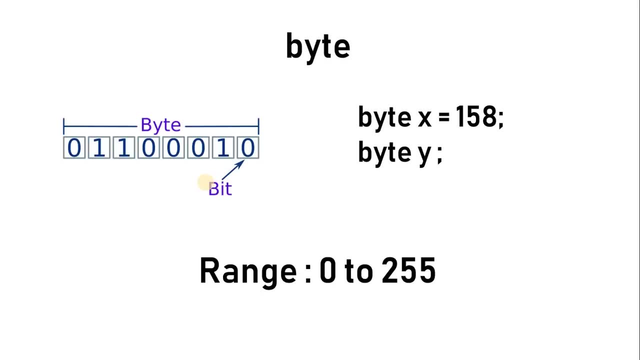 study logical operators or when we study the comparison operators. we will now move on to another data type, which is known as byte. the next data type which have is byte, so, as the name suggests, it is a byte long data type. it can store up to 8 bits of data, so, as we all know, 8 bits equals to 1 byte. okay, so a byte is. 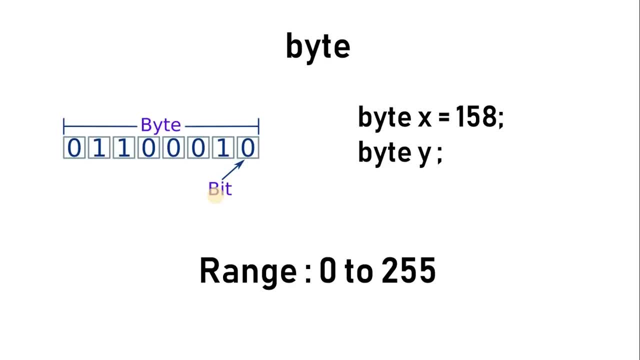 just like an integer, but the only difference is the range is 0 to 255. so if you're sure that your variable is not going to exceed 255, you can always use a byte type data type. so using a byte data type will save your Arduino memory. so 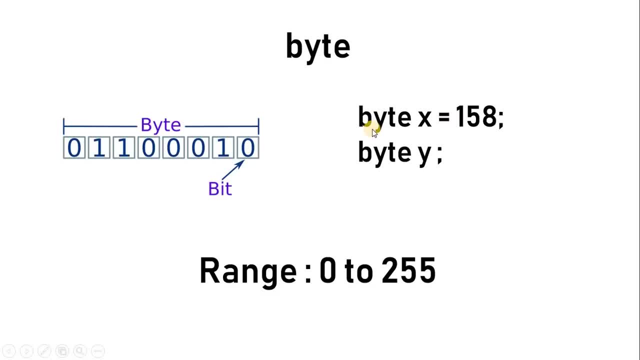 we will now see how to declare a byte. we will write byte space, name of the variable equals 2 and the value which we want to add in that, then a semicolon. we can also declare it without initializing the variable, and in that case the default value it will store is 0, just like integer. so let's just quickly. 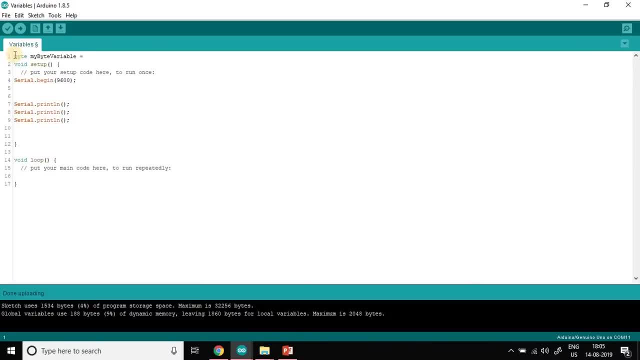 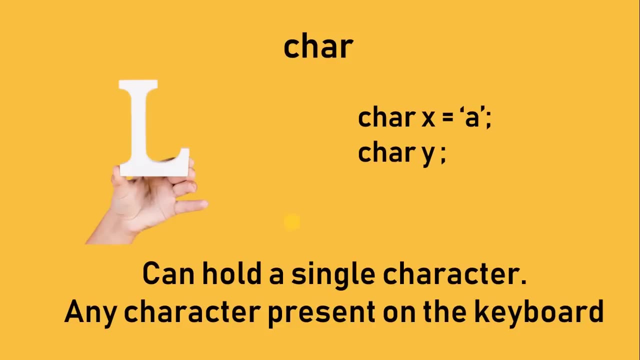 declare our byte and let's print it just like that, right so now we will look at our next data type, which is char, which is a short for character. as the name suggests, it can hold a single character, any character present on the keyboard, for that matter, including all. 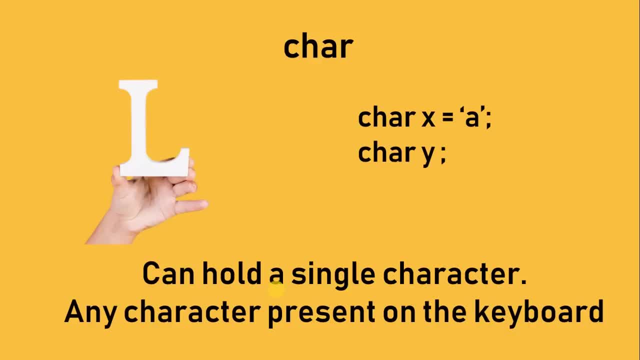 the symbols like Comma, question mark, numbers like 1, 2, 3, characters like ABC, small caps, everything. Let's see how we declare a character. we write char space- name of the variable equals 2 characters- and then enter char space space. in the first case it is a comma. so this is how we declare our character. 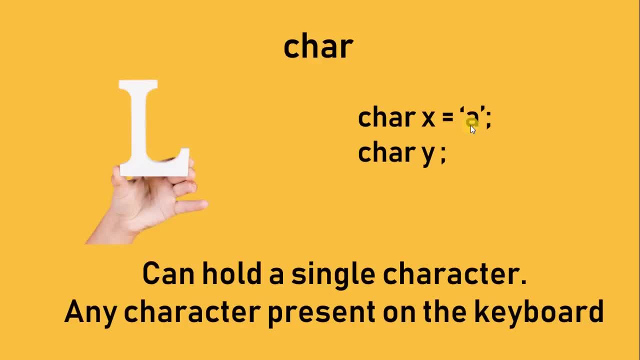 space. name of the variable equals 2 characters and then it is a semicolon. we to and the character which we want to use and that is enclosed in single inverted commas and then a semicolon. We can also declare our character like this, as we have seen it many times already: 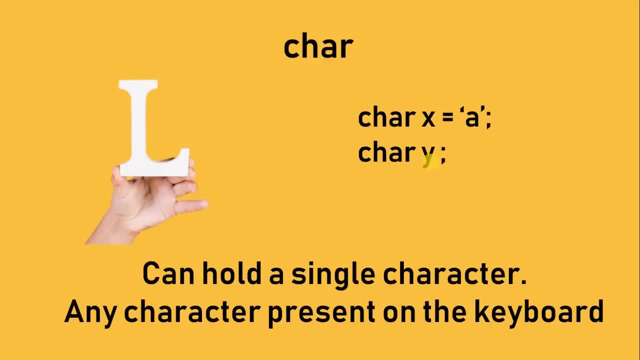 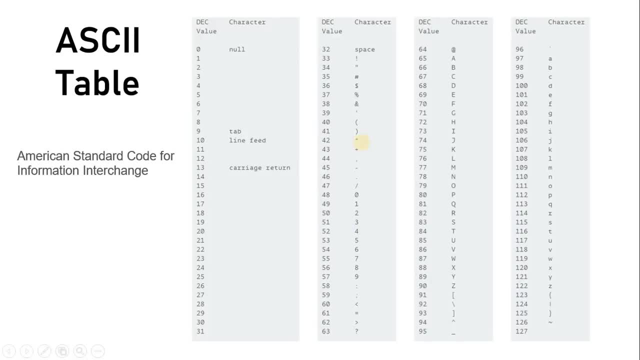 The thing to note about characters is that it is still stored as a number. What I mean by that is there's a full ASCII table. Each character on the keyboard corresponds to a number. For example, you can see a capital- A is 65- and a small- a is 97.. Similarly, you can see the entire table. 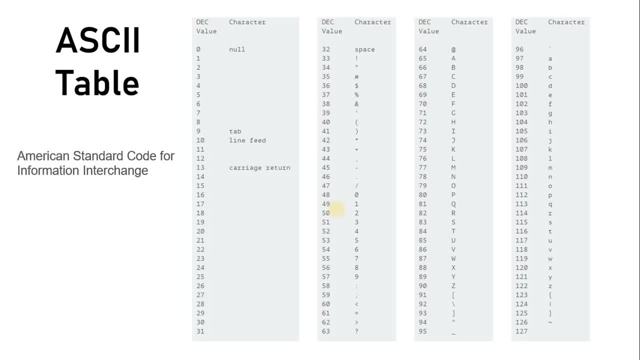 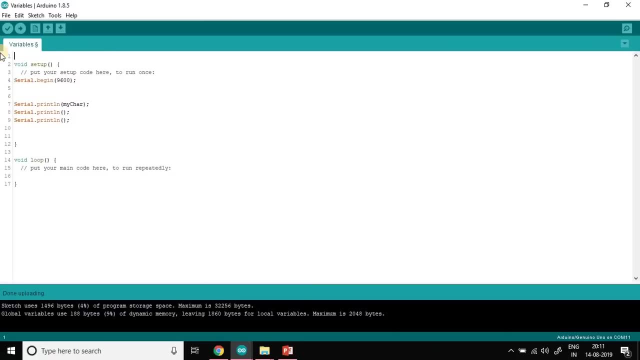 It contains all the characters which are present on the keyboard, and each character has its own number. We'll look at this in a bit more detail. using our coding, We will declare a character char. myChar is equal to 65.. Now we will print it Right. We get an A Now if I write 65, which is the ASCII value of. 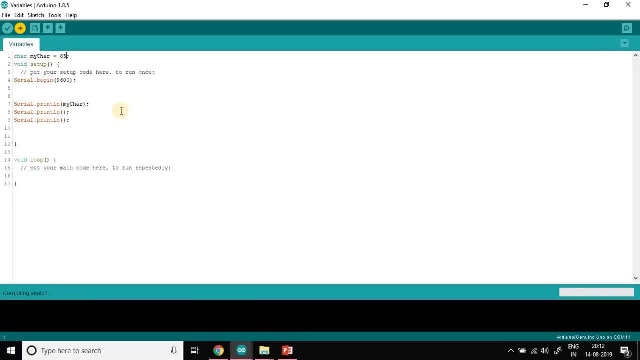 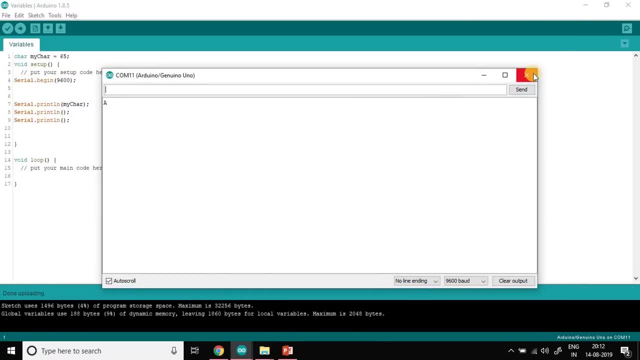 capital A. You can refer ASCII table to verify. Then also it will print A. Let's have a look Right, It printed A. Now still, these are numbers. That means it should be possible for us to perform some arithmetic on that. For example, if I take A here: 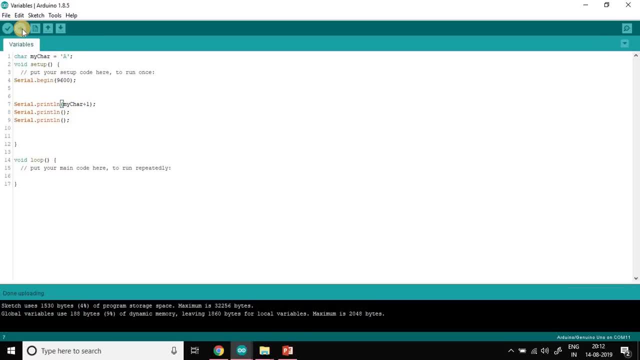 and add 1 here, Right? So what should we get? We should get 66, as expected. Why? Because the value of A was 65 and it added 1 to that, So we get 66. Right. A char data type occupies 1 byte. 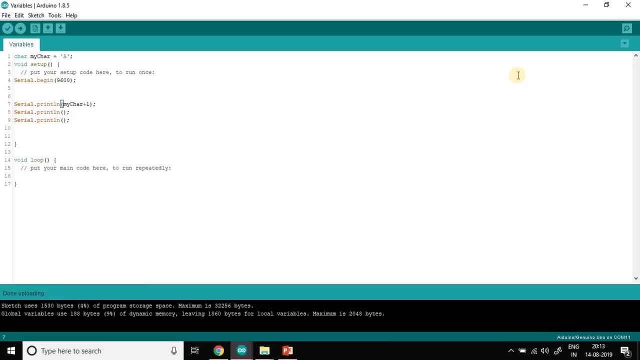 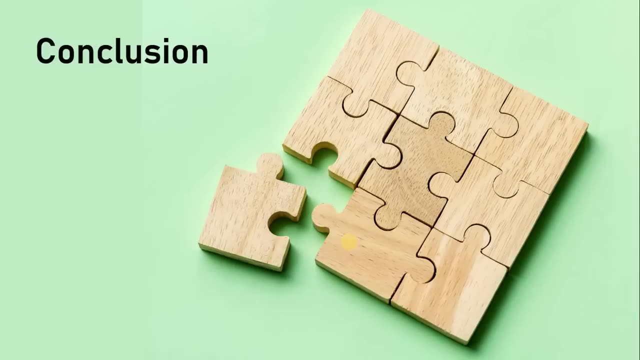 in the memory. Okay, So I hope you understood the char data type. I can understand. if you got a bit confused with the character arithmetic. Don't worry about that right now. This information is enough to start our projects Now. we have discussed all the important data types like int, float, char, bool, byte And you. 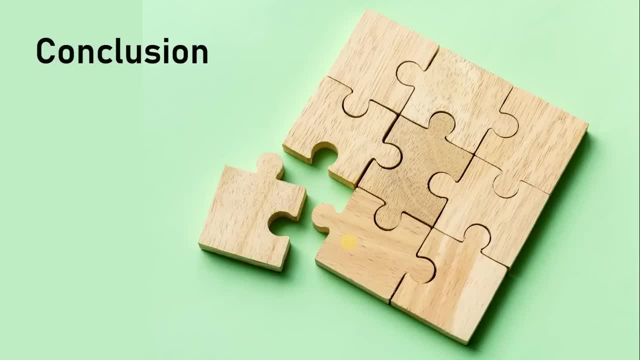 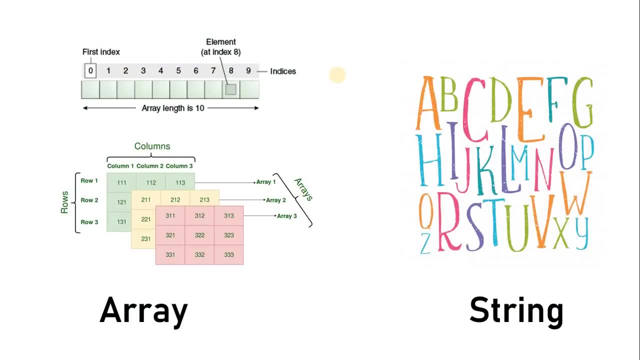 have also learned when to use which type of data type, So I am pretty sure that you won't face any issues while performing your experiments, Although there are more data types, like arrays and strings, which are slightly more complicated than data types which we have already discussed, And they 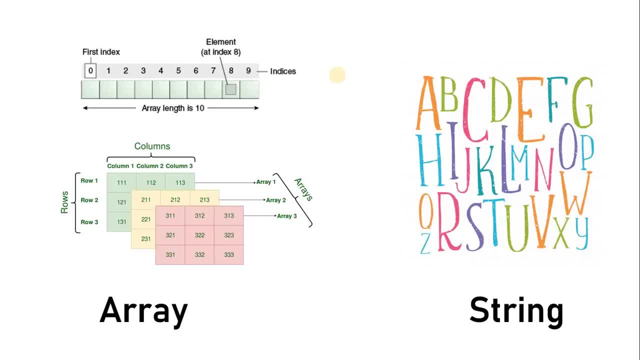 would also involve the usage of loops, So we will cover them after discussing loops, as that would make it easier for you to understand. For now, we will move on to our next topic, which is Variable Scope and Qualifiers. See you in the next video. 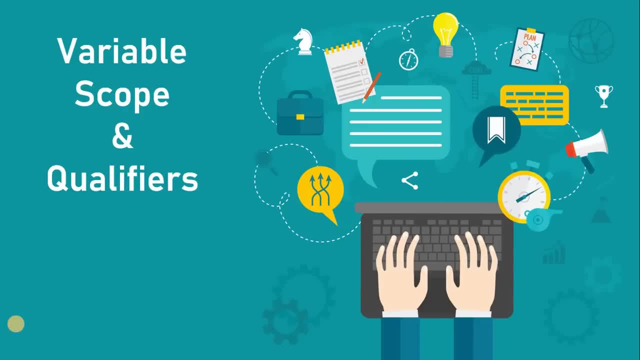 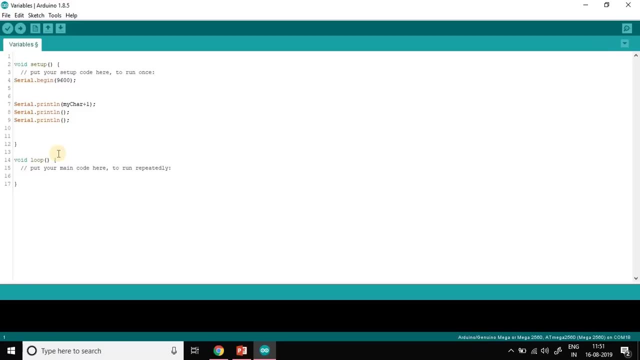 Now, since we are familiar with the data types and what variables are, we can easily understand what is variable, scope and qualifiers. So let's start by understanding what is scope. In many programming languages, including Arduino's programming language, it matters where you have declared. 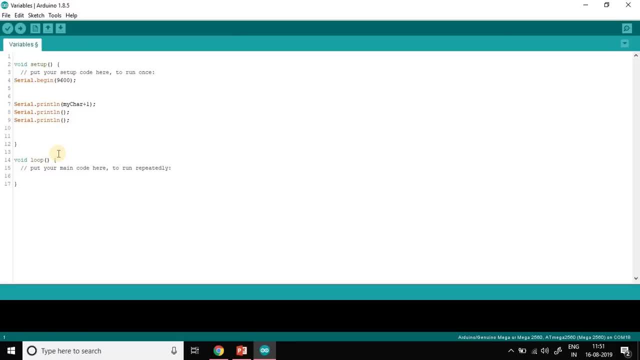 your variable. Speaking of which, we have two kinds of variables: global variables and local variables. A global variable is the one which can be seen by every function in the program, While local variables are only visible to the function in which they are declared in the Arduino. 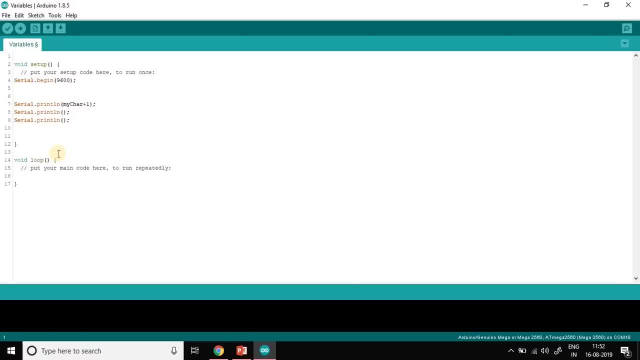 environment. Any variable declared outside of a function, for example void setup or void loop or any other custom function, is a global variable. So let's start by understanding that in a proper manner. So what positions would qualify for writing a global variable? The first position which we see: 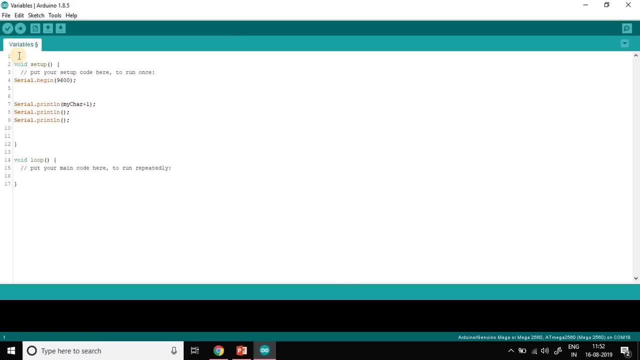 is just above void setup, the place where my cursor is blinking right now. For example, I write int, my variable is equal to 6.. So in this case I will write int: my variable is equal to 6.. So in this case my variable is a global variable. As I told, the global variable is accessible in all the 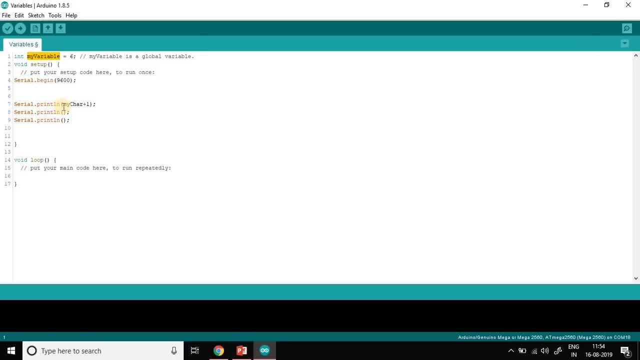 functions. Let's see that by printing my variable in void setup, It will print here as well. It will print in void loop as well. Let's make an identifier so that we can identify in which function it got printed. Serial dot println. printing in setup. 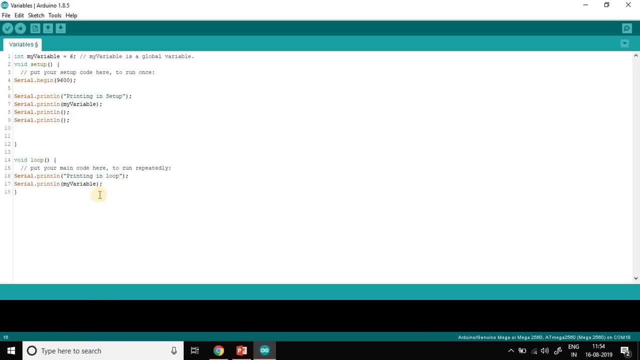 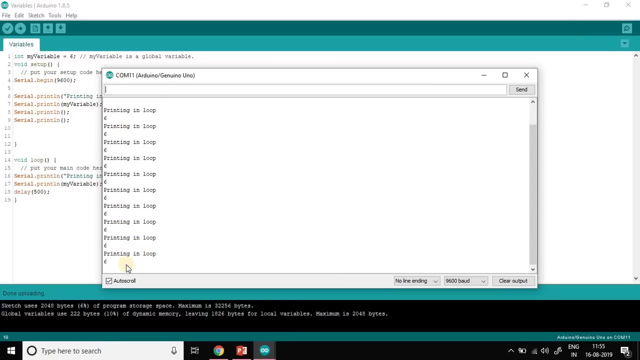 And let's differentiate printing in loop- Alright, let's have a delay here because it will print very fast otherwise. Okay, let's see that now Right: Printing in setup and printing in loop. It is printing again and again because we have written that in loop, As we already know. 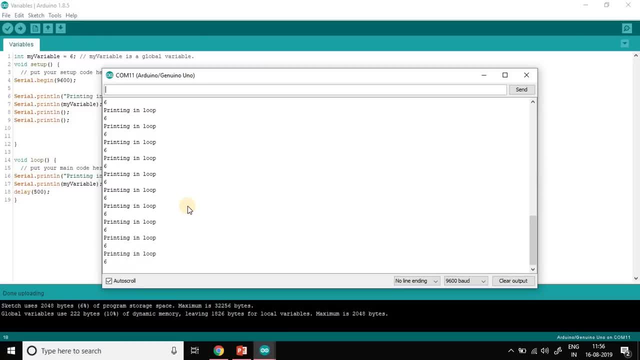 loop function will run until and unless we turn off the Arduino. So that means my variable could be accessed by void setup as well as a global variable. So let's differentiate printing in loop As well as void loop. That means this is a global variable, Now we will see a local variable. 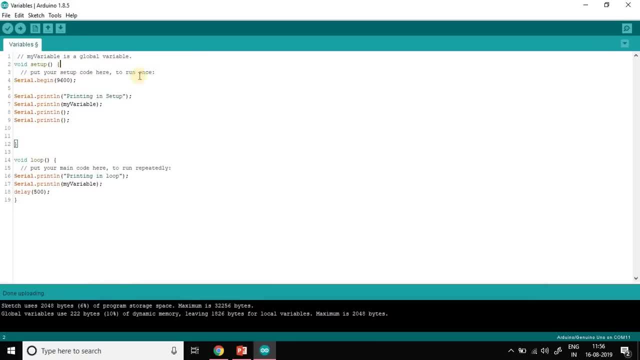 Instead of declaring it above void setup, let's declare it in void setup. So now let's try to compile this. We should get an error Why? Because my variable was not declared in the scope. It is saying: in void loop you did not declare my variable, So I don't know what my variable is. So 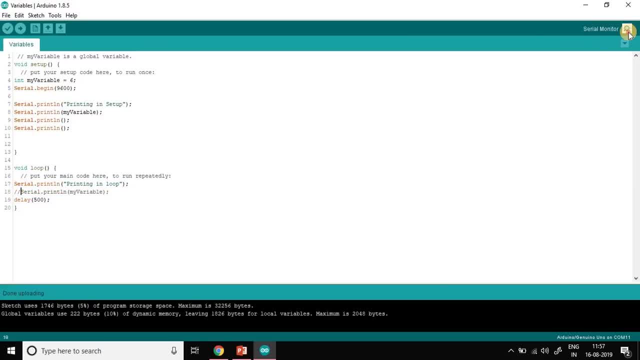 let's comment out this line: Now it will compile. Okay, it compiled successfully and it will just print in setup once. Right, So now it will compile successfully and it will just print in setup once. If we declare my variable in void loop and just uncomment this line Now, we will get an error in. 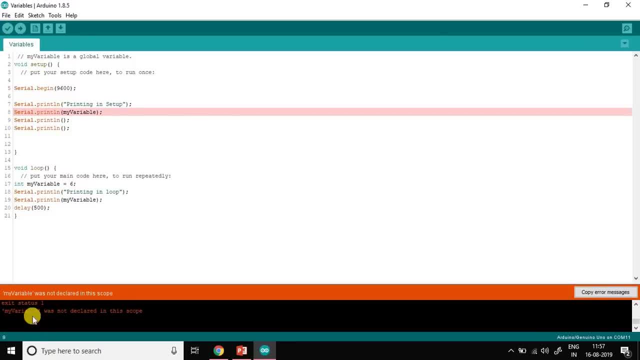 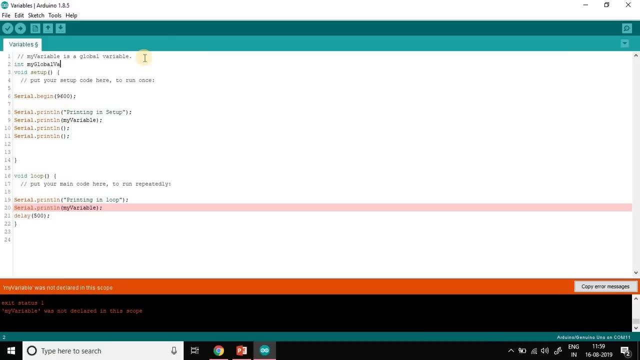 void setup because it was declared in void loop but it was not declared in void setup. You see, in void setup my variable was not declared in the scope. Now let's see a consolidated example of using global and local variables together. The variable which I declare here is in my global. 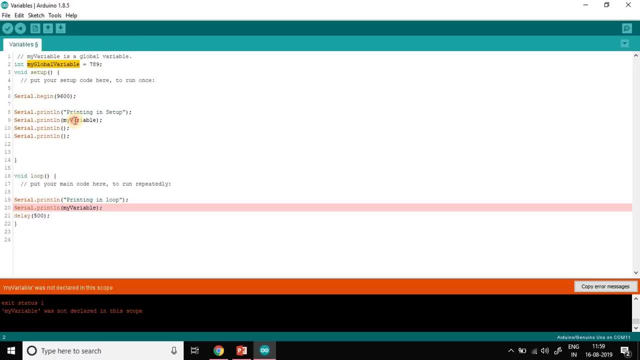 variable is equal to 789.. So let's print it here and let's also print it here. Okay, this one is accessible to both void setup and void loop. Let's declare a local variable here and my local variable is equal to 852.. So this is a local variable and it will be accessible only to void setup. 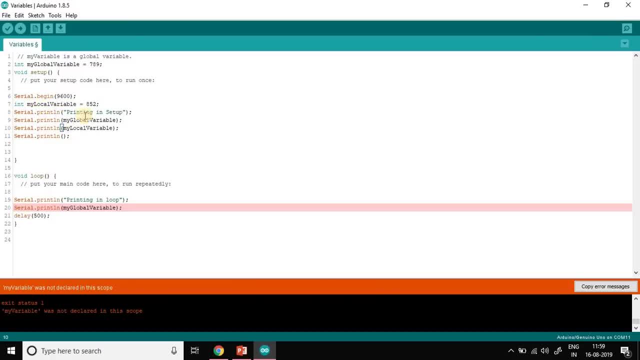 Now let's try to print this: my local variable. Note that we can use same names if we are using a different scope for a variable. For example, we can use my local variable in void loop as well, and we can give it a different value. 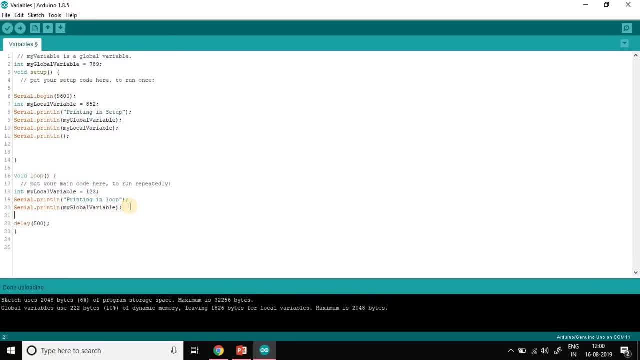 123, for example, and let's print this as well. So what should be the expected result? When we print my global variable, it should print 789, and when we print my local variable, when the code is running in void setup, it should print 852, and when it is running in void loop, it should print 123.. So let's 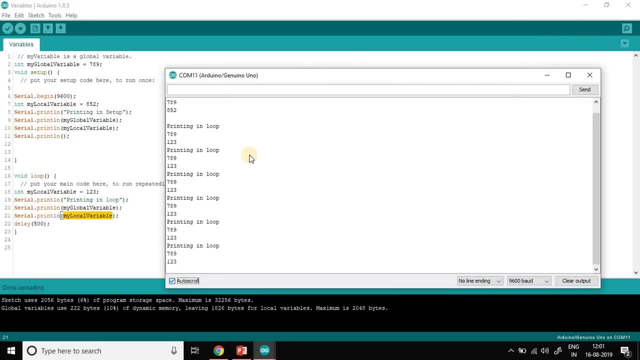 upload this code. Is that as expected? Let's see Printing. in setup, it printed my global variable, which is 789, and my local variable, which is 852. right Now, in printing in loop, it printed my global variable 789 and my local variable, which was 123.. So I hope you are clear with the scope of the variable. 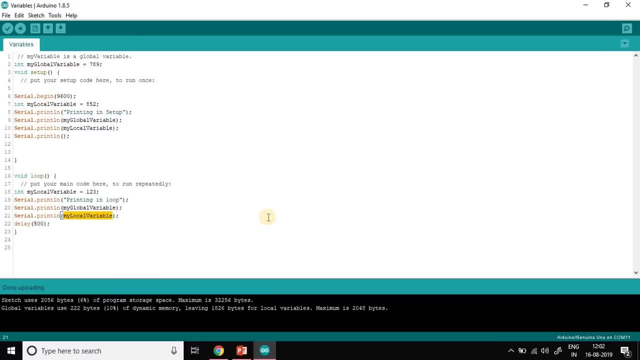 When programs start to get larger and more complex, local variables are useful way to ensure that only one function has access to its own variables. This prevents programming errors when one function modifies the variables used by other functions. This concept will get clearer to you as we progress in the course. So now we will look at qualifiers. Qualifiers basically define additional. 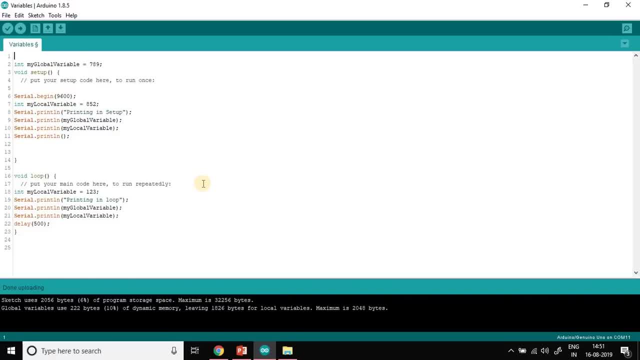 behavior to our variables. There are two main kinds of qualifiers: One is constant and one is static. The constant qualifier is declared by using const keyword. It is a variable qualifier that modifies the behavior of the variable. It is a variable that modifies the behavior of the variable. 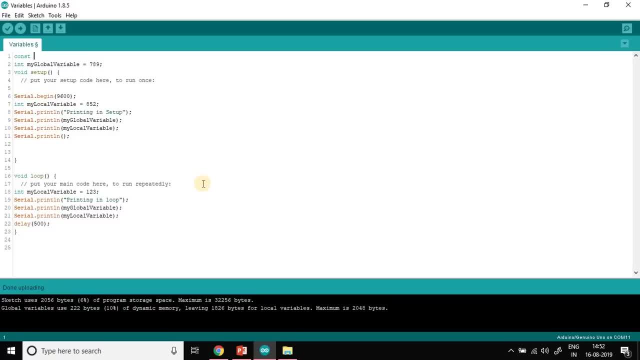 Making a variable read only. This means the variable can be used just as any other variable of its type, but its value cannot be changed. You will get a compiler error if you try to alter a value to a constant variable. We will just see by an example. We will declare our variable constant. 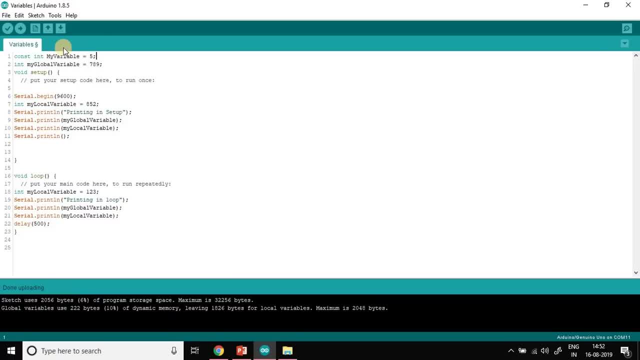 int. my variable is equal to 5.. Now, my variable is a constant integer. You cannot add anything to it, You cannot subtract anything to it, You just can't alter it. Now, let's try to alter it, Let's see what happens. 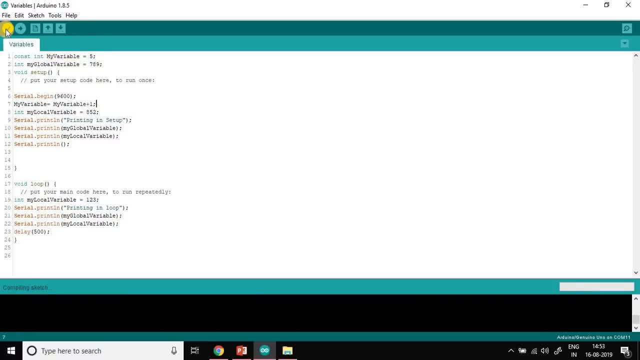 You can create your ratios and add holidays to employee variables on the column and convert these values to seconds. We got a error. Self happened. assignment of a read only variable- my variable. However, you can use constant variables for doing the math. For example, I take another variable here. 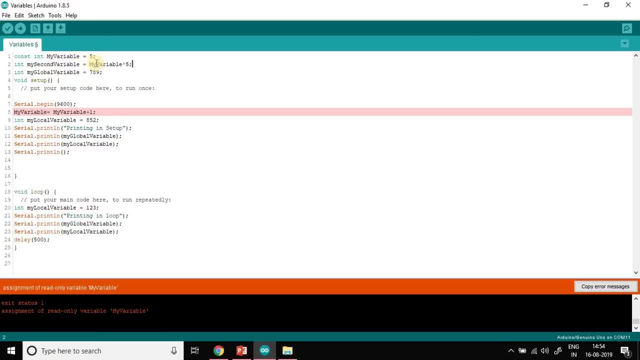 I've just printed out my variable into 5.. Right, since this is not possible, we will remove it. Right, let's try to dip arrogance So we can check that We can also. you can see here, since you don't have time to lubricate it to a full condition. 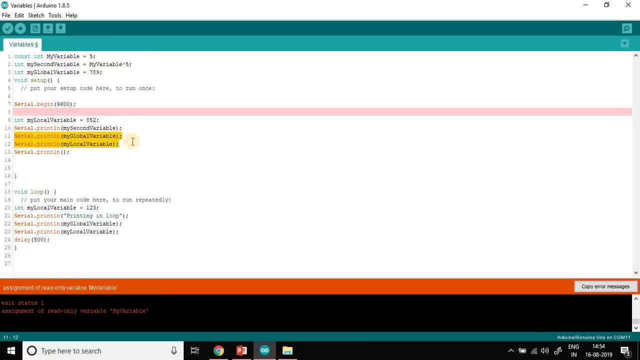 check below for the meaning of how long you are using it. plus it is set to 0 data. basically you get 0 data. so e2 is set as 2 event, second variable, right. so can you guess what will we get? we got 25 right because my variable was. 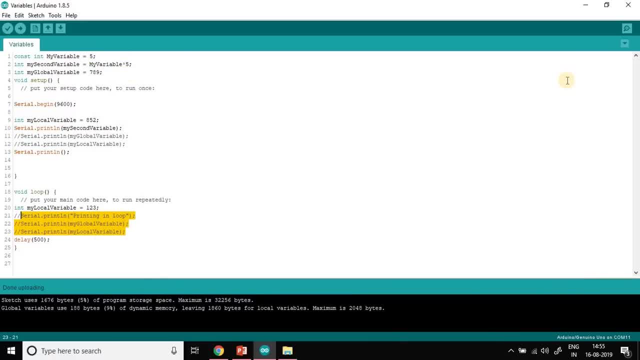 5 and we multiplied it by 5 so we got 25. so you may wonder: what purpose do constant variables serve in the code? well, we can use constant variables wherever we don't want our variables to change their value. for example, they are constants like pi, which is 3.1 for, and we can have order no pins as constants. 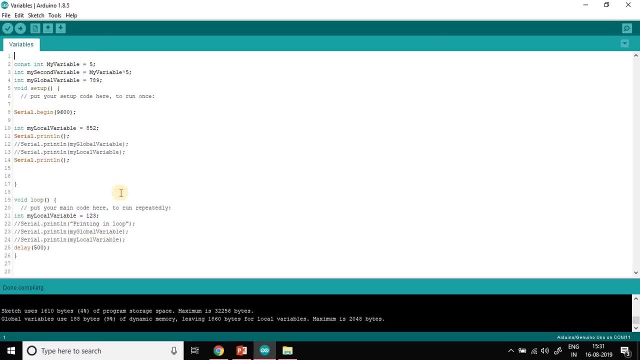 like if we don't want to change them in the code. I would also like to tell you that there is an alternative in C++ language to define our constant variables, which is hash define. hash define is a useful C++ component that allows the programmer to give a name to a constant. 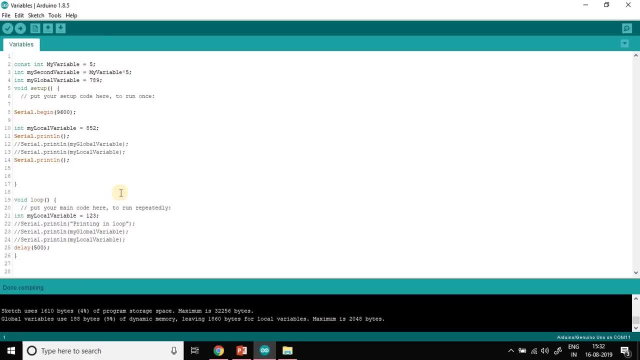 before the program is compiled. define constants in order. no, don't take up any program memory space on the chip. the compiler will replace the reference to these constants with the defined value at the compile time. So let's see this by an example. We start by writing hash. define then the name of the. 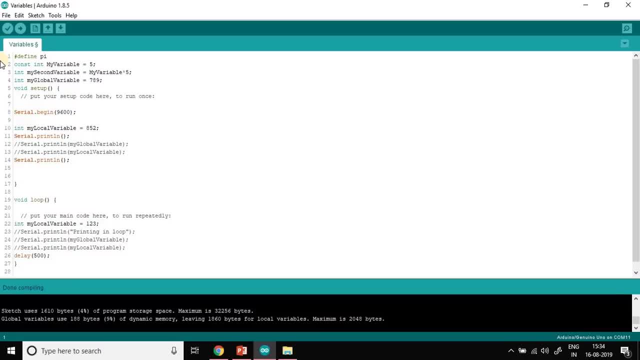 variable which you want, Let's say pi. okay, and the value of that variable which you want? It can be anything, for that matter. It can be an integer, it can be a float, it can be a character. So let's say the value of pi is 3.14. 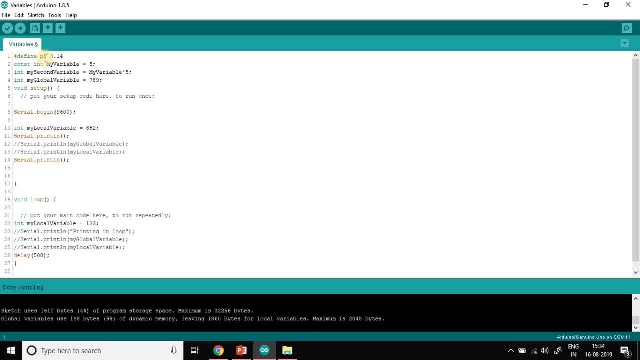 right. Also, note that we don't terminate the defined lines by a semicolon, We just write this. So whenever we use pi in our code, the compiler will replace the value which is written next to it. there, The compiler won't care if it makes any. 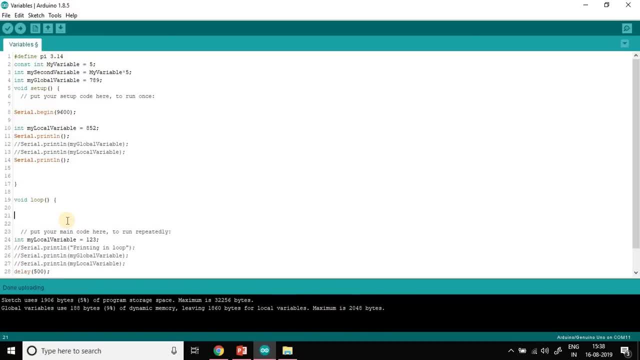 sense or not. You have to make sure that it makes sense. Okay, so now let's declare another variable of float type and let's name it area of circle. Okay, and let's do the math: pi into pi r square. Let's say r is 5.. So right, and now let's print the area of circle. 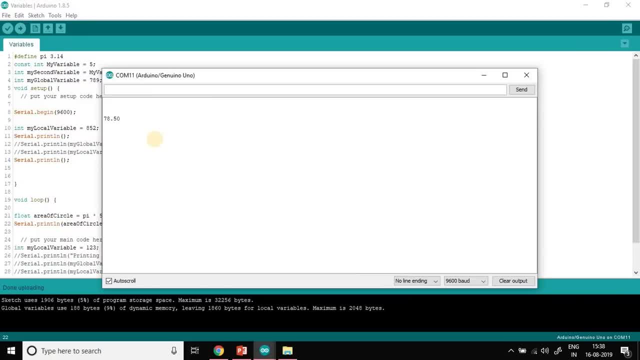 Right, let's upload it. We see it has automatically picked up the value of pi from here and it has done the math and it is giving the answer to us Right, as hash define doesn't use any memory in the Arduino. it is really tempting to use. 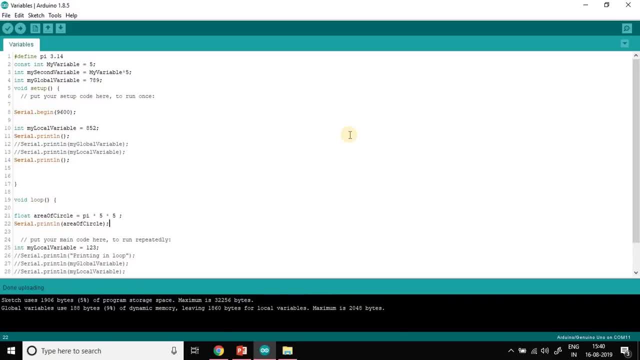 hash define, But it certainly has some downsides. The compiler will replace all the references to pi in the code and you will start facing problems. So it is recommended that you avoid using hash define. So use constant int in place of hash define, unless you are falling short. 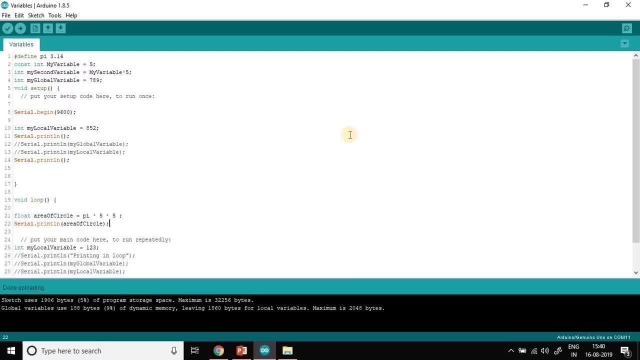 of memory. So in the next video we'll talk about the static qualifier. See you in the next video. So we will discuss about static qualifier in this video. Let me just quickly clean up this mess first, because it's looking so confusing. So 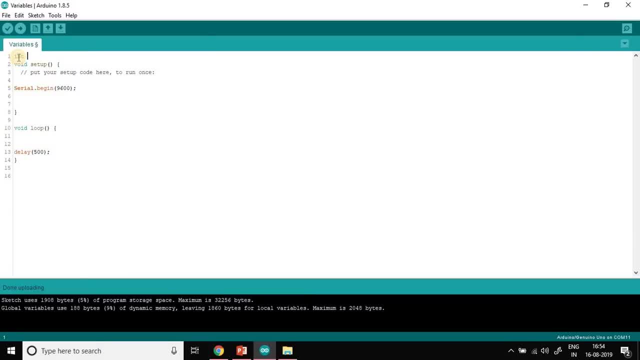 just observe what's happening. Let's declare a variable here. I'm going to call int. x by z is equals to 0, let's increment it here and let's print it. let's see what happens. can you see that we initialized it by 0, we increment it by 1 and then we printed. 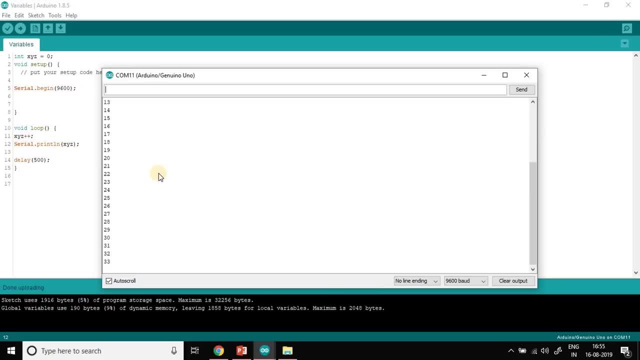 the value. so when the loop started again, the value would be incremented to 2. that can stop this auto scroll. the value will increment to 2, then 3, then 4 and 5 and 6 and then so on. okay, it will keep running until I stop it. so in this case, 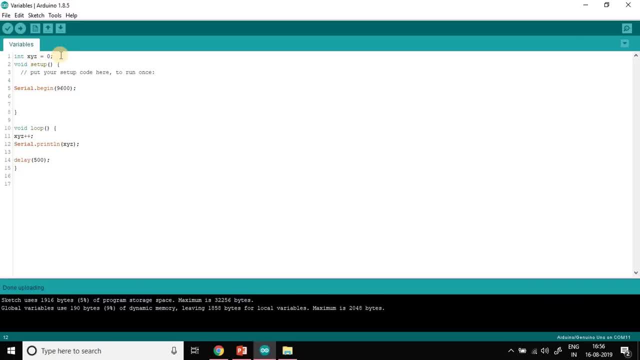 we have declared XYZ as a global variable, but I would like to tell you that it is not a good practice to declare many global variables, so we should try that we use local variables as much as possible. so let's try to use it as a local variable. we will remove it from here. 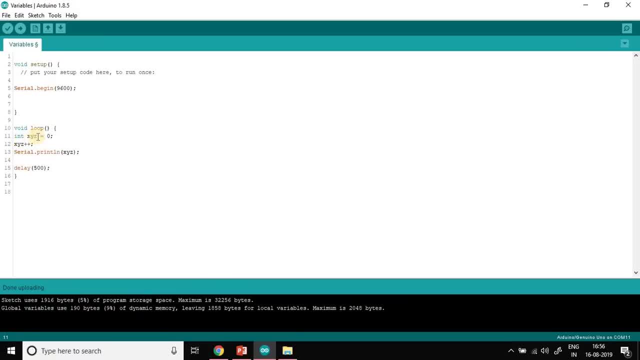 and we will declare it here. right, we declared int XYZ equal to 0, then X Y Z plus 1. then we will increment it by 1 and then we will print it. okay, let's see what difference will it create. can you explain why is this happening? okay, we initialize it by 0. we. 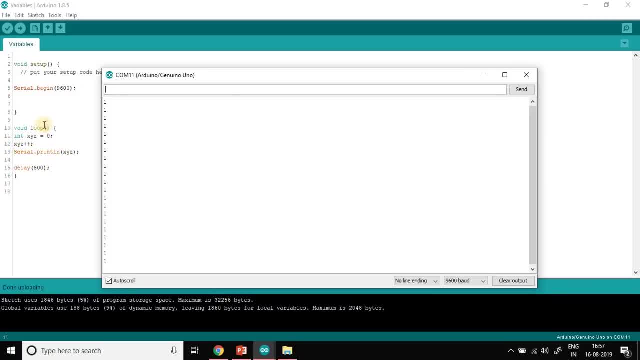 incremented it, we printed it okay, and then it was again initialized to 0. then again it was incremented by 1 and then printed. so it will keep on printing 1 unless I stop this loop. so now we are in a trouble. if we declare it in loop, then it would. 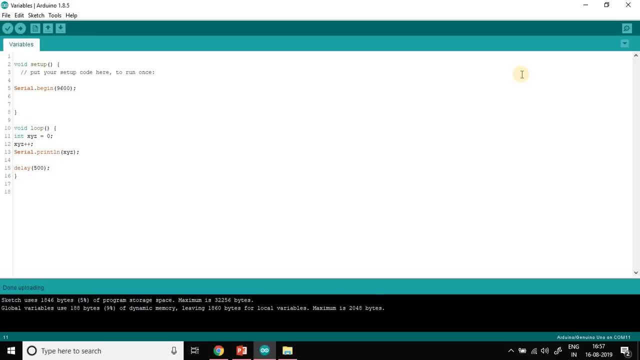 reset every time the loop is called, and it is recommended that we don't use global variables that much. so what is the solution? the solution is that we use a static qualifier to do that. we will just add static in front of our variable. what this will do is this: will just initialize it by 0, and. 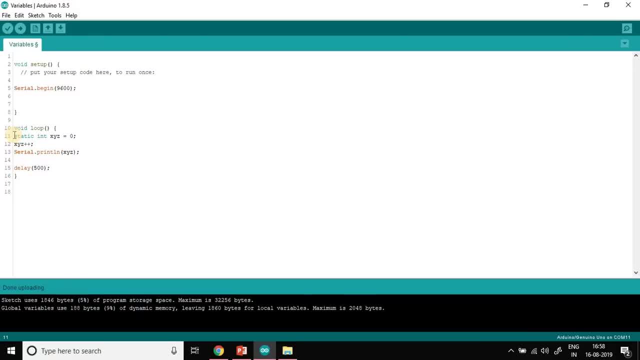 it will not reset it to 0 every time the loop is called. let's see if it solves our problem. yep, it did solve our problem, so using a static data qualifier is a good way to preserve the data of our variables between the function call. I hope it was. 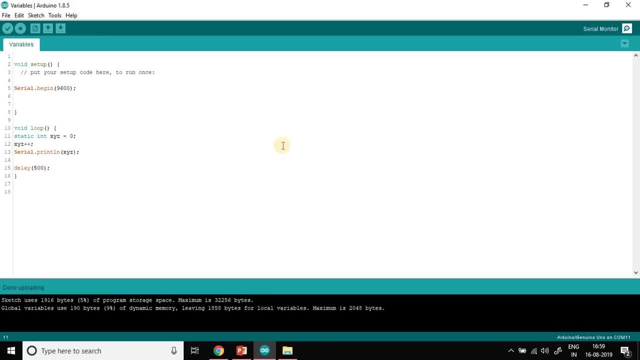 clear to you. please comment down if you have any questions. see you in the next video. in this video we will look at the comparison operators. comparison operators are basically some operators which would tell you if something which we're trying to compare is true or not. they would return a boolean value of either true or false. so we have about. 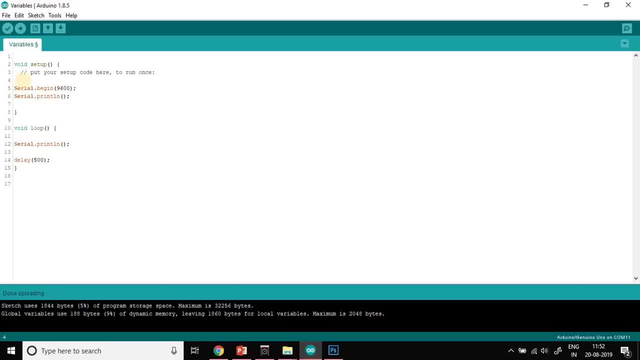 five or six comparison operators. we will just look at them in a moment. the first operator which you have is a less than operator and is represented by a less than symbol. then we have a greater than operator, then we have less than equal to, and we have greater than equal to, then we have equal to equal to, and then we 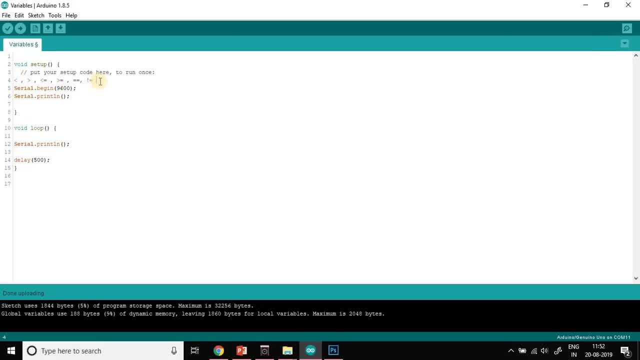 have not equal right. so we have a total of six comparison operators. we will just look at them, what they exactly mean. let me comment this out first. now let's have our variables. int variable one, right, let's say it is seven. then we have int variable two, and it is eight. let's try to. 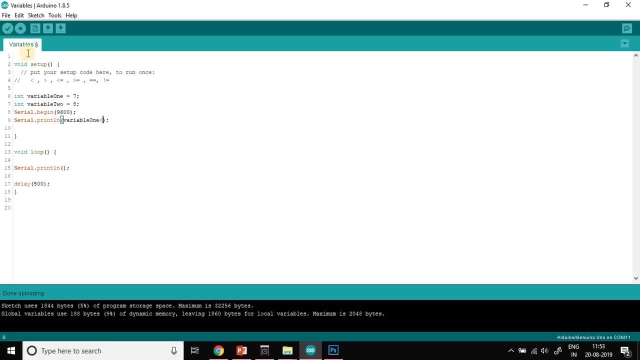 compare them: variable one less than variable two. as I told you, this operator returns something which is true or false. so what will happen here is: since variable one is less than variable two, right, so it will print one. let's see. so now let's do one thing: let us make this variable one as nine. now we should get zero. 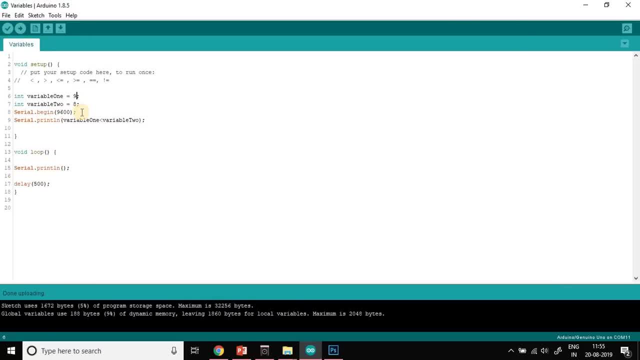 because this statement will become false, right, as we expected. so now can you guess, if I make variable one as eight, what will happen? let's see they should return zero. yes, why? because eight is not less than eight. okay, it is equal to eight, but it is not less than eight. 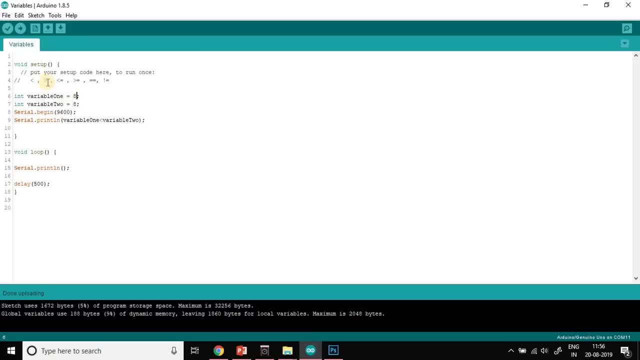 we will talk about this condition very soon. okay, now we will have the greater than operator. let's replace this right and change the variable to nine back, okay, so what do you think it should return? it should return, true, because variable one is greater than variable two, of course. I hope you understood. 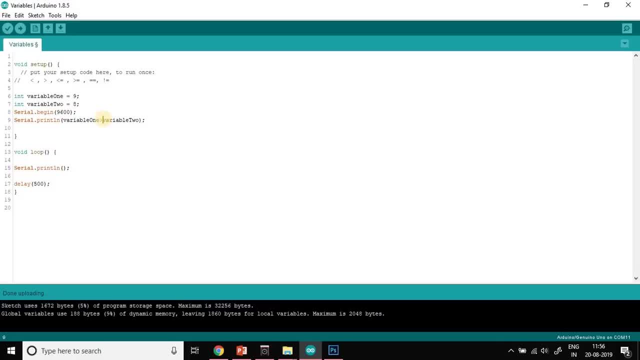 these two operators, then we have less than equal to. we use it like this: a less than symbol and equal to symbol. this is a less than equal to operator. what this does is it will return, true, lesser than the value on the right side, or it is equal to the value on right side. you got my point. 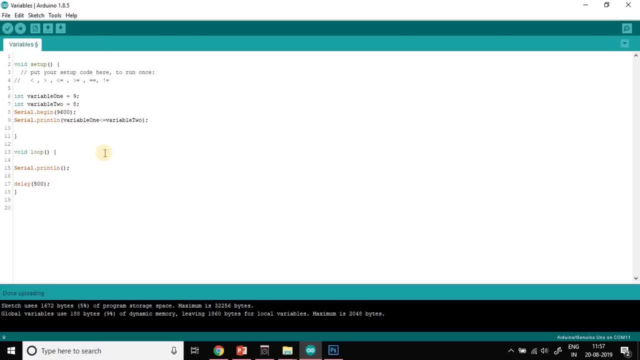 so previously, when I made variable one equal to eight and variable two also eight, it returned zero. but in this case it will return one because eight is equal to eight. so let's try that right. so similarly, a greater than equal to sign also works like this. you can experiment this on. 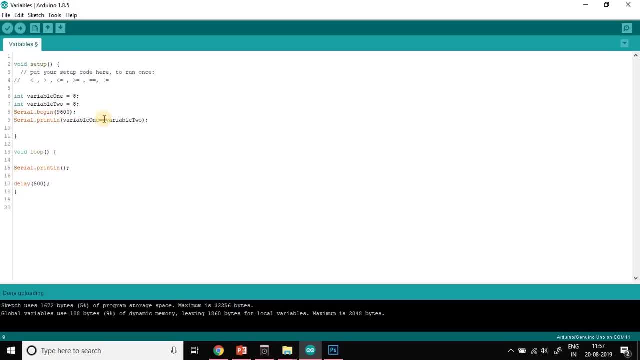 your own. then we'll look at the equal to equal to sign. equal to equal to sign means it will compare if some values are equal or not. it will return true only and only if a value is exactly equal. in our case, we will get one, because our value are eight and eight. 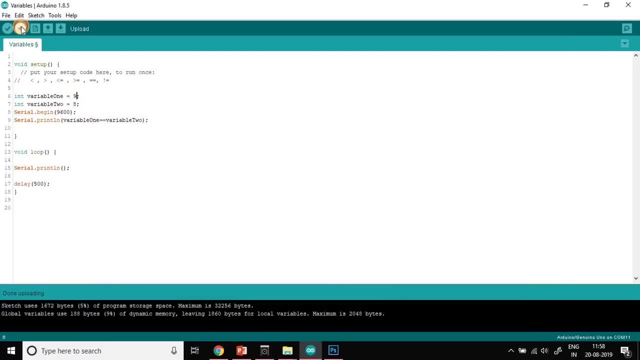 we got one. if I make it nine, for example, we should get zero. then we have a not equal to operator. we use it like we take an exclamation mark and then are equal to symbol. this operator will tell you false only if the values are equal. okay, in all the other cases you will get a one. not equals to right if some. 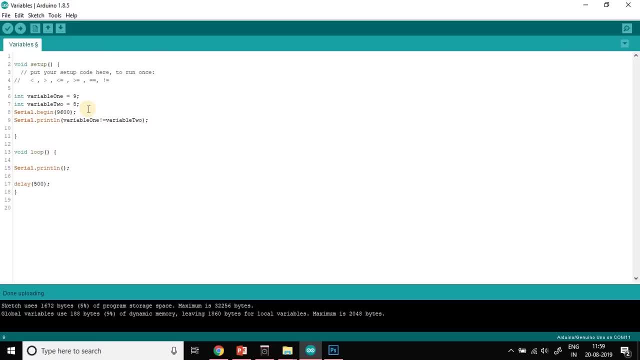 value is equal to some other value, it will say it is false because that is equal. but if you take any value- in our case, for example, variable one is nine and variable two is eight, we should get a one because that is true. right? so we have covered all the operators and how they work. 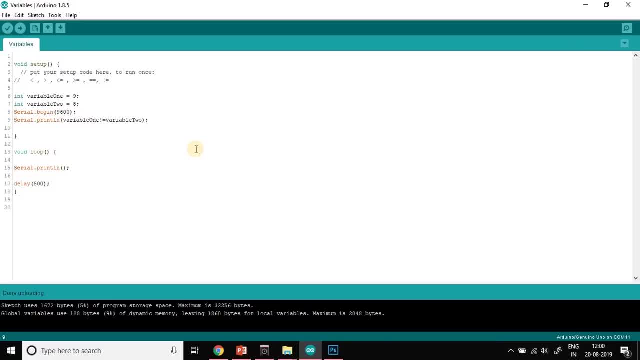 so you may be wondering now what is the use of these operators in programming? well, these operators will help you compare the values. for example, you make a project in which you have to compare the values of the sensors, so you may have to use these operators right. and when you use these operators, you will get some decision making capability in your code. 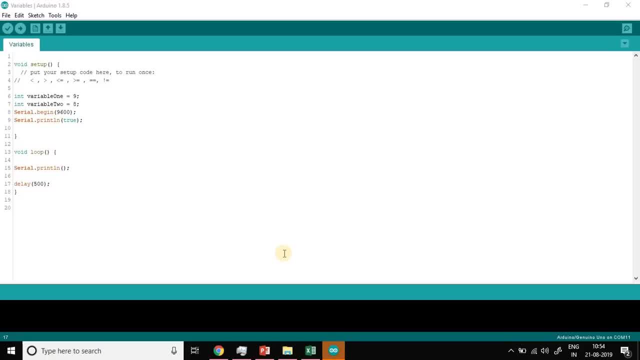 I would like you to note one important thing about the equal to operator. many people make a mistake while using the equal to operator. they use one equal to sign instead of two equal to signs, while one equal to sign is the assignment operator. that means you are assigning a value to a variable. 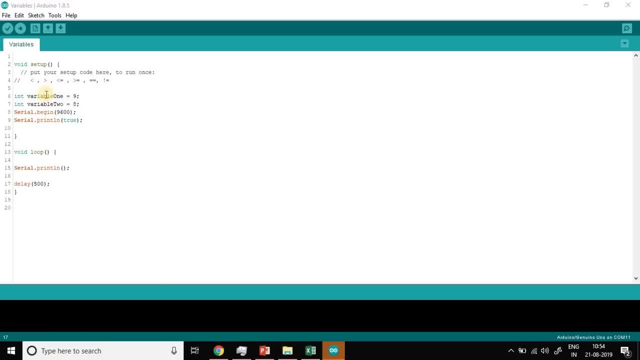 like in this case. we have assigned a value of nine to variable one, we have used one equal to sign okay, and when we use double equals two, that means we are trying to compare something. so to avoid making mistakes, I really recommend that you double check the operator which you have used. I will talk about this once. 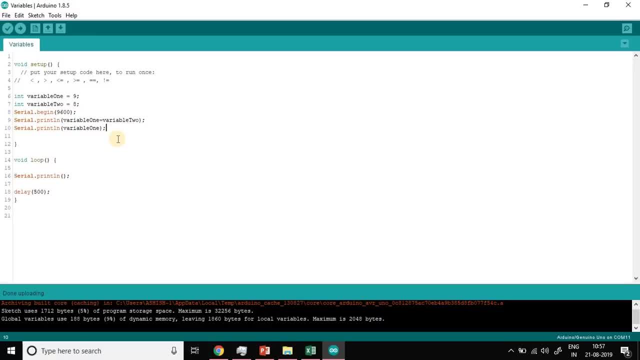 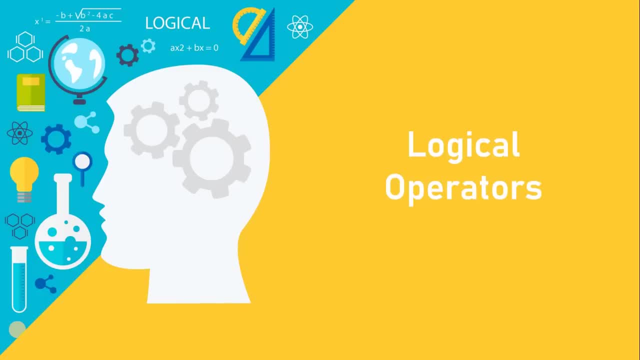 more in the control structures, when we study about the if conditional block, and in the next video we will learn about the logical operators. in this video we will look at logical operators. the concept of logical operators is very simple. we have logical operators whenever we want to take decisions in the code, each operand is applied to. 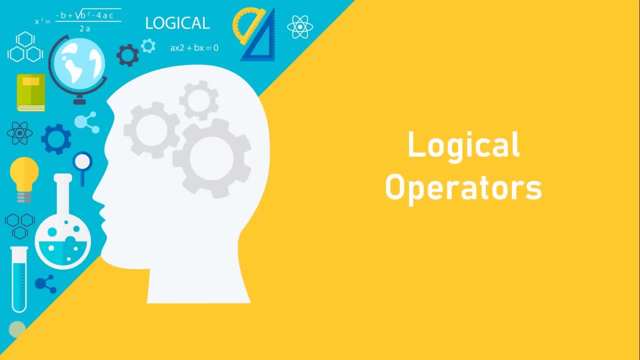 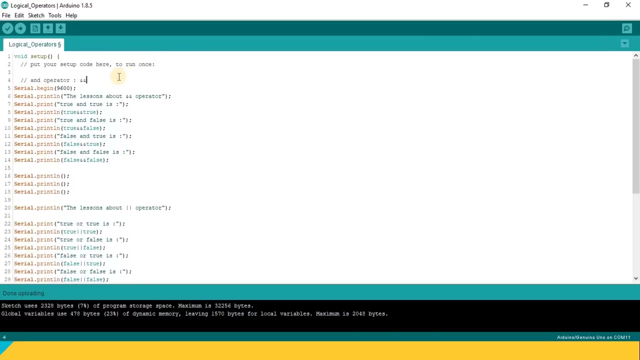 some condition, which may be either true or false. we will just see that in a moment. so basically, there are three logical operators: and operator, or operator and not operator. so let's see how it works in coding. so the and operator, the and operator is represented by two ampersand signs. these signs can: 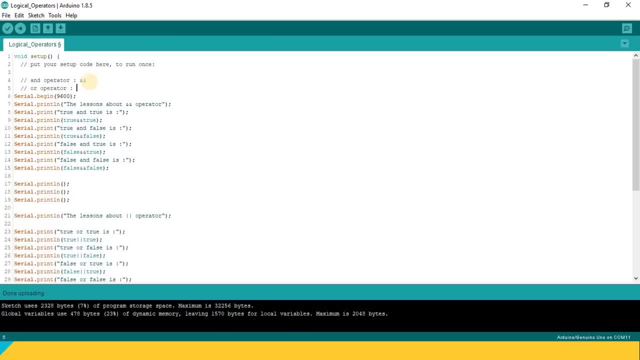 you see that then we have our operator and which is represented by two straight lines we will find just above your enter key, and then we have a not operator. it is an exclamation mark, that's all. so let's see the and operator. so the and operator expects that all the conditions which we are 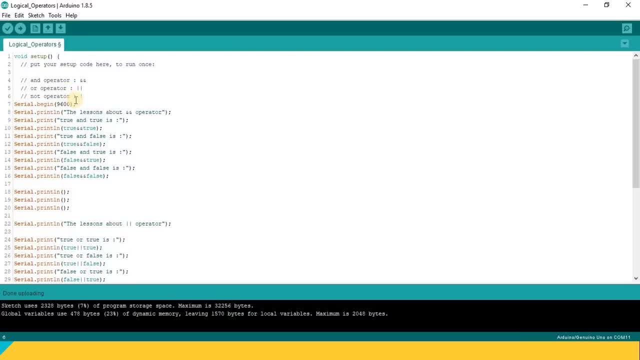 using in it are true in order to return a true. these operators also return a boolean value of either true or false. they also operate on boolean values, which is either true or false. like I told you, they work on some conditions. please hold on as I further clarify this. let's start with. 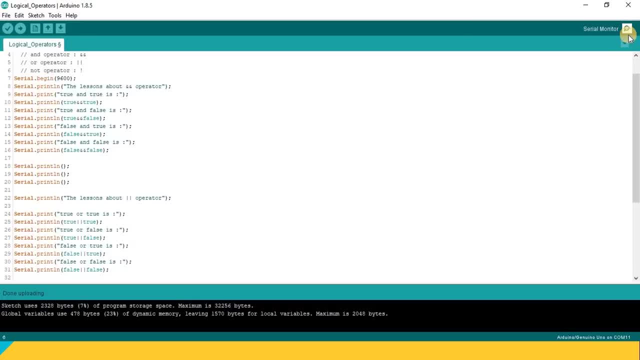 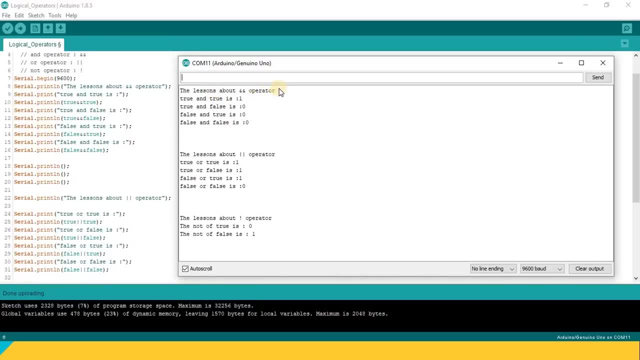 the and operator. so let me just open the serial monitor so that we can understand it side by side. the first thing which we have written is the lessons about and operator. it is printed exactly as we have written it. okay, then it is true and true is true and true is written like this: okay. 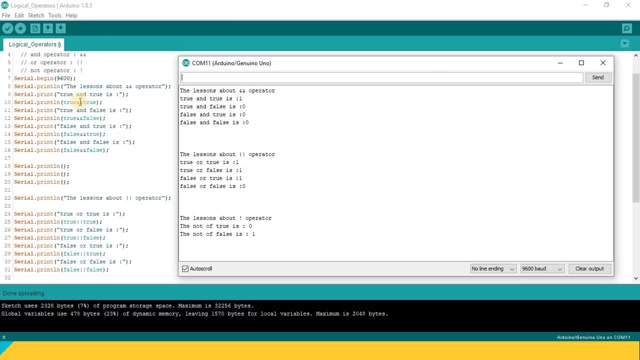 then we have written true, which is the boolean value, then the operator and operator, and then another boolean value, which is again true. the true and true returns a true in both of the two conditions are true, then the answer is true. for all the other conditions it is false. for example, 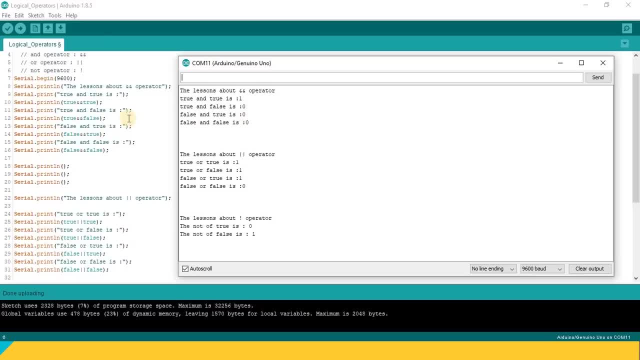 true and false is false. false and true is false, false and false is also false. so whenever we use it to take decisions, we tell the compiler: you have to proceed only if both the conditions are true. okay, if they are false, you don't have to proceed. okay. I hope it is clear. if it is not clear, don't. 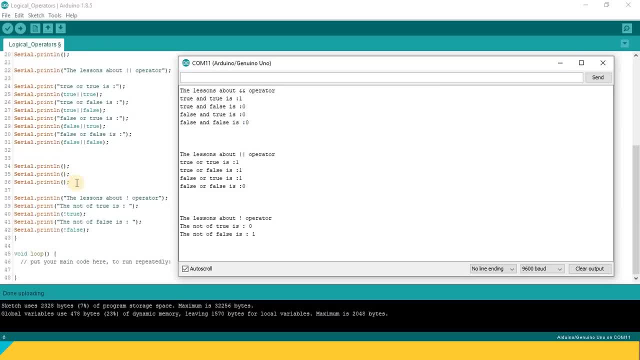 worry, we will just understand. while we write our main programs, then we have printed some empty lines and have a space over here. then we will see the or operator. this is the or operator. it is printing the lessons about or operator with the or operator. even if one condition is true, then the resultant 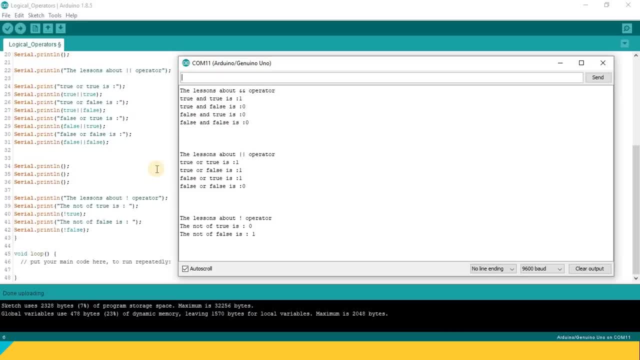 will be true. it will be false only if all the conditions are false. for example, we can see: true and true is true. true and false is also true. false and true is also true. false and false is false. right, then again, we have printed some lines so that we can see the gap here. then we will see the 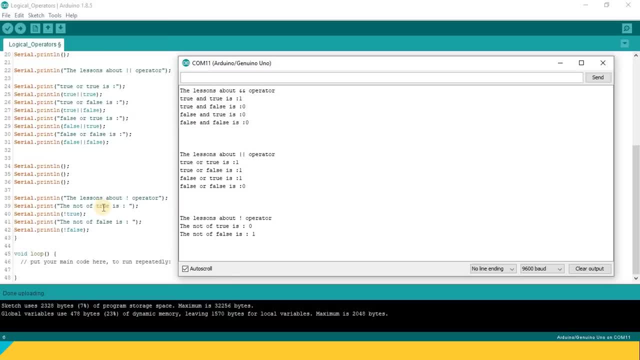 not operator. the not operator basically just reverses the value of the boolean. for example, the not of true is- we have used the operator here- and the not of true is false. as you can see zero, then the not of false is true. right, it has just reversed the values. it is very useful when we 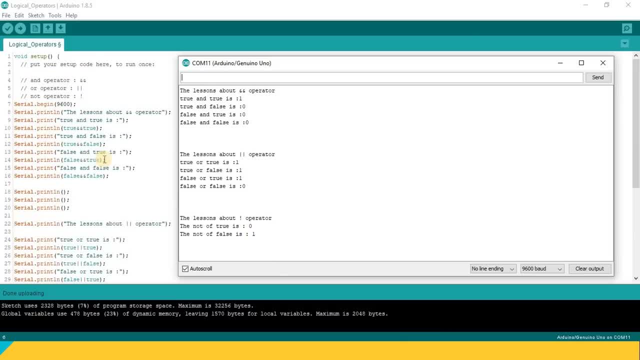 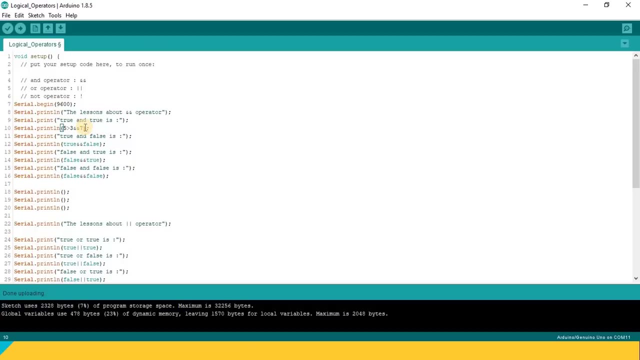 write our conditional blocks, which we will see shortly. all right, so let me just make some changes so that you can connect it with the comparison operators which we used earlier. okay, so instead of straight away writing true here, let's take five less than three, which is true, right. and instead of writing true here, we can say seven is less than. 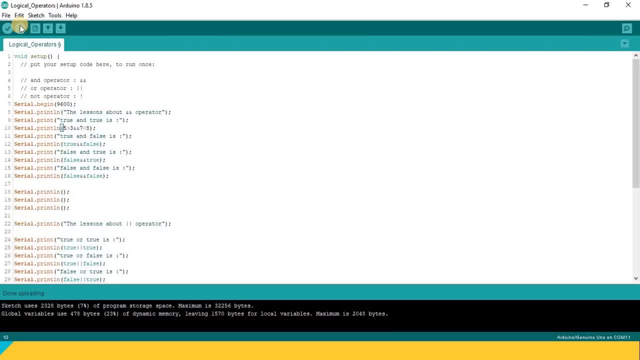 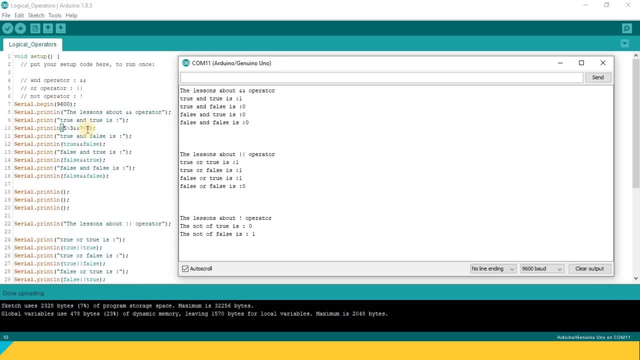 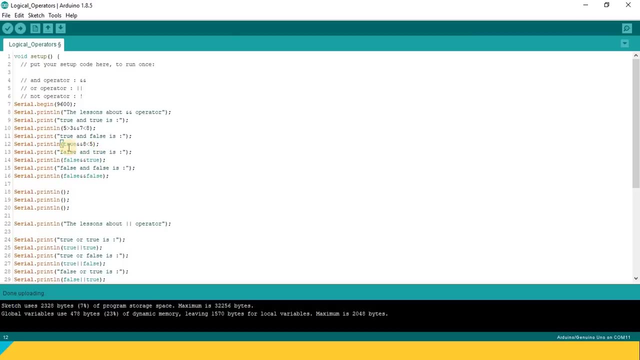 eight. okay, both the conditions are true. hence we will also get true. right then also, we got true because both the conditions were true. if we make one condition false, let's say here, eight is less than five, which is false. right, so true and false is false. let's see that. 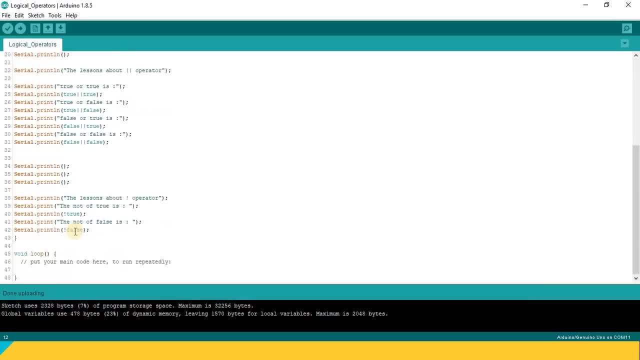 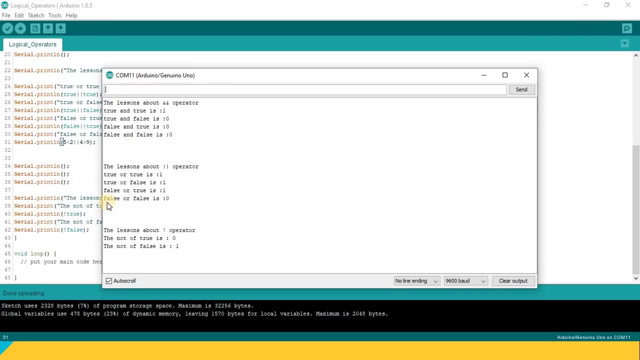 right. this is giving false. we'll just quickly look at our condition. let's say both the conditions are false. let's make false conditions: five is less than two, which is false. four is greater than nine, which is also false. so we should get zero right, which is this line false? and 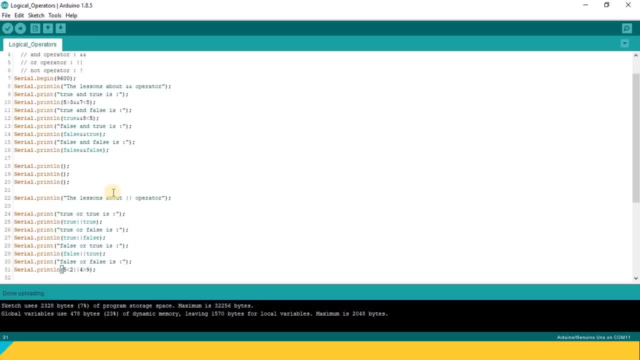 false is zero. I can understand it can be a bit confusing for some people, but I can assure you that once you start writing the codes on your own, you won't face any problem while using these operators. and even if you still have some problem, we are always there to help you. you can always. 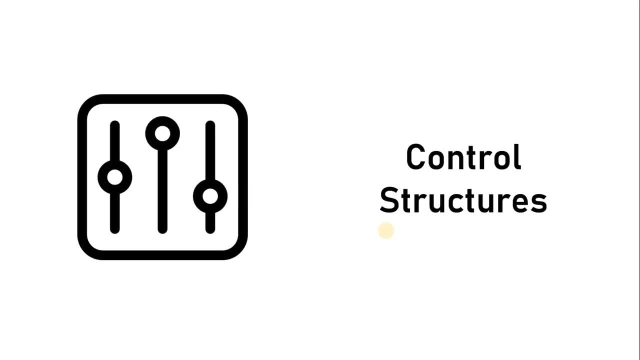 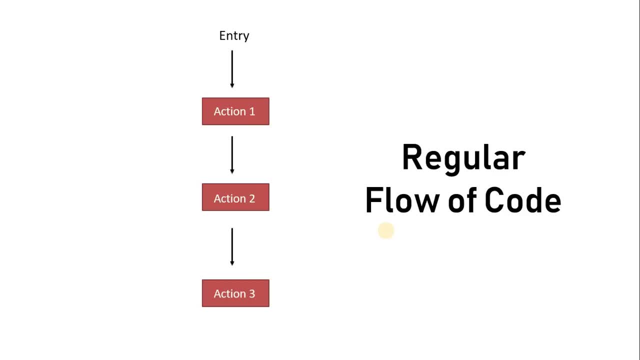 comment down in the comment sections. so see you in the next video. we will now look at control structures. so basically, till now we have seen that the code is executed line by line. that means the lines of codes are executed in the order in which we have written them. for example, we have written 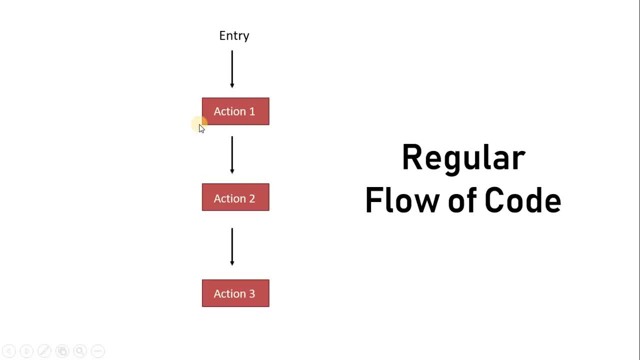 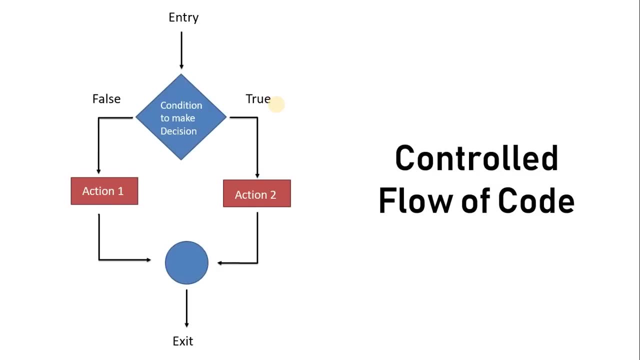 some code to perform action 1, then we have written some code to perform action 2, then in that case the will happen before action two. When the action two completes, then the action three will take place. So similarly, there is a controlled flow of code where we can decide which parts 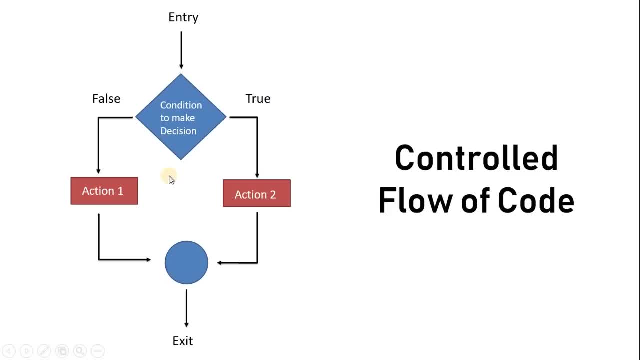 of the code we want to execute based on some conditions. We start our code and then there is a condition. That condition can be anything, for that matter, And based on that condition, if it is true or false, we can take some other actions. Let's say, we have a switch, We will. 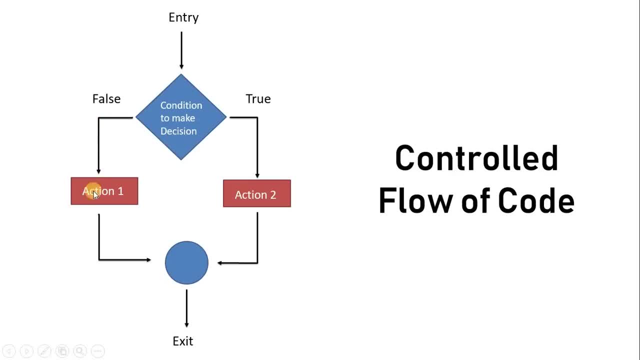 check. if switch is pressed, then we want to take some action. If it is not pressed, we want some other action to take place And the flow of code will depend on that condition. Either it will go this way, either it will go this way, And after completing a task. 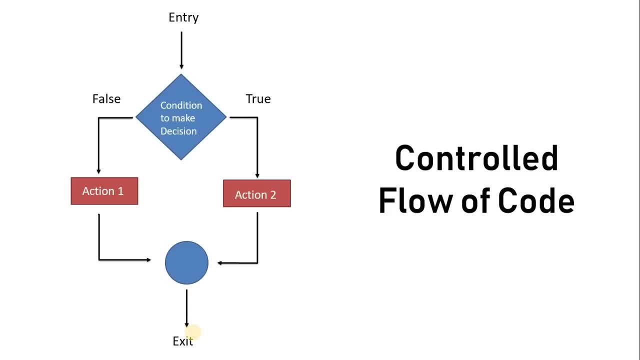 it will jump back to the main code, execute the lines which are present in the main code and then it will exit. So the first control structure which we will study is the if statement. We will understand about if statement and we will see how to use if conditions in our 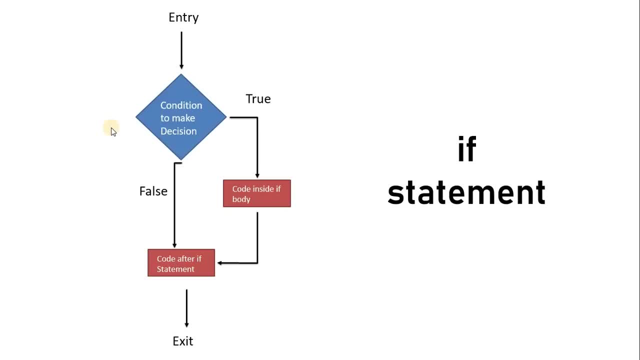 code in the next video. So let us see the if condition. Whenever we write an if statement, we write a condition along with that. Let's say, we are trying to use a if block. We will take a condition which we want should be true. If it is true, then whatever we write, 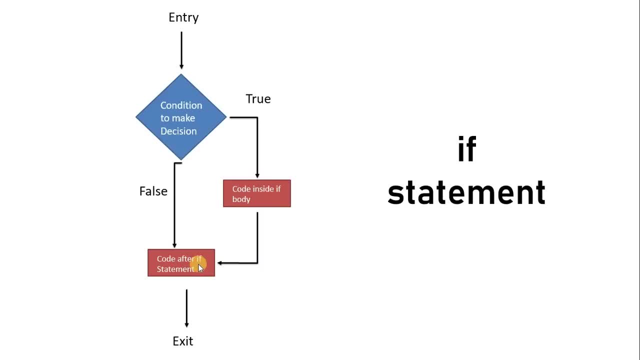 in the if block will execute, And then it will move on to the statement which is written just after if statement. Okay, and it will execute that as well, And then it will exit. But if in case it is false, then it will entirely ignore whatever is written inside the if block. 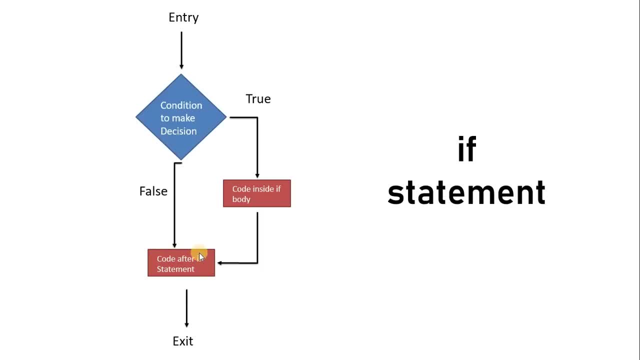 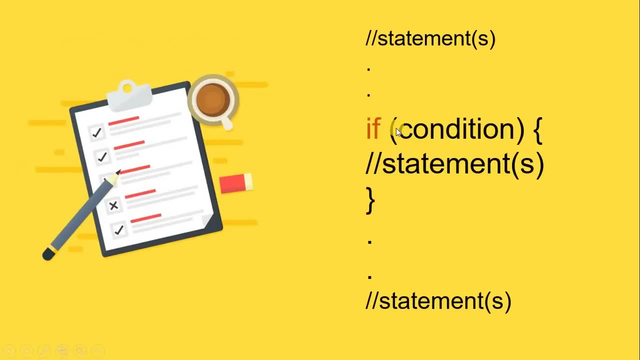 And it will straightaway jump to the code which is written after if statement. It will execute that and then it will exit. Let us quickly look at the syntax of if statement. So let's see this is our code. We have written some statements. We write if statement And. 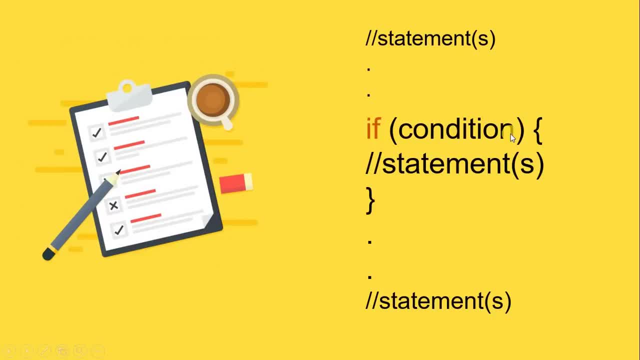 then we start a bracket, We write our condition. Let's say something greater than something, or if something is true, if something is false, if something is not true, anything for that matter, We will put a condition in this bracket. Then we close the bracket and then we open. 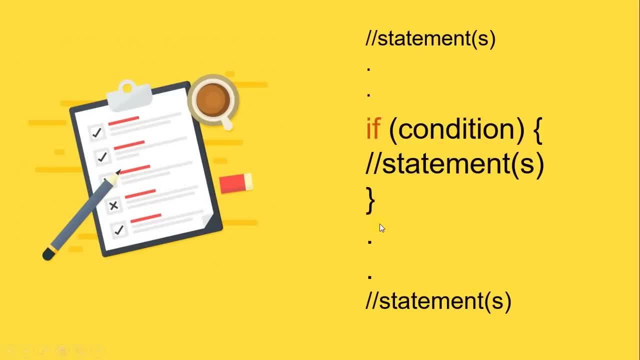 up the curly bracket, Then we write all the statements which we want to execute, Then we close the bracket and then we move on to write more statements in our code. So this is the syntax of if statement. So let us try this in our coding. So we have an example. 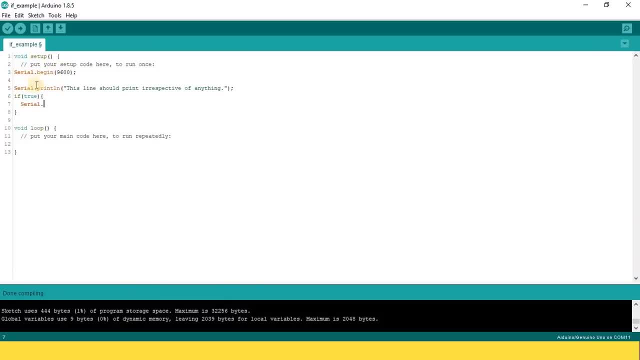 here. We have a standard here so that we can communicate with the computer. So we will write the first statement: Serial dot println. This line should print irrespective of anything. And yes, this line will print irrespective of anything. Then we will write: if true. serial dot println. 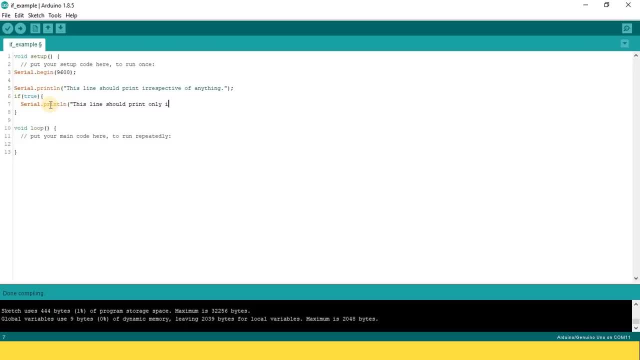 This line should print only if the condition is true. Please note that we don't use a semicolon here. Let's write another statement. If false, Serial dot println. This statement will not print as the condition is false. It is over. 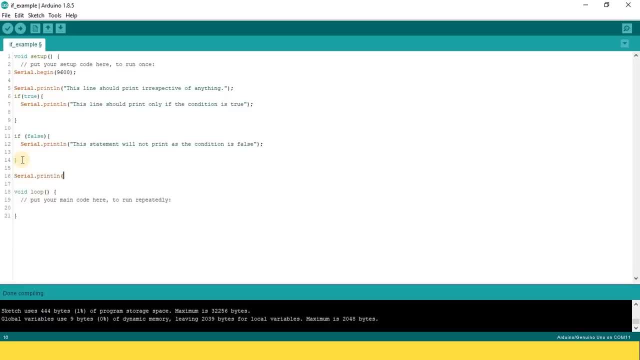 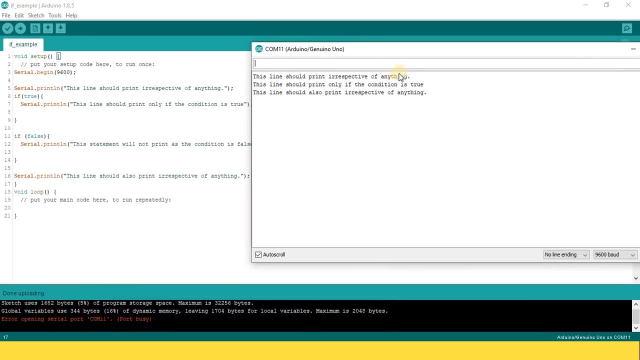 And then again we will write one line which should execute irrespective of anything. Let's say this: only. This line should also print irrespective of anything. So let's upload this code and see what happens. So we see, this line should print irrespective of anything. this line should print only if 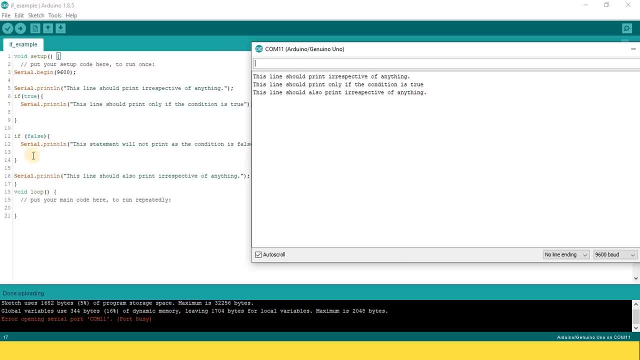 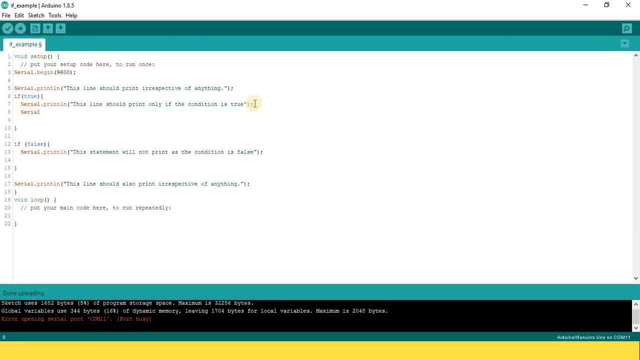 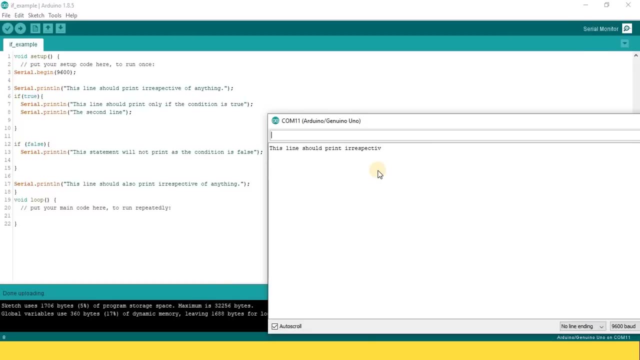 the condition is true, print irrespective of anything. so did you know that when the condition was false, the block did not execute? let me do one more thing. let's see a block of code executing. let's print one more line here, the second line, right, so now this line should also print there, the second line, because it was 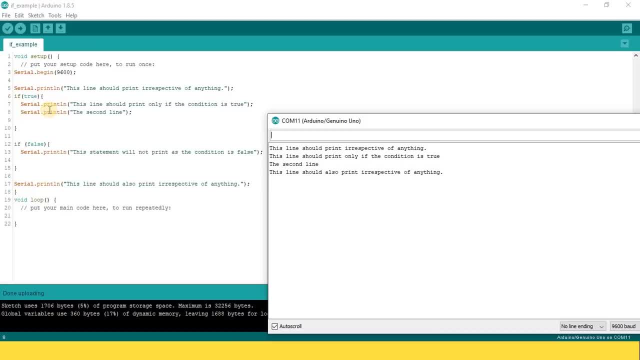 the part of this: if block, so whatever is written inside this block, it will execute no matter what once the condition is true. but of course writing true and false exactly like this does not make any sense right. so we have to build our conditions. let's say, if five is greater than three, then this: 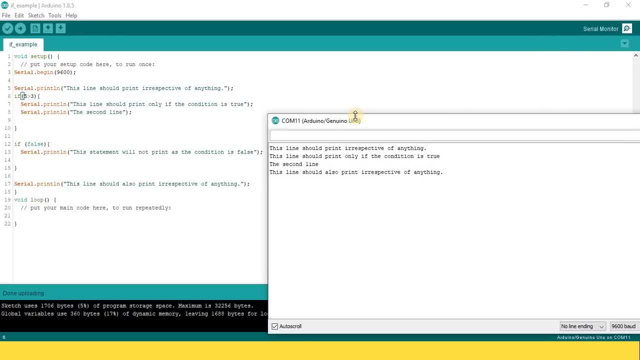 should execute, we'll see the same result, because this evaluates to true right. so basically, we should keep in mind that a boolean value should come inside this. okay, in this bracket there should be a boolean value. then only it would be able to take some decision based on that boolean value. so 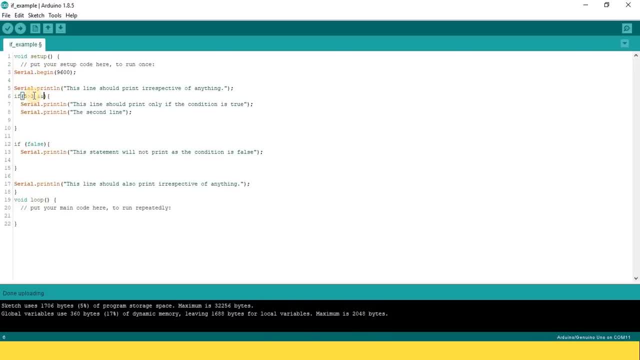 now we can complicate the condition as well, like, for example, and two greater than five, but this is false right, like if we take a boolean value and we take a boolean value and we take a boolean value, like we saw in the and operator. both the conditions should be true in order to return. 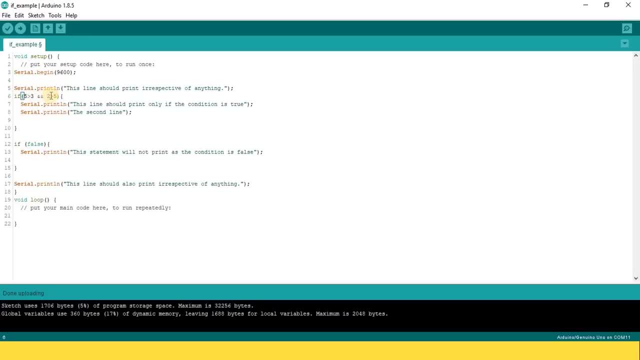 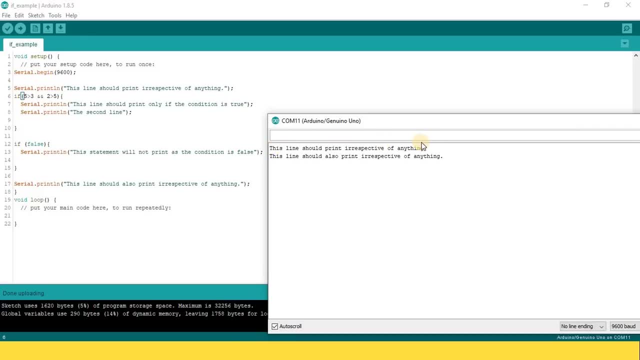 true, right, but this is true and this is false. so we'll now see that this block of code will also not execute. let's see: right as expected, this line should print, irrespective of anything, this line will print anyway. this line will also print anyway. so now let's try to print this line. we'll 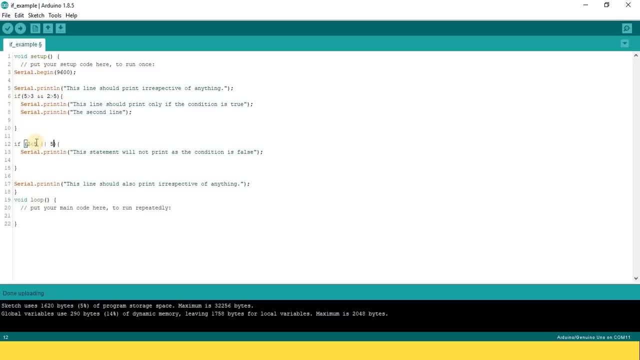 make this condition true: two is less than five or five is less than two. this condition is true because one of the conditions is true and the other condition is false. so we'll try to print: one of the condition is true, right, two is less than five, that is true, but five is not less than. 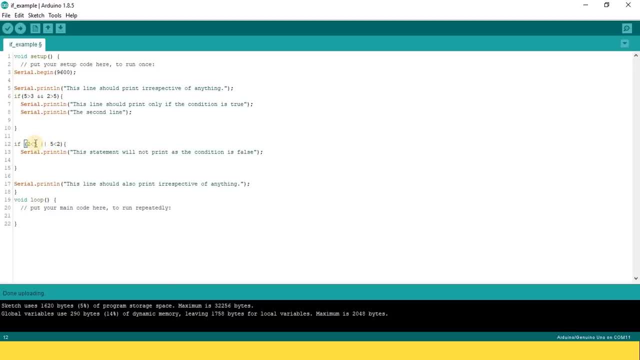 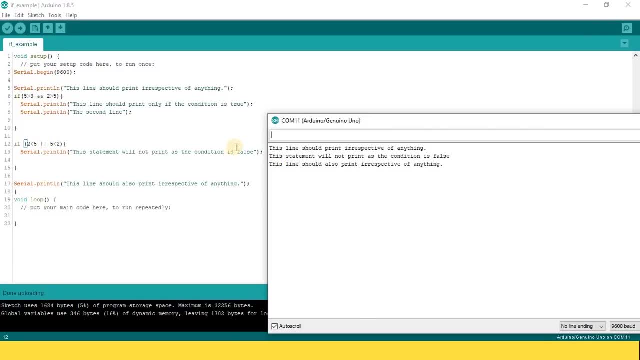 two, this is false. but in the or condition, one statement has to be true to get the resultant as true. so this line should print. now let's see: yep, so we were able to print this line because we made the condition true. okay, so when we will be making our projects? what kind of conditions? 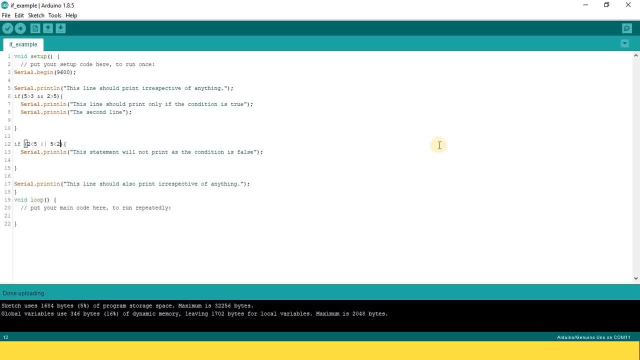 will we use? we will be using conditions like: the sensor value on the left hand side should be greater than the sensor value on the right hand side, then these things should happen. so i think we should be able to relate with this thing. okay, now i will tell you another thing. for example, i 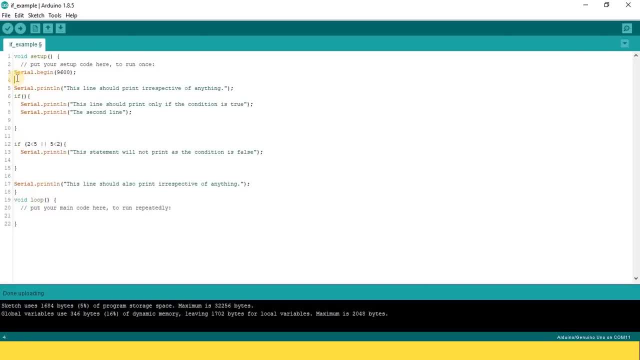 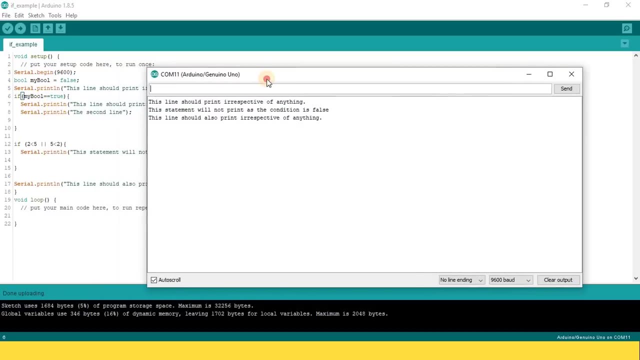 took a bool. many people do mistake in this, so let's start by taking a bool. my bool is equal to false. so now what i want to do is i want to print these lines only if my bool is true. so i'm comparing it. if it is true, then only it should print. but this is not true, right? because the value 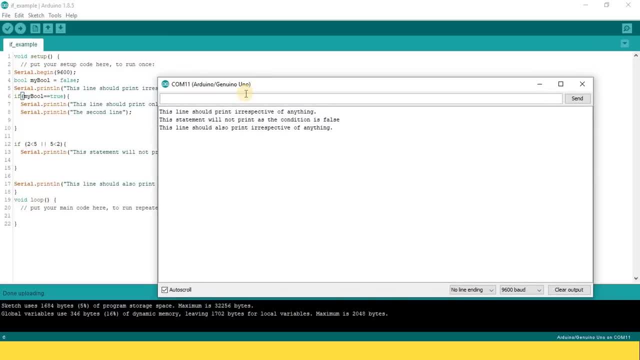 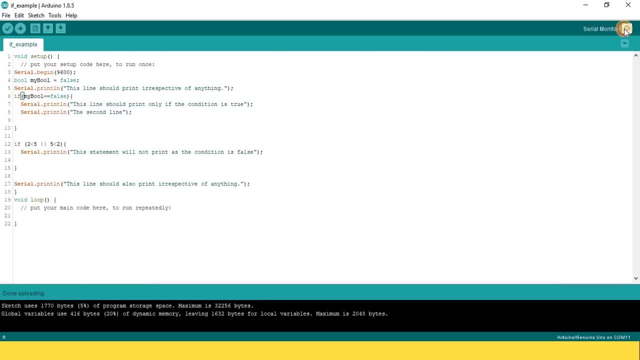 of my bool was false, so that's why the resultant was false. so hence the lines present in this: if block will not execute. so now let's see what happens if i print this line. if i print this line now, if you write false, then it will execute because it is actually false. 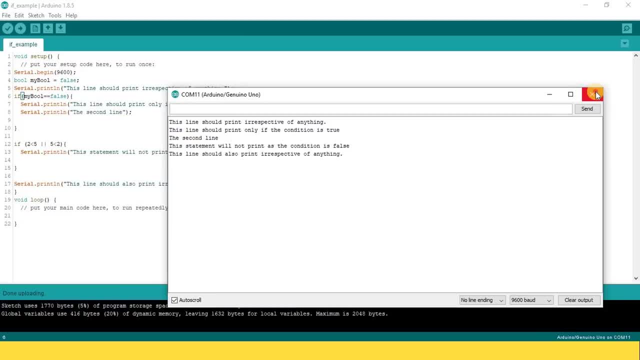 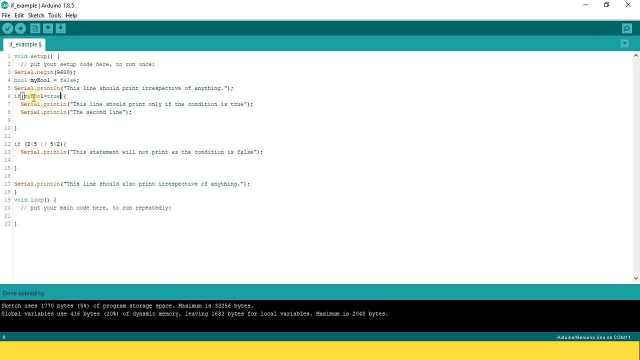 so we can see these lines got printed. so now i'll talk about the mistake which people do. what they will do is they will use one equal to sign instead of two signs. so what will happen is the compiler will assign a value of true to my bool and the resultant value of my bool will 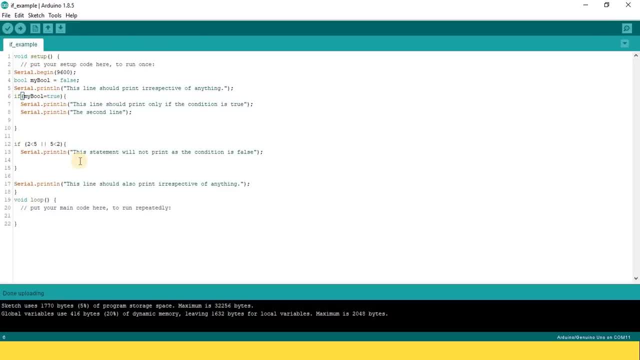 become one, okay, and this block of code will execute right. so the expression which we write in the if condition is executed first, and then the value of that thing is taken into consideration, if it is true or false. okay, in our case, my bool was assigned a value of true, and then the value of my bool was used. 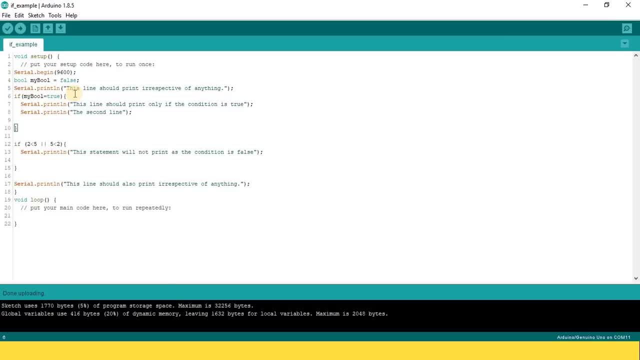 so please take care you use double equals to if you want to compare the values. now we can do nesting of ifs as well. what nesting means like this is our if block. we can write more if blocks inside our the parent if block. let's say we write another if if true serial dot println. this is nested, if right we. 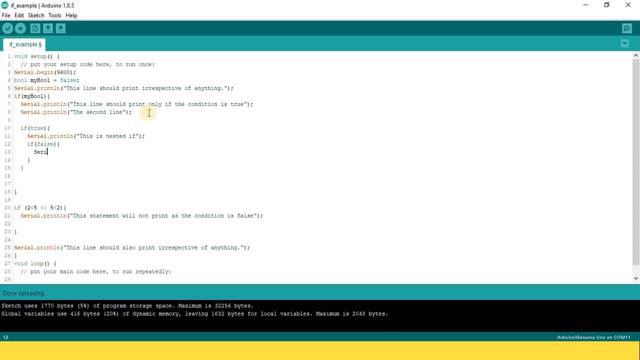 can write another if inside that, if false serialprintln, this is another line which will not execute. so this was nesting of: if this is the parent, if this is the child, if- and this is a further child of this, if right, we can see like this: this is the flow, This bracket다가 is실 when we書ire, let's say, we write another if. 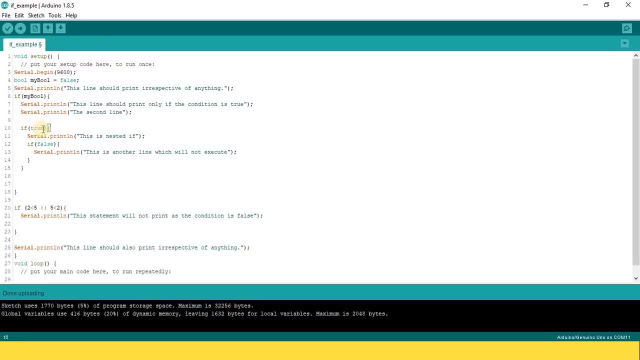 closes here and this bracket closes here, For example. in any case, the parent if is false, then all the child ifs will never execute. Please keep that in mind. I hope you understood this point. I'm pretty sure that you will be able to understand it in a better way when. 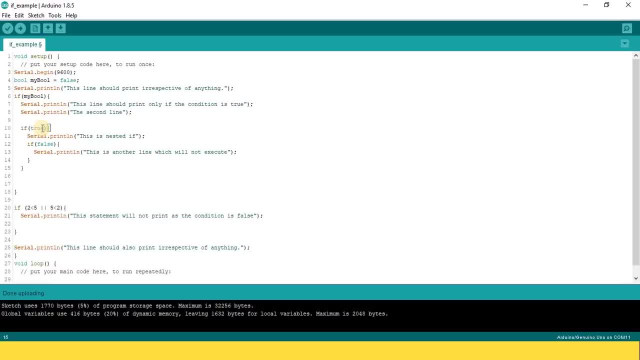 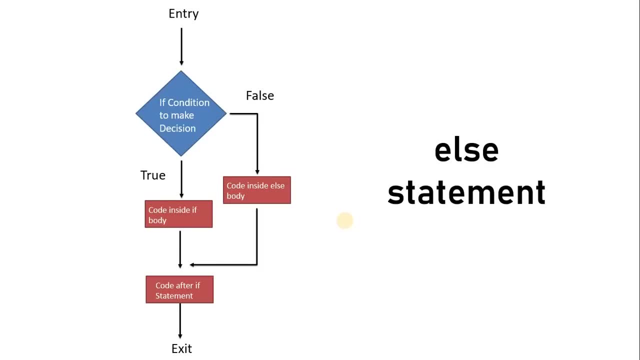 you perform your experiments. So in the next video we will look at the else statement. See you in the next video. Now we will try to understand the else statement. First of all, let us look at the flow of the code. We always write an else statement preceded. 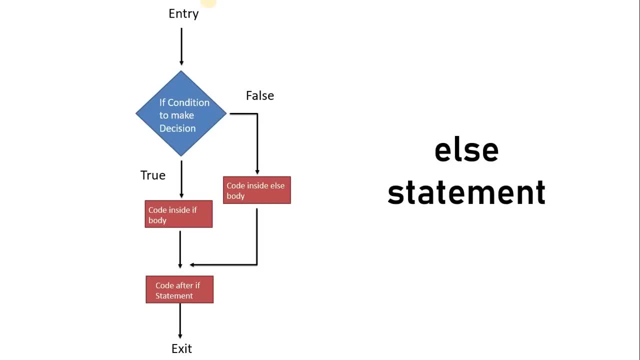 by an if statement. Let's have a look at the flow of code when we use an else block. There's an entry of code. There is an if condition. If that is true, the body inside the if block is executed. the body inside the else block is entirely ignored. Then it moves onto code after if. 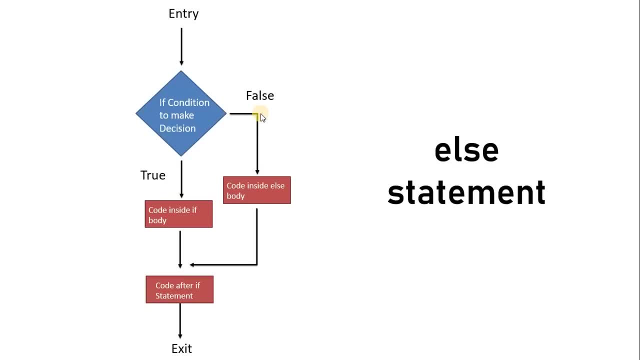 statement after executing that code. In case, if it is false, it will straight away go to else block and it will execute the code which is present inside the else block and it will ignore the code which is present inside the也f block. After executing the else block, it will go to the main code. 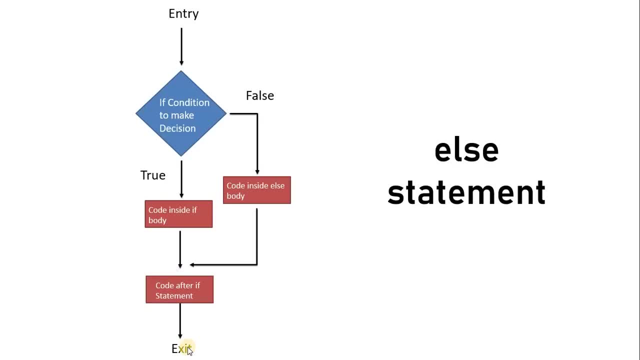 The code which is written after the if statement. it will execute that and it will exit. before looking at the syntax of else block, let us compare it with just the if block. so this was the if statement in if statement. if the condition was true, it would execute the body inside the if block. then it will go. 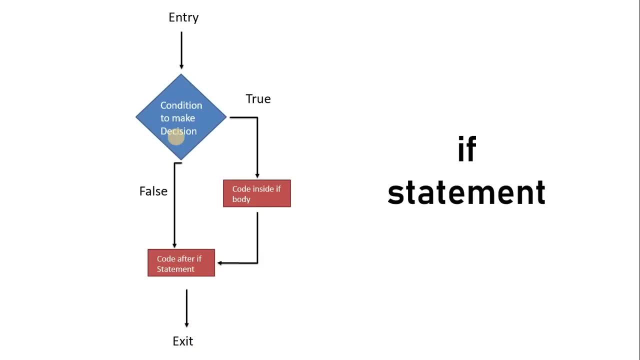 to the main code, execute that and then it will exit. so when we use just the if condition without else, that means we don't define what we want to happen if the condition which we have specified is false. if it is false, it will entirely ignore the if body and it will jump to the main code. but in else we define what. 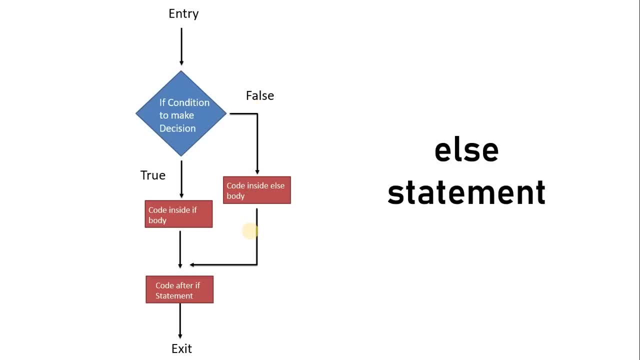 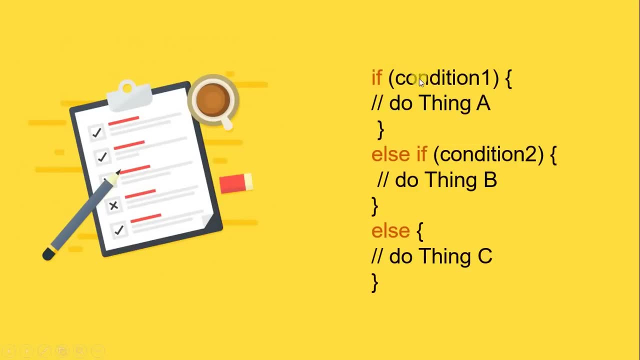 we want to happen if something is false, so that we write in the else block. so now let us look at the syntax of else block. we start by writing: if we specify the condition, we open the bracket. we write our actions here. if the condition one is true, then we close the bracket and then we write else. if if we have. 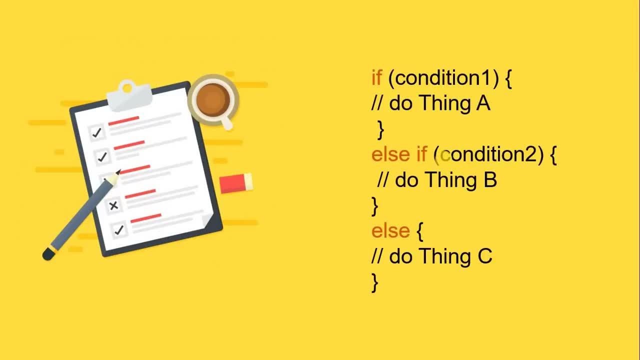 more than one conditions. for example, if you want different sound levels of an alarm based on the temperature ranges. for example, at a lower temperature an alarm would ring slowly, and at another condition, let's say another range, it will ring a bit louder. and if it exceeds something, then we want it to ring at the maximum intensity. okay. 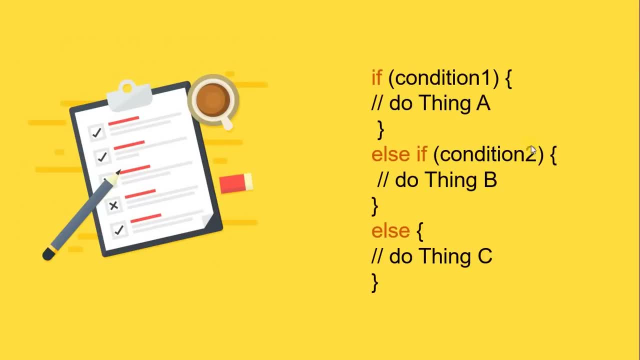 so these things can be controlled by if and else blocks okay after writing else. if we write condition two, if that condition is true, thing B will happen okay, and then finally we write an else. if none of the conditions is true, then the else block will execute. the thing which you need to notice here is if the 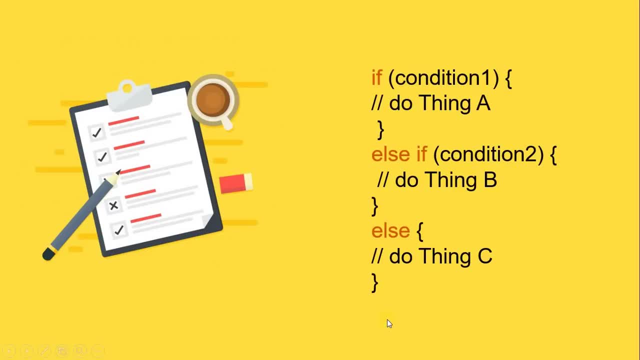 condition one is true, it will execute the thing a and it will straight away jump to the main code. after this, the control won't go in else. if it will go in else, if only if the condition one was, for example, the code was running. here it found that condition one was false. so it will jump and check if condition two is. 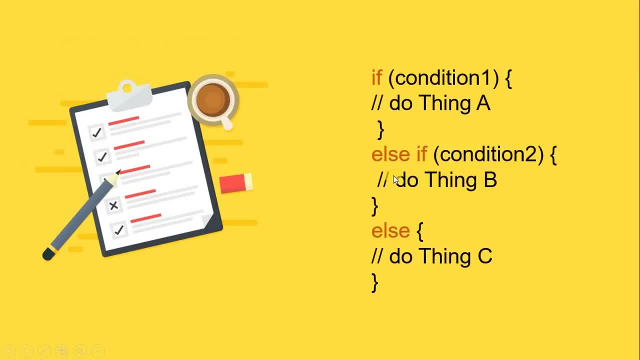 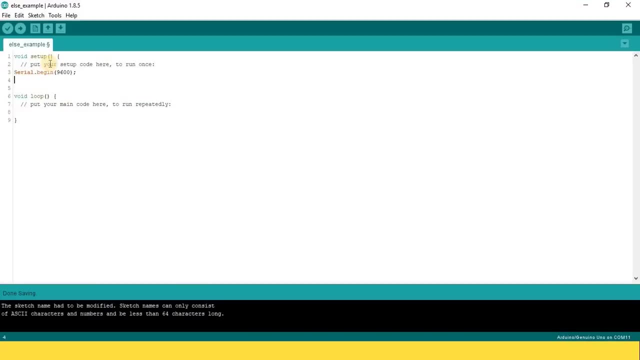 true or false. if it is true, then it will do the thing B. if it is also false, then it will go to else block and do the thing C. we will just understand this with the coding example. so here we have example for understanding the else statement. let's do this. we'll write, if true. serial dot print. 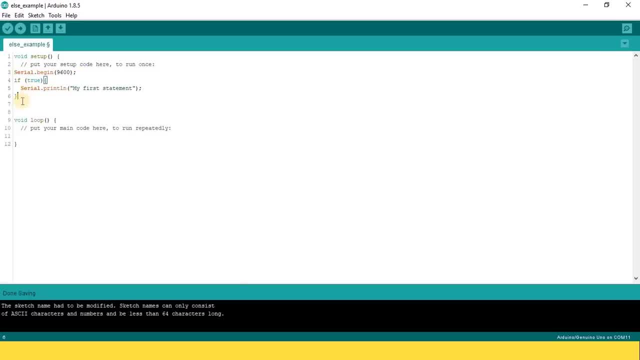 ln- my first statement. so you can see the compiler has automatically considered this bracket which was originally for void setup for the if block. okay, we have to make sure we are using our brackets correctly. now, after closing, the if block will write else: serial dot print ln- my else statement. all right, so now we will. 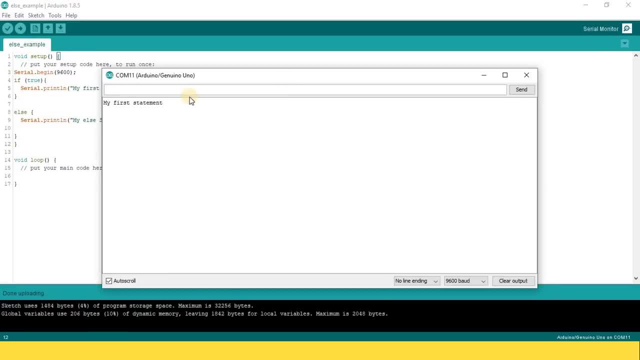 close the void setup bracket. now let us upload this code. okay, so my first statement got printed because my initial if condition was true and it will ignore the else block. Now let's make it false. Now we will see the statement written in. the else block will print. 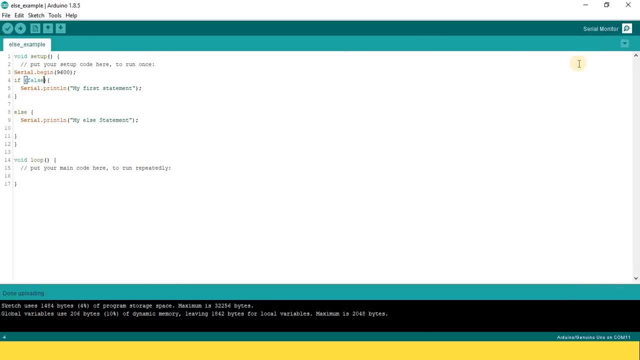 Let's have a look My else statement. Okay, We can do the nesting in if else statements as well, Like we saw in the if video. Like I can start another if here If some other condition will write another task here. So we can use endless if and else and the nesting of them as well. 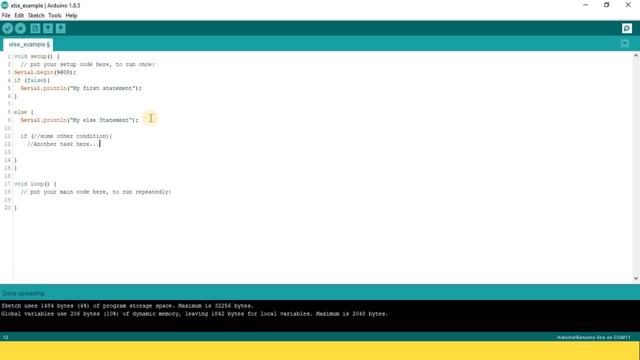 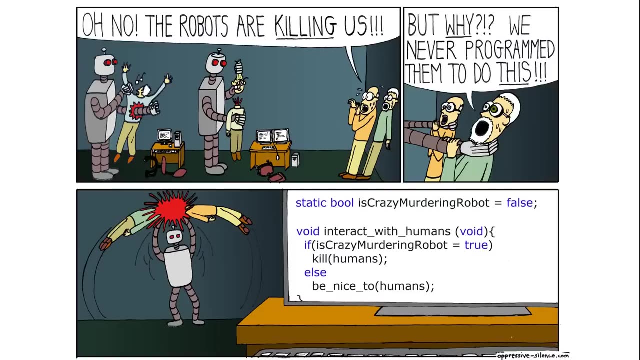 By now you must be feeling a little bored by just printing the statements here and there and not doing any real things. So in the next video I will show you a small simulation by using if and else blocks. See you in the next video. So before I show you that if else simulation, I would like to show you this comic. 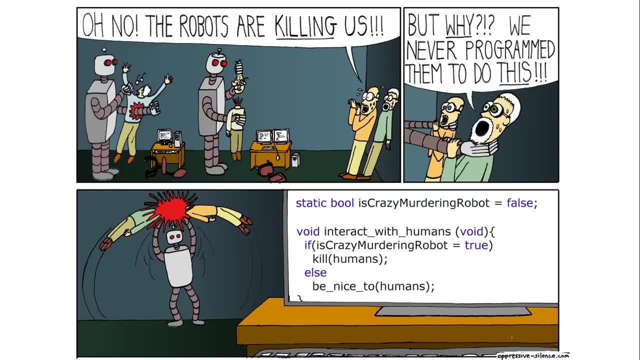 Just have a look at this comic for like 5-10 seconds And if you get the joke in this comic, I can say that you have pretty much understood the concepts which we have discussed so far. Okay, Don't worry if you could not understand this. 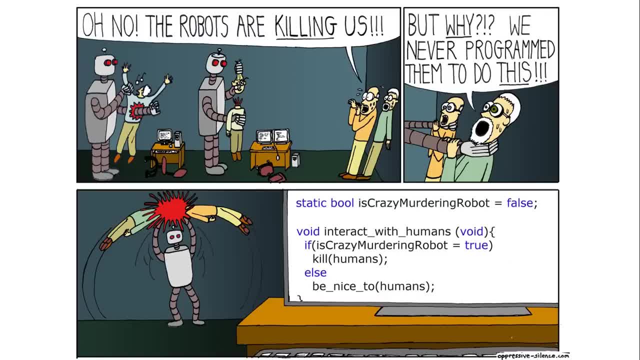 Once you finish the part Where I am teaching about functions, I am sure you will be able to understand it really well. So, just in case, if you could not understand this, I would say that please complete that section and then come back to this comic again, and I am pretty sure that you will have a. 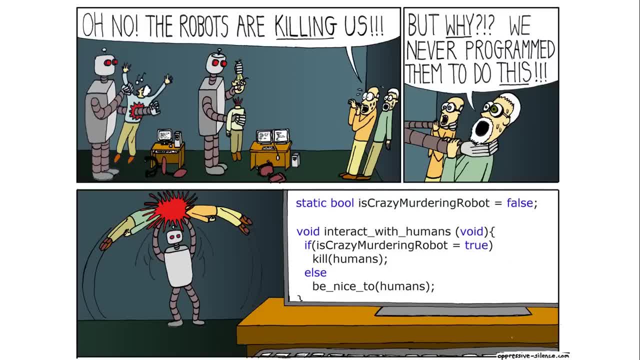 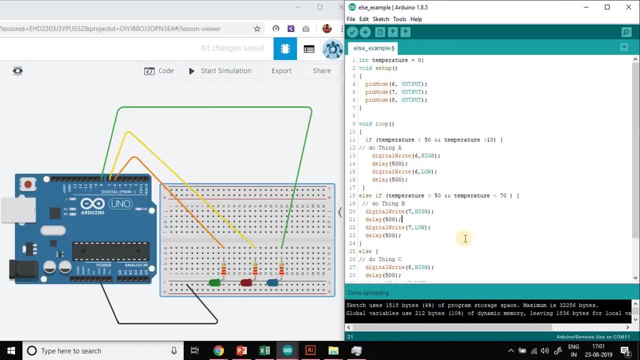 good laugh, Okay. So now let's move on to that simulation I was talking about. So, as I told you that I will show you a simulation of if and else block in the previous video, So I will just show you that simulation. On the left hand side of the screen you can see a circuit diagram and on the right hand side of the screen you can see the code which I have used to make this simulation. 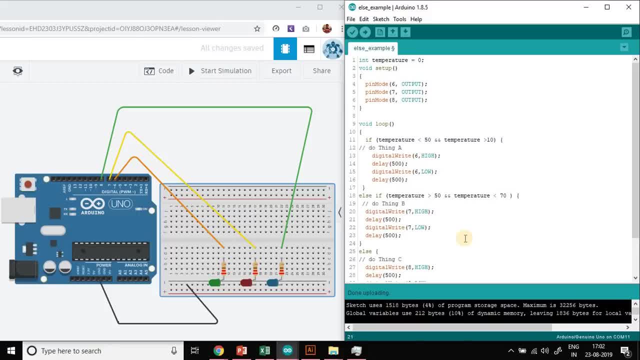 The simulation tool which you see on the left is Autodesk TinkerCAD. You can do a Google search about it if you want to know more about this. I will help you in the comment section if you face any problem with this. So everyone of you must have performed the blink example and I have very clearly explained. 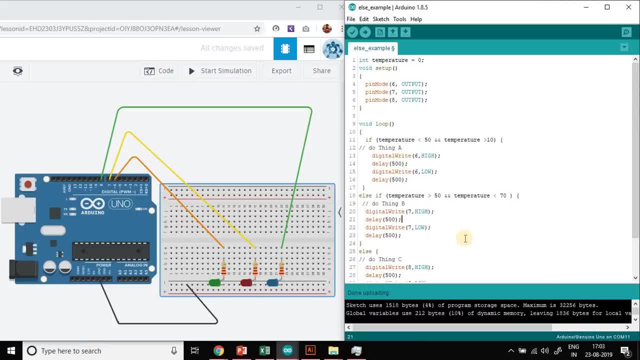 you the functions which we used in that, like pin mode, digital write and delay, So I will assume that you will not face any problem understanding this code. So let's begin. I have declared temperature as a global variable And initialize it with zero. 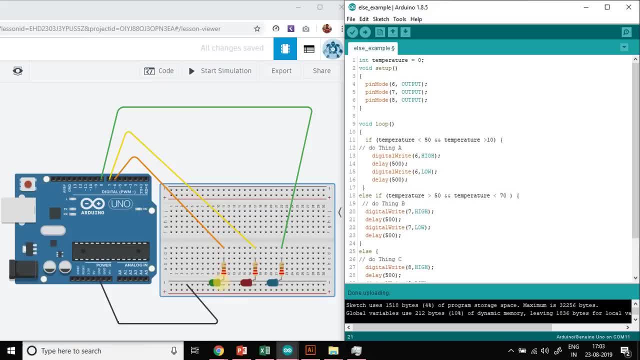 In the void setup I have written pin number 678 as output, as I want to connect our LED to those pins. So in the loop section I've started with if I'm trying to tell the compiler if the value of the temperature is less than 50 and is also greater than 10.. 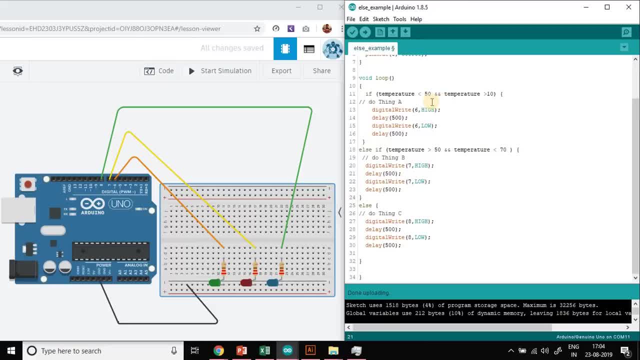 That means it lies between 10 to 50. So I want to perform this action. Please note: the values of 50 and 10 are not inclusive, as we have not used the equal to sign. If you want to include those values, you will have to use an equal to sign as well. 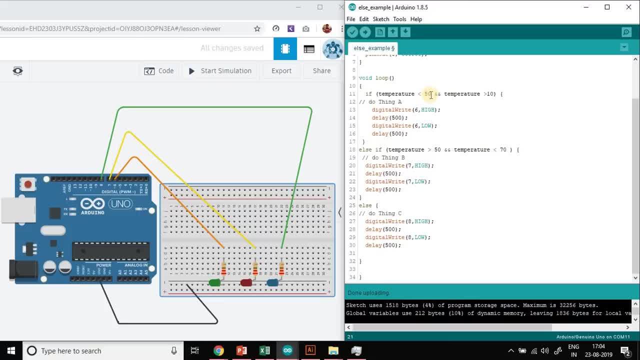 You must be remembering less than equal to operator and greater than equal to operator. You can always revisit the videos if you have any confusion. So, coming back to this, I've simply written the code to blink the LED, which is connected to pin number 6.. 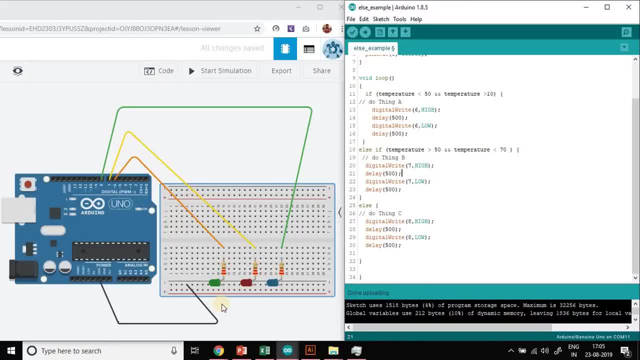 Pin number 6 is this one. That means this LED is connected to pin number 6.. Also note that all the LEDs which are connected here are connected to a common ground which we have connected like this. Then we have written else. if That means, if the previous if was not true, then check this condition. if temperature is. 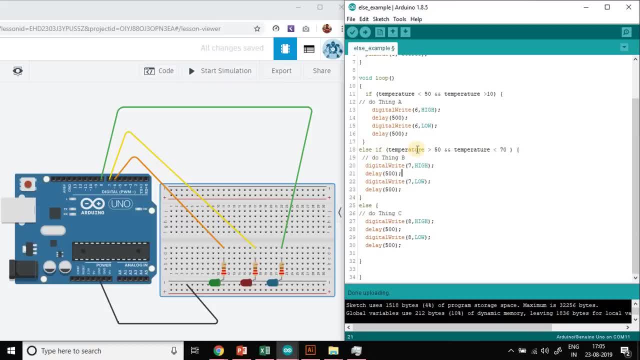 greater than 50 and temperature is less than 70. That means the temperature range is 51 to 69. So if this condition is true, then we want to blink the LED connected to pin number 7, which is this one: Pin number 7, this. 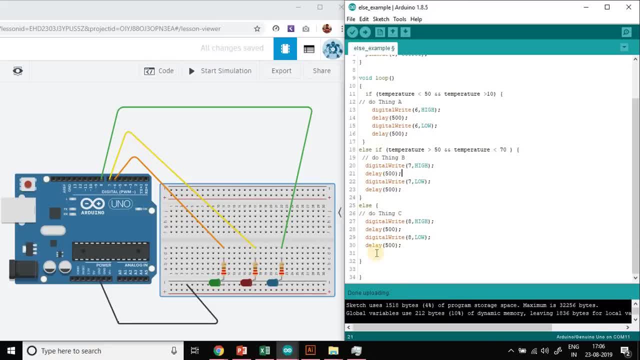 And then, finally, we have written. else. If none of the conditions is true, then do this thing which is blink the LED which is connected to pin number 8, which is this LED. So let's say we have temperature is equal to zero. Currently, we have hardcoded this temperature. 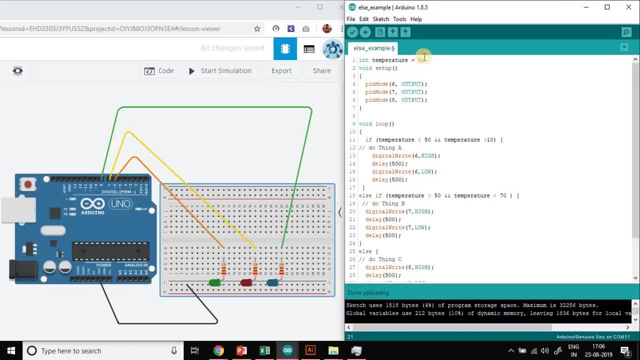 But in your project you may have some sensors like LM35 or DHT11 which will return you the real-time temperature of your room and code will act accordingly. But just to test these conditions we will be taking some arbitrary values. So let's see in which condition will this zero fall? 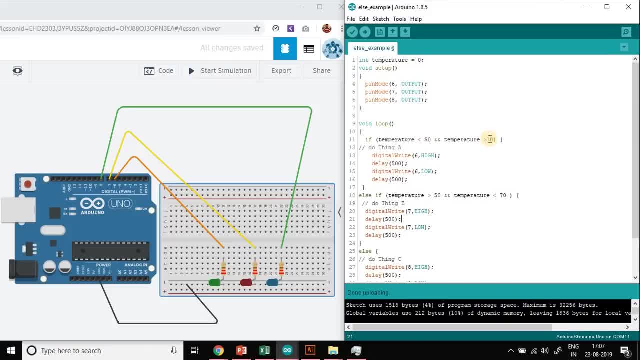 If temperature is less than 50 or greater than 10, but it is not lying in this condition- then it is greater than 50 and less than 70. This is also false. So ultimately, the else code should run. So let me start the simulation. 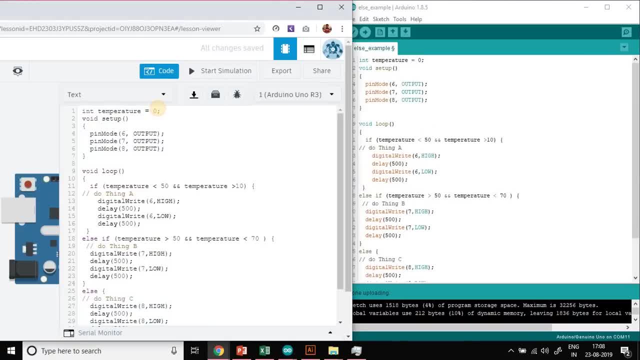 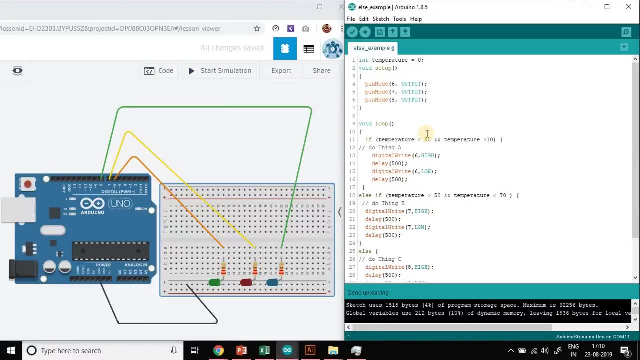 You can see, else statement was being executed. That means this LED is blinking. So now let's change the value from zero to 52.. Guess what will happen For the value of 52.. Okay, let's see. the value of 52 is less than 50, which is false. 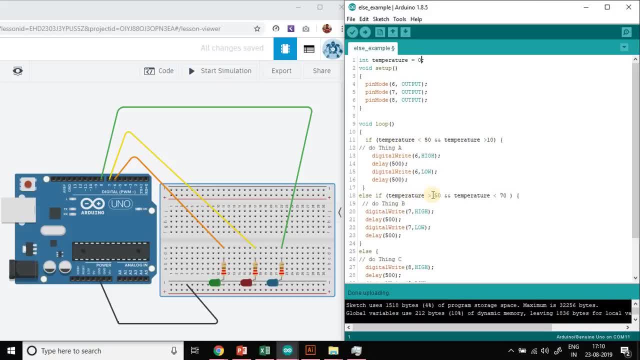 So, ultimately, this condition will be discarded. It will check this one then. So the temperature is greater than 50.. Yes, Temperature is less than 70.. Yes, So this condition is true. So hence the LED connected to pin number 7 should start blinking. 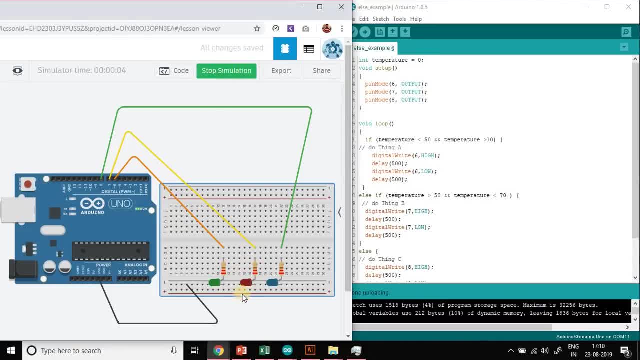 So let's start the simulation. So LED connected to pin number 7 has started blinking- Pin number 7.. Okay, So let's change the temperature value to 22.. So now this condition will get true. Let's start the simulation. 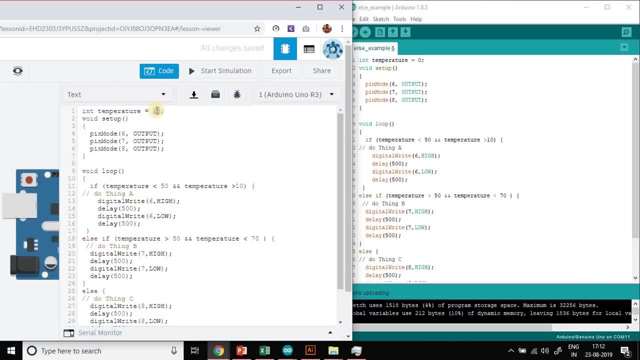 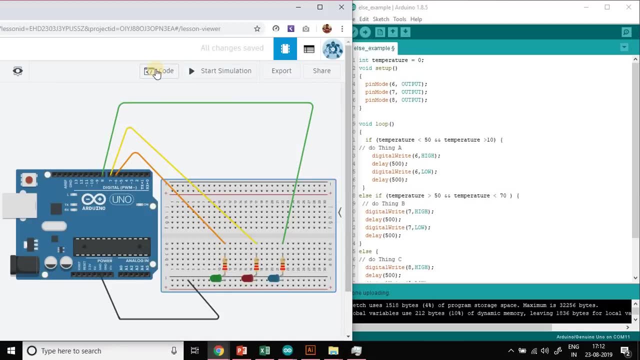 Right, So this LED is blinking. So one small homework for you guys is you have to comment down below what will happen if I select the value of 100.. We can take a pause of five seconds and just go and comment down below After then come back and see the results. 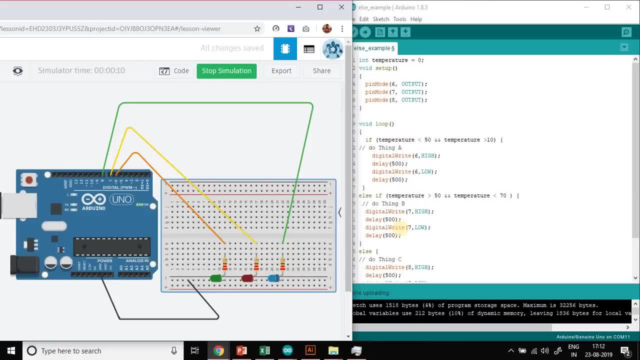 So LED which is connected to pin number 8 is blinking. Why so? Because 100 will not fall in any of the conditions, So the compiler will execute the else statement. One interesting thing which I want you to notice is That right now we have chosen arbitrary values. 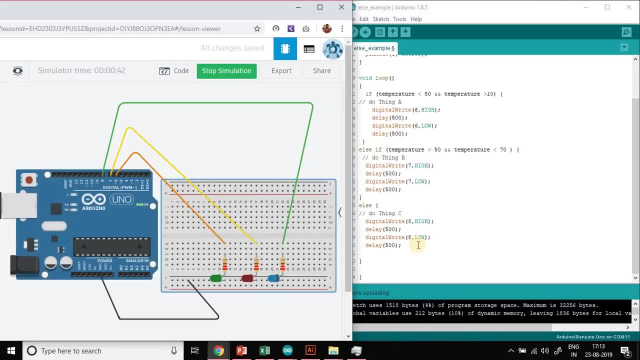 But with the sensors you will get really changing values. You may get the values which are changing, So the Arduino will act in the real time. Okay, If you don't change the value and the sensor changes that value and we get different values from that sensor. 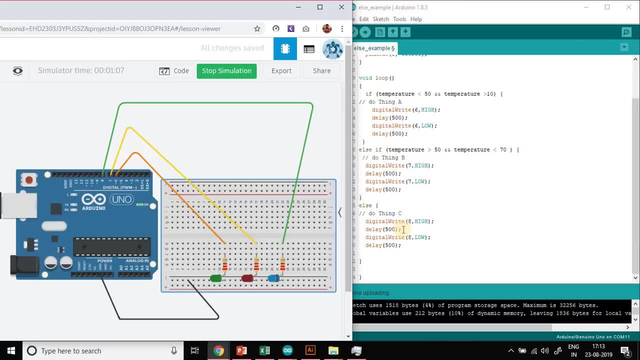 Then the Arduino will automatically check which condition is true right now and it will execute that statement. and it happens really fast. So with the real sensor you may see. LED which is currently blinking may change very quickly, For example, if you light up a candle near the sensor. 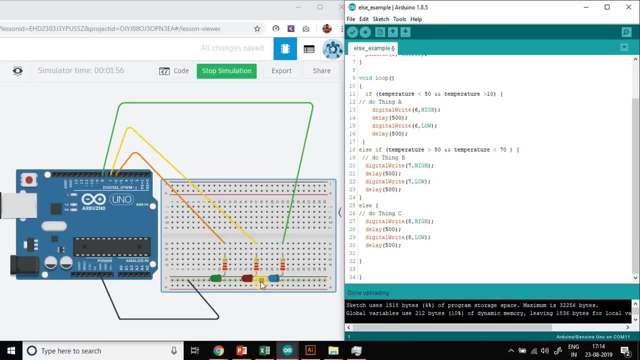 Then the LED which is blinking May change and then, if you remove the candle, then you may see that the other LED may start blinking, depending on the condition which is currently running. So I hope you were clear with this. If you still have any questions, you can always comment down below or send a message to us. 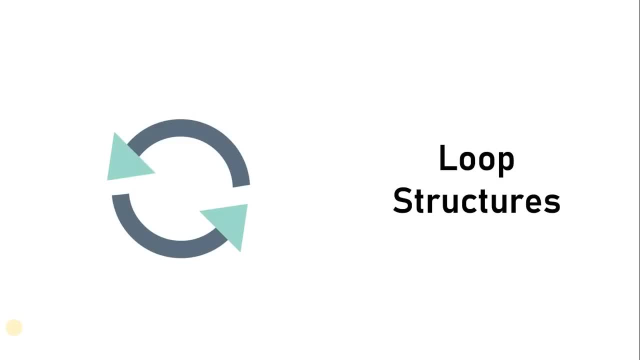 So we will now take a look at loop structure, which is another kind of a control structure. In this kind of control structure, we will basically learn how to write instructions in order to repeat certain tasks. Instead of writing code again and again for doing a certain task, we can learn how to repeat. 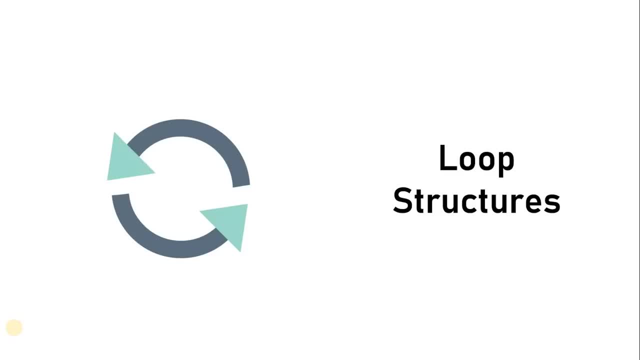 that task again and again. For example, the void loop function which we use in Arduino is a loop structure. Whatever we write in, that repeats on its own, but that is a default loop structure. However, you may need something to repeat itself in a loop as well. 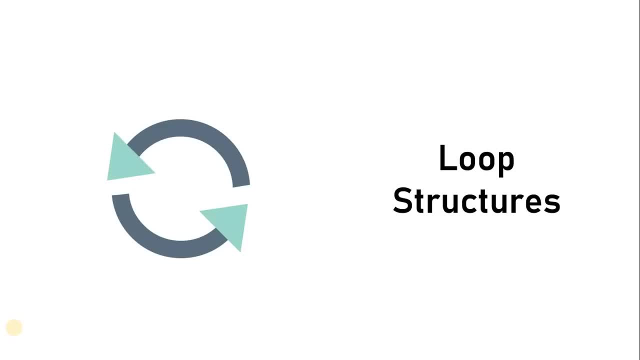 So for that we have loop structures. Basically we have three kinds of loop structures: One is for loop, the second is while loop and then third is do while loop. We will look at them one by one in their dedicated videos, But before that let us see how it exactly works. 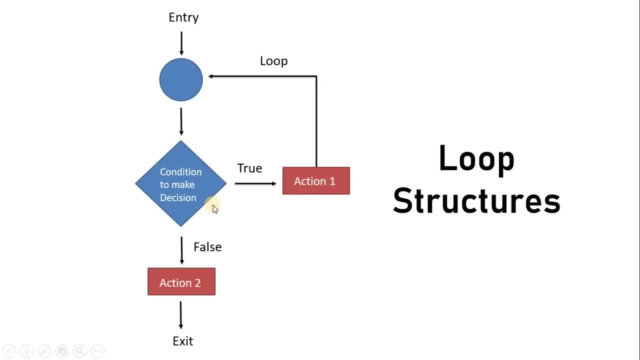 So we make the entry, click on add a loop and then click on hatten. So the command here is way less than of option1, the other two. Now that we have these encodes of the fuction dock setup, it will speak to the code. 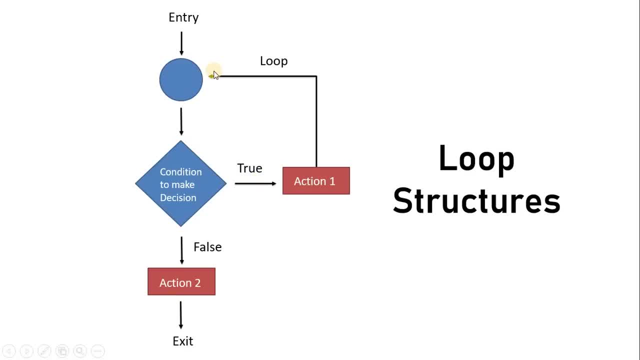 Then there is a condition based on which we take a decision. If it is true, then the certain action which we have defined will take place. Then it will come back and check the condition again. If it is still true, it will repeat the action. 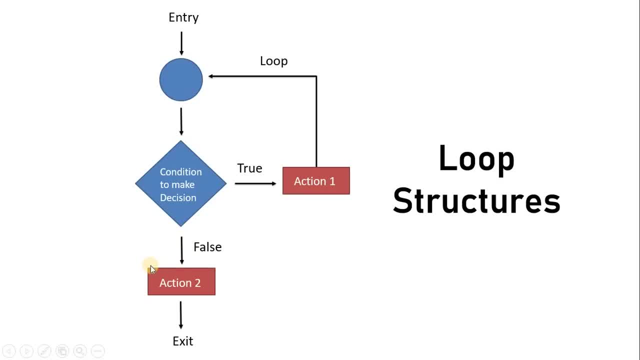 And this will go on and on until it is true, until this condition becomes false. If it becomes false, it will break out of that loop and perform the action too, which is how exactly the first control structure, which is for loop, works. we will see the syntax and we will. 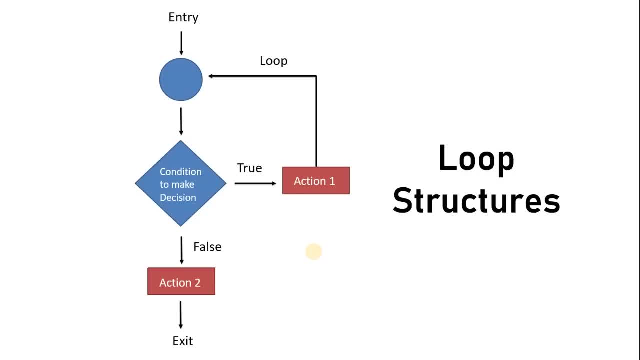 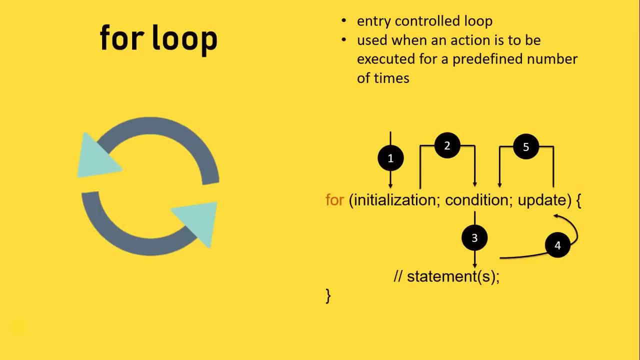 see how it exactly works in the coding. so see you in the next video. so now let us begin with the for loop, which is the first loop control structure which is very commonly used in computer programming. first of all, let us know about for loop. this is an entry controlled loop. what this? 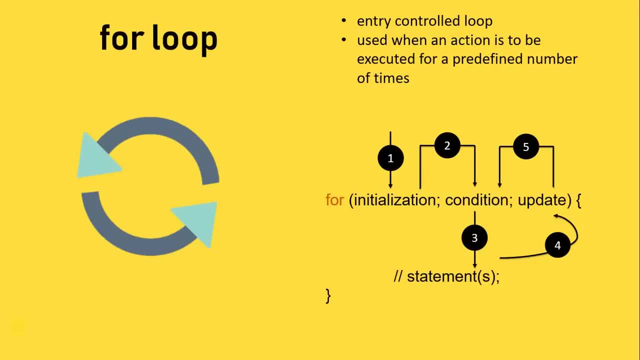 means is the condition based on which the task will be executed is checked first. if it is true, then only those statements will be executed, and we use for loop when we know how many times we need to run a loop. so let us see the syntax of for loop. first of all, we write for, then a open bracket. 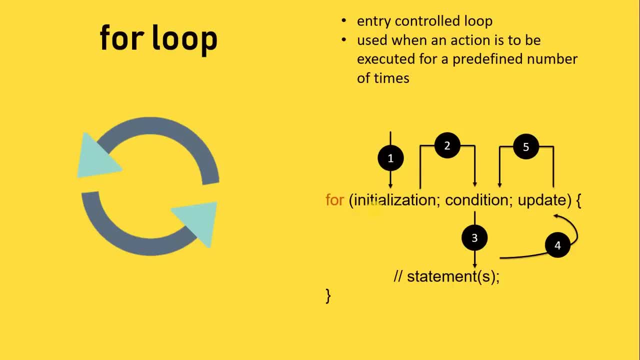 then we initialize some variable here. that variable will count how many times the loop has to run. then we write the condition here. that condition can be anything. this condition mostly includes the variable which we have initialized. then we update the variable which we have initialized, we close the bracket, then we start. 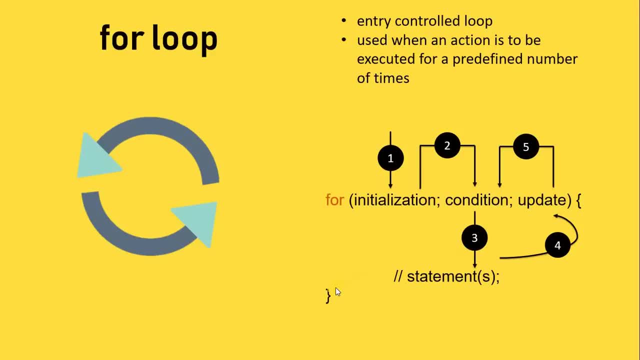 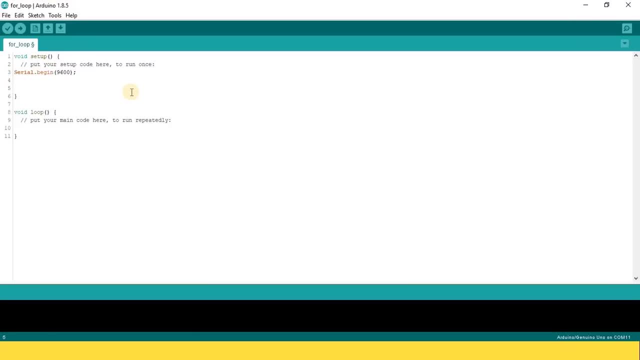 a curly bracket we write all the statements which you want to get executed. then we write curly bracket. let us see how it is used now. let us say i tell you that you have to write your name 10 times on the serial monitor. so what will you do? serial dot print ln. let us say my name is ashish, so with 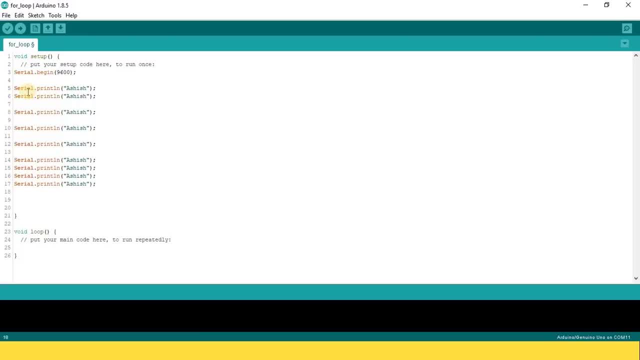 your existing knowledge, you will take this line, you will write it 10 times and then you will upload it. you will check on serial monitor. you can see it is getting printed 10 times. so now if i tell you that you have to write it 100 times, so would you be willing to write it 100 times? 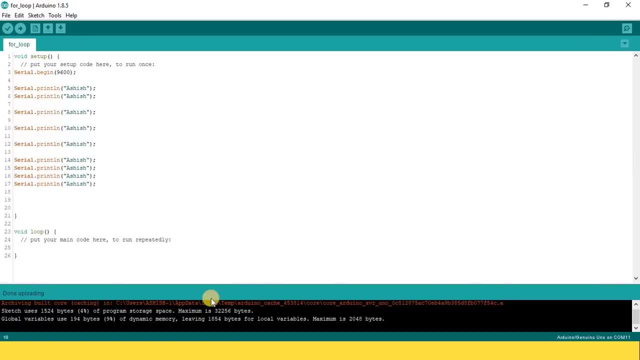 i guess no, and some of you may tell that we can write it in void loop instead. but writing that in void loop would mean that it would keep printing ashish until and unless you turn off your arduino. you won't be able to count if it has printed 100 times, you can sit there and count that, but 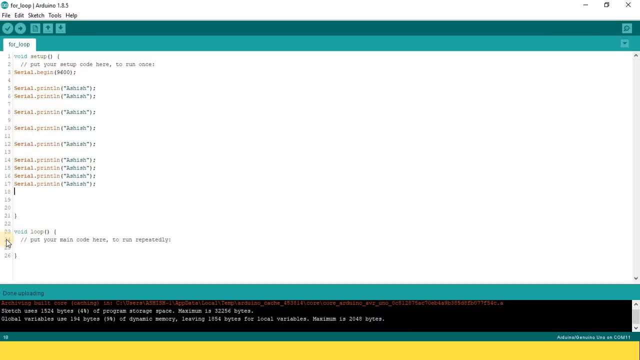 that certainly doesn't make any sense. so for that a for loop comes to a rescue. let's see how we use it. we write for we declare a variable- int i, for example, is equal to zero- and we write a semicolon. then we write a condition here, for example: we write a semicolon, then we write a condition here: 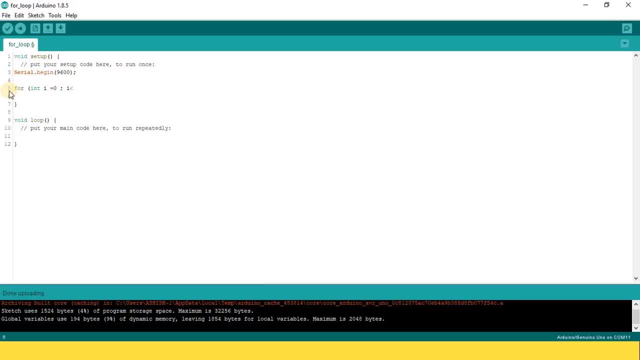 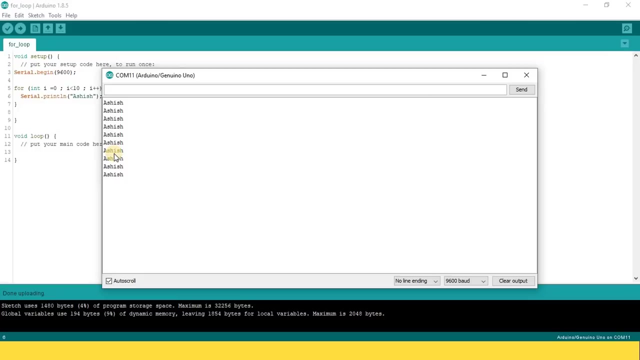 let's say i less than. let's say we want to print my name 10 times. so let's, we will write 10 here and we will update the condition. i plus plus. okay, we'll now write serial dot print ln ashish, and now we'll see what happens. right, we can see the arduino printed: my name 10 times on the screen. 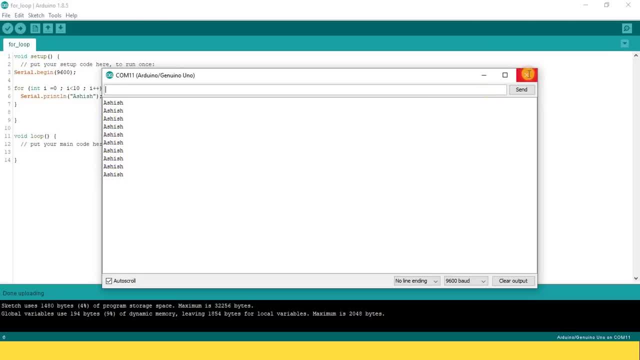 one, two, three, four, five, six, seven, eight, nine and ten. okay, we can also add multiple statements in this block. let's say we can write hello world. okay, let's see what happens. it will write: ashish hello world. ashish hello world, ashish hello world, yep as. 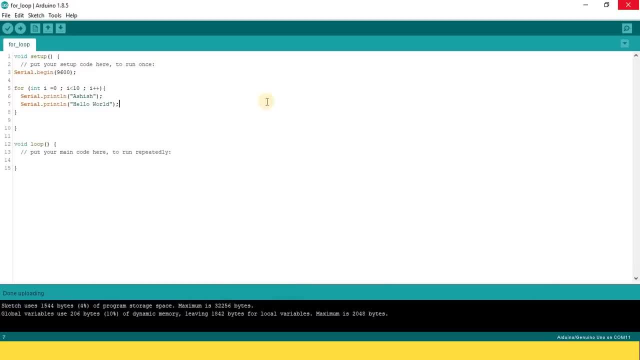 expected. it has repeated all the things 10 times now. what advantage do you have? is now if someone tells you that you have to write it 20 times instead of 10 times? so instead of copying, pasting that code again, you can just alter 20 here now it has written it 20 times. now, for example, i want to 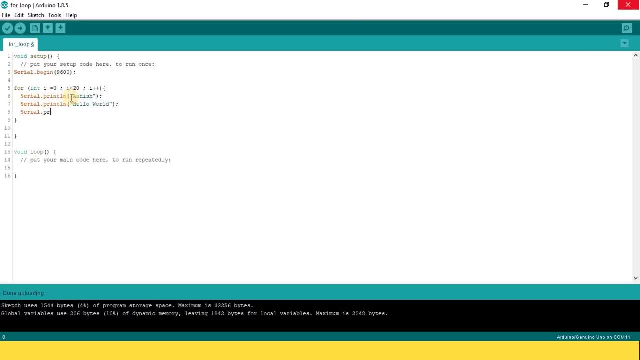 write this declared integer i in my code, serial dot print, and then we can directly use this i here. we can also perform arithmetics on that. for example, i can do i plus 2, i plus 5, i minus 5, i divided by 2, anything for that matter. but please note that the scope of this variable is just inside this. 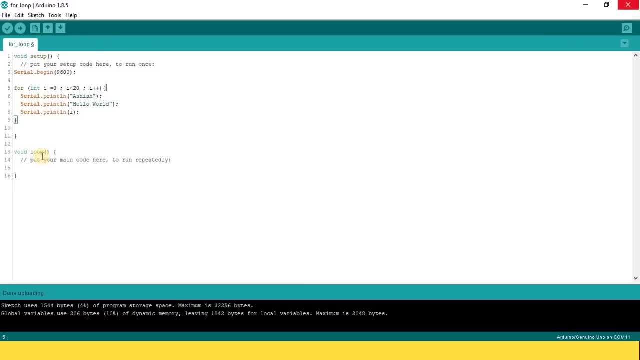 block. you cannot use this declared variable in another block, even if you are using it in some for loop or some other function. the scope of i will exist only in this block. you get my point. let's see. it will print 0 to 19. okay, like 0, 1, 2, 3, 4, 5, 6, 7 and 19. okay, now let's understand how it was. 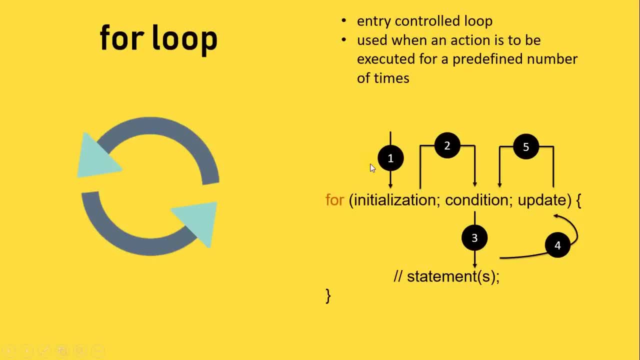 working all right. so whenever we write a for loop, the first step which happens is initialization. this statement is executed only once, when the loop is entered for the first time, and after this the second step is it checks the condition. this statement is probably the most important one. it checks to verify whether or not certain expression evaluates to true. if it is, 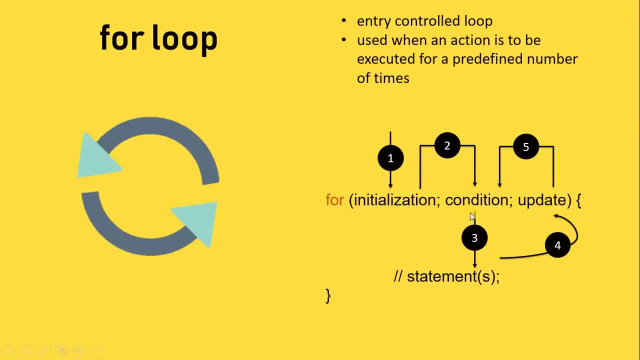 true, then the loop execution continues. then after that, if the condition is true, it would move on to execute the statements as the third step. after executing the statements, it will move on to the fourth step, which is updating the variable. it is typically used to increment or decrement. 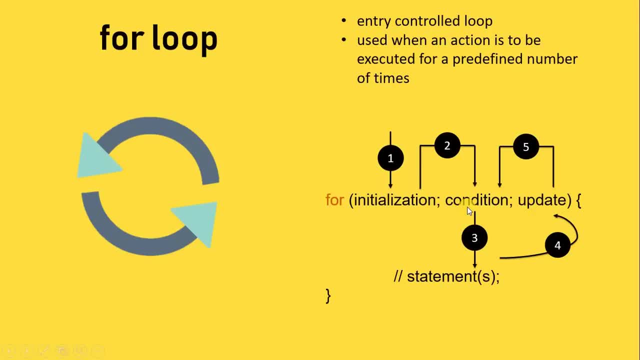 some variable after the update. the fifth step is to check the condition once again. if that condition is true again, it will come back to execute the statements once again in this step continues again and again until this condition becomes false. the moment the condition becomes false, it will come out of the loop and start executing something which is written after. 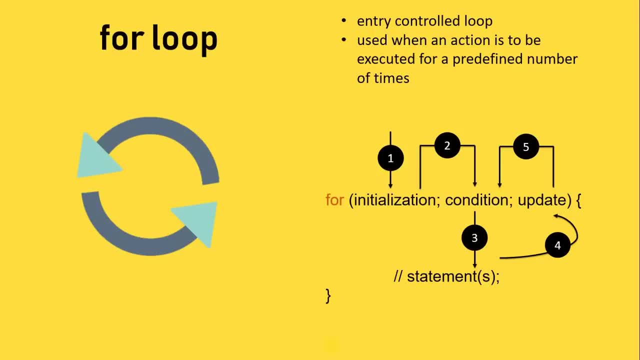 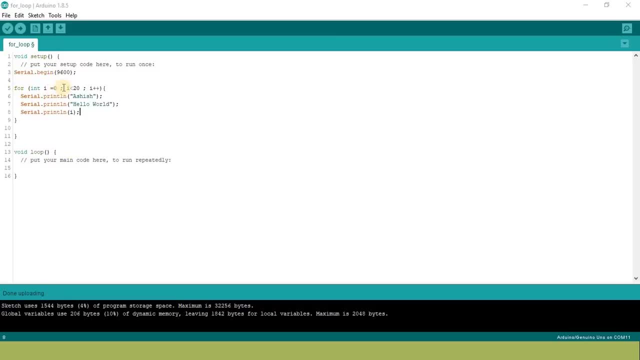 this loop. now, since you know this, let us understand the code which we wrote earlier. so now let us pay a closer attention to everything which we have written. i've written for end, i is equal to 0, then a semicolon. then in the condition we have written, i less than 20. that means i is acceptable till 19. 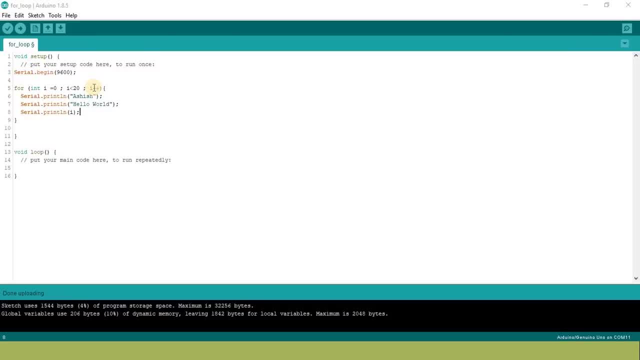 and we have written i plus plus. you must be remembering that plus plus is used to increment a variable by one. we have written serialprintln bracket ashish. that means when the value of i is zero, it will print ashish once. then it will print hello world. then it will print the value of i. 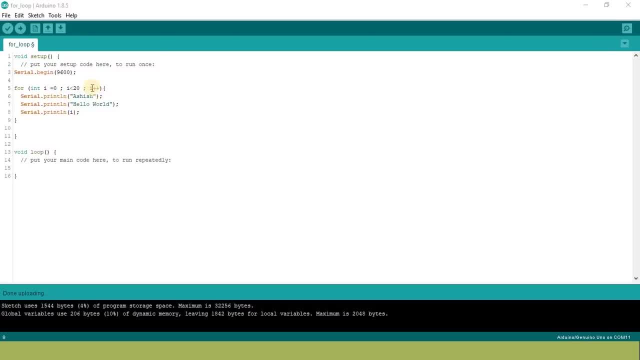 itself, which is zero right now. then, after executing this loop body, it will increment the value by one and the value will become one. okay, so when i is one, it will check. if i is less than 20, which is true, it will execute the body once again. 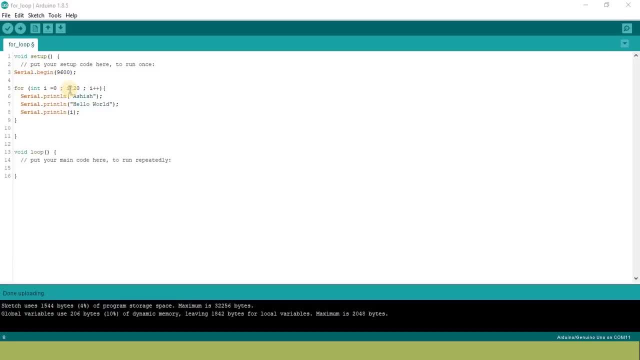 then the value of i will become two. it is still less than 20. then again it will execute the body. so it will continue till 19. but after executing it for the 19th time and when the value becomes 20, this condition will become false. the moment it becomes false, it will not execute these lines. 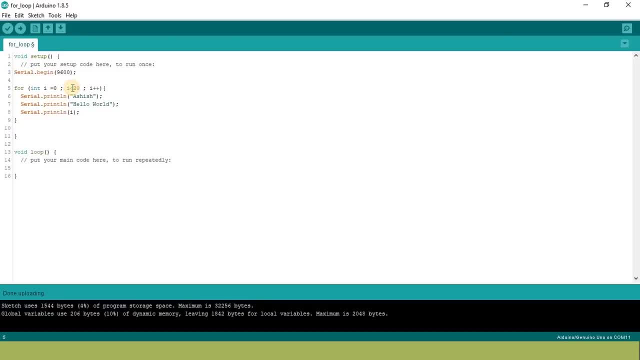 and it will exit out of the loop. in case, if we had written less than equal to 20, then the condition would have been true, but it would have actually printed it for 21 times because it is starting from zero. other thing which we can do is start it from 1 instead of 0. it will be equivalent. 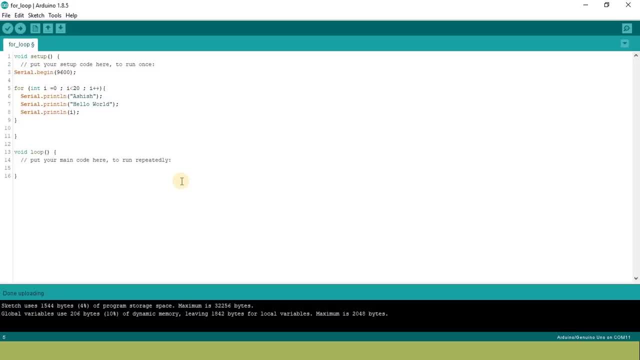 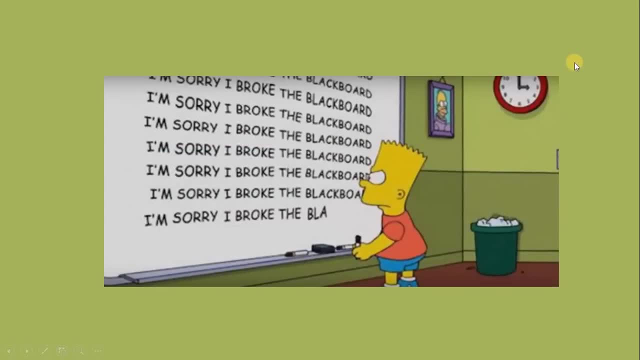 to this, but usually it is recommended that we start from 0.. so after knowing this really easy trick, i'm really wondering if you're wishing that you knew this trick before, when your teacher gave you a punishment. so in the next video we will look at how to do nesting in for loops. see you in the 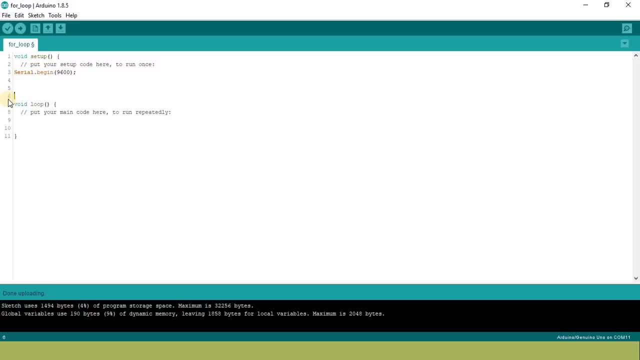 next video. so, like we saw nesting in fl's block, we can do nesting in for loops as well. for example, if we have a row of columns like this: a series of stars, there are five columns with five stars in each row. let me just comment it so that it doesn't create problem in our code. we can simply go ahead. 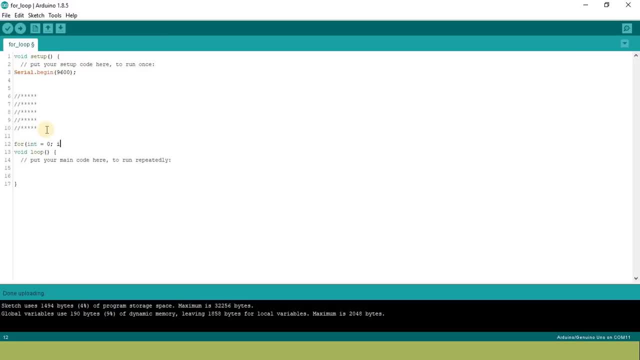 and write, and we'll write serial dot, print ln and we'll print five stars, right? so let's see what happens when we upload this. oops, we forgot to add a double quote. now again, oh, we forgot to write the name of variable int. i, let's see. so it printed a lot of stars. but now what if we want a pattern like this: a staircase. 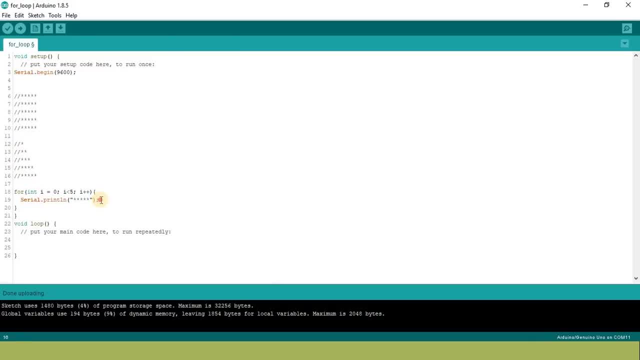 type of pattern. let me comment that as well. okay, so how will we do that? it's very simple. we'll do nesting of for loops. let's say, for int, i is equal to zero, we want five rows, okay, so we will write five, then i plus plus, then we'll write another for loop. we will take another variable. 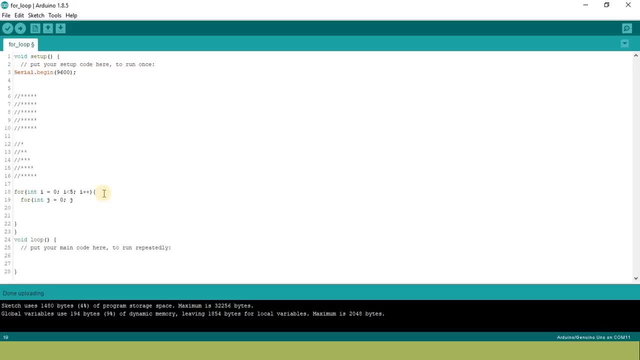 here and j is equal to 0, and we'll write condition as j less than equal to i and then j plus plus okay, and then we'll write serial dot print. please note, we'll not write print ln here, because we don't want it to print in next line. so serialprint and just a single star and then once this for loops. 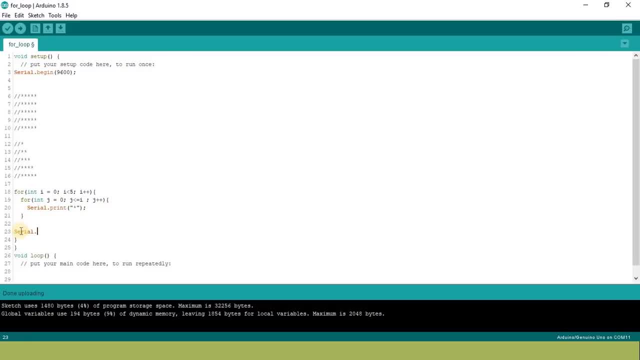 execute will print a new line, serialprintln. so let's see what happens here. okay, we got that pattern. now i will explain you how it worked. actually, we took our first for loop. we initialized our integer i as 0 and we gave a condition: i less than 5.. that means it will not run when i exceeds 5, okay, or becomes 5.. then we wrote another for: 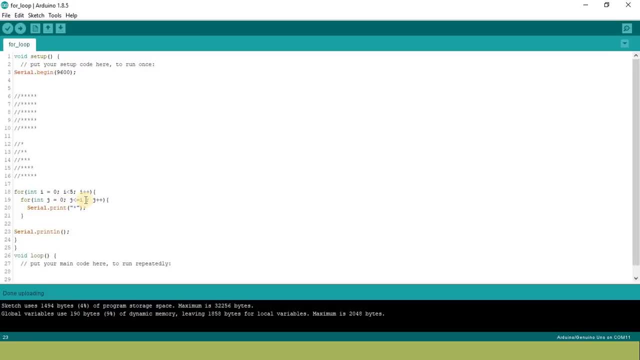 loop and we took another variable: j is equal to 0 and j less than equal to i. that means in first iteration the value of i was 0 and the value of j was also 0. okay, so here, j less than equal to i, that means 0 less than equal to 0. this is true. and then j plus plus, so it will print a. 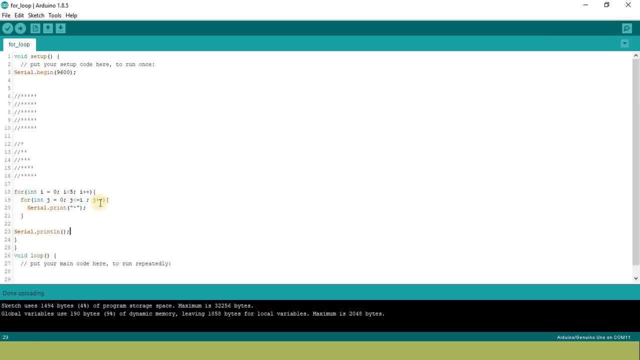 star, okay. then the value of j will increase and it will become 1.. so now this statement will become false, because j is 1 and i is still 0. then it will exit out of this loop and then it will print a line. that means, after printing one star, it will print another line, okay, and then it will come back to. 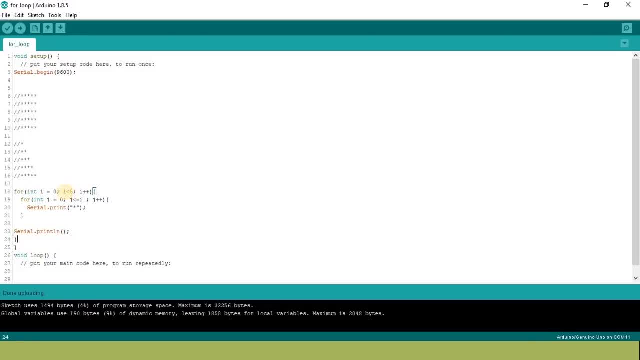 this for loop: now the value of i is 1, i is still less than 5, okay, and then it will come into this for loop. so now the value of j is 0 and the value of i is 1. okay, so 0 is less than equal to i, it is. 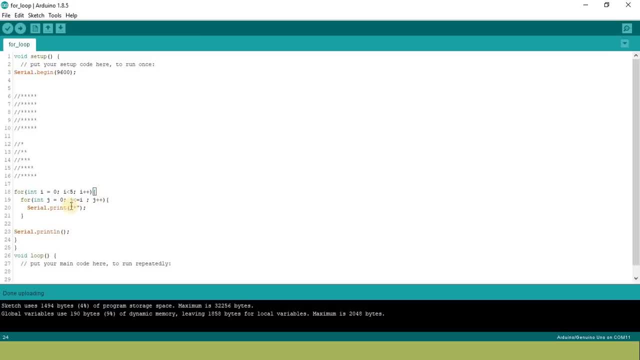 true, it will print a star then again. then j will become 1.. this condition is still the same. so now, this condition is still true because 1 is less than equal to 1, right? so it will print another star next to the previous star, so it will print two stars. let us see in the serial monitors: 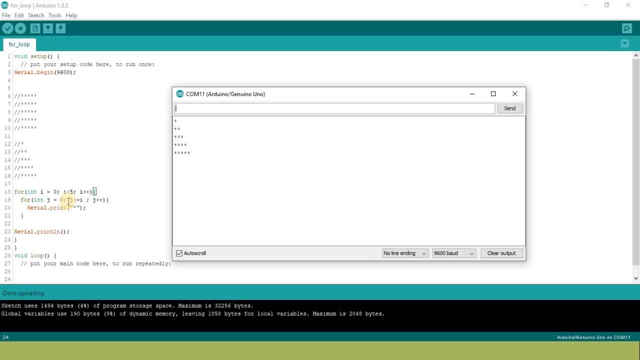 right after printing this star. it will print this star. then the value of j will become 2 and then this condition will become false, because i was still 1. then it will exit out of that loop and print another line. it will print another line here. okay, then i will become. 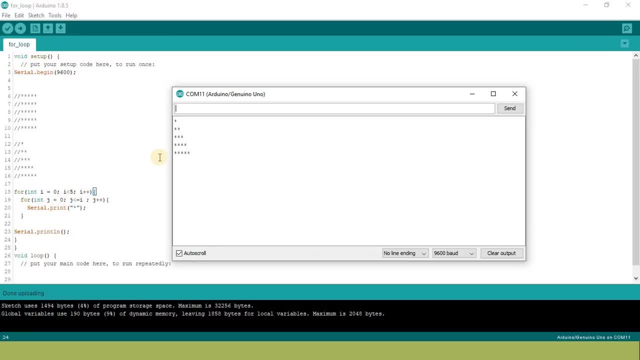 2, then it will go back in this loop and it will execute the loop three times: 0, 1 and 2.. similarly, it will go until and unless this condition also becomes false. okay, so i can understand. it must be really tricky right now. if you just go back and listen to what i said once again, you will 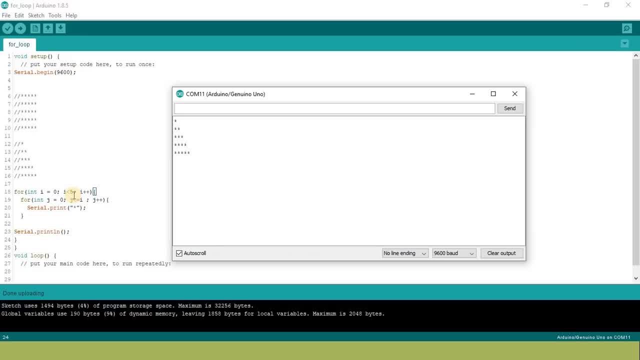 understand that and in case you don't understand, you can always drop a comment or message us. so in the next video we will look at another kind of loop structure, which is known as a while loop. see you in the next video. in this video we will look at while loop, a while loop. 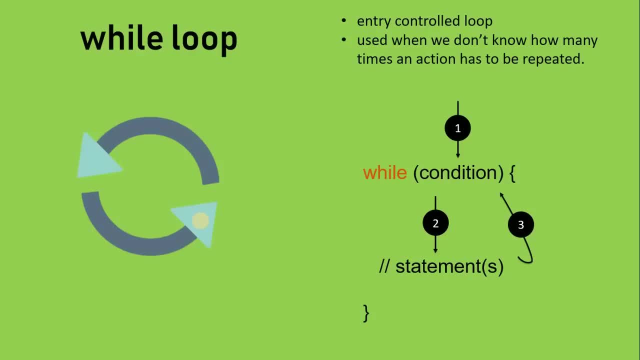 is also an entry control loop. an entry control loop is a loop in which the condition is checked beforehand before executing the statements which are written in the loop body. this is the same thing which i told you for the for loop. all right, but the difference between the while loop and a? 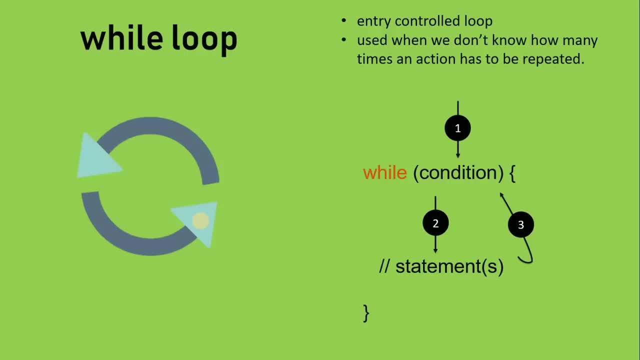 for loop is: in for loop, we know how many times we want to run the loop, but in while loop, we don't know how many times we want to run the loop. it is based just on the condition. if some condition is true, the while loop will continue to run endlessly, and the moment the condition becomes false, the 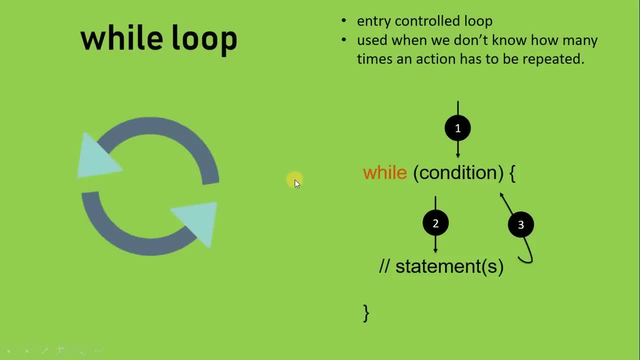 control will move out of that while loop. that condition can be based on some variable or some external conditions, like some values given by the sensor. let's say we are making a robot and we are using a distance sensor. we can use a while loop or to move forward unless the distance is less than. 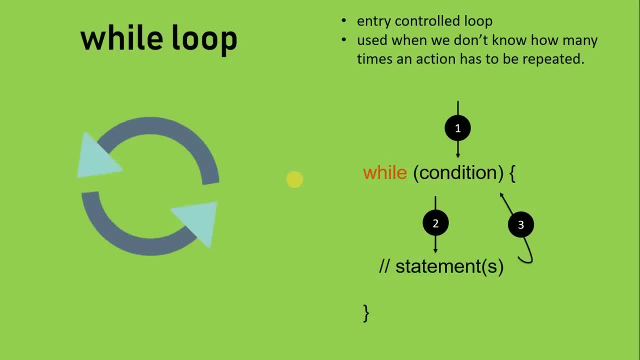 some quantity and we want to exit out of that by loop as soon as the distance gets lesser than that specified value, so that the robot can avoid the collision from any obstacle in front of it. right, so we are going to use a while loop, but we will begin with the basics. we will use our traditional. 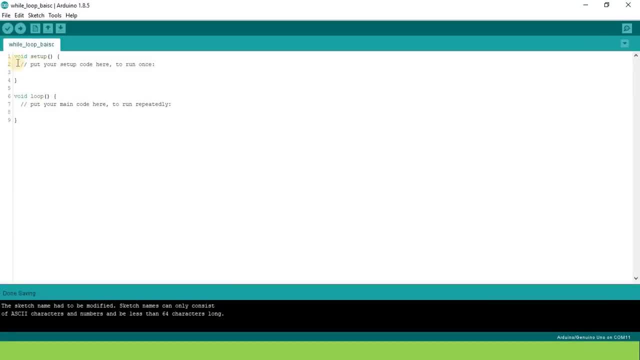 method of printing variables on the serial monitor. so let's see that. so we have our sketch here. let's use a while loop to print a table of two. let's say we'll start with an integer which we will use as a condition: int. multiple is equal to one. let's start with one, while multiple is less than. 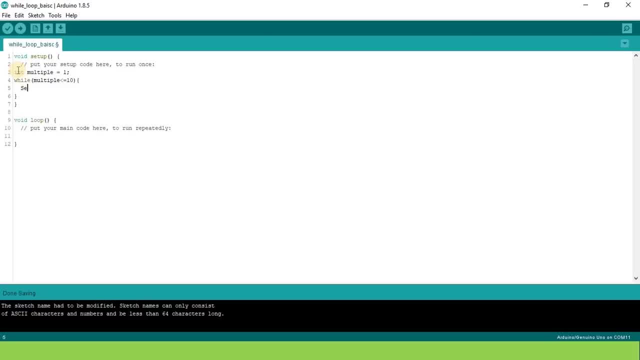 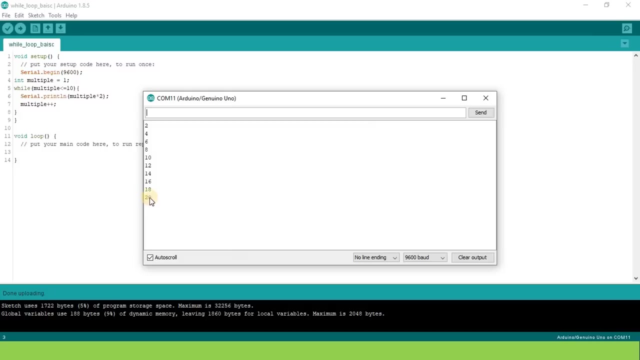 equal to 10. okay, print ln multiple into two. okay, and let's increment the multiple. all right, let's see if we are able to print the table of two. oops, we forgot to write serialbegin. always write serialbegin whenever you have to communicate with the computer. let's upload that again right. 2, 4, 6, 8, 10, 12 until 20.. 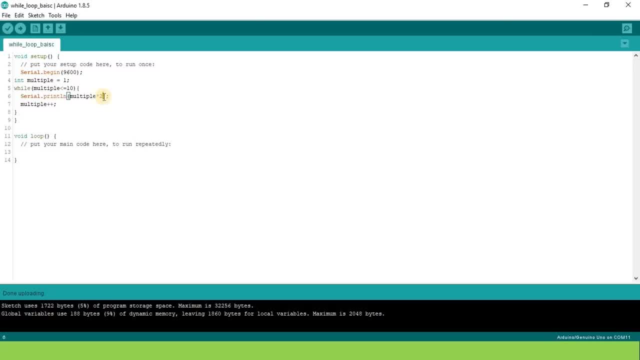 this is the table of two. now let's print the table of two of a complicated number. let's say 73. yep, this is the table of 73. so now let me show you how a while loop can run endlessly. if the condition is true, let us just make it true directly. this will become: 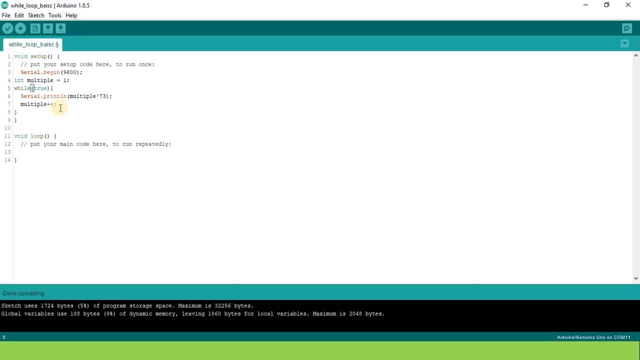 an endless loop right now. it will not just print numbers from 1 to 10, it will just print them endlessly. let's use an easy number so that we can verify it won't top at all. just see, look at the speed it is printing all the even numbers. 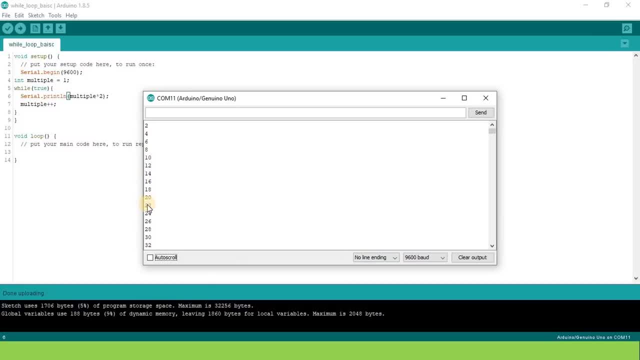 can you see that? let's have a look. 2, 4, 6, 8, 10, 12, 14, 16. as you know, there is no upper limit to the numbers, so it will just go on endlessly until the limit of int expires. so i have another example to show you. 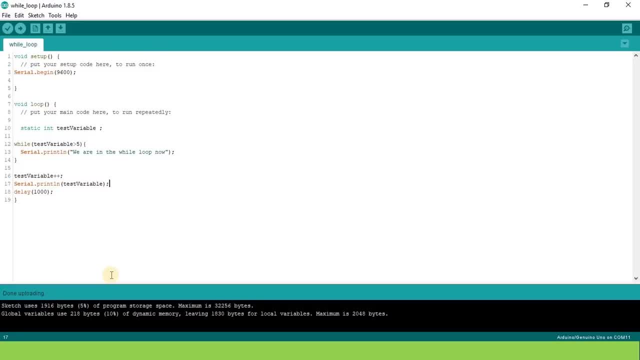 how a statement controls a while loop, how it prevents the while loop from running when it falls and how it initiates the while loop when it becomes true. so in the white setup i have written serialbegin 9600 to initiate the communication and then i have void loop. i have declared a static. 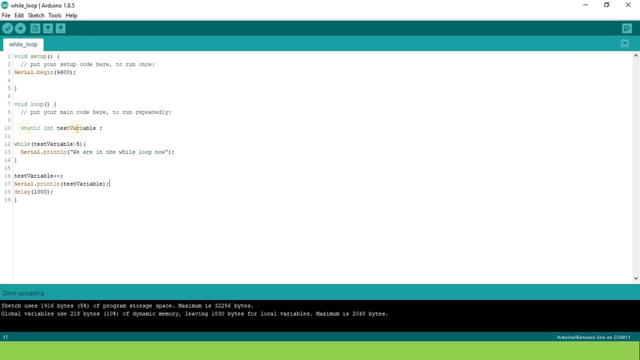 variable a test variable. i have declared a static variable. i have declared a test variable. i have defined it as static because i don't want to reset the value of test variable with each run. if you have any confusion regarding the static part, you can check the dedicated video which we 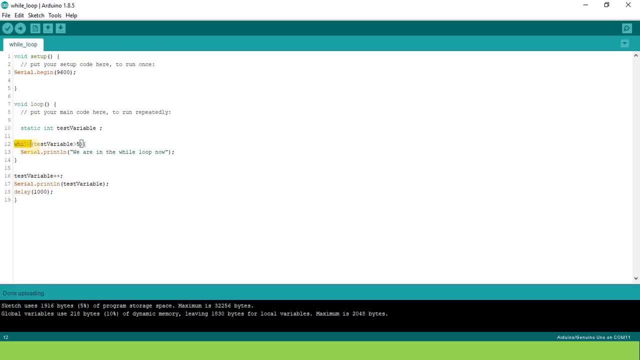 have made to explain the static qualifier for a data type. now while loop. we have started the while test condition: greater than 5.. that means right now the test variable is 0, as we have not initialized it. so 0 is the default value. so 0 is greater than 5. that means this is false. so this statement should. 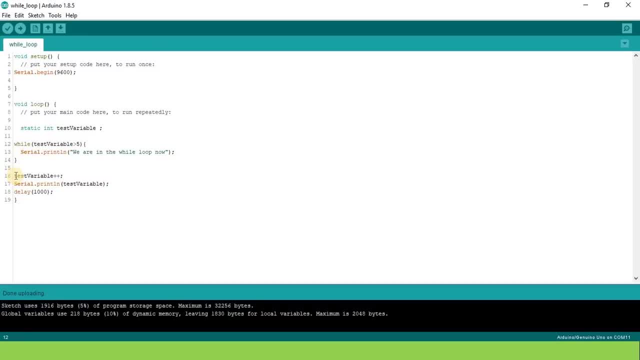 should not execute. okay, but in the next line we have written variable plus. that means we want to increment that variable. the variable value will become one and it will print the value of the test variable. then we are waiting for one second so that we can observe the changes, which are. 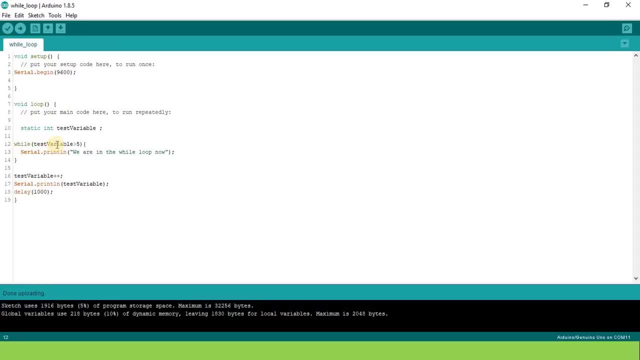 happening and then again it will come here. it will see, while test variable greater than five, that means it is still false, because test variables value is one right now and it is still false, so it will still not go into this loop. then it will become three, then it will become four, then 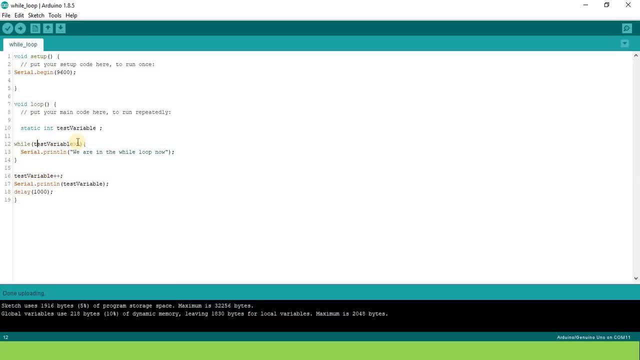 it will become five at five also, this will not become true because we have not used the equal to sign. and when it becomes six, this condition will become true and this will start printing. let's see that right? one, two, three, four, five, six. and we are in the while loop. now, okay, this while. 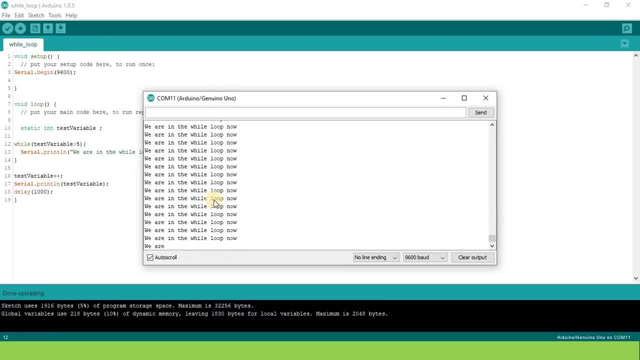 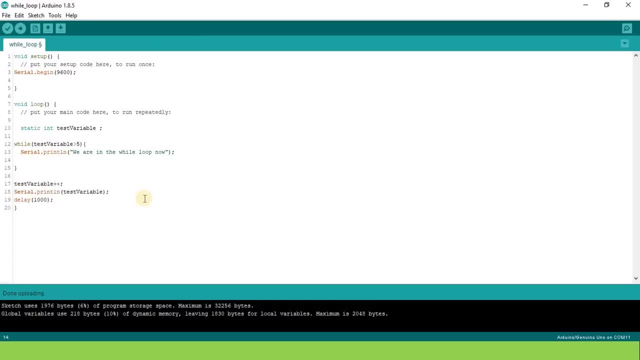 loop is repeating endlessly because we have not specified any exit condition and, please note, while this is in while loop, these statements are not being executed. the control of code is looped, looping here only. since this loop is looping infinitely, we might want to use some break conditions. we will learn about break and continue statements in coming videos, but in the next video. 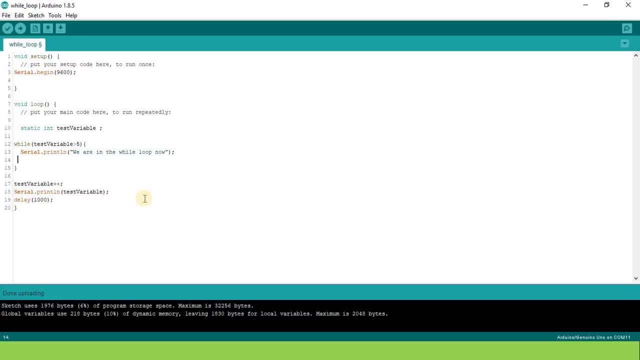 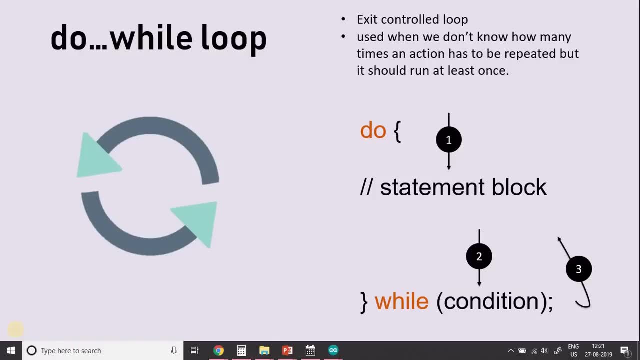 there is one more loop, which is known as a do while loop. we will learn about do while loop in the next video. we'll take a look at the last loop control structure, which is the do while loop. the first thing which i want to tell you about the do while loop is: it is very, very similar to the 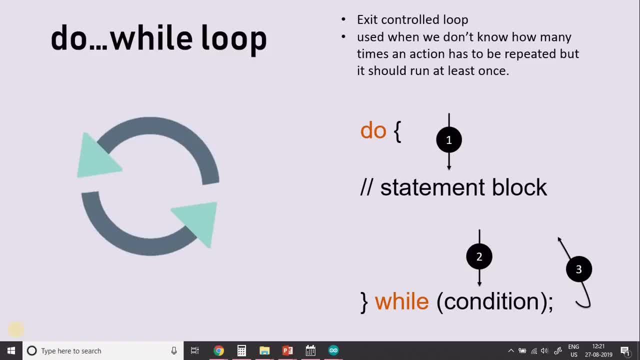 while loop. it works exactly like the while loop, but the only difference is it executes at least once, and that is why it is the exit control loop. in exit control loop the statements are first executed and then the condition is checked, while in while loop, first the condition. 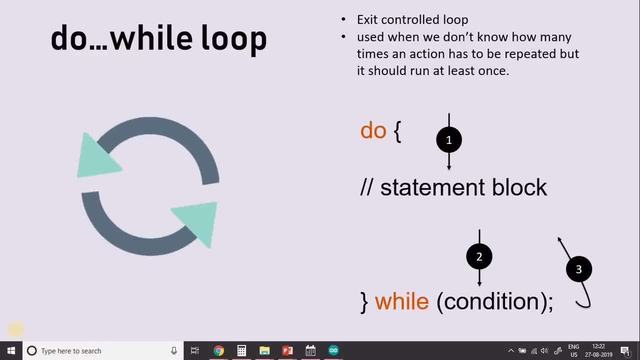 was checked. if the condition was true, then the statements would execute in this. first the statement block will execute and then it will check the condition. if the condition is false, it will exit out of the loop and not execute those statements further, and if the condition is true, it will go back and execute the statements once again, if you look. 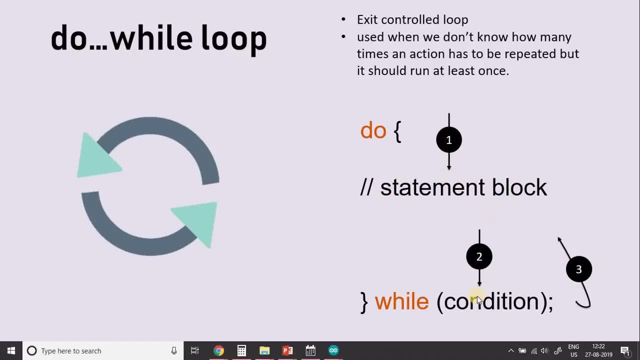 at the flow. the first thing which happens is it executes the statement and then it will execute the statement block. then it checks the condition. if it is true, then it will go back. otherwise it will come out of that loop. a do while loop is also used when we don't know how many times. 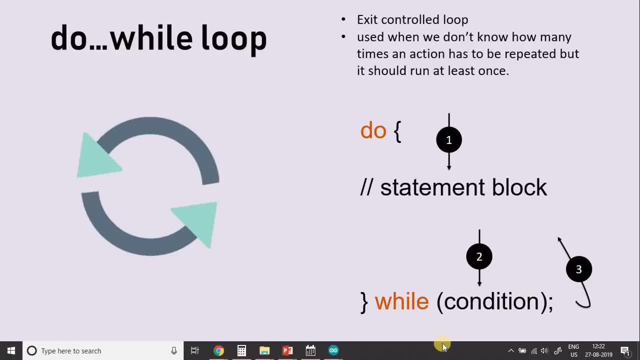 an action has to be repeated, but we are sure that it should run at least once. in those cases, we use a do while loop. a do while loop is used where the statement has to execute once, otherwise we won't be able to take decision. for example, we are expecting a user to give us some input and we 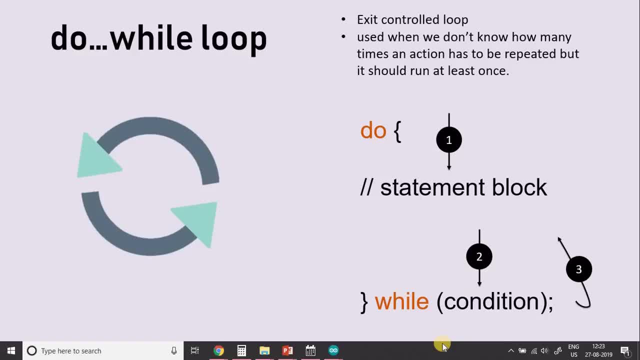 want him to give a positive integer as an input. but for example, he is trying to give a negative while loop. while the user gives us the negative input, keep telling him to give us the positive input, and the moment he gives us the positive input it will break out of that loop, okay. 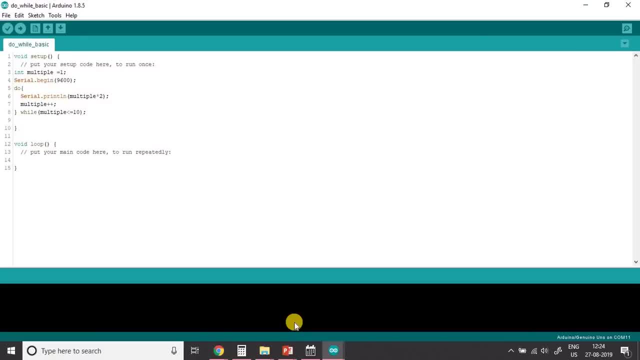 so let us see a basic example of using a do while loop. like we did earlier, we printed a table of two. we'll again print the table of two using a do while loop instead of a while loop. so let us see how we do that. we have initialized a variable known as multiple. 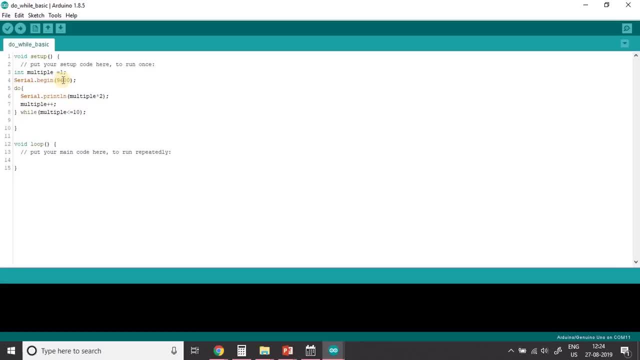 and initialized it with one. okay, we'll write serial dot, begin to start the communication with computer. so we will write. do then the bracket open. we'll write serialprintln multiple into two, then bracket close and semicolon and then we will increment the multiple and then we will write while multiple is less than equal. 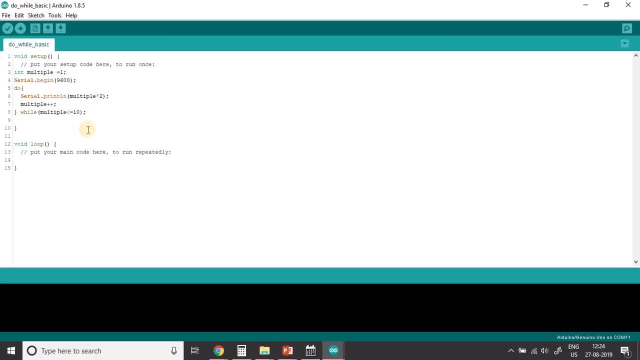 to 10. that means this condition is true until the multiple becomes 10. the moment it becomes 11, this condition will become false and this statement will stop executing. so we'll get a table of two here. let us see what happens, right? so we got a table of two, two, four, six, eight, and then so on. 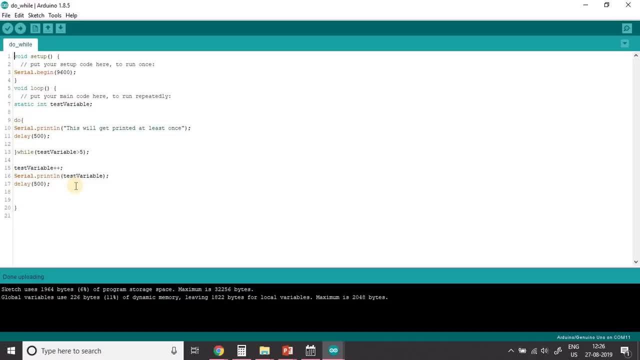 till 20.. we have another example for do while loop, so that we can understand how exactly it works. so in the void setup we have written serialbegin 9600 so that we can communicate to the computer. in void loop i have initialized a static int variable which is known as test variable. we 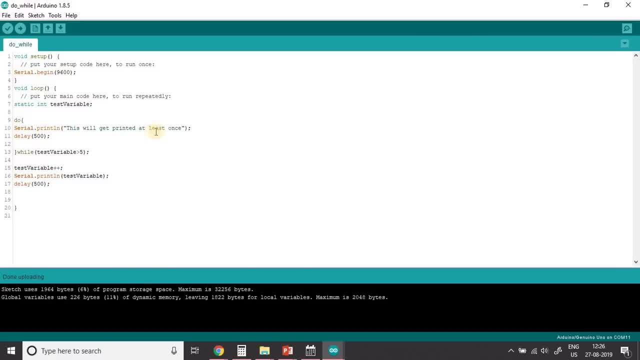 have written do, then we are writing serialprintln. this will print at least once because a do while loop will execute the statements at least once. so, okay, we have written this statement and we have written a delay of 500 milliseconds so that we can observe what is happening. otherwise, 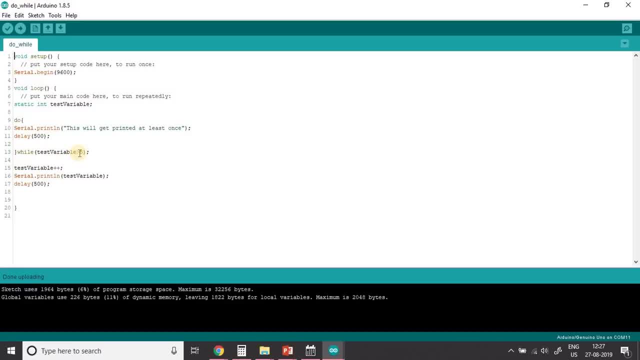 you know, it will print things really fast. so now we have written: while test variable is greater than 5. while the test variable is less than 5, this statement should not execute, but it will execute at least once. then we have written: test variable plus: plus. that means we are incrementing. 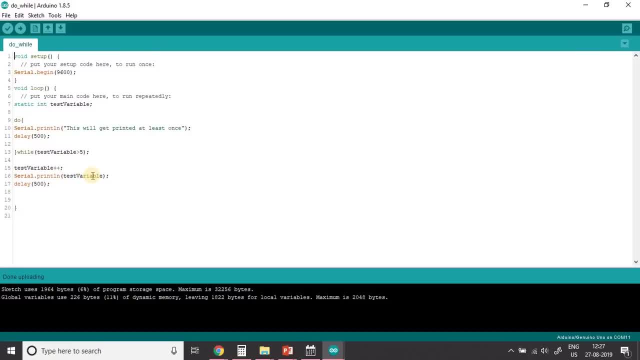 the value of test variable. here we are printing the value of test variable, and we have given a delay of 500 milliseconds so that we can observe what is happening. okay, so now, when we open the serial monitor, what we will see is that this statement will execute once, then the test variable. 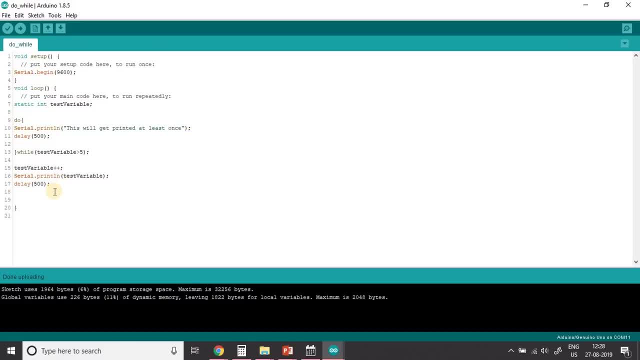 will increment okay, and then the value of test increment will print. then it will go back into do while loop and print this statement once again, because in do while loop it has to execute once at least. then while it will check the condition it is false, then it will come back here. it will. 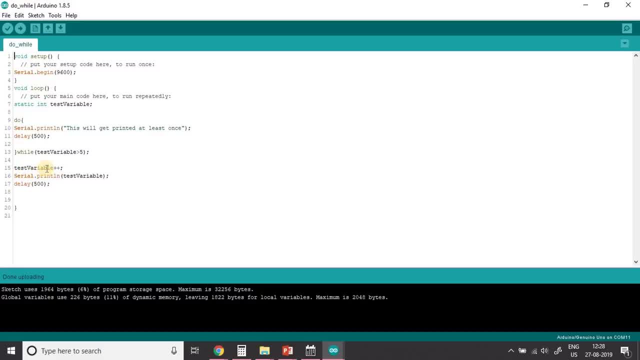 increment the variable and it will repeat till the test variable becomes greater than 5. okay, the moment it becomes greater than 5, so this do, while loop will keep on repeating. let's see how it happens. let us upload the code first. right, this will get printed at least once, and this is printing again and again. but now just see. 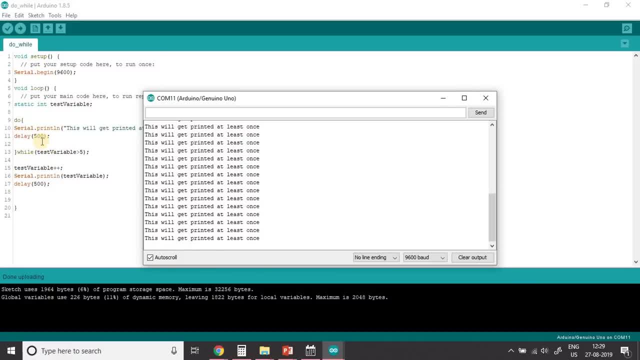 the loop control didn't come out of this. okay, because this condition is true. now it will go back again and execute the statement. these statements are not being executed because it is still in do while loop. so i hope you understood this do while loop. so now i have a really interesting 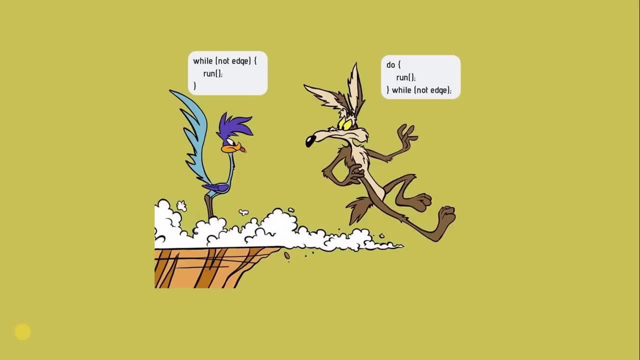 illustration which you can see on the screen to explain the difference between a while loop and a do while loop, and i think it is a really good example to show the difference between the two. every one of you must have seen the roadrunner show and we see this guy was using the while loop, while this guy was using the do. 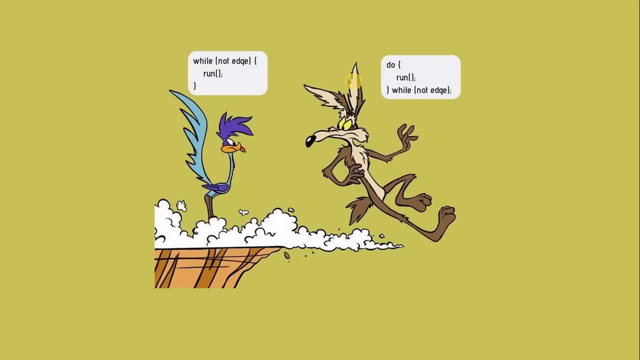 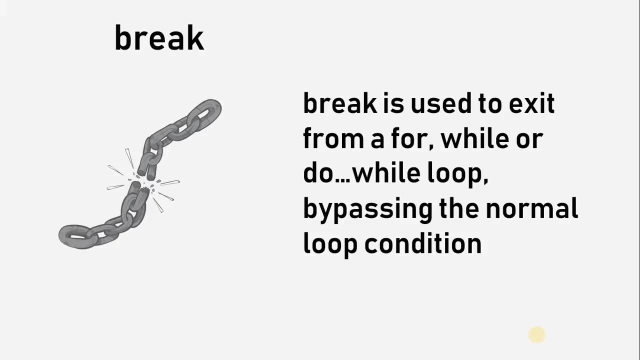 while loop. let's discuss in the comments who was using these control loops in a proper manner. if you remember, i told you that we might have to break out of the loops based on certain conditions, like, for example, in an endless loop. we might need to do something to stop that loop. so the break keyword. 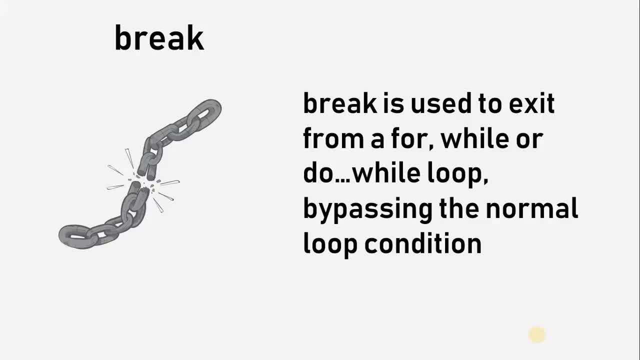 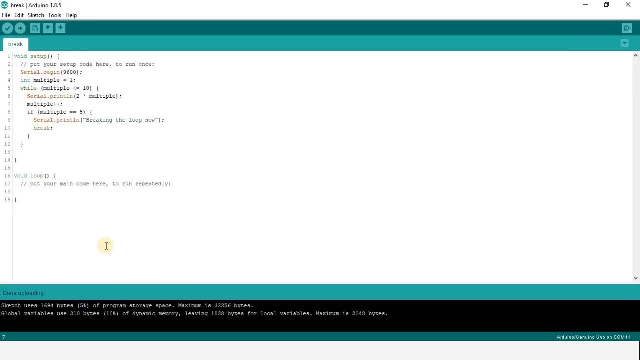 is used to exit from a loop by bypassing the normal loop condition which we have specified. let's see how we do that. so this is the modified version of the code which we use to print the table of two. okay, this is the regular while loop which is running. okay, we are printing a table of two. 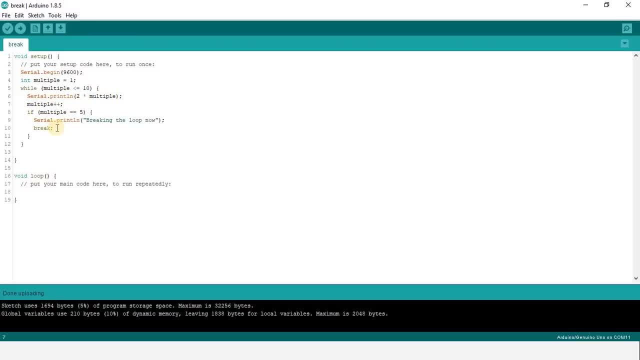 here and we are incrementing the multiple here. but now we have specified a break condition, okay, like if multiple is equal to five, then we will write breaking out of the loop now, and we will break out of the loop by just using this keyword. let's see what happens, right? so we printed it till. 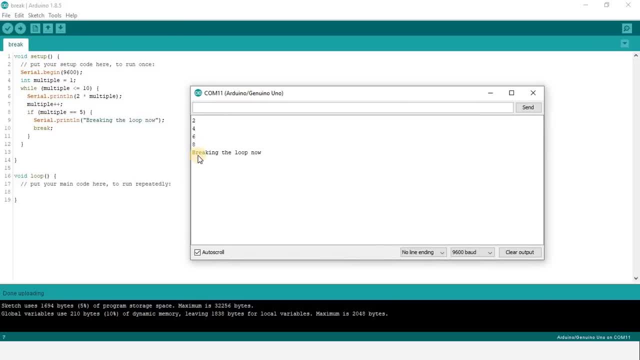 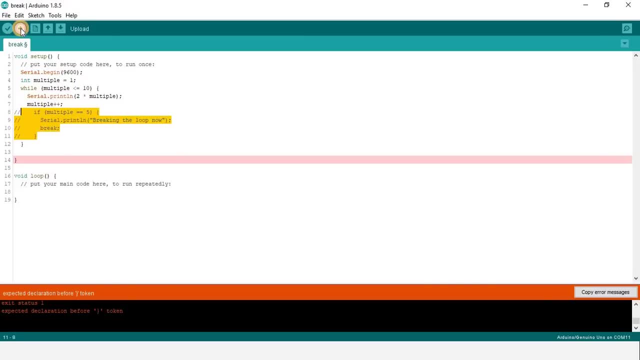 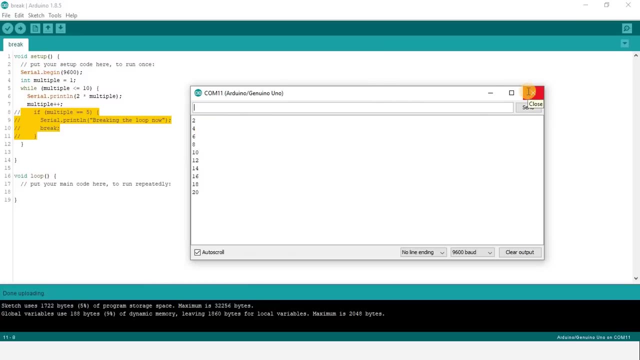 four, four, six and eight and then it braked out of loop. although it should have run till 10, it should have printed till 20.. so if i comment this break condition and upload the code again, so we got the entire table. so this is the basic use of breaking out of the loop. now let's see if 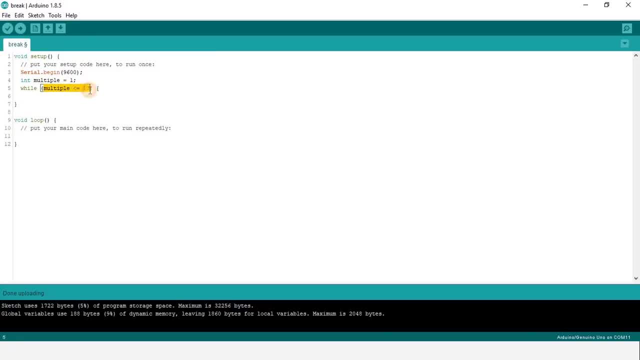 we are inside an endless loop. let's say, while true, this is an endless loop, we are writing serial dot print ln- endless loop, okay, and we will increment the multiple multiple plus plus. okay, let's say, i want to exit after printing it 10 times. if multiple greater than 10, we'll just break out of it. let's see what happens. 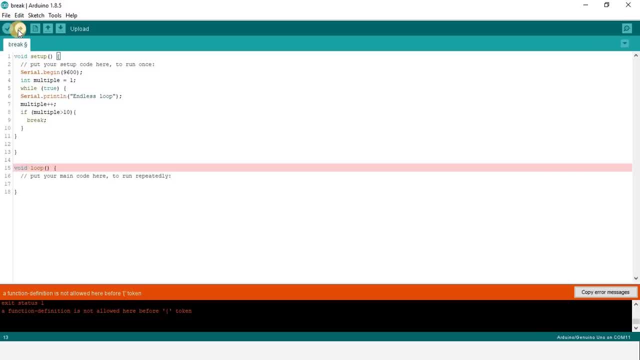 okay, we forgot to close the void setup bracket, right? if we didn't use this break statement, it would ultimately keep running endlessly. let's see that quickly. okay, can you see that it's printing endlessly, so i hope you understand. we use a break statement wherever we want to break out of the loop, so in the next video we will see the continue keyword. 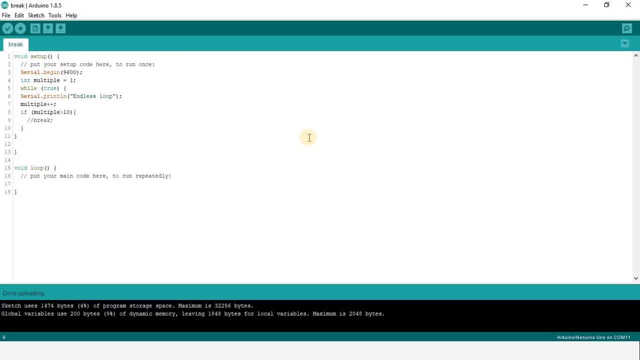 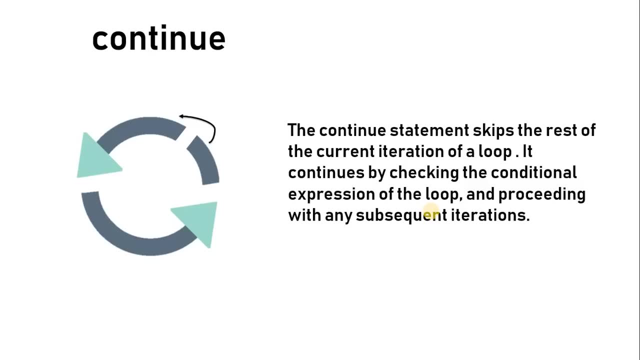 and we will also compare the break and continue keywords, like we saw in the break statement that whenever we use it, code control instantly moves out of the loop entirely, discarding all the remaining iterations of the loop right now. so if we look at the secondary, you see there are three. 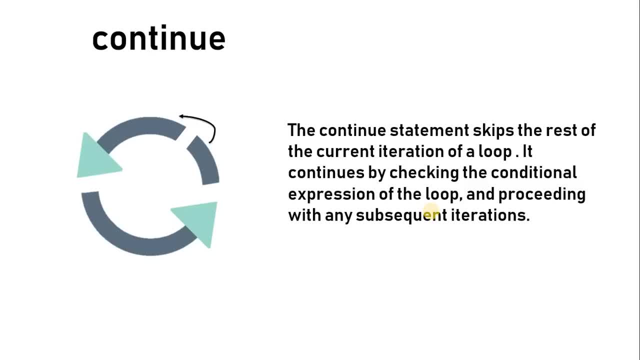 iterations of the loop, right like we were trying to print numbers from 1 to 10 and when we used: if our variable is equal to 5, then break out of the loop. so it entirely skipped 6, 7, 8, 9, 10, but in some 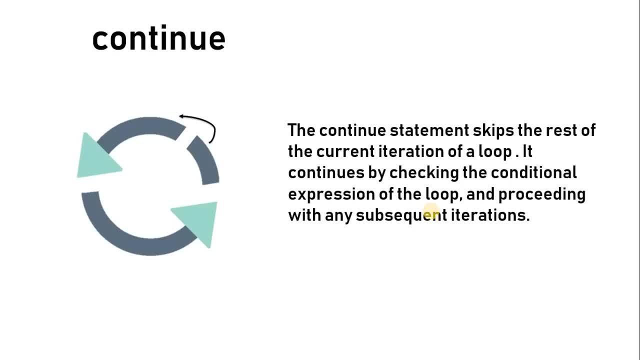 situations we might want to use the remaining iterations, right? so in that case the continue keyword helps us with that. the continue statement skips the rest of the current iteration of the loop and it continues by checking the conditional expression of the loop and proceeding with the subsequent iterations. that means it won't skip the rest of the iterations. let us see how it. 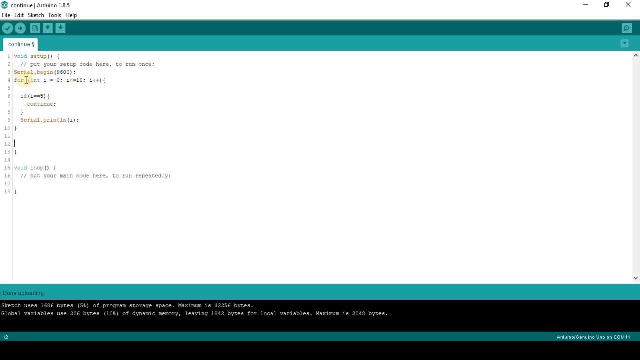 works. so we have void setup serial dot begin 9600, as usual. then we are writing for loop to print numbers from 0 to 10. right, because we have initialized i with 0 and we have used less than equal to sign. so that means both the ranges are inclusive. so it will print 0 to 10, and then we 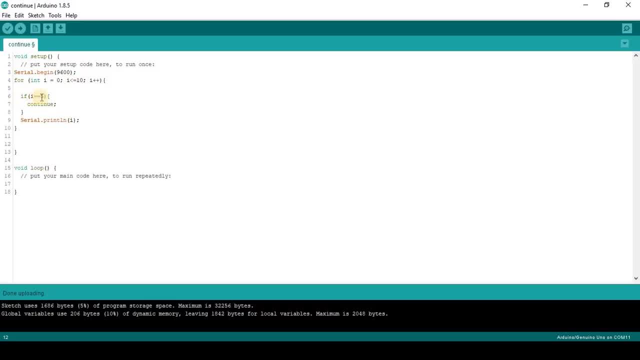 are incrementing the variable. now notice we have used: if i is equal to 5, then continue. whenever we use the continue keyword, it would straight away take us to the condition back and it would skip all the statements which are written after that. so let us see what happens. 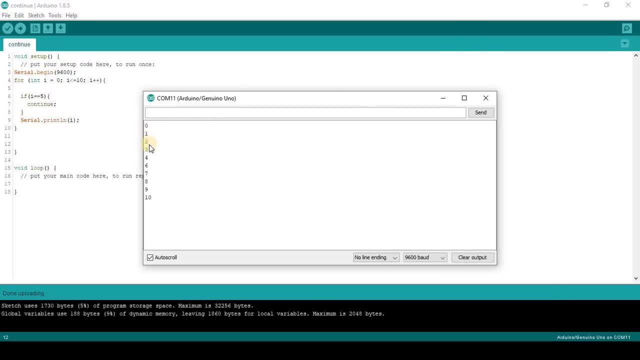 so we see 0, 1, 2, 3, 4, 5 is missing, then 6, 7, 8, 9 and 10. so it skipped the iteration in which i was equal to 5. right, but it did not skip the rest of the iteration if we had used the break keyword. 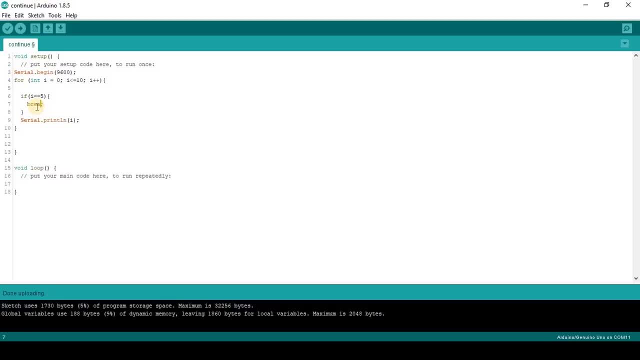 it would have skipped the rest of the iterations. it stopped at 4 only. let me switch back to continue here again. let me explain the difference between the break and continue statement. let us say we write a statement here: serial dot println. end of our for loop this. 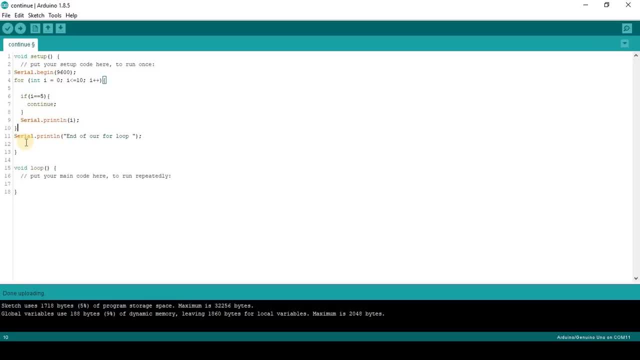 is the end of our for loop. that means after our for loop completes. this statement should print regardless of anything. so when we use continue, we will see the loop was going 0, 1, 2, 3, 4 and when the value became 5 it jumped back to check the condition. okay, so in this way it had. 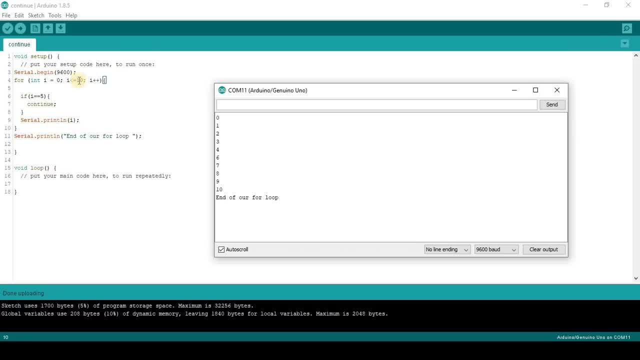 to skip this statement. it cannot execute this statement, right? so when it became 6 again, then it will start printing it again, can you see that? and after completing the loop, it came and printed this line. when we use break, then the control will directly come here whenever the break statement is encountered. 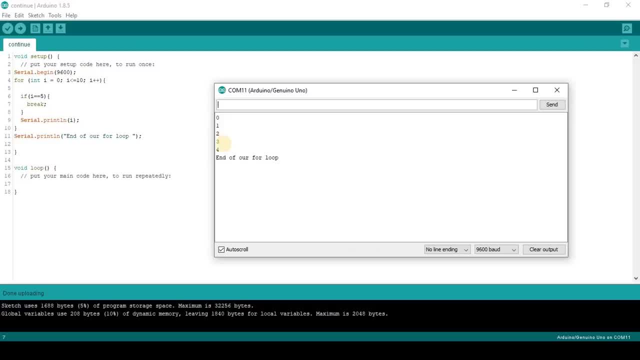 the code control goes directly out of the loop. can you see that after printing 4 it printed end of for loop. so we may have different situations to use continue and break statement and we have to make sure we use them correctly. so in the next video we will look at 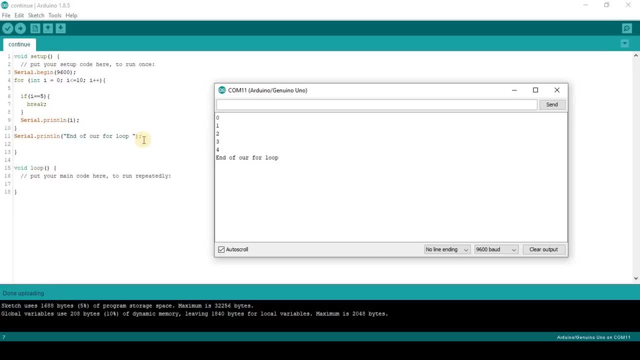 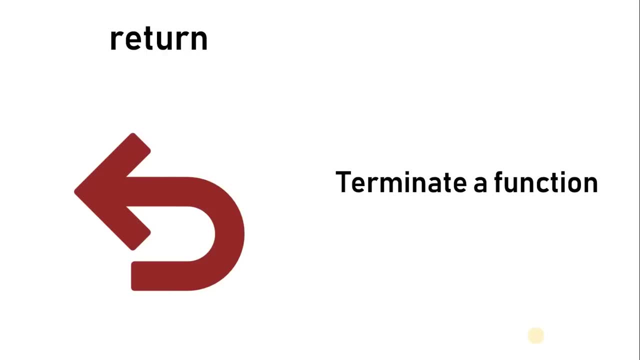 the last keyword, which is return. so see you in the next video. the return keyword. the return keyword would probably the easiest thing to learn. right now, the only function of the return keyword is to terminate the function, no matter what. it doesn't take any conditions. it doesn't take any. 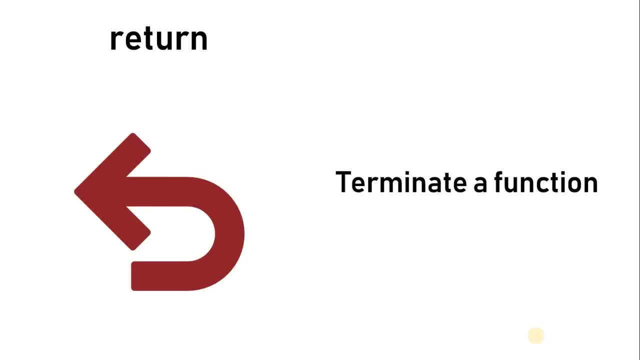 limitations or anything. whenever a code encounters the return keyword, it would just terminate the function. there are two ways to use a return. we will be covering the first way to use the return keyword. we will cover the second way in the coming videos. so let us see how to use a return. we will 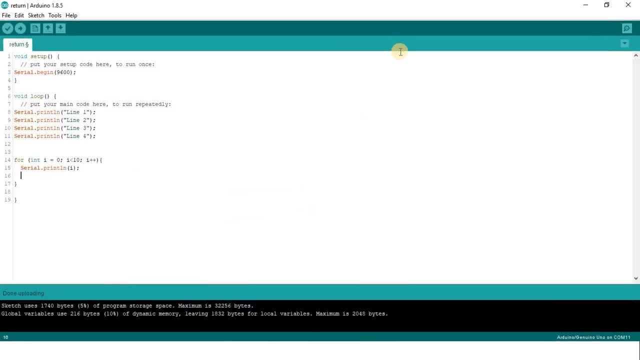 see how we use it in one manner. all right, so i have this code written here, okay, in the void loop. what i'm trying to do is i'm trying to print line one, line two, line three and line four, okay, and then i have a for loop which prints number from zero to nine. right, let's see if it. 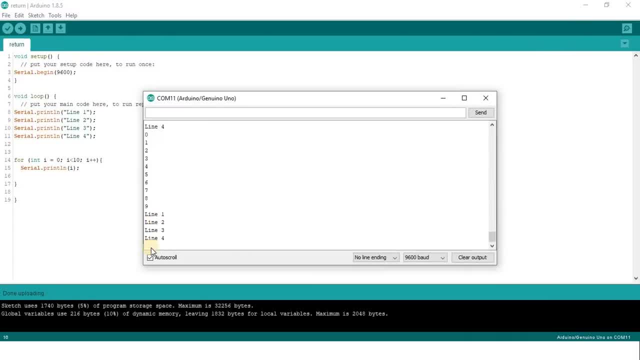 is working properly. yes, it is working as expected. line one, nine, two, nine, three, nine four and zero to nine: right. so now i want that. anything written beyond this point should not execute, so i'll just write return, so we'll see what happens. it will just print line one and line. 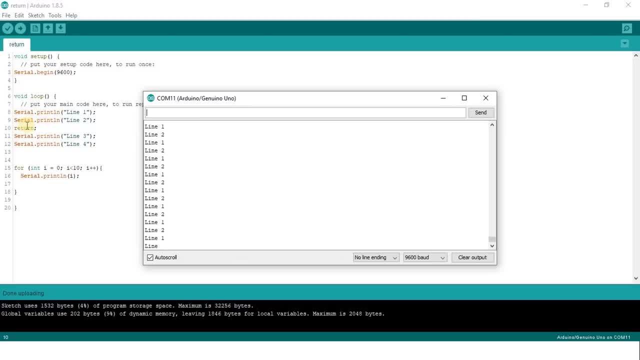 two, it will go back here and execute this lines only. anything written after return will not execute. okay, now you may want to remove it from here and use it here. right, let's see what happens. it will just print zero, because when the value of i was zero, it printed zero. then it encountered 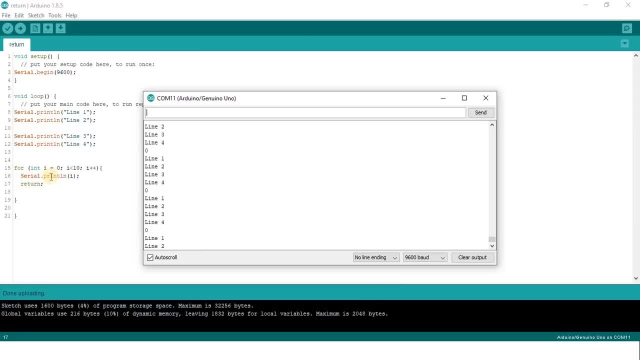 return, so it will just terminate this function. can you see that it is not printing one, two, three, four, five, six, seven, eight, nine, because return keyword just terminates the function. all right, so now i will see you in the next video. so the next topic in our course is switch case, like if statements. switch case controls the. 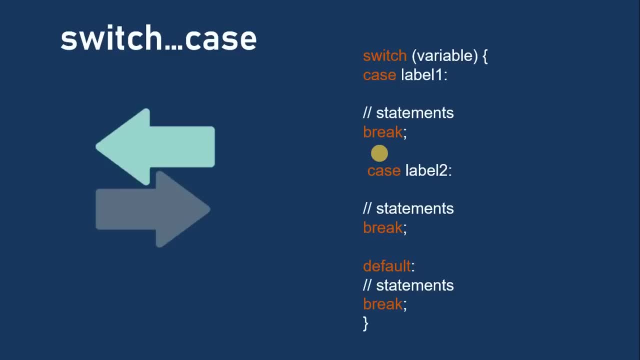 flow of programs by allowing us to specify different code that should be executed in various conditions. in particular, a switch statement compares the value of a variable to the value specified in the case statements. when a case statement is found whose value matches that of the variable, the value is not specified in the case statement. 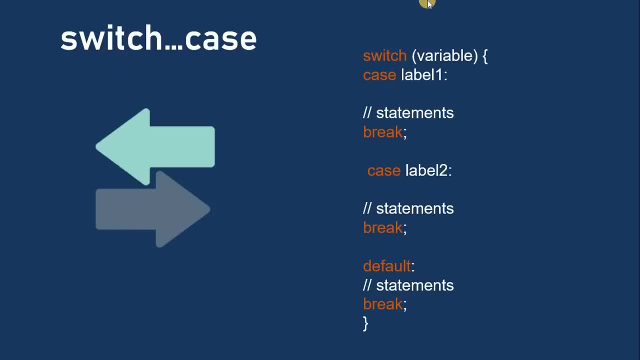 Then the code in that case statement is executed. So let us see the syntax of switch case. First of all we write switch, then an open bracket, Then we write the variable which has to be compared, Then we close the bracket, Then we start a curly bracket. 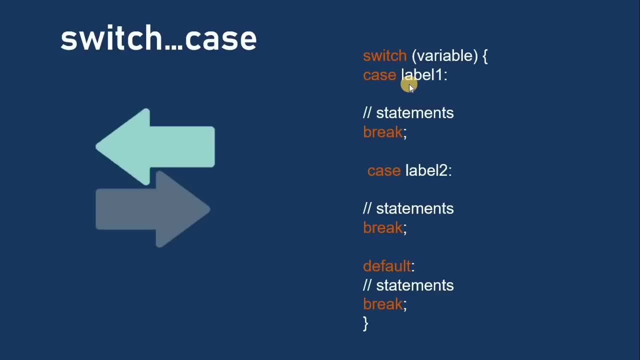 Then we write case space label 1, where label 1 is the number which has to be compared to the variable. Okay, then we write colon. Note that this is a colon not a semicolon. Okay, then we write the statements. 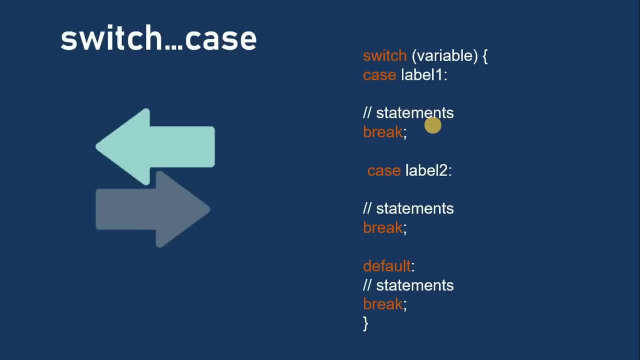 All the statements which we want to be executed. when label 1 is equal to the variable, We write those statements in this block. Then we write break semicolon. Then we write case, another label, then all the statements, Then we write break. 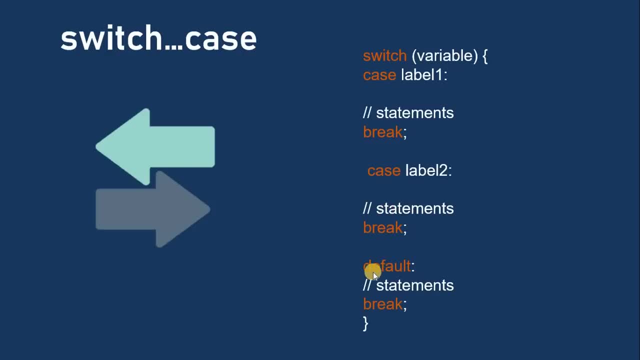 We can write as many labels we want in our code And the last statement which we write is default colon. all the statements break When none of the labels is true, then the default statement is executed. If we don't write default and none of the statement is true, then nothing will happen. 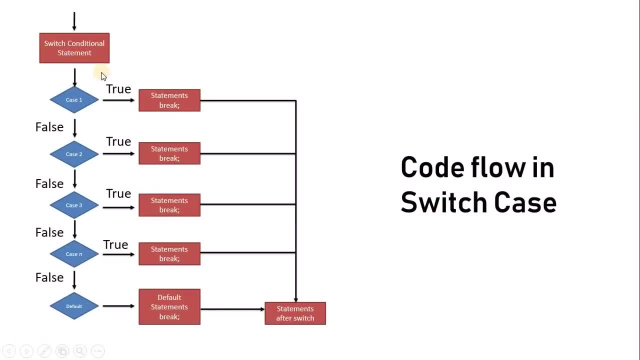 All, right, now let us see the flow of code in switch case. Here is a switch conditional statement. Then it will see case 1.. If it is true, it will execute the statements written in that block. If it is false, it will check case 2.. 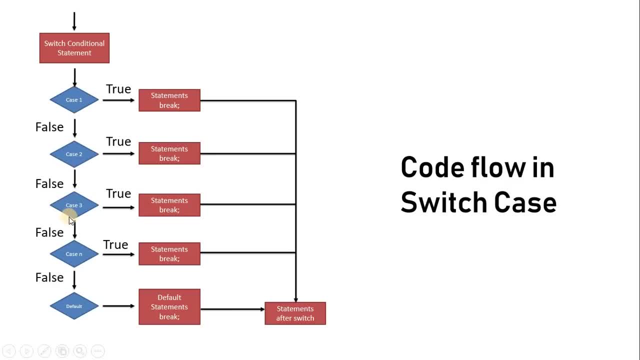 If it is true, then it will execute the statement. If it is false, it will go to case 3.. Okay and so on. If none of these are true, it will automatically jump to default and it will execute the default statements. 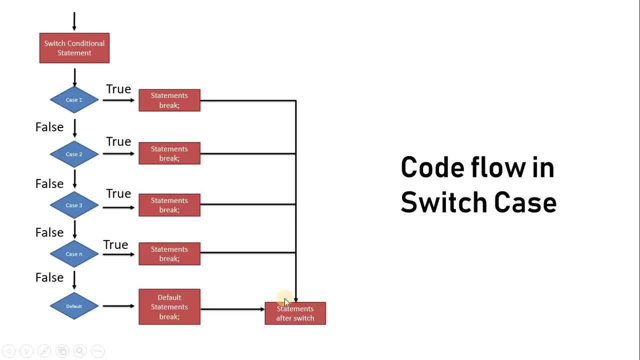 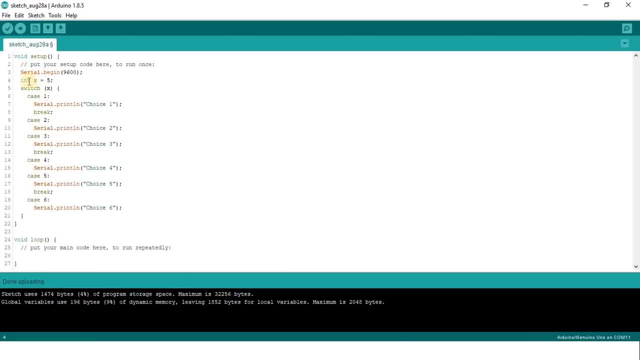 And after executing one of these statements, the flow will go on to the statement which is written after the switch. Let's see in the coding Right In the void setup we have written serialbegin as usual. Then I'm writing int, int. 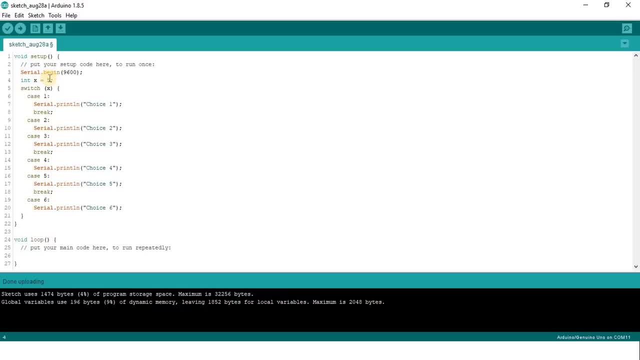 X is equal to 5.. Here X is the variable which we want to be compared. Okay, then I'm writing switch, then X, here, because I want X to be compared. Then I'm writing case 1, colon, serialprintln, choice 1, break. 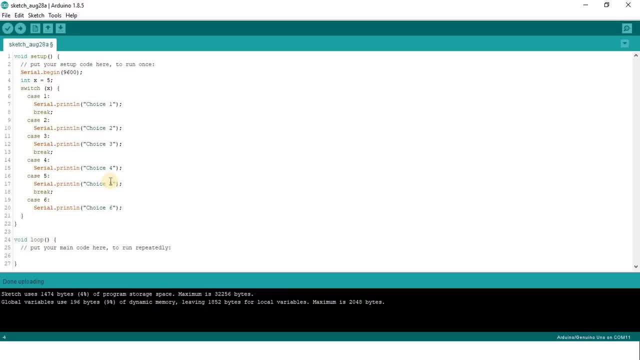 Similarly. I've written six cases. Now can you guess what statement will be printed here? Since X is equal to 5, my guess is: choice 5 should be printed, because it is not equal to 1.. It is not equal to 2.. 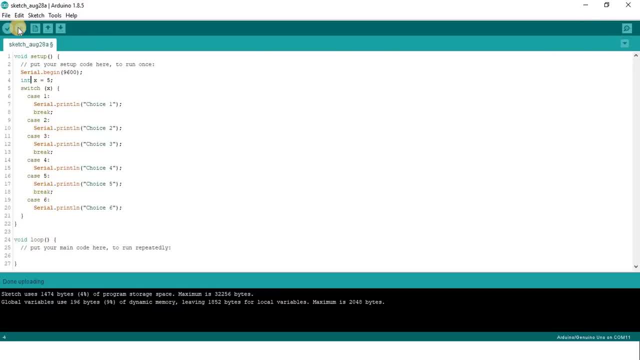 It is not equal to 3, and so on. Okay, so let us see what happens Right Now if I change the value of X to, let's say, 1, so now choice 1 will be printed, Right. 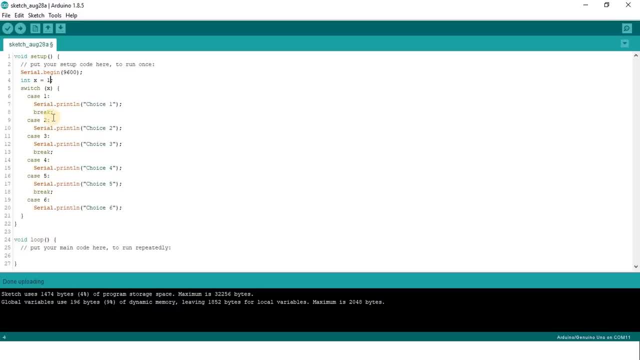 Now in case if we don't write break here? the purpose of writing break here is that we want to exit as soon as one condition becomes true. Let's say, if we don't write break here, so it will continue to execute the statements, since X is equal to 1.. 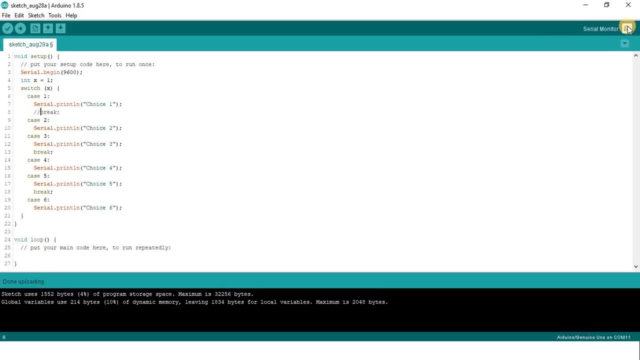 So now it should print choice 1, choice 2 and choice 3.. Okay, Because there's another break after choice 3.. Right, Choice 1, choice 2, choice 3.. That is the purpose of break. Now let us see one more example without break. 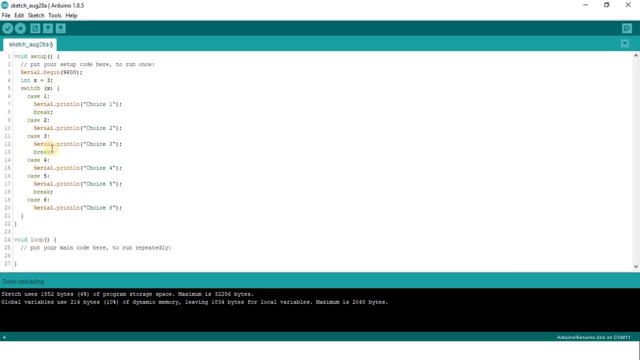 Let me use: X is equal to 3. Then it will start from here. We'll not use break here. It should print choice 3, choice 4 and choice 5.. Right, As expected. Now the important thing which you need to notice is the variable which we use here and the labels which we use. 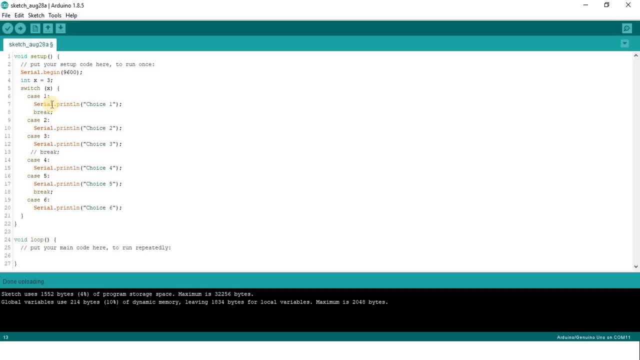 Here should be of int or character type. if you use float or if you use another array type, it will just throw an error. This switch case is a really handy tool if you want to write a lot of if-else statements. Instead of that, you can just write case 1, case 2, case 3.. 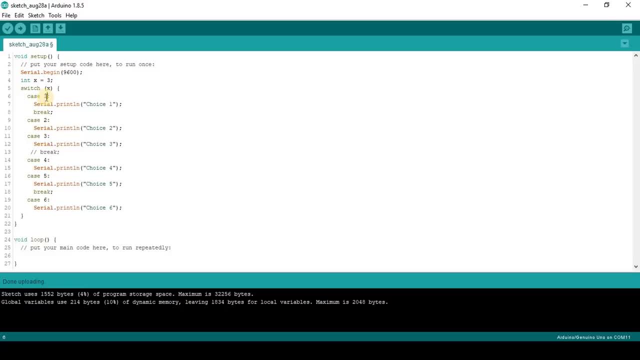 You can also specify ranges in case statements and how we do that. Let's say, we want to take a range of 1 to 10.. We'll write 1,. we'll write 3 dots and then 10.. Okay, Then let's say 11 space. 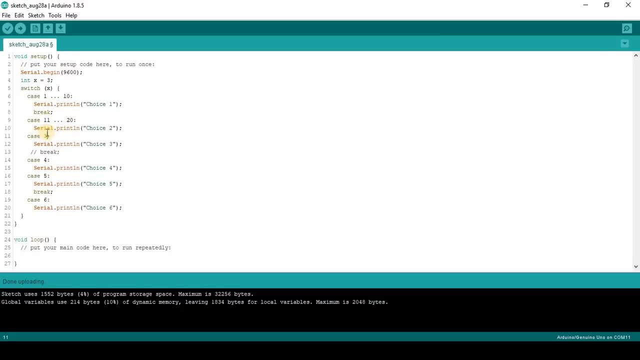 2, 20.. Okay, Let's say 21,, 3 dots to 30. Then we write 31 space. You have to write a space there. Okay, If you don't write a space, you will get an error. 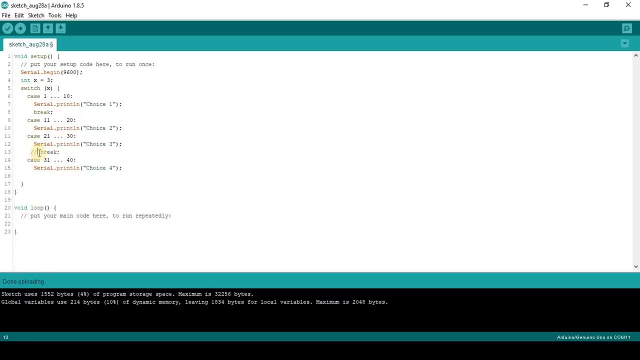 So let's see these cases. only Let me write break again. Okay, So now let us see 3. What will happen? It will write choice 1.. Right Now, for example, if I take 35, it should write choice 1.. 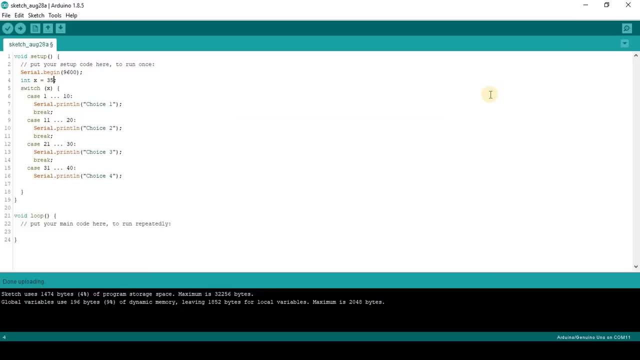 So it will write choice 2.. So it will write choice 3. Right. So I guess you got an idea how easy it is Right. Instead of writing if-else, we can use switch case. So I hope you understood this topic. 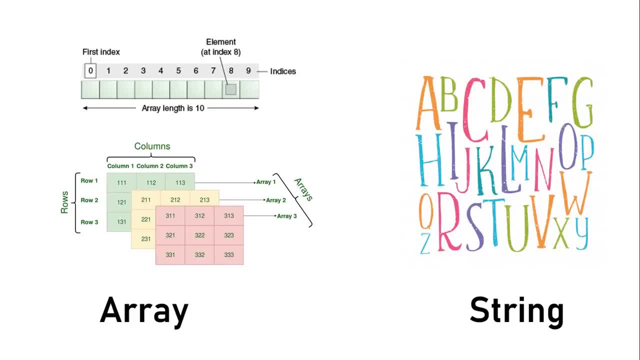 So I'll see you in the next video. So at this point we are in a position to study about the two remaining data types, which are arrays and strings. These two data types are also very commonly used in the projects which are made using Arduino. So in this video, I'm going to show you how to use these two data types. So in this video, I'm going to show you how to use these two data types. So in this video, we will look at arrays. 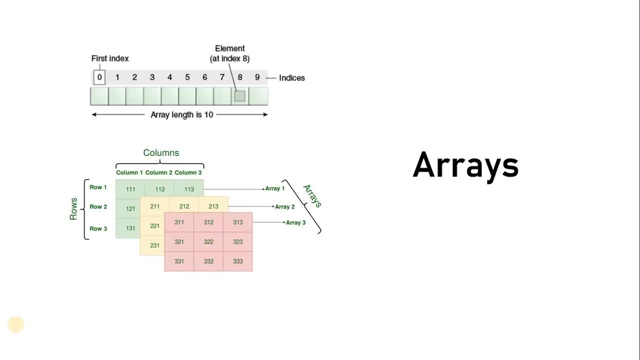 An array is a variable which can store multiple values of same type. Let's say we have a compartment of a defined size which has multiple containers in it like this, And those containers can store same kind of information. So let's see this by an example. 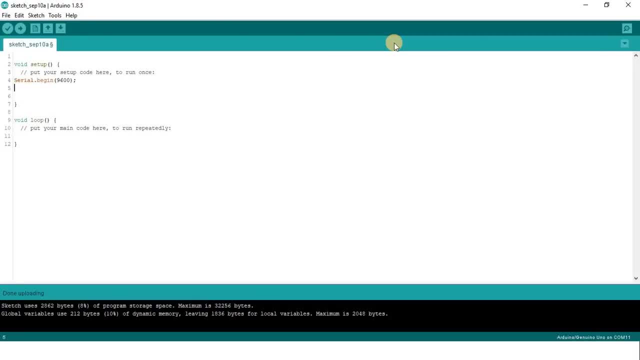 To declare an array, we first write the type of data which we are going to store in it, Let's say int. Then we write the name of that array, Let's say myArray, Okay. And then we write a square bracket. 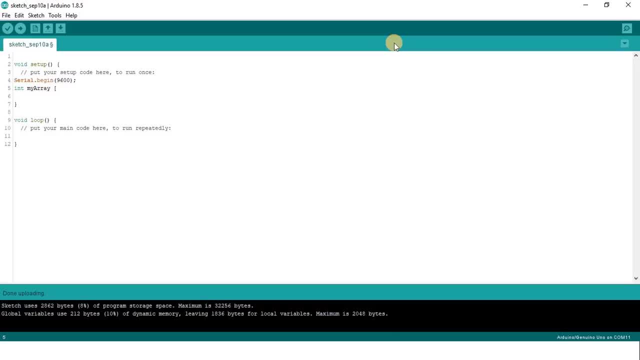 And we write a number inside it. That number denotes the size of that array. Okay, Let's say 5.. So when we write this, the compiler will create a space in memory where you can store those 5 integers. Okay, 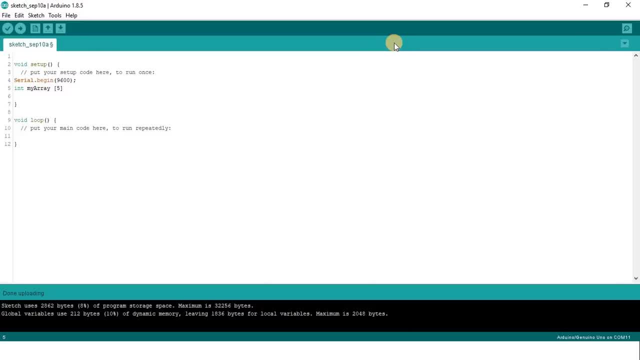 Now let's store some values in this array. To do that, we write equal to, Then we write curly bracket And then we will write 5 values which we want to store in it. Let's say 1,, 2,, 3,, 4, and 5.. 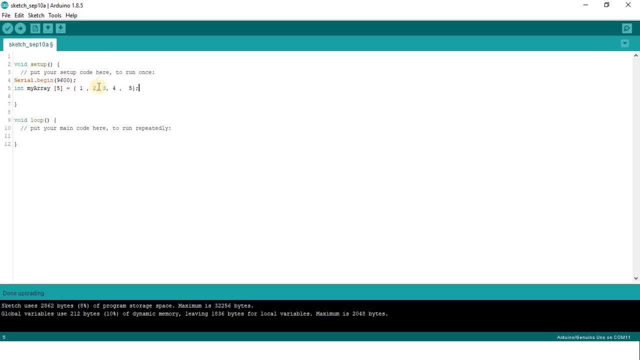 Semicolon- Semicolon. Each value is separated using A comma, And each value inside an array is known as element of array. Okay, And each element has an address of its own. That address is known as an array index. 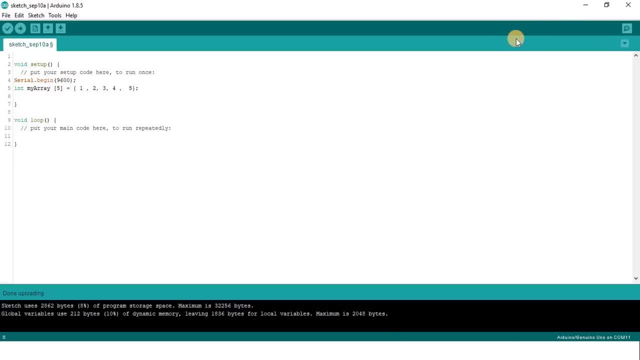 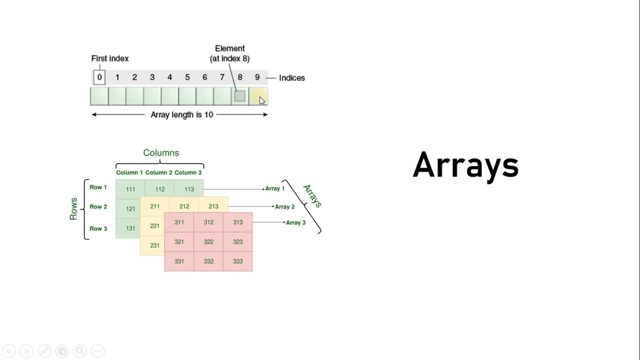 That index starts from 0.. Okay, Let me show that to you again. Let's say we have an array of size 10.. So 0 is the first index and 9 is the last index. Okay, And the value which is present at that index is known as element. 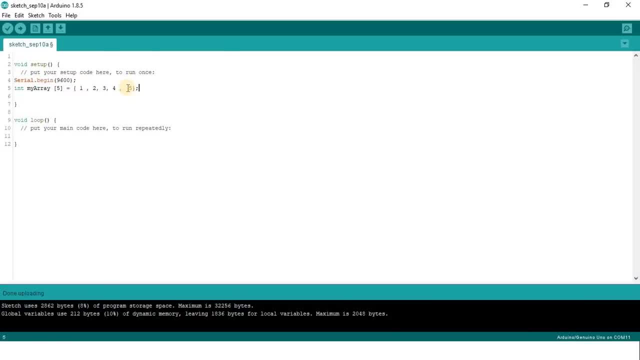 Let's see that again in coding. So this is the first index, This is the 0th element and this is the 4th element. Okay, Now let's try to access them. How do we access them? Serial dot println- my array. 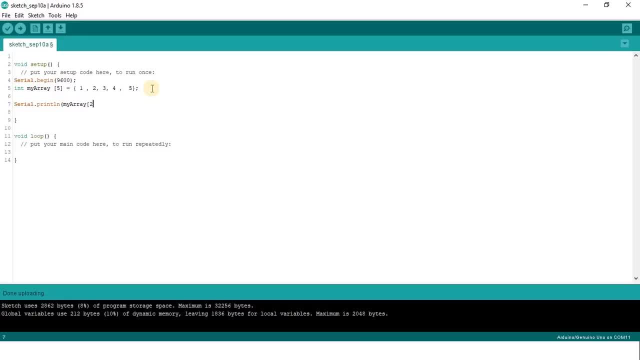 And then the value which we want to use, Let's say 2.. Can you guess what will be printed here? Tell me 0,, 1, and 2.. So 3 should be printed. So 3 has been printed here. 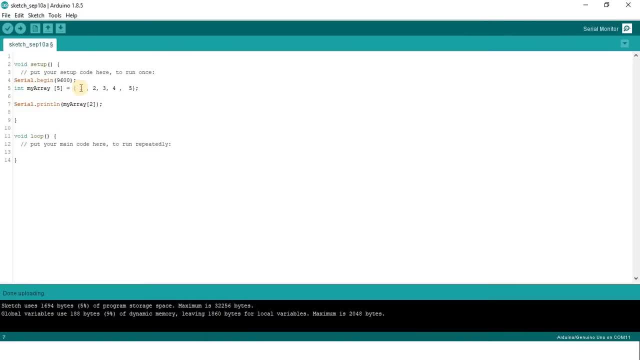 For the first time users. it must be really convenient. It's really confusing that why it was started from 0. It is very simple: because computer counts from 0. While humans are in a habit of counting from 1, that's why we are finding it a little confusing. 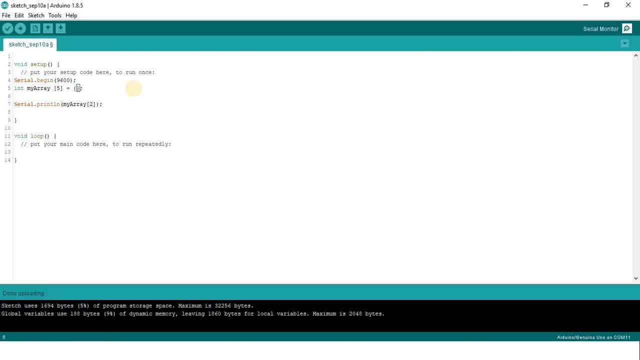 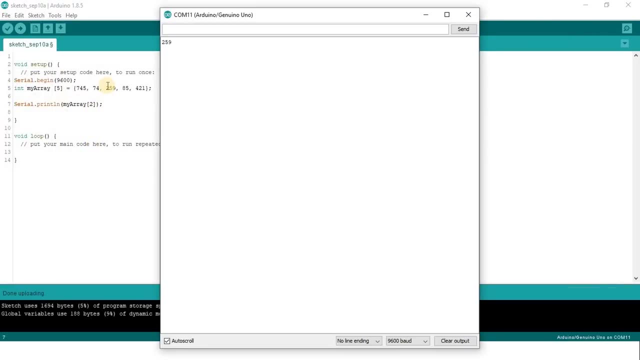 Now let's change the values which are present inside this. We'll take bigger and complicated values. Let's say 745, 74,, 259,, 85, and 421.. These are the random values which I have chosen. Now, if we try to print the second element, it will print 259.. 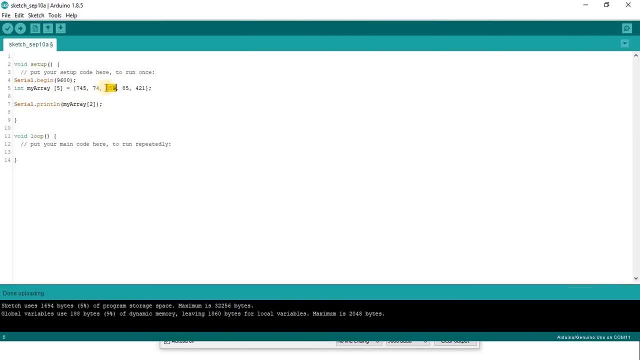 Because 259 is the first element. So 259 is present at second index, while 0 is this one, 1st is this one, 2nd is this one, 3rd is this one and 4th is this one. 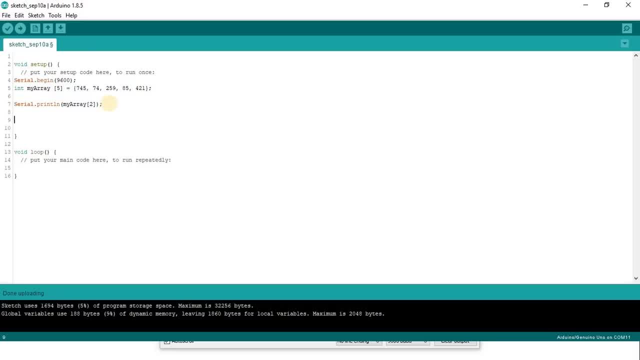 Now we can alter these elements as well directly. Now let's say I want to change the value which is present at second index. So we will write: my array 2 is equal to, let's say, 706.. Now the value of 259 will be replaced by 706.. 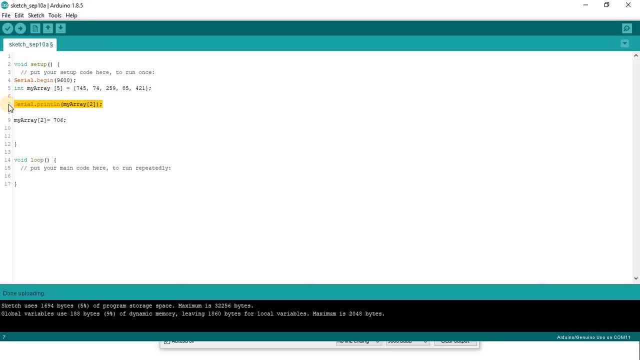 Let's see, Let's print that again. Now it should be printing 706.. Right, We can alter any value. for that matter, We can do our regular calculations on array elements as well. Let's say, I have one variable int, myVariable. 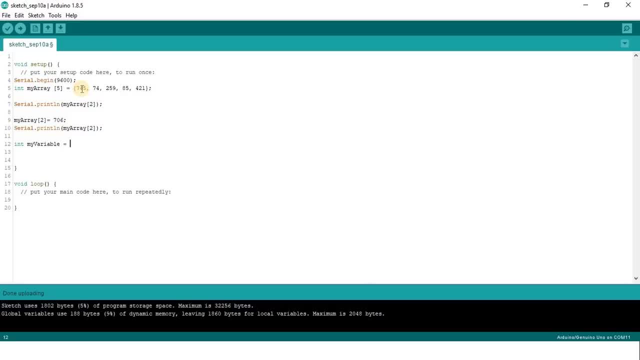 Now let's say I want to add some elements and store that value in myVariable. I will write myArray 0 plus myArray 0.. Now let's say I want to add some elements and store that value in myVariable. 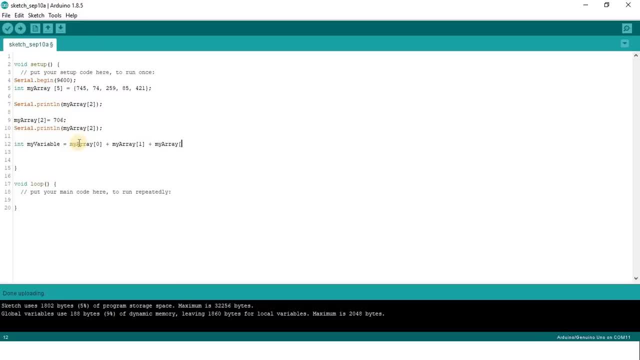 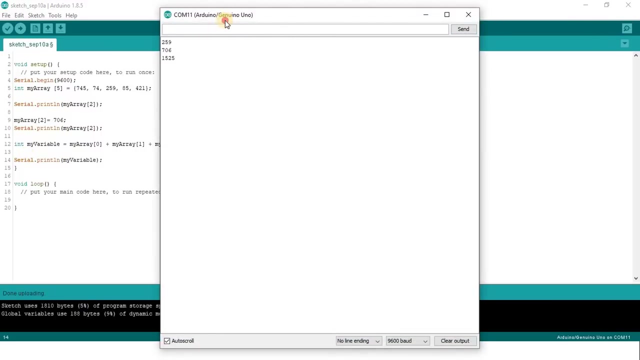 1 plus myArray2.. So now myVariable will be holding the sum of 745, 74 and 249.. Not 249, 706, because we have altered it here. So let's try and print myVariable. You can check on your calculators if the answer is correct or not. 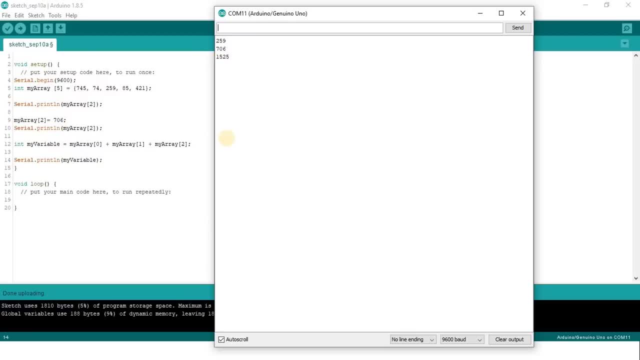 So the sum of 745, 74 and 706 is 15.. So let's check 15, 25.. 15, 25.. Okay, Similarly we can also do multiplication, subtraction, division, etc. 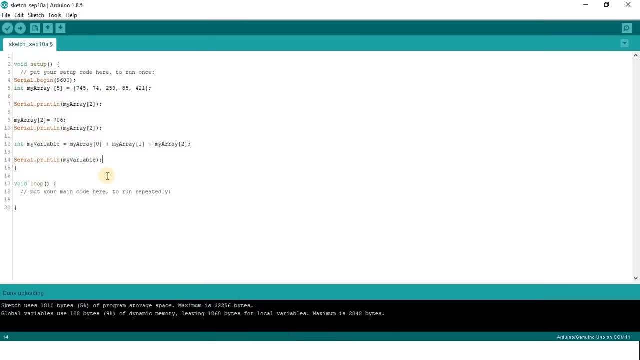 All the operators can be used here. Okay, Now we can also use elements of these arrays in for loops as well. Now let's use a for loop to print all the elements inside my array. So how will we do that? For int i is equal to 0,, i less than 5, because size of my array is 5, then i plus plus. 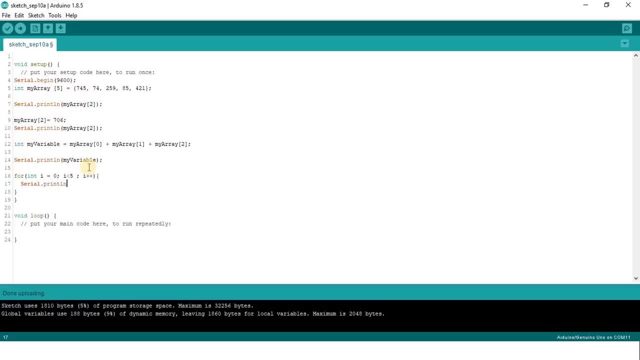 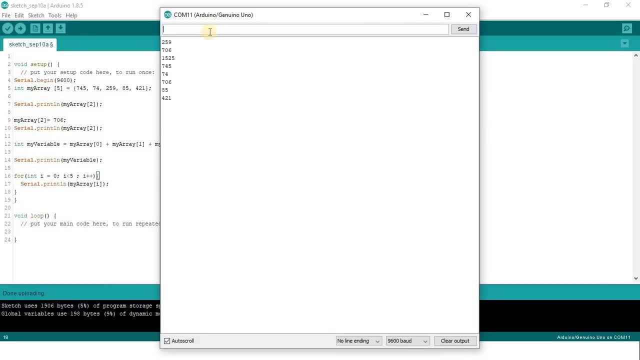 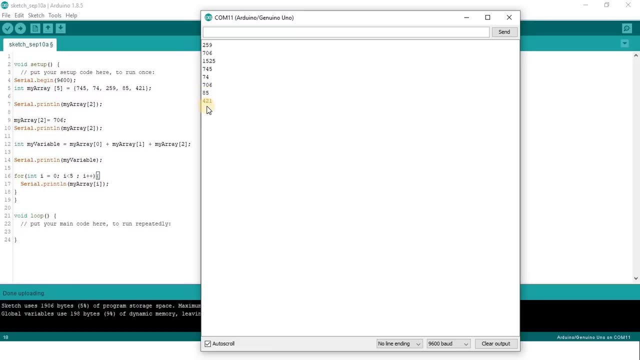 Okay, So now what will we do is serialprintln my array. then i: Okay, So it should print all the elements which are present inside this array. So it is here: 745, 74,, 706,, 85, and 421.. Right, You can compare them here: 745, 74, 706, because we updated the value here. 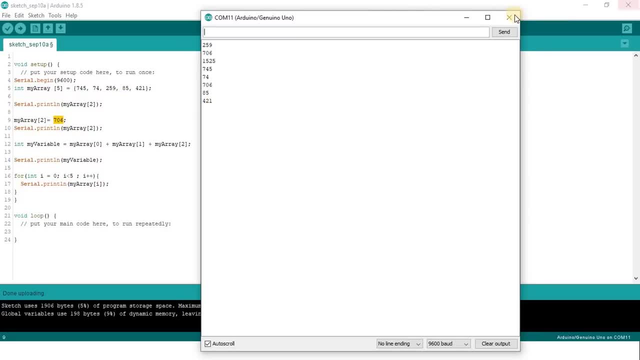 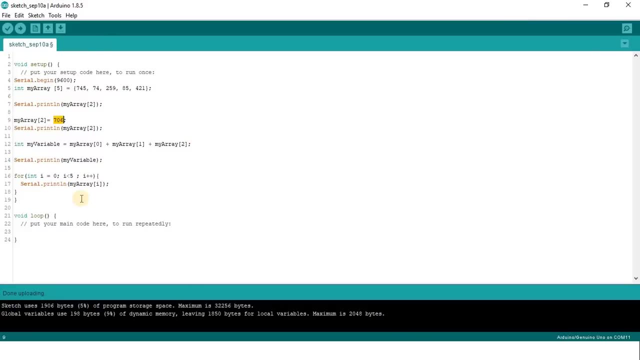 Then we have 85,, then we have 421.. Okay, Now can you tell me what will we do if we want to add 5 to all the elements of my array? Okay, So now let's say we will write for. 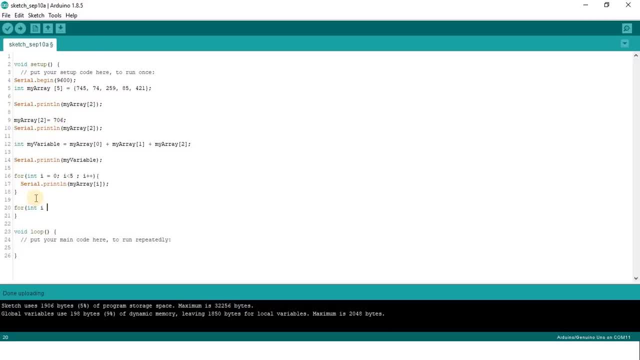 int. i is equal to 0, i less than 5, then i plus plus will take my array. i is equal to my array, i right, plus 5.. So now 5 will be added to all these elements. So now 5 has been added. So now let's print this: 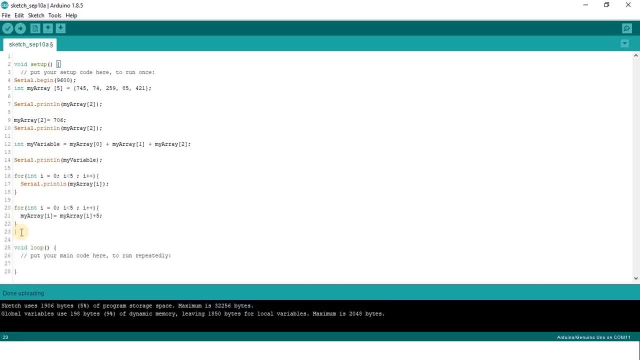 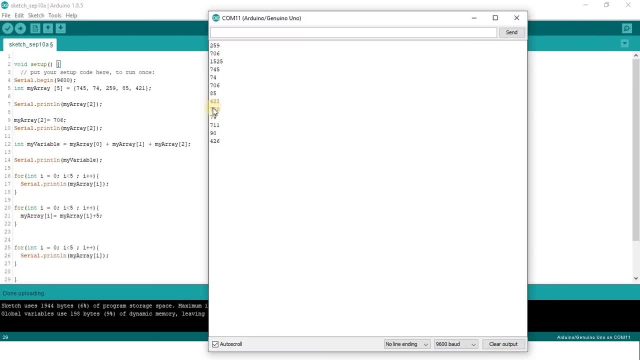 again If we print this again. So now we will see 5 has been added to all the elements. Let's see, We are here. It is printing from here Right: 745 plus 5 is 750.. 74 plus 5 is 79.. Then 706 plus 5 is 711.. 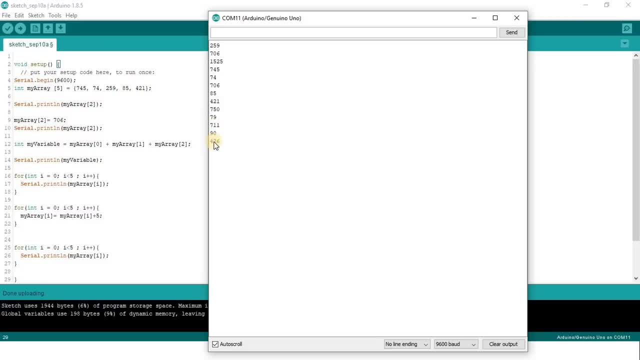 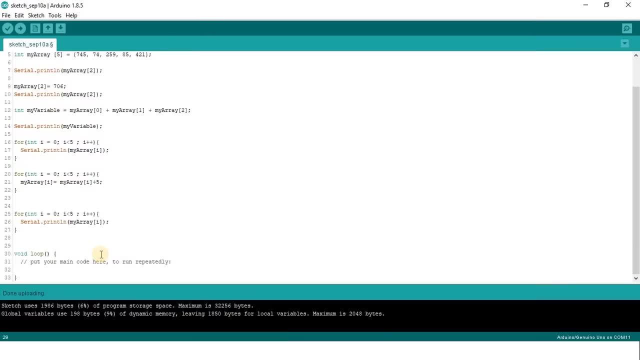 85 plus 5 is 90.. 421 plus 5 is 426.. Okay, This way we have added 5 to all the elements. Now we can take sum of all the elements in the array as well. How will we do that? Let's say int sum is equal to 0.. We have initialized it by 0.. And for int i is equal to 0.. 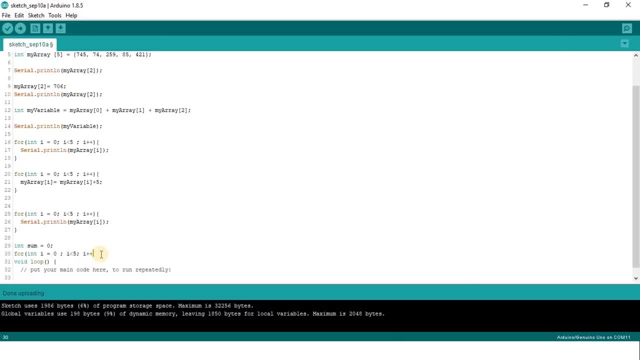 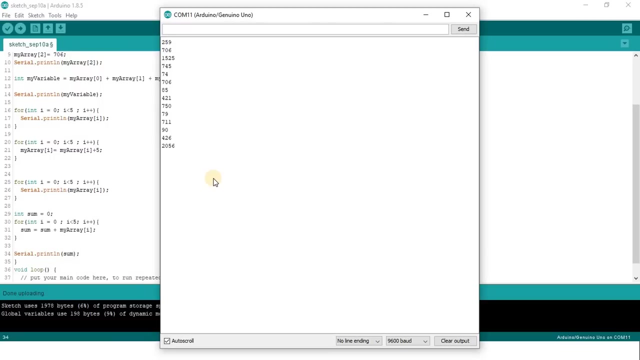 i less than five, then i plus plus. okay, what will be right is: sum is equal to sum plus my array. i, okay, and after that we'll just print sum, right? it is printing 2056, so you can check on your calculators if these values are summing up to 2056, but just make sure you don't add these. 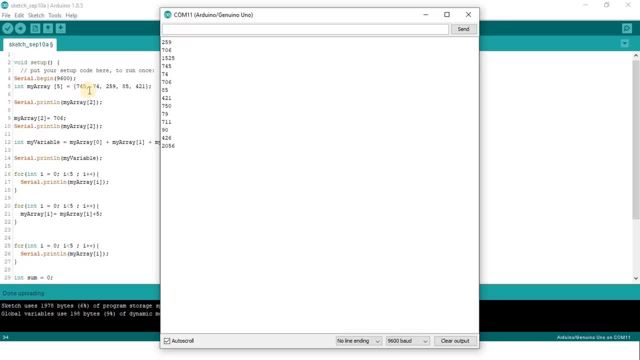 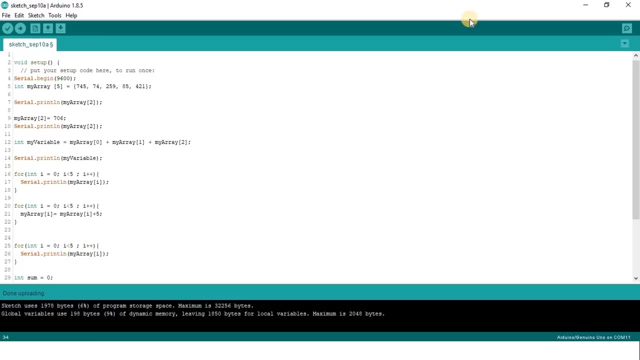 values. you add the new values. the new value was 750, 79, 711, 90 and 426. these were the new values. these, okay, if you add these values, you will get 2056. so now we have learned about how to use arrays, how to access the values in an array and how to manipulate those values. what we saw till. 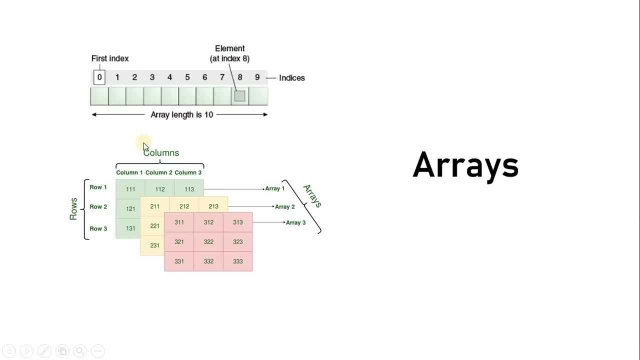 now in this video were one-dimensional arrays. that means they just have one dimension. now there can be multi-dimensional arrays as well, like two-dimensional arrays, three-dimensional arrays. like you can see here, This pink box is a two-dimensional array. It has rows as well. it has columns as well. okay, 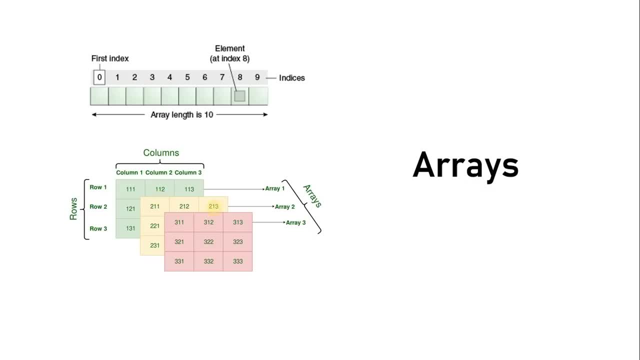 And then we have three-dimensional arrays as well. Like: it has depth as well, it has rows, it has columns and it has depth as well. Multiple two-dimensional arrays, make three-dimensional arrays. I'll just give you one use case where two-dimensional arrays are used. 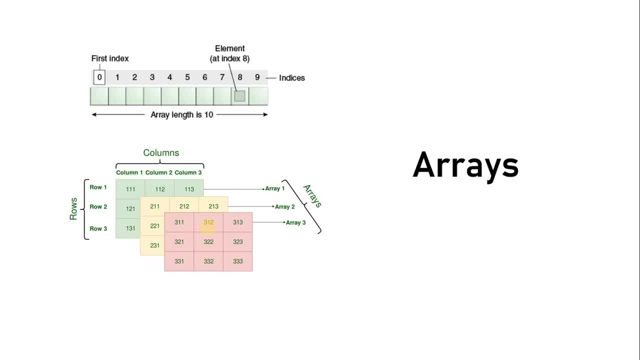 For example, we want to store the pixel data image, pixel data of a black and white image. okay, So we use two-dimensional arrays And let's say we have to store pixel image: pixel data of a colored image which also has RGB values. 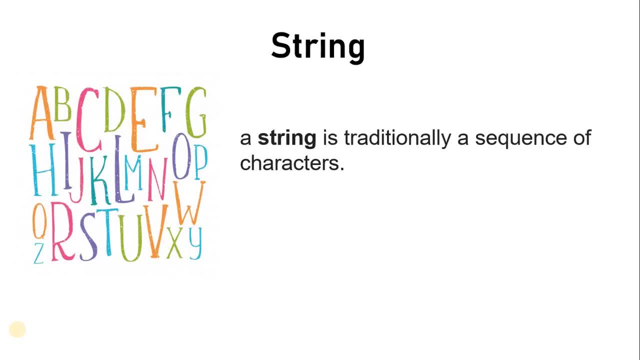 So we use a three-dimensional array for that. In this video we will talk about strings. Strings are basically a sequence of characters. Whatever we write, Or you can say, whatever messages which we write in our code are all strings. Let us see in the code: 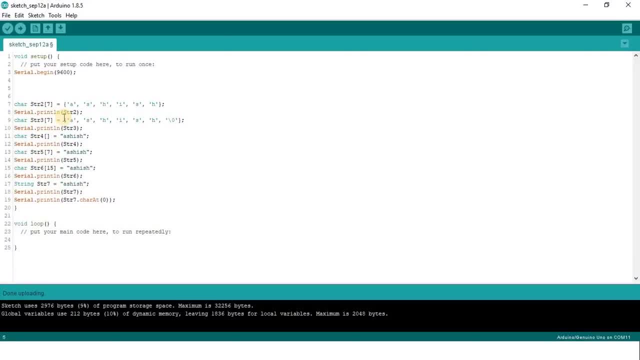 The easiest way to spot strings is that you will find them written inside double quotes, For example, serialprintln. this is my string. okay, This is my string is a message which is going to be printed on the serial monitor, But in itself, this is my string is a string, okay. 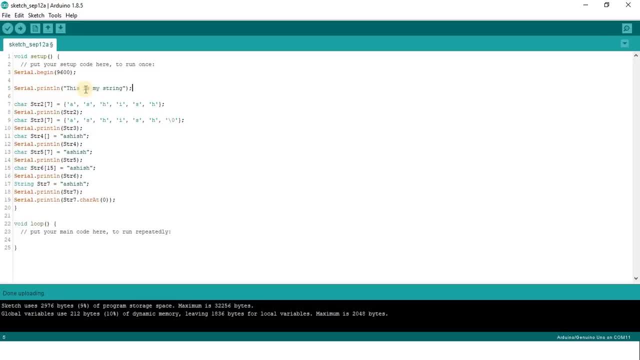 Now, technically speaking, a string is nothing but an array of characters, And as we have already studied arrays, it would be really easy for you to understand. So now to declare a string, we write char in the name of the string which we want. 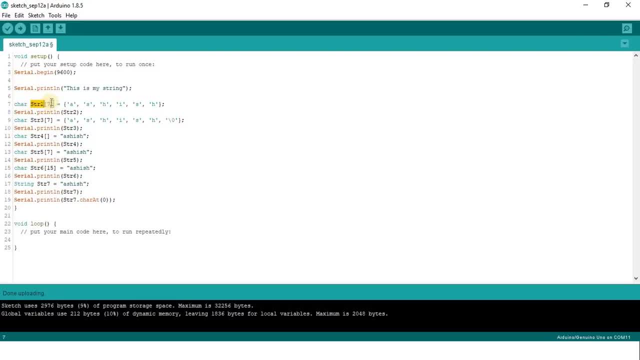 For example, I have written str2.. Then, as we start an array by a square bracket and a number inside it, we similarly write it for string as well. For example, I want to write ashish, which has A-S-H-I-S-H as characters in it. 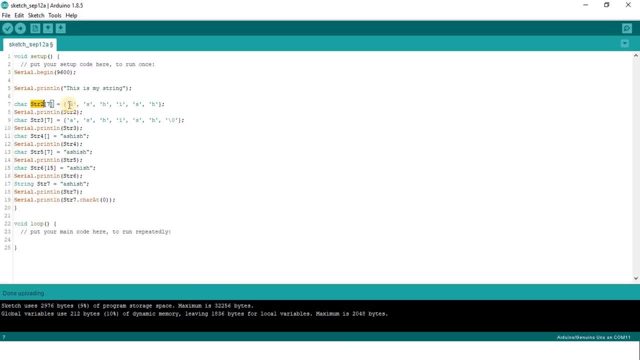 Okay, And the number of characters in ashish are six. Okay, So what we will do is we will always take one additional number to declare our string, because an ending to the string is denoted by a special character, which is known as a null character. 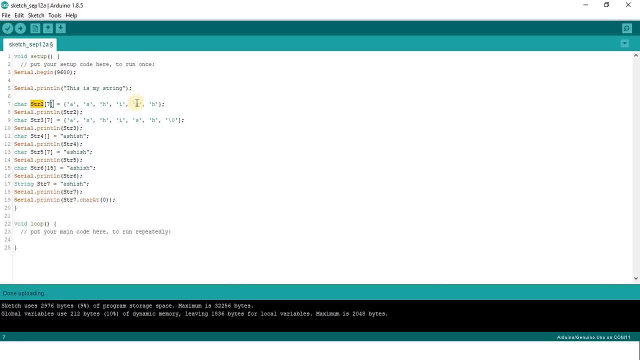 Okay, The compiler automatically takes that into consideration when you write a string or when you declare a character array. Okay, In this case, compiler will see: okay, the person is trying to declare a character array which has these characters, So it will automatically add a null character at the end. 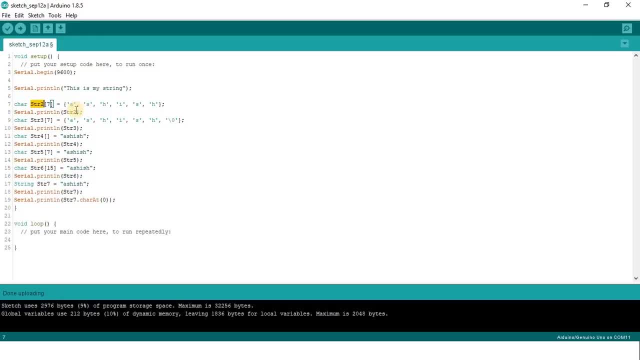 So now, when we print this line, it will print ashish. Okay, Another way is to declare that null character explicitly. For example, I will write char str3,, then seven is equal to ashish and then a null character. This is the null character, which is denoted by a backslash and a zero. 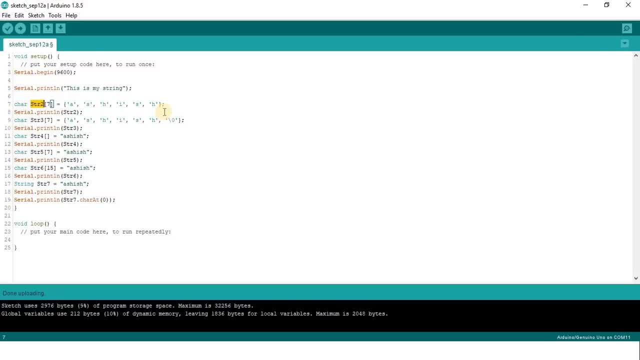 This way, the compiler identifies that. okay, this string has come to an end. Okay, So it can differentiate between one or more strings. Without this character, there will be problems. The compiler may think that another string which is coming after this string is a part. 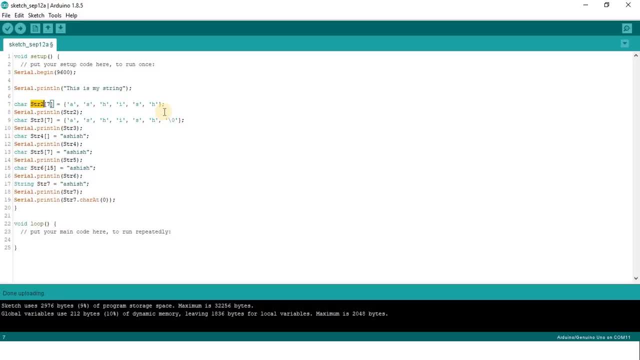 of that same string. There has to be some way to differentiate between different sentences. Okay, So that's why we use a null character which is backslash zero. Another way to declare a string is we write char str4,, which is the name of the string. 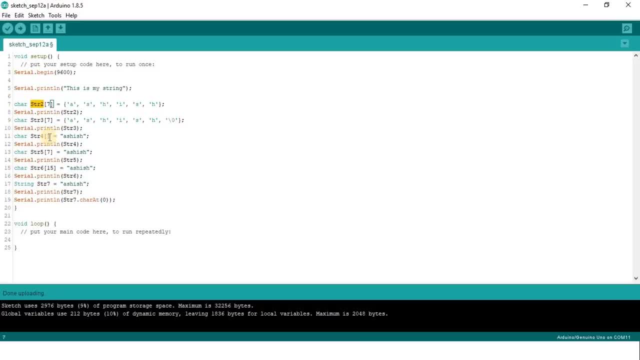 And then we write square brackets without a number inside it. The compiler is smart enough to dynamically allot a number to this. It will see, okay, the user has written a string which has ASH ISH inside that It will automatically allot a memory of seven to this string, because ashish has six characters. 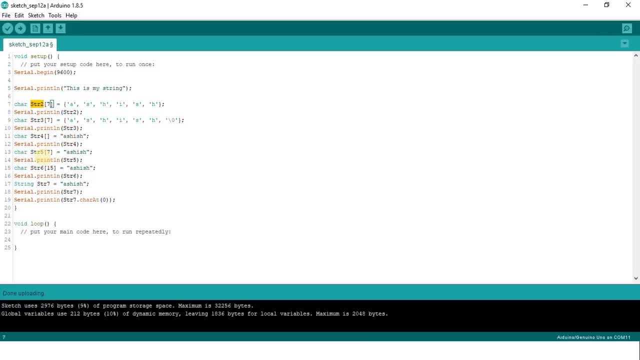 in it and including a null character, it will become seven. Okay, We can also write it like this: str5, seven ashish, simply in double quotes. We don't have to work this much. It is also okay if you take a larger memory for a smaller string, but it is not okay to. 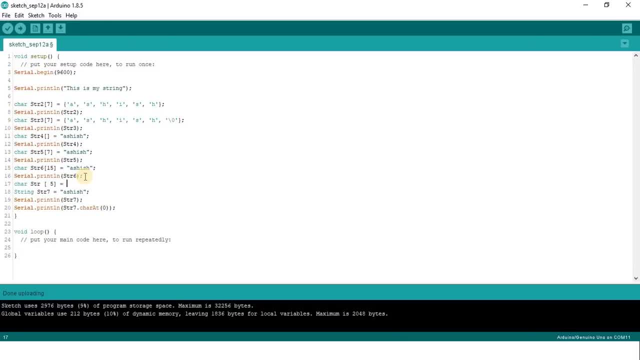 take a smaller size string, Let's say five for a longer. Okay, Now you will see it will only print five characters. And then there is another way. we will talk about it shortly, but right now let me comment this out. Okay, 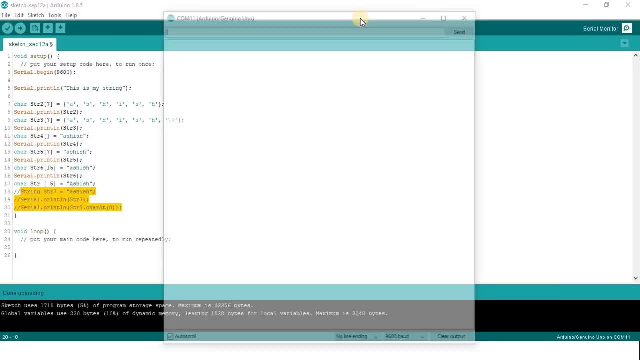 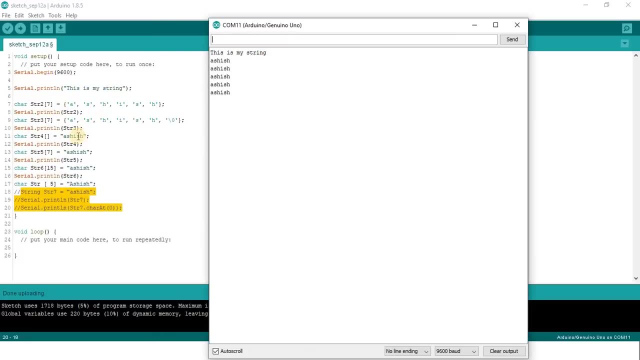 We'll just upload this code and we will see what we are getting. All right, this is my string. Then it wrote ashish for this, ashish for this, ashish and ashish for this again, And it printed it till here. 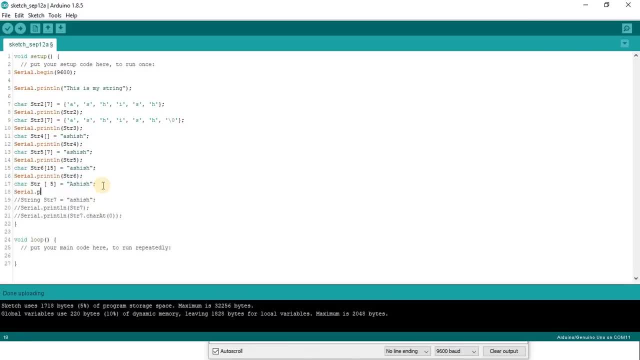 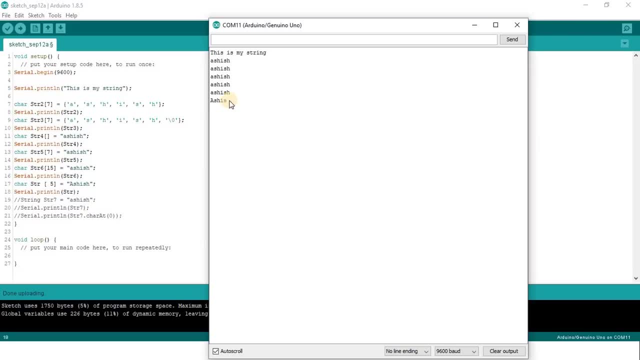 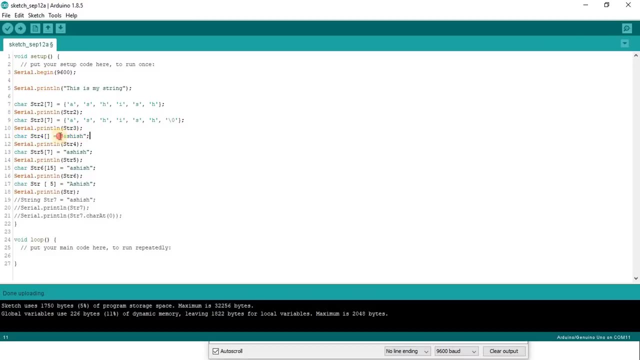 Okay, So we got to write serial dot println for str, right, It just skipped the last character because we didn't give necessary memory to it. So according to me, this is the best way to start writing strings, because obviously you do not know how many characters your string will contain. 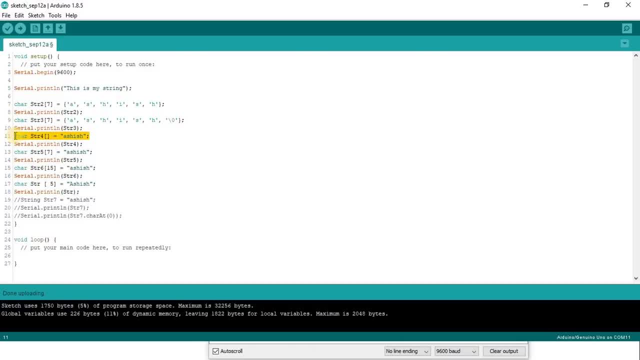 And obviously you don't want to spend that time to count those characters right. The compiler is smart enough to calculate the size for you. Okay, So there is another way to write a string, which is by using a string class. Okay, 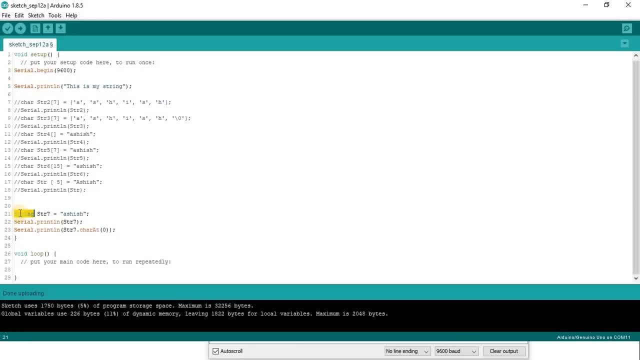 Here. let me just comment this out: This is a string class. We are calling a string class and we have named str7 inside it And we have just written whatever we want inside that. Let's say ashish, And when we print this, it will straight away print this. 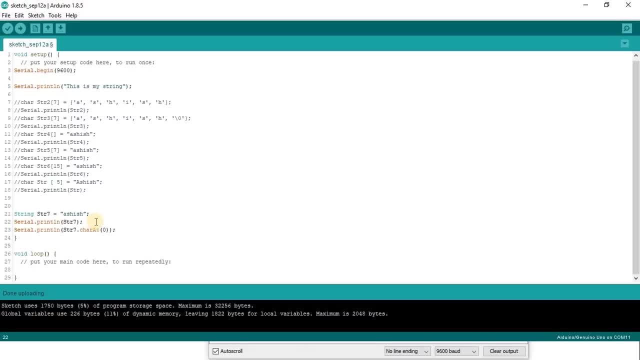 Okay, What's the benefit of using a class is that it is a built-in class, First of all, and it has a lot of functions inside it, And those functions can be like: we can compare a string. Okay, Easily, We're just writing string: nameequals. 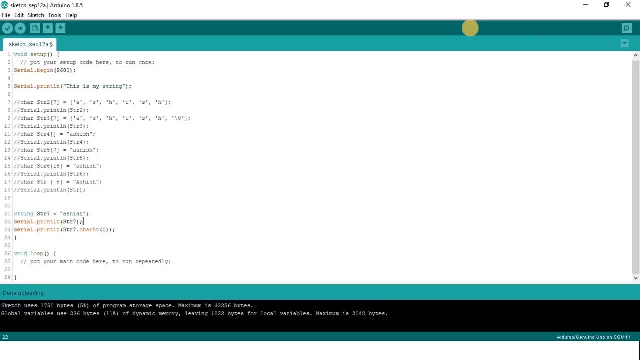 If it is equals, it will turn true. And similarly, there are many more built-in functions inside the string class. For example, I can tell you we can print a character at a particular sequence. For example, I wrote str and then serial dot, println, str, char at zero. 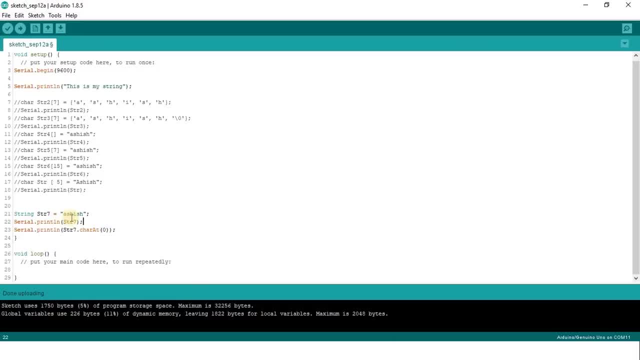 So it will print a because at zero position, a is present. Okay, Similarly, there are many more functions like or starting with, ending with, and there's a function like we can convert the entire string which is written in lowercase to uppercase. 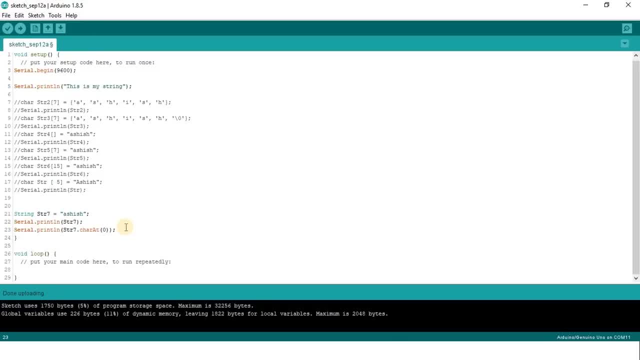 and vice versa: Uppercase to lowercase. Okay, We can convert integers into string. We can convert strings into integers. Okay, So you may be needing all these functions while we perform our experiments. Strings are used to contain information messages or error messages or any logs. 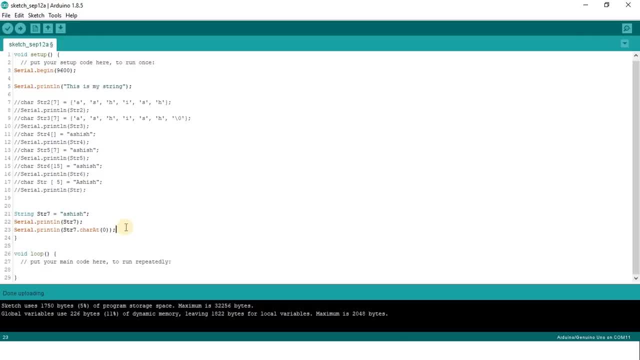 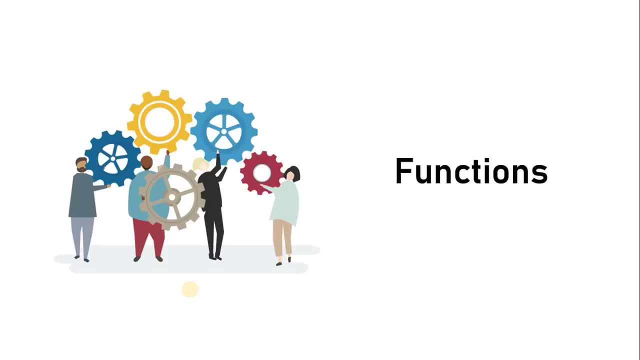 Okay, We can store them inside strings And we can also display strings on our serial monitor, on the LCD display or any kind of display. Okay, We will now understand what are functions. A function is a set of statements that take inputs and do some specific computation, and 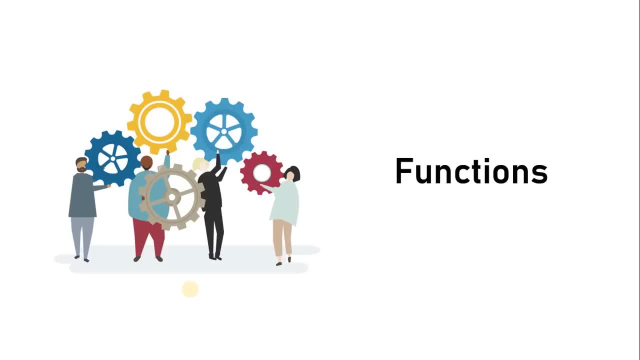 produces some output. The idea is to put some commonly or repeatedly done tasks together and make a function so that, instead of writing the same code again and again for different inputs, we can call the function. We'll understand what I just said as we progress in the video. 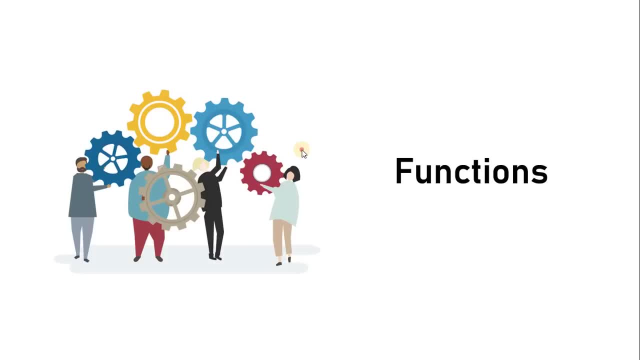 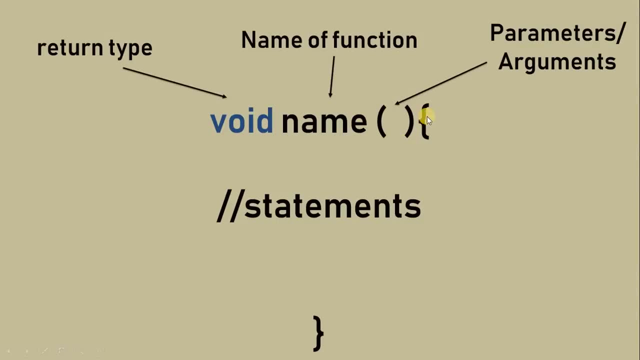 So, before anything else, let us first understand how to identify a function In the code. whenever we see something like this, like void name, and then there are brackets, then there is a curly bracket, then there are some statements written and then there. 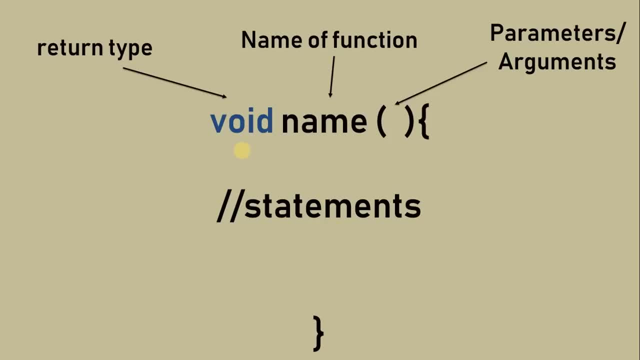 is a curly bracket. again. This is the basic structure of a function. okay, where void is the return type, That means we start writing a function by telling the compiler the return type of that function. where void means that function will not return anything. 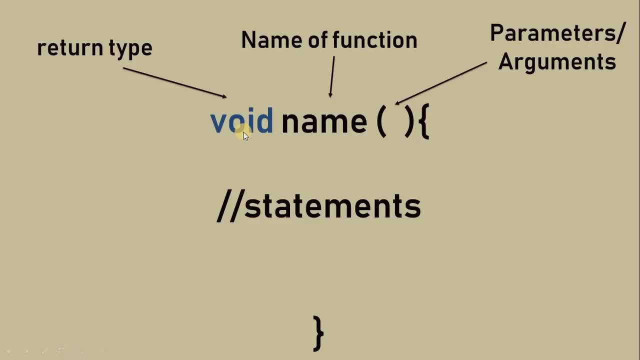 Now, instead of void here we can use int, boolean or float or anything for that matter. whatever we want to return from the function, Then we write the name of the function. We can name it whatever we want, Like we saw digitalWrite or pinMode. they were the functions. 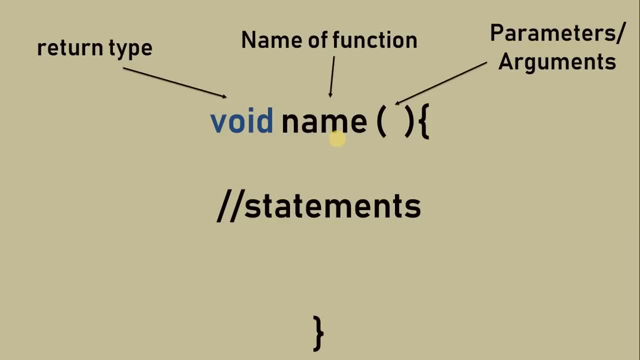 And the name of that function was pinMode and digitalWrite, And then in the bracket we write parameters, or some people call them arguments. If there are no parameters or arguments to the function, we just keep this bracket empty. Or if there are parameters, then we specify those parameters. 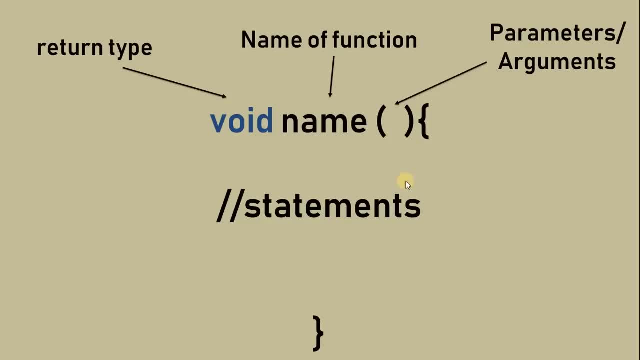 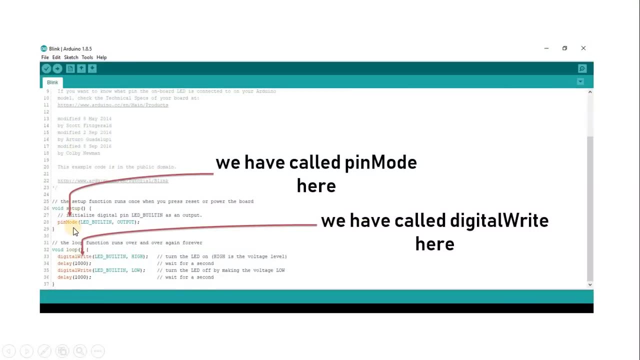 How do we specify the parameters? We will see in the next video. okay, So I'll just basically tell you how do we call a function. Now, like this: in the blink example, we called pinMode function. To call a function, we write the name of the function along with the parameters of that. 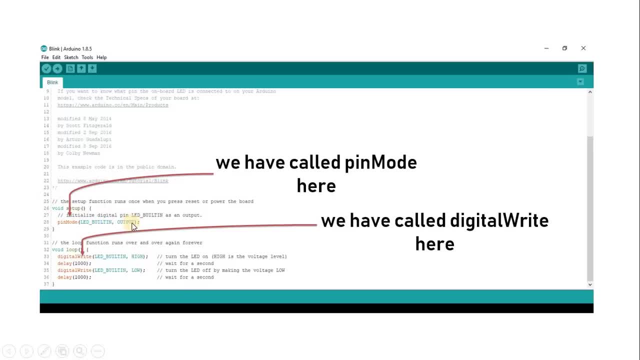 function In pinMode ledBuiltIn output was the parameter of this function Right? Similarly we have called digitalWrite here And the parameters of that digitalWrite was ledBuiltIn comma high. These were the two parameters of digitalWrite. So in the built-in libraries of Arduino pinMode and digitalWrite must be defined somewhere. 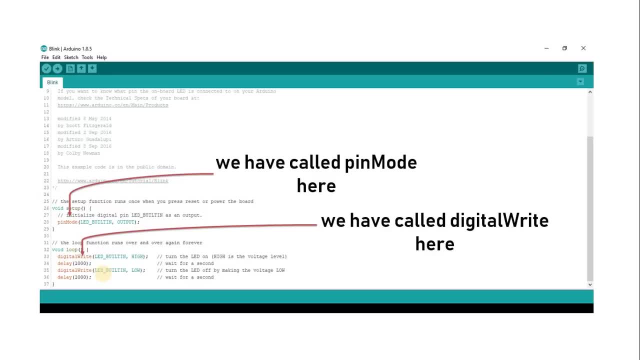 That's why Arduino is able to understand what this exactly means. Otherwise, it won't be able to understand, right? Okay, so it has made us really easy that Arduino guys have defined this function somewhere for us, Okay, and we just have to call it. 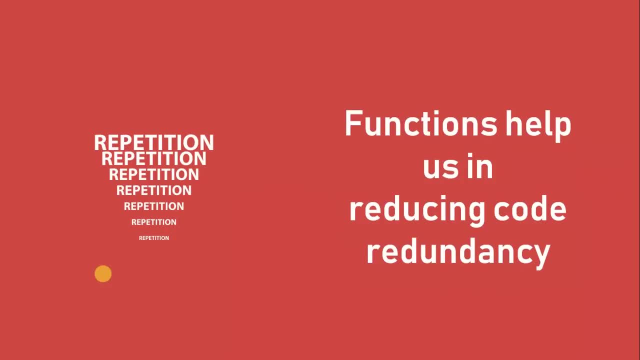 So now let me tell you The benefits of using the functions. The first biggest benefit of using the function is it helps us to reduce the code redundancy. What that means is, for example, we want to do certain tasks, So we may write the statements again and again, again and again. 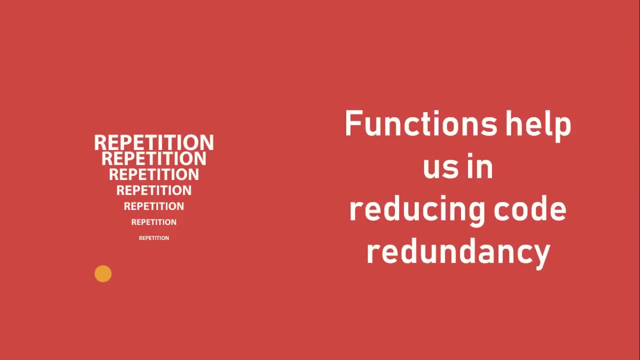 So that would make the code unnecessarily bigger. So what we can do is we can make a function and we just call that function whenever we want to do that task. You will understand this point better when we write our own functions. Then the functions make the code modular and reusable. 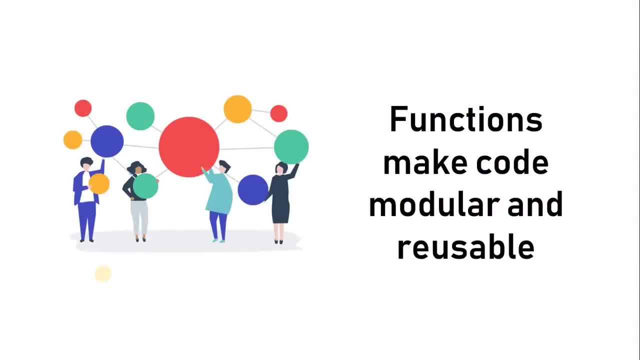 What that means is, for example, we are making a robot. There must be thousands of lines to make the robot go forward. So what we can do is we can make a function to make the robot go forward, and we can use that function whenever we want to make the robot go forward. 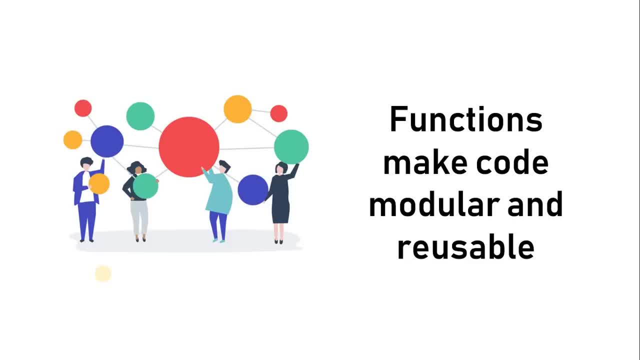 And you have written the code to make the robot go forward. So now you are trying to make another robot So you can use that same code for the another robot as well. So that means it became modular and it became reusable Then. the other advantage of using functions is that it provides abstraction and aids in 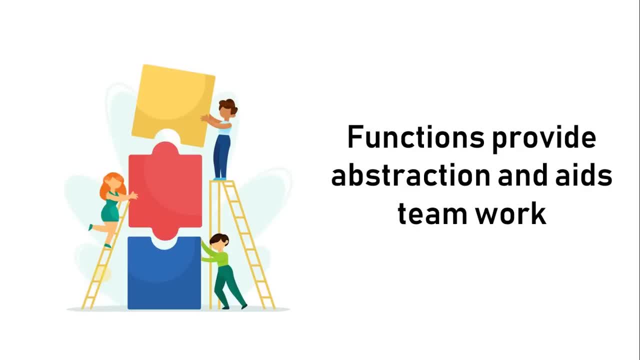 teamwork. For example, you are working in a team of four, So one person can write the code for robot to go forward, One person can write the code to go backward, One person can write the code to move right and left and one can write the code to make. 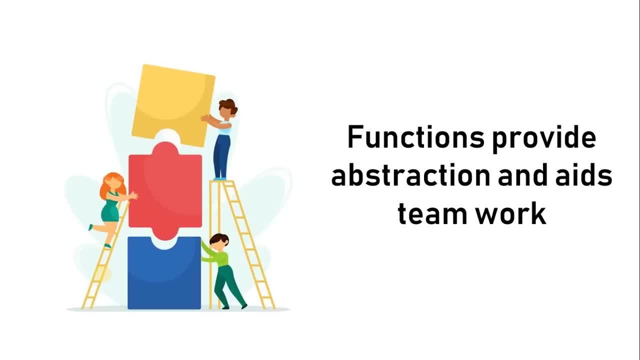 the robot jump. Okay, so once these functions are written, so they can together be used as one code. Alright, so these are the advantages of using a function Now. in the next video, we will learn how to write our own functions. 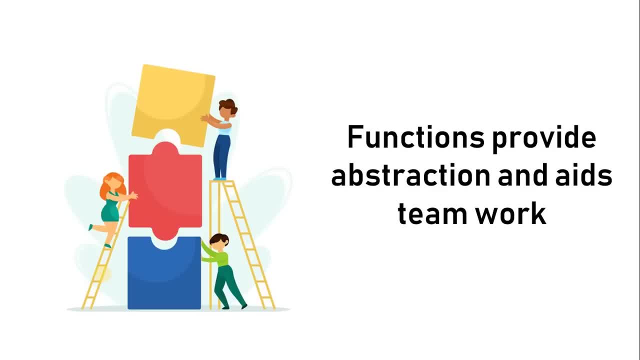 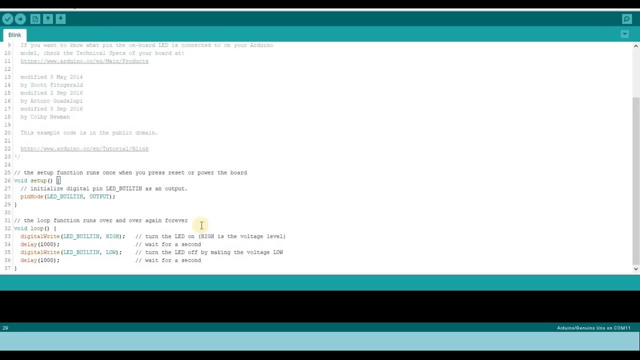 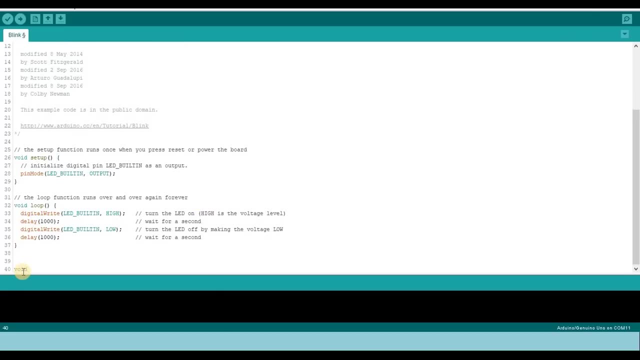 So you will understand these points in a better manner. So I will see you in the next video. So let us now create our very own function. we will create a customized function to blink the LED. Okay, so let's do this. After void loop, we will write void. 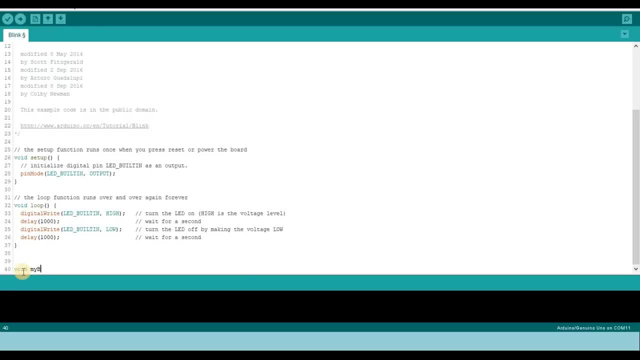 Let's say, the name of our function is my blink function. okay, since there are no parameters in this, we will leave the bracket empty Now. So let us just cut this code from here and paste this exactly like this in my blink function. 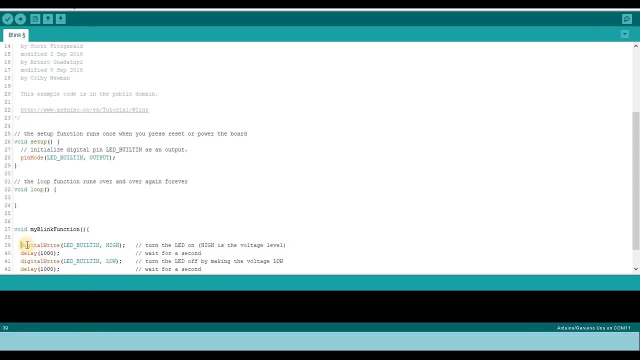 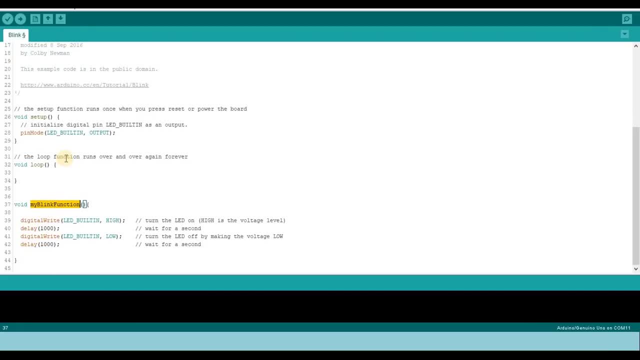 Okay, So now we have created our customized blink function. Now let's try to call this function in void loop, right? This way, we have called our function in the void loop, Alright. so when we upload this code on Arduino, you will see exactly the same results. 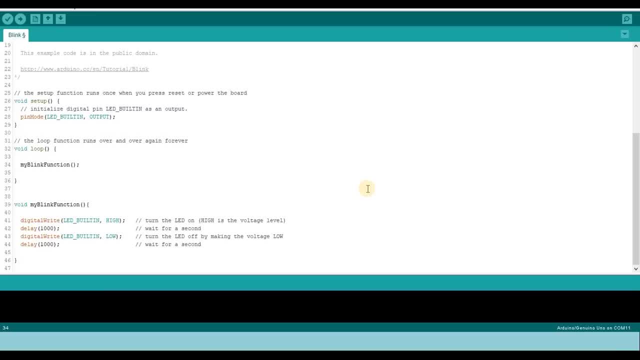 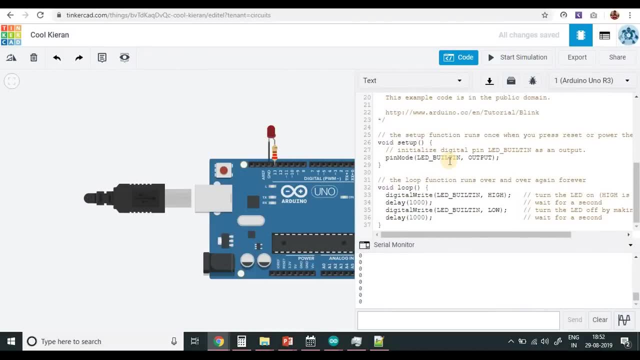 Alright. so let us see this. Let us compare both the codes with the help of a simulator. Alright, so we had this code right. This is the same blink code. Let's see how it is working. Right, as expected. 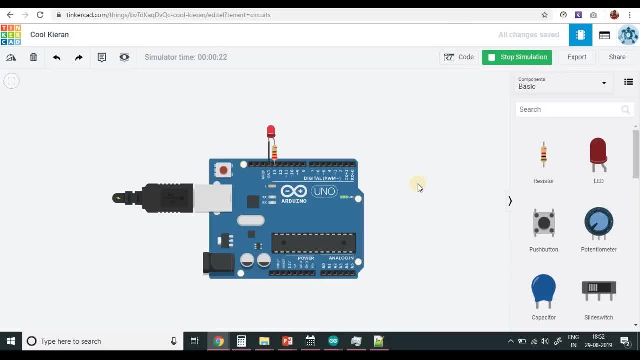 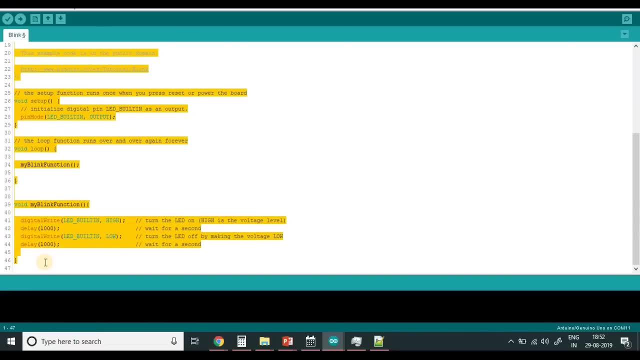 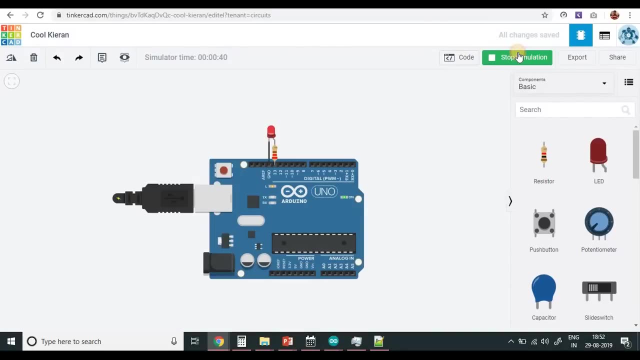 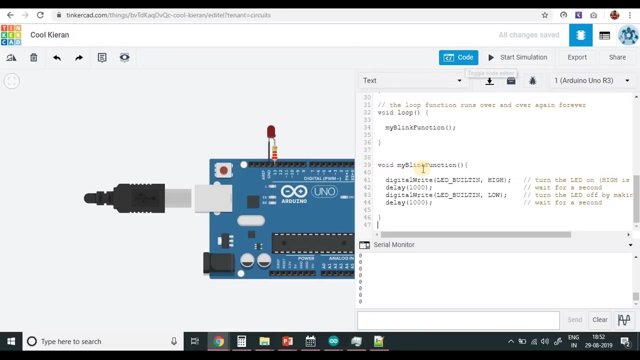 The LED at pin number 13 is blinking- right, So now let us replace the code which we have just written. Alright, so now let's replace the code which we have just written. Let's try to call this code. We will just take it as it is, right. so now let's start the simulation. 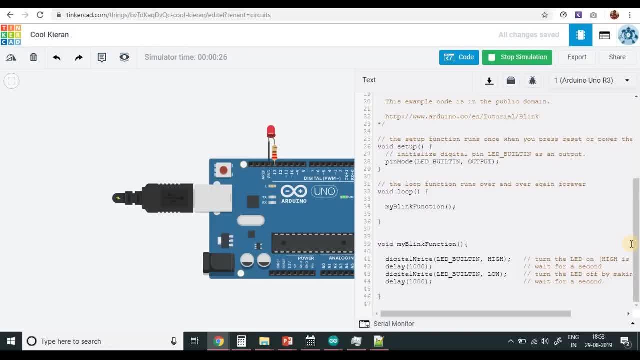 So I hope you got my point about creating our own functions. But now most of you must be wondering what's the point of making this right? yeah, I agree with you, There is no point of making a function for this small task, right? but you will find. 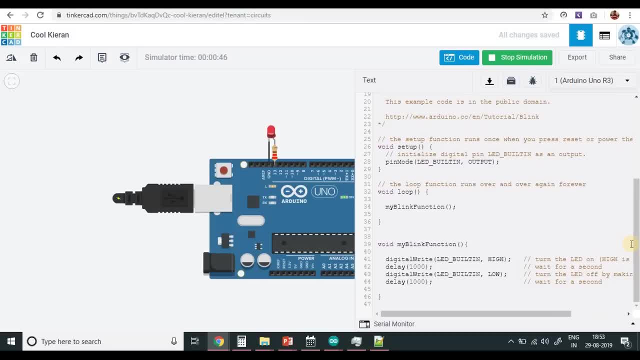 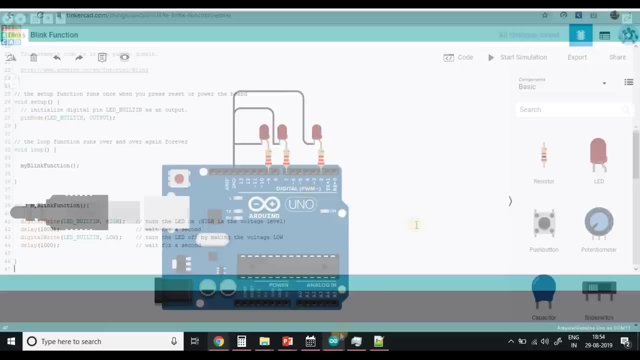 it useful when you're writing really huge programs or you want to customize this thing. I will show you a customization right now. alright, So now let's say you have more than one LEDs which you want to blink in a row. okay, 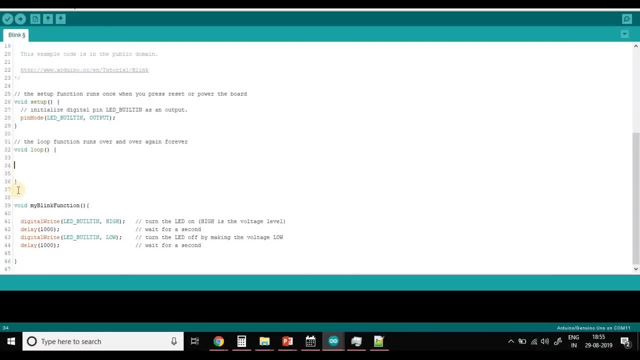 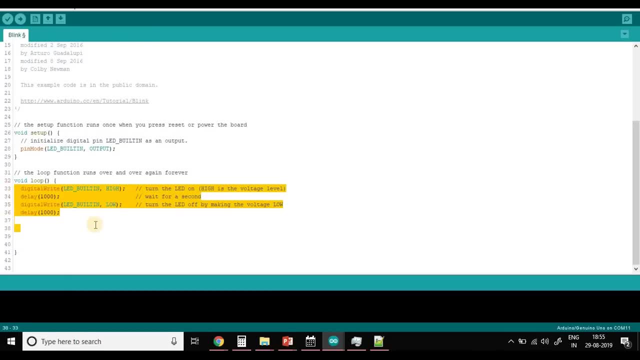 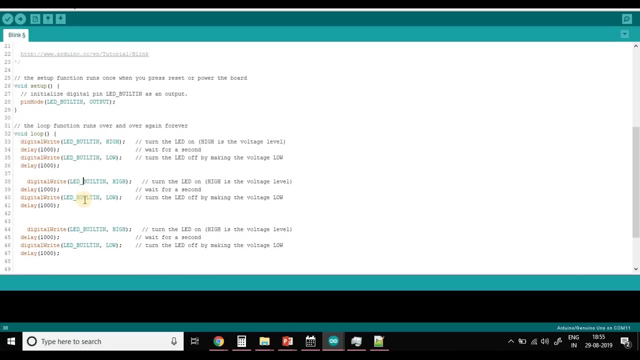 So, with your existing knowledge, what would you have done? You would have done it like this, So you would have repeated these lines of codes and just replaced the pin numbers here, right. and then you would have declared these pins as output, right. but now what we can. 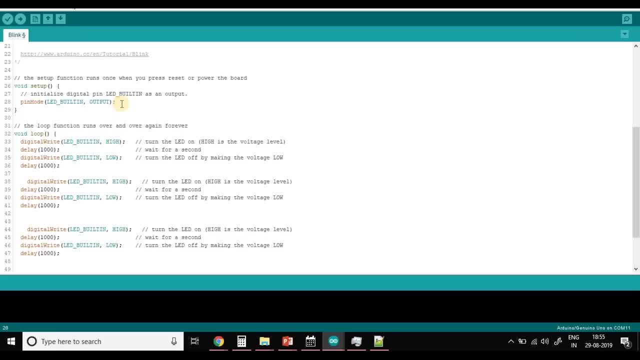 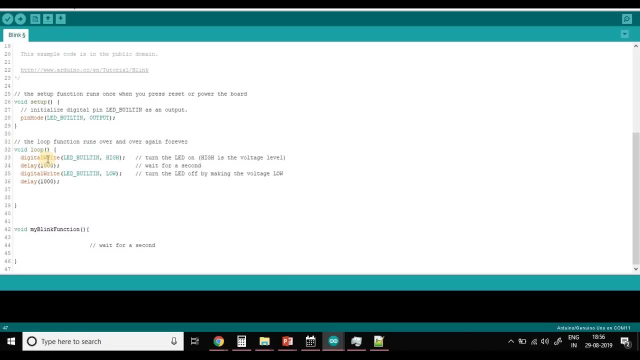 do is: we can make a customized function. let us do that. We are here, So let us now make a new function. void my custom LED right now. what we will do is we will specify a parameters in which we can tell the compiler LED pin number. 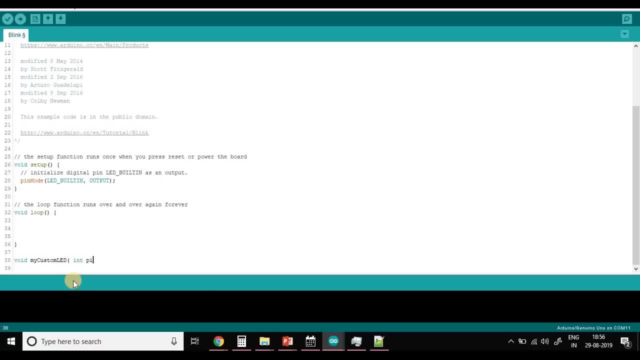 So for that we will write int pin number. okay, So this function is going to accept one parameter, which is pin number, right, So now let's do this. We have this code, okay? So now, instead of LED built-in. 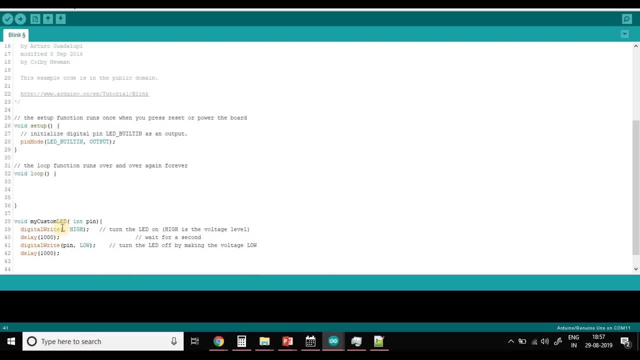 We will write pin here, okay, So automatically, whenever we call this function with the pin specified, the compiler will replace this pin number with the specified pin number. okay, So let's do this. Let us just confirm what pins we have used. 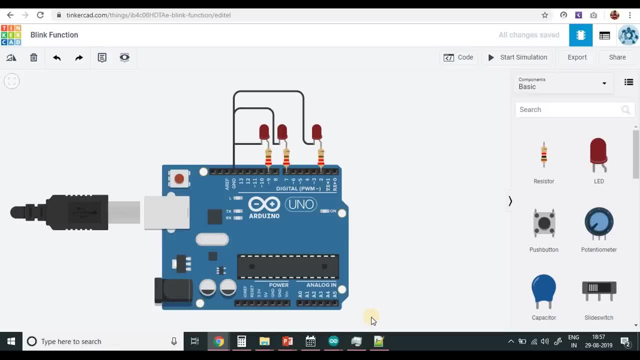 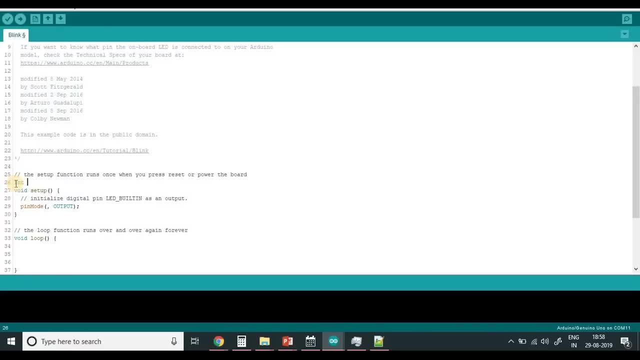 We have used 9,, 7 and 2, okay, 9,, 7 and 2.. So let us say int LED1 is equal to 9, int LED2 is equal to 7 and int LED3 is equal to. 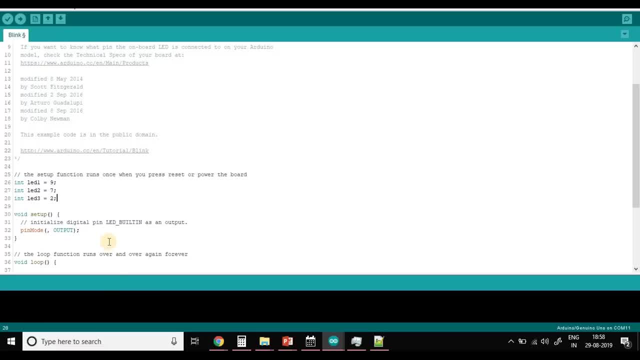 2, right, So now we just have to declare all these pins as output: LED1, okay, C1.. C2.. C3., C4., C5., C6., C7., C8., C9.. C11., C12., C13., C14., C15., C16., C17., C18., C19., C21., C22., C23., C24., C25., C26., C27., C28.. 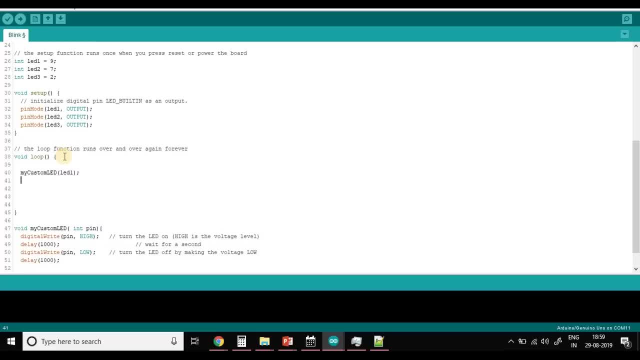 C29., C31., C32., C33., C34., C35., C36., C37., C38., C39., C40., C41., C42., C43., C44., C45., C46. 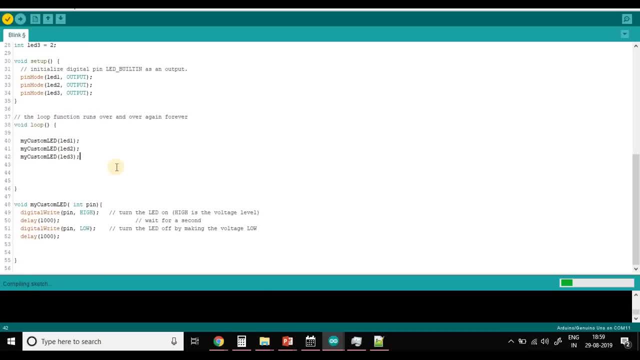 C47., C48., C49., C50., C51., C52., C52., C53., C54., C55., C56., C56., C57., C58., C59., C60., C61. 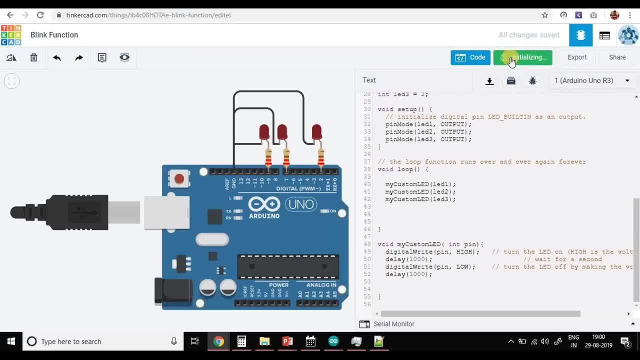 C62., C63., C64., C65., C67., C68., C69., C61.. 1., 2., 3., 4., 4., 5., 4., 5., 6.. 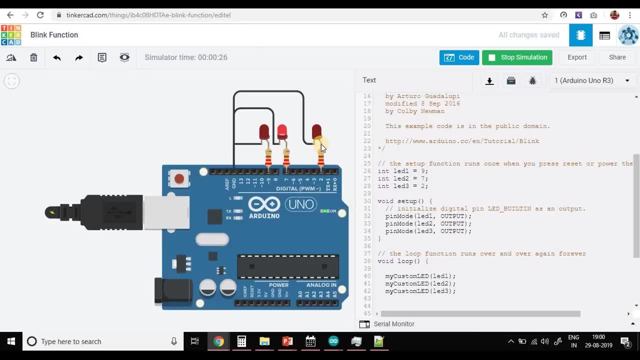 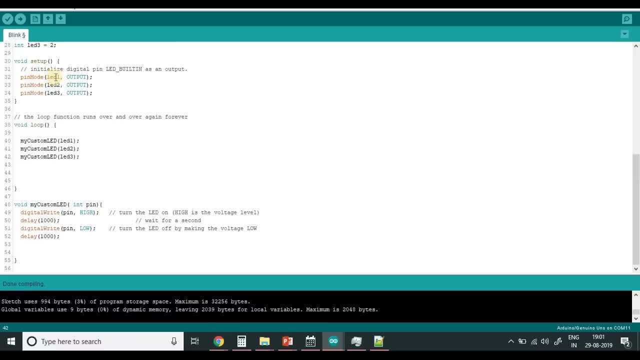 7., 8., 9., 10., 11., 12., 13., 14., 15., 16., 17., 18., 19. 20.. sure you know how to do this. We have done this many times till now. Okay, so now we. 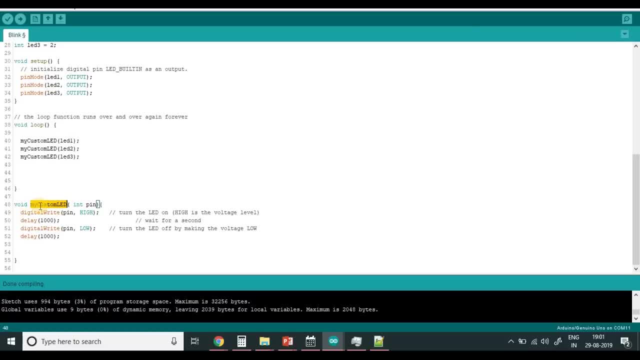 have created a function void my custom led with the parameter of pin. If you wanted more parameters here, we'll just write comma and then int, let's say parameter two, right, So this way we can specify endless number of parameters in our functions. But since we 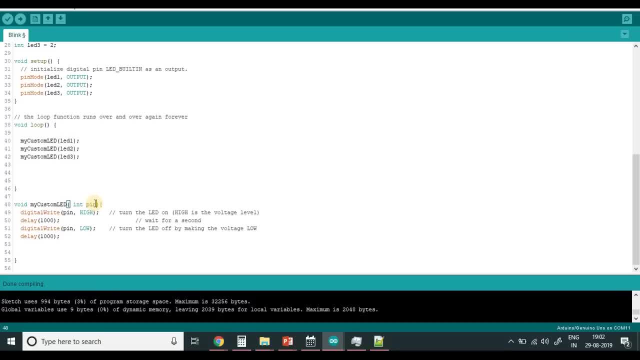 don't need them, we'll not use them. Okay, then we have started to define what this function will do, which is it will blink the LED. Okay, which LED will it blink? the LED which we have passed as the parameter? Okay, because we have used pin here. For example, if you had 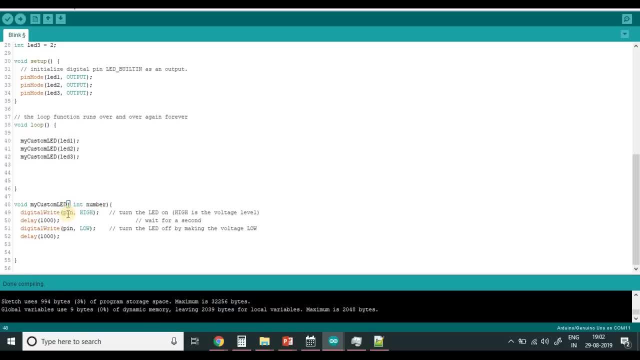 declared number here instead of pin, then you would have used number here instead of pin. Got my point? So now, since we have finished declaring our function, now we can use it successfully. We'll just take this function and we will call it here with the parameter. 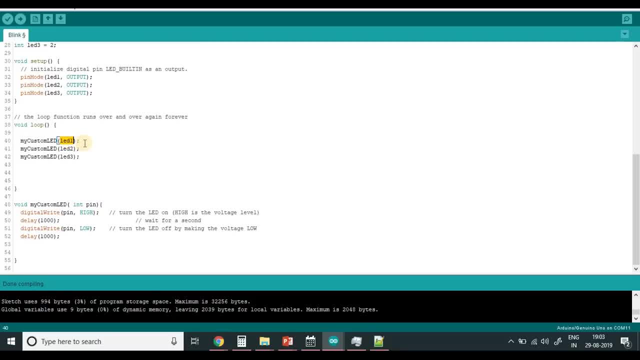 So now we have called it for the first time with led one. Now what will happen? The compiler will see: okay, a function has been used which is my custom led, with the parameter led one, So it will see the value of led one which is declared as nine. Okay, so it will call. 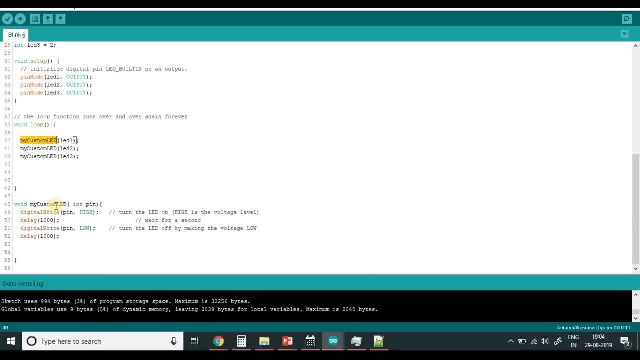 my custom led with nine. So the control will go to my custom led with pin nine and it will execute. Once it is done executing, it will come back. it will see it has been called again with another parameter, which is led two, and the value of led two is seven this time, So it 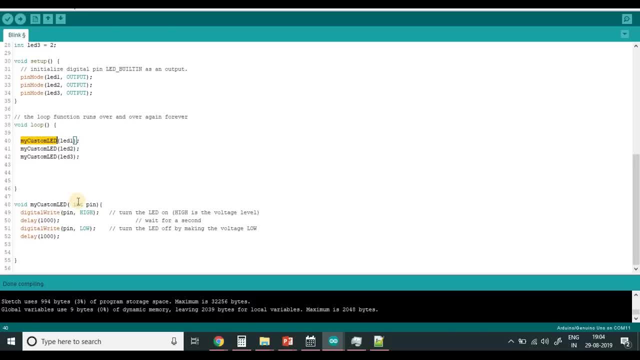 will go back and execute the function again with the value of seven. All right, this is the basic concept of function customization. Okay, so instead of writing this code again and again with changed pin numbers, we can just do this. So I think all of you can agree. 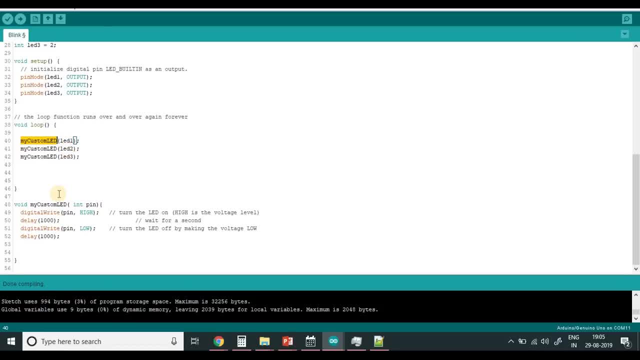 with what I'm saying right now, Right? One more thing which needs emphasis is I've used void here. Like I told you, we use void whenever our function is not returning us anything. Okay. so by the time you must have realized void loop and void setup are two functions of their own. They are the main. 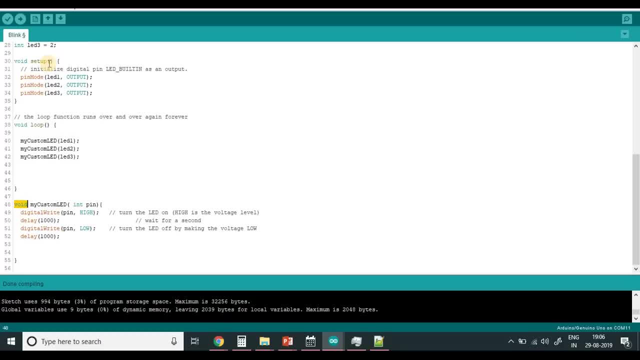 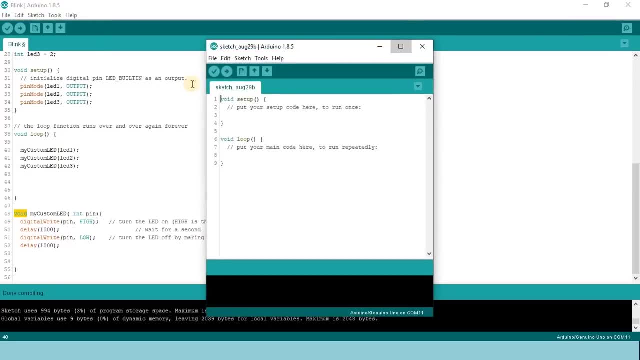 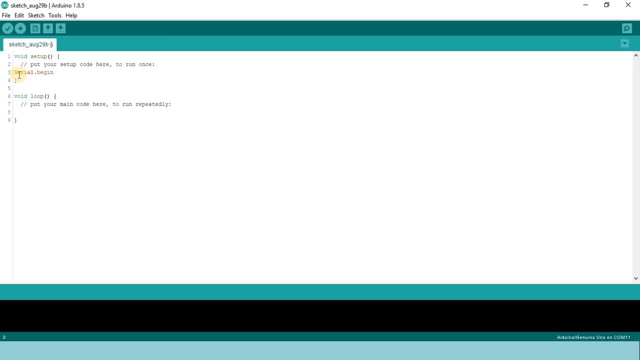 functions which are used by the compiler. We have discussed about this earlier as well, So now let us try to make another kind of function. We'll open a new file And we will start writing Our function. First of all, let's write serial dot begin. This is the most crucial thing. 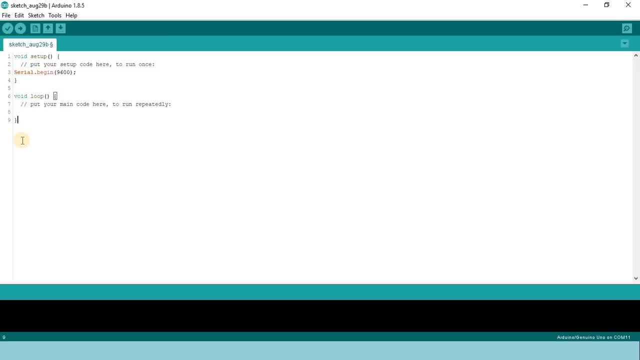 to start communication with the computer. Okay, so now let us try to write a function which would return us something. Okay, so let's say it will return us an integer, So we'll write int. Earlier we wrote void because we didn't want it to return something to us. 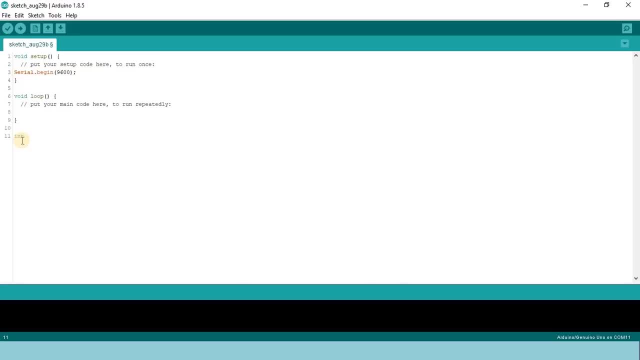 If you're not able to understand what returning exactly means, you will just see that in a moment. We will repeatedly calculate sum of two numbers, Okay, or let's say sum of three numbers. So we will write int sum- Okay, int a comma, int b comma, int c: Okay, we're a, b and. 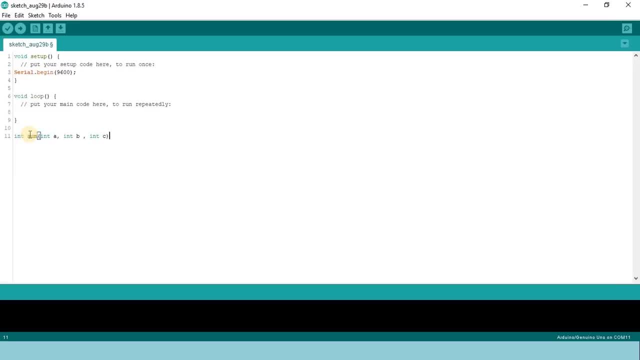 c are the three numbers which we want to take some of. All right, So now we will write a curly bracket And then we will write return a plus b plus c. Let's say a And then we will write a. So we will write a curly bracket And then we will write return a plus b plus c. 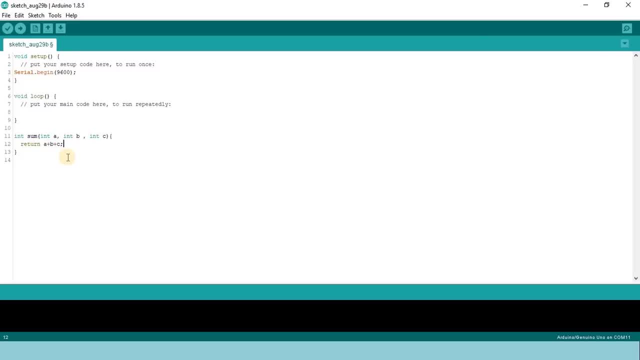 Okay, so whenever we call this function, we'll get a value of a plus b plus c. Let's see how we get it In void loop or void setup. you can use this function anywhere you want. So let's say we'll use this in void loop, okay. 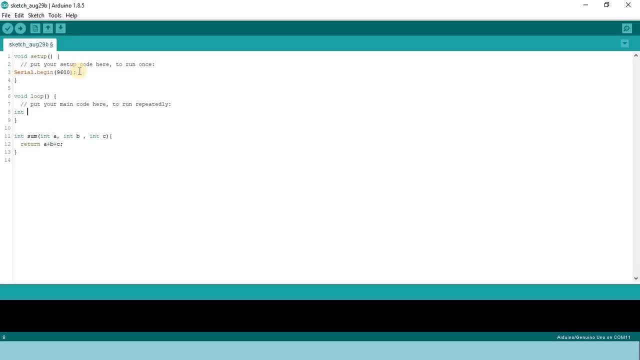 Let's say we write int, let's call it d, okay, equals to sum of 7 comma 8 comma 9.. Alright, and let's print the value of d, okay. So what should it print? The sum of 7,, 8, and 9,, which is 24, right. 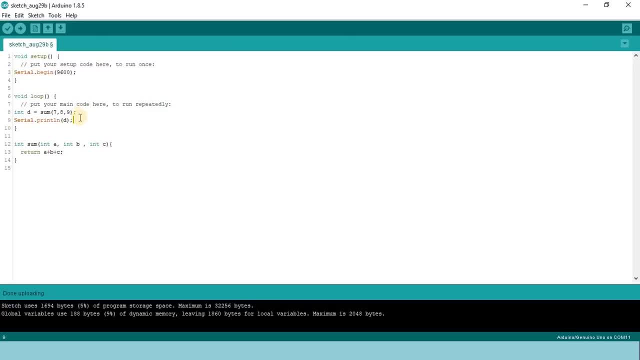 We can use it again as well with the different set of values. Let's say we'll make another function. int e is equal to sum 1 comma 2 comma 3.. Let's print this: We should get 6, right. 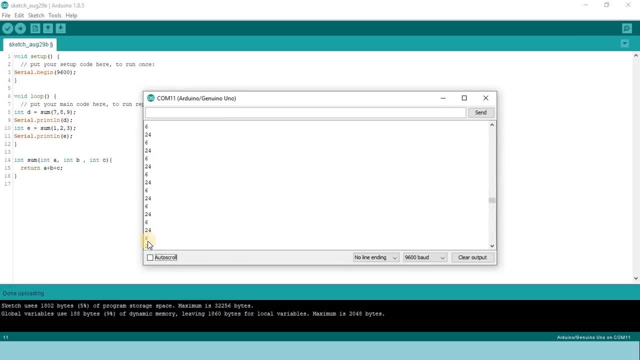 So we're getting 6, 24 and 6.. It's repeating as we have used it in void loop, So you don't have to worry about that, okay. One thing which I want to tell you is you can use this function like this as well. 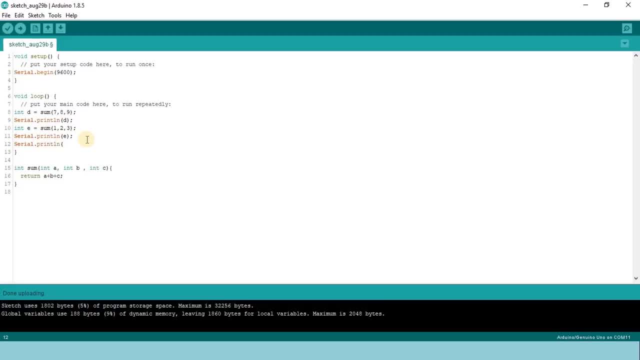 Serial dot println directly in serial print sum 4 comma 5, comma 6, right, Just make sure to close all the brackets. Here we have closed the bracket Of the function sum. here we have closed the bracket of serial dot println. okay, 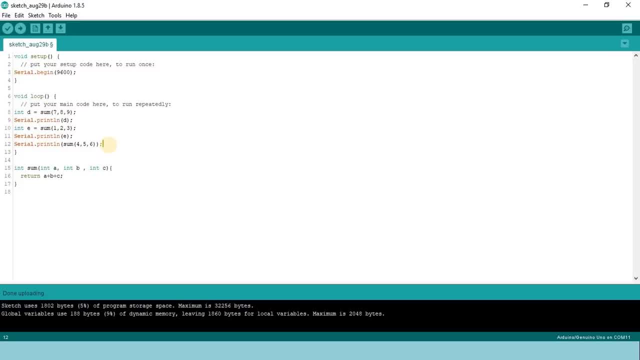 So this is called as calling function inside a function. This is a very useful thing which we can do in programming, But first of all let us see the result: if it is working or not. right? So we are getting 15 here because this function call here is printing its value. okay, 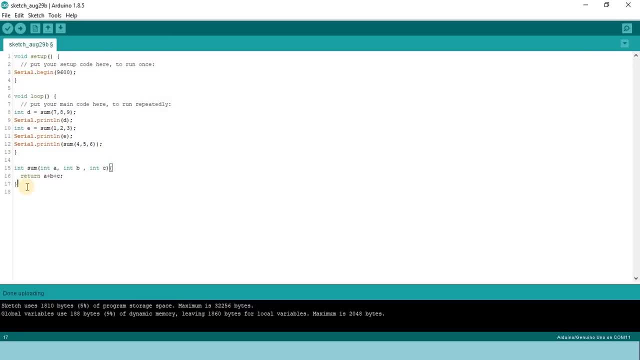 Now we can have More than one functions in our code. Now let us declare another function which would return a boolean value, Let's say bool. Now we are making a function to check if a person is tall or not based on the height we enter as the parameter. alright, 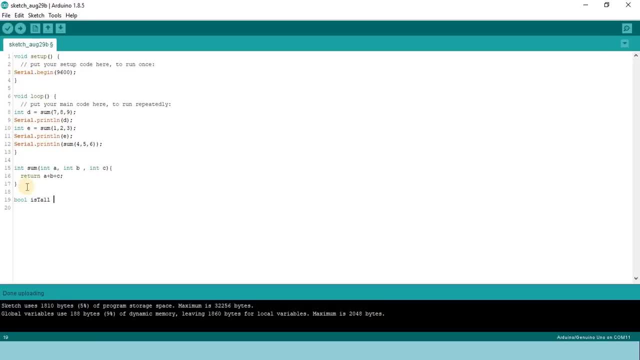 So let's name it isTall, okay, And int height, okay. So this function's name is isTall And the parameter is height, okay. So we'll write if height is greater than 100, return true, okay, or else return false, okay. 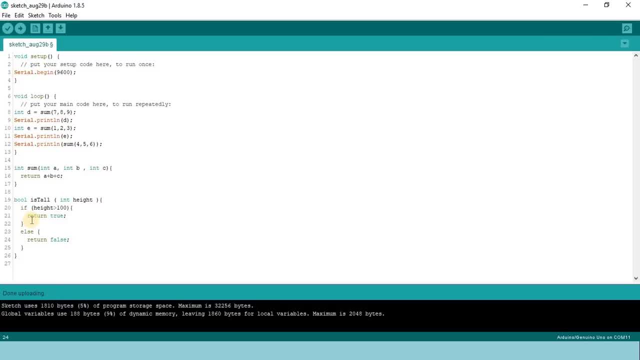 So this function will just return true if the entered height is greater than 100. And if it is less than 100, it will say false. okay, So now let's see. Now you'll see how handy it becomes when you have to check height of multiple people. 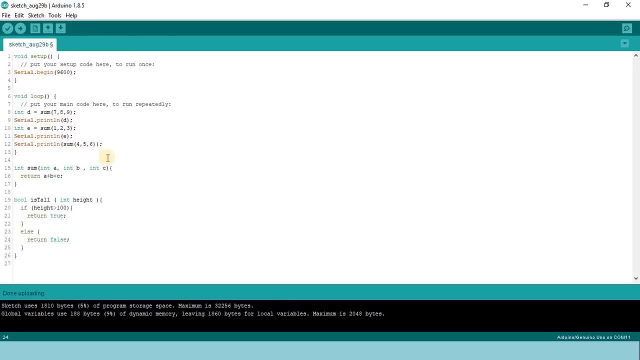 okay. So now let's call this in void loop. Here we have void loop. Let's say serialprintln isTall. Let's say 123, okay, Okay, Let's just comment out the print statements so that they don't interfere, okay. 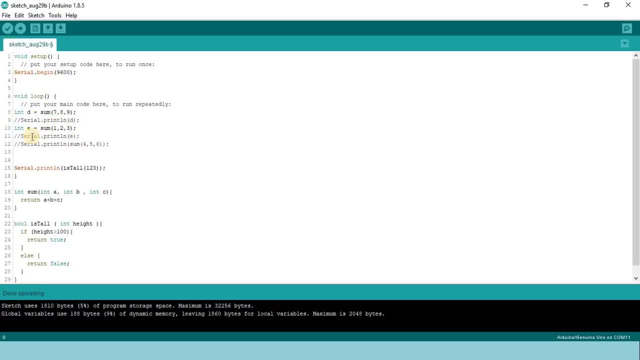 This function is still being used in int D and int E, So you can say these functions are working simultaneously. So we are just checking isTall or not. okay, Let's see Before I open the serial monitor. you can guess your values, right. 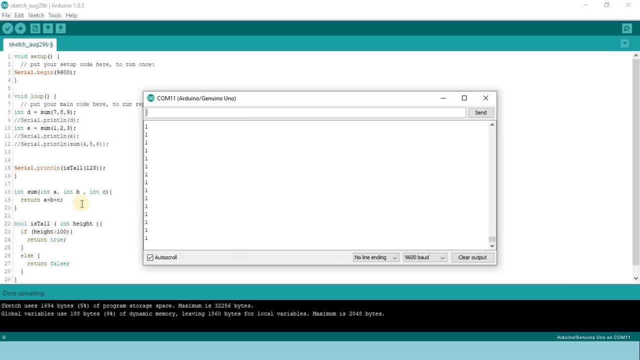 It's printing one because it has returned true. So now let us take another value which is less than 100.. Serialprintln isTall 20.. So now we should get false. So it would be printing 1010, because one is for isTall 123 and zero is for isTall 20.. 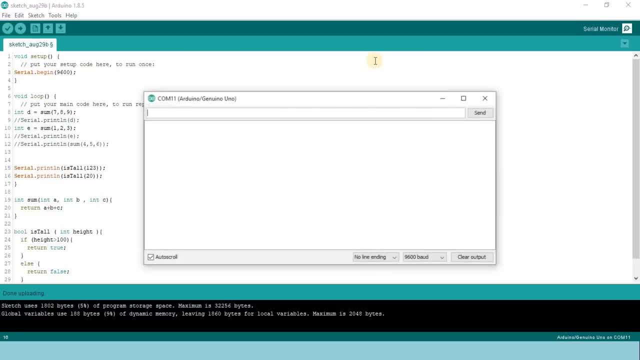 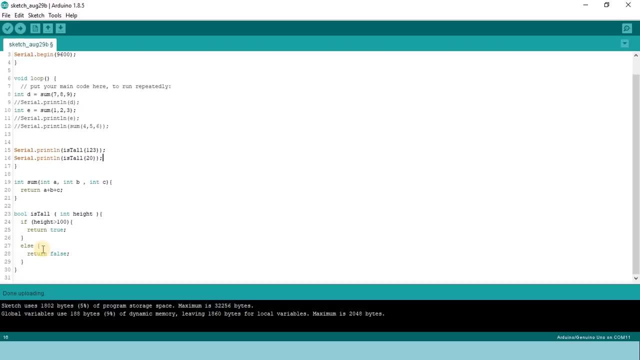 So let's see. Okay, So if you have to check height of multiple people, instead of writing this code again and again for that specific height, you can just call this function and enter the height, So you can see how much work you have reduced for yourself, right by writing the functions. 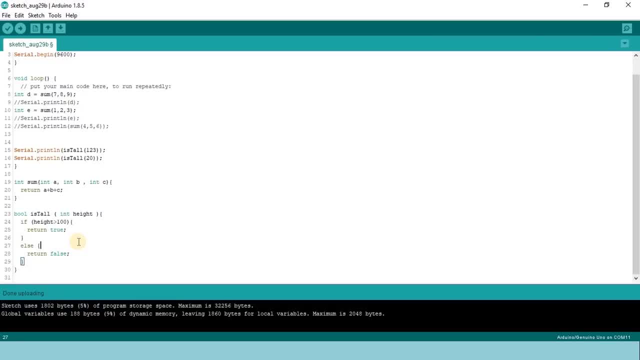 So this was all about writing a custom function. There is no upper level to the complexity of the code which you write in your functions. You can write endless number of lines in this function. Okay, Like I told you in the introductory video, there may be thousands of lines which are: 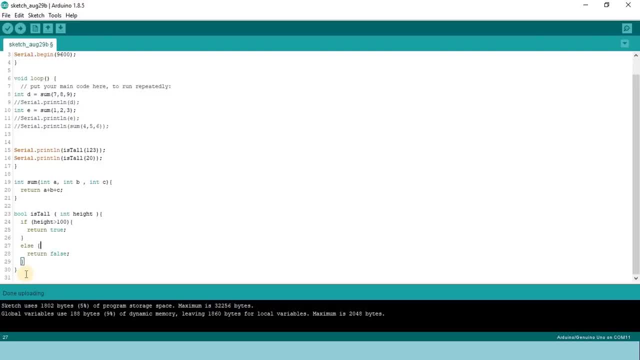 responsible for making robot go forward. So in that case we can write void- move robot forward, and we can just define our parameters here and we can just write our statements like this: right, And this is our function. This block of code won't make your robot go forward. 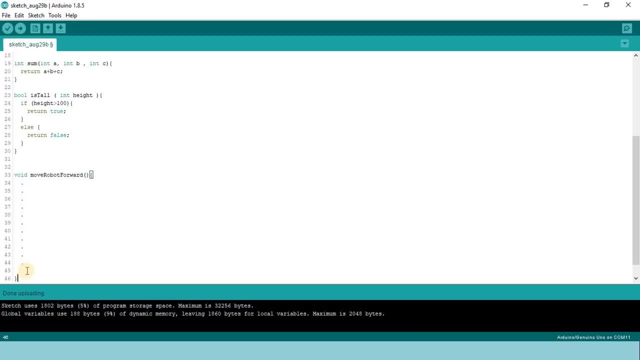 I'm just giving you an example of how do we write functions. Okay, So whenever we call move robot forward in void setup or in void loop, so the compiler will take this function and it will execute that, All right. So in the next video we will take a deeper look at some of the inbuilt functions which 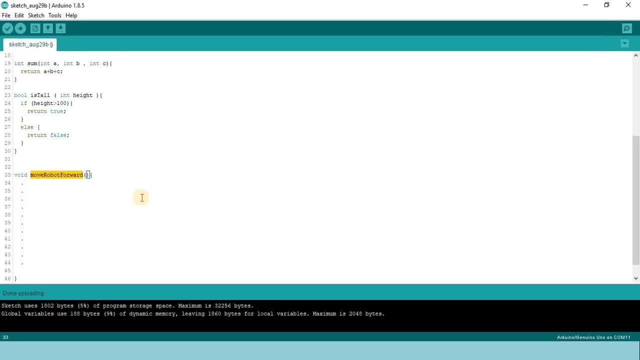 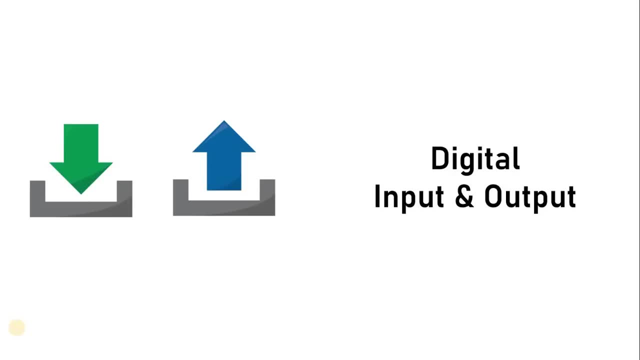 the Arduino makers have made for us. So see you in the next video. Now, in this video, we will talk about digital input and output. What that means is we'll take a closer look at the functions which are made by the Arduino makers to read or write any sort of digital data. 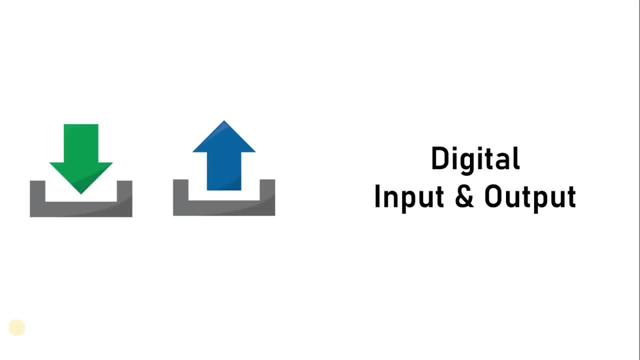 All right, That data can be some sort of input given by external sensors and it can be some sort of output data which is given by Arduino to other peripherals or components. right? So there are basically two functions, which are digital read and digital write. 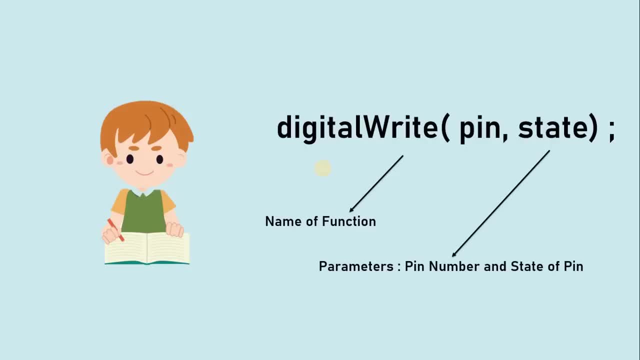 So let's take a look at digital write. Digital write is a function which we have seen multiple times before as well, So can you recall what it is? Okay, So what it used to do? It used to write a state of low or high to a digital pin. 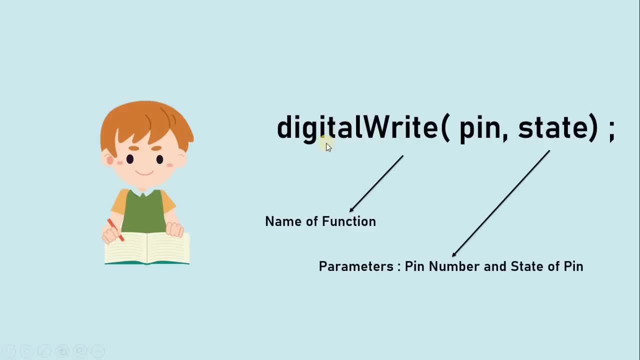 So we'll see. digital write is a function where digital write is the name of that function, All right- And it has two parameters, which are pin and state, where pin is the pin number which we want to manipulate and the state is the value of either high or low, where high means 5 volts. 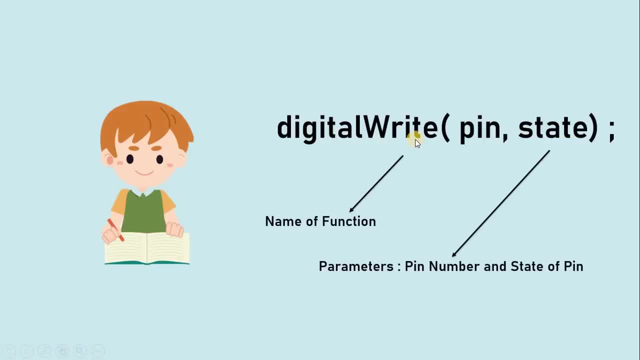 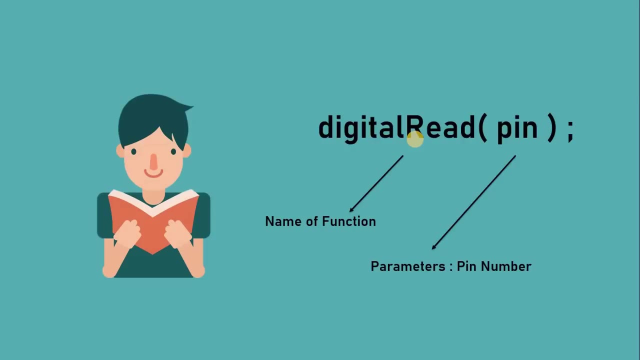 and low means 0 volts. Okay, Just make sure, whenever we use digital write, we have to declare that pin as output using pin mode. All right, And I have told you this earlier as well. Right, Next, we will see digital read. as the name suggests, it will read the state of that pin. 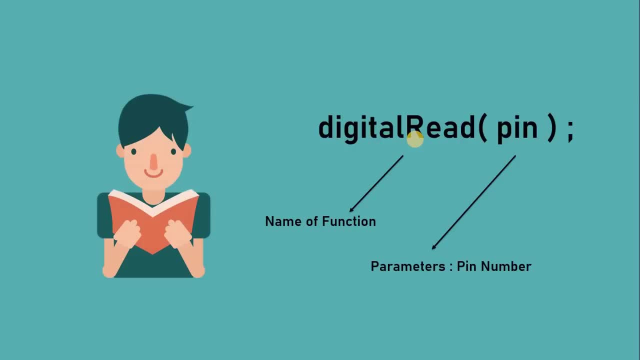 Okay. So here, digital read is the name of the function which we are calling and pin number is the parameter which we pass into it to read the state of that particular pin. Okay, If it is high or low. So we'll now see a combined example of using digital read and digital write. and how will. 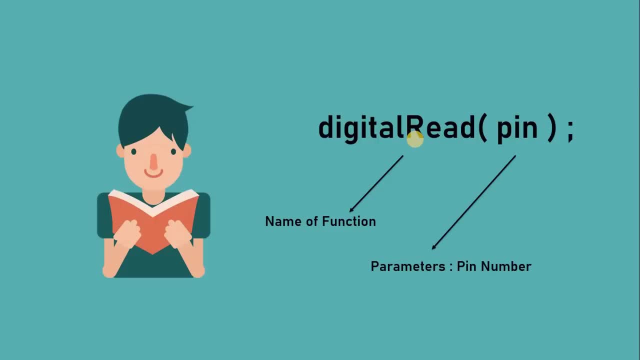 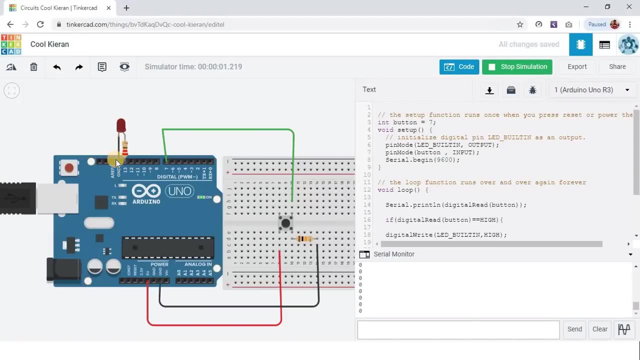 we do that. We will turn on one LED if a switch is pressed. Okay, So let's see how we do that. So I have the circuit diagram here, in which I have used a regular LED with a resistance in series, which you can see, and here I have used a push button switch. before we move further, 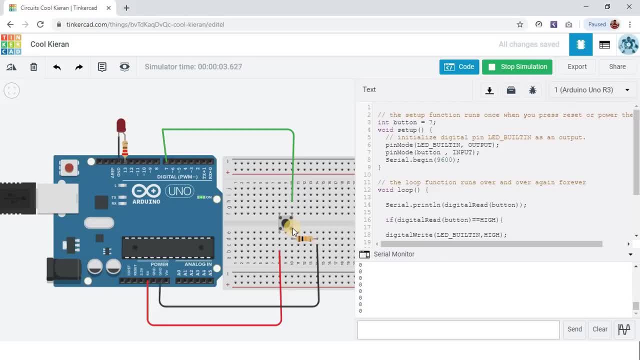 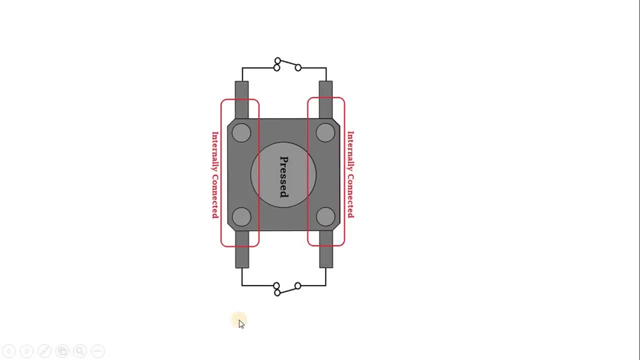 Let us first look at what a push button switch looks like from inside. Then only you will be able to understand it in a better manner. So here is a push button switch- all right- which has four terminals, out of which these two terminals are internally connected. and these two terminals are internally connected. 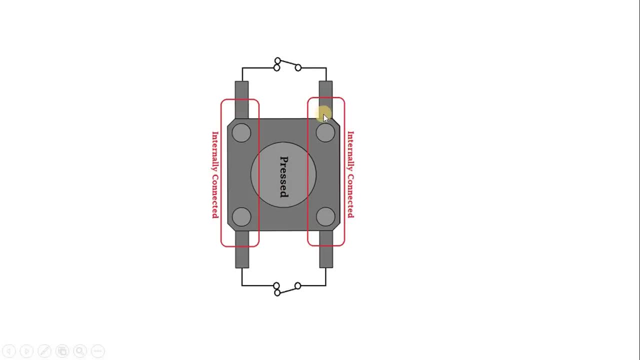 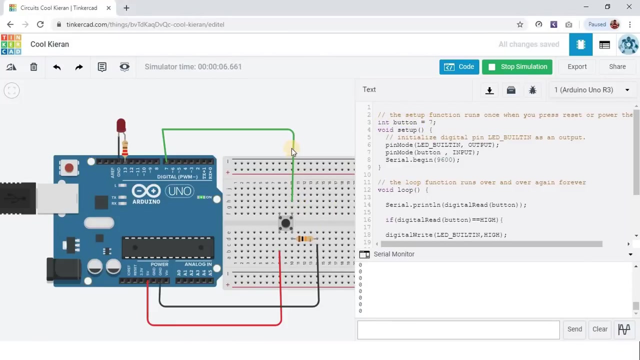 as well. Okay, So when we press the switch, These two terminals get interconnected, and these two terminals get interconnected when it is not pressed, These two are not interconnected. Okay So, let's get back to our example. Okay, So the code is: we have started with. int. button is equal to seven, as we want to read the state. 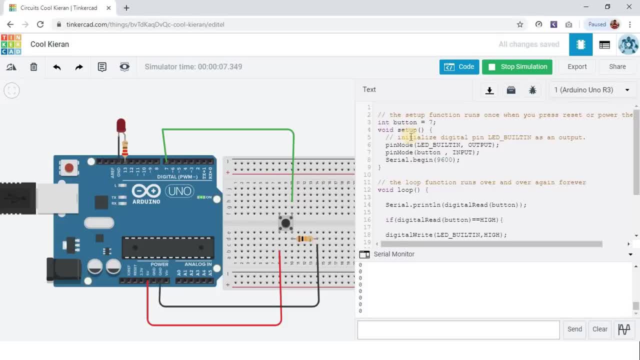 of that button on a digital pin number seven. All right In void setup. I have declared pin mode LED built in, which is the LED connected to pin number 13, as output and using pin mode we have declared the button as input because 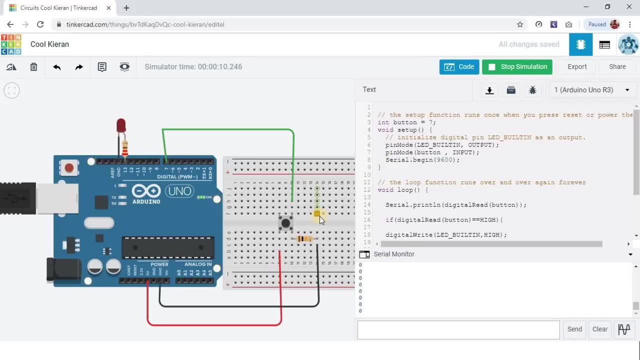 button will be telling its state to the Arduino. Hence This is the serial dot: begin 9600. as usual, then in void loop I have written serial dot println- digital read and bracket button. So here I'm asking it to print the state of the button: either it is pressed or not, in 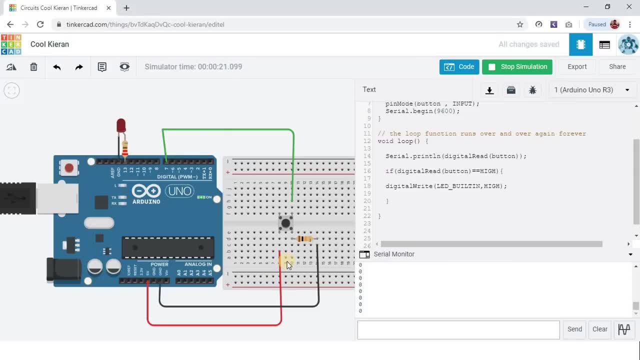 the circuit which we have used. we will get one on pressing the switch and we'll get zero when we do not press the switch. All right, So let us see that once when I'm pressing the switch, I'm getting one here and I'm releasing. 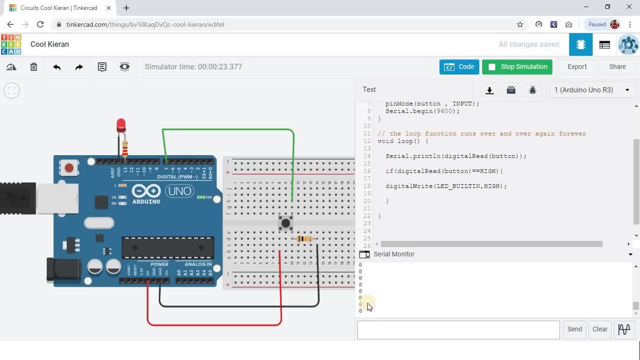 the switch. I'm getting zero here. Look at the serial monitor here. Right now I'm not pressing it, So it's saying zero. when I'm pressing it, It's saying one. Okay, Most of you must have also noticed the LED which is connected on pin number 13 when I'm 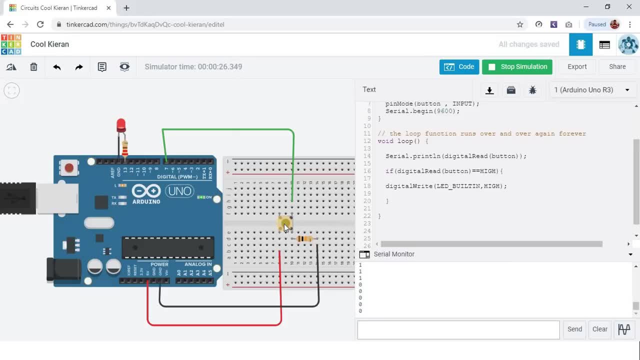 pressing the switch, the LED is getting turned on, and when I'm releasing the switch, oops, it's not getting turned off. Why? We'll see that in the moment. Probably there's some error in the code. I've done this intentionally so that you can pay attention to that. 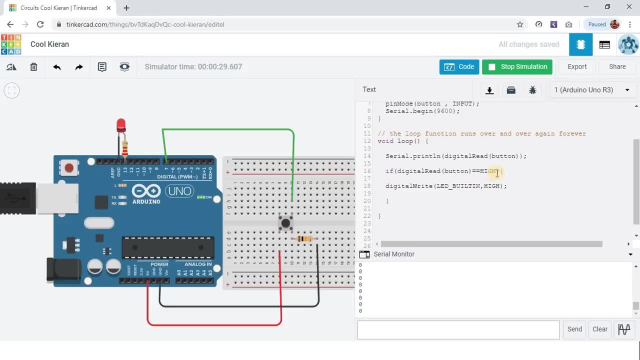 Okay, So here I have written: if digital read button is equal to high, then digital write LED built in to high. So write a high state on pin number 13,. but I have not written what to do if the button is not pressed. 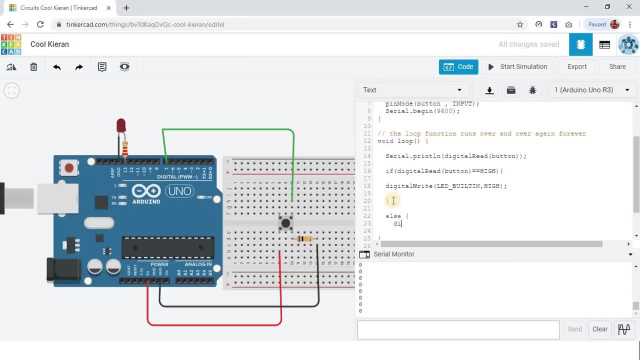 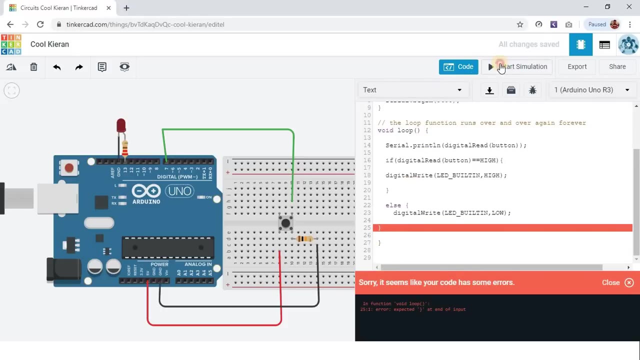 So let us do that now. We will write else. digital write LED built in low. Okay, So now let us start this again. There was an error. The closing bracket to void loop was missing, So let us start that again. All right, 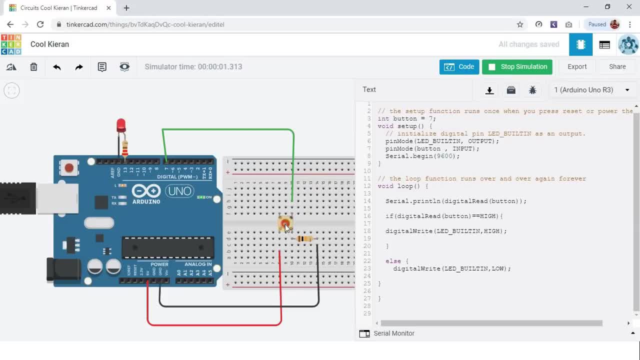 So when I press it, the LED turns on, and when I release it: there was an error. The closing bracket to void loop was missing, So let us start that again. There was an error, So let us start that again. So when I press it, the LED turns off. 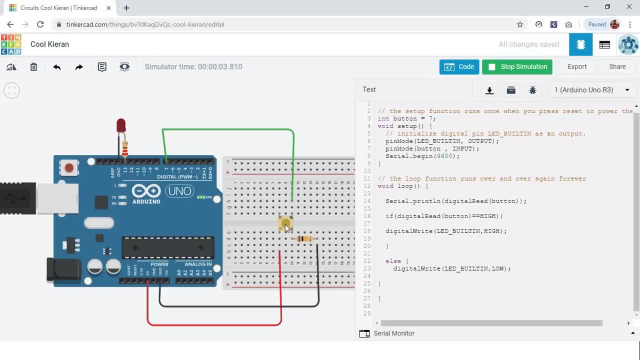 Okay. So you guys must be wondering what's the point of doing this. We can use a simple series connection and we can turn on the LED. Why are we using Arduino? in that I absolutely agree with you. You can do that very easily using a series connection. 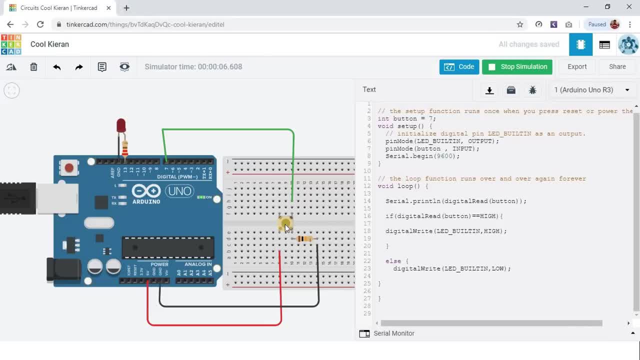 But what you have learned here is you have learned how to use the functions like digital read and digital write. You will be able to implement this learning in further projects, the experiments which you do. All right, So now let me just quickly explain you the circuit which we have made here. as most of 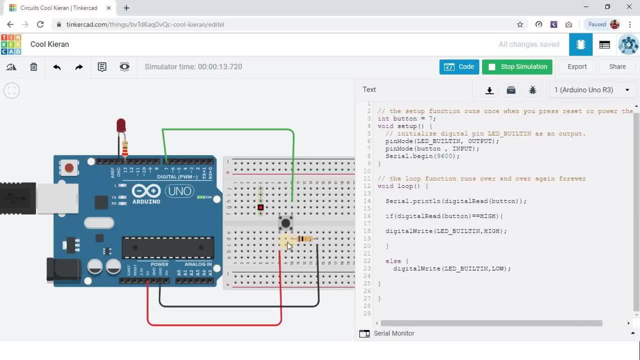 you must be facing difficulty in that. all right, so here is the switch. I showed you the diagram previously, right? so these two terminals are interconnected automatically. when I press the switch, this terminal will get connected to this terminal. okay, so I have taken a wire and connected one terminal to 5 volts, okay? 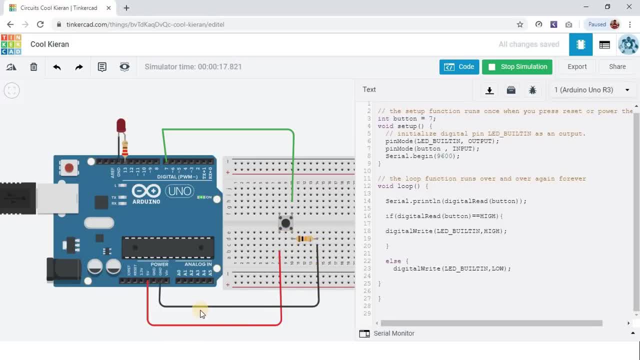 and then I have taken a resistor and I have connected it to ground. so here we have made a series connection of a switch and a resistor like this and from this point, as all these points are interconnected, we can connect them anywhere. at this point we are reading the voltage which is present between 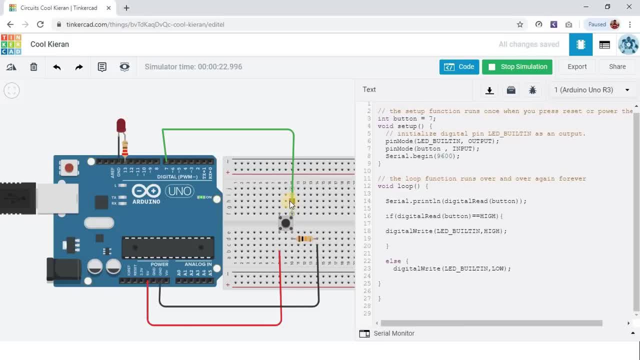 this and this point. okay, so, as we want to read the state, we have connected it to the pin number 7. so when we press the switch, this line will get connected to this line. an entire 5 volts will drop across this resistance. okay, so hence the 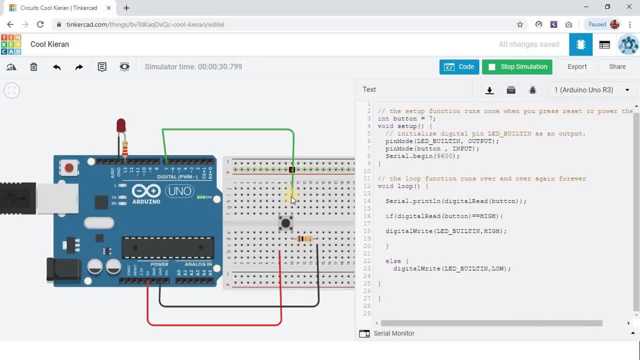 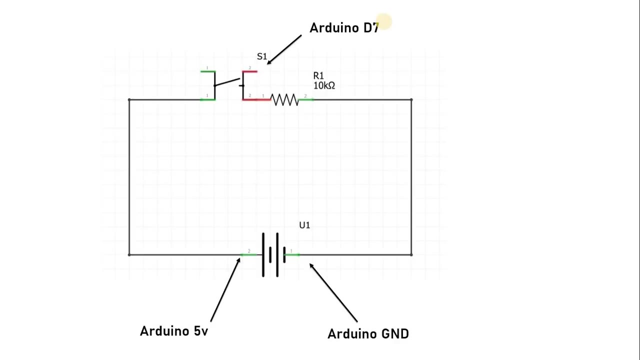 Arduino will read it as high state and when the switch is released, this point will be connected to ground via resistor, so it will be read as low. okay, so I hope you understood the basic idea. let me try to clarify it even more. so this is the equivalent circuit of the circuit which: 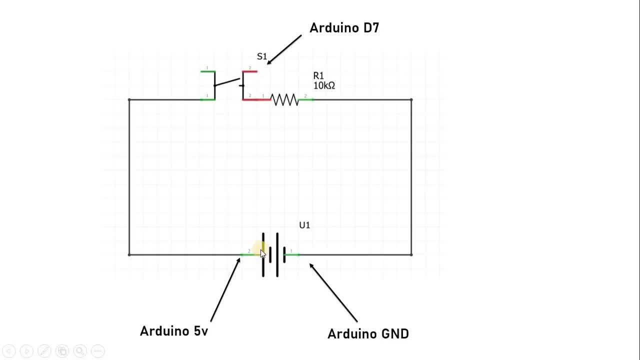 you saw earlier. okay, you can consider Arduino's 5-volt pin connected to this switch. this is a push-button switch, right? similarly, these terminals are connected and when we press the switch, these two terminals will get interconnected. okay, so in the series we have used a resistance and we have 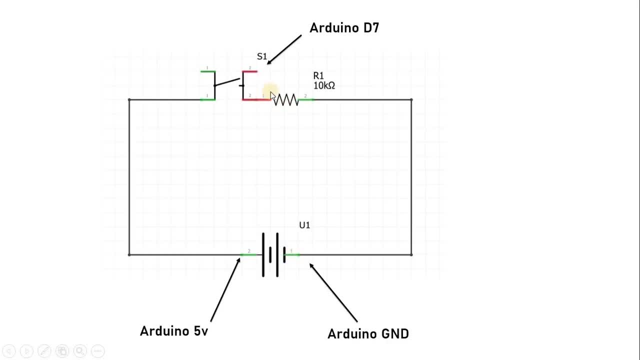 connected one point of that resistor to ground. okay, we are trying to read voltage from this point. can you see that we have connected this point to Arduino's pin number 7? all right, so this way we are able to read the state of a switch now. what advantages can you have after? 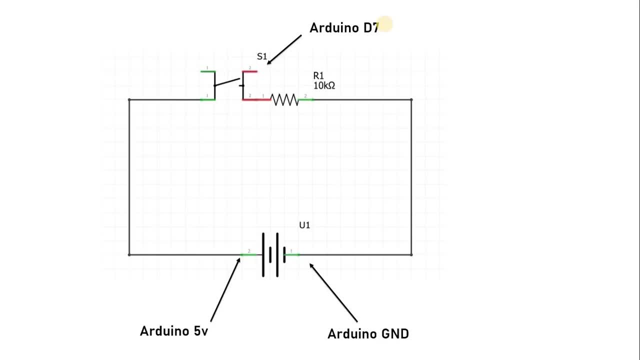 reading a state of a switch. you can trigger multiple actions like running a motor or sending some message. right, you can do anything for that matter. so now you have learned about digital input and output, and in the next video we'll look at other functions like analog read and analog. 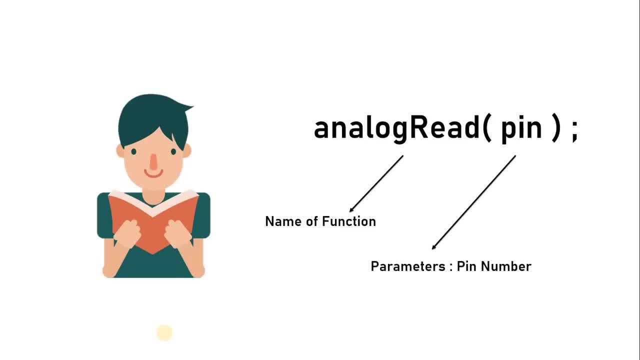 write. so see you in the next video. in the digital input output video we saw that we can use a function called a digital read to read the state of a pin, if it is high or if it is low. that means we can just read the binary situation if. 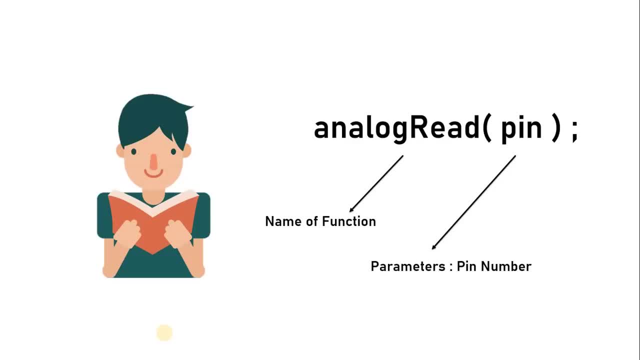 it is on or either off, that's all. but while making a projects we may have situations in which we have to read not just those discrete values. we may also have to read the continuous voltages. so for that we have analog read. this function can be used only on the analog salt. 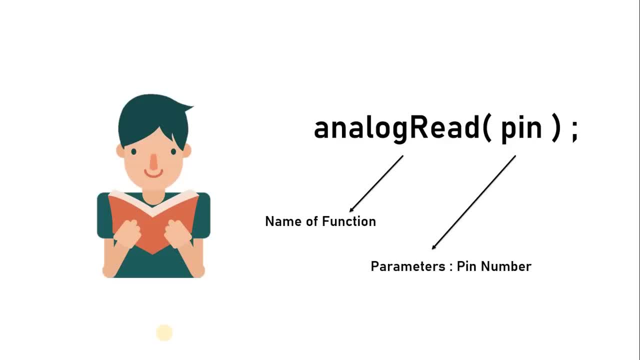 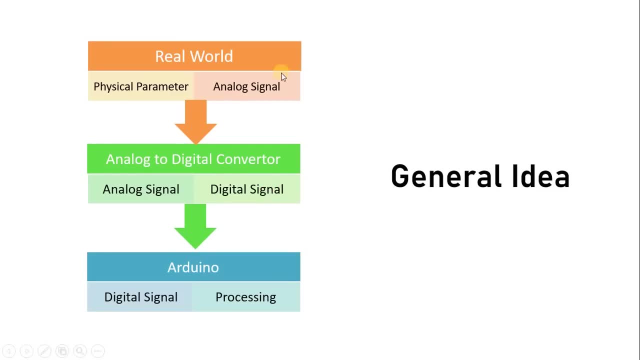 pins which are numbered a0 to a5. right before seeing how it works, we'll have a basic idea of analog information in the environment. so just look at this flow chart. we have the real world, which is our environment. at the top we have some sensor which is converting that physical parameter. 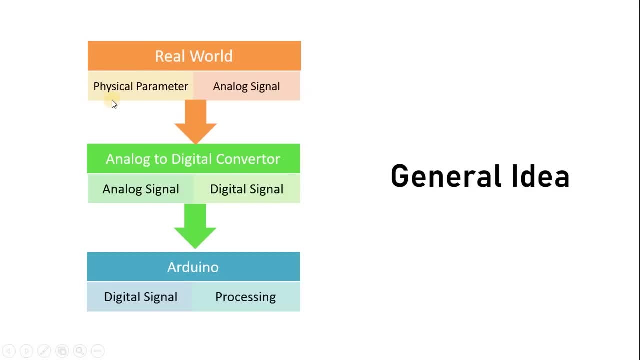 into an analog signal. that physical parameter can be temperature, some distance or humidity, or anything for that matter. that analog signal is then converted into digital signal by an analog to digital converter. arduino has a built-in 10-bit adc. the short for analog to digital converter is: 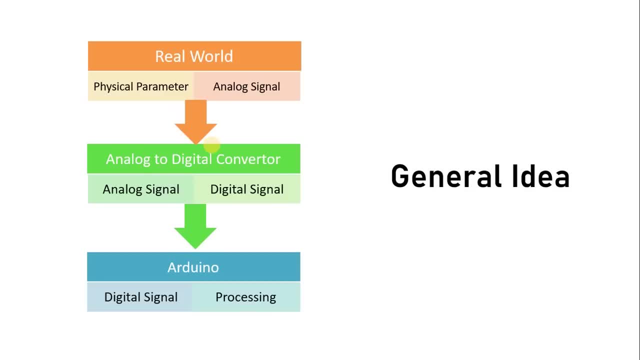 adc. so whenever i say adc, you can understand that i am saying analog to digital converter, so that digital signal which is converted from analog signal that is used by arduino to make decisions. our arduino board is capable of measuring voltage between 0 to 5 volts and this is the 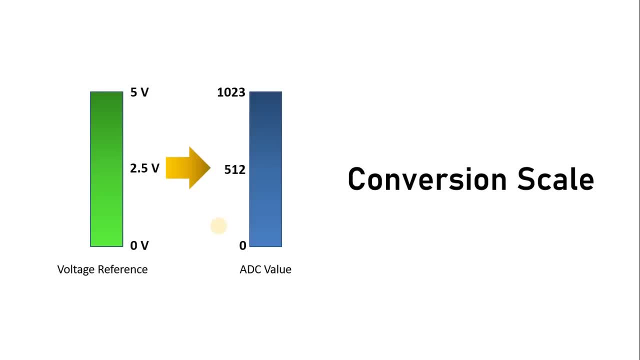 conversion scale. what i mean by that is, since the resolution of adc on the arduino board is 10 bits, it can hold up to one thousand and twenty three values. okay, so if we compare that if the arduino reads zero volts, so the corresponding adc value will be zero, and if it reads five volts, the corresponding adc value will. 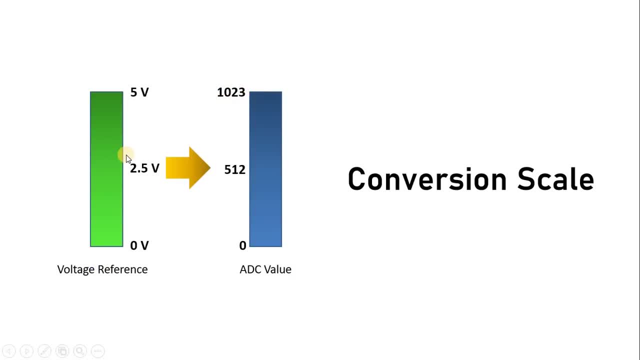 be 1023 and we can use unitary method to find out values in between. for example, you can tell me what will 3.3 volts mean? i hope i don't have to explain you the unitary method. right, this is the scale. if zero volt means zero and five volt means one zero, two, three, so one. 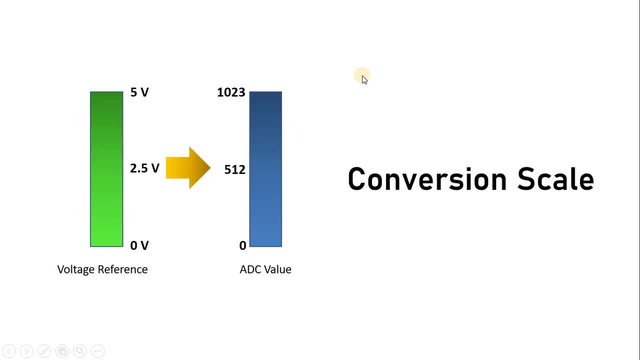 volt will mean one zero, two, three divided by 5.. so if you know the value of 1 volt, you can find out value of any voltage. so now many of you must be wondering from where this value of 1, 0, 2, 3 came. 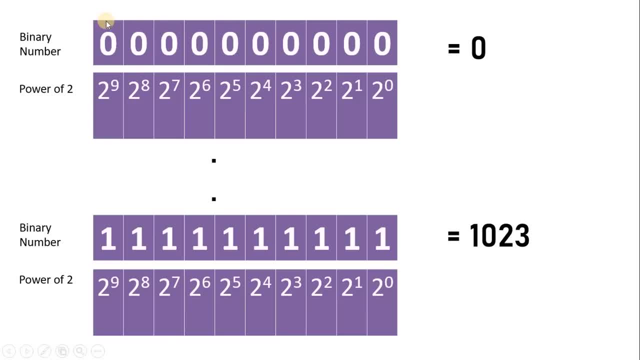 from, so i'll quickly explain it to you. we have a cupboard here which contains 10 boxes, and each box can contain a value of either 0 or either 1.. okay, so this is the cupboard and these are the boxes, individual boxes. to find the value of the cupboard, we take the value of each box. 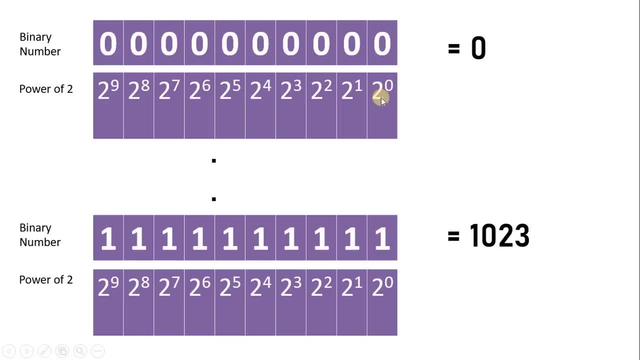 and we multiply it with the multiplier. the multiplier is this: two to the without command 2u, the power 0 is 1.. 2 to the power 1 is 2.. 2 to the power 2 is 4.. And similarly, 2 to the power 9 is. 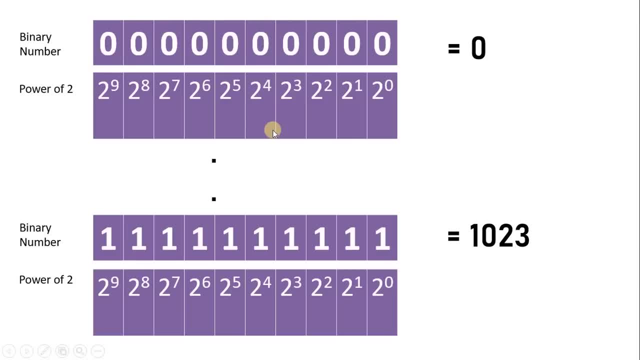 512.. So when we have values of all the boxes, we take sum of all those values and we get the value of that entire cupboard. So the maximum value which can be held by a cupboard in which all the boxes contain a value of 1 will be 1023.. How This box will evaluate: to 1.. Why? Because 2 to the power. 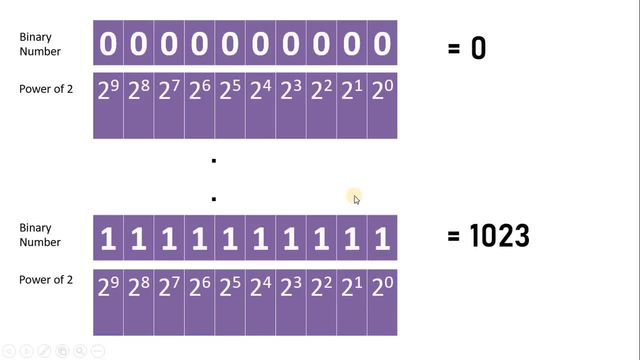 0 is 1 and 1 multiplied by 1 is 1.. Okay, so now 2 to the power. 1 is 2 and we multiply 1 by this So we get 2.. So we will be summing all the values from here to here, like 512,, 256,, 128,, 64,, 32,, 16,. 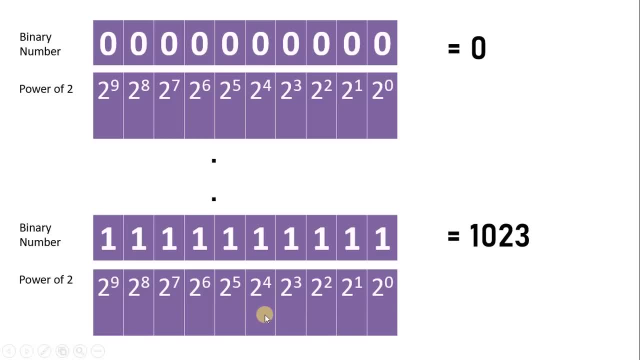 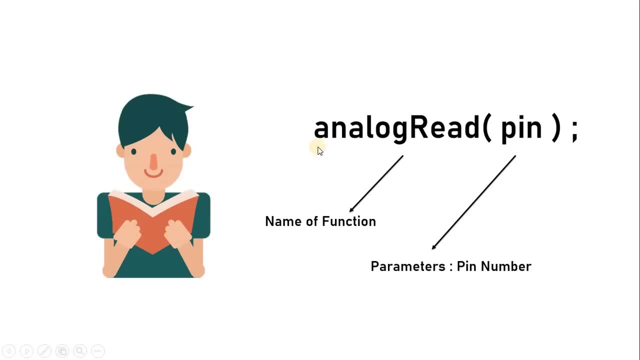 8,, 4,, 2 and 1.. When you sum all these values, you will get 1023.. You can try it on your calculator right now. So now let's take a look at analog read function. This function is simply used by: 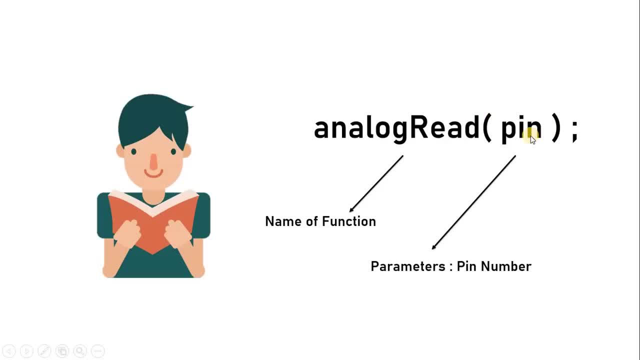 calling analog read With the parameter of pin number, where pin number is A0 to A5. So whenever you call this analog read function, it will return you the value it read on that pin. So let's see how we use that. 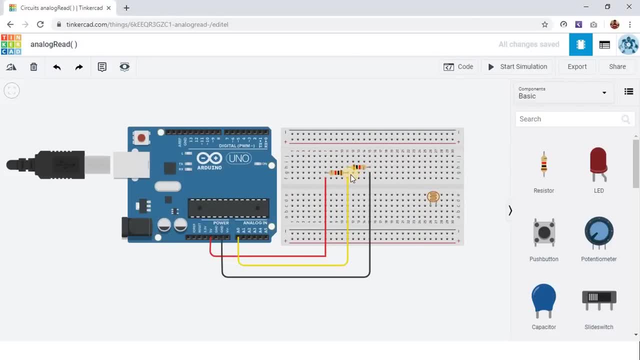 So now I have used two 1 kilo ohm resistances in series. Can you see that? So now I have connected it to 5 volts. This point is connected to 5 volts and this point is connected to ground, So you can. 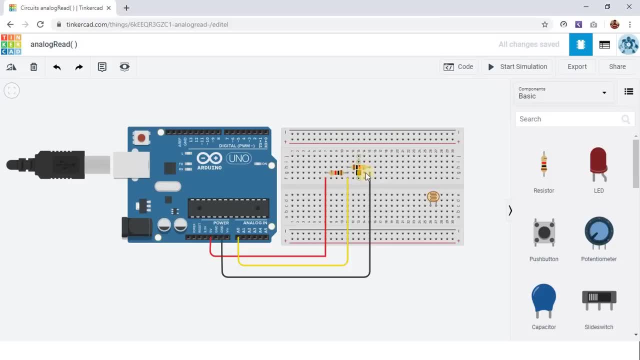 imagine a series circuit. So now I want to read voltage across this resistance. Since both the resistances are equal, the 5 volt will sum the value of 1 to the power 0.. So now I have used 2, 1 kilo ohm resistances in series. So now I. have used 2, 1 kilo ohm resistances in series. So now I have used 2, 1 kilo ohm resistances in series. So I have used 2, 1 kilo ohm resistances in series. So now I have used 2, 1 kilo ohm resistances in series. So 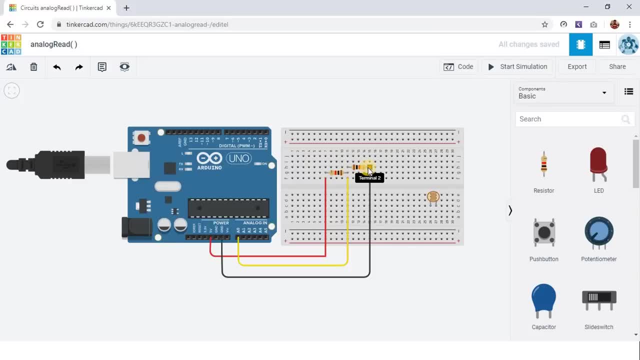 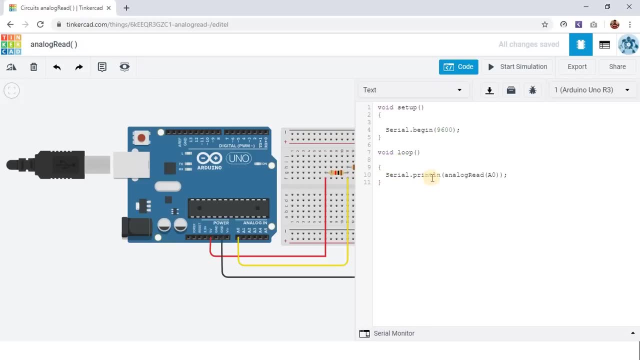 split equally on both the resistances, So we should be getting 2.5 volts. Let us see that. So in the code we have written serial dot- begin to start communication with the computer. And then we have written serial dot: println bracket analog read A0.. That means I want to read the voltage which is 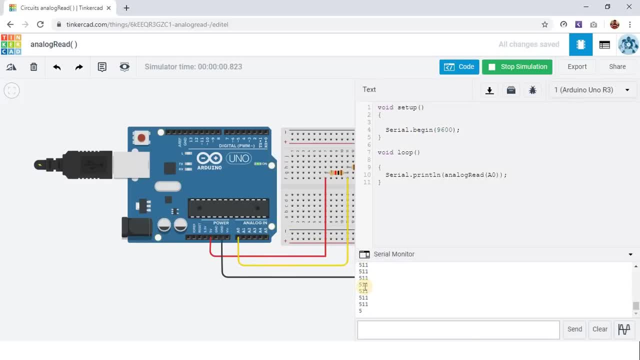 given at A0.. So let's try this code. So we are getting 511, which is nearly 2.5 volts. We saw in that scale right. So let's change the resistance and see what value do we get. Now let's make this: 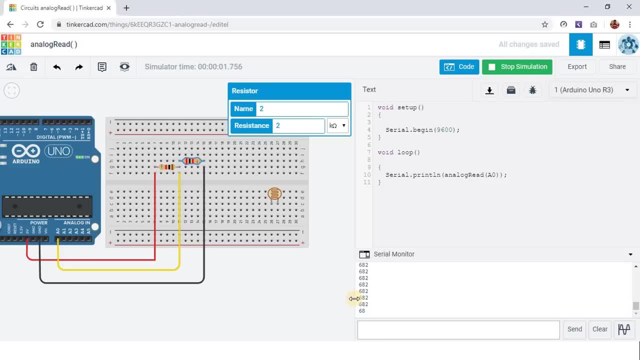 value as 2 kilo ohms. So we got a change in value. More the value of resistance, more the voltage will drop across it. We can see the value of voltage across this resistance is increasing. If we make it too high, it will increase. It will also change if we change the value of this resistance. Let's 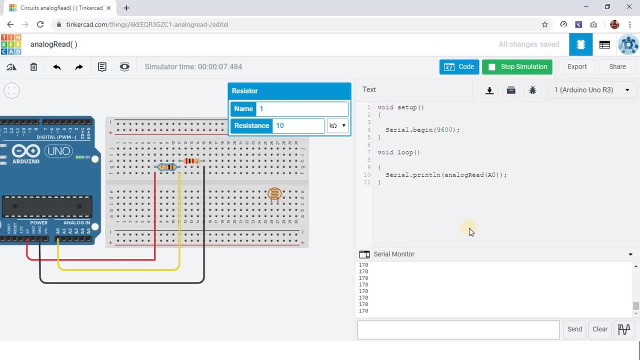 say, we make it 10. So now the voltage across this resistance will drop and hence we get a lower value. Now let's see this with a light dependent resistor. This is a special kind of resistance which changes its resistance when light falls on it. In most of the light dependent resistance, 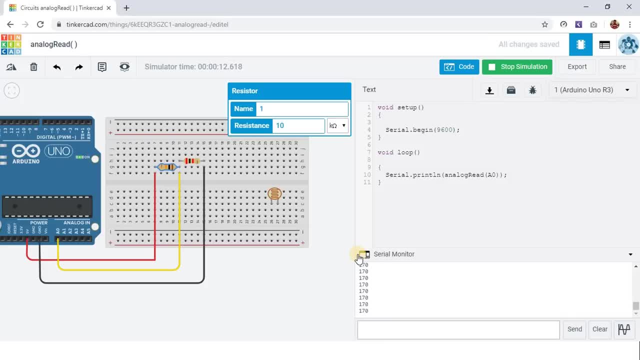 the resistance will decrease, So it may increase, even if light on it increases. okay, Let's try this. Let's replace this resistance with a light dependent resistor. okay, We connect this in series. I'll kick it here. alright, We take this wire. 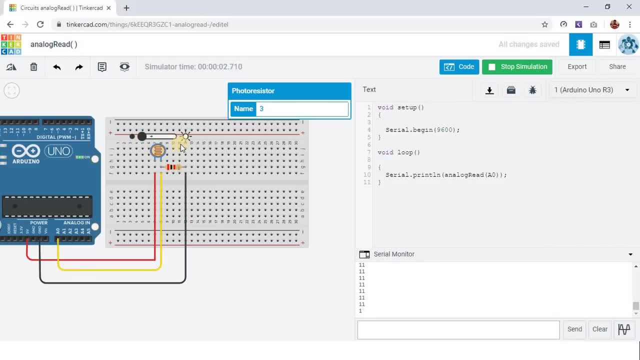 So now you see, this bar will represent the amount of light falling on it. right, I can control it like this: here it is total darkness and here it is very bright. okay, so when it is dark, the resistance of this component is very high. okay, so the voltage which drops across this resistance will be very 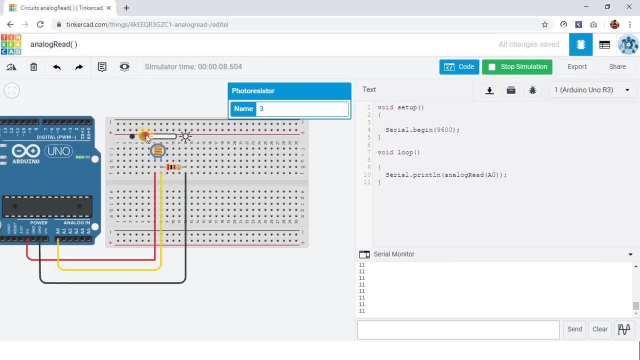 low. you can see the value is very low right. as soon as i increase the light on it, you will see the value in the serial monitor is increasing. can you see that? because the resistance of this component is getting lower and and more voltage is dropping across the resistance. okay, so this. 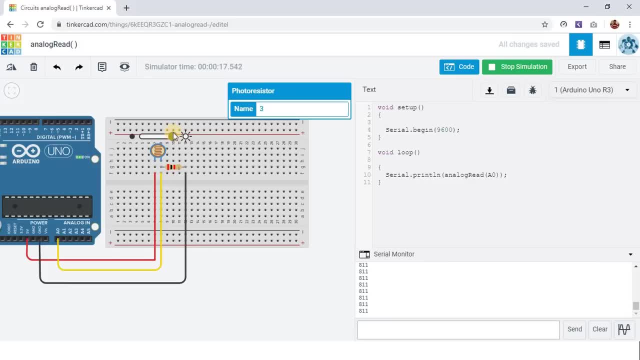 is the principle of analog read. now you can see how we can read the value of analog sensors using analog read. all right, so in the next video we will look at the another function, which is known as analog write. so see you in the next video. in this video we'll take a look at analog write function. 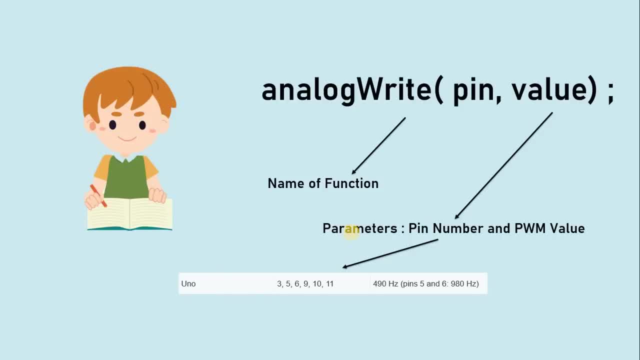 which is another important built-in function of arduino. all right, so to begin with analog right, i would firstly like to tell you that it has no relation with the analog pins or analog read function. it is absolutely a different thing. what exactly it is we will see shortly. so. to use analog write function, we write analog write bracket pin. 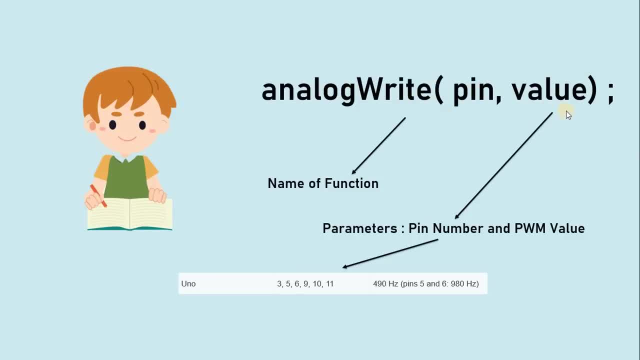 number on which we want to use analog write and then we specify a value which ranges from 0 to 255, we close the bracket and use a semicolon right. the important thing which we need to note is the pin numbers which we can use. here are specific, which are pin number 3, 5, 6, 9, 10 and 11 only. okay. 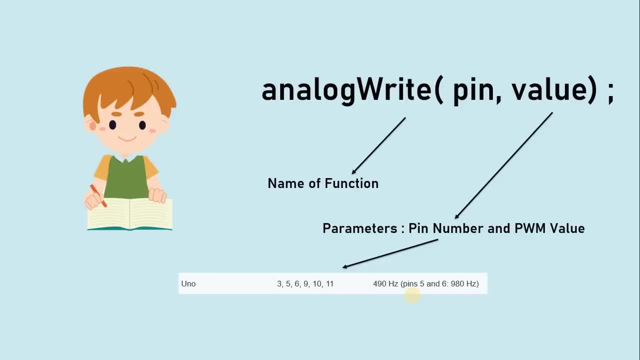 while all of these pins, except pin number 5 and 6, support a frequency of 490 hertz, and pin number 5 and 6 support a frequency of 980 hertz, we don't need to worry about this frequency right now. i'll explain as we progress. before we dig deeper into this, we need to understand a few terms like pwm. 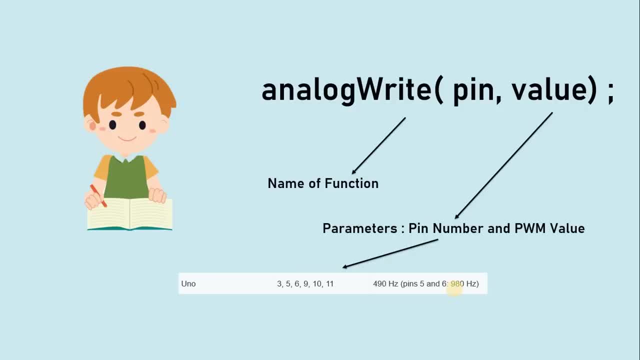 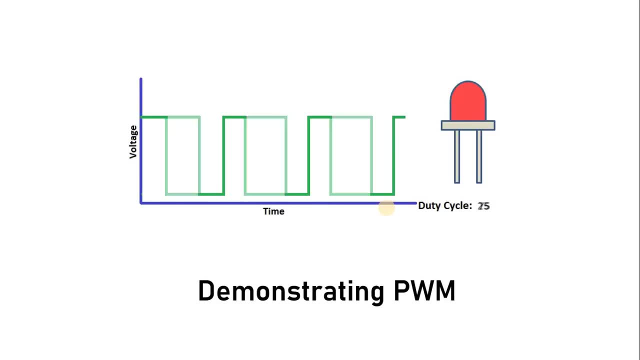 pulse, width and frequency. and even before that, we need to know what exactly this analog write function does. the analog write function generates a square wave of a specified duty cycle, and we need to know what exactly this analog write function does. the analog write function generates a square wave of a specified duty cycle on that specified pin. the major purpose of using. 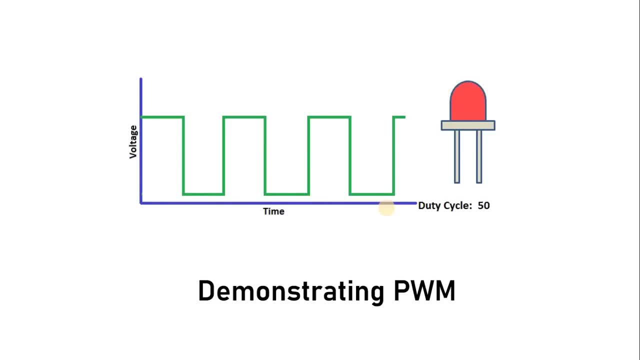 on that specified pin. the major purpose of using analog writers to control the brightness of led. analog writers to control the brightness of led or to control the speed of a motor right. the first or to control the speed of a motor right. the first thing which we need to see now is a square wave. 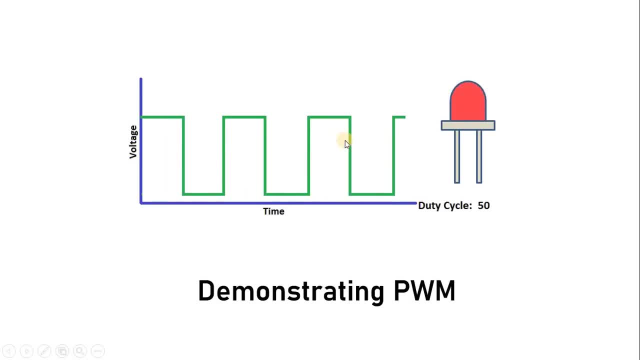 thing which we need to see now is a square wave. what a square wave is on the screen? you can see what a square wave is on the screen. you can see a square wave is coming. this is a square wave. okay, a square wave is coming. this is a square wave. okay, although this is a varying square wave now. 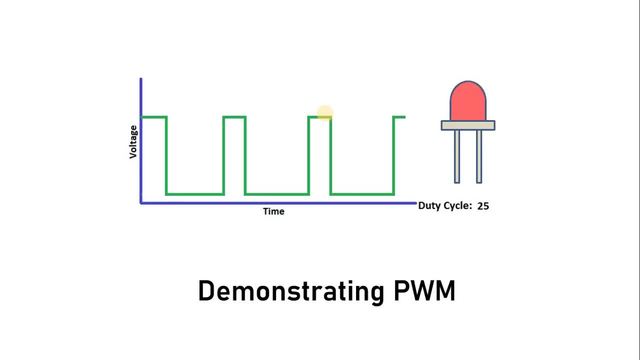 although this is a varying square wave. now, a square wave is nothing but a signal which has only two. a square wave is nothing but a signal which has only two discrete values: either on or off. as you discrete values, either on or off. as you can see, here it is on and here it is off, and the time for which. 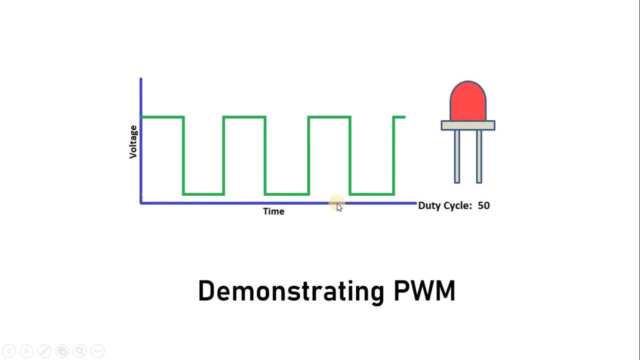 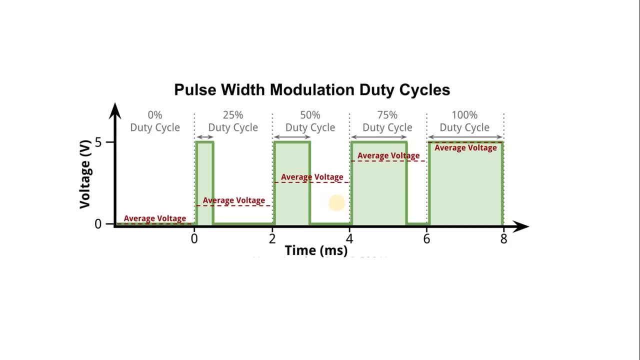 it is on and off is varying. you can see here, right, i can understand. it must be little difficult to comprehend, but please stick with me, okay? so the next term is pulse width. the amount of time for which a signal is on is known as pulse width. for example, in this way, this is the pulse width. 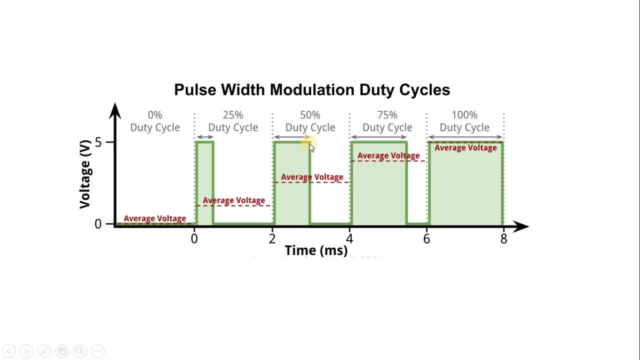 denoted by this arrow in this portion. this is the pulse width denoted by this arrow in this portion. this is the pulse width noted by this arrow. all right, the next term is duty cycle. duty cycle is the fraction of period for which the signal was on right. so we have five sections here. 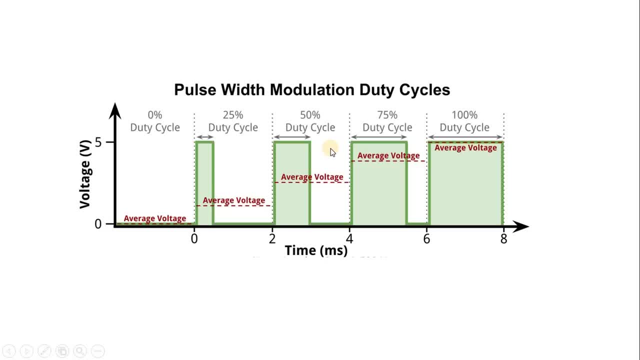 with zero percent duty cycle, 25 percent duty cycle, 50 percent duty cycle, 75 percent duty cycle and 100 percent duty cycle. okay, so in this section the voltage for entire time was zero. okay, so that means the duty cycle is zero percent. in this section we have about one fourth of the time. 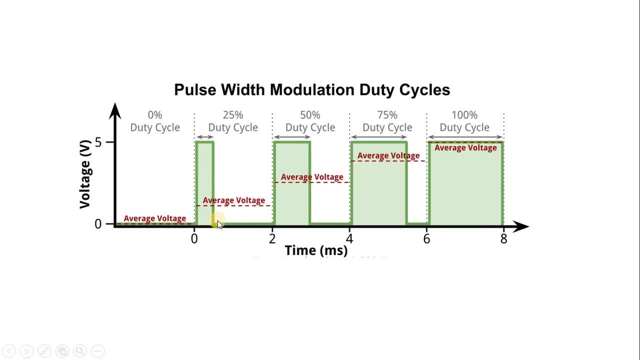 as on. you can see that right. for the one fourth time it is on and three fourth time it is off. so that means the duty cycle is 25 percent. in this section we have about half of the time as on time and half of the time as off time. so here the duty cycle is 50 percent. similarly, here the on time is: 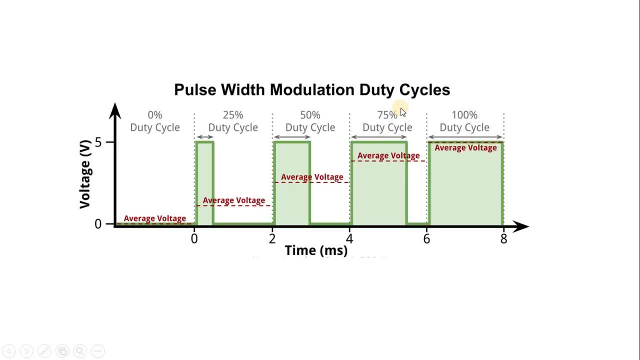 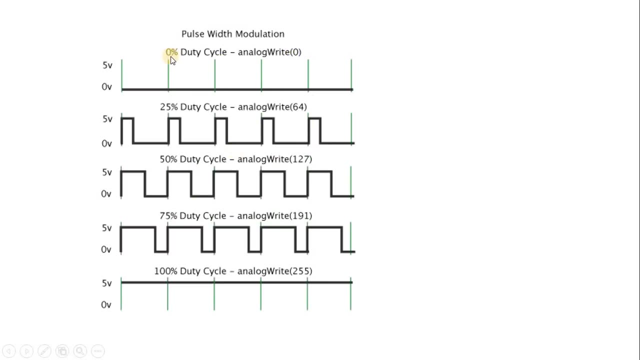 three, fourth. hence the duty cycle is 75 percent. and here, for the entire duration of time, the voltage was on, hence the duty cycle was 100 percent. okay, now, if we look in terms of arduino, when we call right with a value of 0, it will give us 0 percent duty cycle. that means the signal will be off for 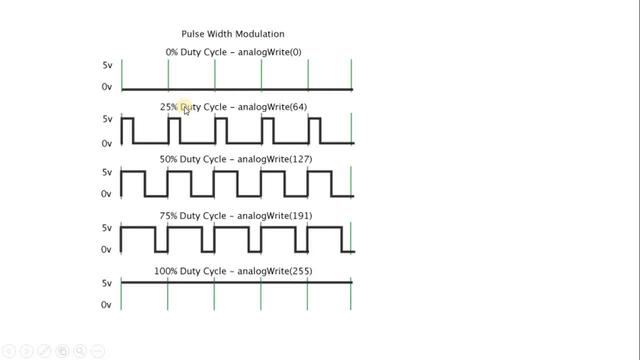 the whole time. if you write analog, write 64, then it will give us a duty cycle of 25 percent. if you write 191, it will give a value of 75 percent and 255 will give us a duty cycle of 100 percent. okay, so now to summarize: pulse width modulation, or pwm, is a technique for getting analog results with. 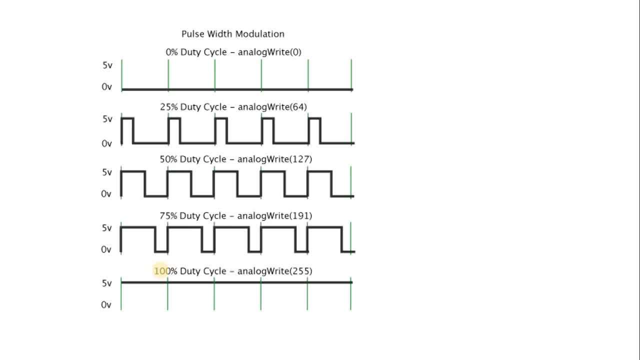 digital means. digital control is used to create a square wave, which is a signal switched between on and off. all right, and this on and off cycle takes place really fast. and this on off pattern can simulate voltages in between full on and full off by changing the portion of the time. 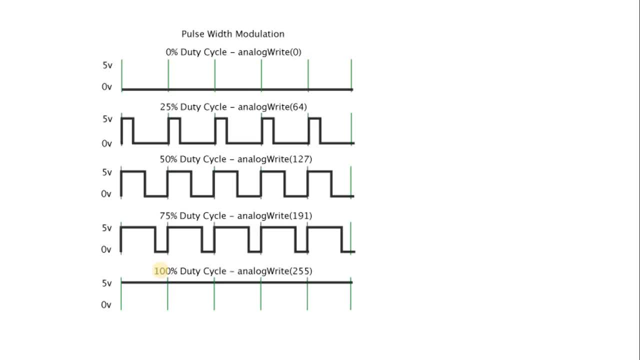 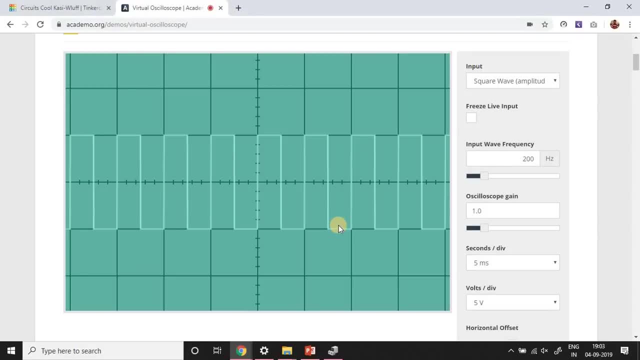 the signal spends on versus the time that signal spends off. all right, so the next thing which we need to look at is the pwm frequency. okay, so let's see, this is a wave which has a duty cycle of 50. that means half of the time the signal is on and half of the time signal is. 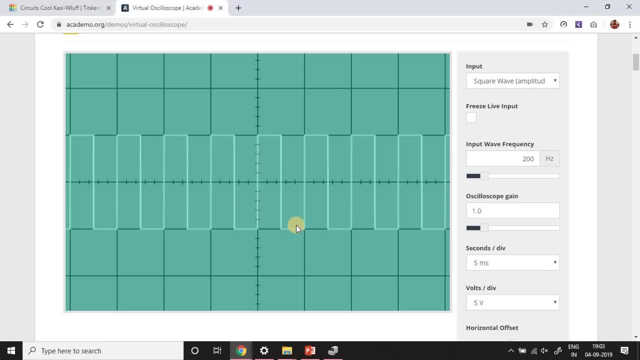 off. changing the frequency of the signal will not change the duty cycle of the signal. okay, so let's say we have a signal of 50 duty cycle here and if we make the frequency to 400, so the waves will become closer. that means now it will turn on two times and turn off. 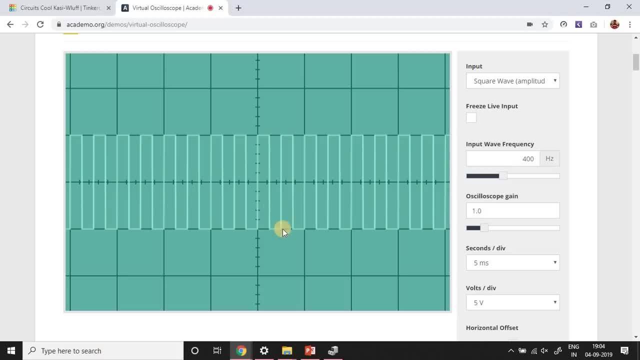 two times. right, you can see here on and off. earlier it was on one time and off one time. okay, but you see the duty cycle is still 50. you're getting my point. so you see, the duty cycle of the signal is not changed because it was still on for the half of the time and off for half of the time. 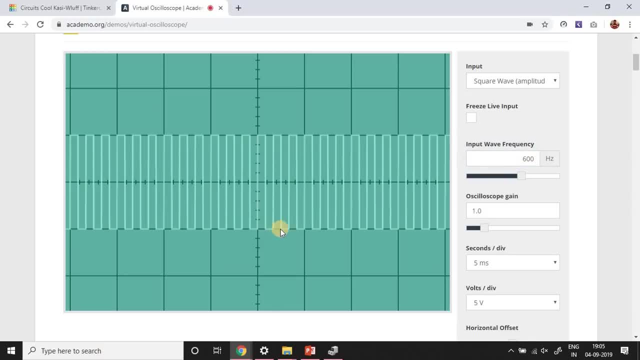 even if i make it 600, it is still on for the half of the time and off for half of the time. okay, so i hope it was clear to you and if in case it was not clear to you, we'll take an example and blink the led and change the brightness of the led. all right, and we will also monitor it, along with the 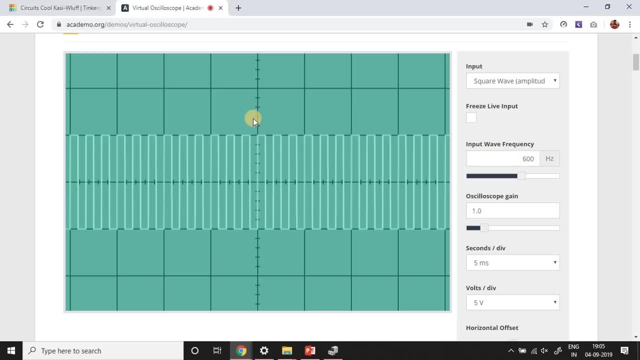 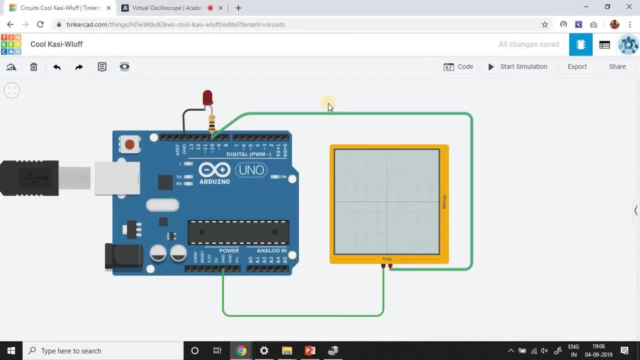 digital oscilloscope. an oscilloscope is nothing, but it is a device which is used to analyze the signals. okay, so let's see that. so here, what we have done is we have changed the frequency of the signal, we have taken an led on pin number 10 and, correspondingly, we have connected these wires. 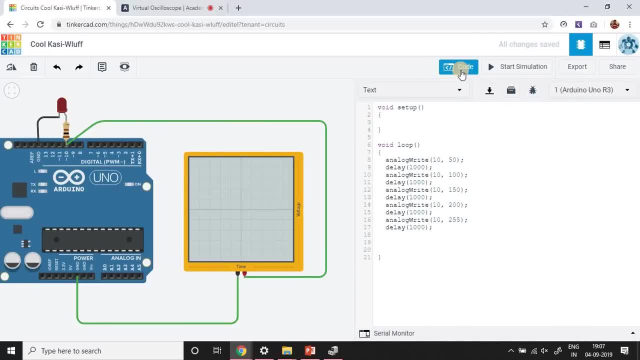 to an oscilloscope to see the signal. so let us see the code first. so you must have noticed that we have not written anything in void setup and we don't have to use pin mode whenever we want to use analog write function. okay, so now in void loop i have written analog write pin, number 10 and a value. 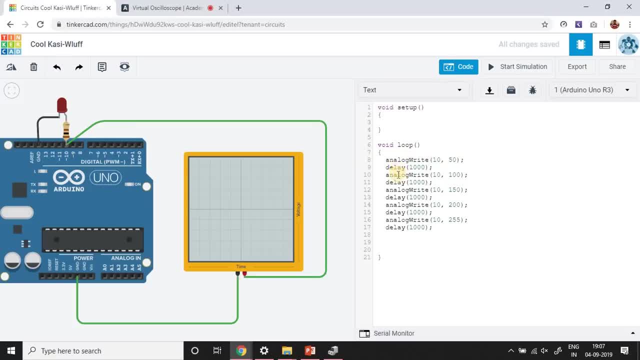 of 50, okay, and then i've given a delay of one second. then analog write 10 with the value of 100, so we get a duty cycle of 100, okay. so now let's see how it looks like, pay attention to the wave which is coming on the oscilloscope and also note the brightness of this led. i'm starting the. 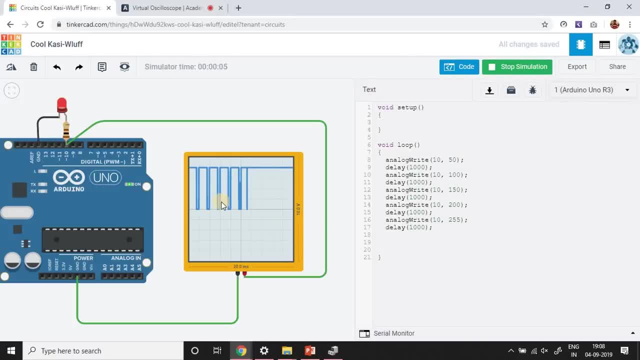 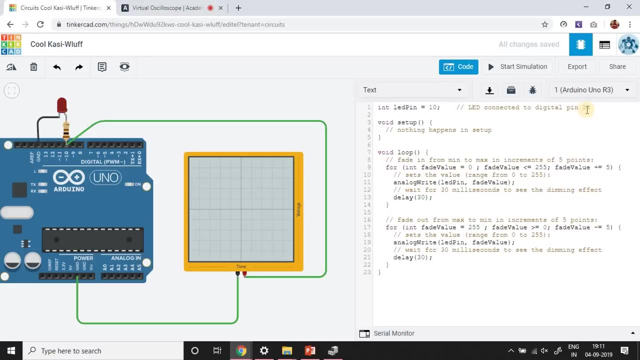 simulation. let's see. can you see that the brightness of led is increasing gradually as the code progresses and it gets back to 50 and then it again increases. also note the pulses which are coming in the oscilloscope. so now we will see an example in which we are changing the brightness. 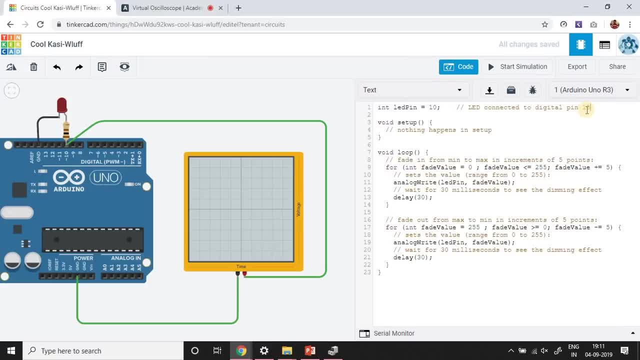 of led in steps of 5.. we will also look at the pwm wave simultaneously. let's look at the code first. we have defined an led pin which is connected on pin number 10 in white setup. we don't have to do anything in void loop. we have written 4, which is a for loop, and we have defined 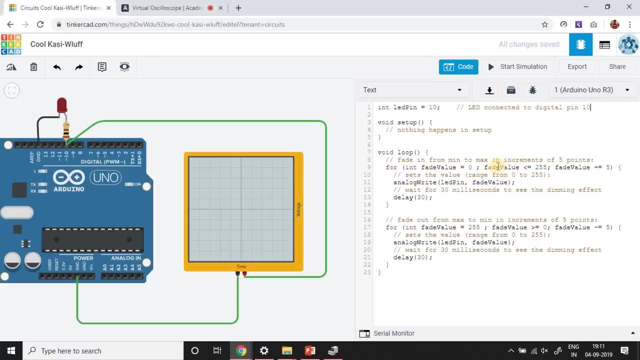 a fade value. int. fade value is equal to 0 and you have to do this till the fade value is less than or equal to 255. okay, and then we are incrementing the value of fade value by 5.. this is in another compound operator. you can say it is similar to writing fade value. this is equal to: 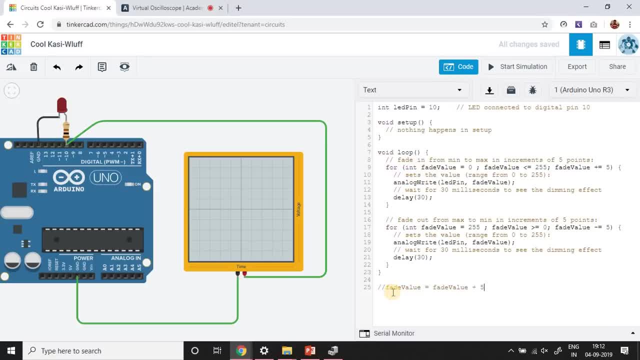 fade value plus 5.. all right, so now we have written analog write and we have written led pin here, which is pin number 10, with the fade value. okay, so how it will go: it will write 0 here, then, after the delay of 30 milliseconds, it will write 5 here, then, after a delay of 30 milliseconds, it. 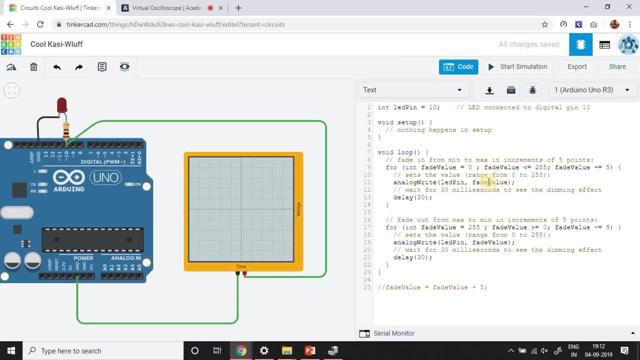 will write 10 here, 10 15, 10, 20 and 25 and so on till 255.. once this value becomes 260, you know, in the last iteration the value will become 260. so this condition will remain the same, will become false and it will exit this for loop and come inside this for loop. in this for loop we 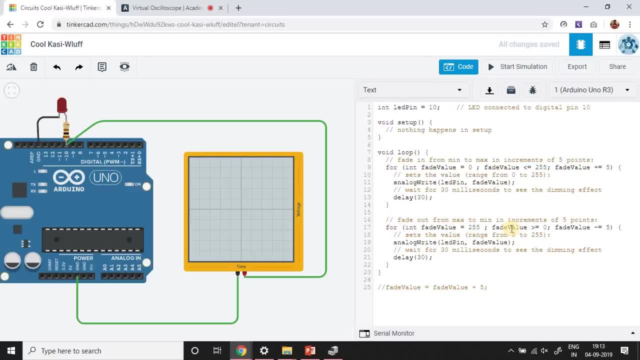 have used fade value starting from 255 and we have written a condition: fade value greater than equal to 0. that means you have to do this till the value is greater than or equal to 0. okay, then we have to use fade value minus equal to 5, and this is similar to writing. yes, you guessed it. 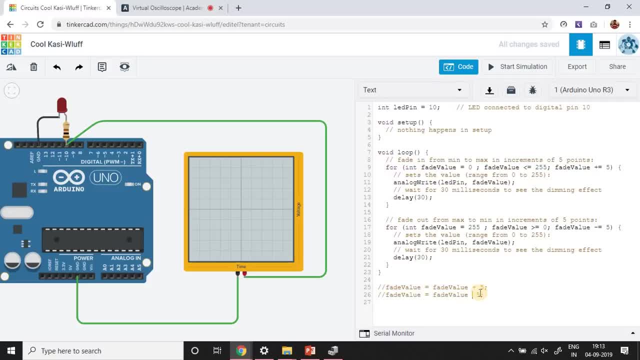 right, it is similar to writing: okay. so now it will start at two values. after a delay of 30 milliseconds it will write 250 and 245, then 240 and 235, and so on till zero. in the last iteration, when the value is zero, the value will become minus 5 and the condition will: 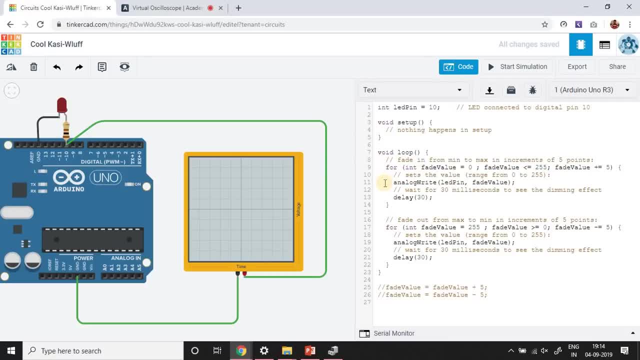 become false, so this loop will exit and it will come back into this for loop and this will repeat endlessly till we turn off the Arduino. let's start the simulation, note the brightness of the led and note the signal which is coming in the oscilloscope. let's see. 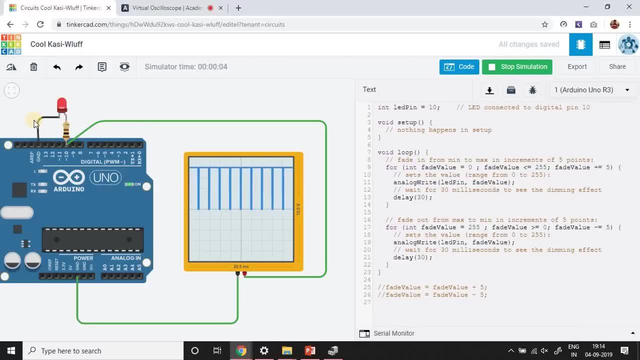 okay, it's interesting, right. the brightness of led is increasing from 0 to 255 and the pulse width is changing. when it is 0 you can see it is entirely off, and when the duty cycle becomes 100 it becomes entirely on. the pulse width is changing here, so 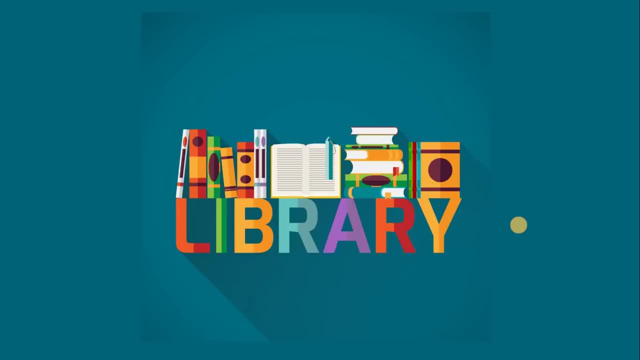 i hope you have understood this really well. the last topic which we need to learn about before starting our experiments is the Arduino libraries. so libraries are a collection of code that makes it easier for you to learn about the Arduino libraries. so the Arduino libraries are a collection of code that makes it easier for you. 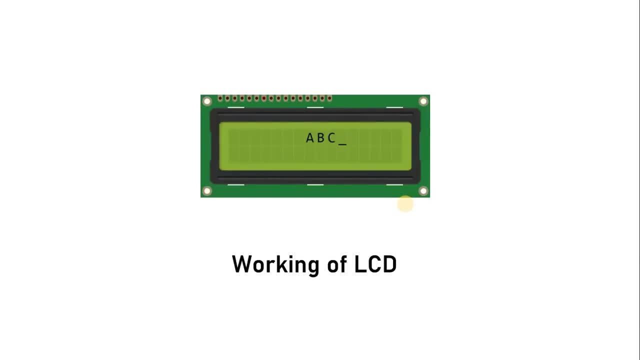 to connect to a sensor display or a module. for example, there is a built-in library to control a liquid crystal display. that library makes it easier for us to talk to that display. right, for example? you can see that library will control what character will come at what position, apart from 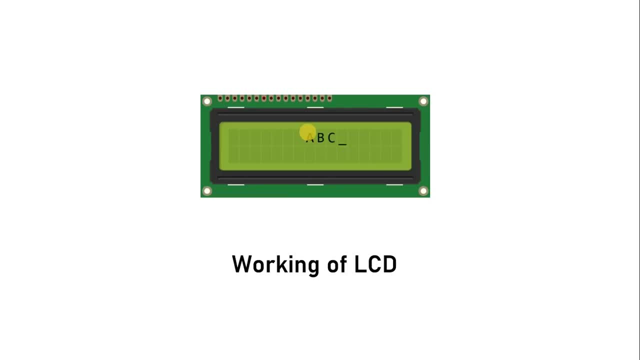 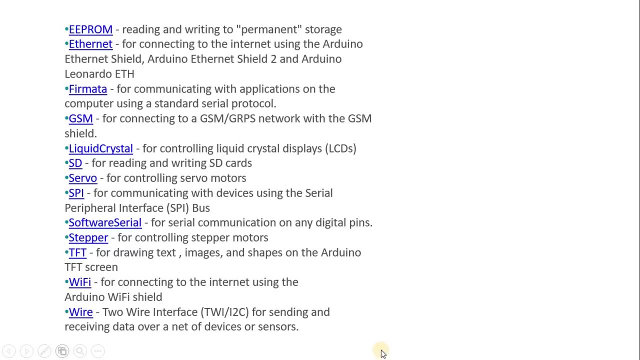 this library. there are many more libraries which are available for download on internet, and there are also built-in libraries. for example, the built-in libraries are these libraries which are already present in Arduino IDE. i'll just name them and show you how to use them. so let's start the simulation. 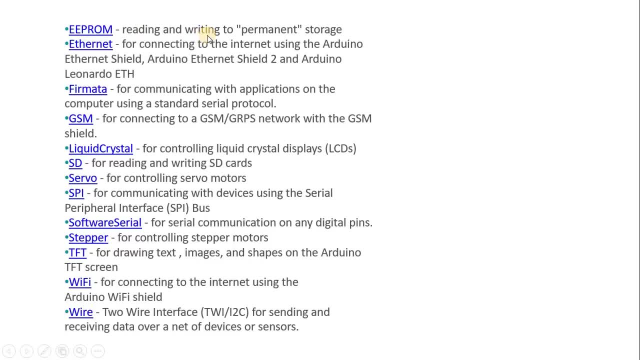 of you like. EEPROM is used to read and write elements from the permanent storage. the GSM library is used to connect GSM or GPRS network with the GSM shield. the liquid crystal library which you just saw controls the liquid crystal display which is used for reading and writing. 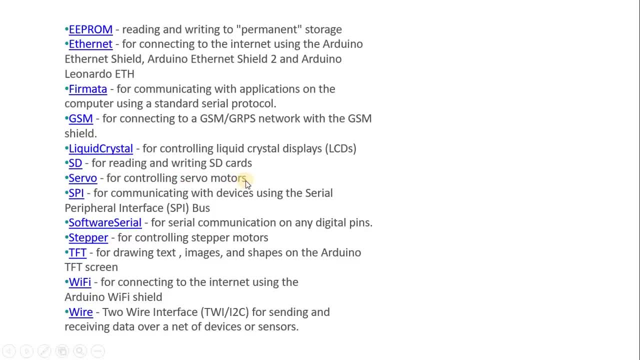 data on SD cards. a servo library will be used to control servo motors. similarly, there are many more libraries which are already there on Arduino. the code which is written inside those libraries can be written by someone else, or you can write the code on your own as well. once we have the 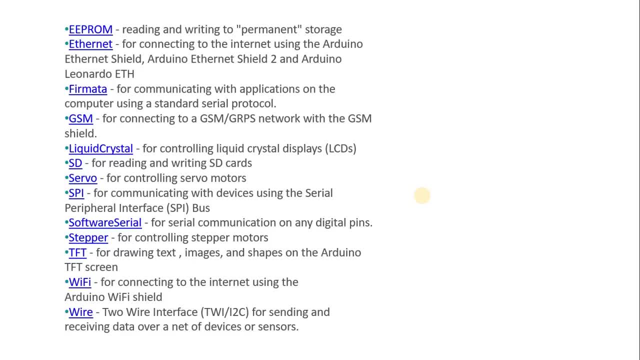 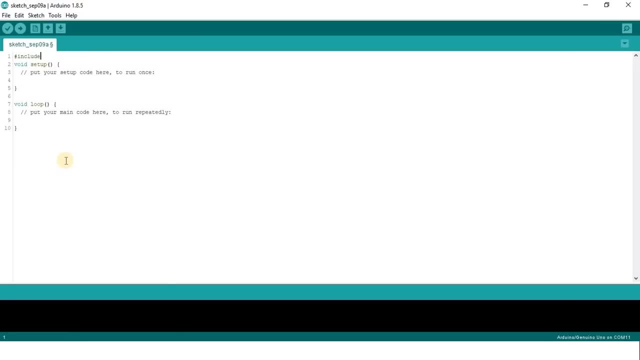 in our Arduino IDE. it's very simple to use that library. i'll just show you how. so this is our code. let's say we have to use liquid crystal library, so we will write hash, include liquid crystal dot h. okay, whenever we use this library, we'll be able to use the functions which are: 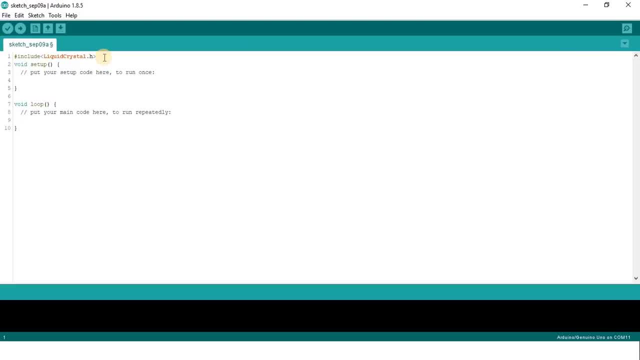 written inside the liquid crystal library- okay. similarly, if we have to include another library for sd cards, we will write sd dot h. okay, this will include the sd library in our code. we'll be able to use all the functions which are written in sd library. i would 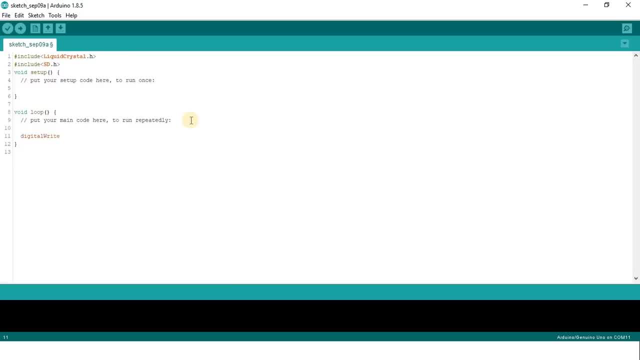 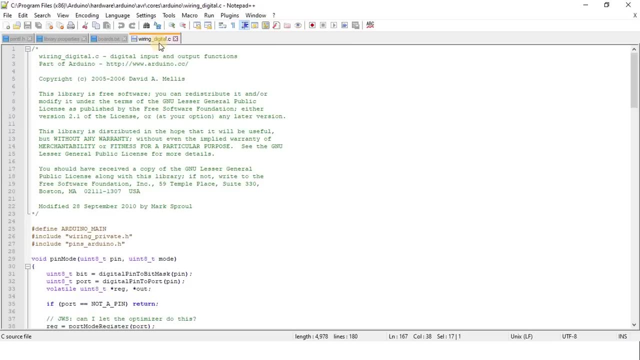 also like to tell you that the functions which we were using, like digital write, were also declared in some library. i will just show you how it was written. so there's a built-in code which is written inside wiring underscore digital dot c, which is located at this location: see program files Arduino. 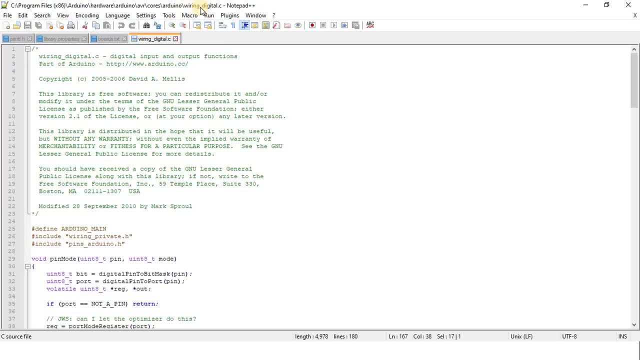 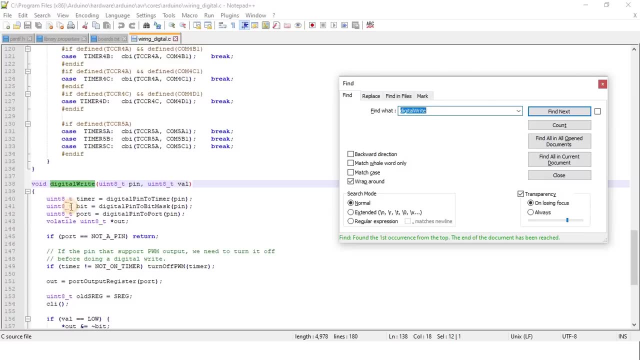 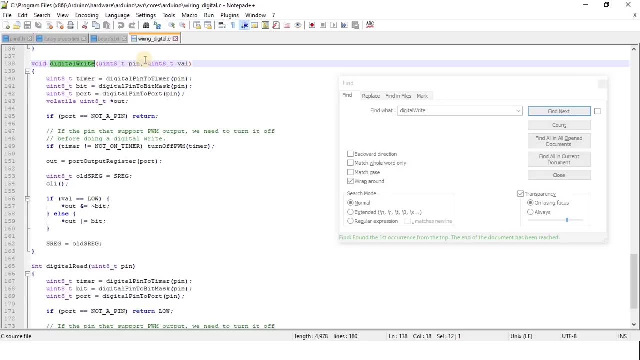 hardware: Arduino, AVR course, Arduino and then finally the file. now if we see the declaration of a digital write function is declared in that library. okay, you just see that void. digital write, pin number and value. okay, where pin is the pin number and value is high or low. it accepts two. 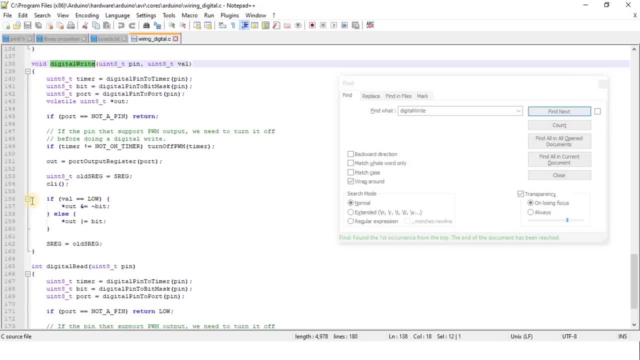 arguments. right, we saw that while calling this function, so this is how the digital write is called. we'll not get into details of this function as it may be very complicated for you to understand, okay, similarly, digital read has been declared here. this is a declaration of digital read. similarly, 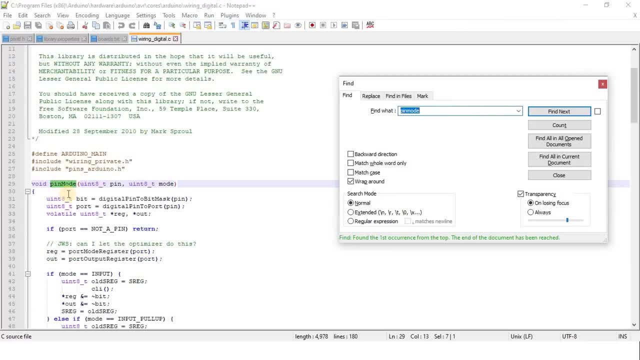 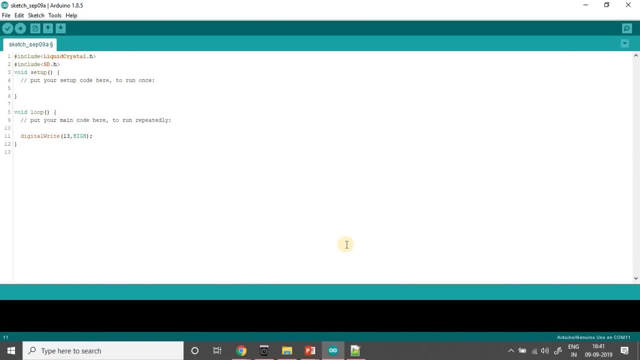 pin mode is also declared right. so i hope you were clear with libraries and i hope you understand how using libraries saves a lot of our time. okay, so in the next video we will see how to add additional libraries in our Arduino IDE. so see you in the next video. so now let's see. 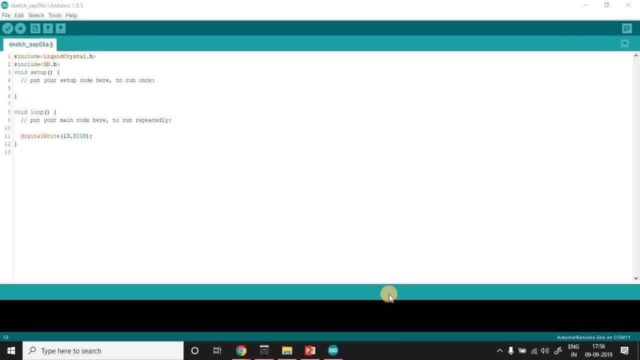 how do we install external libraries in our Arduino IDE? there are basically two methods. one is through the library manager and one is through adding external files. okay, let's look at the library manager first. we will go to sketch: include libraries, then manage libraries. it will open the library manager. this is 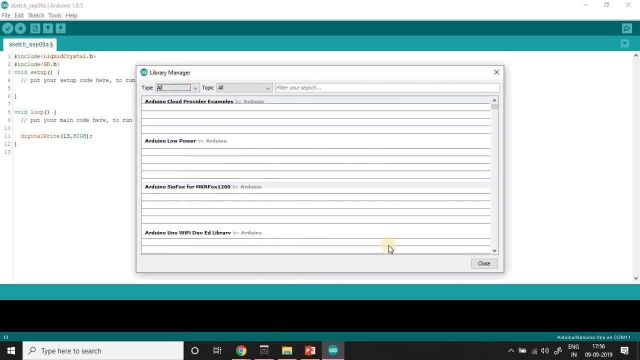 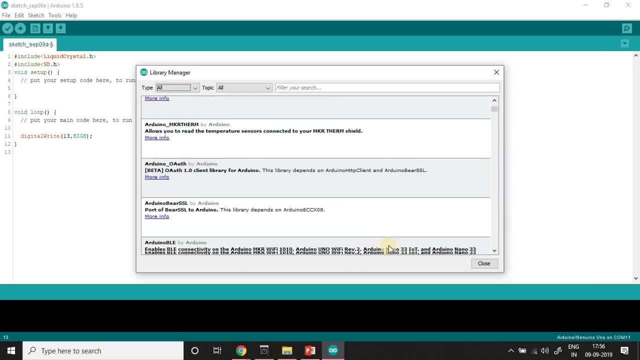 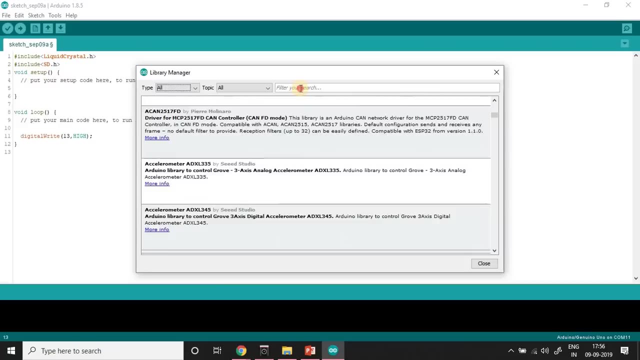 the library manager. it will update all the libraries which are already there in their database and it will show us the list of available libraries for us. you can see there are a lot of libraries already there, right? these are all the libraries which are present in their database right now. 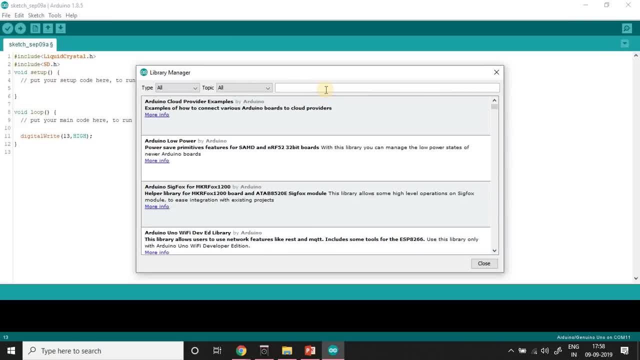 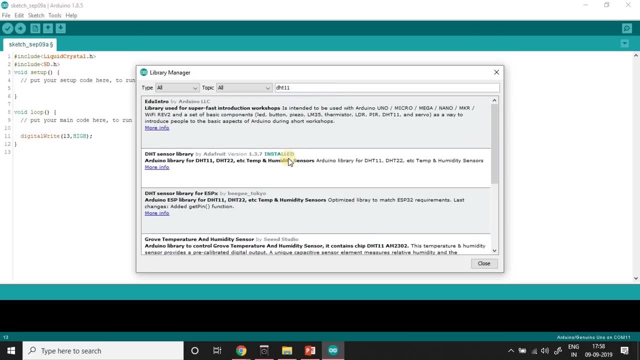 so let's say we need a library for DHT 11, which is a sensor which captures temperature and humidity of our environment. so we will write DHT 11 here and it will search all the libraries which are available for DHT 11 by different authors. so let's say this is a very reliable library by Adafruit, which 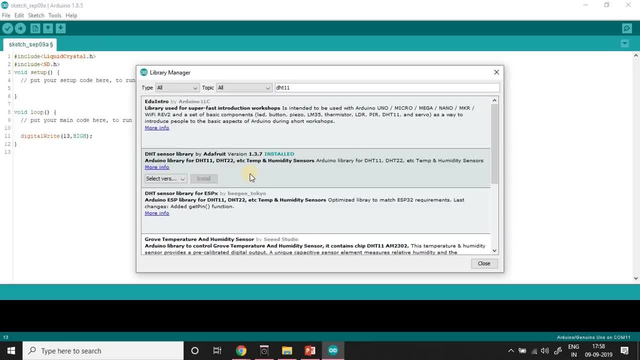 I have already installed. okay, so just in case you have not installed it already, install here. you can select the version here, which version you want to install. usually this is the latest one- and then you just click on install and it will install the library in your ID. okay, once it is installed, we can use it in a 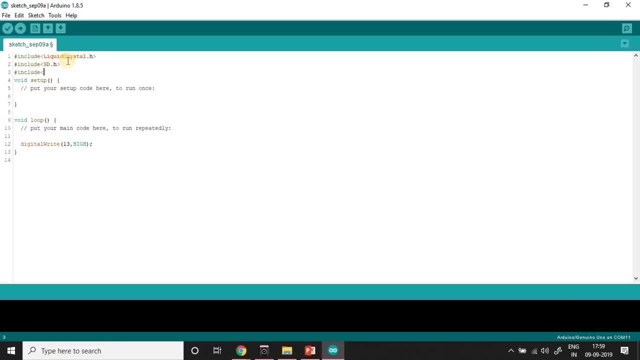 regular manner hash. include DHT dot H. okay, if this DHT library was not installed in my ID, it would not appear in this orange color. okay, let's take an arbitrary name: include hashish dot H, since there is no library named hashish, so this hashish is not coming in orange color, although this 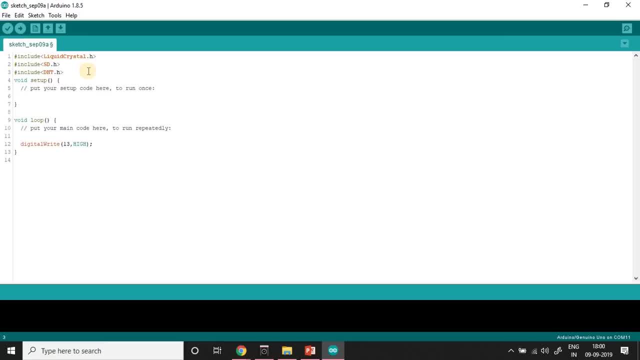 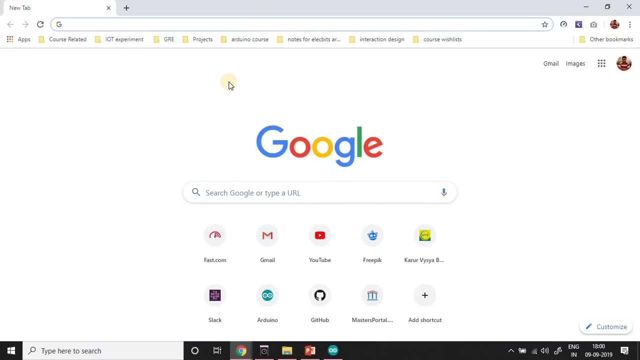 is not a very hard and fast rule. you might not get orange color in some libraries, but it is a really good indication that you're working in a right direction. okay, so now let us look at the other way, which is adding them manually. let's say again: we want a library for a DHT 11 sensor. we will. 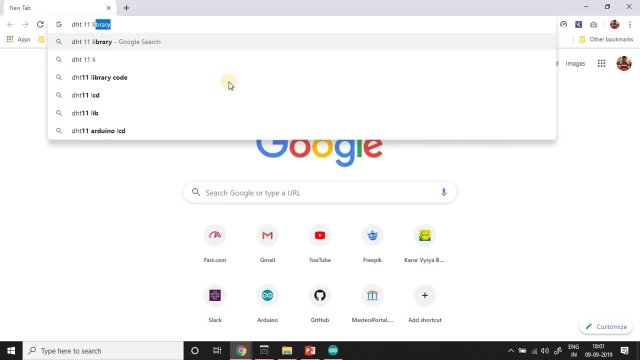 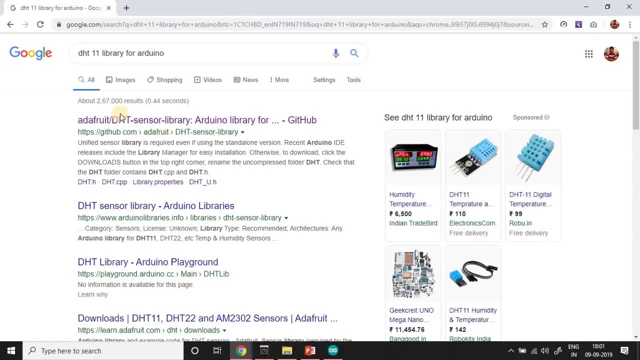 write DHT 11 library for Arduino. usually libraries are available on github. you may also find zip files on some of the websites, but github is usually preferred, as you would get the latest version of the library from there. so again, Adafruit has hosted their library on github, so let's click on that. 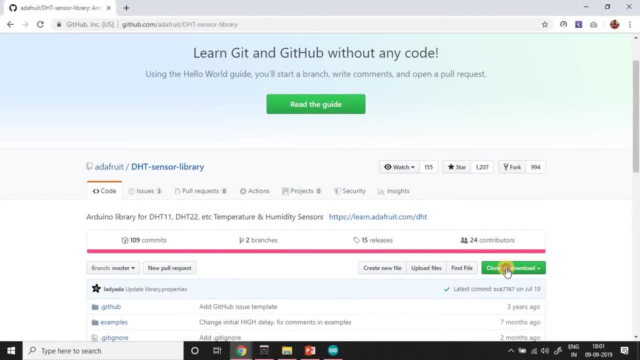 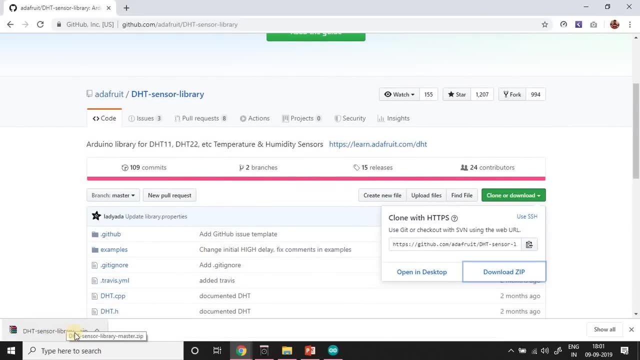 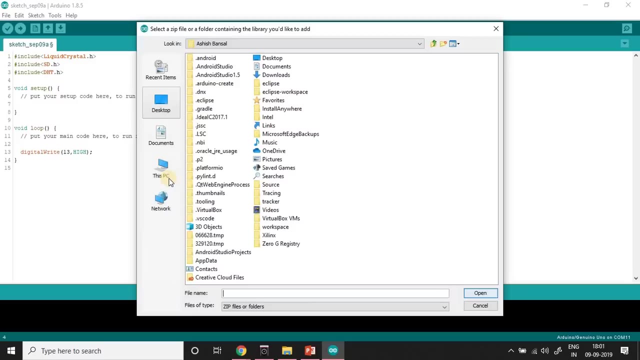 and then we'll go to clone or download. we'll click download zip and it will start downloading it. you have to see where you have downloaded it. you have to go to sketch, include library and add dot zip library. in my case, I downloaded it in my edge drive, so it is here. we'll click on this and just click. 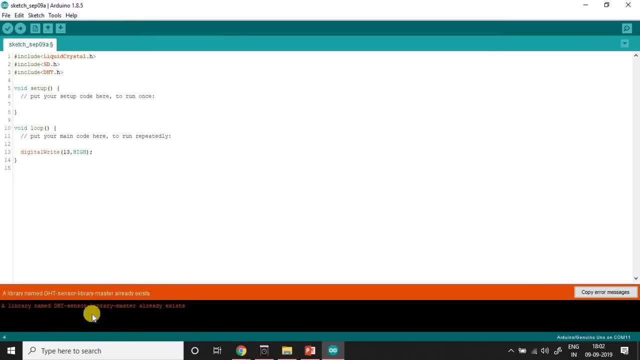 on open. in my case it was already installed, so it gave me a warning. a library named DHT sensor library master already exists. okay, but in your case it will say the library has been successfully installed. so these are the basic two ways in which we add libraries. 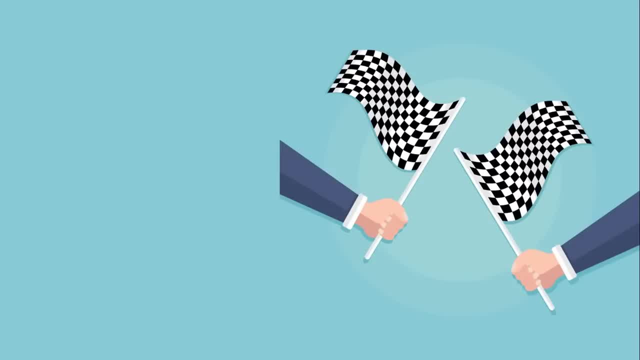 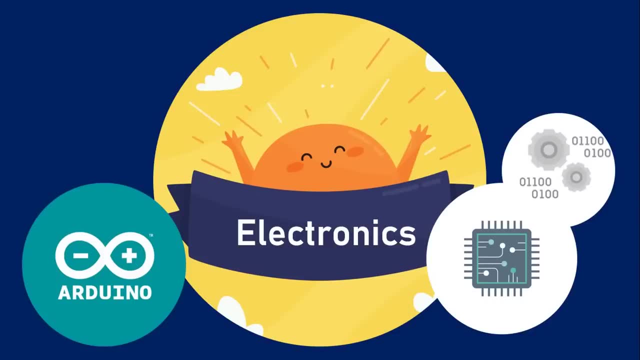 and this point is important because if you want to add a library to your system, at this point I can really say that you have reached a milestone and you are in a position to dig deeper, as you have so many tools under your belt now. we have covered the foundations of electronics. then we covered what is an Arduino board. 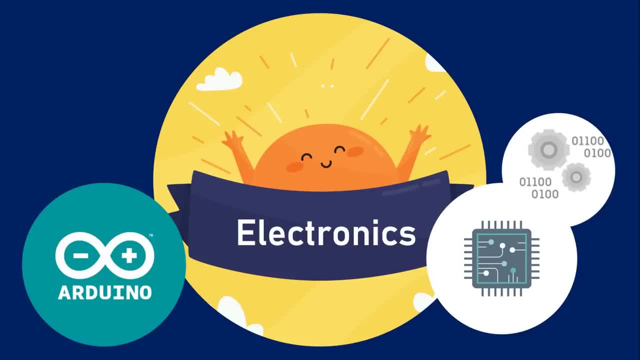 and then we discussed what is inside Arduino. we covered the difference between the microcontroller and microprocessor. then we saw the Arduino IDE, how it works and how we use it. we also saw an online simulator which can be used if someone doesn't have an Arduino right now. then we saw how to use a breadboard.